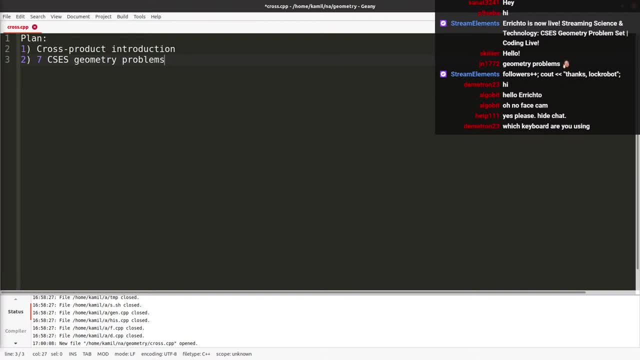 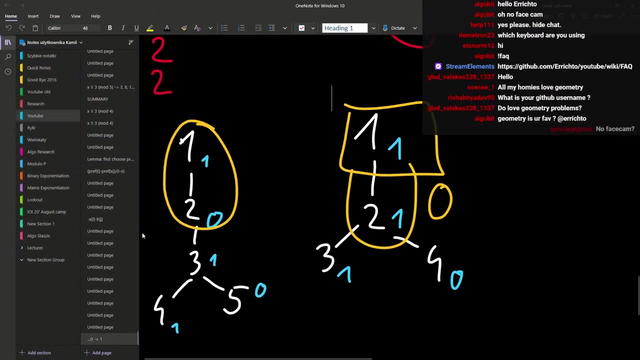 Which keyboard? Logitech Ultra X Premium, which is a cool name, but it's a very old keyboard. Hi there, Everybody loves geometry. I don't know about that. My username everywhere is just Richter, same as channel name: Geometry. it is indeed my strong point. Is it favorite? Depends on the problem. 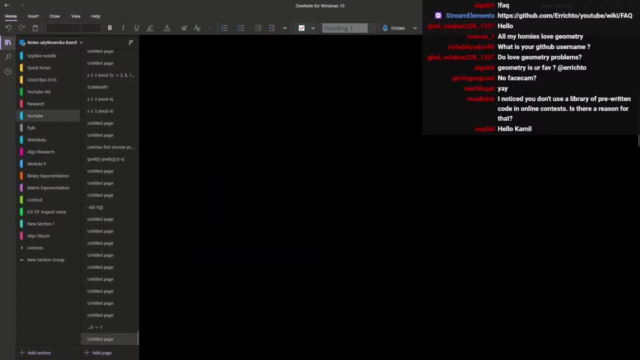 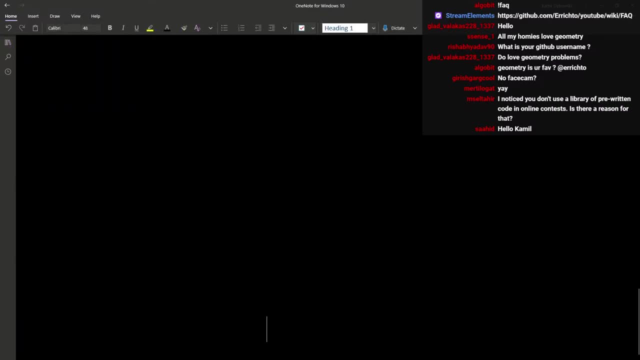 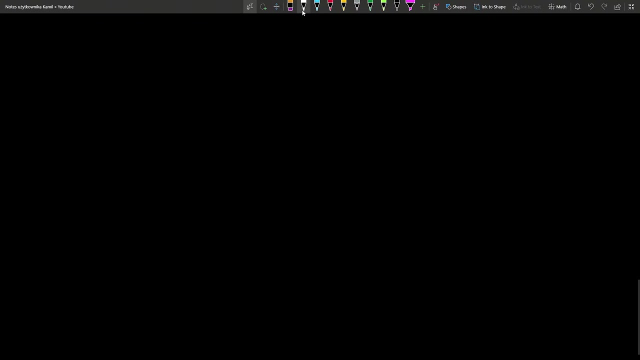 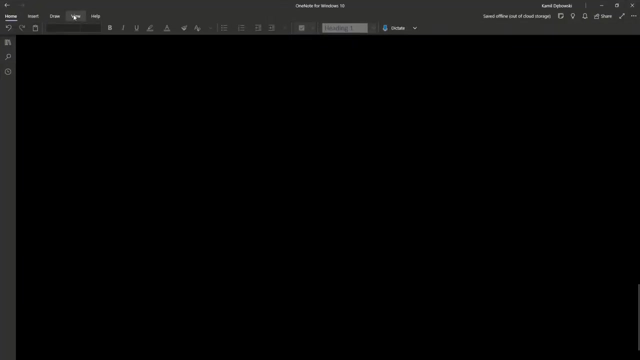 Let me prepare something to draw And then we can start. We'll start with, as I said, cross product recap and then we'll move to problems. I'm hiding the chat. Alright, Got one more thing, If it's possible, I believe to do this. 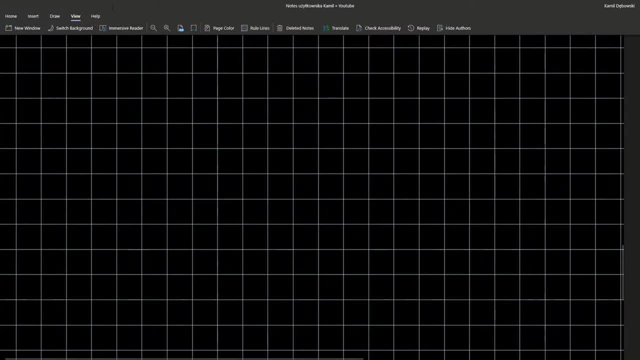 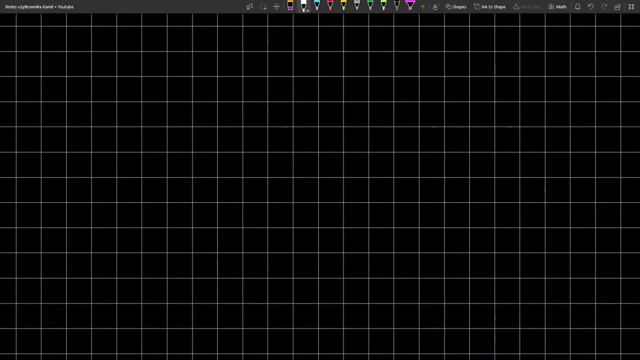 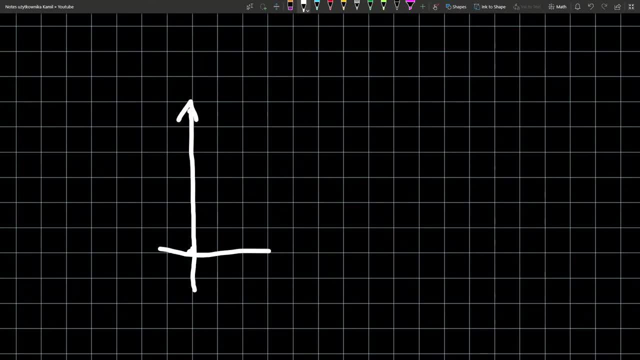 what is cross product? still, this stream won't necessarily be boring for you, because later we'll do harder problems. Well, for given two points, this one is what? four comma two, and this one is one comma five. Let me know if this grid 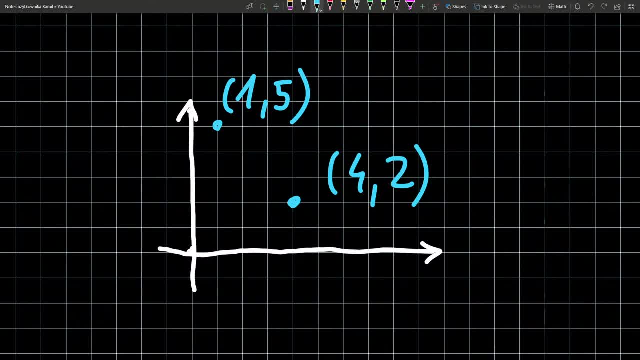 helps or not, I can hide it. One, five and four, two. Then cross product tells us two things: Area of a triangle, and which point is more to the left. More to the left when looking from the zero, zero point, We carry on. 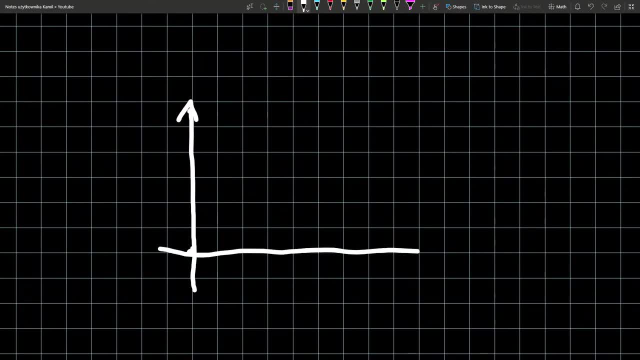 this stream won't necessarily be boring for you, because later we'll do harder problems. well, for given two points, this one is what four comma two, and this one is one comma five. let me know if this grid helps or not. i can hide it on. five and four, two, then cross product. 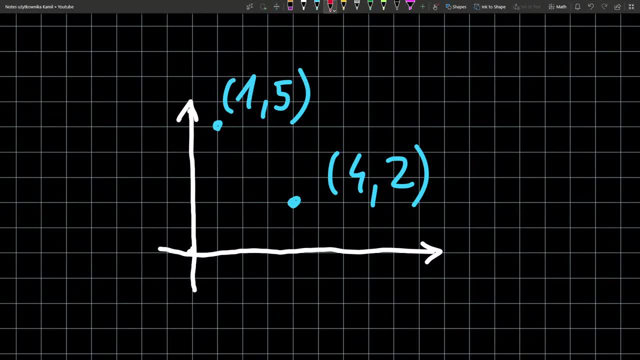 tells us two things: area of a triangle and which point is more to the left, more to the left when looking from the zero zero point. now we care about this triangle and cross product gives you twice the area of that and the sign of cross product tells you if this point or this point is more to the left. 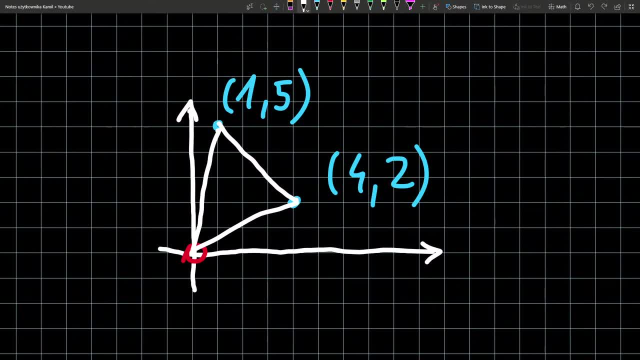 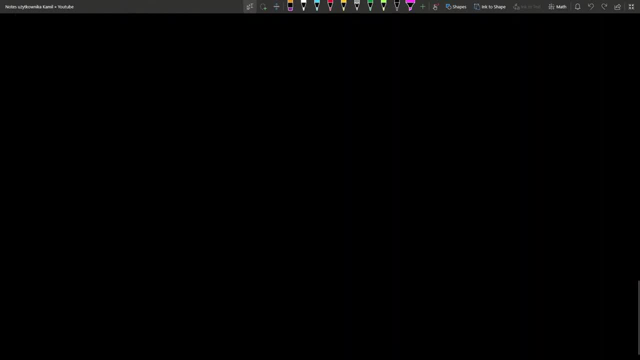 and grid is very good, all right, cool, but can i actually hide it in the next tab? okay, that's cool. formula is x1 multiplied by y2 minus x2 multiplied by y1, and we will actually derive that. i will show you why it makes sense. let's try to apply this formula here. in this example, this is x of the first. 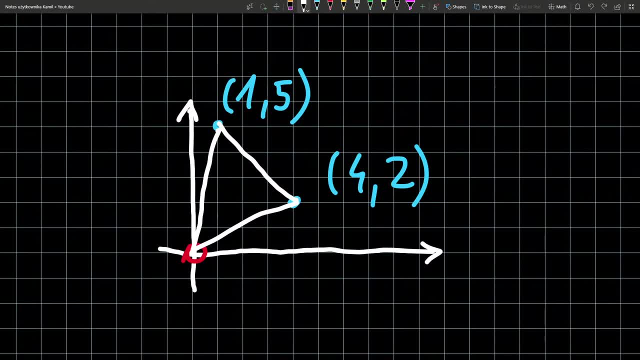 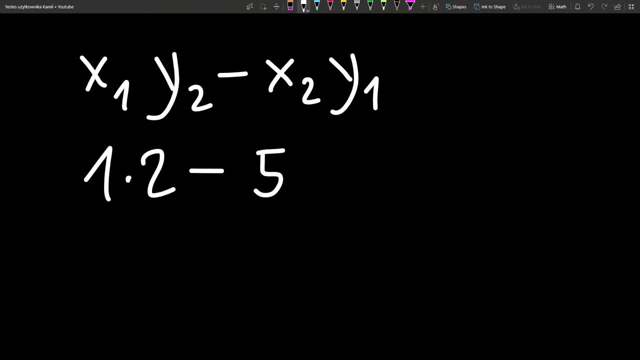 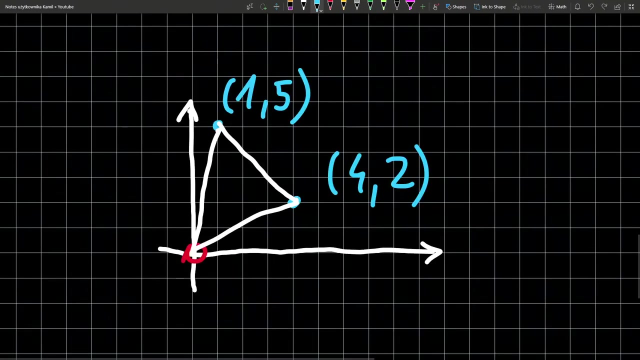 point multiplied by y of the second one. so one one times two minus the other, minus five times four. this is what minus 18 in our example, and i claim that this is twice the area. this is twice the area of a triangle. so area of this triangle is nine. you can kind of 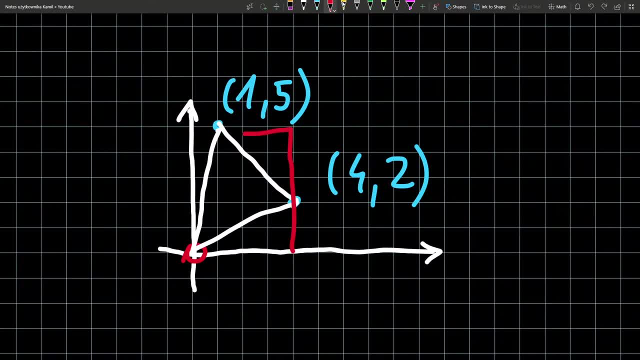 you can confirm it in some other way by computing area of this rectangle. that's 20- and is it always not so 20, and you can subtract those smaller triangles. this is four times two divided by one, so this has area four. this has area 4.5, i believe. and final this: 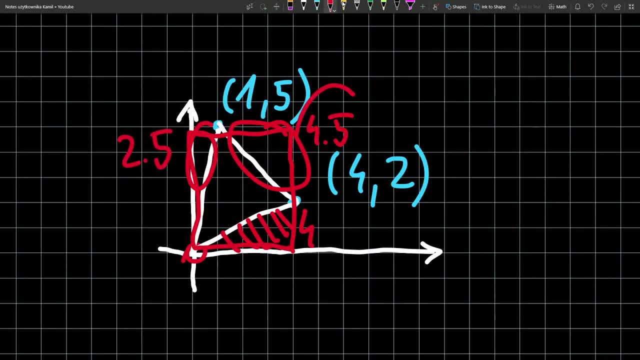 one is 2.5.. if you get 20, minus this triangle, then you can transform it by 12 billion px and minus those red numbers you should get 9.. Is it the case here? Yes, it is a case here. 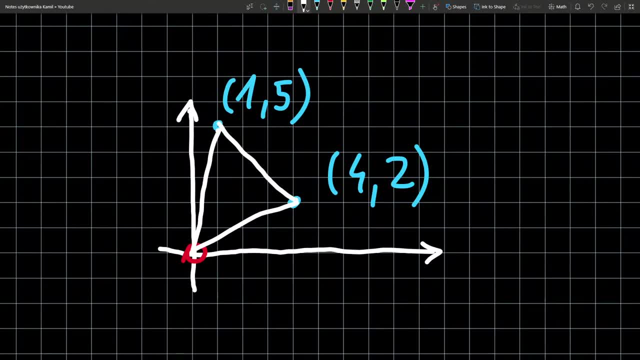 We care about this triangle and cross product gives you twice the area of that and the sign of cross product tells you if this point or this point is more to the left. And grid is very good, All right, cool, But can I actually hide it in the? 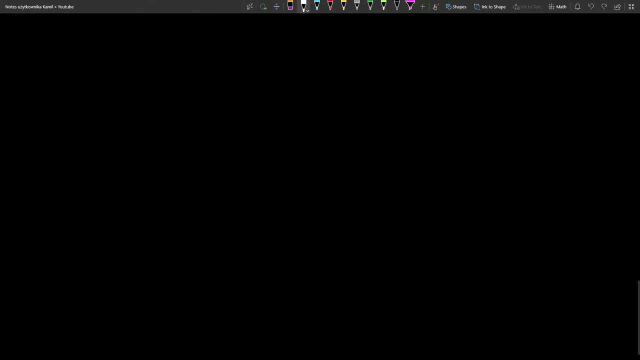 next tab. Okay, that's cool. Formula is x1 multiplied by y2, minus x2 multiplied by y1.. And we will actually derive that. I will show you why it makes sense. Let's try to apply this formula here. in this example, This is x of the. 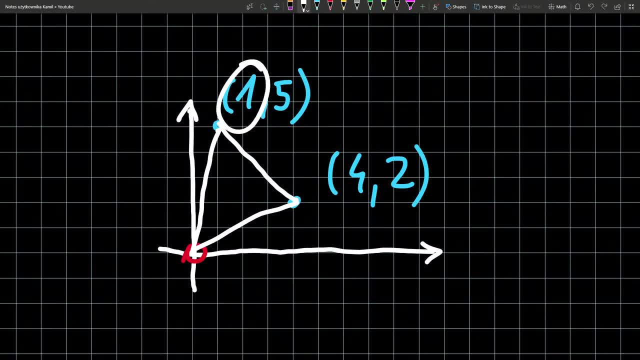 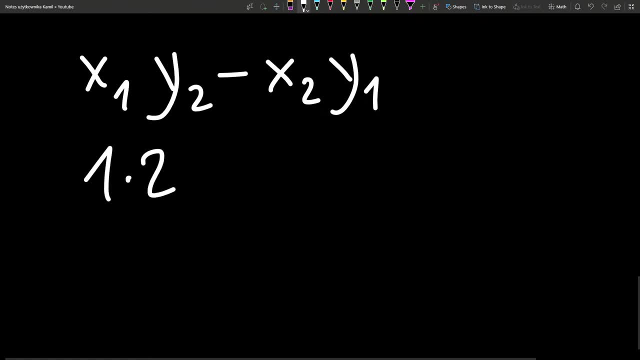 first point multiplied by y of the second one, One times two minus the other, Minus five times four, This is what Minus eighteen in our example, And I claim that this is twice the area. This is twice the area of a triangle. So area of this triangle is: 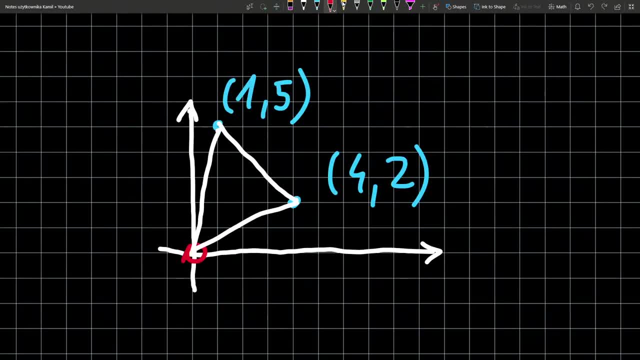 nine. You can kind of, you can confirm it in some other way- by computing area of this rectangle, That's 20.. And is it always So 20? and you can subtract those smaller triangles. This is 4 times 2 divided by 1.. So this has area 4.. This has 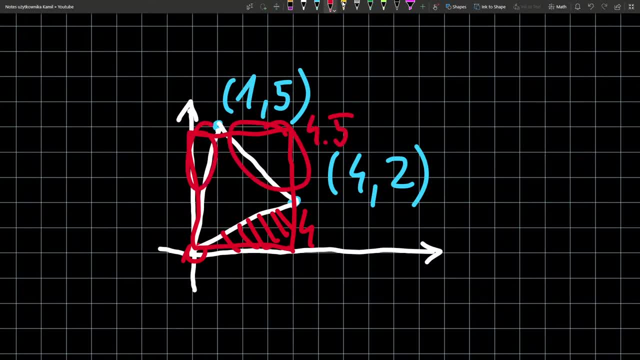 area 4.5, I believe. And finally, this one is 2.5.. If you get 20 minus those red numbers, you should get 9.. Is it the case here? 7. Yes, it is a case here, But it is just to confirm that. 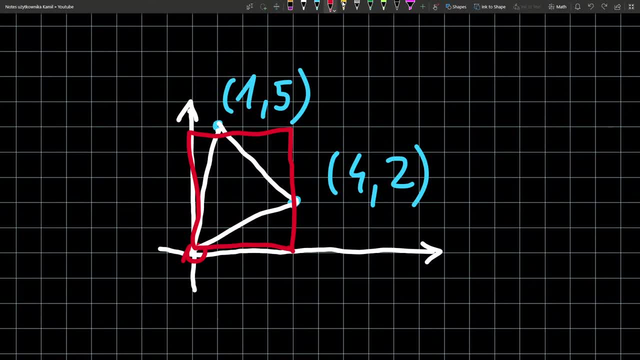 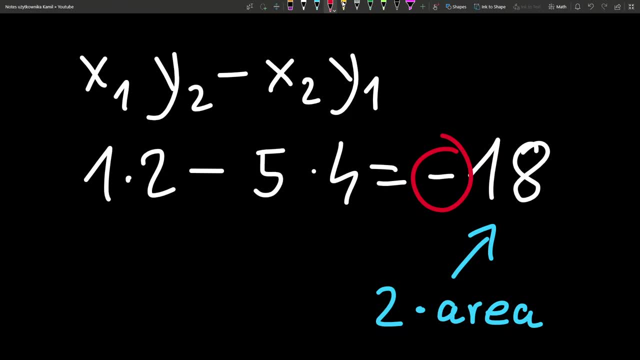 our computations make any sense And additionally, checking the sign here- negative versus positive- tells you if the first point is on the left or on the right, As x1 and y1, I took this point 1, 5.. This is my first point, This is my second point And if I 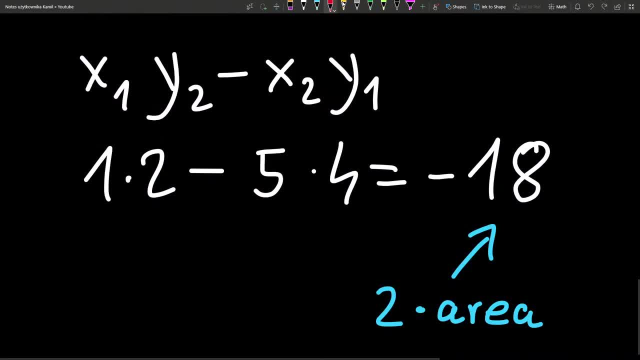 took them in this order, I got negative area. So apparently, whenever I get, with respect to 0,, 0,- this is p1 and this is p2,, then this cross product will be negative. This is negative if, and only if, p1 is on the left from p2.. Okay, Why? 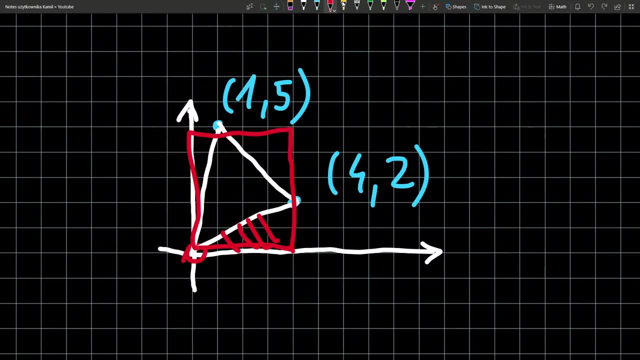 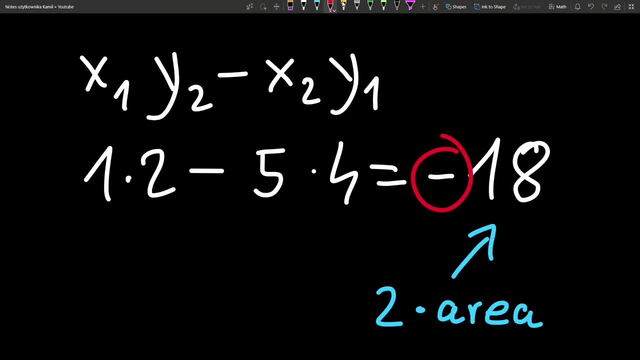 But it is just to confirm that our computations make any sense. And additionally, checking the sign here, negative versus positive- tells you if the first point is on the left or on the right As x1 and y1,. I took this point. This is my first point. 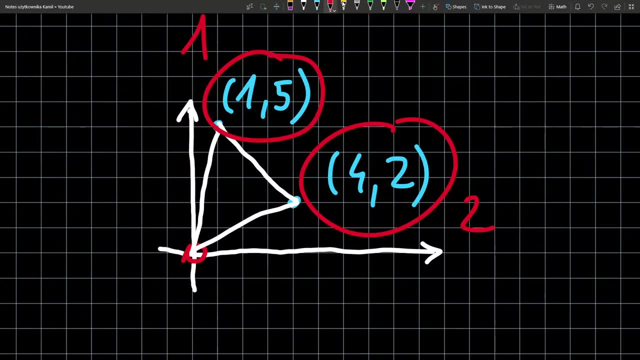 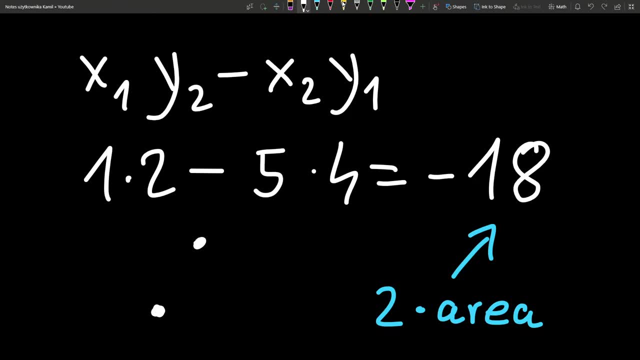 this is my second point, and if I took them in this order, I got negative area. So apparently, whenever I get with respect to this is p1 and this is p2, then this cross product will be negative. This is negative if, and only if, p1 is on the left from p2.. Okay, why it makes sense. 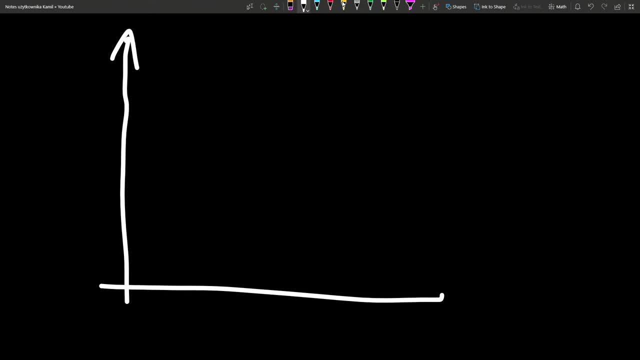 Let's look at it like this: What's the slope of point? Or maybe I would want to put it higher. Imagine that this is 2 and 5.. Then slope of this line, also related to this angle, is y divided by x. This has slope 2.5.. 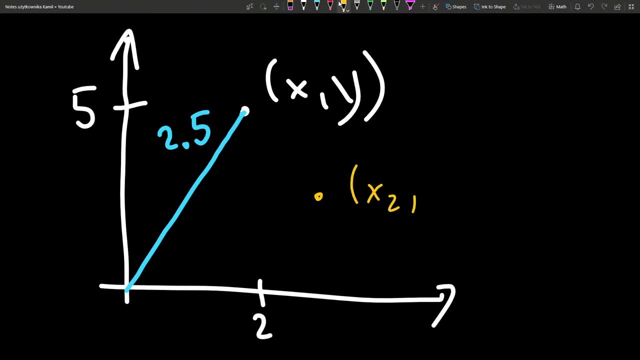 If you have some other point, say this one: x2 comma, y2.. And let's say that this is 3 and 2.. This slope is 2 divided by 3.. 0.66.. This slope is bigger, so this point is more on the left. 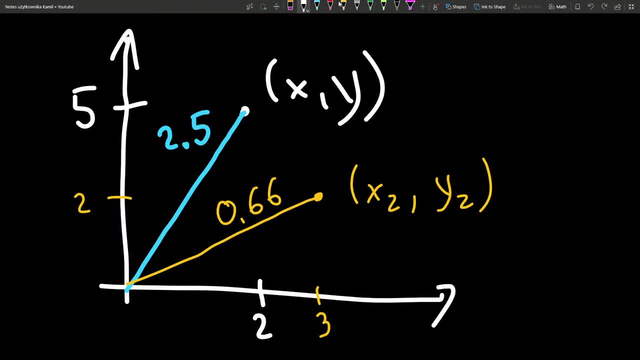 But how to write this down? with a formula: y divided by x is greater than y2 divided by x2.. multiply both sides. Well, there's something tricky here because you might get It doesn't work if X is negative. but let's say for now that we can multiply both sides by X's to get rid of fractions. 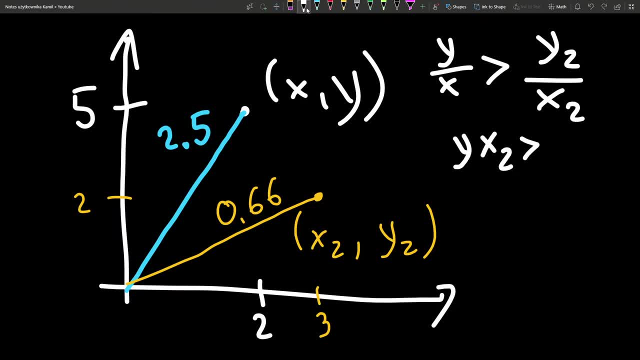 Then we have Y X 2 greater than X Y 2, and let's move everything to one side, Let's say to the right side. I will get X Y 2 minus Y X 2 Is smaller than zero. This is a condition when this guy is more on the left and this is cross product. 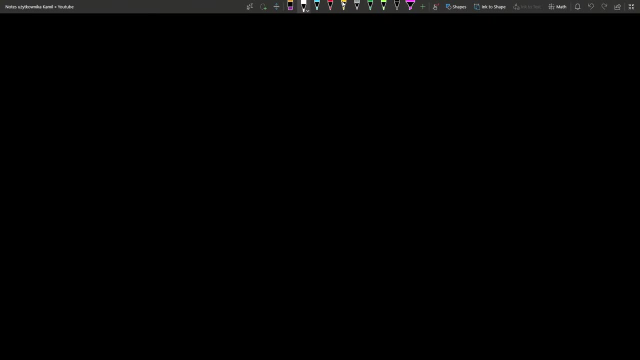 It makes sense. Let's look at it like this: What's the slope of point x, y- Or maybe I would want to put it higher: x, y. Imagine that this is 2 and 5. Then slope of this line, also related to this angle, is y divided by x. 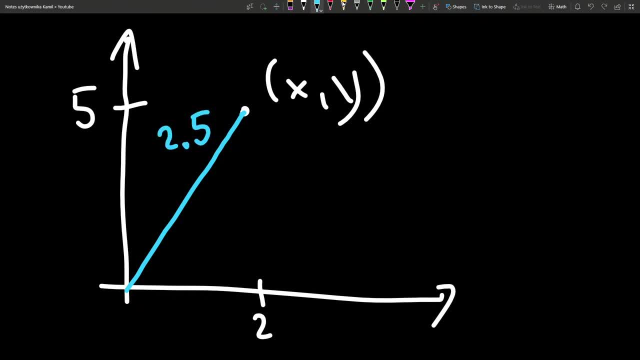 This has slope 2.5.. If you have some other point, say this one: x2, y2.. And let's say that this is 3 and 2.. This slope is 2 divided by 3, 0.66.. 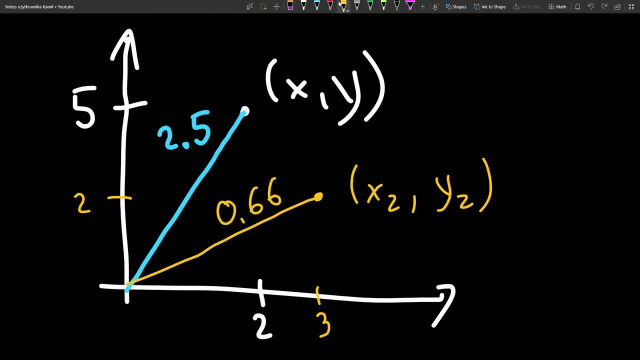 This slope is bigger, so this point is more on the left. But how to write this down? with a formula: y divided by x is greater than y 2 divided by x2.. Multiply both sides. Well, there's something tricky here because you might get it doesn't work if x is negative. But let's say for now: 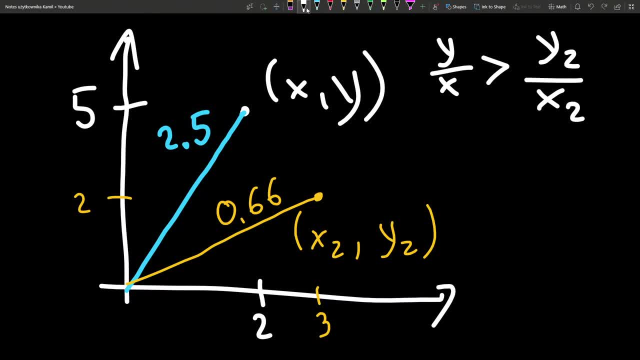 that we can multiply both sides by x's to get rid of fractions. Then we have yx2 greater than xy2.. And let's move everything to one side. Let's say to the right side, I will get xy2 minus yx2.. 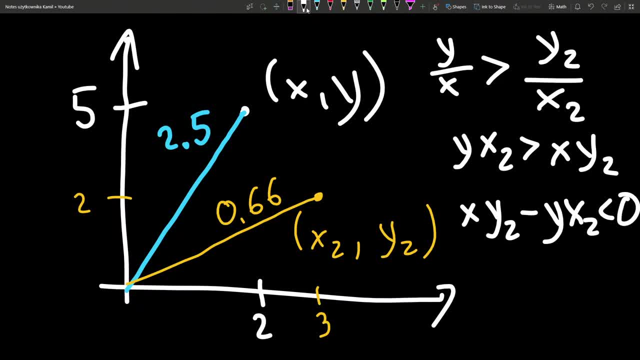 Yx2 is smaller than zero. This is a condition when this guy is more on the left, And this is cross product. We will discuss CSES problems, but first this is cross product recap. This is exactly the formula that we use. This is why it makes. 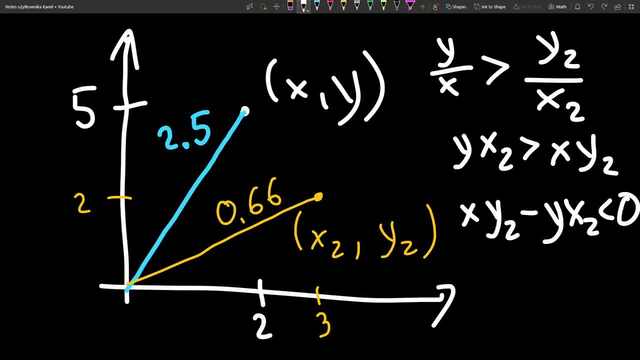 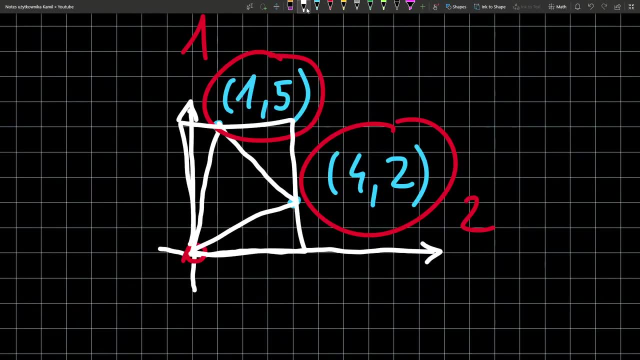 sense. So this is how you can prove that sine matters. If this is positive, on the other hand, then you will have the other way around. the first point would be on to the right and, in terms of area, you would need to Get some formula to compute rectangle area. subtract those three, reduce everything and you will again get this formula. 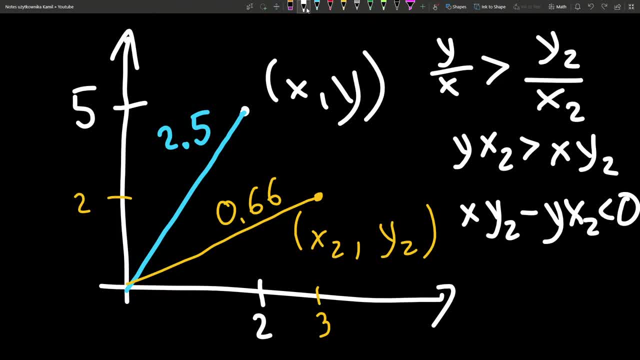 We will discuss CSEs problems, but first this is cross product recap. This is exactly the formula that we use. this is why it makes sense. So this is how you can prove that Sine matters. if this is positive, on the other hand, then you will have the other way around. the first point would be on to the right and 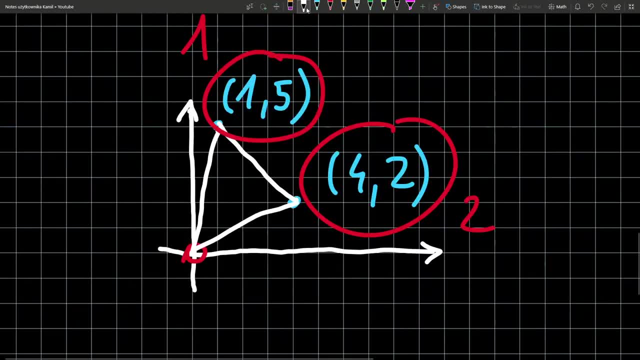 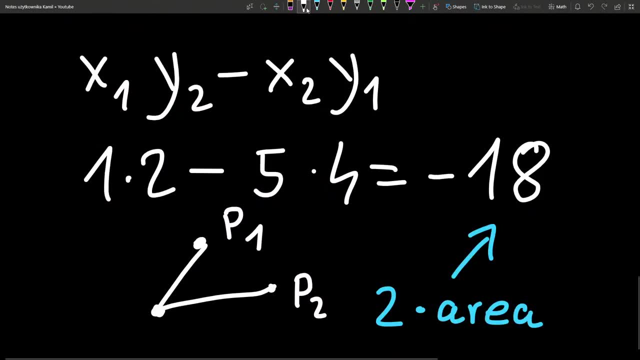 in terms of area. You would need to get some formula to compute rectangle area. subtract those three, reduce everything and you will again get this formula. so this is called cross product of two points: X 1- Y 1 and X 2- Y 2. Very important. This app is called OneNote. 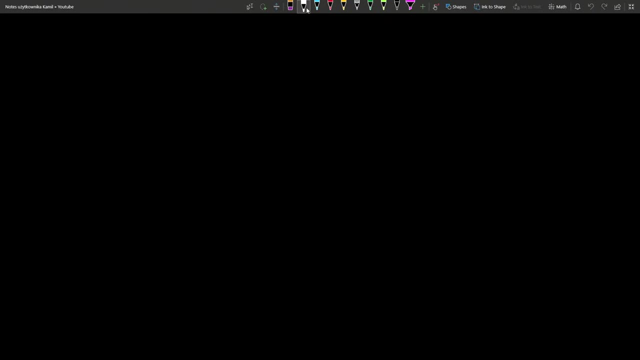 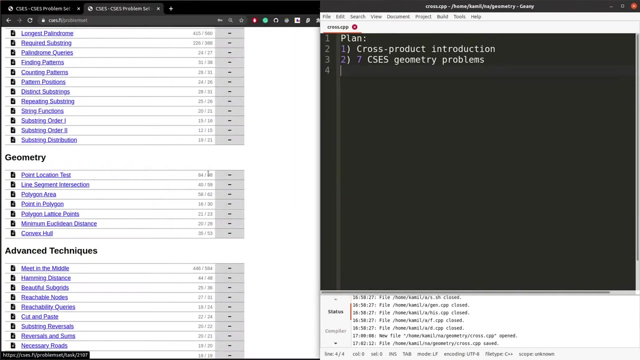 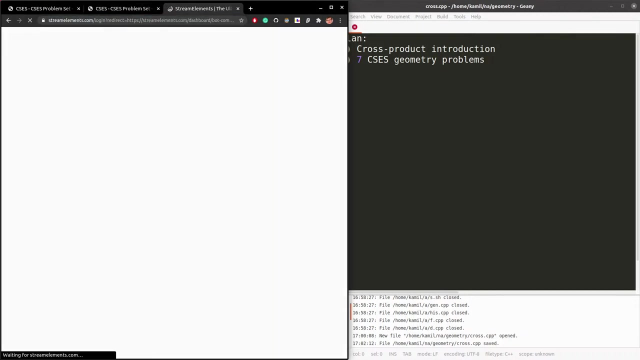 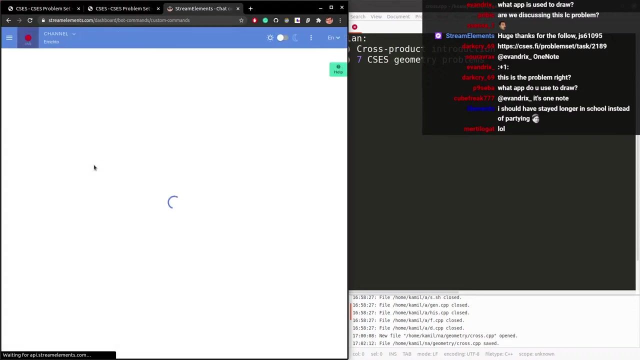 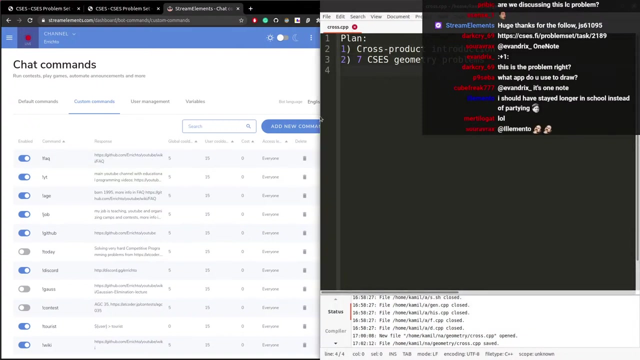 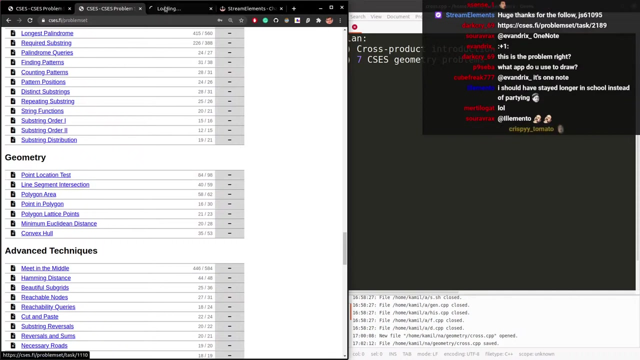 Right, Let's use this knowledge to start solving problems. The first problem, and I think I didn't provide a link One moment. We are, by the way, done with first point of our plan: cross product recap, And now we will move to solving problems. Start with this guy. 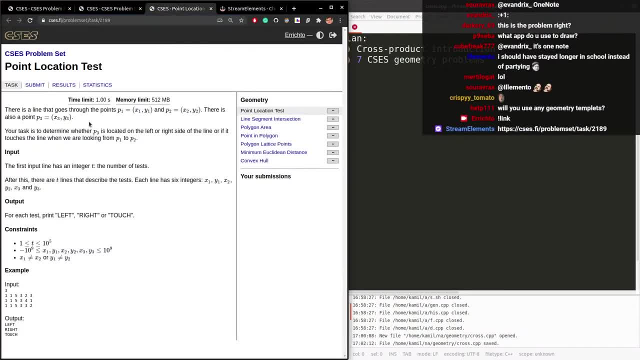 Here we go. The first problem is point location test. there is a line that goes through points p1, p2. There is also a point p3. Your task is to determine whether p3 is located or not, If p3 is located on the left or right side of the line. 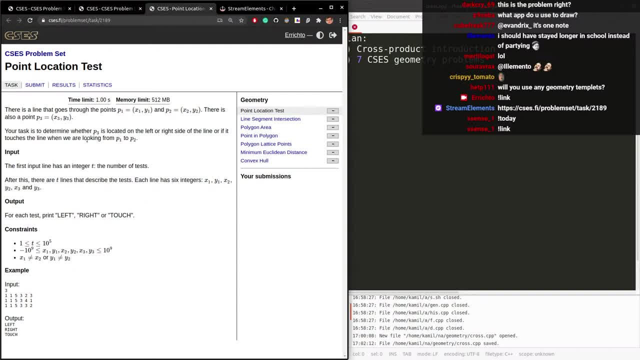 Or if it touches the line. when we are looking from p1 to p2, We just need to say left, right or touch. whether three points are collinear or Something is to the left or to the right, We will use cross product, which shouldn't surprise you. 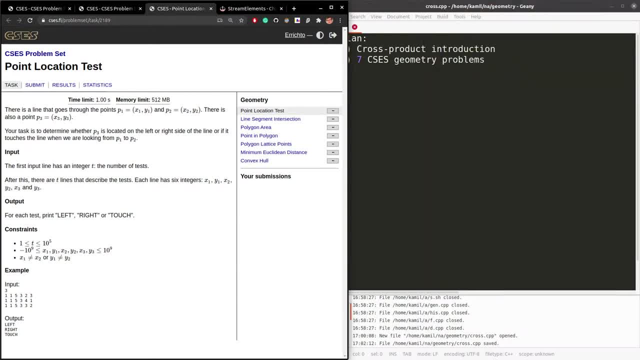 And also, please, mainly questions about the stream I don't really want to focus on, you know, other questions No, and to make it easier later To get back to some part, I will just Write the current problem. This is p1 point location test To move it somewhere. 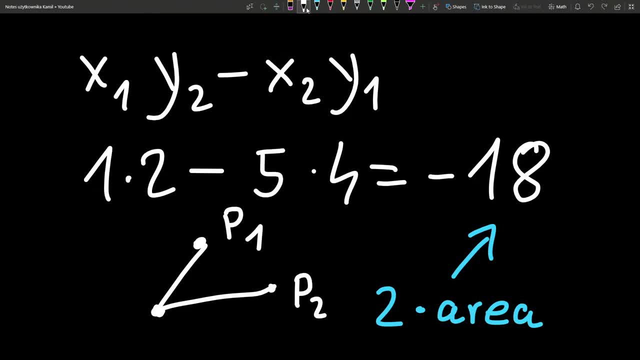 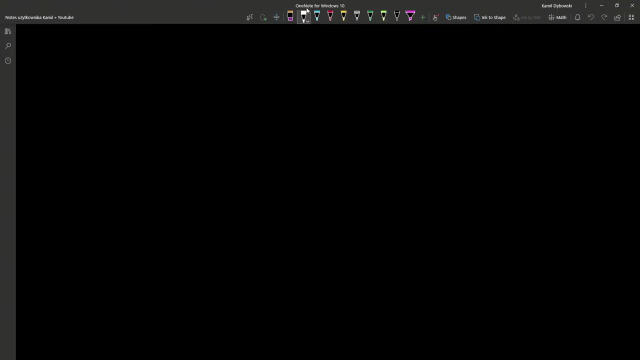 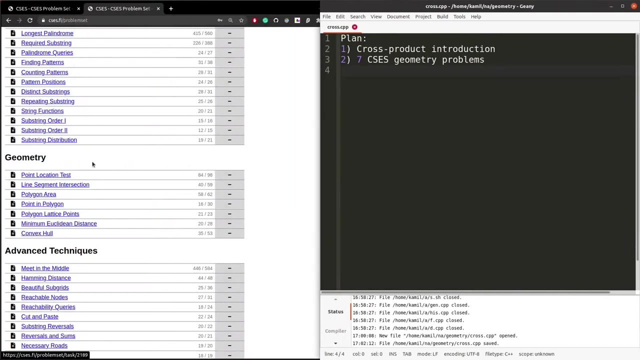 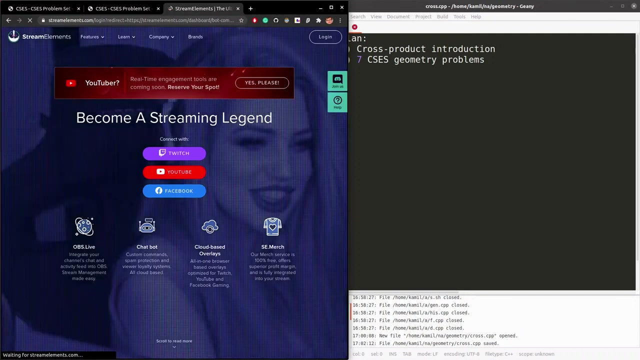 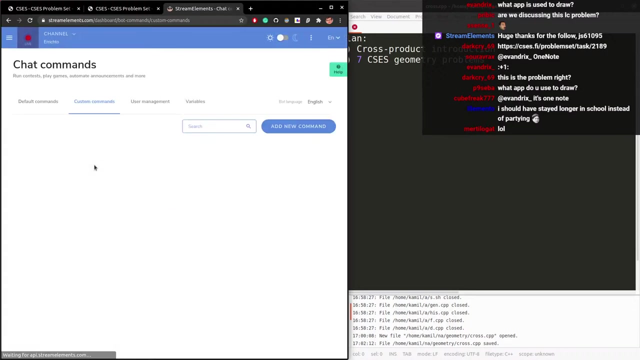 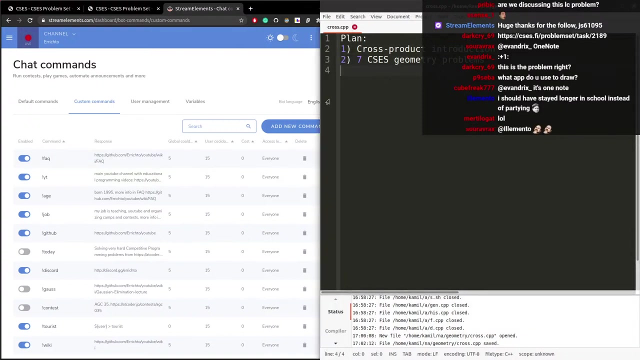 so this is called cross product of two points: X1- Y1 and X2- Y2. very important. This app is called OneNote. Let's use this knowledge to start solving problems. The first problem, and I think I do provide a link One moment. We are, by the way, done with first point of our plan, cross product recap, and now we will move to solving problems. 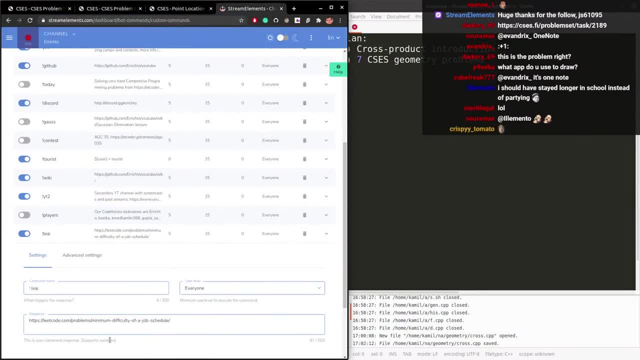 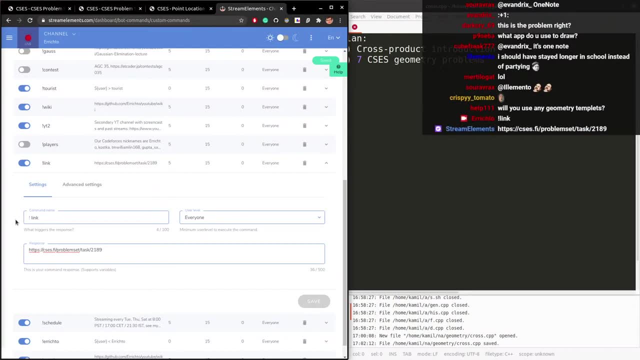 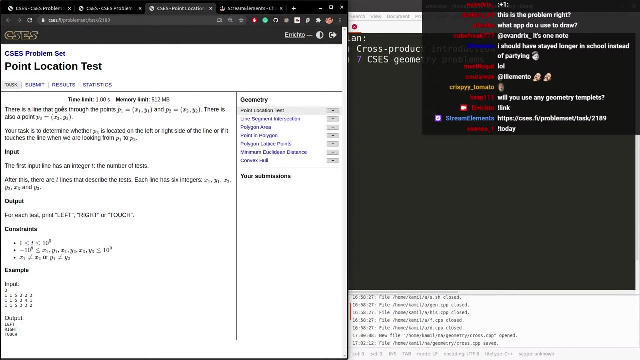 Start with this guy. Here we go. The first problem is point location test. There is a line that goes through points P1, P2. There is also a point P3. your task is to determine whether P3 is located on the left or right side of the line. 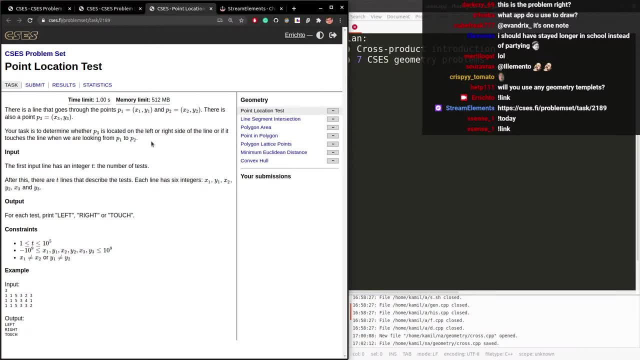 Or if it touches the line. when we are looking from P1 to P2, We just need to say left, right or touch. whether three points are collinear or Something is to the left or to the right, We will use cross product, which shouldn't surprise you. 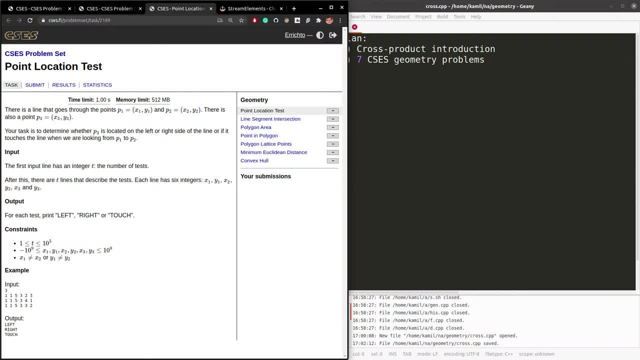 And also, please, mainly questions about the stream. I don't really want to focus on- you know- other questions now, and to make it easier later To get back to some part, I will just Write the current problem. This is P1 point location test. 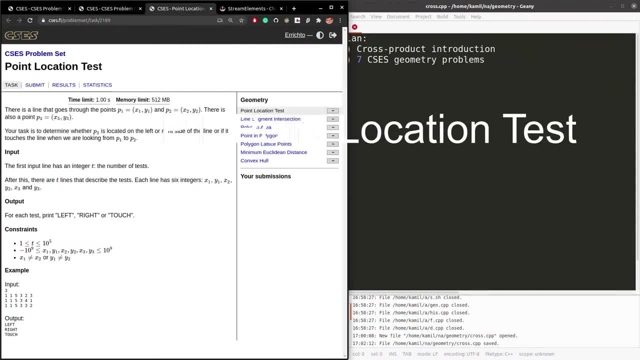 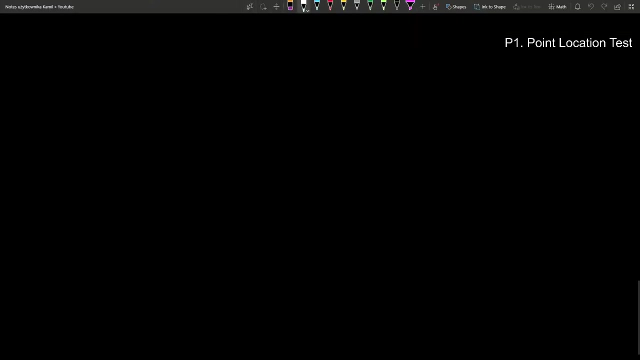 To move it somewhere. This should work most of the time. Maybe we'll make it nicer later. Right, let's solve the problem. They told us that we need- we are given three points: P1, P3, P2. Now we need to consider a line going to the left or to the right. 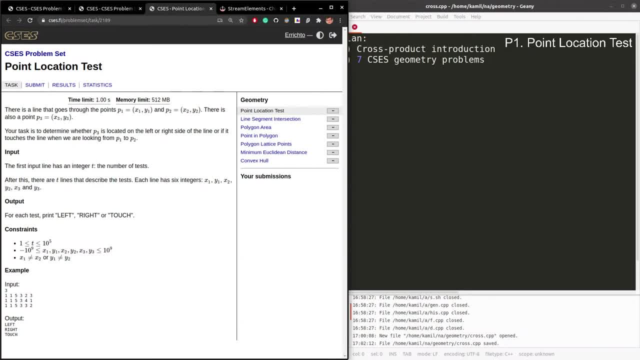 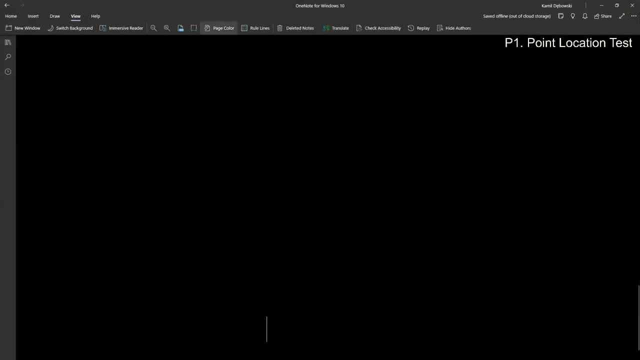 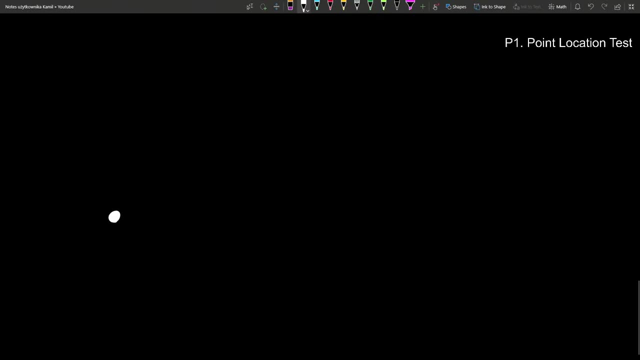 This should work most of the time. maybe we'll make it nicer later on. right, let's solve the problem. they told us that we are given three points: p1, p3, p2. now we need to consider a line going through p1, p2. and they said: if we look from 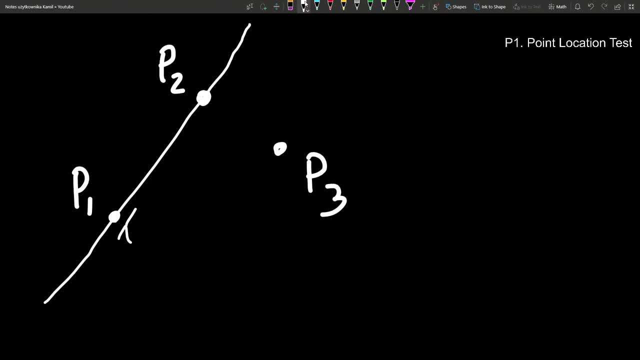 p1 to p2,. so imagine that you stand there, you're an ant or a human, and you look there is p3 relative to this direction. is it on the right or on the left? if it was here, we need to say on the right. if it is anywhere there, we need to say on the left. 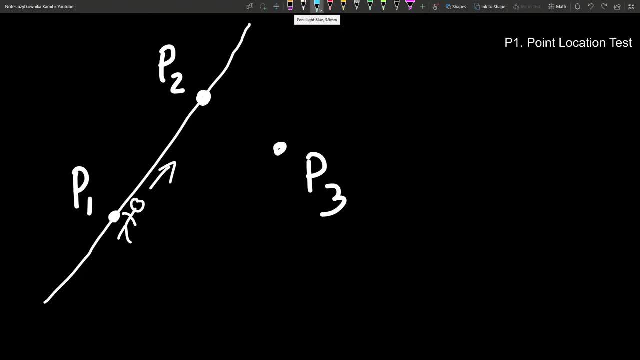 what will we say? and let's use an example of particular data. let's say that this is point 3,4, this one is 5,10 and this is something more to the right 8,67. it's very useful technique to move everything. 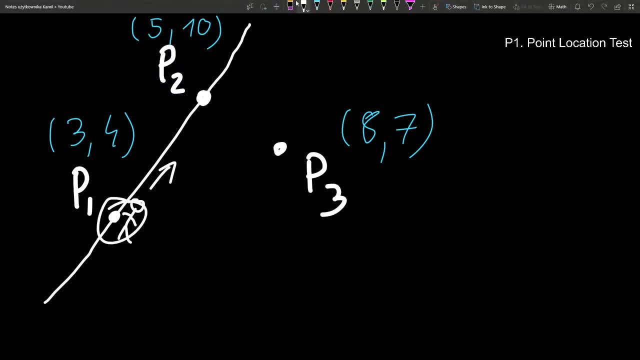 to imagine that one point with respect to which we take everything, this point 0,0. I want to say that this is actually 0,0, and you know, I have this axis with coordinates x and y, then everything kind of shifts by 3,4. 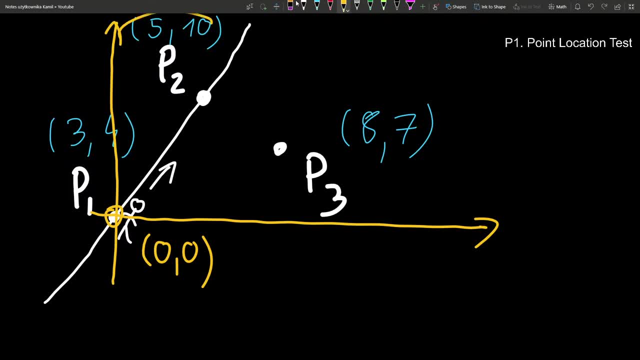 if I want 3,4 to become 0, then, with respect to that, 5,10 becomes 5-3 a 2 and 10-4 a 6 and 8,7 becomes, with respect to 3,4, 8,7 is 5,3. 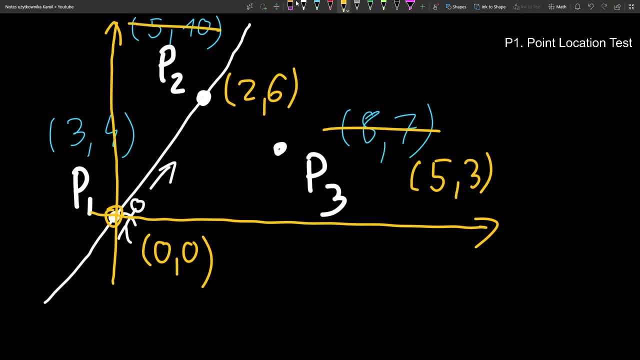 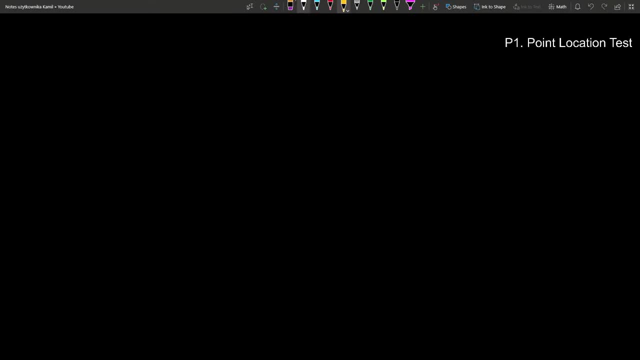 now we can forget about blue values. the answer will be the same, because we just shifted everything. the other way to look at it is: if you want to say that with respect to p1, you are looking at p3, then this segment with direction is called a vector. 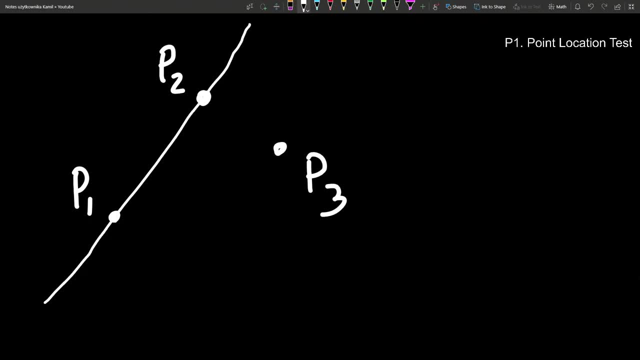 So if we look from P1, P2, and They said, if we look from P1 to P2, so imagine that you stand there, You're an ant or a human and you look, there Is P3 relative. relative to this direction. Is it on the right or on the left? 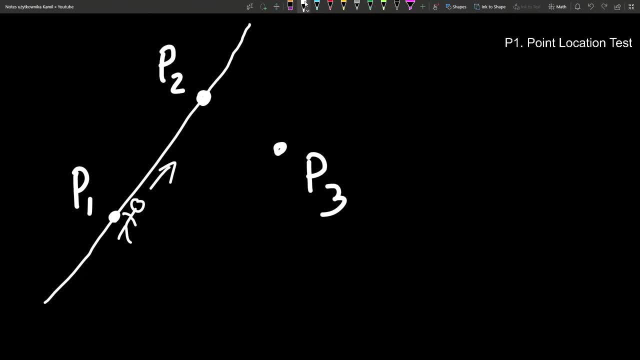 If it was here, we need to say on the right. if it is anywhere there, we need to say on the left. What will we say? and let's use an example of Particular data. Let's say that this is point three comma four. This one is five comma ten. 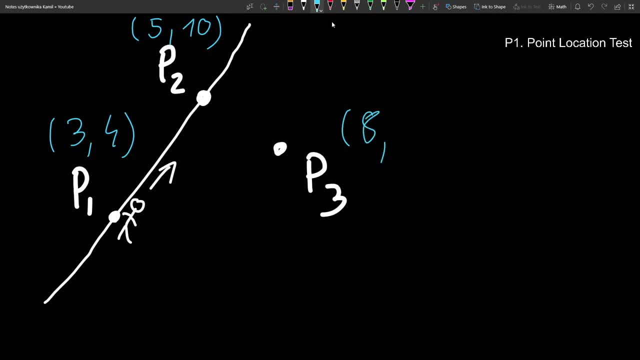 And this is something more to the right eight comma, six, seven, right then, It's very useful technique to move everything, to imagine that one point with, With respect to which we take everything, that it is point zero, zero, I want to say that this is actually zero, zero and 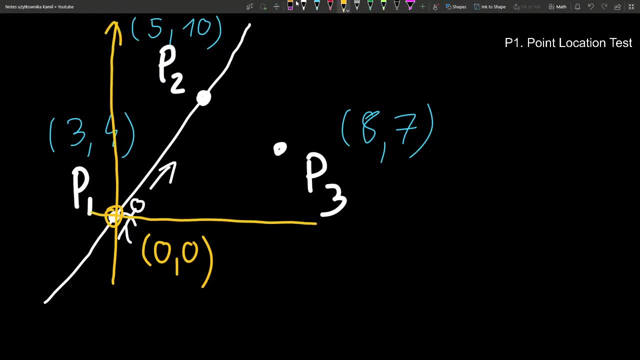 You know, I have this X's with coordinates x and y, then everything kind of shifts by three, four, like if I want three, four to become zero and with respect to that, five, ten becomes five minus three, a two and ten minus four, six and eight, seven becomes. 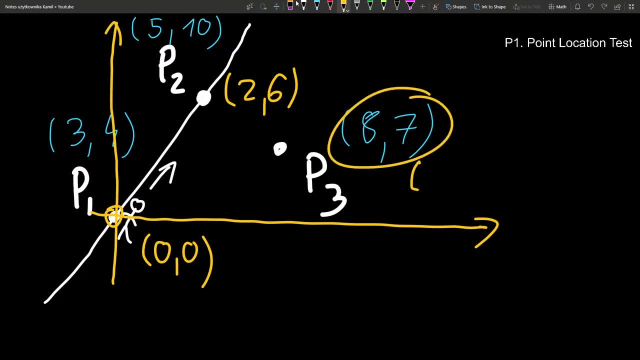 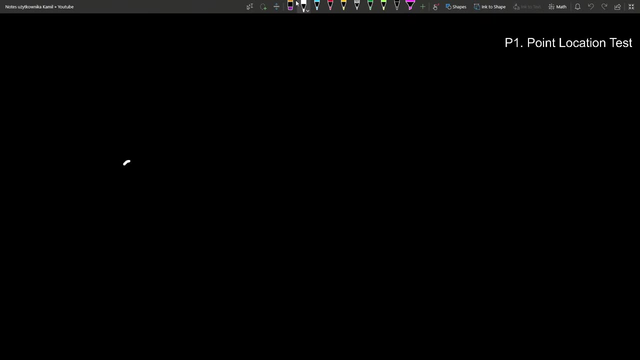 No, we comes. what with respect to three, four, eight, seven is five comma three. Now we can forget about the blue values. The answer will be the same, because we just shifted everything. the other way to look at it is: If you want to say that, with respect to P1, you are looking at P3. 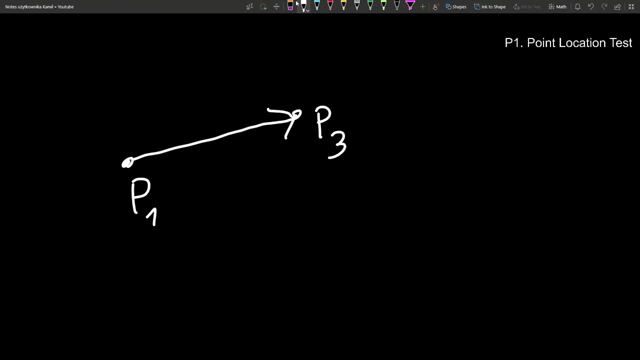 then this Segment with direction is called a vector, vector P1, P3 is what you get when you kind of subtract coordinates. and In the long run, if you want to solve hard problems, Then for sure you want to use vectors, you want to understand vectors, but this is not a must. 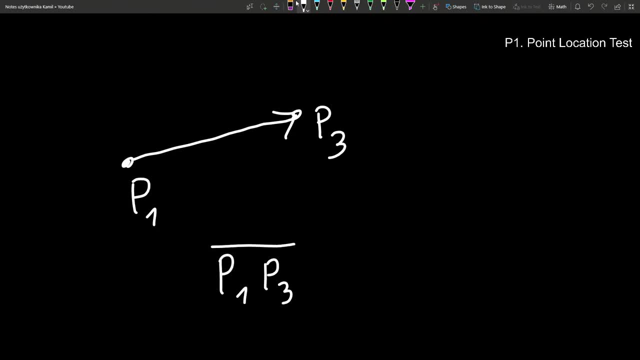 vector p1,p4. p3 is what you get when you kind of subtract coordinates. and in the long run if you want to solve hard problems, then for sure you want to use vectors, you want to understand vectors. but this is not a must, it's just useful way to think about it. 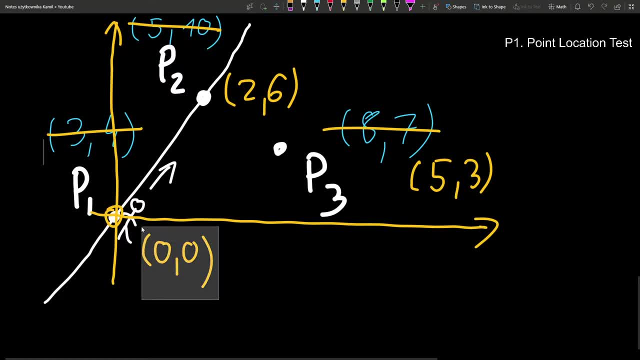 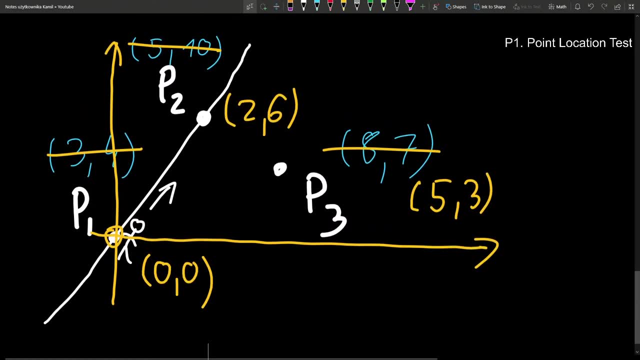 thinking about vectors is equivalent to saying that one point becomes 0,0. with respect to this point, we are looking at everything else. we need to subtract coordinates. and then it's about using our cross product. we already know that if we take cross product of p2 and p3 in this order, 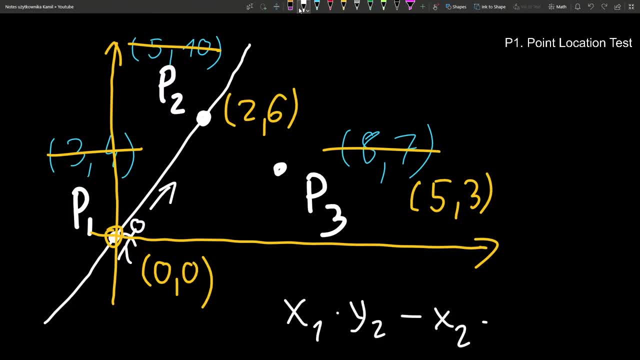 using a formula: x1 minus y2 minus x2 times y1, and then we'll get sine. we'll get area of this triangle doubled and we'll get sine. negative, positive or 0, 0 is a case. if the ratio is the same, slope is the same. 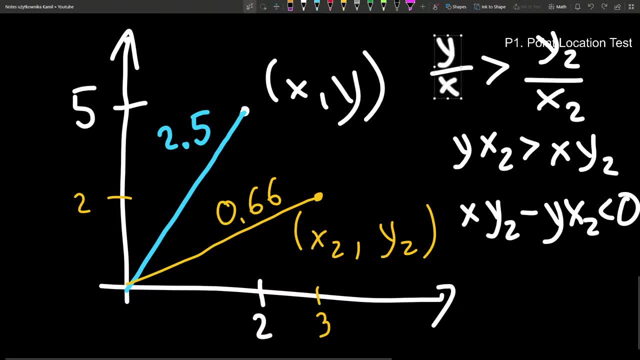 remember how here we compared y divided by x with y2 divided by x2. well, we have equality if, and only if, here at the end, we have equality with 0. I said one moment that we assume that x's are negative. actually, all the math also works out in that case. 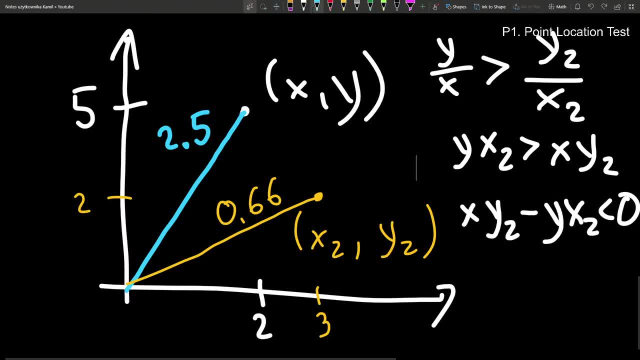 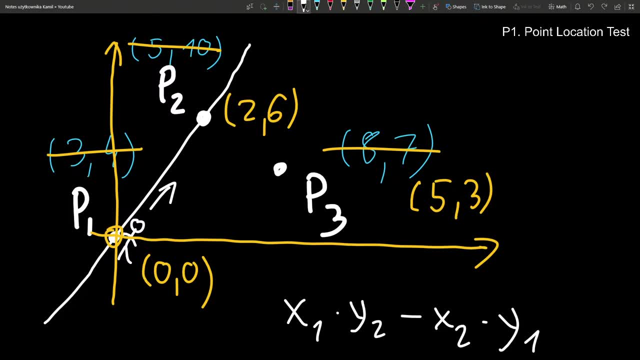 but it's more tricky. let's just assume that it always works, no matter if points are positive or not. I just wanted to show you some intuition and it was easiest to work with positive coordinates. but we know a solution. this is it shift everything. with respect to p1. 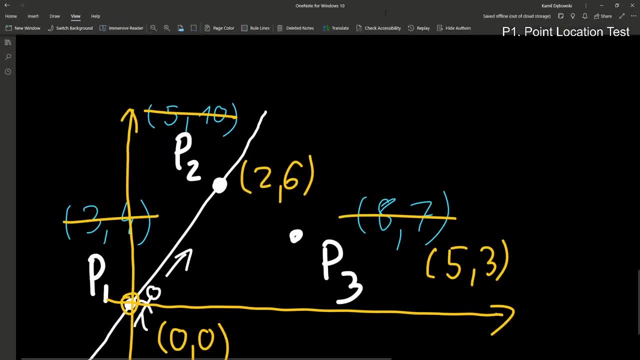 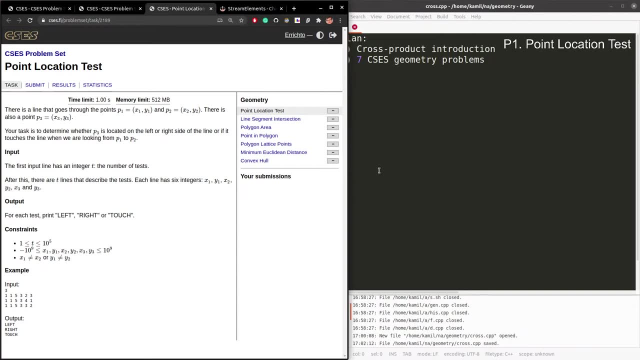 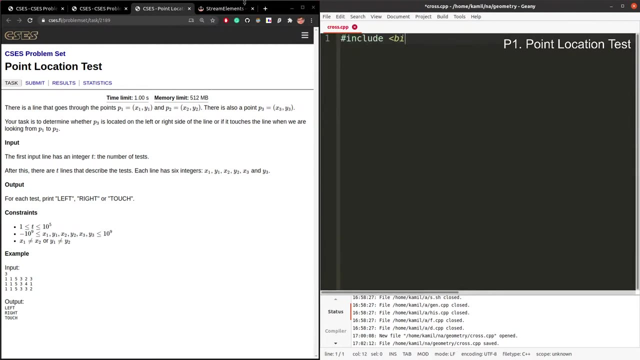 and then check the cross product. let's do some coding. this text would be too low now. it is not aligned. no, it is, as I said, no prewritten code. we'll start with something very basic here and then we'll use a C++ track to make it nicer. 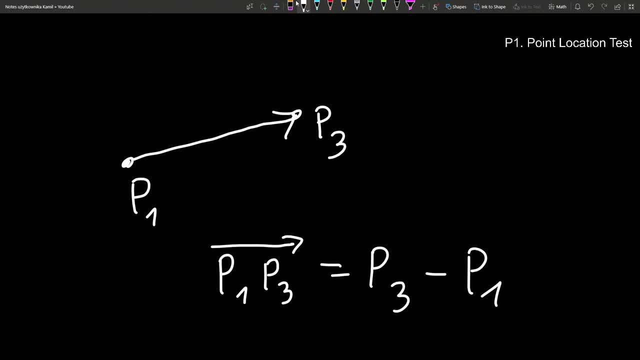 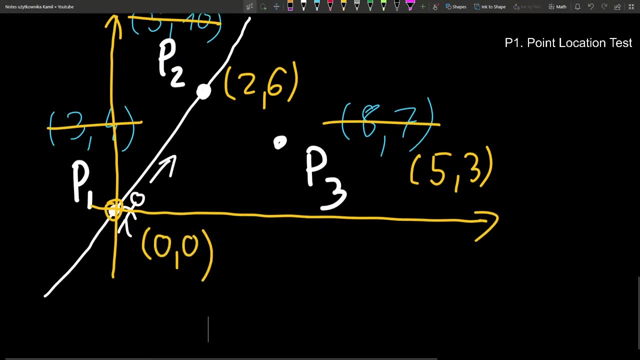 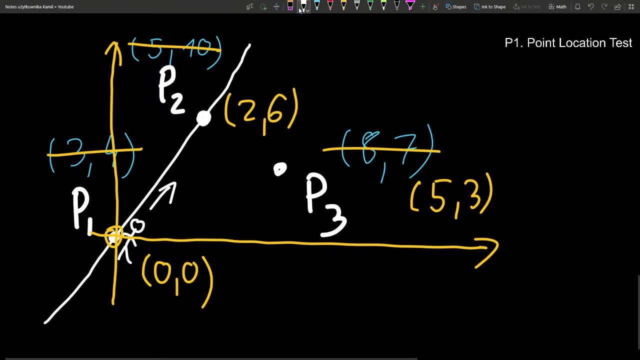 It's just useful way to think about it. Thinking about vectors is equivalent to saying that one point becomes zero- zero with respect to this point. We are looking at everything else. we need to subtract coordinates. and Then it's about using our cross product. We already know that if we take cross product of P2 and P3 in this order, using a formula x1 minus y2 minus x2 times y1, 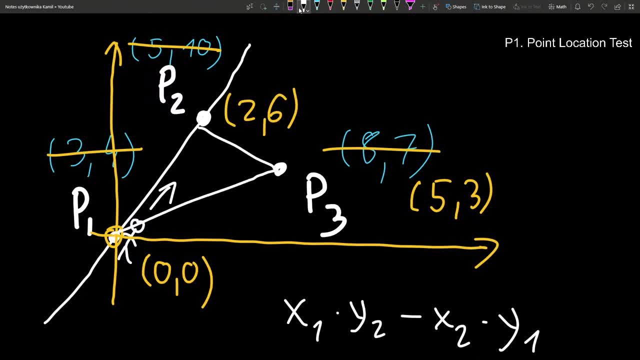 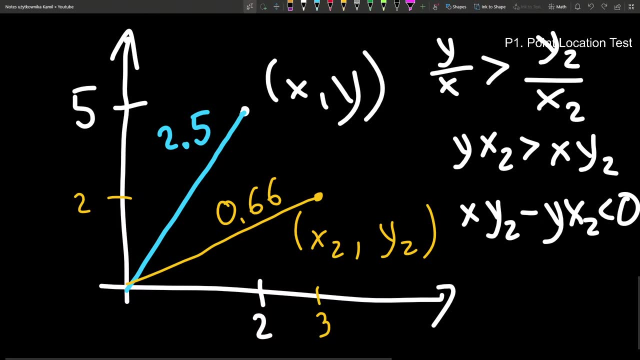 And then we'll get sine, We'll get area of this triangle doubled and we'll get sine negative, positive or zero. zero is a case if the ratios is this time slope is the same. remember how here We had. we compared y divided by x with y2 divided by x2. 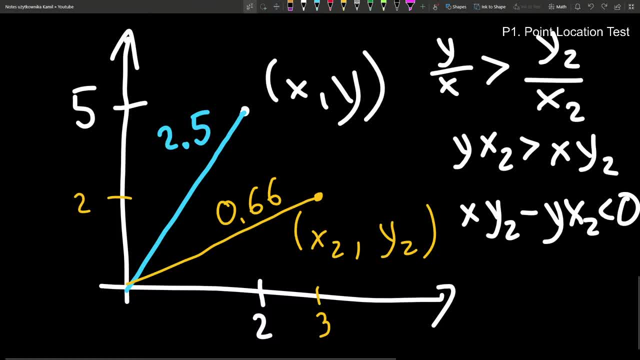 well, We have equality if, and only if, here at the end we have equality with zero. As I said one moment that, oh, we assume that X's are negative. Actually, all the math also works out in that case, but it's more tricky. Let's just assume that it always works. 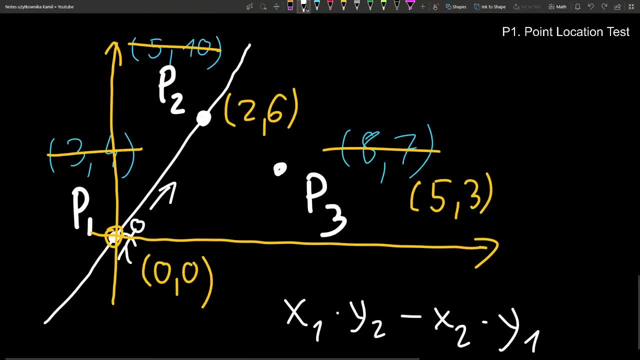 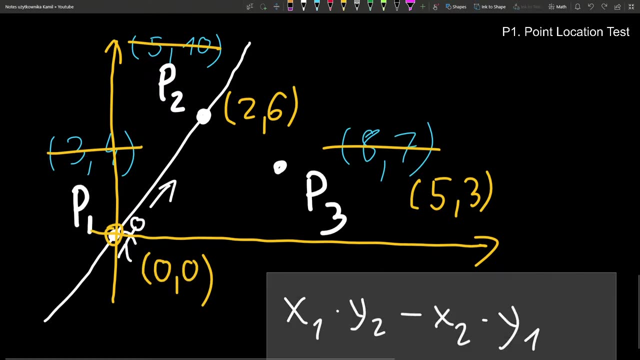 No matter if points are positive or negative. I just wanted to show you some intuition, and it was easiest to work with positive coordinates. But we know a solution. this is it: shift everything with respect to P1 and then check the cross product. Let's do some coding. 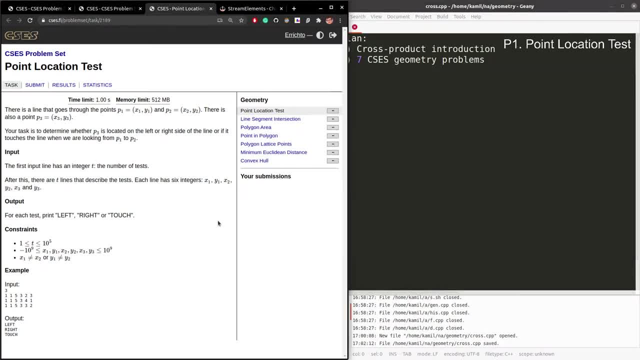 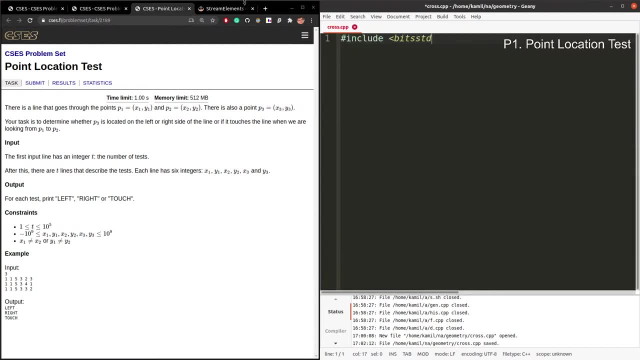 This text would be too low. now, It is not a line, No, it is, As I said, no pre-written code. We'll start with something very basic here and then we'll use a C++ track to make it nicer. Vector algebra and coordinate geometries must a must for doing geometry problems in CP. 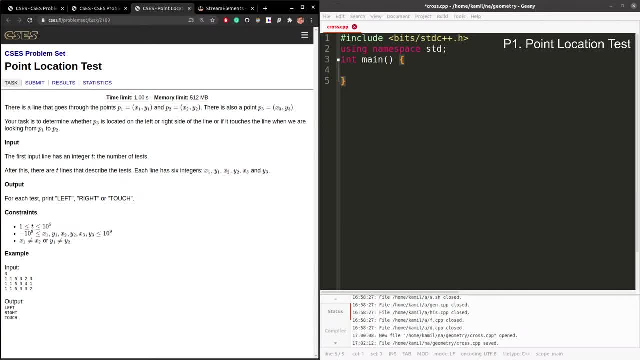 Yes, yes, like coordinates and vectors are very, very important. All right, there are test cases in this problem. It's not really important for every test case. For every test case. this is important. When you start with geometric problems, You will, just you know, create a lot of variables and read them one by one, which becomes very ugly. 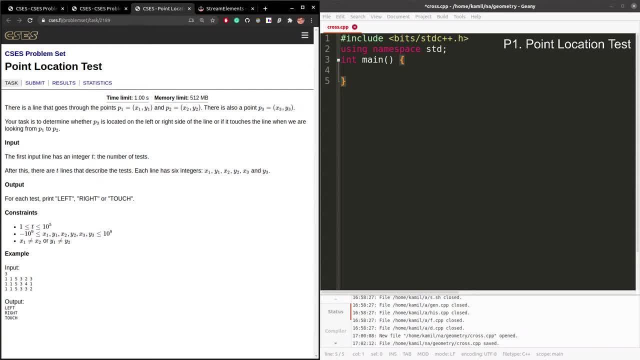 vector algebra and coordinate geometry is a must- a must for doing geometry problems in CP. yes, coordinates and vectors are very, very important. there are test cases in this problem, which is not really important for every test case. this is important when you start with geometry problems. you will just create a lot of variables. 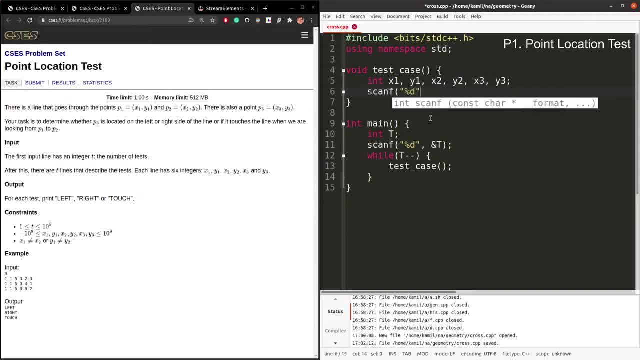 and read them one by one, which becomes very ugly. what if you are given 5 points and you need to, let's say, check if it's convex polygon? you don't want to create 10 variables. for now we'll do, and then I will move to nicer implementation. 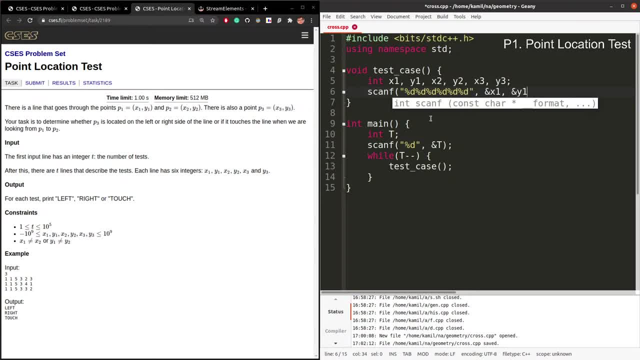 6?? yeah, there are 6, so it's going to be 3,5,6,7,8,9,10,11,12,12,13,15,16,17,18,19,20,22,23,24,25,26,27,28,29,30,33,35,36,37,39,40,41,43,44,44,45,46,47,48,49,49,50. 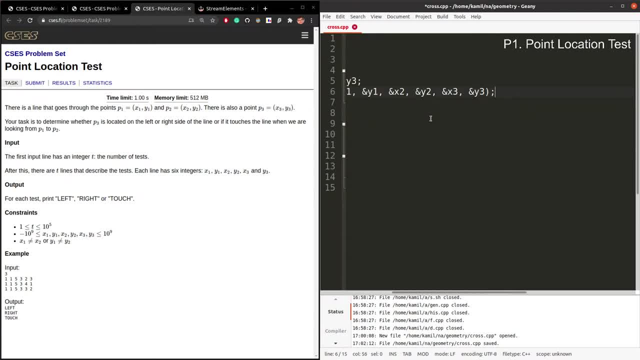 ah, very ugly. maybe I should have used scene. uh, yeah, sorry, this will be more readable for you, so let's keep using it. scanf isn't really reading. friendly, human, friendly, right, read this. we subtract coordinates and I can do it like this with respect to the first point, p1, which has coordinates x1, y1. 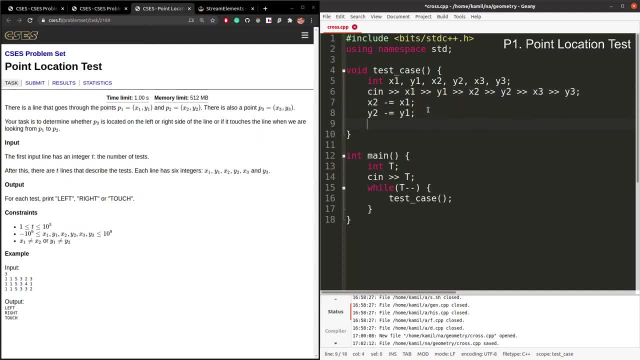 I need to take other coordinates. so one way is to do it like that and then kind of be done with it when I, whatever formula I will use, I almost make it made a mistake. y3 minus equal y1, right, and now those two coordinates of p2 and p3 are computed correctly with respect to p1. now the cross product. 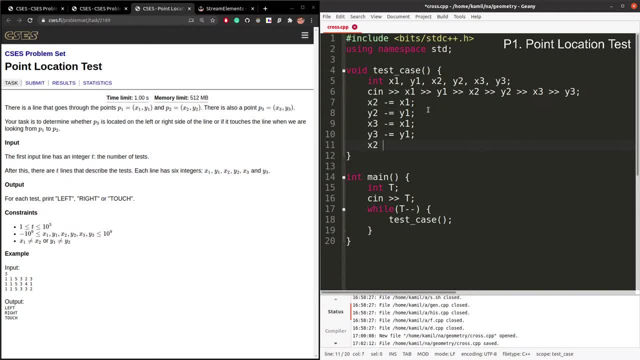 x, x of first point multiplied by y of the other point, minus the other way around. if this is negative- we already saw that- then the first point is more to the left. what do we need to check? if we need to check whether p3 is located on the left side, I will use maybe. 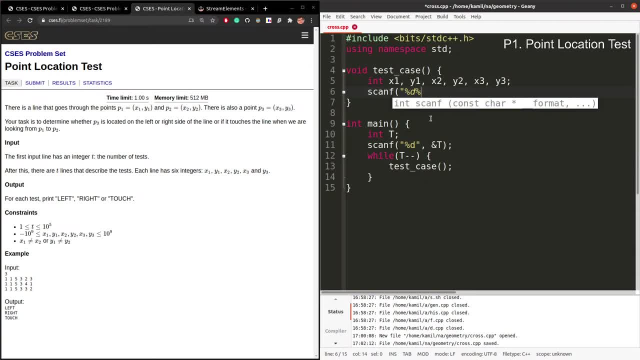 If what? if you are given five points and you need to, let's say, check if it's convex polygon. You don't want to create ten variables for now will do and then I will move to nicer implementation. Six- Yeah, there are six. Very ugly, maybe I should have used to seen. I 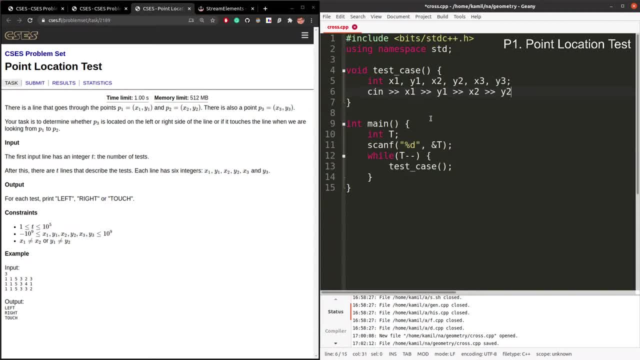 Sorry, this will be more readable for you, So let's keep using it. Scan isn't really reading. friendly, human, friendly, right, read this. We subtract coordinates and I can do it like this With respect to the first point: p1, which has coordinates x1, y1. 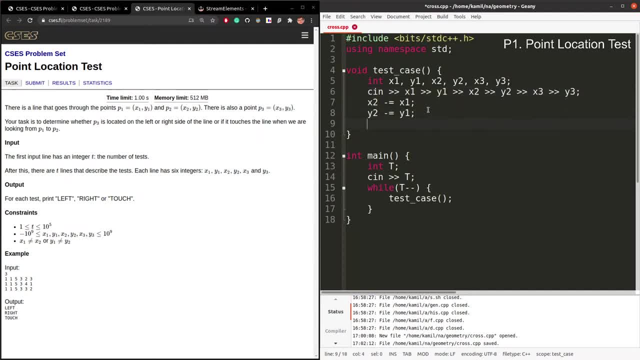 I need to take other coordinates. So one way is to do it like that and Then kind of be done with it. When I, whatever formula I will use, I almost make it made a mistake: Y free minus equal y right. and now Those two coordinates of p2 and p3 are computed correctly with respect to p1. 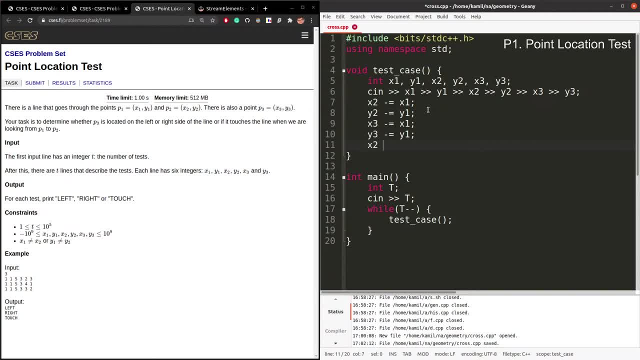 Now the cross product X: x of first point multiplied by y of the other point, minus the other way around. If this is negative- we already saw that- then the first point is more to the left. What do we need to check? If we need to check whether p3 is located on the left side, 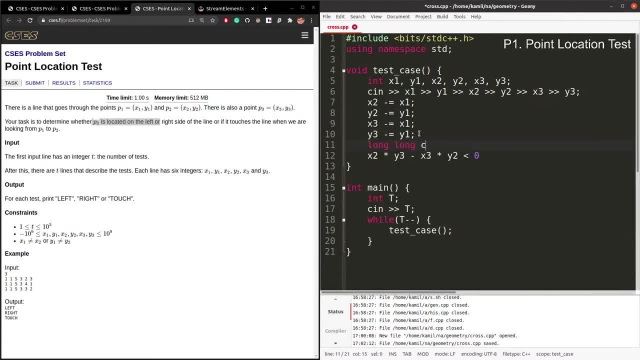 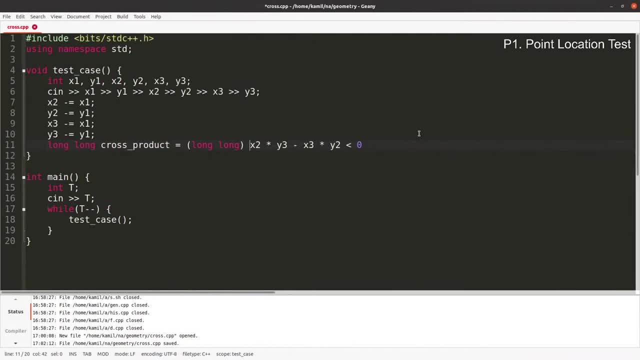 I will use. maybe Let's use a cross product And Be careful with overflows here, Because I created ints. They will not hold product if cross product Smaller than zero, then we saw case. this means that p2 on the left from p3. But what we need to print is what's the location of p3 with respect to line p1, p2. 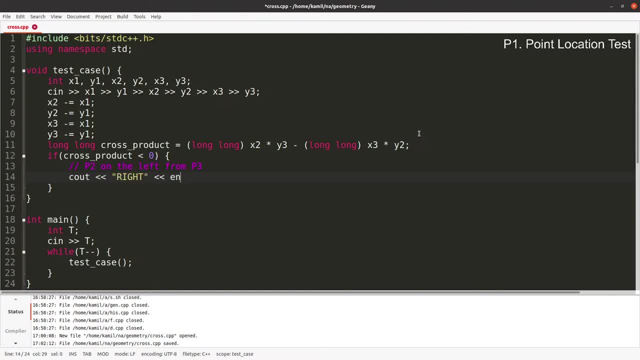 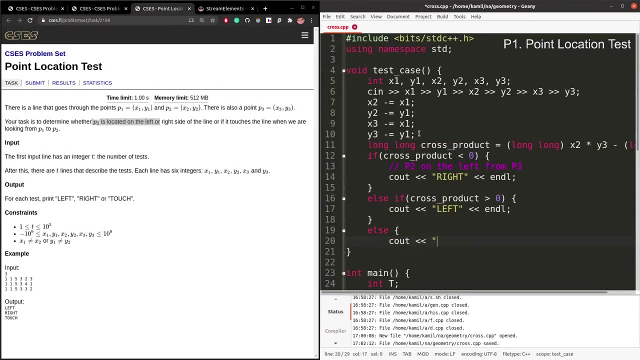 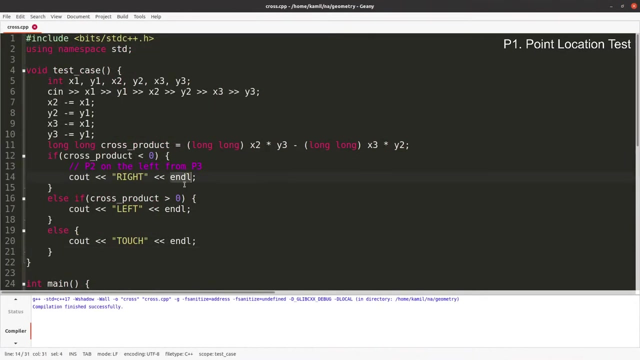 In this case we say right, because p3 is on the right, Symmetrically the other case. and Finally, cross product is 0. what do we need to print? touch One more thing in c++. ENDL always flushes the output and it is quite slow. 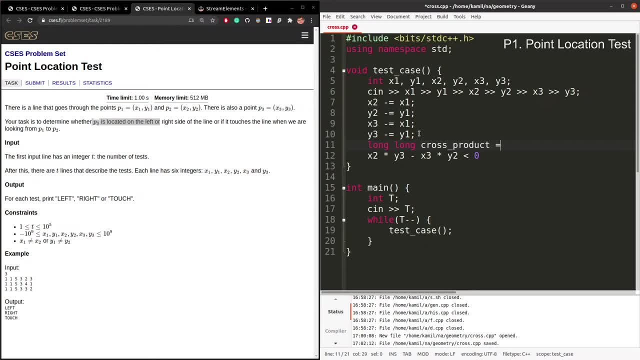 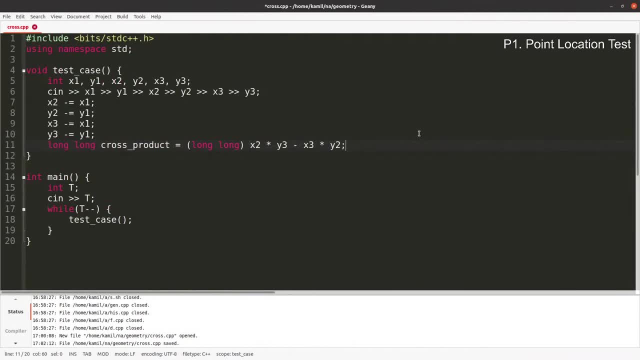 p3. let's use a cross product and be careful with overflows here, because I created ints. they will not hold product if cross product smaller than zero, then we saw case. this means that p2 on the left from p3. but what we need to print is what's the location of p3 with respect to line p1, p2. 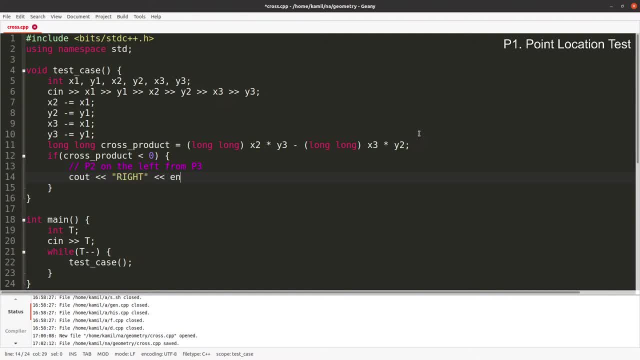 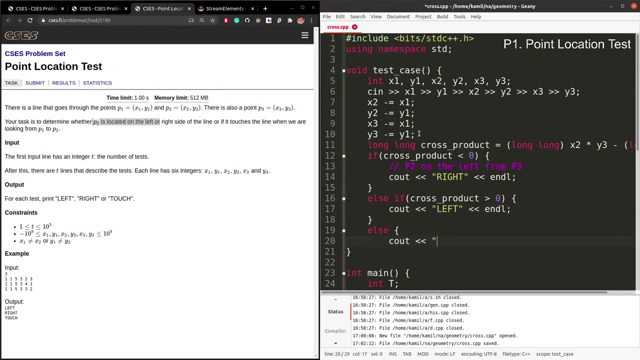 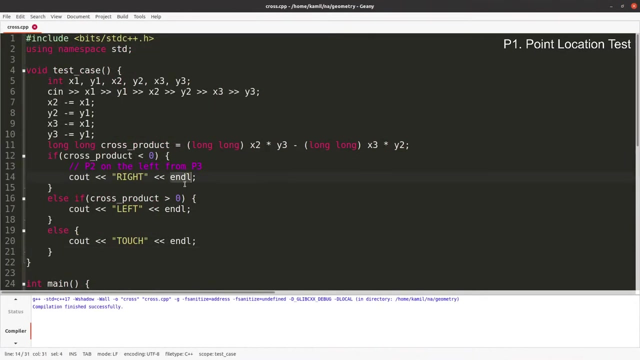 in this case we say right, because p3 is on the right, symmetrically the other case. and finally, cross product is zero. wat do we need to print? touch? one more thing: in c++, ENDL always flashes the output and it is quite slow. I don't know if it would be an issue in this problem, but 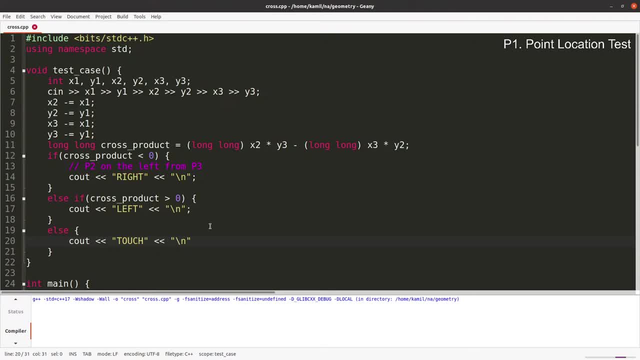 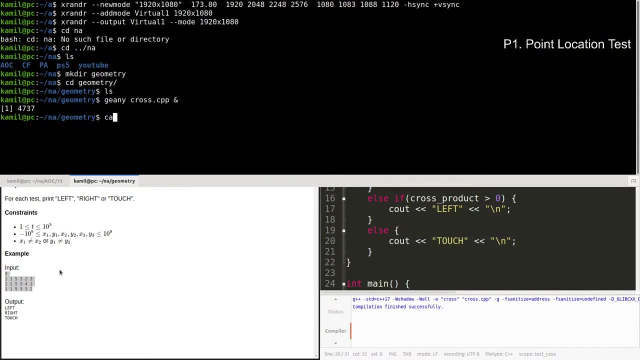 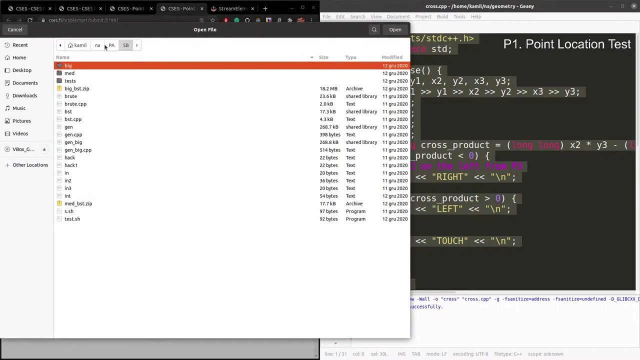 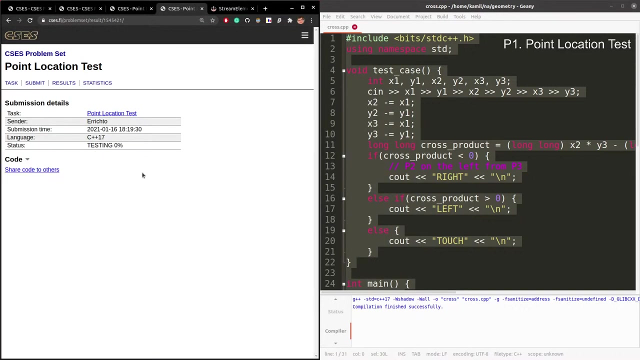 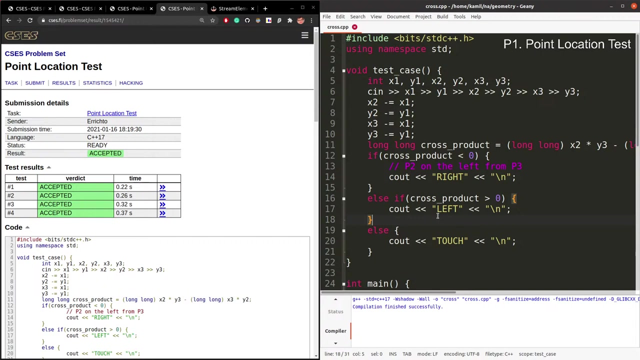 it's better, in general, to use this. This is new line without a flash. All right, let's test. Fingers crossed, Cross run on this file Left-right touch. Cool Works here. This is geometry. Crosscpp Accepted. We can move to the next problem. Oh no, we cannot. I told you that this is a messy. 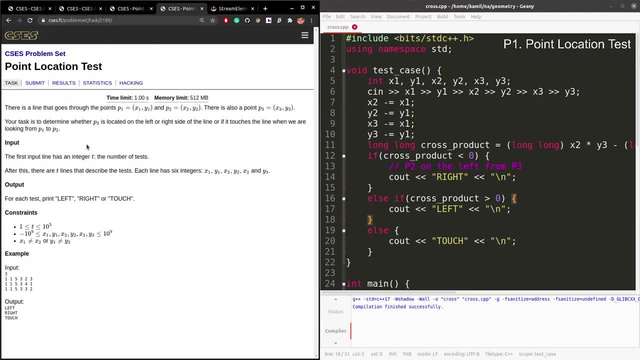 implementation. Before we move to other six problems. let's try to make this code better. It becomes a mess when we deal with more than five problems at once. This is a problem we have to solve. Let's try to make this code better. It becomes a mess when we deal with more than five problems at once. 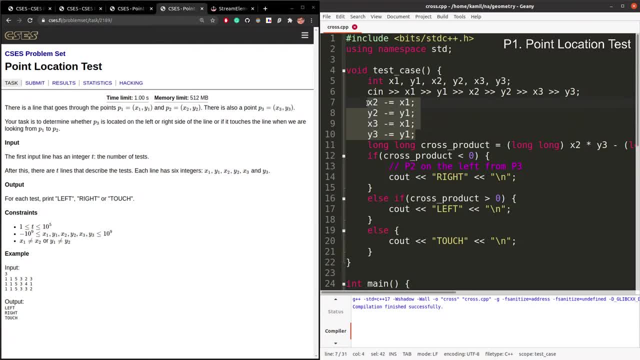 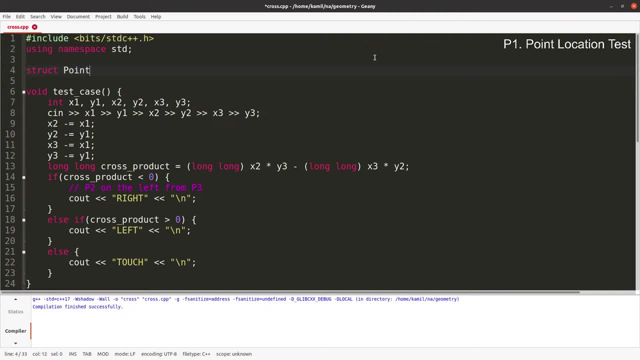 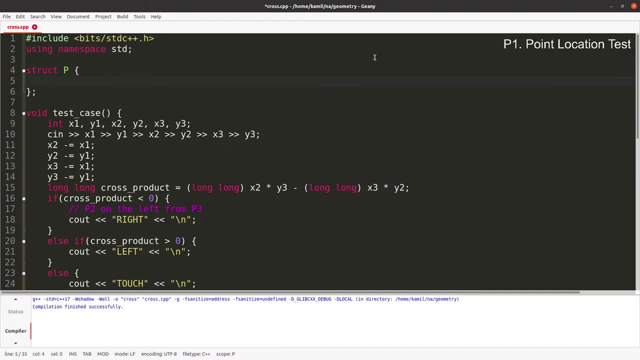 three points already. here it was ugly and it would be very easy for me to make a mistake. let's use a class or actually struct. you don't need anything public. we can call it, some people call it point, I would. I prefer just writing P. let's go. 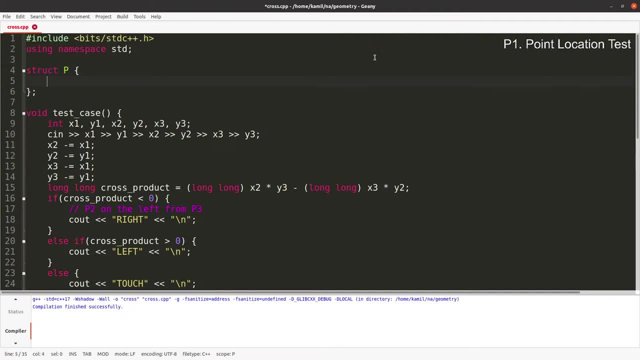 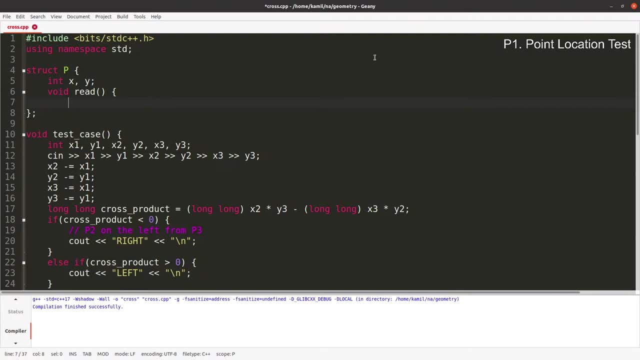 with my method, but you can call it point if you want to type more. it has just two attributes, x and y, and I will create a function so it would be able to read. and how will the code change? I want to say that there are three points, each of them. 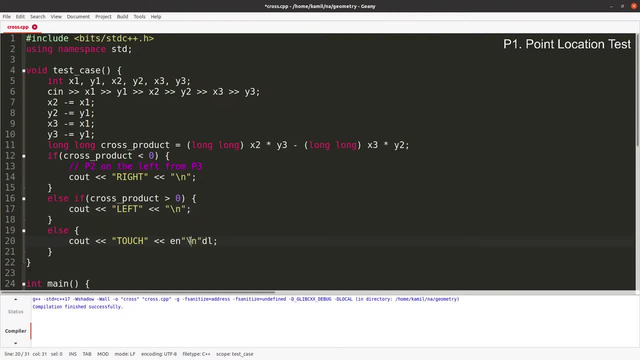 I don't know if that American technique is correct or not. I will try to use one, but I don't think so. I hope that it's true. know if it would be an issue in this problem, but it's better in general to use this. this is: 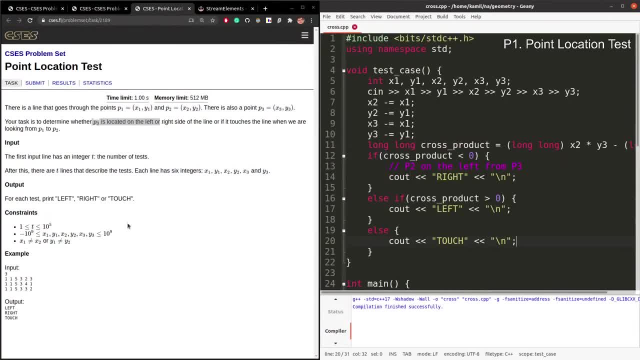 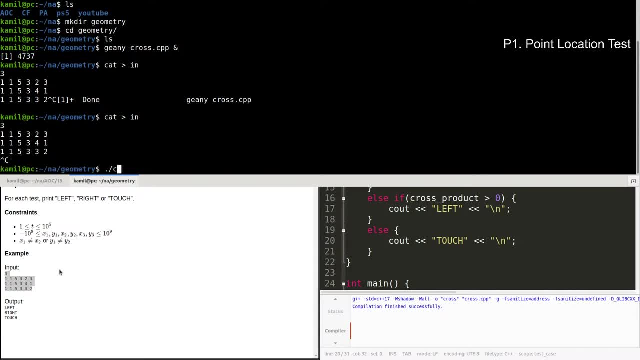 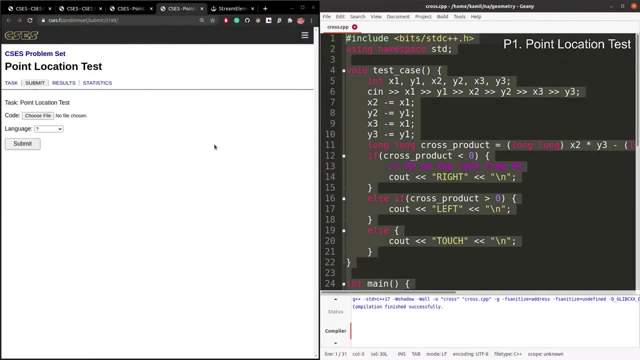 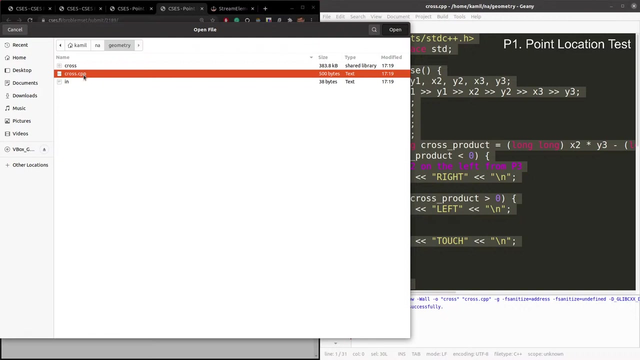 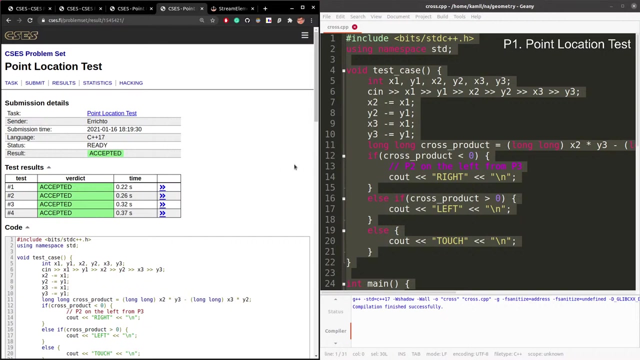 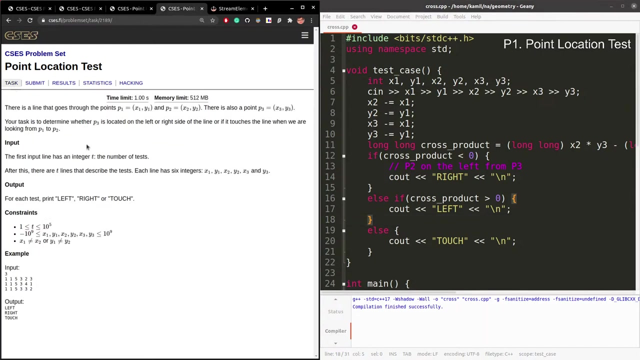 new line without a flash. all right, let's test. fingers crossed, cross, run on this file left, right, touch. cool works here. this is geometry crosscpp. accept that we can move to the next problem? oh no, we cannot. i told you that this is a messy implementation. before we move to other six problems, let's try to make this code better. 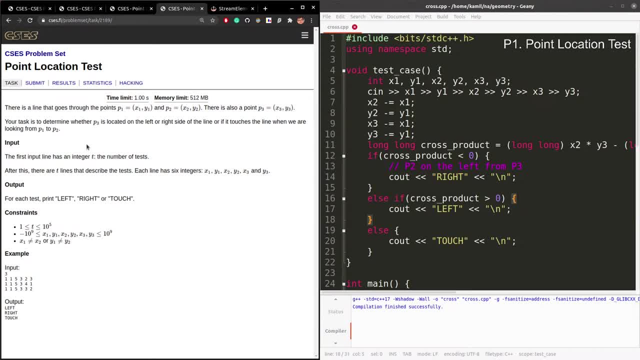 it becomes a mess when we deal with more than four problems. so let's try to make this code better now, and in our case, here it's a mess so we can create a new one. so we will just set it to three, three points. already here it was ugly and it would be very easy for me to make a mistake. 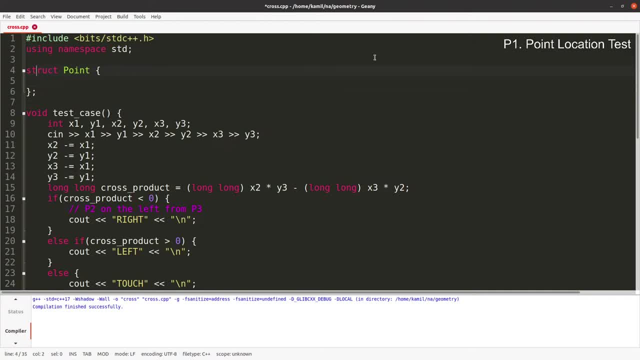 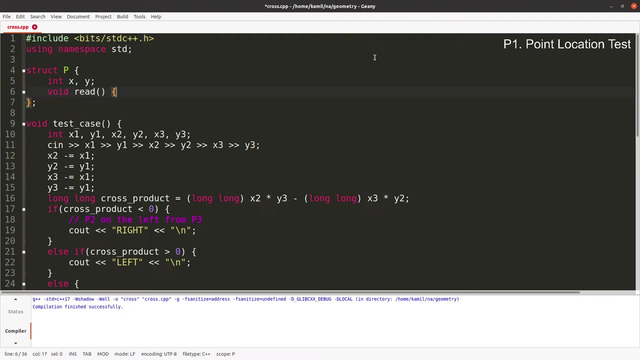 let's use a class or actually struct. you don't need anything public. some people call it point. i would i prefer just writing p. let's go with my method, but you can call it point if you want to type more. it has just two attributes, x and y. 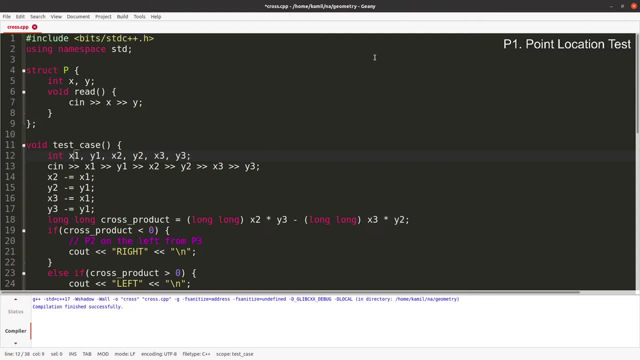 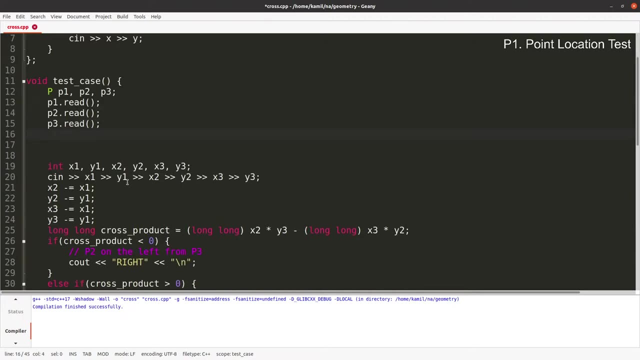 and i will create a function so it would be able to read: it has just two attributes, x and y, and how will the code change? I want to say that there are three points. each of them needs to read from the input. you could also read in constructor: and now: 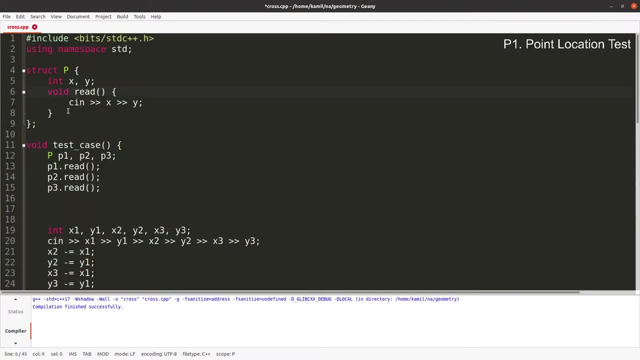 some trickier C++ stuff. when implementing something, you can do this: this would be equivalent to what we did previously, and so on. that that's fine, but even better not to repeat that and make sure that you use proper coordinates everywhere. you can create a function here, and in C++ you can make it into an. 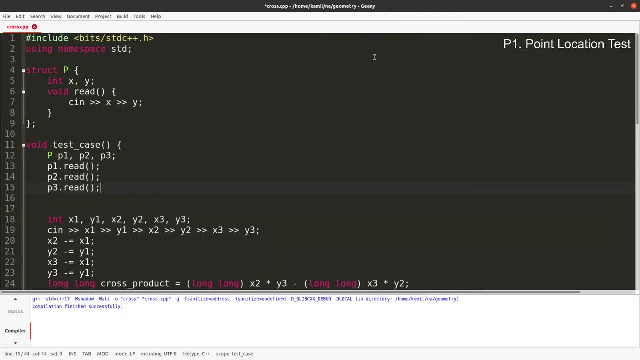 needs to read from the input. you could also read in constructor. and now some trickier C++ stuff. when implementing something, you can do this: this would be equivalent to what we did previously, and so on. that that's fine, but even better not to repeat that and make sure that you use. 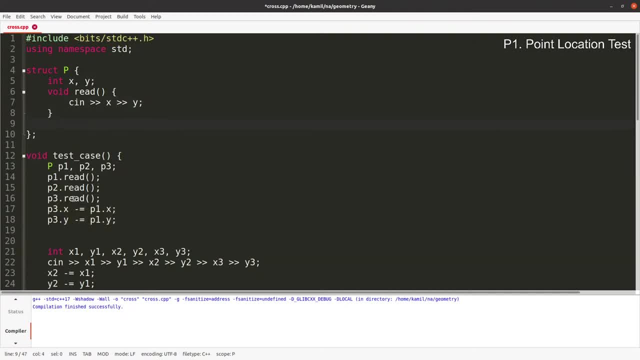 proper coordinates everywhere. you can create a function here and in C++ you can make it into an operator like minus, to subtract two points. one thing is this: this creates operator minus. this is name of a function and it returns minus, like other points. name of other point. return x minus b dot x, x minus b dot x and y minus b dot y. 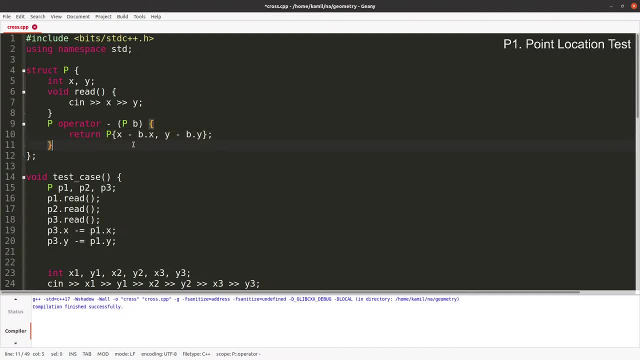 this is a default constructor, so it returns a point like: if you run something like this point with coordinates five, three, minus point with coordinates two, two, you want to get a point with coordinates three comma one, subtract corresponding coordinates. this is what happens there in operator minus. this allows us, after you type that, to do this. 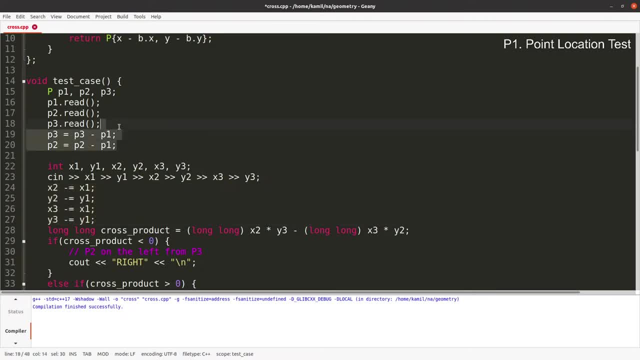 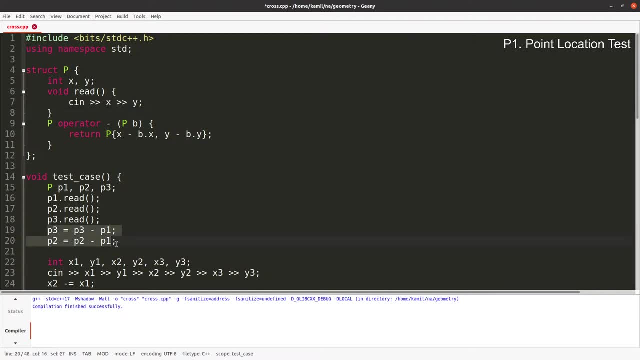 so much better than that, especially in the long run, especially if you always i just copy paste this thing when i deal with geometry problems and then i can simply type that even better. you can also- let's make it void. you can also say: minus equal, what it does. 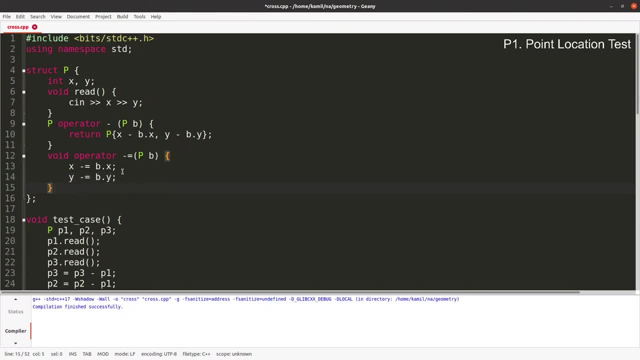 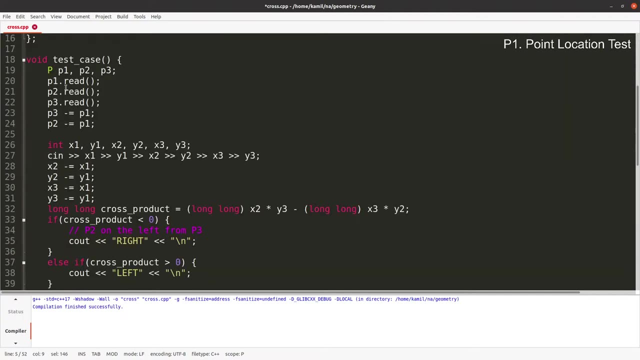 you can do it like that. you could always. you could also here use this function doesn't matter too much, and then you can do that even short. it's nice to do something once, to then speed up your work many, many times, and you can do this even the 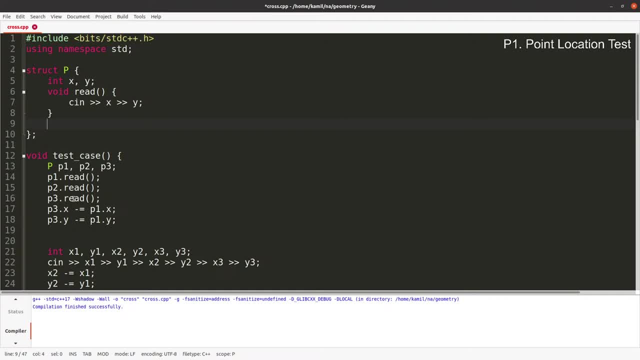 operator like minus to subtract two points. one thing is this: this creates operator minused. this is an operator that creates a function to subtract with this name of a function and it returns minus, like other points. name of other point. return x minus b dot x, x minus b dot x and y minus b dot y. this is a default constructor, so it returns a point. 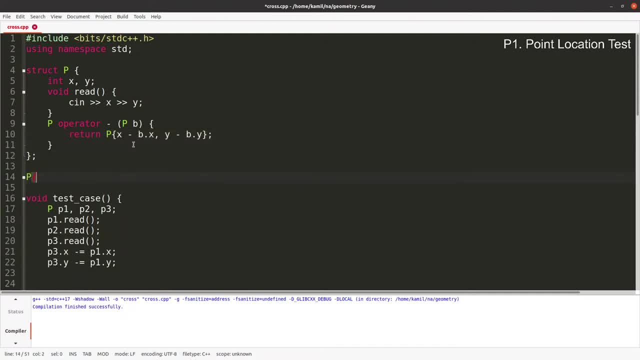 like, if you run something like this: point with coordinates five, three, minus, point with coordinates two, two, you want to get point with coordinates three, comma one, subtract corresponding coordinates. this is what happens there in operator minus. this allows us, after you type that, to do this so much better than that, especially in the long run, especially if you always. 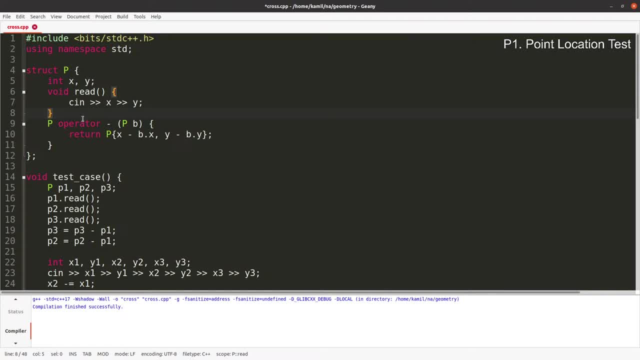 i just copy paste this thing when i deal with geometry problems, and then i can immediately type that. even better, you can also- let's make it void. you can also say: minus equal what it does. you can do it like that. you could always. you could also here use this. 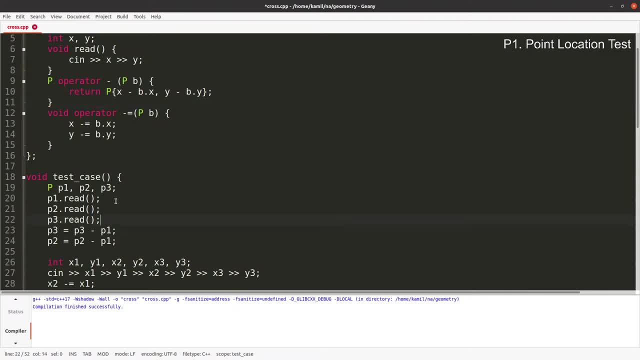 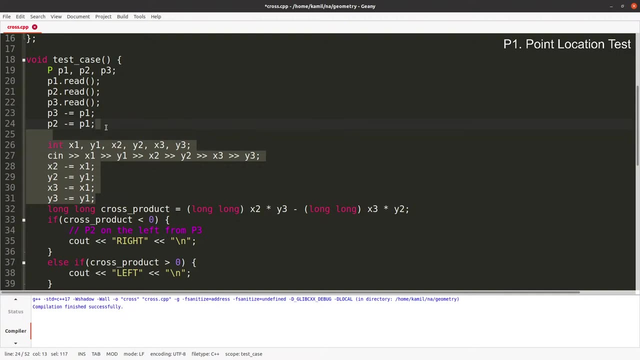 function doesn't matter too much, and then you can do that, even short. it's nice to do something once to then speed up your work many, many times. finally, cross product. sure, we can write p2.x, p3.y and so on. it will work, it will compile. 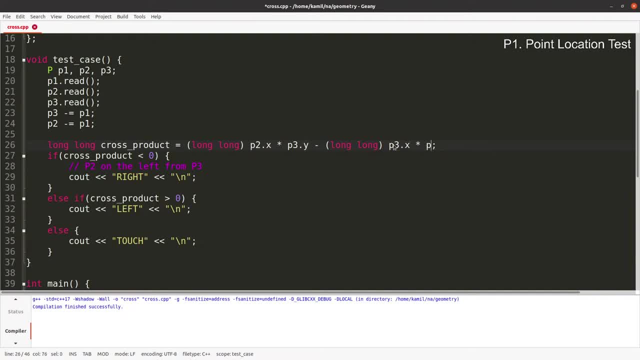 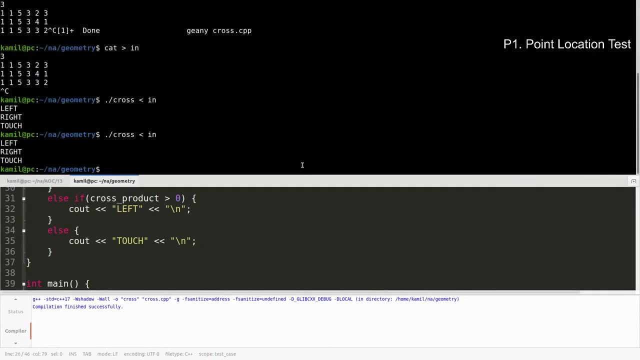 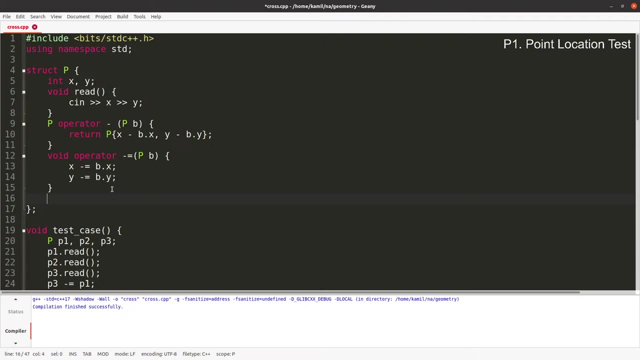 actually let me finish, because just a few characters away this compiled gives still the same answer, but i usually overwrite multiplication operator and then you can do it in other ways. so for example, let's say you want to do a star to return cross product. it returns long, long. 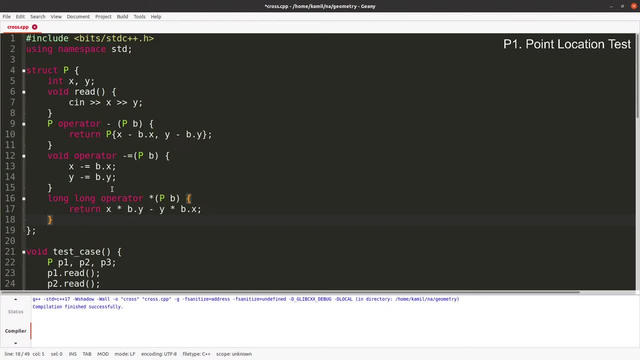 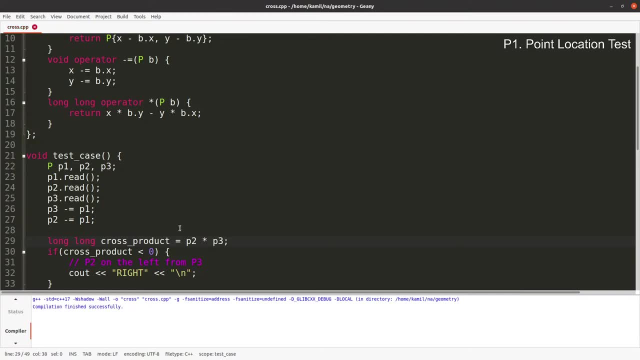 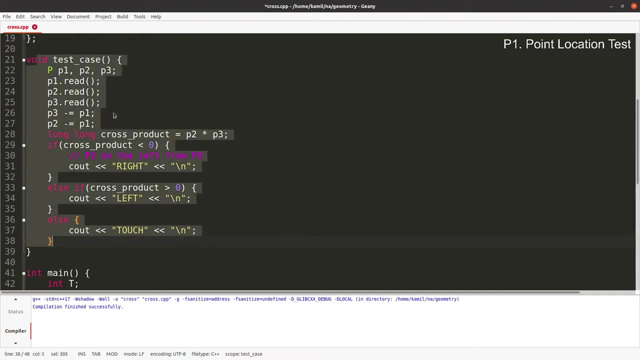 and it does x times b, dot, y minus the other way around. all of that is simplified to this very short line and usually when we deal with a geometry problem, you will just implement that. you will not care exactly like how to subtract, but you will know how to compute a cross product. 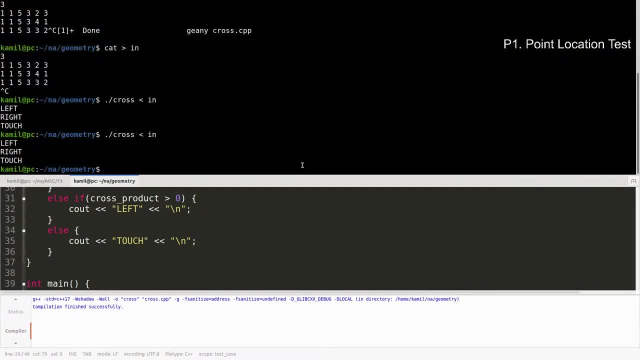 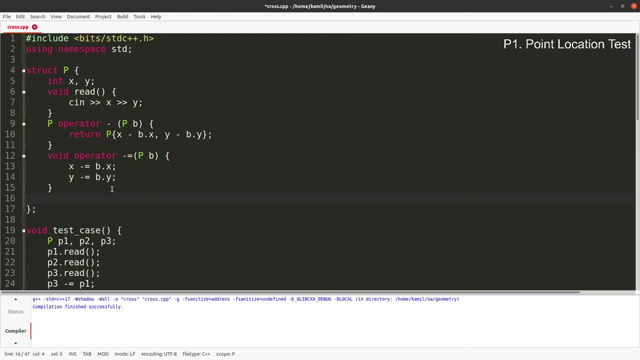 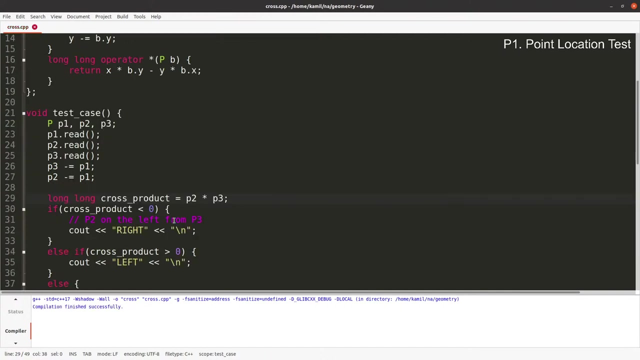 same way. so so you can do this for to return cross product. It returns long, long and it does x times b dot, y minus the other way around. All of that is simplified to this very short line, And usually when we deal with a geometry problem, 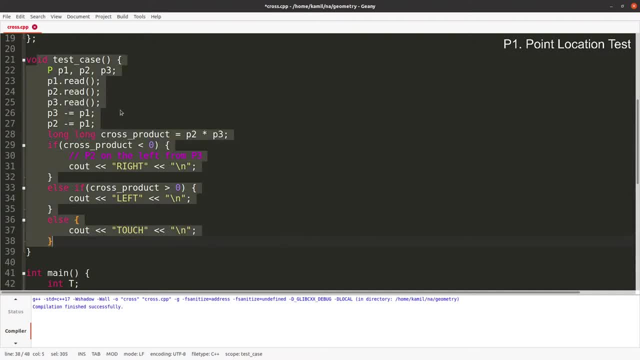 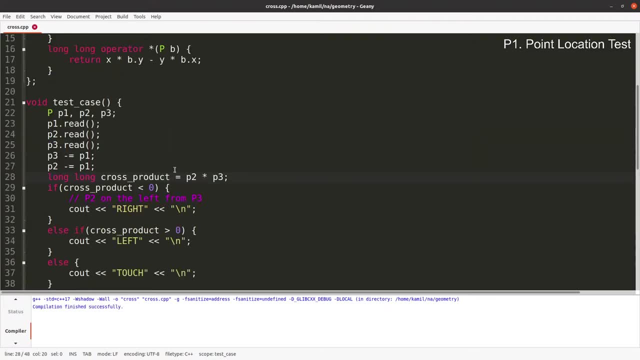 you will just implement that. You will not care exactly like how to subtract, how to compute a cross product. Compile again, it works. One last thing, but this is just in C++. If you are Python user, don't worry about it. All of that is slightly faster if you use a reference. 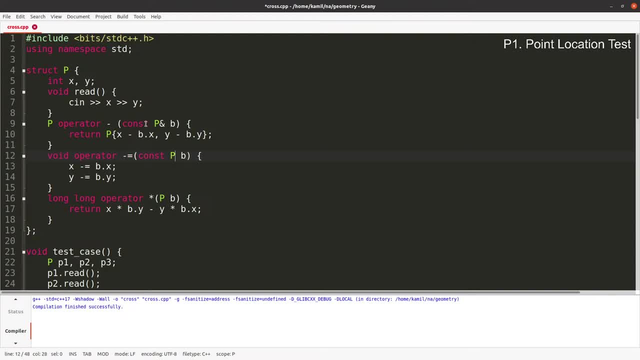 and for safety, use const as well. You don't want to copy the value And some detail, but this is just nice implementation. Put const here as well to tell compiler that you don't want to modify your own value. And now, after that, this is how I implement it, Without all those const references, as you saw. 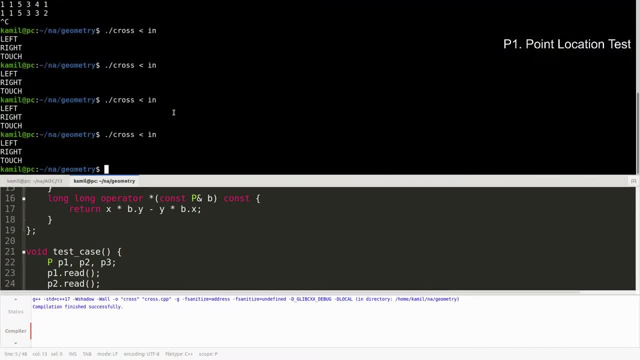 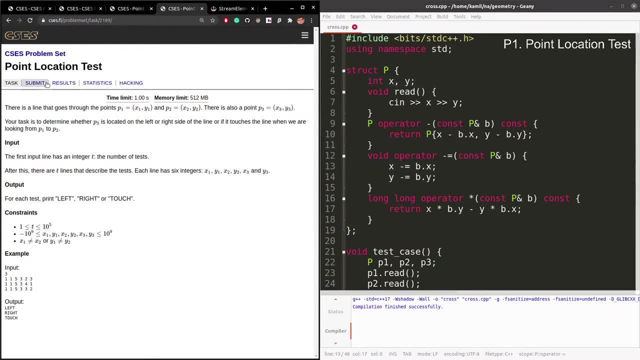 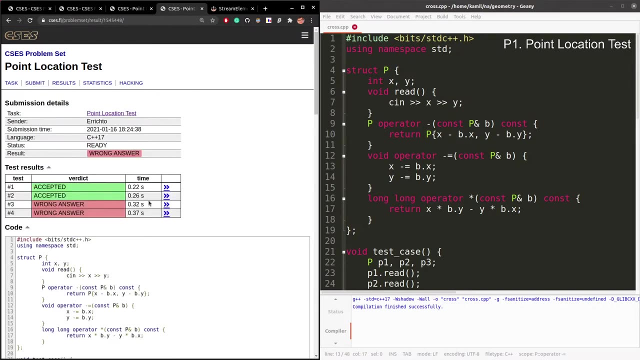 everything compiled. It gave correct answer on the sample test. Just, this is a bit better way to code and it's a bit faster with references. I will submit again just to make sure that everything is fine. Then we move on to the second problem. 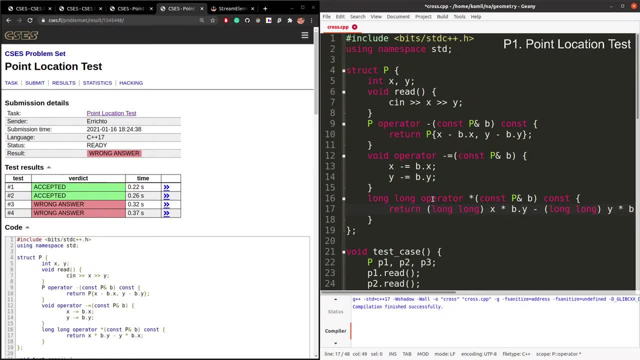 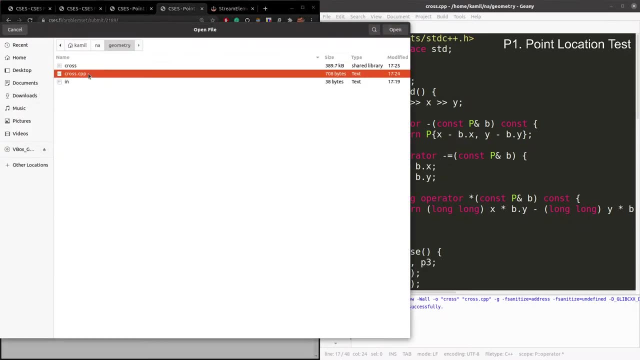 It's safer to make your coordinates just long-long in the first place. Here you can do long-long. I usually just prefer to suffer and use proper types and, whenever needed, use long-long In my defense. normally I don't type this, I copy-paste it. 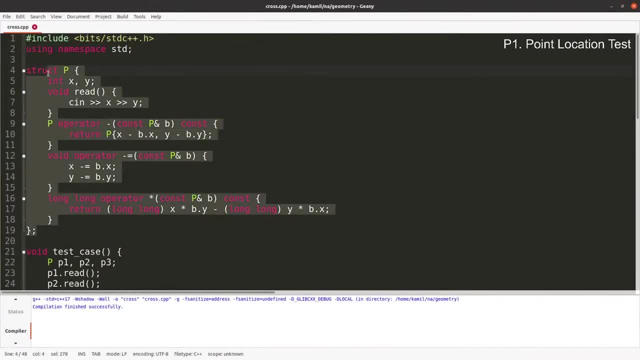 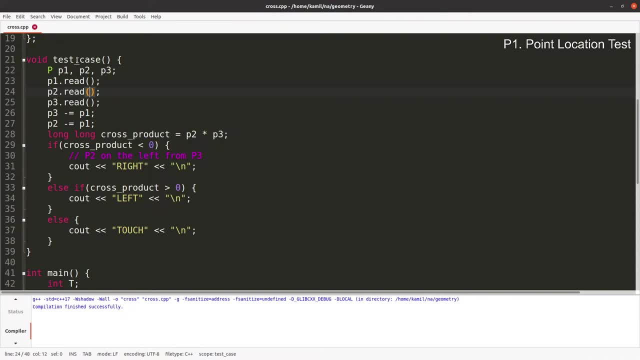 Accepted This. you can call this your geometry template and then everything. here is just very short. This is how you solve geometry problems. Cool, I will answer questions, if there are some. now I don't think it's faster. Point is just two ints. 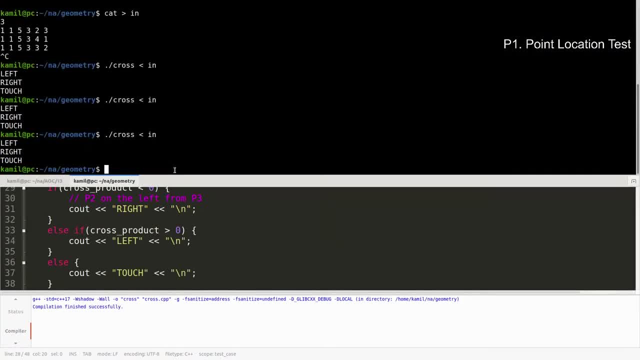 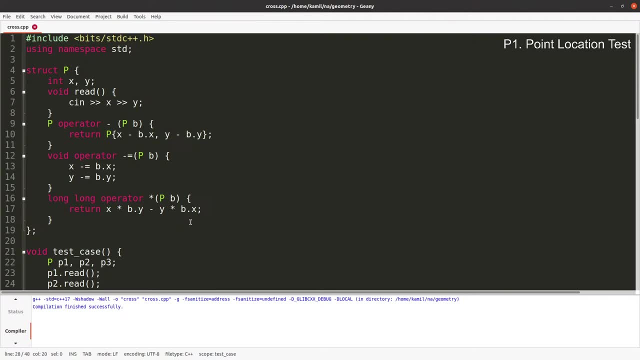 compile again. it works. one last thing, but this is just in c plus plus. if you are python user, don't worry about it. all of that is slightly faster if you use a reference and, for safety, use const as well. you don't want to copy the value. 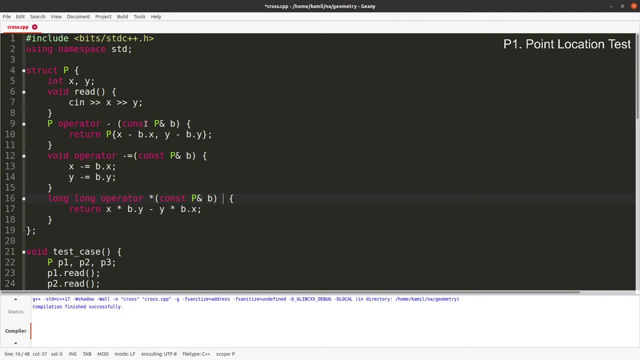 and some detail, but this is just nice implementation. put const here as well, and this is the same thing for the other thing that we didn't have the last one, but let me do it again for this one, and then we'll see what happens next time. we'll see how it works. 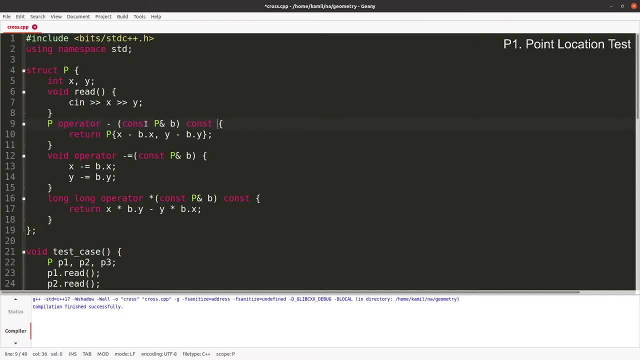 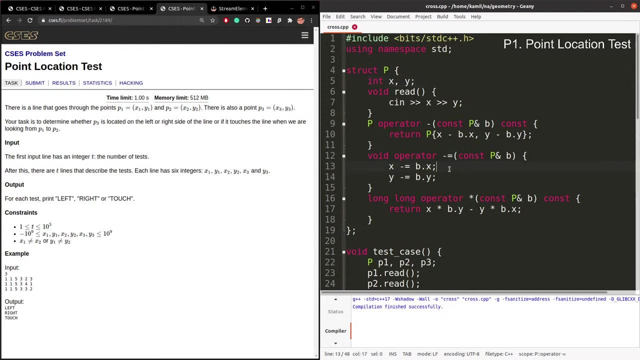 as well, to tell compiler that you don't want to modify your own value. And now, after that, this is how I implement it, Without all those const references. as you saw, everything compiled. it gave correct answer on the sample test. just, this is a bit better way to code and it's a bit faster with references. I will. 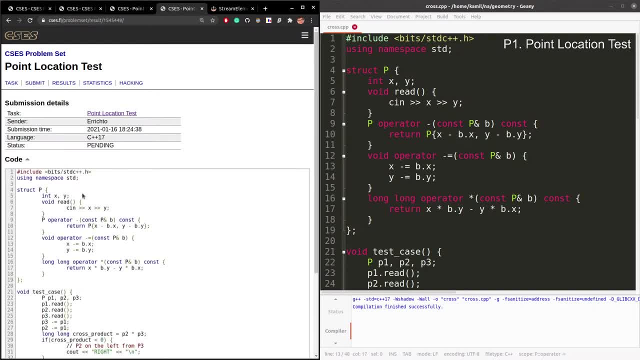 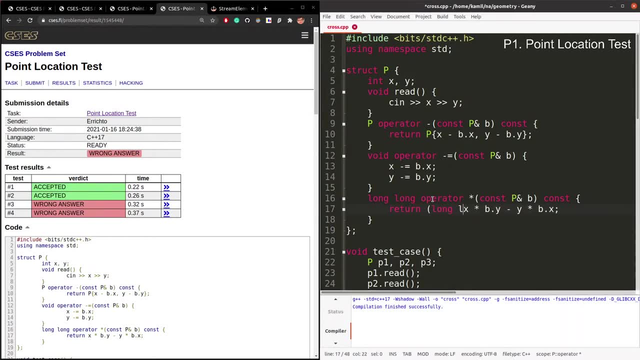 submit again just to make sure that everything's fine. Then we move on to the second problem. It's safer to make your coordinates just long-long in the first place. Here you can do long-long. I usually just prefer to suffer and use proper types and whenever needed use. 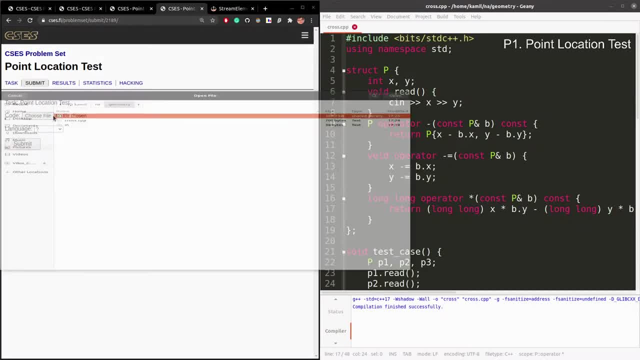 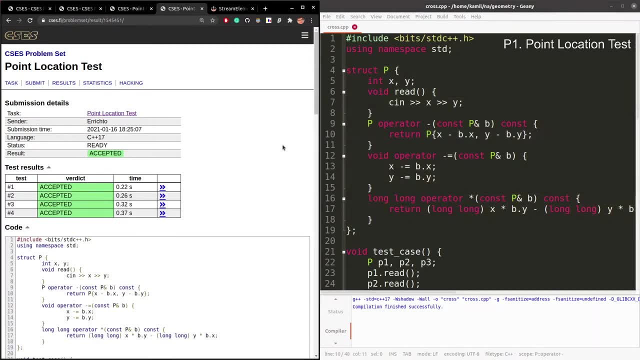 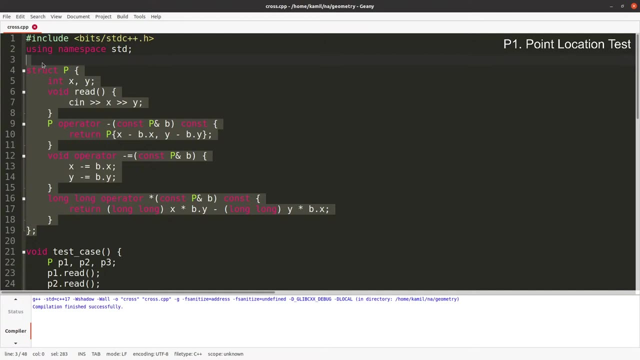 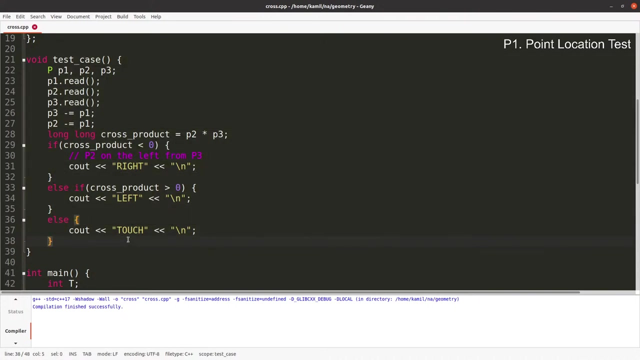 long-long In my defense. normally I don't type this, I copy-paste it. Accepted This. you can call this your geometry template, and then everything here is just very short. This is how you solve geometry problems. Cool, I will. 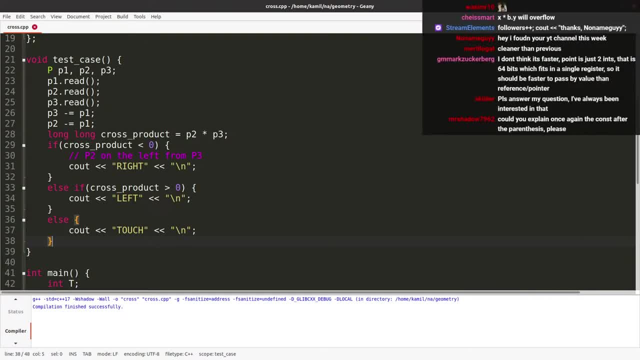 answer questions, if there are some. now, I don't think it's faster, but point is just two ints faster to pass by value than the reference pointer. oh, that's interesting. I would say that in practice I saw speedups coming from passing by reference. but I see what you're saying. maybe indeed, if it's just. 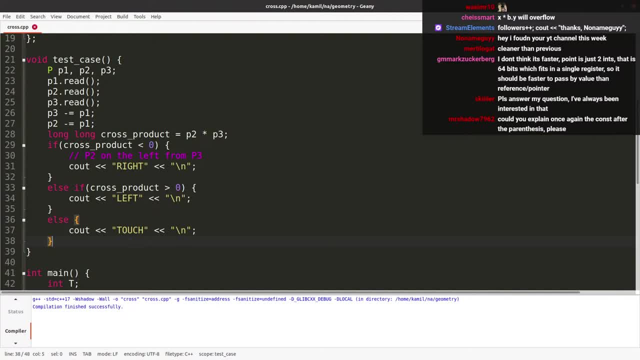 I would say that it would just work if you set that faster to pass by value than the reference pointer. Oh, that's interesting. I would say that in practice I saw speedups coming from passing by reference. But I see what you're saying. Maybe, indeed, if it's just two ints, then it's the same thing. 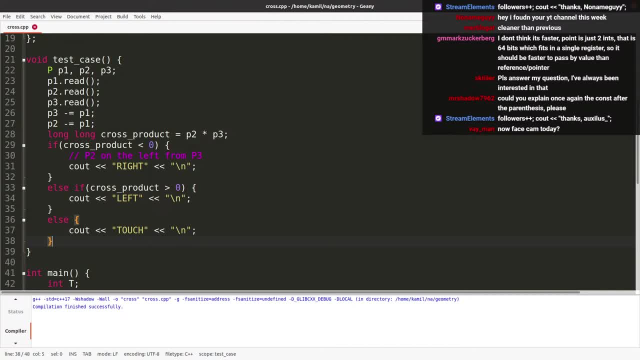 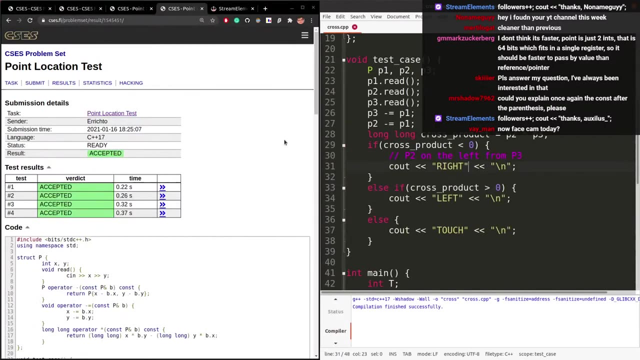 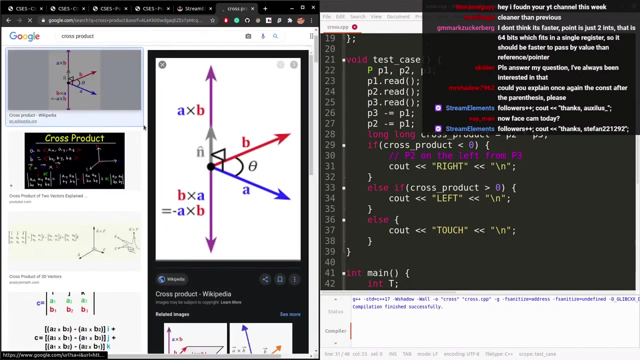 But i'm surprised. But when You know instant we copy them, don't we create two new pointers. Maybe that takes time. Previous question: Isn't cross product result vector? In some languages it is called vector product. All right, I'll answer that. In physics, cross product is really a 3D geometry thing. 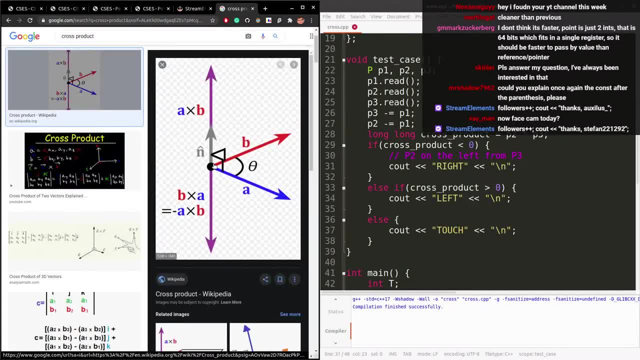 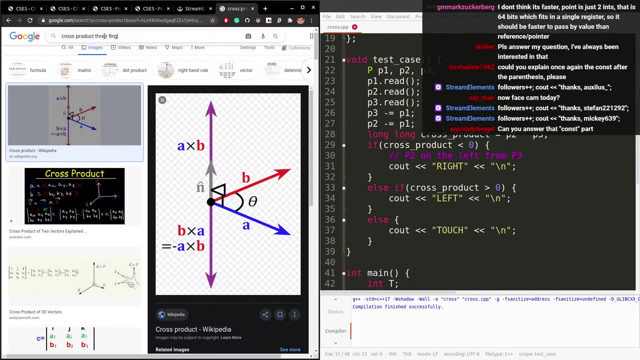 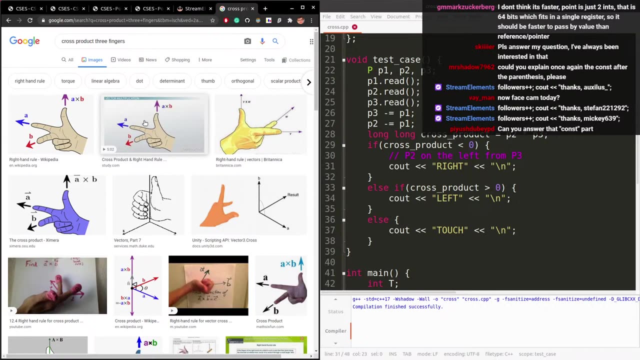 It's this Cross product points up or down, but this up versus down is actually sine, and then we care about the length of that. In physics it is useful to do this and there are like three fingers rule. There is this rule to say what is the sine, but we don't use it in computational geometry. 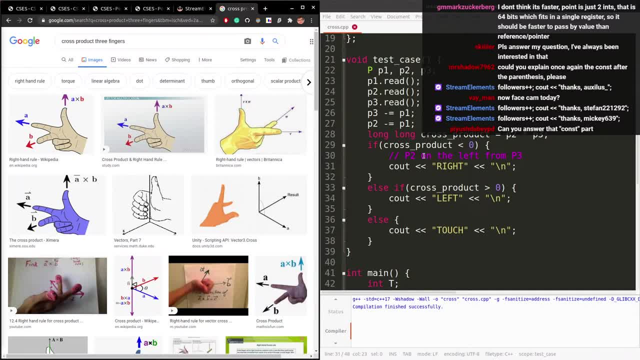 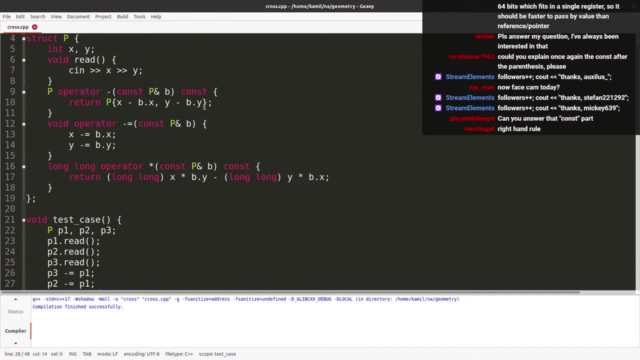 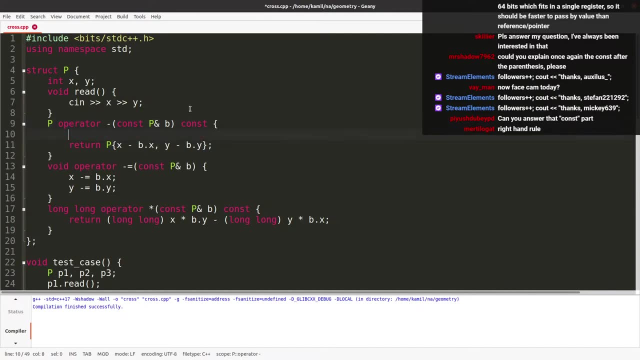 And can you explain once again the const after parentheses? I don't really want to spend time on that because this is C++. It's unrelated to geometry. Const says that me, I'm constant. If you type this, you will get compilation error. 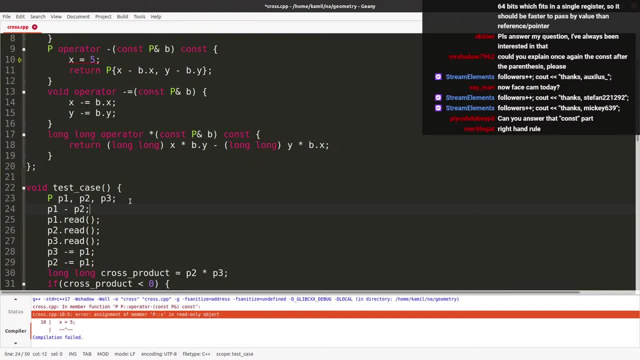 When I write p1 minus p2, this actually on function p1, it runs function. sorry, on struct p1 it runs minus. And this line would try to modify p1.x. but I'm saying: no, I'm constant, just like he is, So constant. this const refers to b. 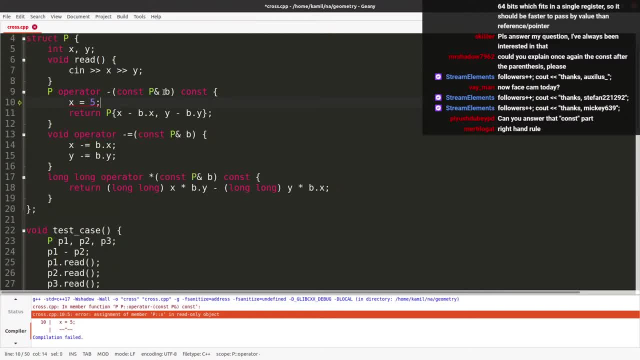 this const refers to me, Because this is function that I p1, run and I get p2 as argument. I will not spend more time on this, though You can read more about it online, I'm sure Right hand rule maybe- I don't know how it's called in your country. 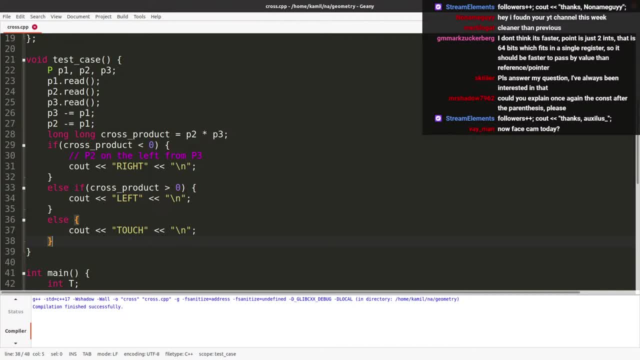 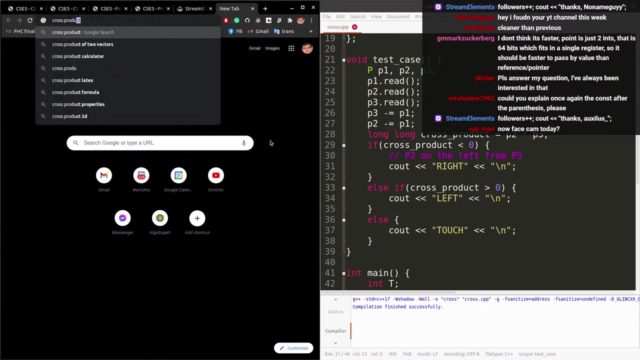 two ints, then it's the same thing. but I'm surprised. but when you know, when we pass two ints and we copy them, don't we create two new pointers. maybe that takes time. previous question: isn't cross product result vector? in some languages it is called vector product. right answer that in physics cross product is really. 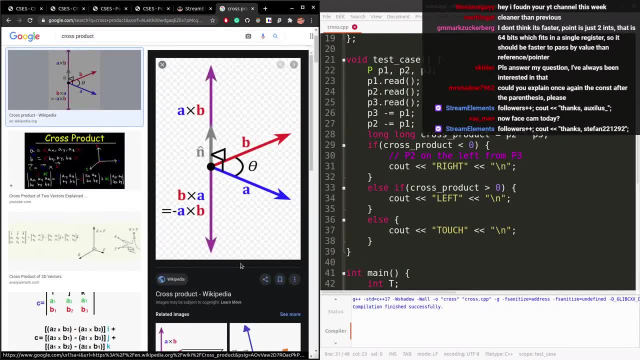 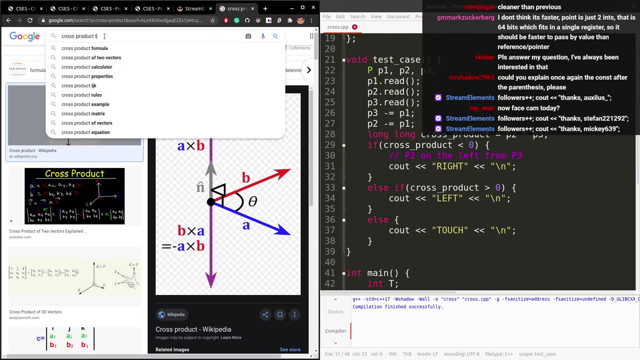 a 3D geometry thing. it's this Cross product points up or down. but this up versus down is actually sine, and then we care about the length of that. In physics it is useful to do this and there are like three fingers rule. There is this rule to say what is the sine. but 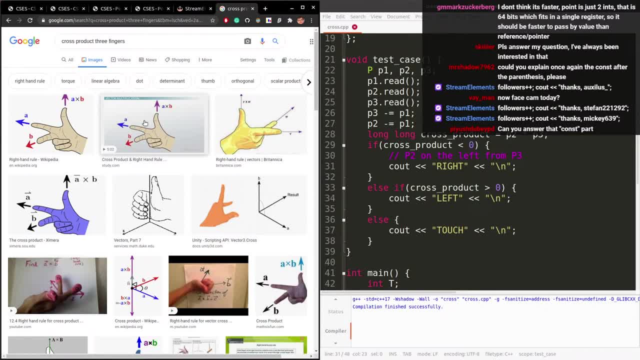 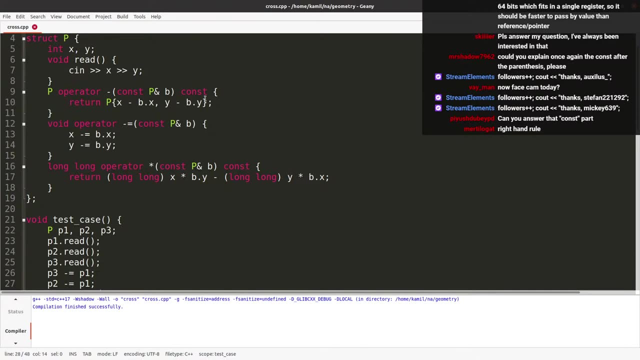 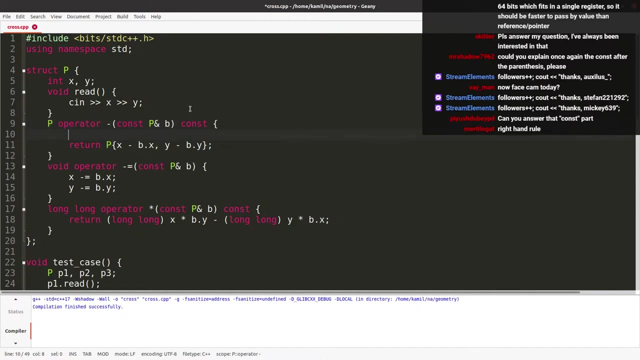 we don't use it in computational geometry. Can you explain once again the const after parenthesis? I don't really want to spend time on that because this is C++. It's unrelated to geometry. Const says that me, I'm constant. If you type this, you will get compilation error When I 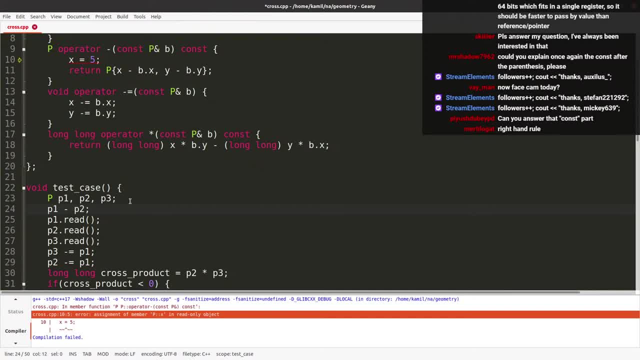 read the code, it says that I'm constant. In this case I'm constant. If you type this, you will get compilation error. When I read the code, it write p1 minus p2. this actually on function: p1- it runs function. sorry, on struct: p1- it runs minus. 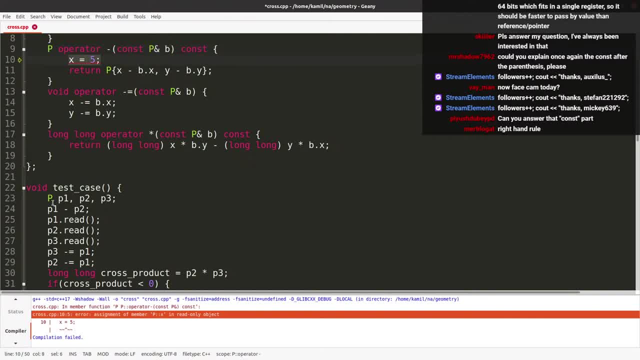 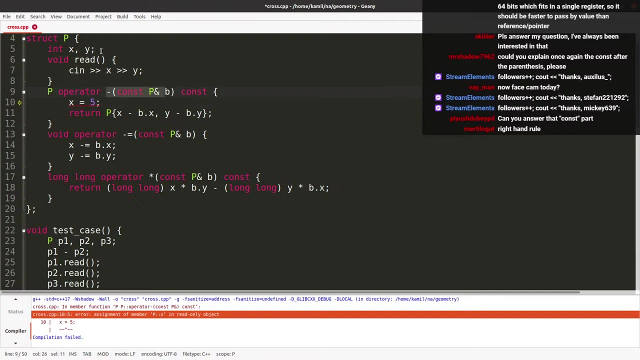 and this line would try to modify p1.x, but I'm saying no, I'm constant, just like he is so constant. this const refers to b. this const refers to me. okay, because this is function that I p1 run and I get p2as argument. I will not. 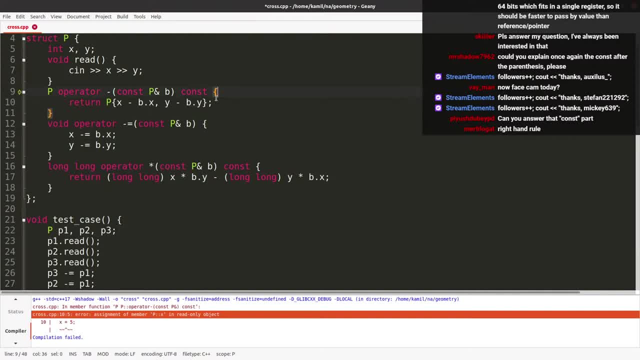 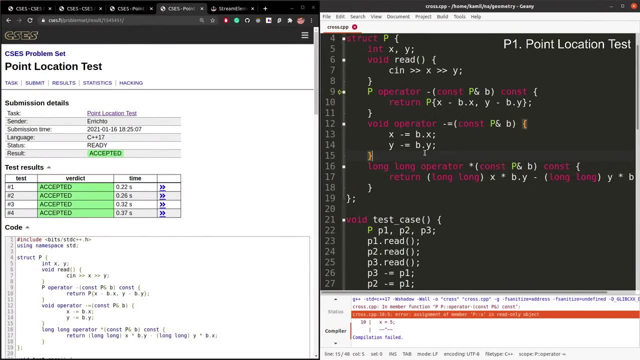 spend more time on this, though you can read more about it online, I'm sure. right hand rule maybe- I don't know how it's called in your country. fine, we move on. is it still compiling? it does? yes, yes, let's see. let's see if it works. 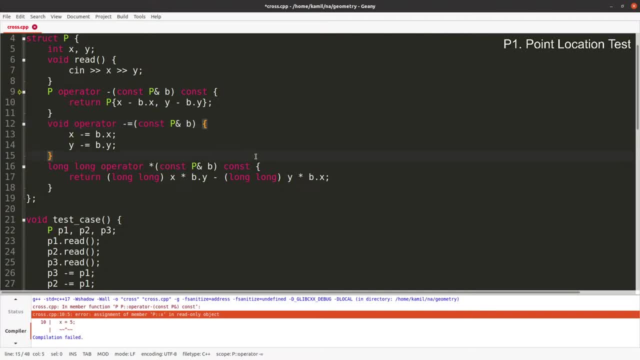 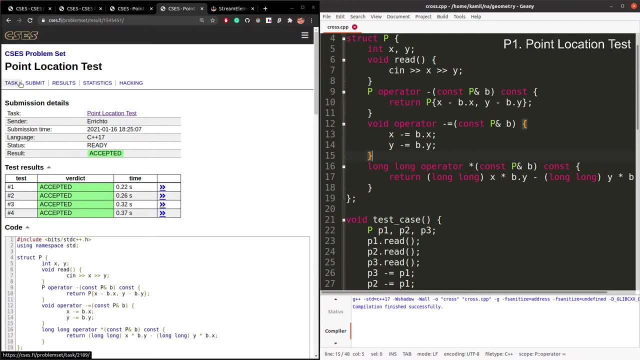 Fine, we move on. Is it still compiling? It does Yes, no facecam today. Would it too messy to compute the line equation? I mean you can, but then you don't want to deal with real values. That's an important thing. 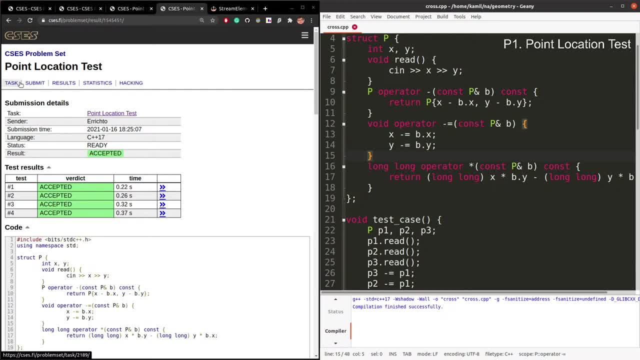 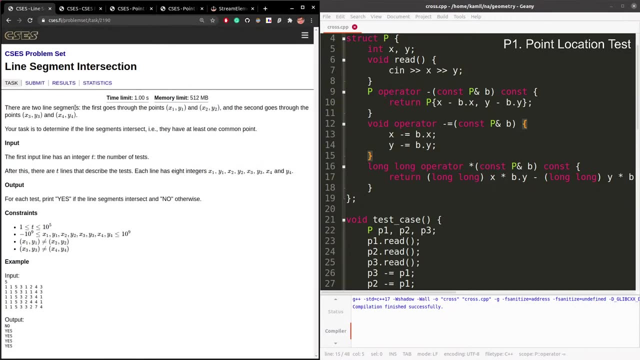 facecam today. Would it too messy to compute the line equation? I mean you can, but then you don't want to deal with real values. That's an important thing. Then we move here When you deal with non-small values once you start using real values. 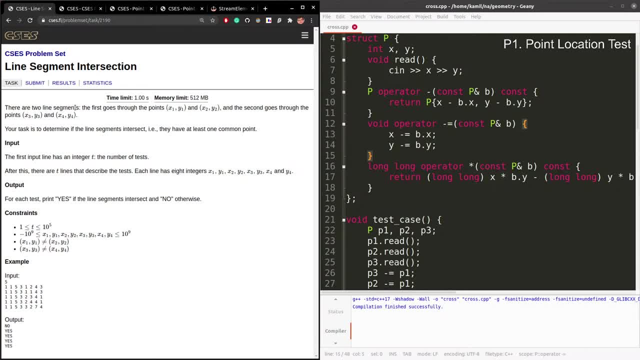 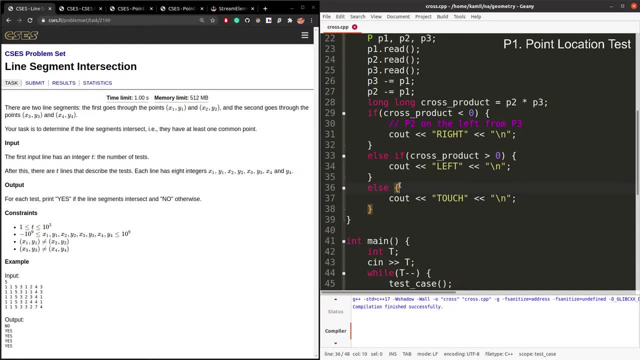 you will get precision errors and you cannot that easily compare stuff Like equality. checking if something is zero on real values is a pain. Like what if it's epsilon? No, you want to use integers whenever possible. Second problem is called line segment intersection. 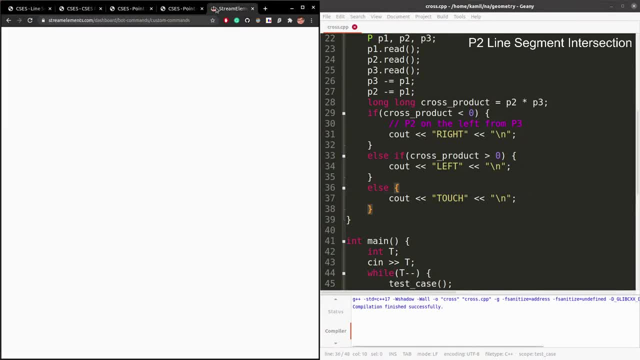 What do we need to do? And that's a new link. Cannot we view in something less than 1080p? Yes, you can go to YouTube. I'm streaming there at the same time and you can adjust the resolution over there. Link is now in Twitch chat. 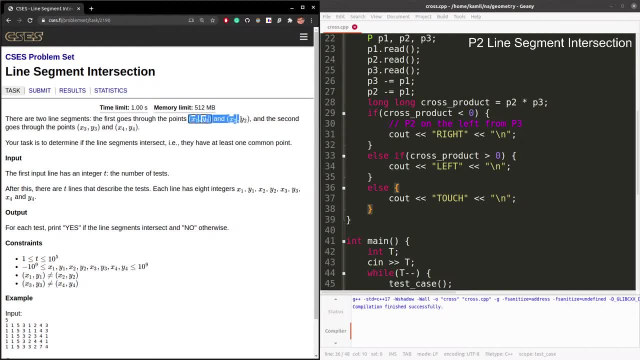 There are two line segments. The first goes through points x, y, points one and two. The second goes through points three and four. Determine if the line segments intersect, That is, they have at least one common point. When you don't know how to approach this, you will have so many ifs. 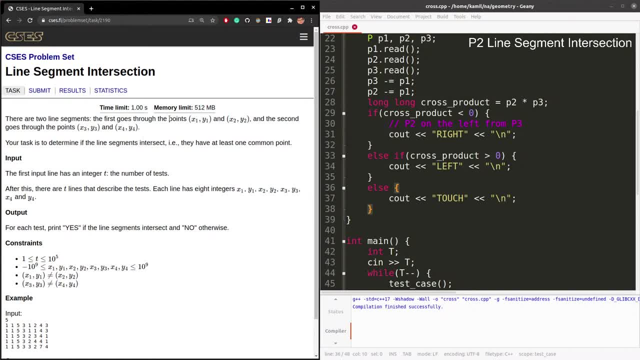 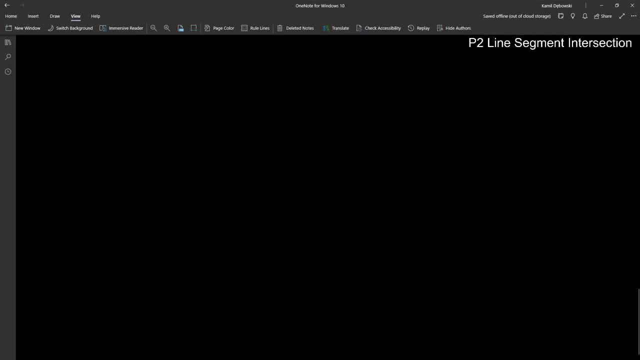 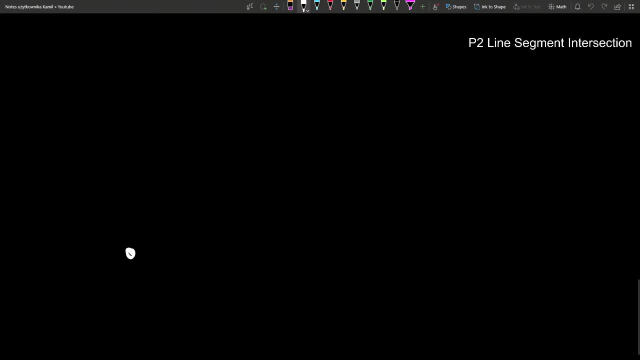 in this problem and so many issues with like parallel segments and so on, Let's, let's do it drunk: CYCLE, CYCLE, CYCLE, CYCLE. Of course, I know a song called solution, so I know a good explanation, but I don't claim that I would think. 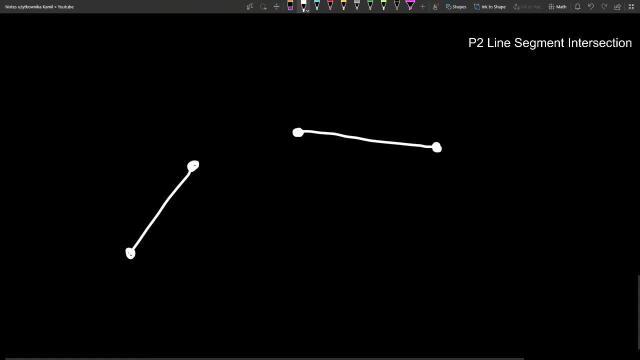 about it this way: when I start Two segments, even if they don't intersect most of the time, when you draw extension of them into a line, the two lines intersect unless segments were parallel. If two segments aren't parallel, then the two lines intersect somewhere. In this case, the intersection point is here. 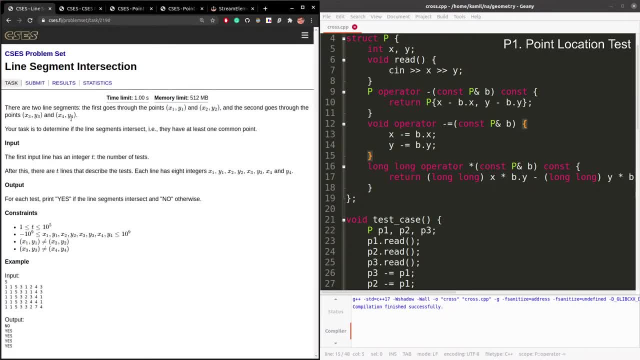 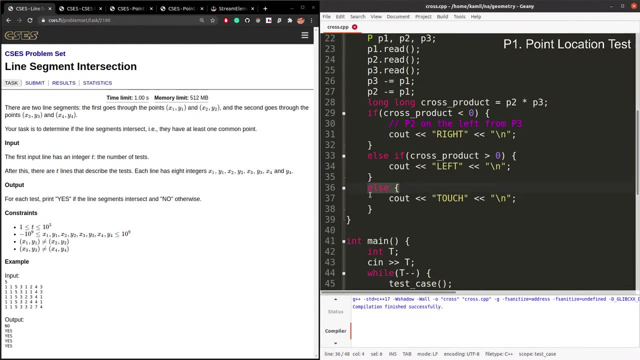 Now we move here When you deal with non-small values. once you start using real values, you will get precision errors and you cannot that easily compare stuff Like equality checking. if something is zero on real values is a pain Like what if it's epsilon? No, you want to do. you want to use integers whenever possible. 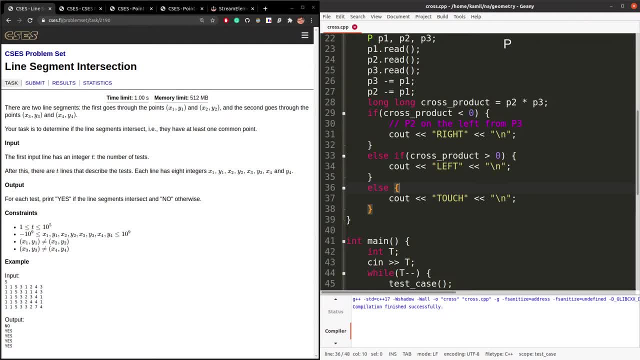 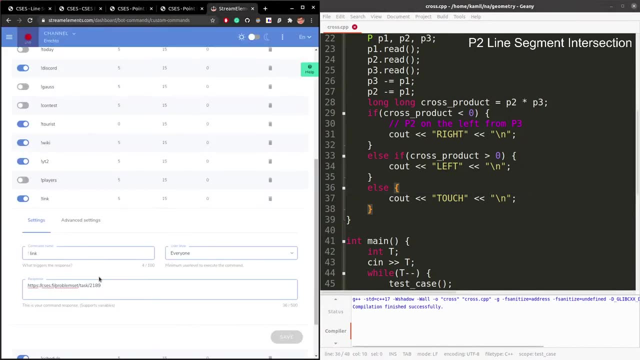 Second problem is called line-segment-intersection. What do we need to do? And that's a new link, Cannot we view in something less than 1080p? Yes, you can go to YouTube. I'm streaming there at the same time and you can adjust the resolution over there. 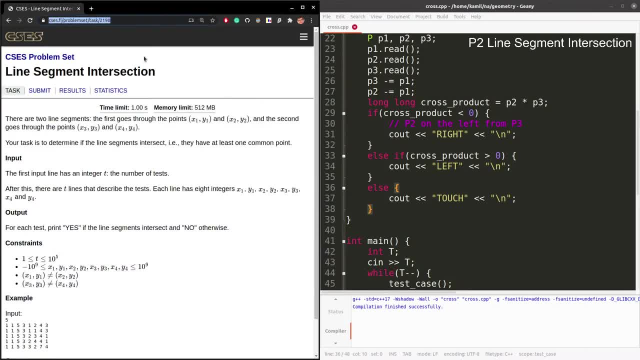 Link is now in Twitch chat. There are two line segments. The first goes through points x, y, points one and two. The second goes through points three and four. Determine if the line segments intersect, That is, they have at least one common point. 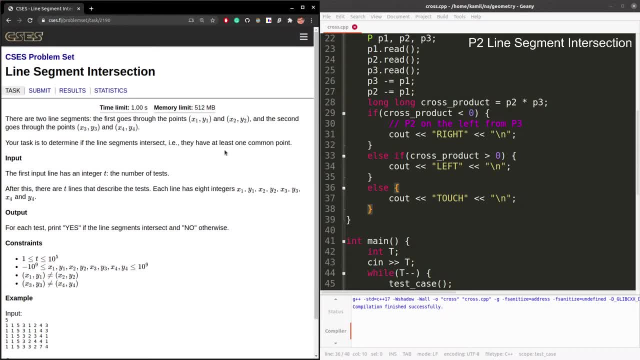 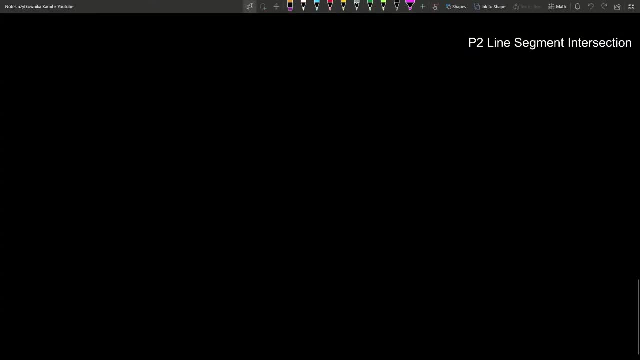 When you don't know how to approach this, you will have so many ifs in this problem and so many issues with like parallel segments and so on. Let's, let's do a draw. Of course I know a solution, so I know a good explanation, but 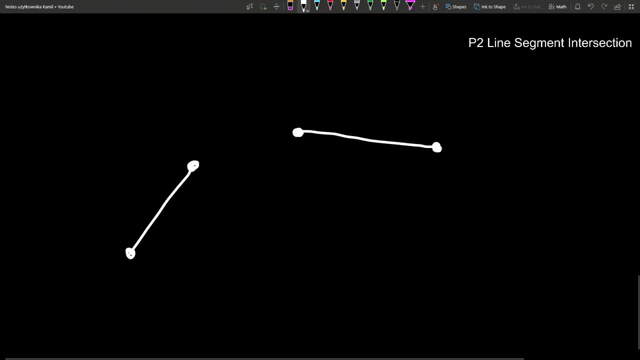 I don't claim that I would think about it this way when I start Two segments, even if they don't intersect most of the time, when you draw an extension of them into a line, the two lines intersect unless segments were parallel. 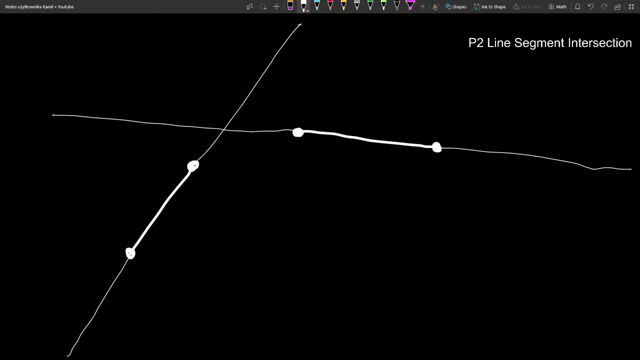 If two segments aren't parallel, then the two lines intersect somewhere. In this case, the intersection point is here. The main idea is to say that, okay, this intersection exists, I just need to check if it's within the segments. How to check if it's within segments? Well, let's first focus on this line. 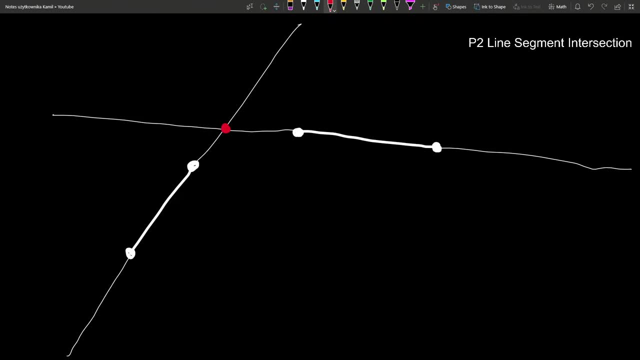 The main idea is to say that, okay, this intersection exists, I just need to check if it's within the segments. How to check if it's within segments? Well, let's first focus on this line and check. if I need to name segments, Let's call them segment 1 or just. 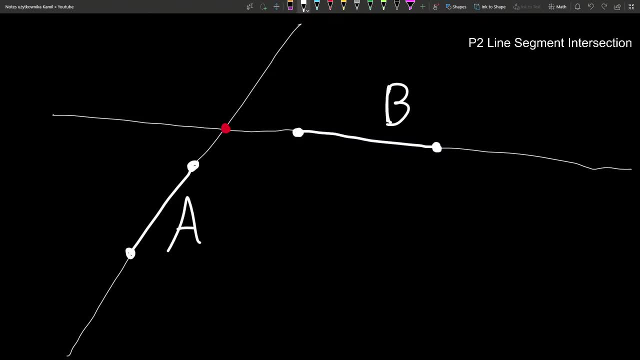 segment A and segment B. This is some intersection. point P: I need to check two things. if A contains point B, sorry, if P is inside A and if P is inside B, Let's focus on the second condition. first We need to check if the drawing is. 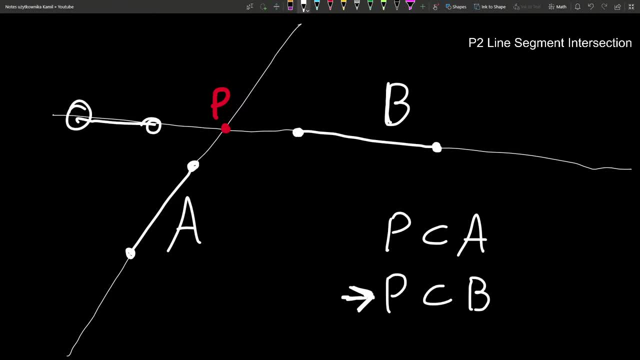 like that. so B is on the right, Maybe B is here on the left, but if those two cases aren't true, then apparently B will contain P. In other words, with respect to this extended A, I need to check if B is completely on the right or. 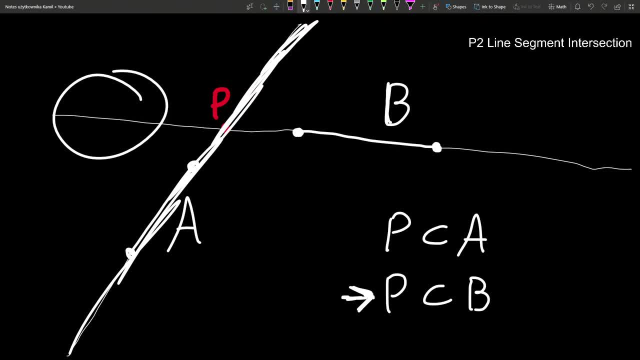 completely on the left. if either of those happens, like here, then no matter where exactly segment A is, even if A is here, if B is completely on the right or left, then we need to say there is no intersection of those segments. Remember, segment is just between two points, a line. 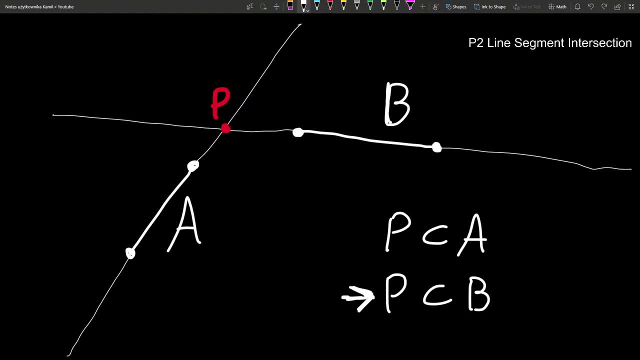 is infinite. One final time To check this. we check if B is complete or webpage. Let's check completely on the right from this line how to do it. we say that this is reference point 0 or anything like that. with respect to call it p0, we check this. 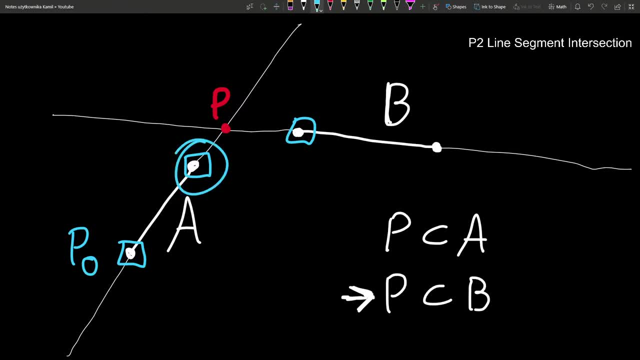 pair of points. we check if this is more on the left than that, and we check if this is more on the left than this. if both those statements are true, then this is completely on the right. so I will compute cross product with respect to that of those two points and this way I will assign a sign plus or minus meaning. 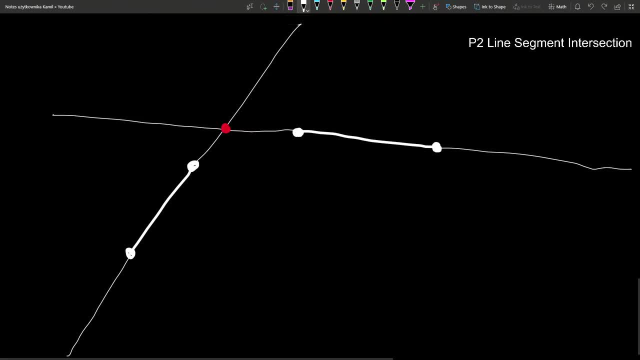 and check if I need to name segments. Let's call them segment one or just segment A and segment B. I- and this is some intersection point- segment A, segment B and segment B section point P. I need to check two things. if A contains point B, sorry, if P. 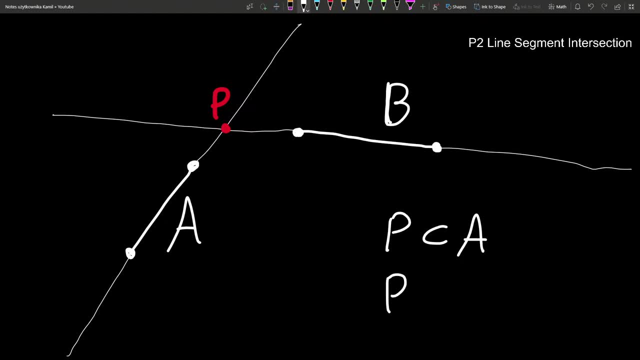 is inside A and if P is inside B. Let's focus on the second condition. first. We need to check if it's the drawing is like that. so B is on the right, maybe B is here on the left. but if those two cases aren't true, then apparently B will. 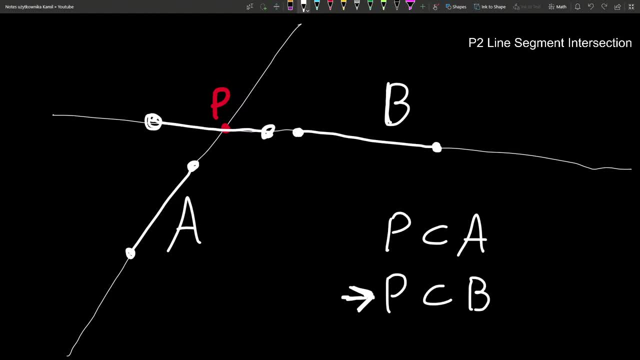 be will contain P. In other words, with respect to this extended A, I need to check if B is completely on the right or completely on the left. If either of those happens, like here, then no matter where exactly segment A is, even if A is. 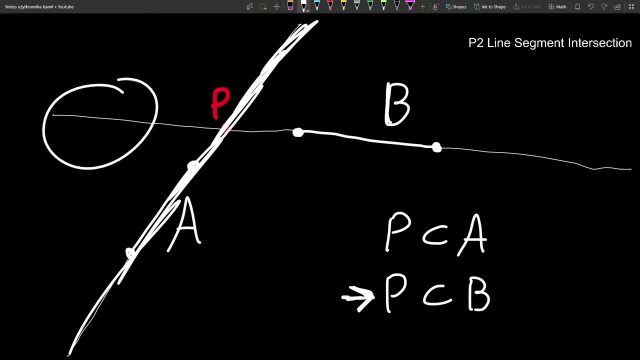 here, if B is completely on the right or left, then we need to say there is no intersection of those segments. Remember, segment is just between two points. A line is infinite. One final time To check this: we check if B is completely on the right from this line. How to do it? We say: 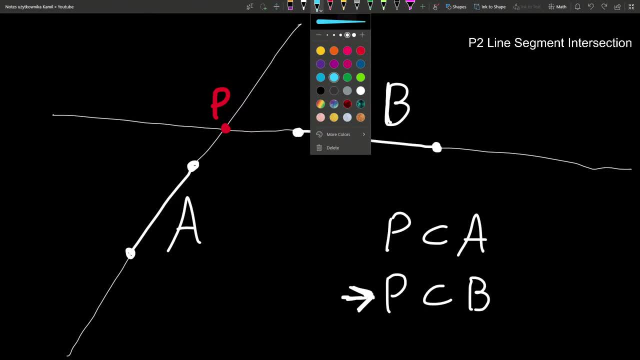 that this is reference point zero or anything like that. with respect to that, We call it P0.. We check this pair of points. We check if this is more on the left than that, and we check if this is more on the left than this. If both those 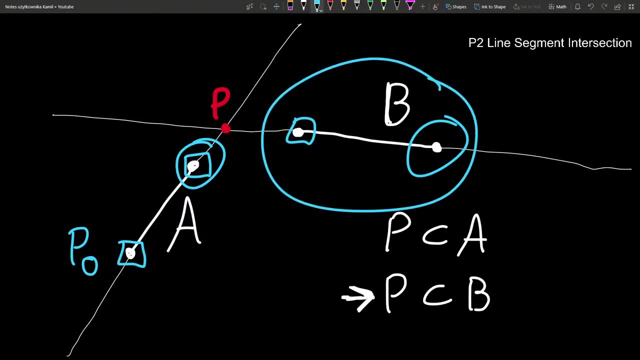 statements are true, then this is completely on the right. So I will compute cross product with respect to that of those two points and this way I will assign a sign plus or minus, meaning right or left. So let's say I did that, I computed this cross product, got area and 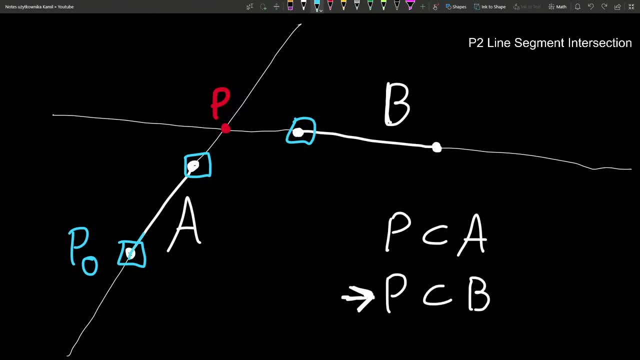 right or left. so let's say I did that. I computed this cross product, got area and I got information that when I take this first and then the second, this is, I got negative cross product. then this first point got mine minus. then Then I check this point with respect to that and I got minus again. 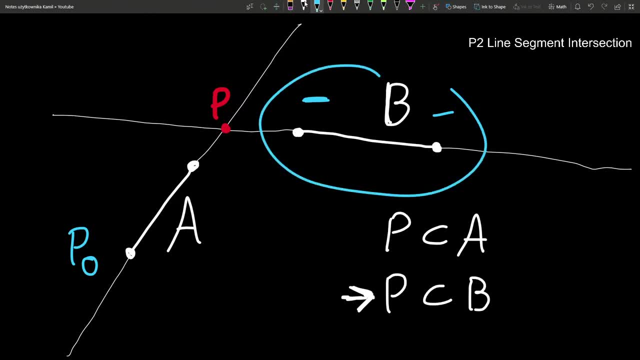 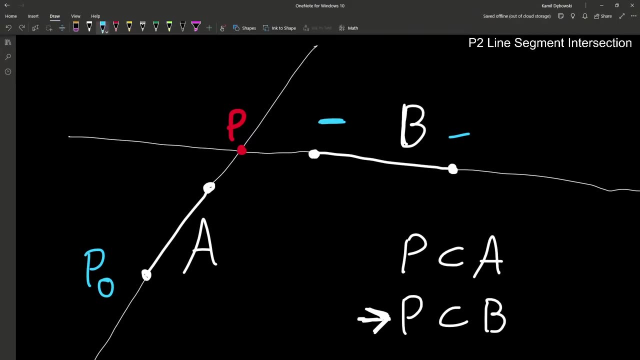 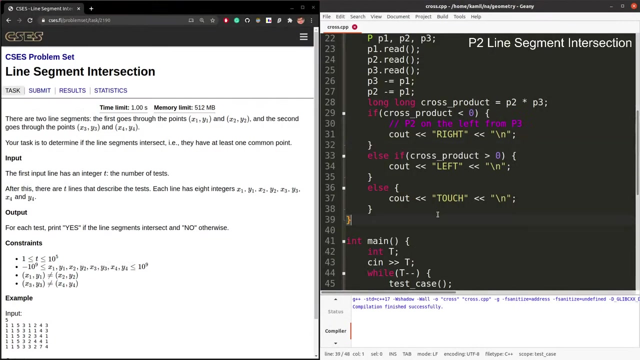 What does it mean? It means that, with respect to P0,, both those points are in the same direction and I need to say there is no intersection because B is strictly on the right from the line. Before we move on, I will implement this small part. 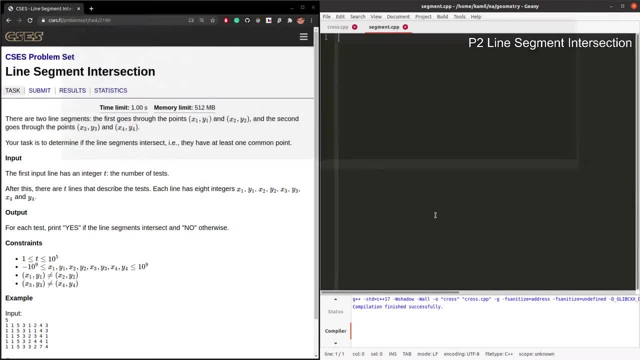 This is what segment. I'm copy pasting the library, the template. What if both segments are parallel? We will get to that. But, Ayush, good point. Can you use linear programming for this? I don't know what you mean. 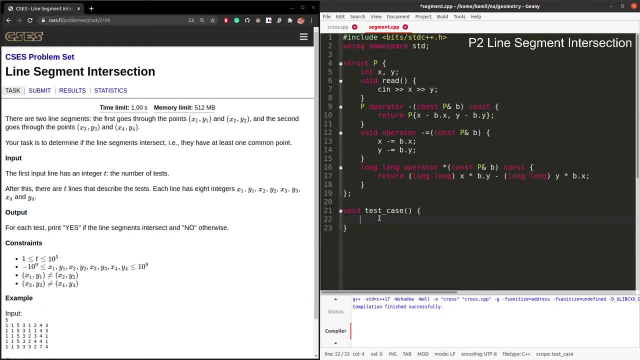 Linear programming is something much harder. We read the input. we will do that later. But what happened With respect to P1, we check P2 and we check P3.. P3, we will do this and that, Those two triples. 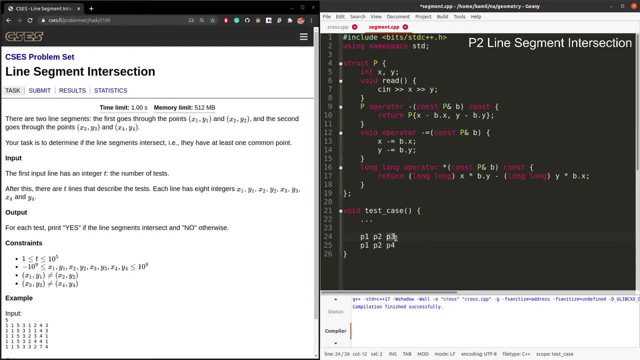 With respect to this first guy, I check if P3 is on the right than P2, and this as well. So sine 1 is P2 minus P1 times P3 minus P1.. I will explain this line Just first let me do the other one. 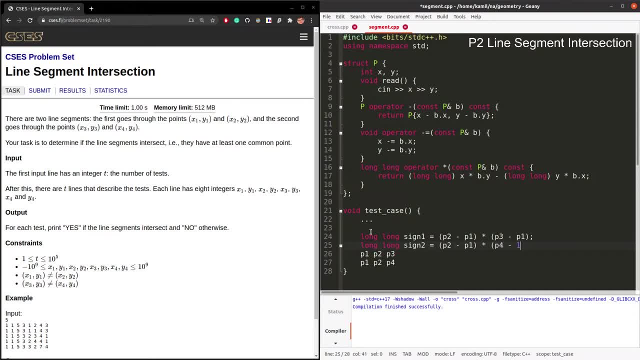 P2 minus P1 times P4 minus P1. Doing this is equivalent, just one line version of doing taking everything with respect to P1, assuming that P1 is 0, 0 now, And then doing stuff. But I can do it in one line. 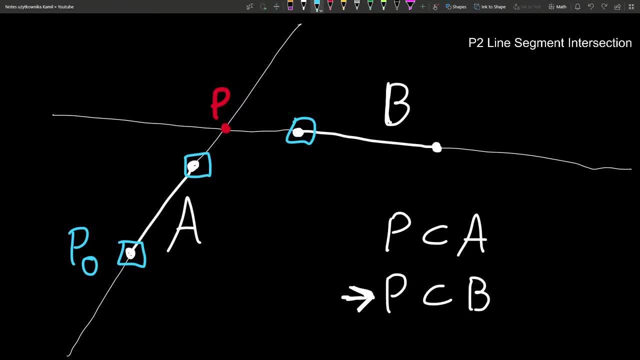 I got information that when I take this first and the second, this is, I got negative cross product. Then this first point got minus. Then I check this point with respect to that and I got minus, indeed Minus, again. What does it mean? It means that, with respect to P0- both those points- and with respect to 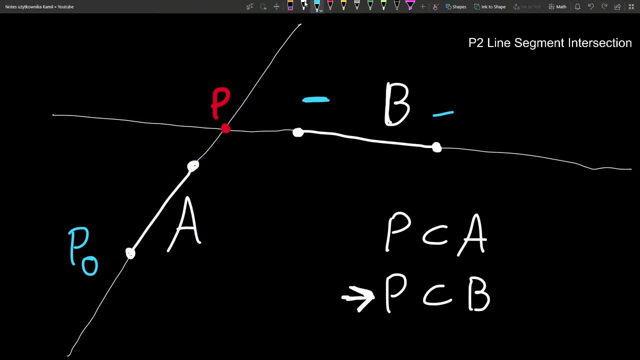 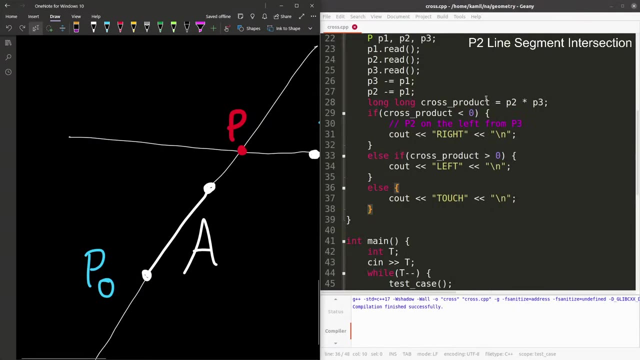 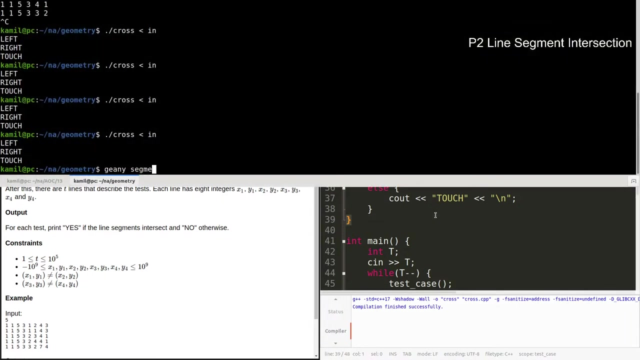 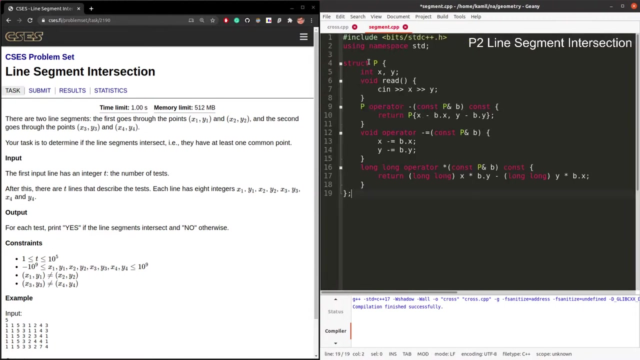 that both those points are in the same direction and I need to say there is no intersection, because B is strictly on the right from the line. Before we move on, I will implement this small part. This is what segment I'm copy-pasting: the library, the template. 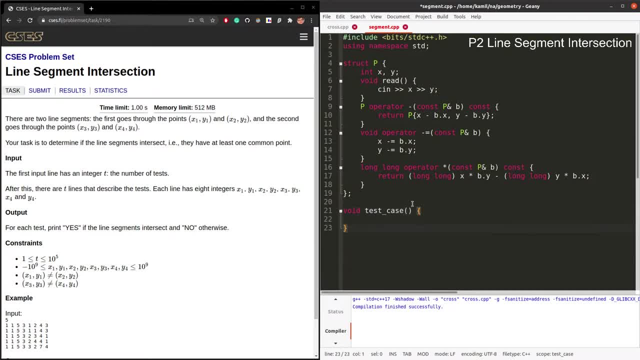 What if both segments are parallel? We will get to that, but, Ayush, good point. Can you use linear programming for this? I don't know what you mean. Linear programming is something much harder. Okay, we read the input. We will do that later. But what happened With respect to 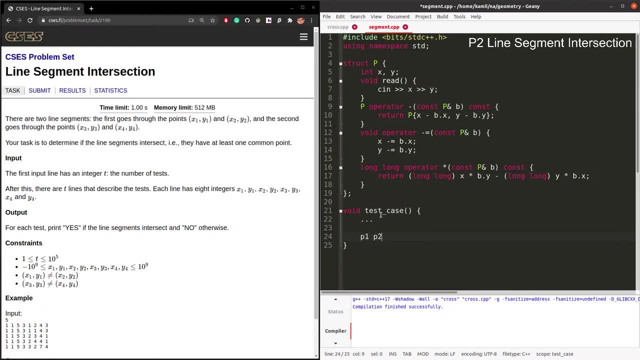 P1, we check P2 and we check P3. We will do this and that Those two triples. With respect to this first guy, I check if P3 is on the right than P2, and this as well. So sine one is P2 minus P1 times P3 minus P1.. I will explain this line Just first. 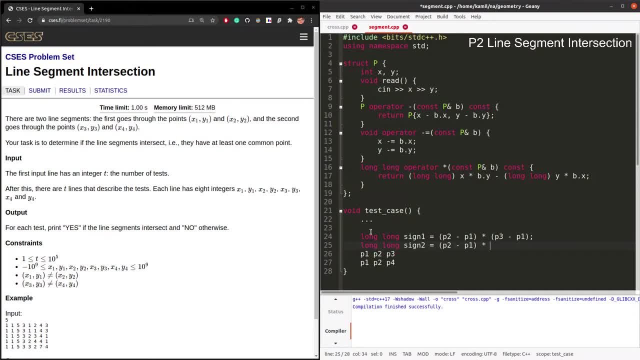 let me do the other one: P2 minus P1 times P4 minus P1.. Doing this is equivalent, just one line version of doing like taking everything with respect to P1, assuming that it is on P1. Assuming that P1 is 0, 0 now and then doing stuff. But I can do it in one line. 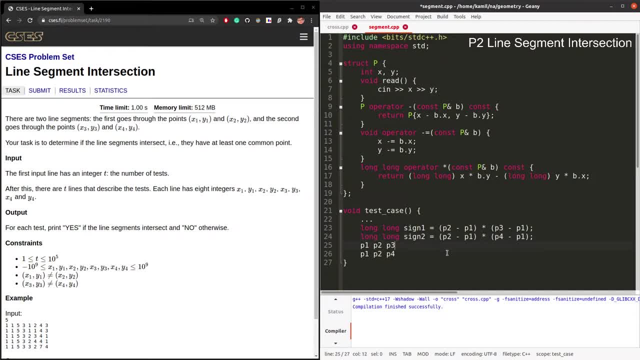 This is maybe one extra operation because I compute this twice, but it's convenient. Now I need to do this. I need to do this. Now I need to say if both are negative or both are positive, sine, actually it's not. 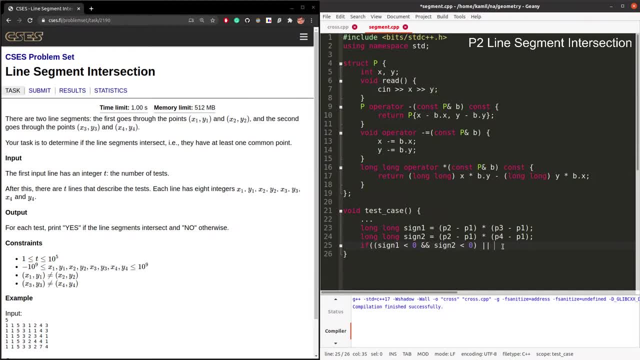 just sine. it's the whole value, but I care if it's positive or negative. Then we say: this means that segment B is on left or right From line A, line meaning extension of segment A. and I need to say what? no, no intersection. 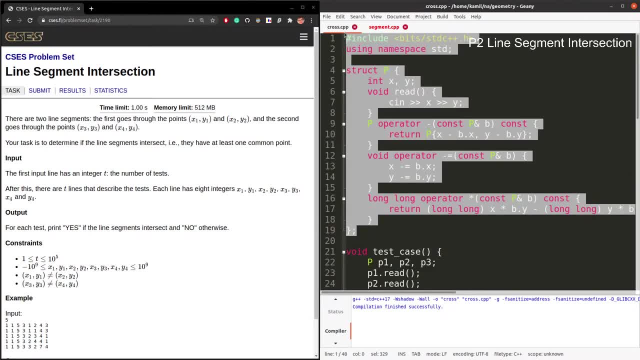 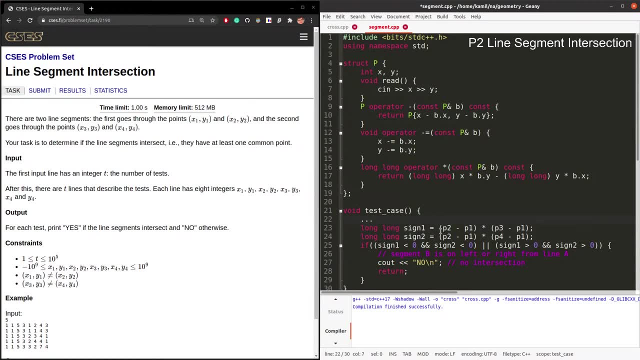 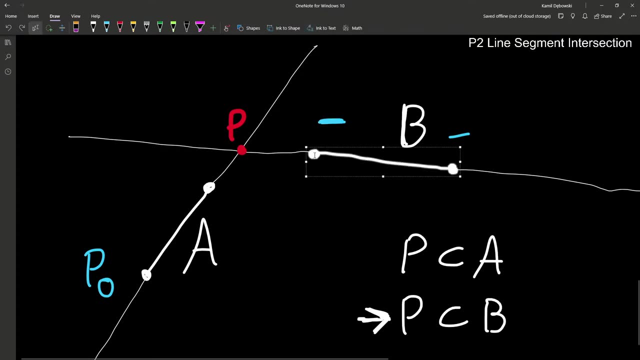 How could we solve the previous problem without shifting the points We did? We, I mean we shifted points and we do it here just in one line, instead of doing it previously. It's alternative implementation. Okay, Right, But there is a case we will continue only if it's something like that. 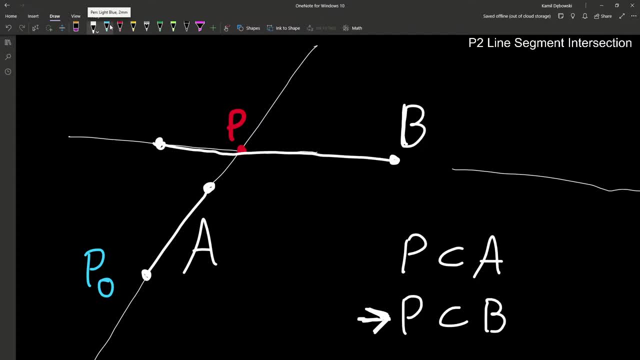 If B is, for example, that and one guy got positive sign, the other negative sign, In this case we continue, but still, intersection might not belong to segment A. We checked this, It's fine. It's okay, Done. 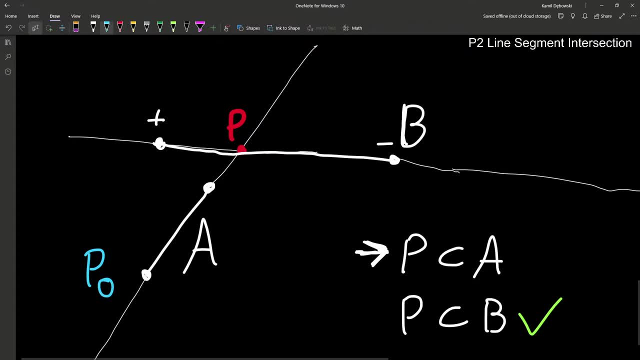 Now we need to check if B belongs to A, And you can. we need to implement the same just for the other segments. So, with respect to this guy P zero, you need to take this one and check this And, of course, you can have twice very similar code. but we're we're smarter than that. 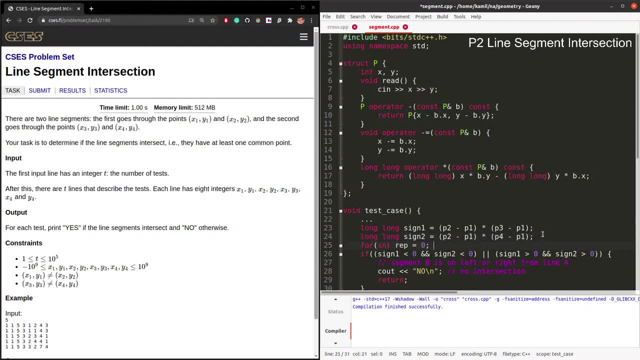 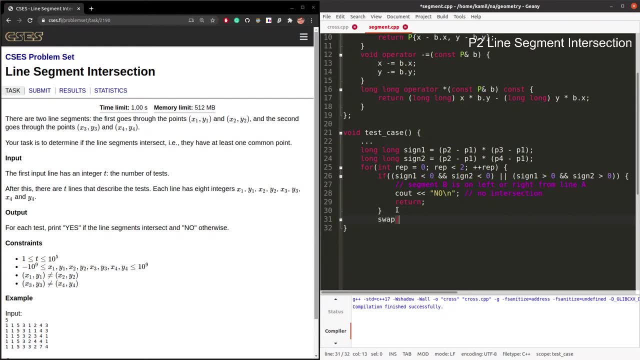 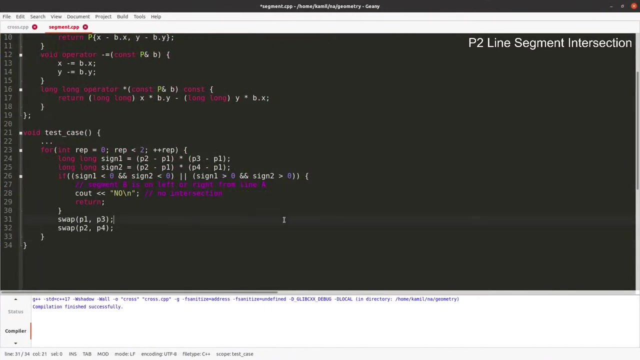 Repeat twice. Okay, Let's do this Just a for loop That does two iterations: Do this and then swap. What do we swap? Swap the two segments. In the second iteration, segments A and B are swapped. So we will check the other condition. 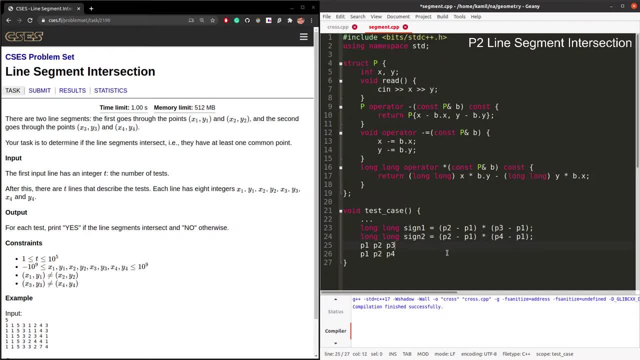 This is maybe one extra operation because I compute this twice, but it's convenient. Now I need to say if both are negative or both are positive sine. actually, it's not just sine, It's the whole value. It doesn't matter if it's positive or negative. 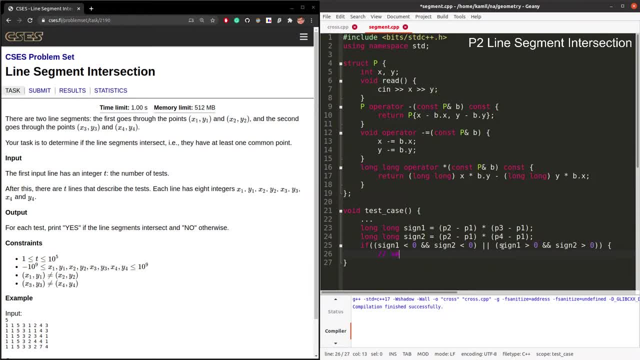 Then we say: this means that segment B is on left or right from line A, Line meaning extension of segment A, And I need to say what? no, no intersection. Okay, How could we solve the previous problem without shifting the points? 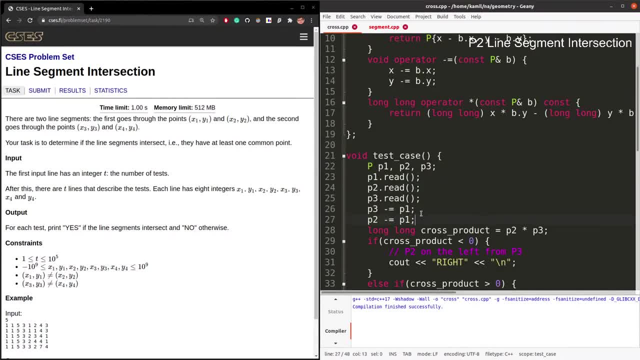 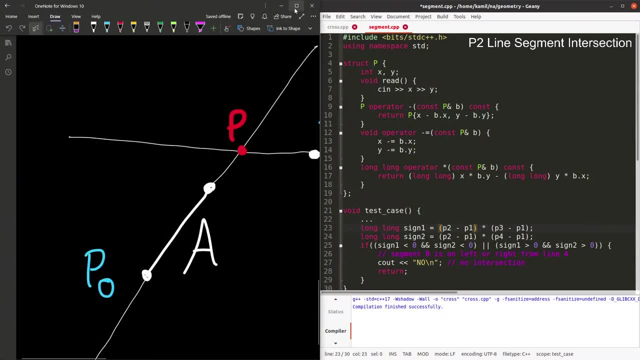 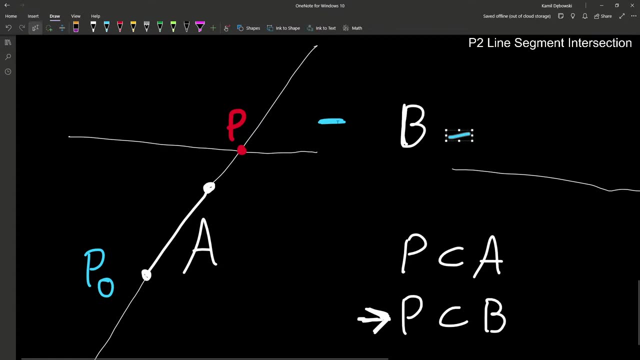 We did. We, I mean we shifted points, And we do it here just in one line instead of doing it previously. It's alternative implementation, right, But there is a case we will continue only if it's something like that. If B is, for example, that: 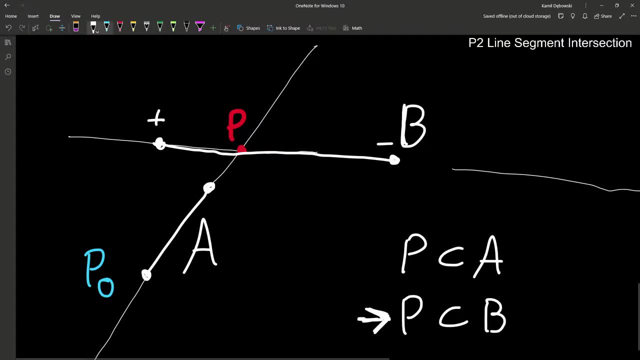 And one guy got positive sine, the other negative sine. In this case we continue, but still, intersection might not belong to segment A. We checked this. This is fine, Okay, Done. Now we need to check if P belongs to A, And you can. we need to implement the same, just. 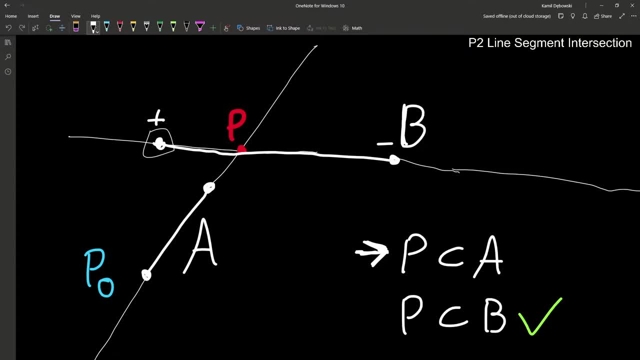 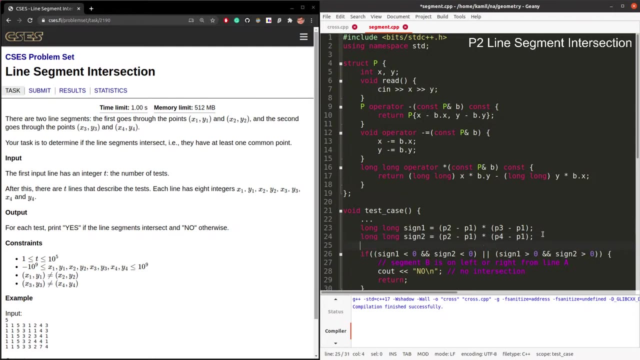 for the other segments. So, with respect to this guy, P0.. Okay, Done, Okay, You need to take this one and check this And, of course, you can have twice very similar code. but we're we're smarter than that. 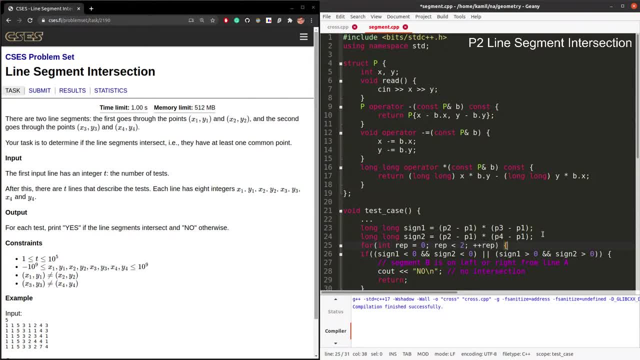 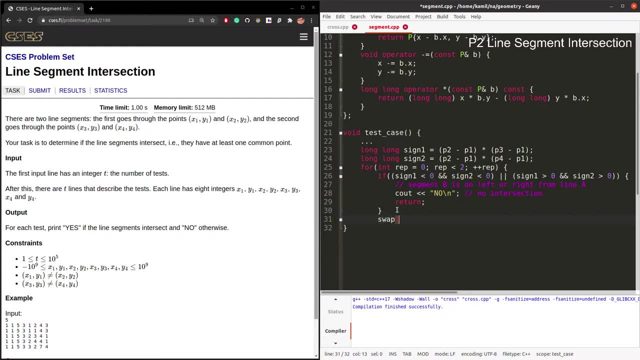 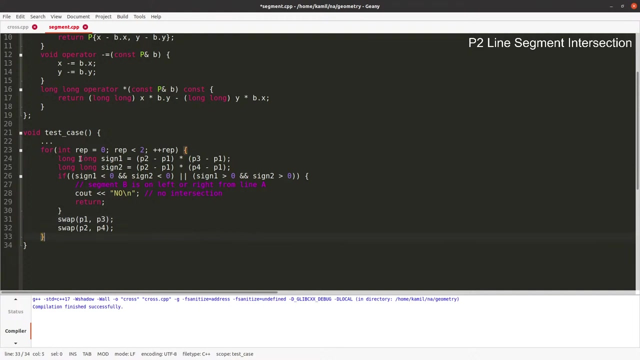 Repeat twice. Just a for loop That does two iterations: Do this and then swap. What do we swap? Swap the two segments. Okay, In the second iteration segments A and B are swapped. So we will check the other condition. 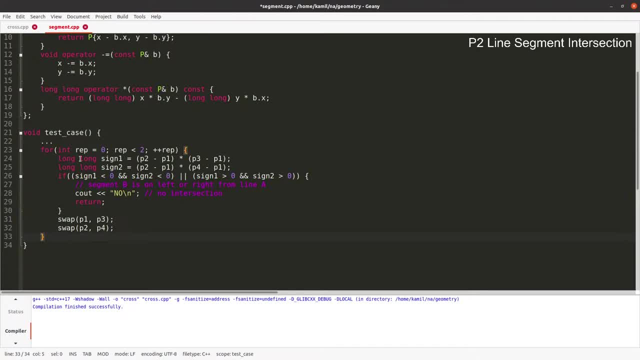 We once checked if P belongs to segment the red intersection, P belongs to segment B. Then we check if it belongs to segment A And otherwise. finally we say yes, We didn't, just we didn't yet consider parallel case. Parallel is to do. 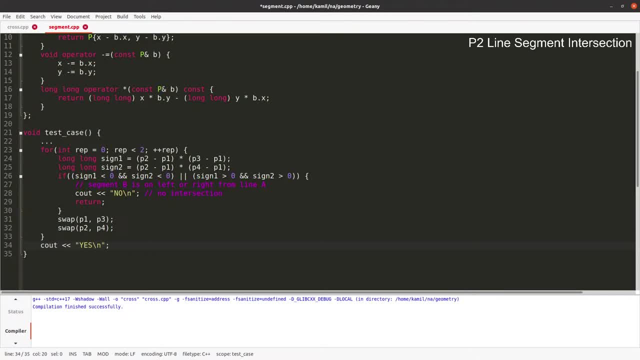 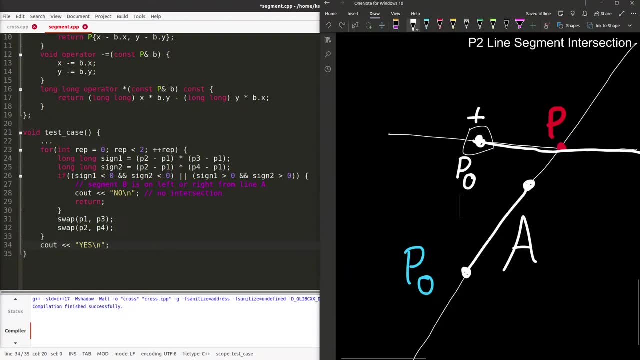 We don't know what will happen then. What if one endpoint of B lies on A? Good question? We can analyze what happens then. Fortunately this approach of saying that there is red intersection P and we just check if it's inside both segments. 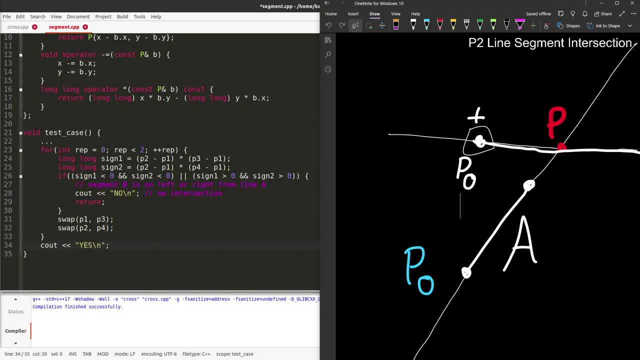 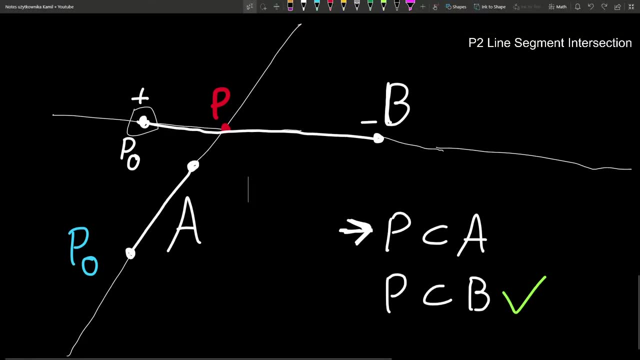 It's quite convenient for us. Okay, Done. Let's see what happens if segment B is exactly on the same line as segment B, Right? Somebody asked what happens if something is exactly on the line. Let's say this is B, Segment B is exactly like that. 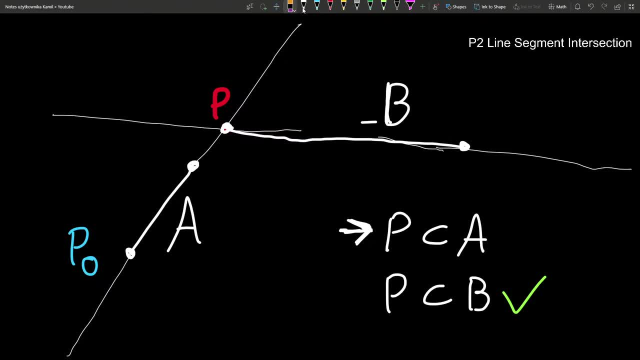 All right, We got some. In this case, One endpoint of B will give cross product zero. with respect to those two points, The cross product sign is zero, but still we have intersection. I said that we check if both values are positive or negative, to check if both endpoints are. 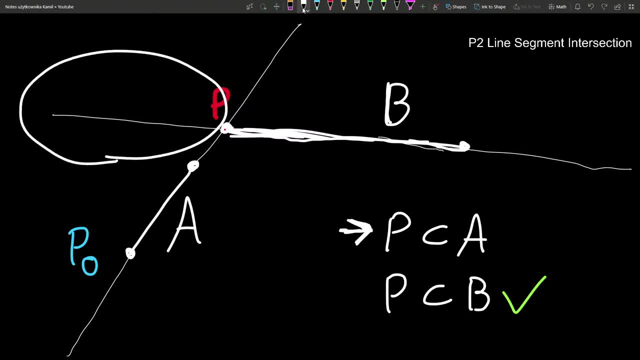 strictly on the right or both endpoints are strictly on the left. If at least one of them is here, then we say that P belongs to B. This is still correct, Okay, So assuming that what I want to happen is, if this is the input, I want to say yes. 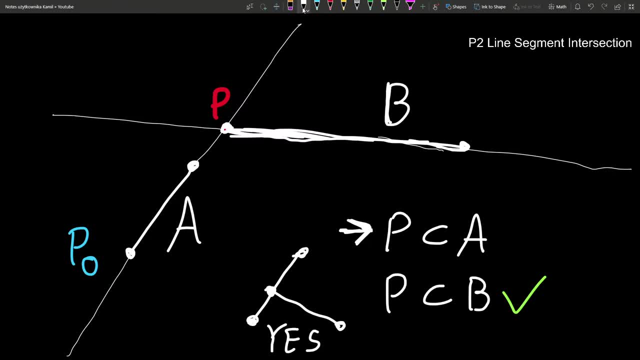 They intersect, Indeed, they have a common point. Intersection means a common point And they have a common point. In this case we say yes, Then everything is fine. But it's good to be careful with those cases Like only slightly touching the line. 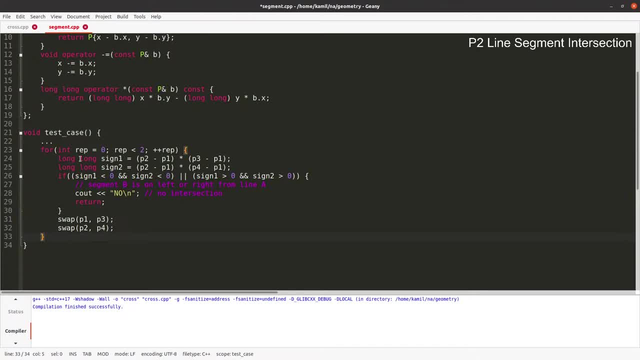 We once checked if P belongs to segment the red intersection, P belongs to segment B. Then we check if it belongs to segment A And otherwise. finally we say yes, We didn't, just we didn't yet consider parallel case. Parallel is to do. 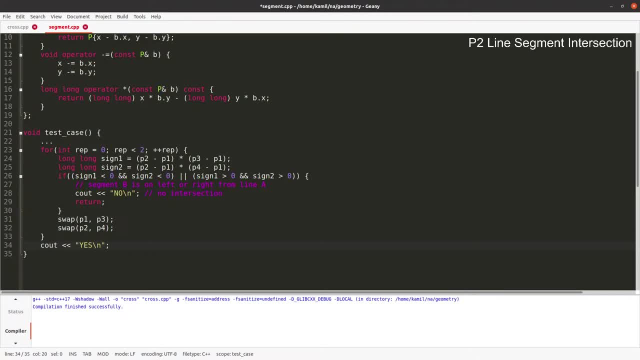 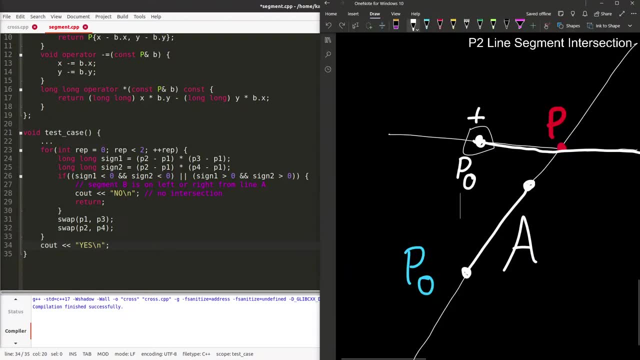 We don't know what will happen then. What if one endpoint of B lies on A? Good question? We can analyze what happens then. Fortunately this approach of saying that there is red intersection P and we just check if it's inside both segments. 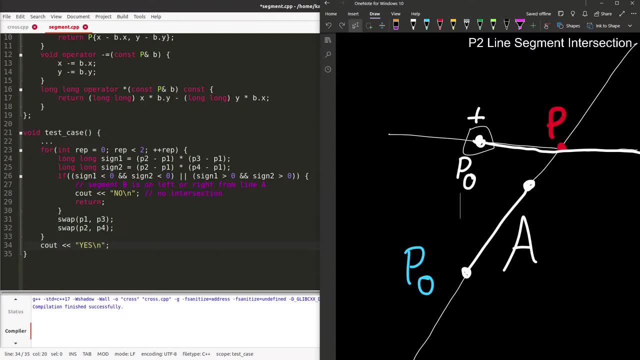 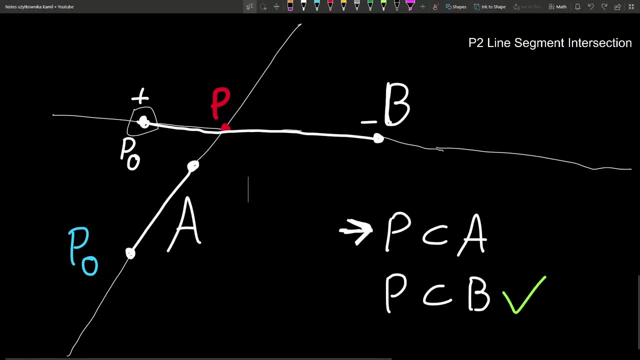 It's quite convenient for us, right? Somebody asked what happens if something is exactly on the line. Let's say this: this is B, Segment B. It's exactly like that. All right, We got some. In this case, one endpoint of B will give cross product zero with respect to those two points. 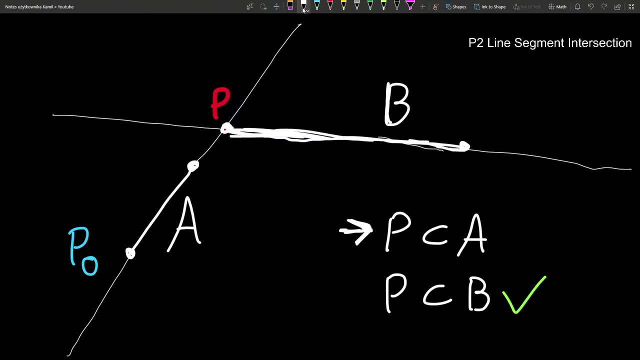 The cross product sign is zero, But still we have intersection. I said that we check if both values are positive or negative To check that we have intersection of B and B. There is intersection, So we have intersection. We check if both values are positive or negative. 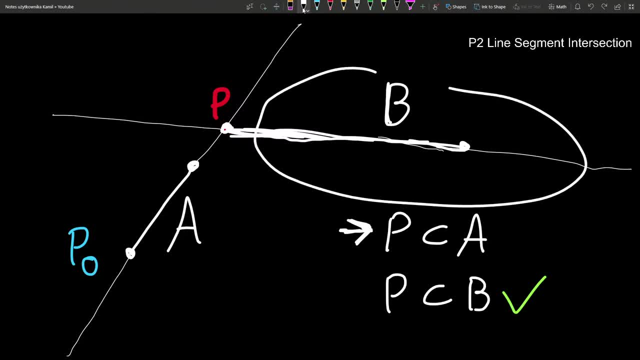 We check if both values are positive or negative, if both endpoints are strictly on the right or both endpoints are strictly on the left. If at least one of them is here, then we say that p belongs to b. So this is still correct. 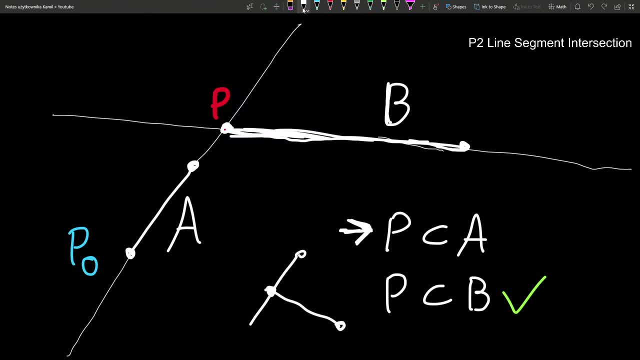 Assuming that what I want to happen is, if this is the input, I want to say yes, They intersect, Indeed, they have a common point. Intersection means a common point and they have a common point. So in this case we say yes, Then everything is fine. But it's good to be careful with those cases. 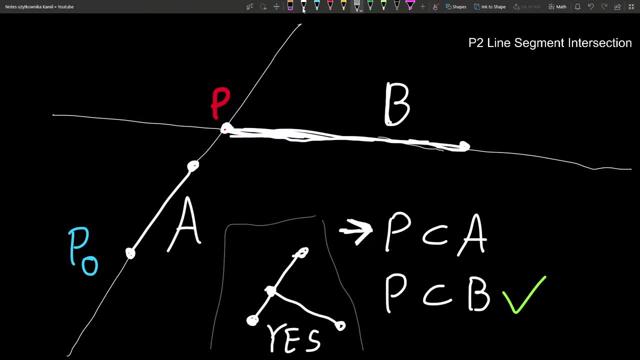 like only slightly touching the line. you know something like that. Any kind of collinearity is often very annoying to deal with. Would it be more efficient to check if the parts of the multiplication have just different signs and not actually doing the multiplication? 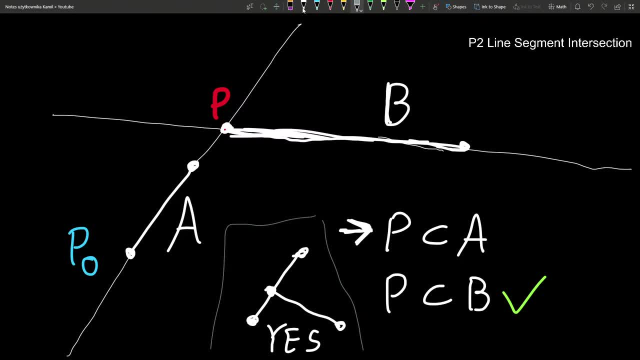 You know something like that. Any kind of collinearity is often very annoying to deal with. Would it be more efficient to check if the parts of the multiplication have just different signs and not actually doing the multiplication? No, you need to compare two values. 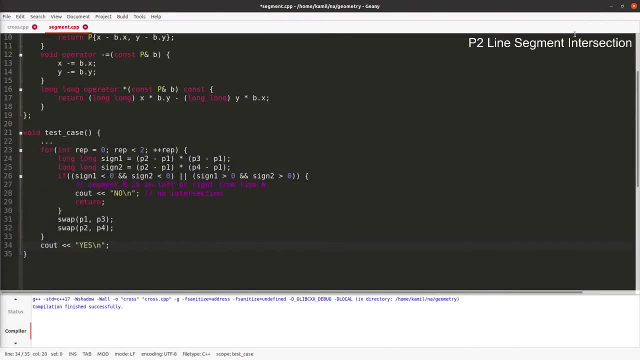 There is no way to speed this up more. I'm answering Ioanni's question Like: Okay, So what is the other way? Oh, sorry, sorry, You are completely right. Okay, I was wrong here. Yes, you can not do multiplication and you just you can take. 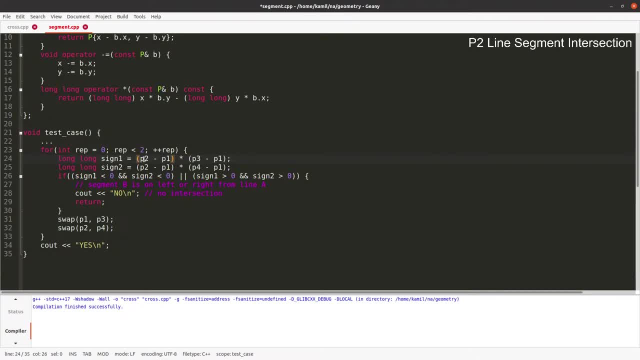 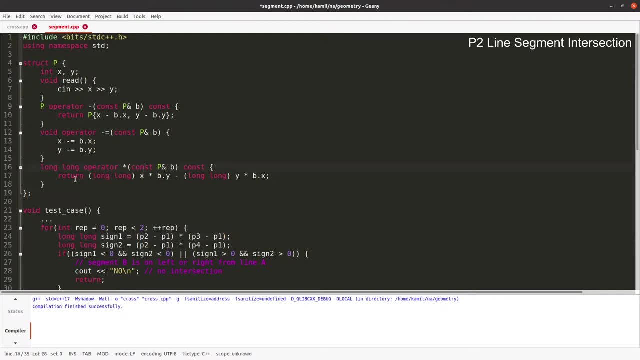 Oh wait, now I'm confused. This sign does cross product. Okay, So this product. it runs this thing To check if this is smaller than zero. you're basically comparing those two values. You need to do that. There is no simpler way here. 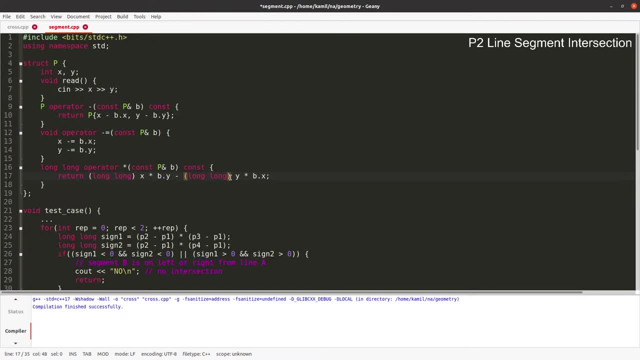 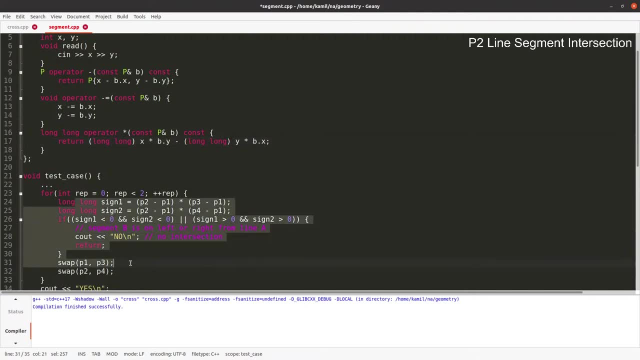 Okay. Why don't you use functions instead of loops here? Isn't this confusing for some people? I guess you're right. Yeah, I could use a function instead of that. What if we asked to find exact point of intersection? Then we would compute it with some ugly formulas. 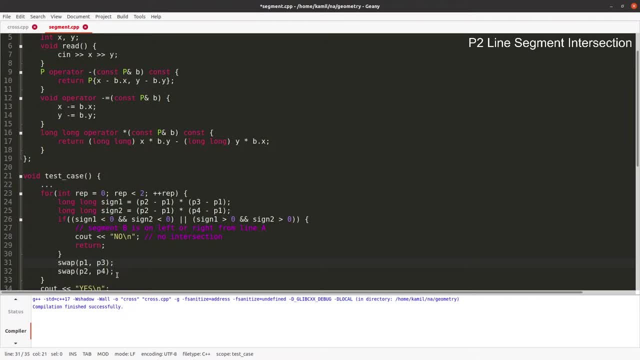 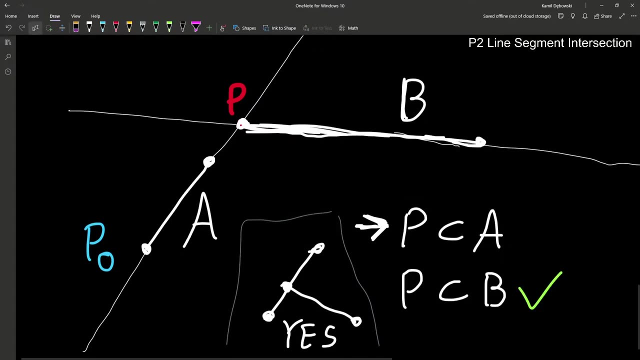 What about just checking if distance to segment endpoints is smaller than segment length? I mean, this seems like some heuristic. I don't know why this would be true. Why do we need to check cross product for both lines? I mean, I explained that we check if P belongs to A and if it belongs to B, right? 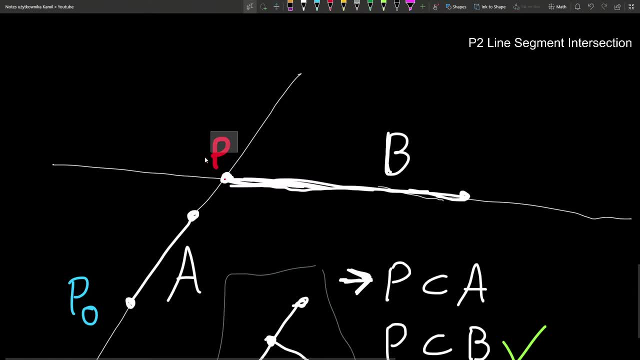 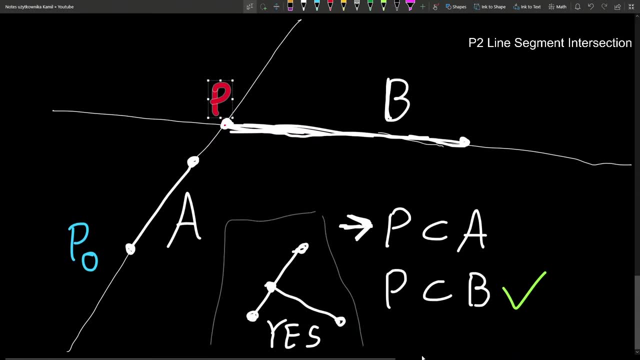 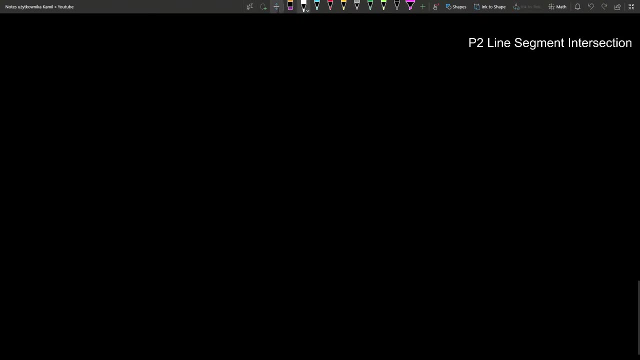 I said, there exists intersection point of the two lines, extensions of A and B, And we check if it belongs to both B and A. If you don't want to talk about this, point P, then these are cases that you want to avoid. 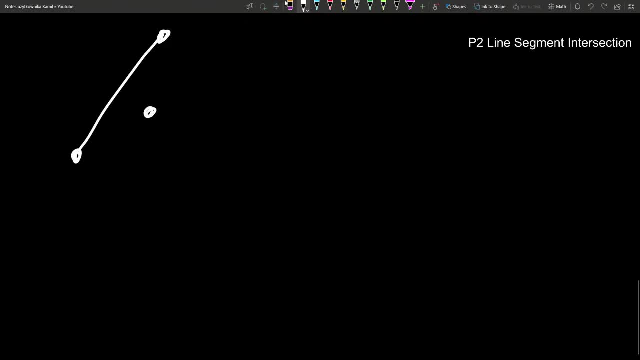 Okay, If A and B are like this, then B is on the right from A. If B is like that and A is like this, then A is on the right from B, And I'm saying on the right. this depends on direction of B. 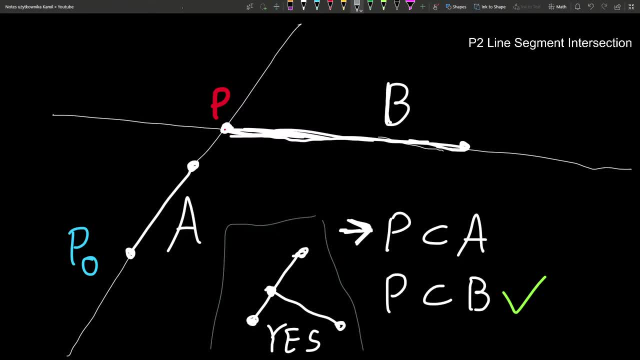 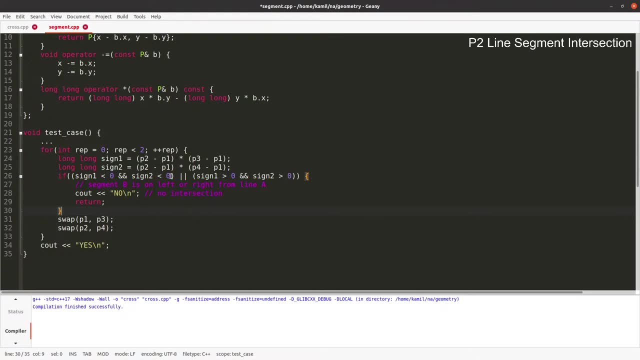 No, you need to compare the values. There is no way to speed this up more. I'm answering Joani's question. Oh, sorry, sorry, you are completely right. Okay, I was wrong here. Yes, you can not do multiplication and you just you can take. 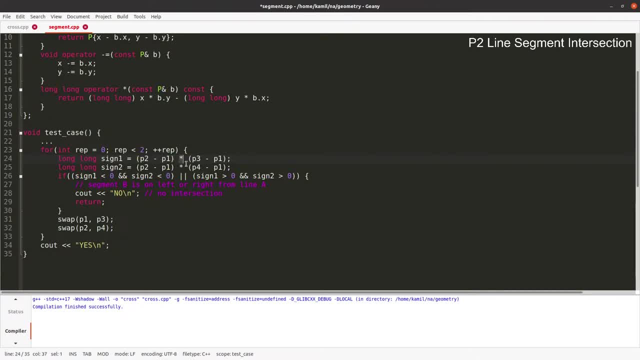 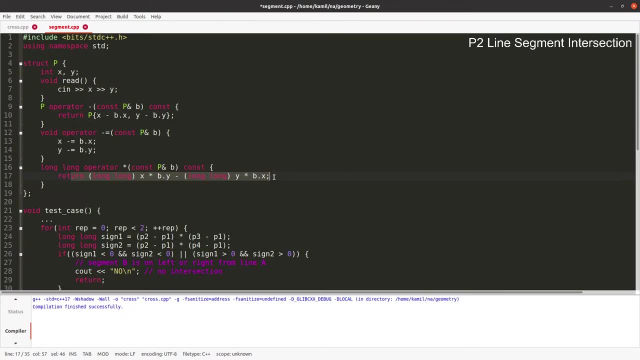 Oh wait, now I'm confused. This sign does cross product. Okay, so this product. it runs this thing To check if this is smaller than zero. you're basically comparing those two values. You need to do that. There is no simpler way here. 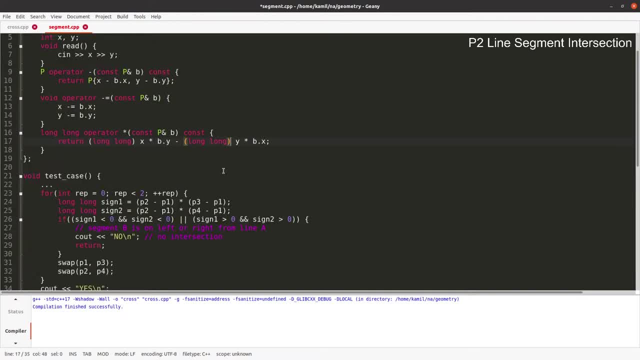 Why don't you use functions instead of loops here? Isn't this confusing for some people? I guess you're right. Yeah, I could use a function instead of that. What if we asked to find the exact point of intersection? Then we would compute it with some. 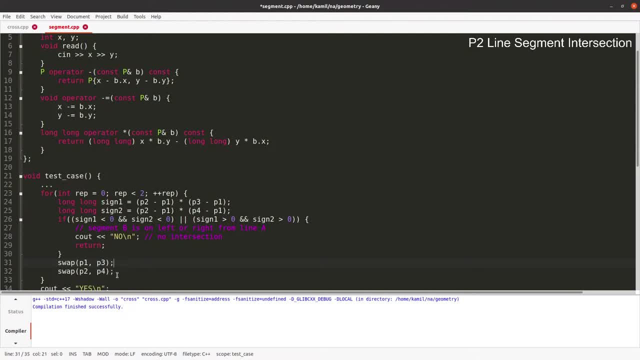 ugly formulas. We would compute it with some ugly formulas. We would compute it with some ugly formulas. What about just checking if distance to segment endpoints is smaller than segment length? I mean, this seems like some heuristic. I don't know why this would be true. 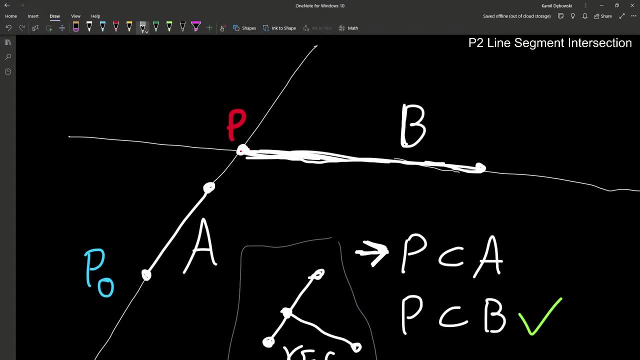 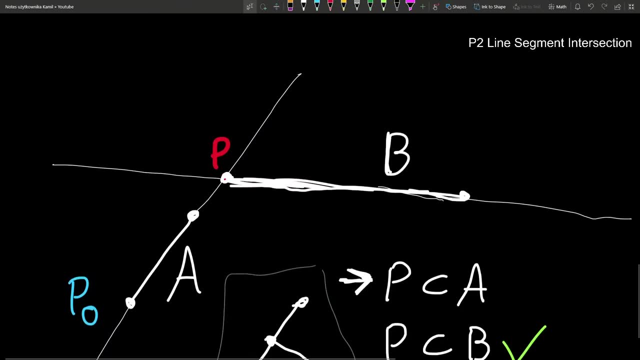 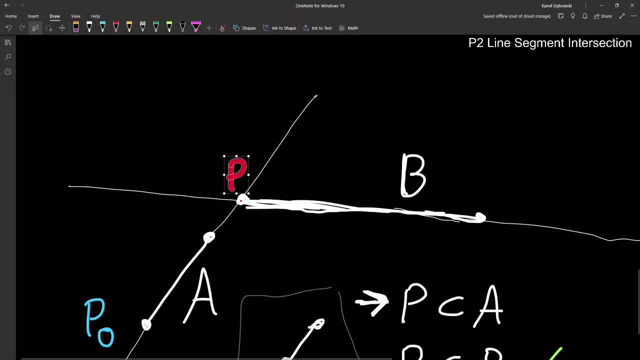 Why do we need to check cross product for both lines? I explained that we check if P belongs to A and if it belongs to B. Right, I said, there exists intersection point of the two lines, extensions of A and B- And we check if it belongs to both B and A. 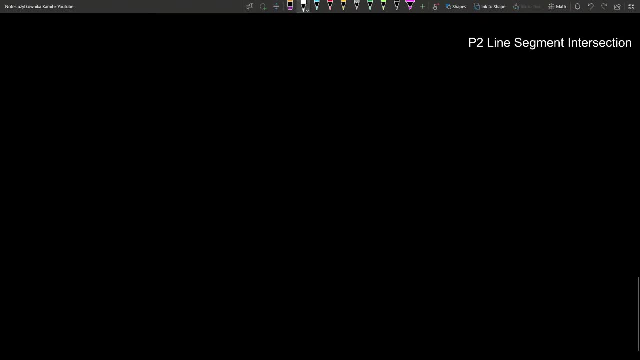 If you don't want to talk about this, point P- then these are cases that you want to avoid. If A and B are like this, then B is on the right from A. If B is like that and A is like this, then A is on the right from B, And I'm saying on the right. this depends on direction of B. 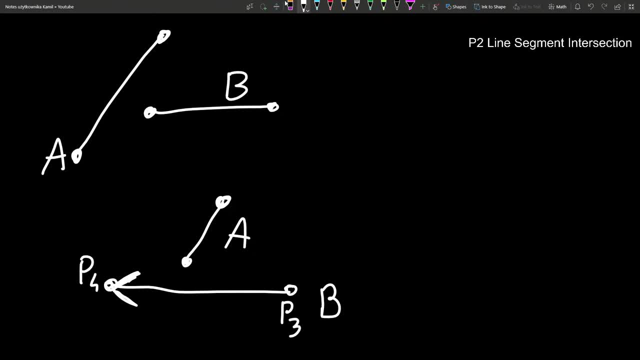 Like if this is first point P3 and this is second point P4. The order is important. The point is, if A is completely on the right from segment B, then there is no intersection, No matter what case you draw with something like that, something like this: 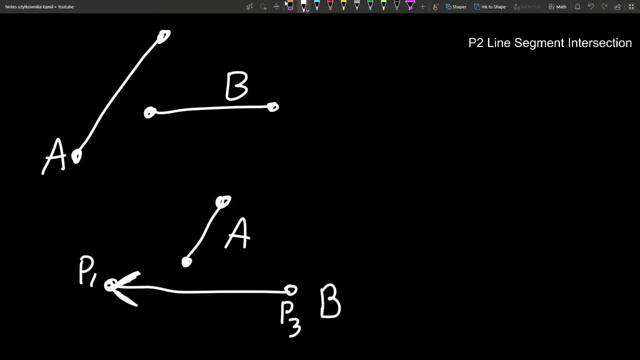 Like if this is first point P3 and this is second point P4. The order is important. The point is, if A is completely on the right from segment B, then there is no intersection. No matter what case you draw with something like that, something like this, maybe some cases will be trickier. 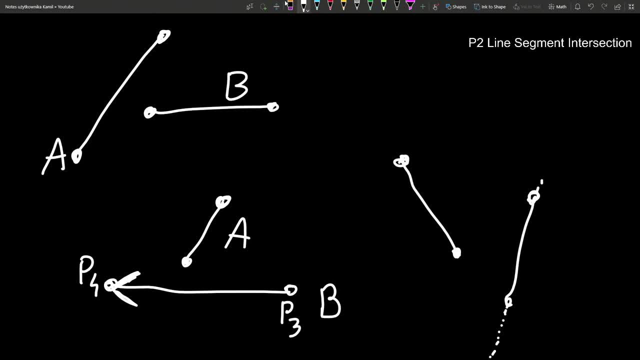 But if they don't intersect, you can expand one of the segments and say that the other segment is completely on one side. Because if you cannot do that, if for both cases when you expand the line, you will see the intersection with the other guy. 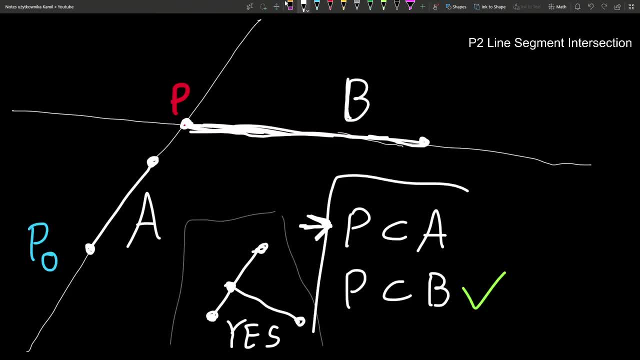 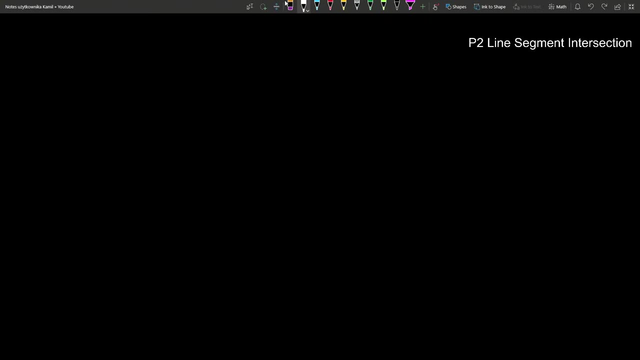 then it implies- and it was shown here using this trick- that the red intersection P belongs to both. How did we get P computationally? We didn't. This is a proof. One last thing is to deal with parallel lines. If there are parallel lines, then P doesn't exist. 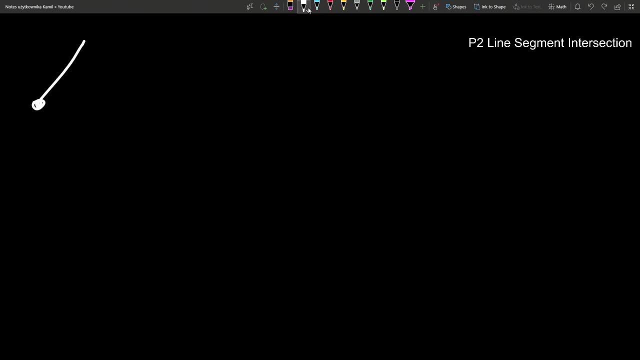 My proof doesn't work. What are parallel cases? A and B can be like that, then no intersection. A and B can be like this: They are collinear, Everything is collinear, but they don't intersect. Or maybe A is like this and B like that, or a lot of other possibilities. 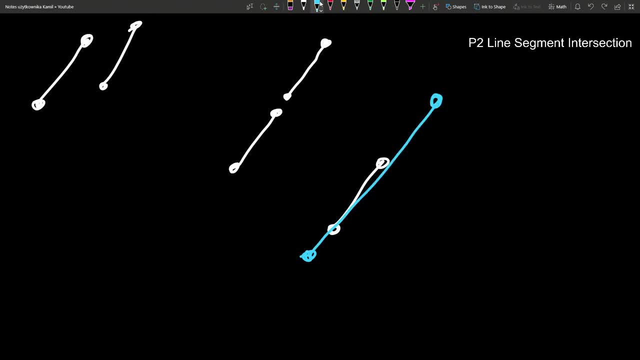 This thing, this thing, one contains the other, and so on. I'm going to go with this logic: If the four points aren't collinear, then I say no intersection. In this case, the four points aren't collinear, but segments are parallel. 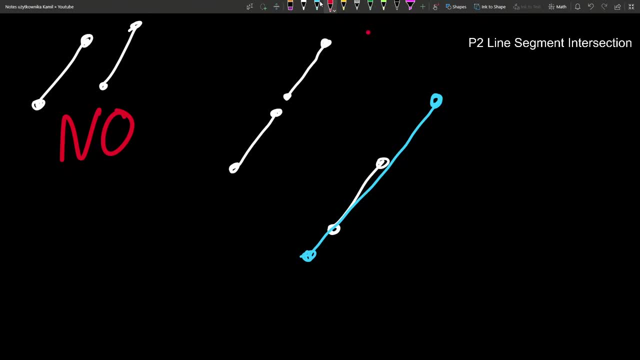 So here I say no, and that's easy to do, And I need to distinguish those two cases. But let's start with this: How to check if two segments are collinear. For this it's useful to think about vectors, To say that when I subtract P2 from P1, I will get this vector. 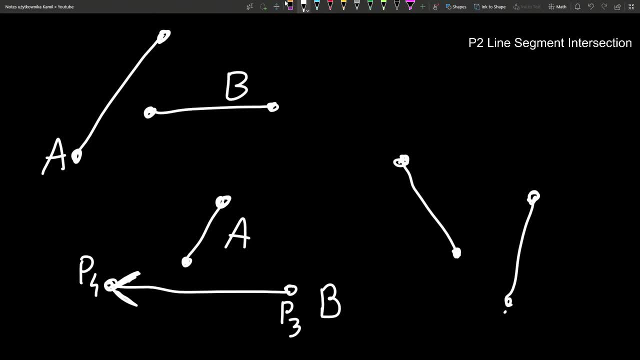 maybe some cases will be trickier, but if they don't intersect, you can expand one of the segments and say that the other segment is completely on one side. Because if you cannot do that, if for both cases when you expand the line, you will see the 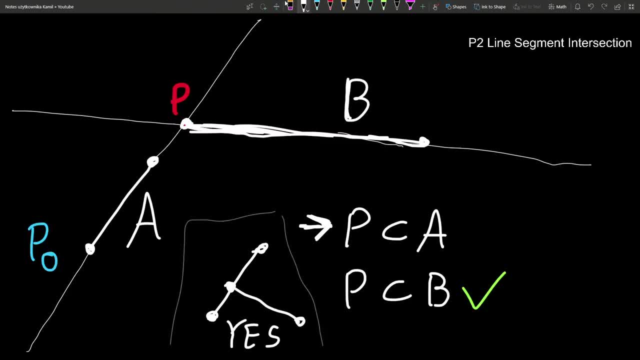 intersection with the other guy, then it implies- and it was shown here using this trick- that the red intersection, P, belongs to both. How did we get P computationally? We didn't. This is a proof. One last thing is to deal with parallel lines. 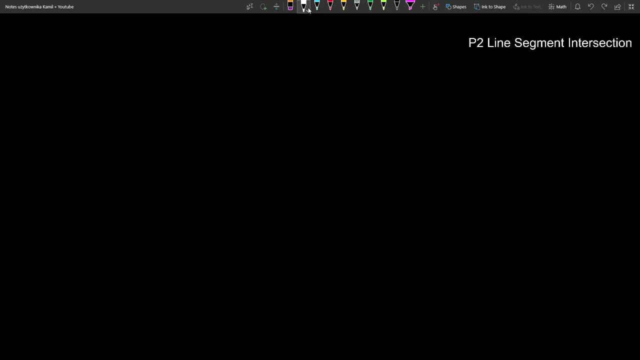 If there are parallel lines, then P doesn't exist. My proof doesn't work. What are parallel cases? A and B can be like that, then no intersection. A and B can be like this. They are collinear, Everything is collinear, but they don't intersect. 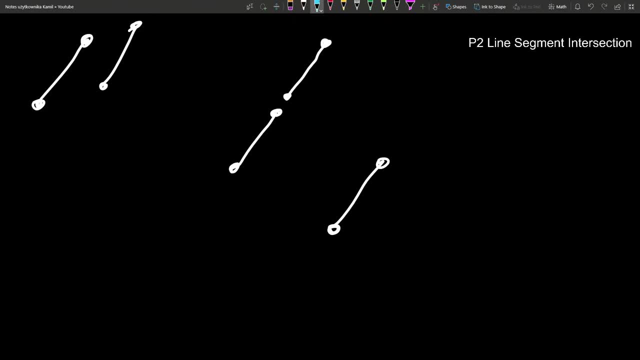 Or maybe A is like this and B like that, or a lot of other possibilities, This thing, this thing, one contains the other, and so on. I'm going to go with this logic. If the four points aren't collinear, then I say no intersection. 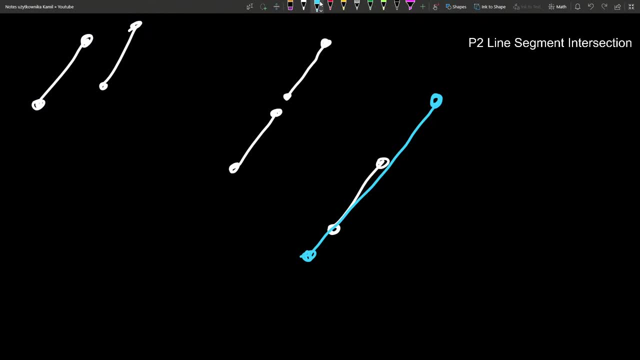 In this case the four points aren't collinear, Right, Right And but segments are parallel. So here I say no, and that's easy to do, And I need to distinguish those two cases. But let's start with this. 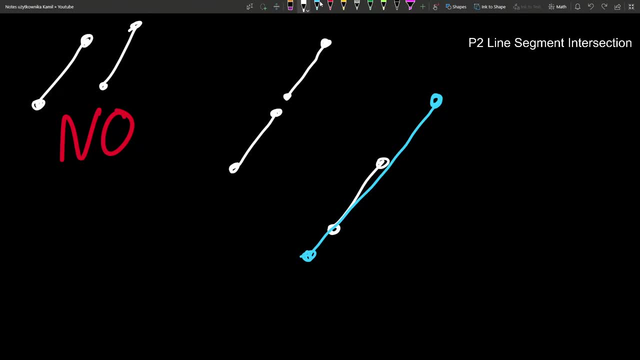 How to check if two segments are collinear. For this it's useful to think about vectors, To say that when I subtract P2 from P1, I will get this vector, kind of transition vector, from this point to this one, P2 minus P1. 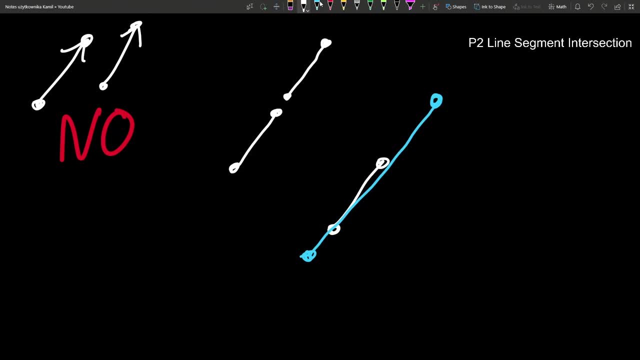 And I also get this vector. And you know two vectors are parallel if, and only if, they have the same slope. You need to compare if Y divided by X is divided by Y2 divided by X2.. This leads to again cross product. 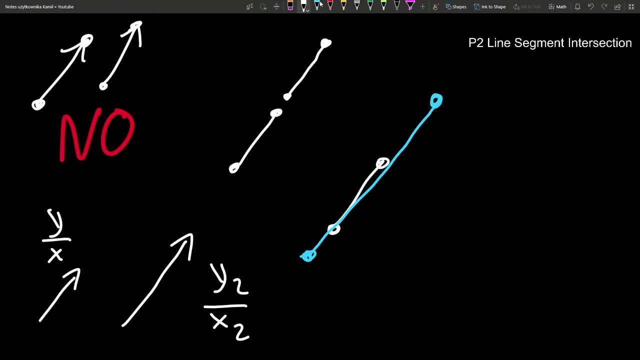 Cross product of two vectors is zero Slopes. always when we deal with cross product in some way, we compare slopes, Just in smart way, without division, So keeping only integers. So to check, So to check if this is parallel to that, we take this vector. 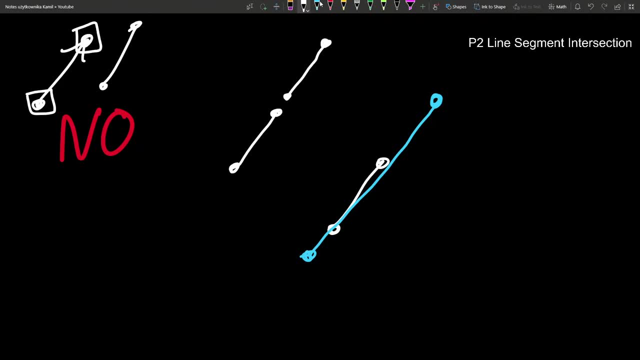 Kind of transition vector from this point to this one P2 minus P1. And I also get this vector. And you know, two vectors are parallel if, and only if, they have the same slope. You need to compare if Y divided by X is divided by Y. 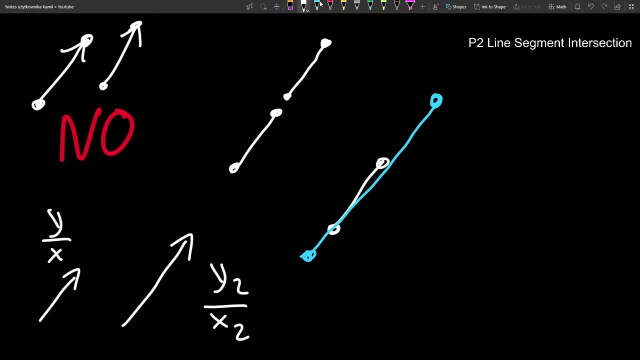 Y2 divided by X2.. This leads to again cross product. Cross product of two vectors is zero Slopes. always when we deal with cross product in some way, we compare slopes, Just in smart way, without division, So keeping only integers. 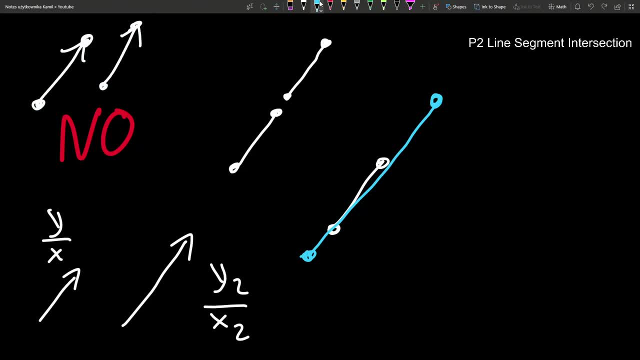 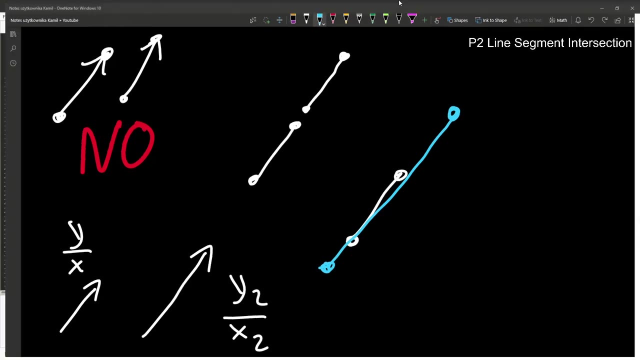 So to check if this is parallel to that, we take this vector, So P2 minus P1. We take this vector P4 minus P3, and we check if they are parallel. Collinear Meaning: the cross product is zero. 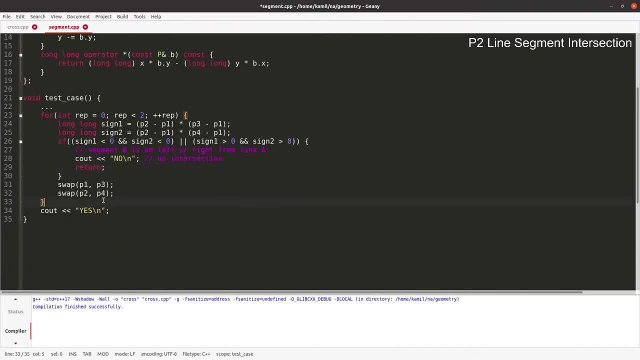 Let's implement this easy part In parallel case. If P2 minus P1.. P4 minus P3. If this cross product is zero, Two segments are parallel. And what do we do If the four points aren't collinear? 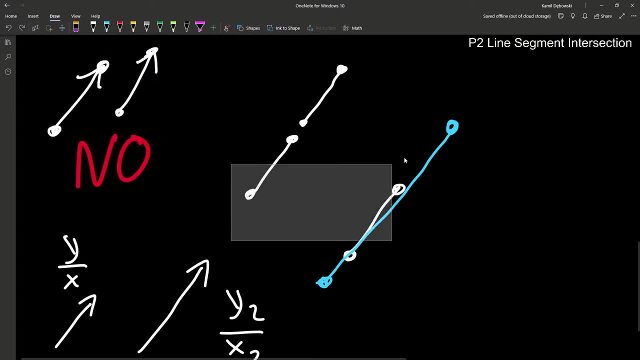 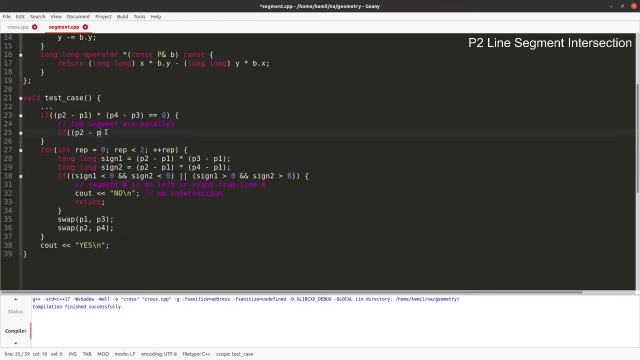 If this is the case, we need to say no, Otherwise it will be one of those two cases. Then it's enough to say If with respect to P1.. P3, let's say If this is not zero. This means that P3 is not collinear with P1 and P2.. 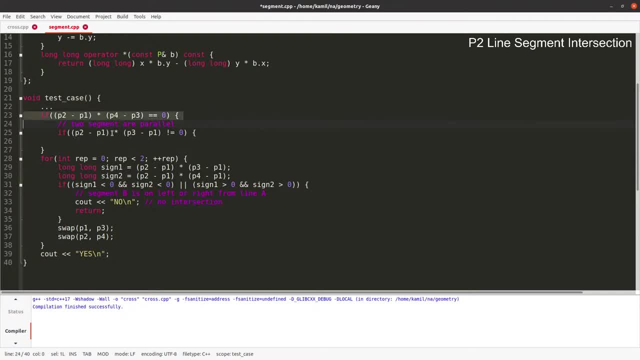 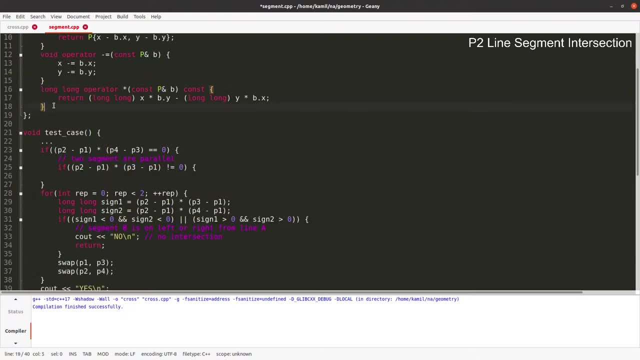 And now I would say I don't know if you agree That all of that becomes a bit tricky to write And it's hard to understand every line. So let's make a helper function Cross. You know, it's maybe a bit confusing. 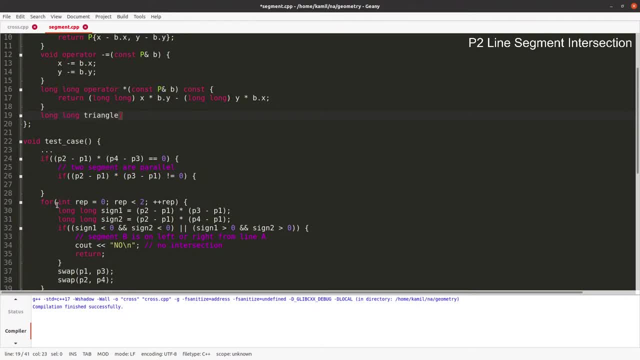 Or triangle, I'm not sure about a good naming. I will explain what it does. If we do this, then our life will become much easier. I say with respect to me: Compare B and C. This refers to myself When I now run. 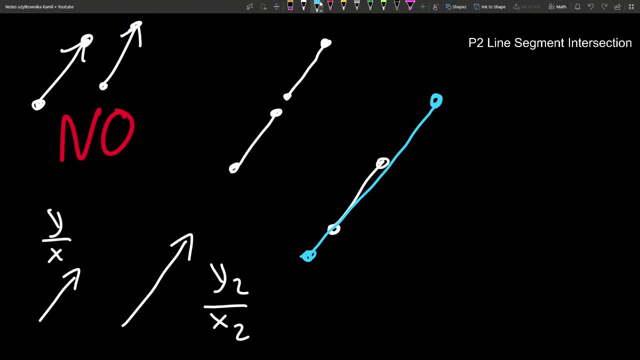 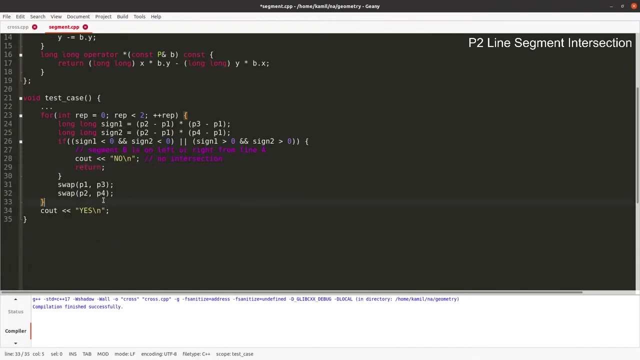 So P2 minus P1. We take this vector- P4 minus P3, and we check if they are parallel. So collinear, meaning the cross product is zero. So let's implement this easy part. So in parallel case, if P2 minus P1, P4 minus P3. 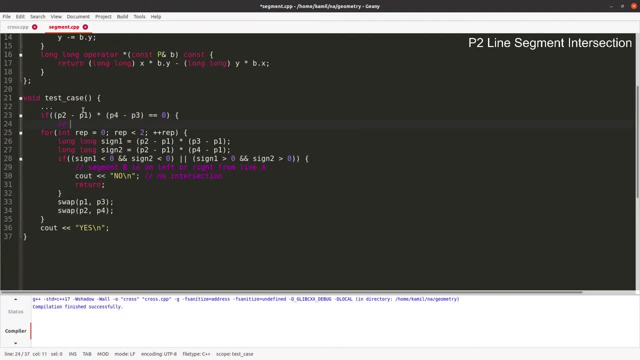 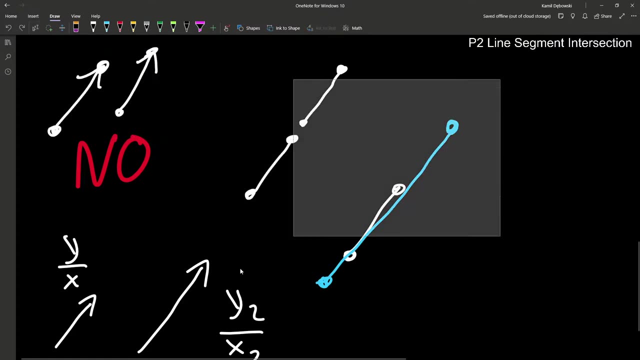 If this cross product is zero, two segments are parallel. And what do we do If the four points aren't collinear, like this is not? If this is the case, we need to say no, Otherwise it will be one of those two cases. 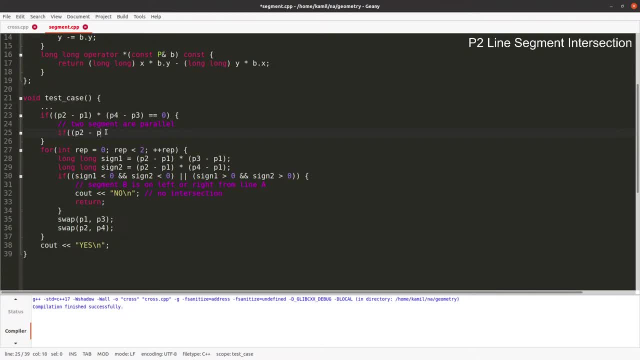 Then it's enough to say: if we respect to P1, P3, let's say, if this is not zero, this means that P3 is not collinear with P1 and P2.. And now I would say- I don't know if you agree that all of that becomes a bit tricky to write. 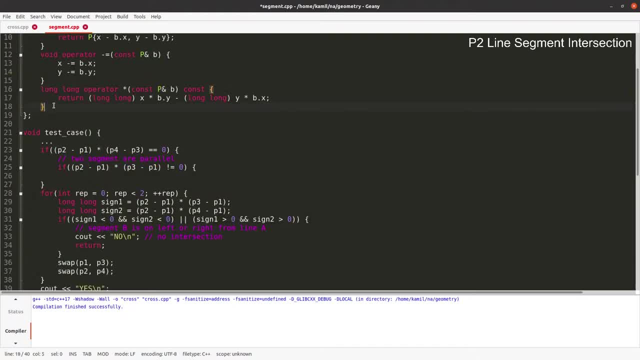 And it's hard to understand every line. So let's make a helper function Cross. you know it's maybe a bit confusing. All right, So let's make a helper function Cross. you know it's maybe a bit confusing. 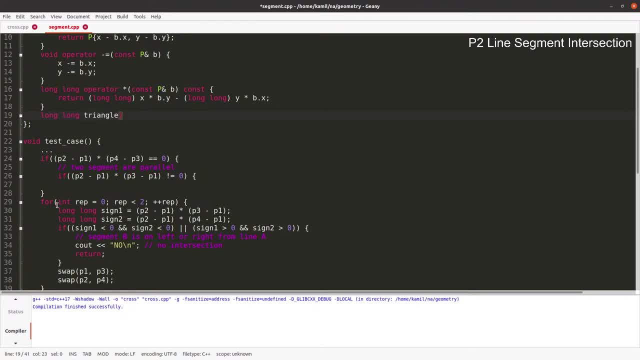 All right Triangle. I'm not sure about a good naming. I will explain what it does. If we do this, then our life will become much easier. I say with respect to me: compare B and C. This refers to myself. 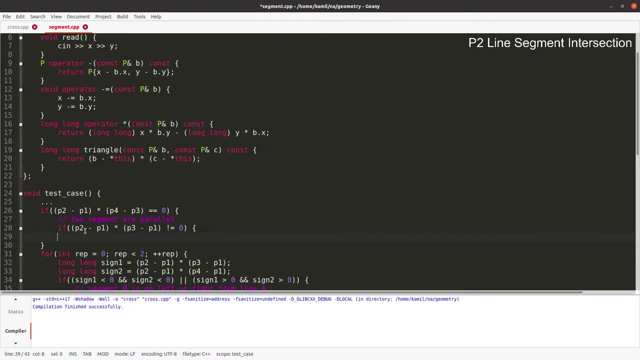 When I now run, this line will be equivalent to that P1.triangle or cross product, however you want to call it. compare P2, P3. Those two lines will mean the same thing. This just boils down to saying: with respect to P1, compare angle of P2 and P3. 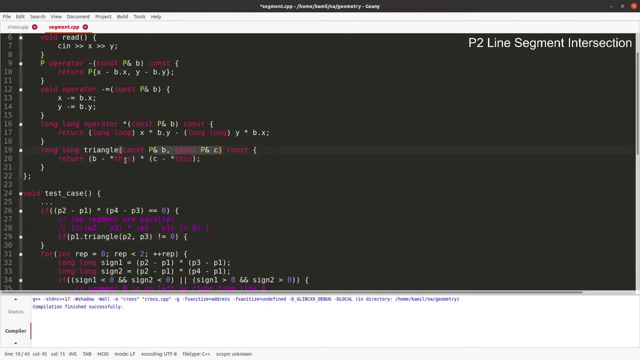 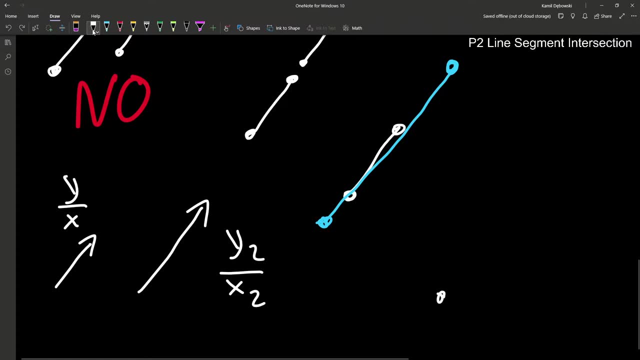 And this is what happens there, Both B and C, the two arguments I subtract from myself. So this function will run. Just do this You're given with respect to P1, P2, P3.. Look from P1 to in both directions and say which one is more on the left. 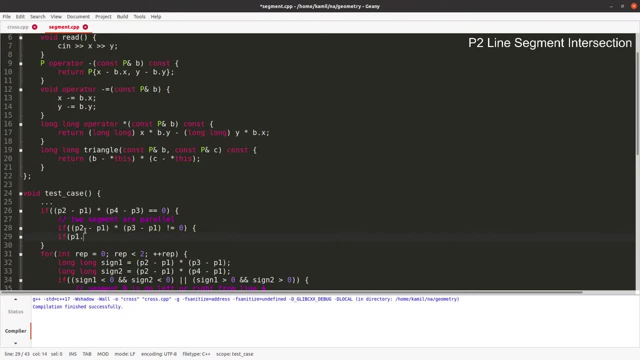 This line will be equivalent to that P1.triangle Or cross product, However you want to call it. Compare P2, P3. Those two lines will mean the same thing. This just boils down to saying: With respect to P1.. 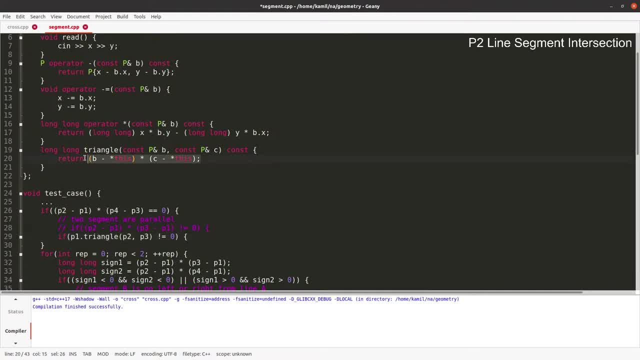 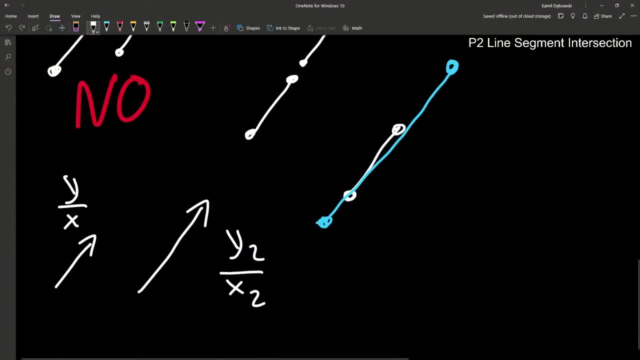 Compare angle of P2 and P3.. And this is what happens there, Both B and C, The two arguments I subtract from myself. This function will just do this You're given With respect to P1.. P2, P3. 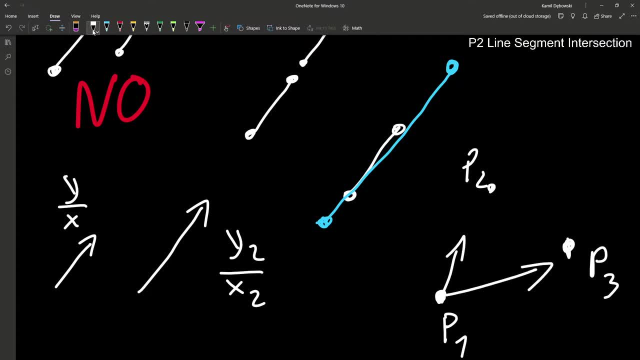 From P1 to in both directions And say which one is more on the left And also say area of this triangle. For that from the very beginning We said we need to assume that this is 0, 0. So we subtract this from P1. 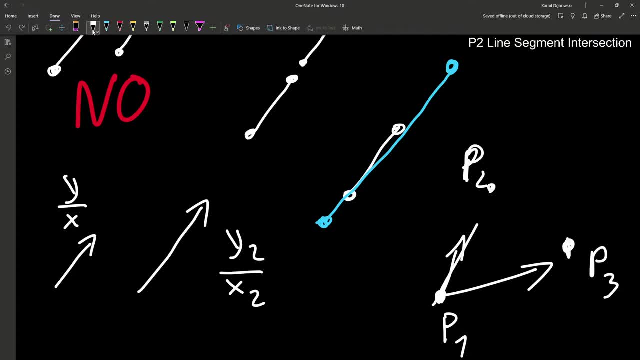 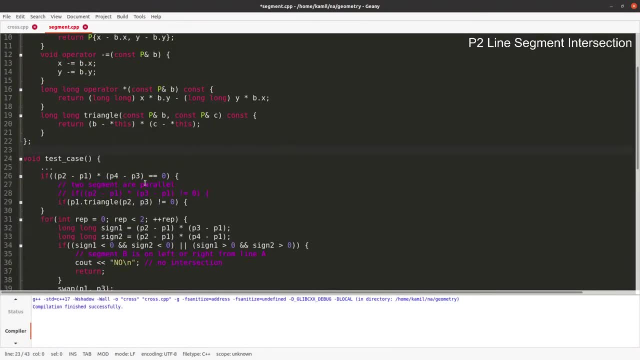 This from P1. And then we take cross product of Two vectors, Basically, And That's it. So if, With respect to P1. P2, P3 aren't left and right, They, I mean They are not collinear. 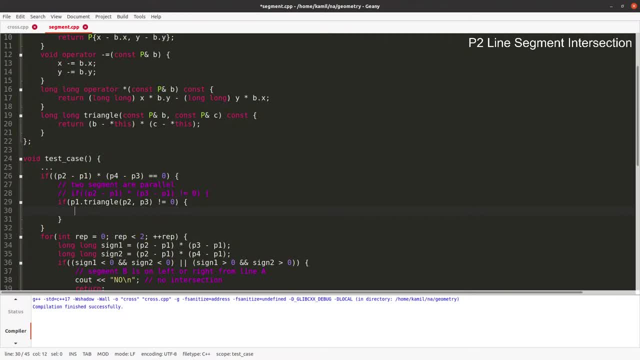 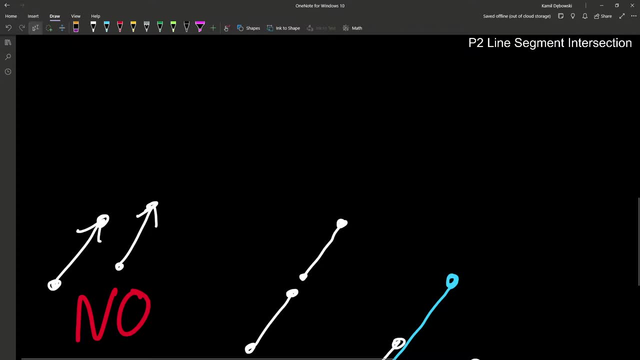 It's not 0. But P2 is on the left from P3. Or the other way around. Then apparently we have this case on the left, When two segments are parallel But the points are not collinear. So we say no. 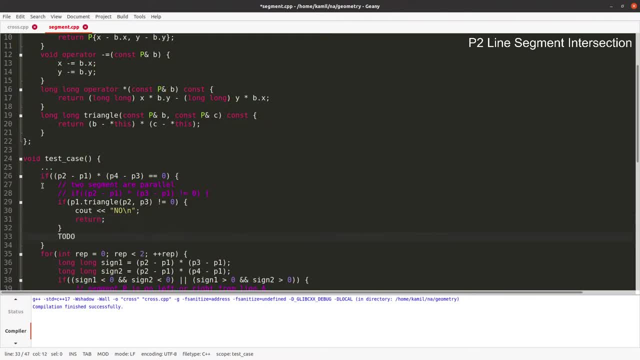 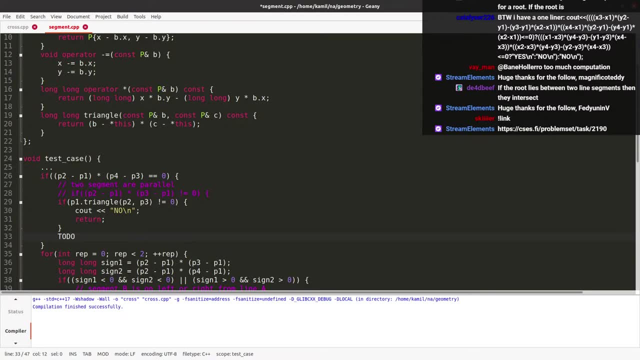 And this is to do? I see a one liner By By whom? By catalyzer, Yes, You can solve problems with like 30, 40 terms, But We don't want to do that. Okay, And this final to do. 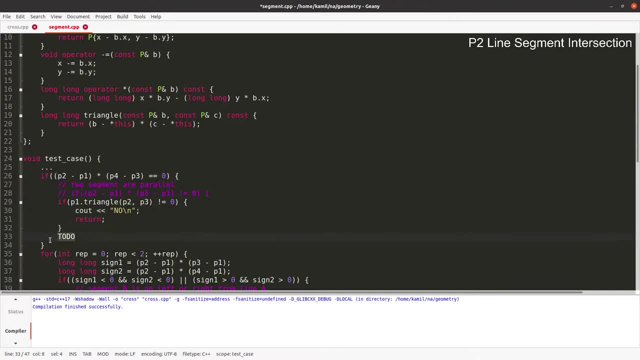 We need to deal with that And there is a nice trick for that. But again, It may be hard to Come up with And you can make a lot of ifs To say If, If you have four points And 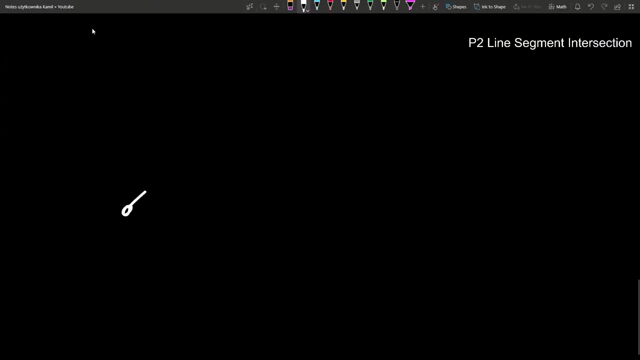 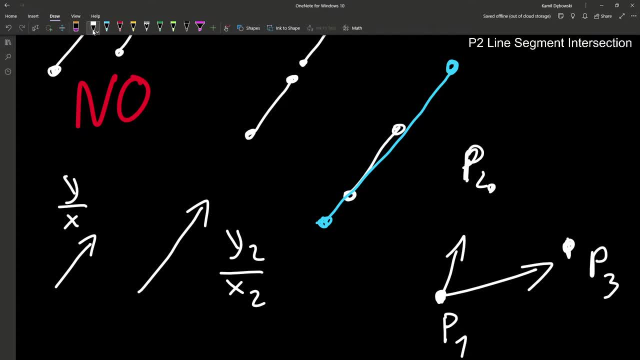 And also say area of this triangle. For that from the very beginning we said we need to assume that this is 0, 0. So we subtract this from P1, this from P1. And then we take cross product of two vectors, basically. 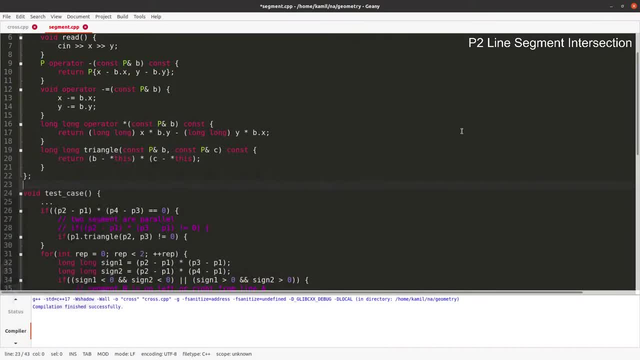 And then we add up this, this to P1.. Remember, this is a cross pattern. So here P1 is in the center and P2 is in the center. So you will know for sure that this is 0, 0.. 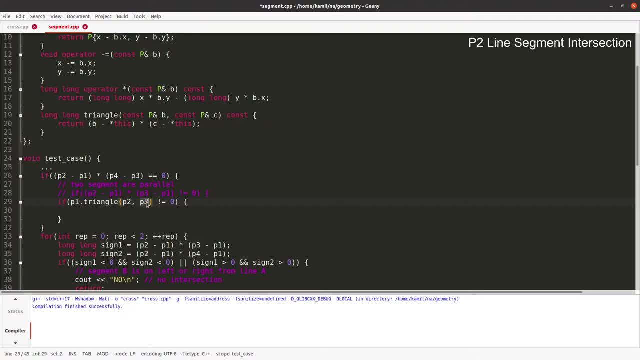 Let's hope that the answer will be the same. Look here And we will do the same same thing here. If we again save this line like this, we're going to И and b. That will give us the same result. Good. 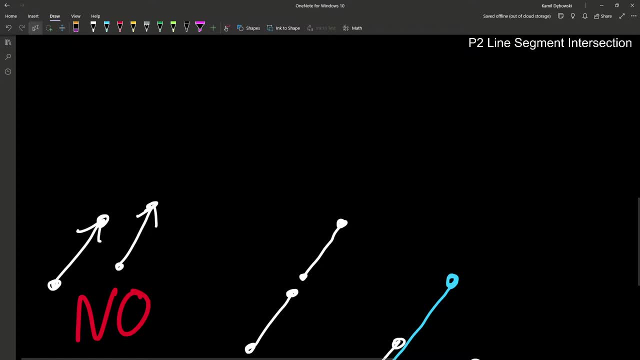 And that's it. So if, with respect to P1, P2, P3 aren't left and right, They- I mean they- are not collinear, it's not 0. But P2 is on the left from P3, or the other way around. 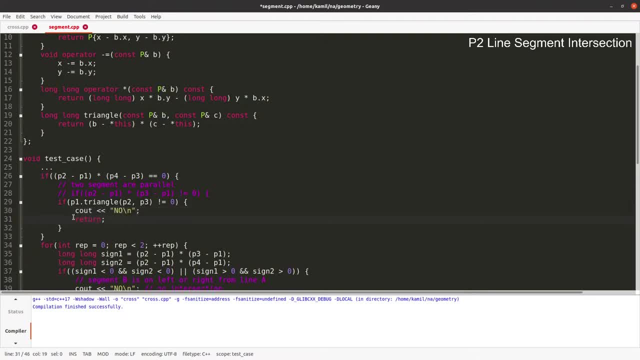 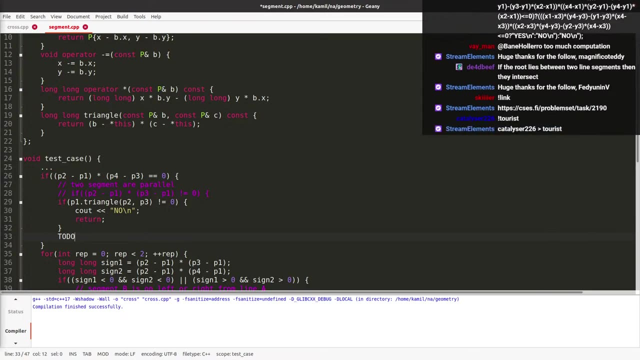 Then apparently, we have this case on the left, when two segments are parallel But the points are not collinear. and this is to do? I see a one-liner: by by whom? by catalyzer, yes, you can solve problems with like 30, 40 terms, but we don't want to do that. okay, and this: 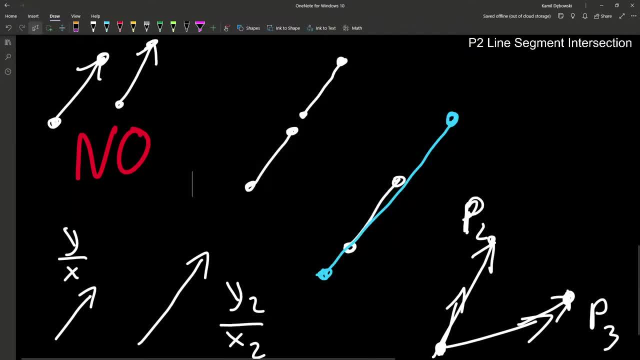 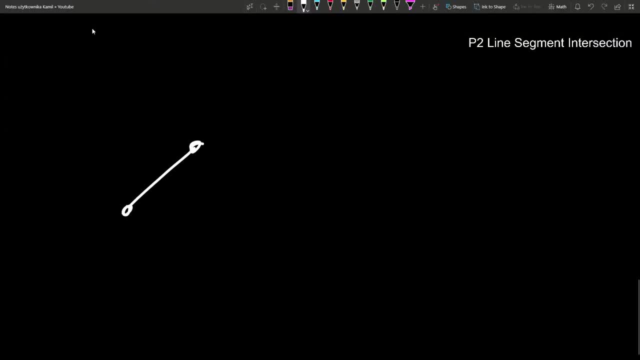 final to do. we need to deal with that and there is a nice trick for that. but again, it may be hard to come up with and you can make a lot of ifs to say if, if you have four points and they are calling here and they create two. 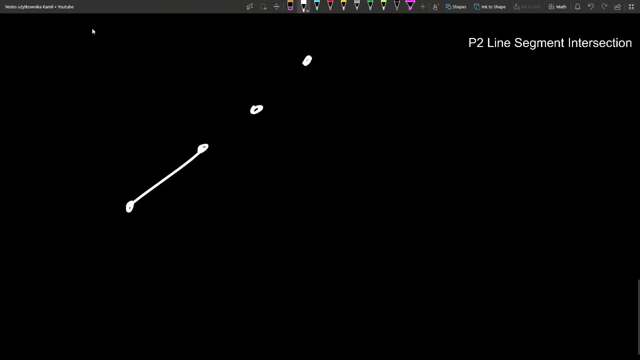 segments only in this case. they do not intersect. in any other pairing like this with that, this with that they do intersect. I curved segments only to for you to see the segments, and this is okay. this case is easiest to check by comparing X coordinates. this is X 1, X 2, X 3 and X 4. then X 2 smaller than X 3 means that 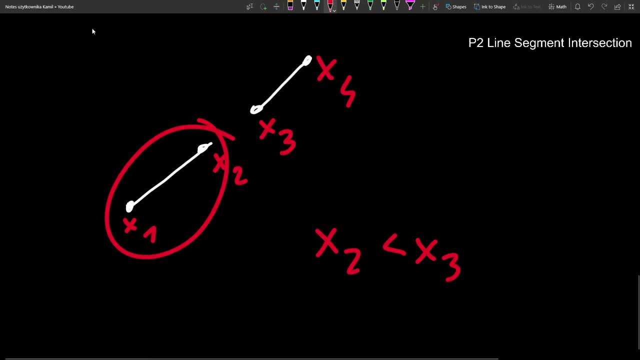 this segment is on the left. if you do something like that, you're crazy, because there are so many possibilities here. like what if they are vertical, then comparing X's isn't a good idea, but what fortunately works is to care about bounding box. bounding box of two points denotes well, vertical. 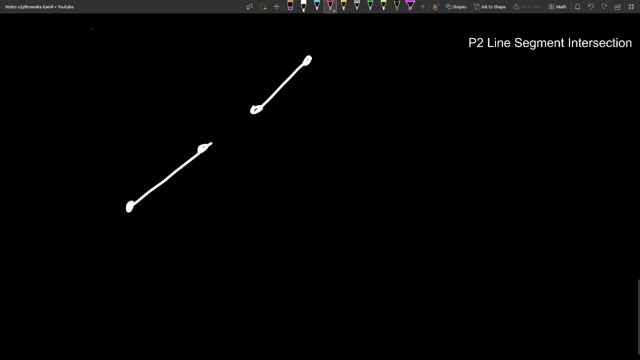 Is En chuck suff control length of। the moment And It will be faster Than if Then it walk through The moment. All this and reading What happened since That the Baby did All these x2 smaller than x3 means that this segment is on the left, if you do. 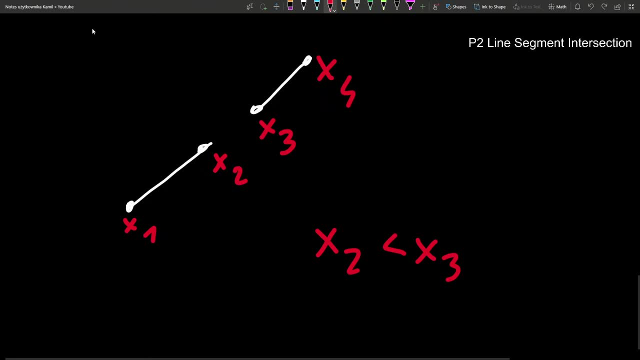 something like that. you're crazy because there are so many possibilities here. like what if they are vertical, then comparing x's isn't a good idea, but what fortunately works is to care about bounding box. bounding box of two points denotes well vertical and horizontal lines that enclose it, and for any group. 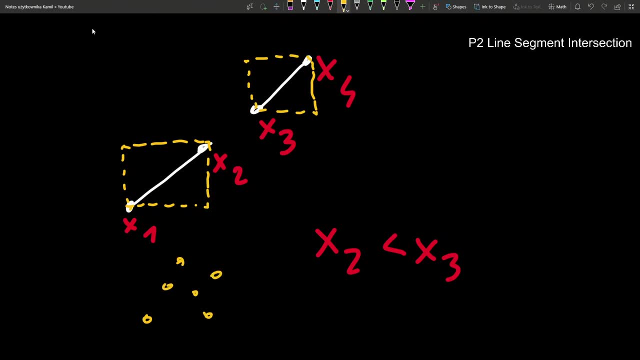 of points. this is just a general technique. for any group of points you can compute the bounding box by grabbing, by finding maximum X, minimum X, minimum Y and maximum Y. and now two boundings box are disjoint: if, and only if, those two segments are disjoint. and it's enough to say that those two bounding box are disjoint. so instead of 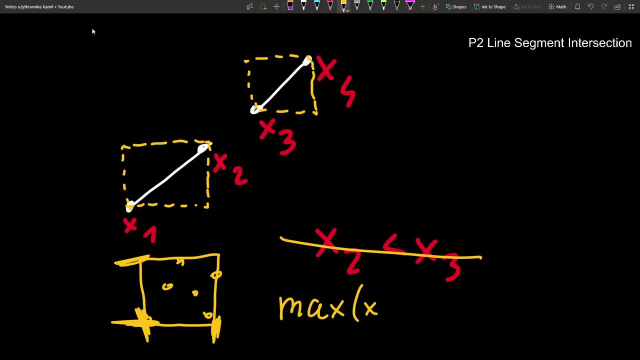 this. we do something more general. max of x1- x2 smaller than mean of x3- x4 say something like that. that's the idea. I will implement exactly what needs to be done here. but the proof of this part boils down to looking at bounding box. 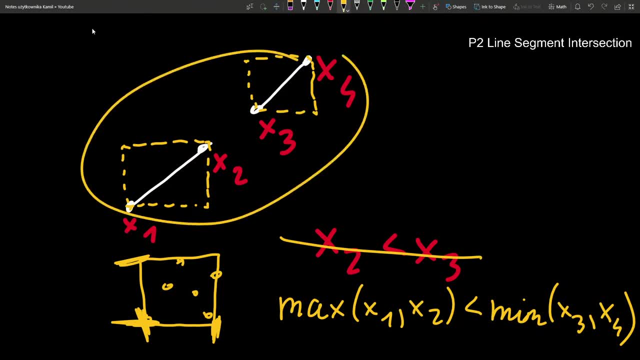 because we don't know which segment is more on the left the case can be. the drawing can look like this: x1, x2, x3, x4 and also wise. in this case, it's stupid to compare x2 smaller than x3. you need to know the orientation, but this works. 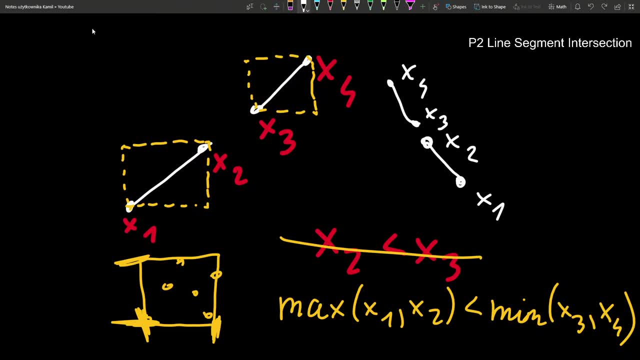 kind of no matter what and to check, basically to check if two rectangles are disjoint, so two bounding boxes. you need to check if x is smaller than x, but this is not enough in this case it isn't, or y is smaller than this y. I will now code it. 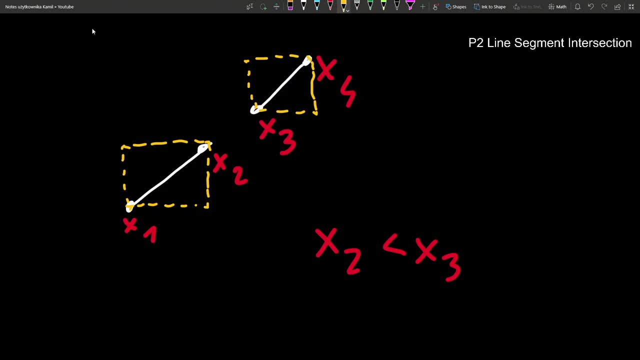 and horizontal lines that enclose it, and for any group of points. this is just a general technique. for any group of points, you can compute the bounding box by grabbing, by finding maximum X, minimum X, minimum Y and maximum Y, and you can find the bounding box by doing this and now two bounding box are disjoint, if and. 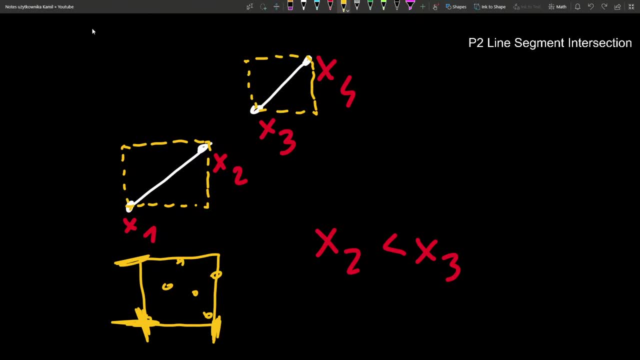 only if those two segments are disjoint, and it's enough to say that those two bounding box are disjoint. so instead of this, we do something more general: max of X 1 X 2 smaller than min of X 3 X 4. that's the idea I will implement, exactly what needs to be done here. but 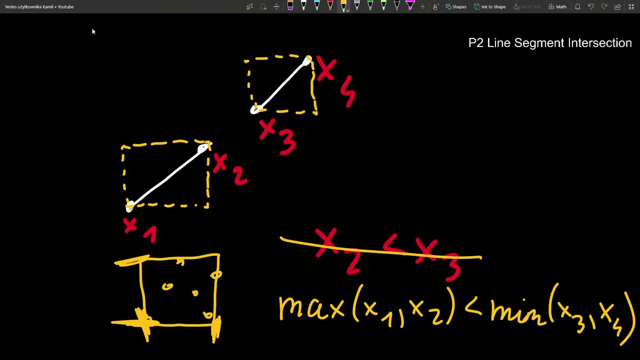 the proof of this part boils down to looking at bounding boxes. we don't know which segment is more on the left the case can be. the drawing can look like this: X 1, X 2, X 3, X 4 and also Y's. in this case, it's stupid to compare X 2. 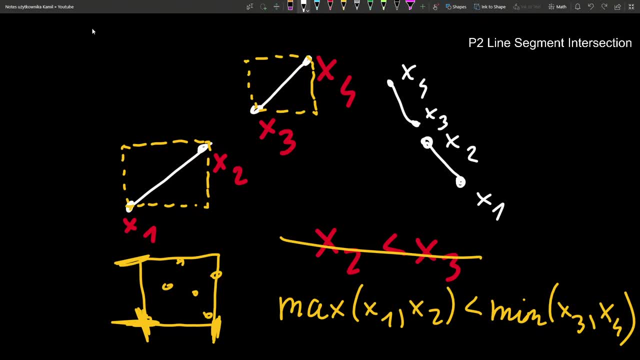 smaller than X 3. you need to know the orientation, but this works kind of no matter what and to check, basically to check if two rectangles are disjoint to two bounding boxes. you need to check if X is smaller than X, but this is not enough in this case it isn't, or Y is smaller. 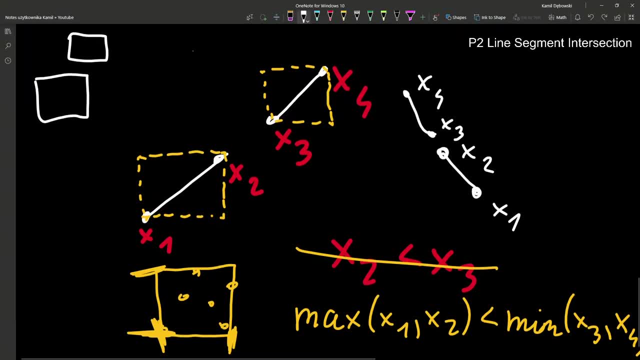 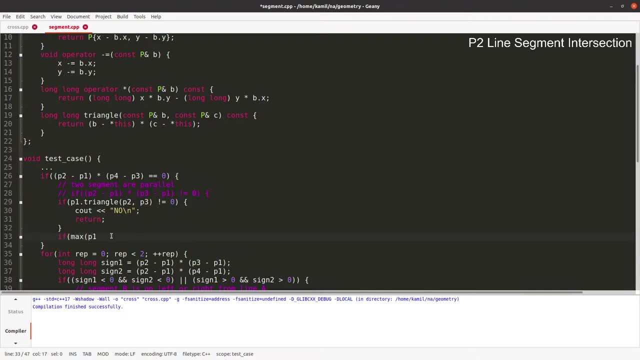 than this Y. I will now code it and then get back to drawing to explain max of p1.x, p2.x. if this is smaller than minimum of p3.x, p4.x, then for sure it's disjoint, Because apparently one segment is completely on the left from the other, Or 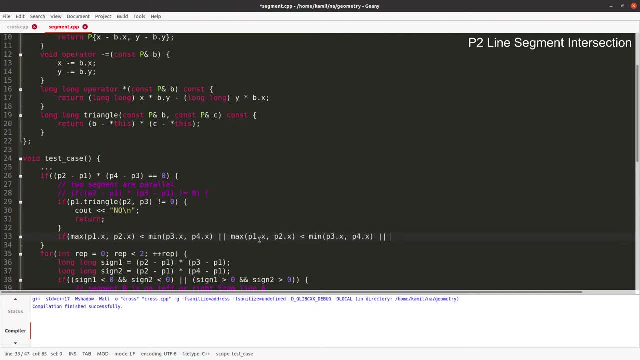 and now, for the first time today, I'm copy pasting. I think it's for the first time, Or this now. this way, we checked if the first segment is completely more to the bottom, And also there are cases like the other way around and I can copy paste and change p3, p4. 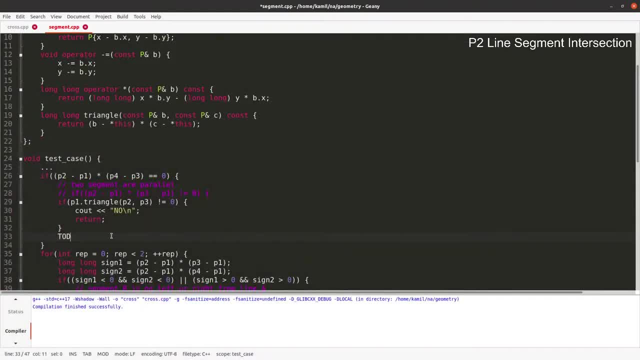 and then get back to drawing to explain max of p1.x, p2.x. if this is smaller than minimum of p3.x, then for sure its disjoint because apparently one segment is completely on the left from the other. and now, for the first time today, I'm copy-pasting. I think it's for the first time. 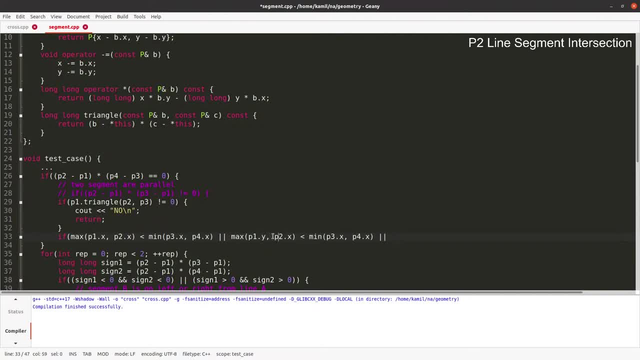 or this. now, this way we checked if Vincent segment is completely more to the bottom and also this tease is the same and we have not checked out new links. we're not gonna do that. in the next time we will show also the first argument here so that we are completelyテiera quantic 15 y. 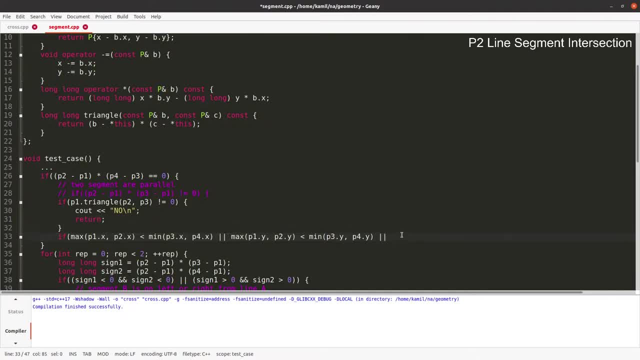 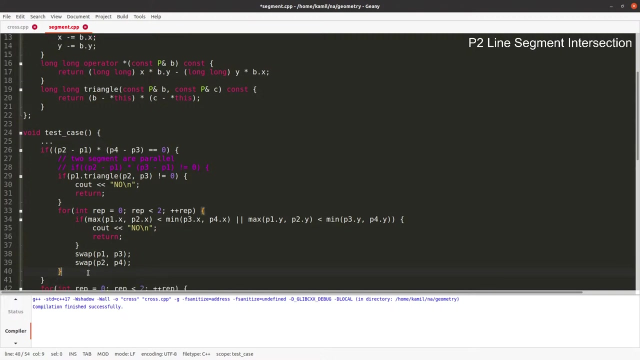 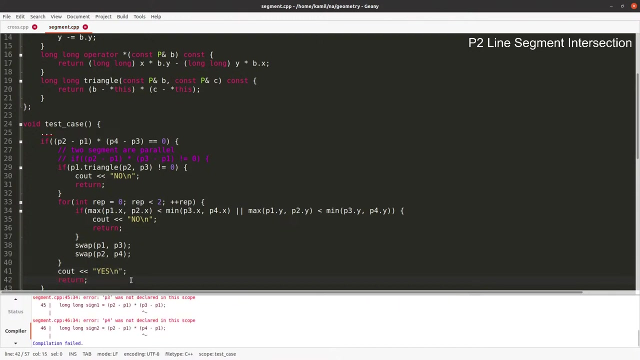 there are cases like the other way around and I can copy paste and change p3, p4 and so on, but again I'm not going to because that's ugly. instead, repeat twice: if this no intersection and after checking this, swap the two segments. nothing was detected, then yes, and now it's done. what? oh yeah, I need to make it. 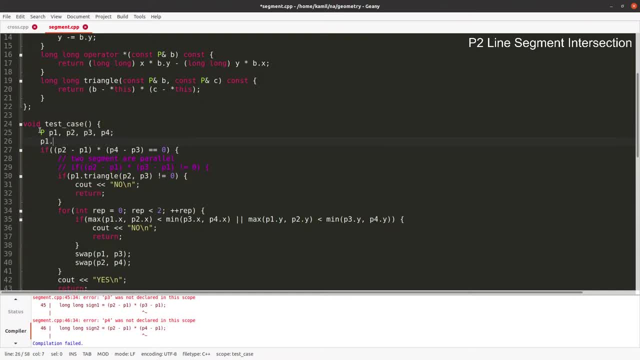 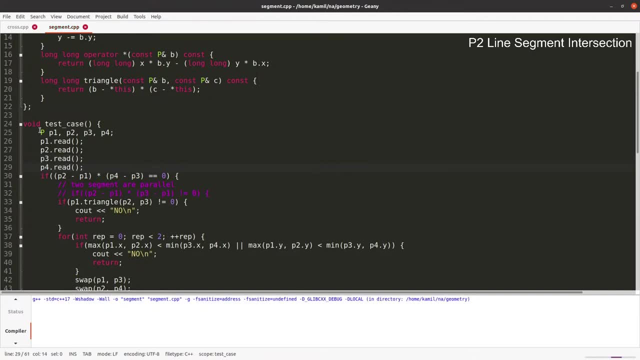 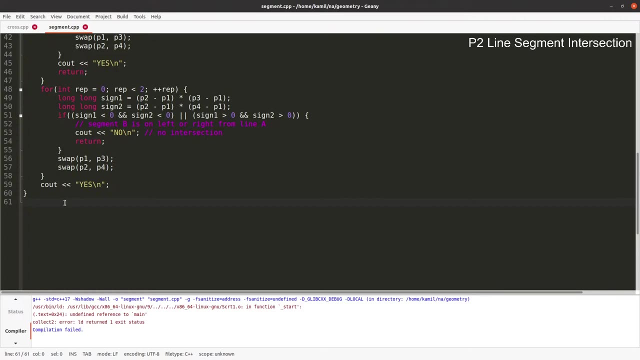 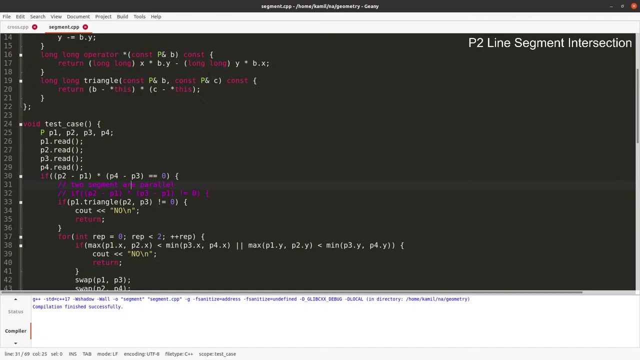 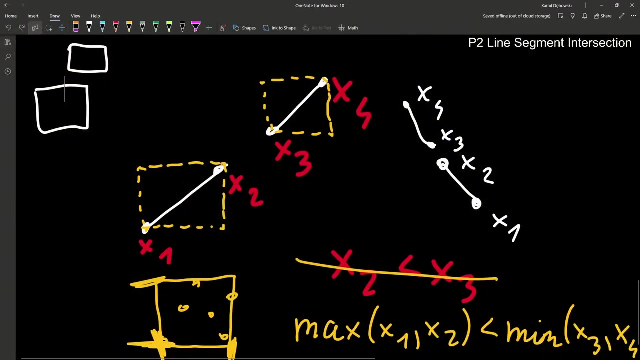 compile. maybe now it would be better to make it into an array, make a for loop. I don't have main main. I will copy from the other. all right done, I will refer. I see some ideas about distances in the chat. I will answer that. just let me finish here. general technique that we used is just: 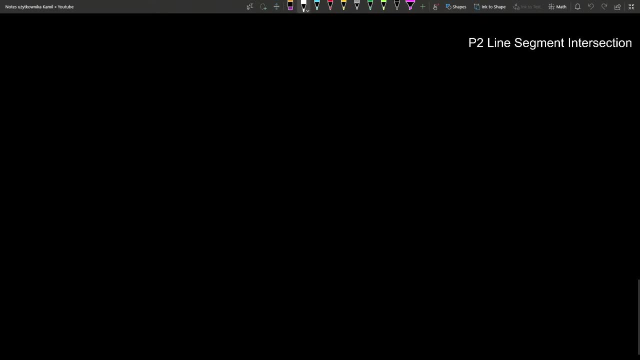 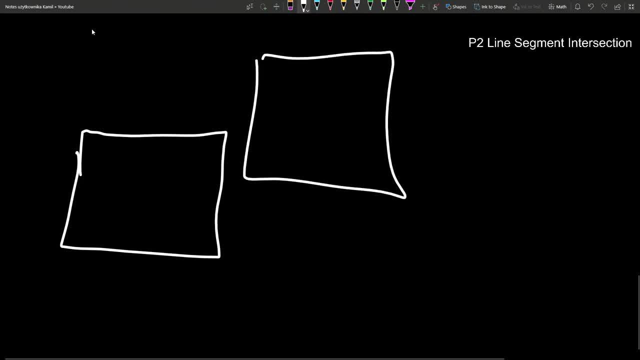 mini mini technique. two rectangles are mini mini technique. two rectangles are mini mini technique. two rectangles are disjoint if, and only if, the max Y of one disjoint, if and only if the max Y of one disjoint, if, and only if the max Y of one rectangle is on the left from mean Y of. 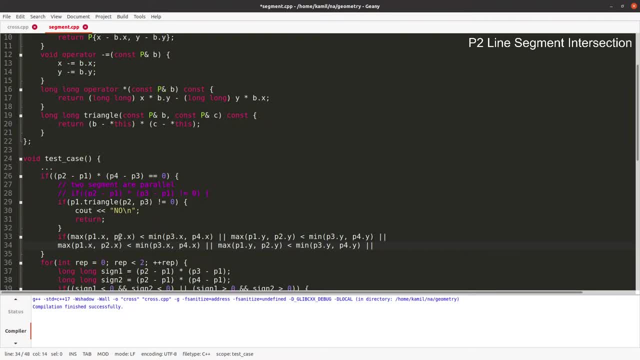 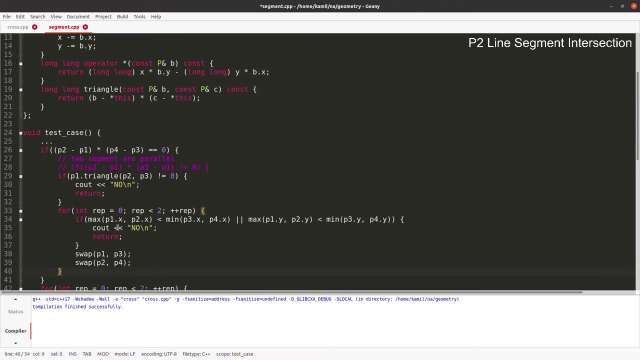 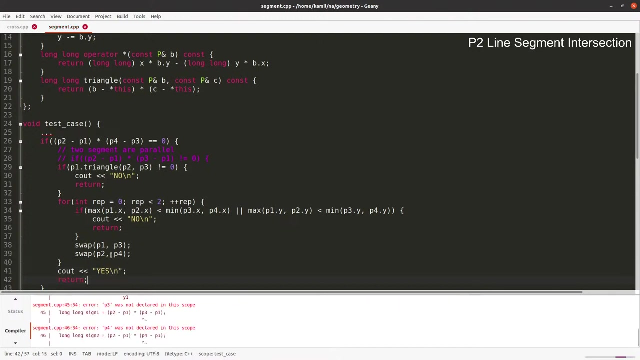 and so on, But again, I'm not going to Because that's ugly. Instead, repeat twice. If this no intersection, and after checking this, swap the two segments. If nothing was detected, then yes. And now it's done. I need to make it compile. 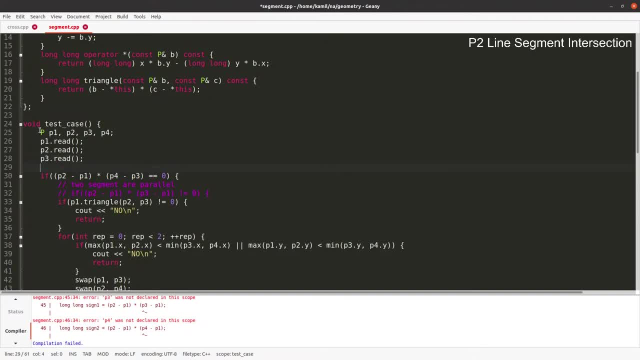 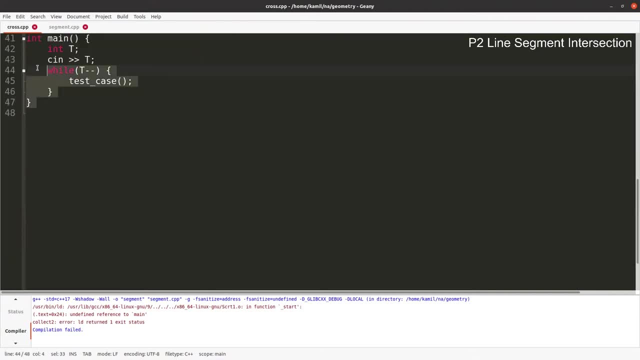 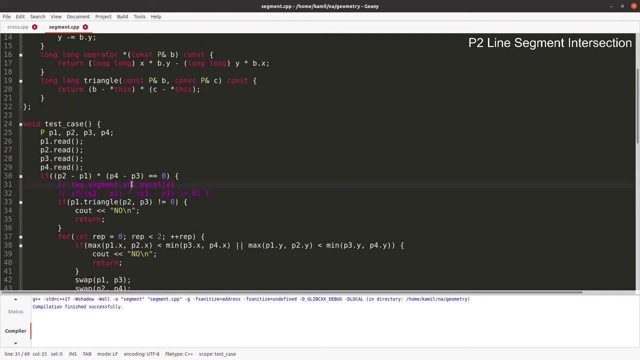 Maybe now it would be better. It would be better to make it into an array, Make a for loop. I don't have main Main, I will copy from the other. Alright Done, I will refer. I see some ideas about distances in the chat. 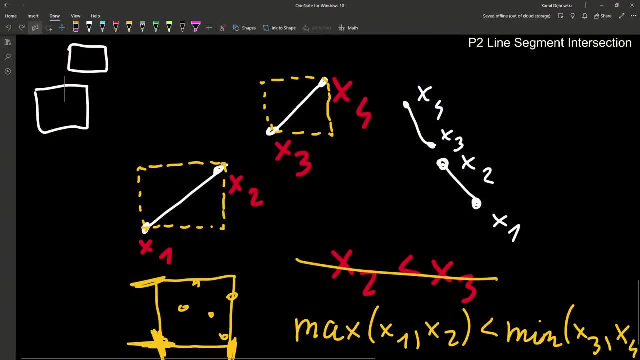 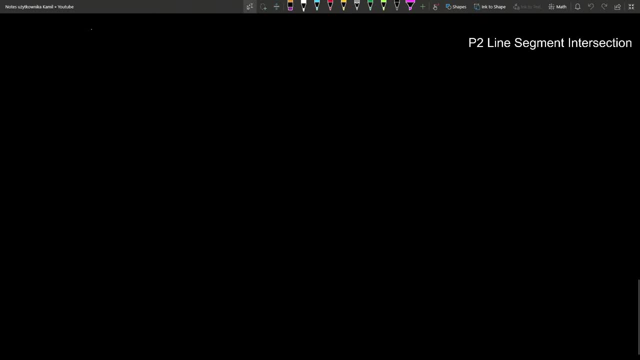 I will answer that. Just let me finish here. General technique that we used is just grabbing bounding boxes. They are defined by minx and maxx, miny and maxy. And now general solution to say if two rectangles intersect or not, Which can be another problem. It is a useful mini technique. 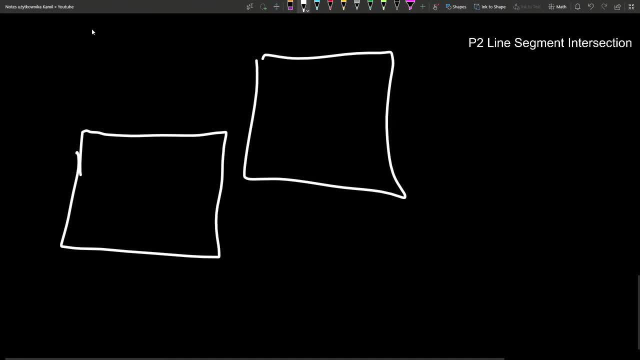 Two rectangles are disjoint if, and only if, the maxy of one rectangle is on the left from miny of the other, So y2 smaller than y3. Kind of Or Like. this is not true if this is the case, But in this. 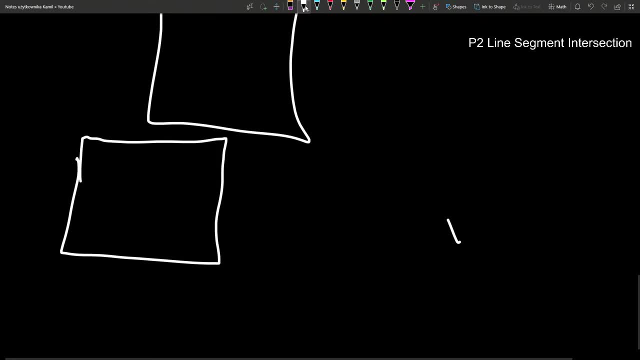 Sorry, I needed to say x's. A moment ago. I said x, I wanted to say this. And in this case y2 smaller than y3. This checks Kind of if If there is a vertical, A horizontal line between them. 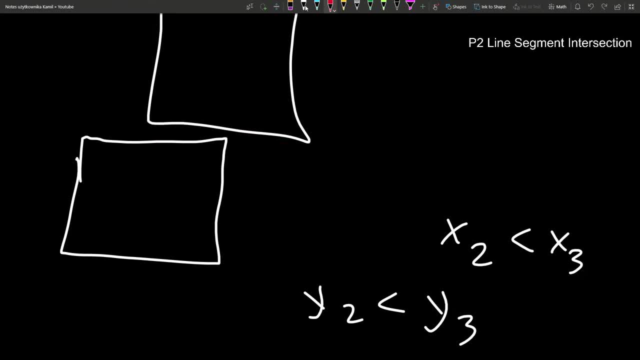 And if there is a vertical line between them. If not, then Apparently they intersect Like that. There are other ways to look at it And also, I don't claim that this is the only solution for the problem, But it's one of many. 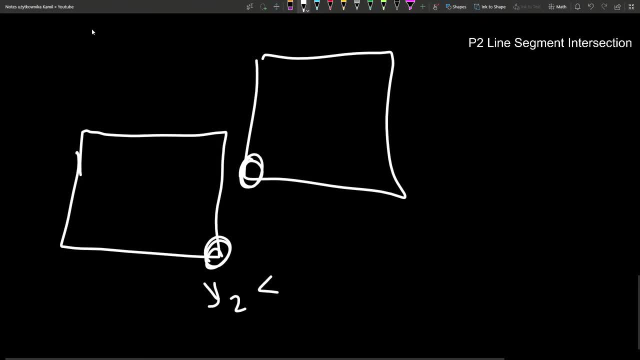 rectangle is on the left from mean Y of rectangle is on the left from mean Y of the other. so y2 smaller than y3 kind of the other. so y2 smaller than y3 kind of the other. so y2 smaller than y3 kind of or like. this is not true. if this is the 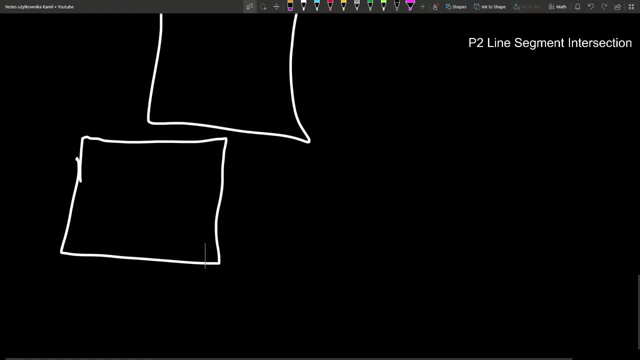 or like this is not true if this is the. or like this is not true if this is the case. but in this, sorry, I needed to say case. but in this, sorry, I needed to say case. but in this, sorry, I needed to say X's. a moment ago I said X. 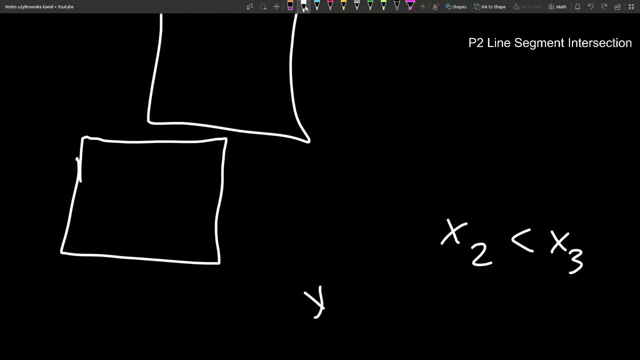 X's. a moment ago. I said X's. a moment ago, I said X's. X's. a moment ago, I said X's, I wanted to say this. and in this case, y2, I wanted to say this. and in this case, y2, I wanted to say this. and in this case, y2 smaller than y3. this checks kind of if. 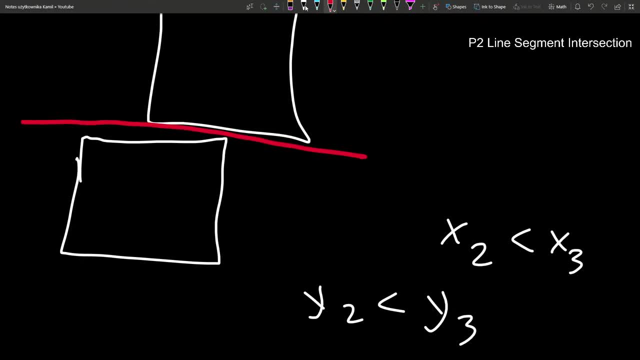 smaller than y3, this checks kind of. if smaller than y3, this checks kind of if. if there is a vertical horizontal line, if there is a vertical horizontal line, if there is a vertical horizontal line between them and if there is a vertical between them and if there is a vertical. 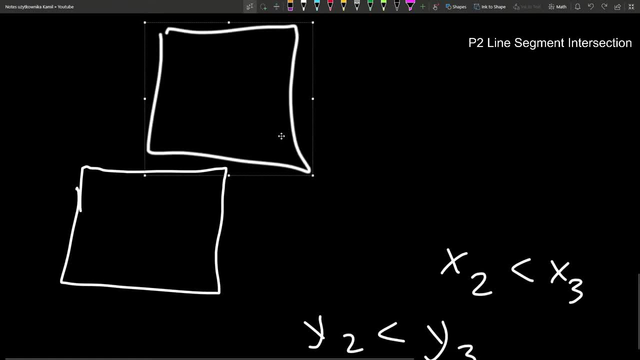 between them and if there is a vertical line between them, if not, then apparently line between them. if not, then apparently line between them. if not, then apparently they intersect. there are other ways to they intersect, there are other ways to they intersect, there are other ways to look at it and also I don't claim that 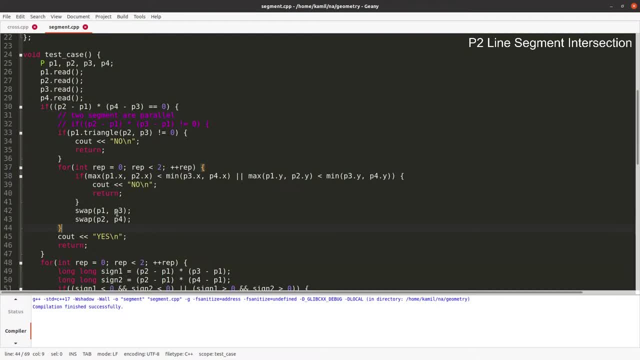 look at it. and also I don't claim that. look at it. and also I don't claim that this is the only solution for the. this is the only solution for the. this is the only solution for the problem. but it's one of men. this is check. 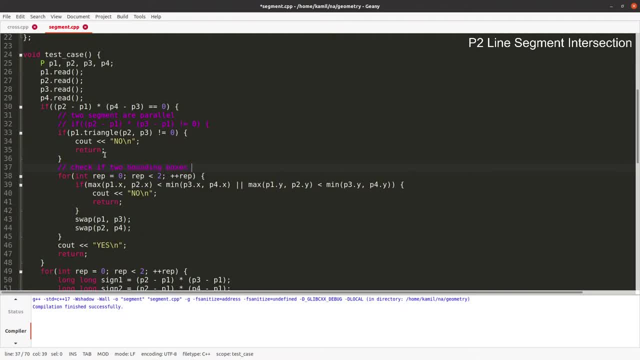 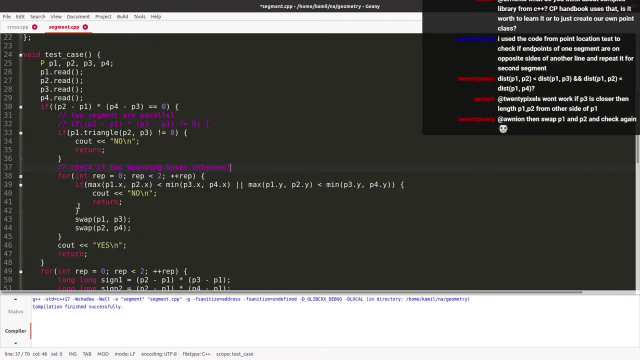 problem, but it's one of men. this is check problem, but it's one of men. this is check. if two bounding boxes intersect, now I. if two bounding boxes intersect, now I. if two bounding boxes intersect now I, will answer chat a little bit complex. will answer chat a little bit complex. 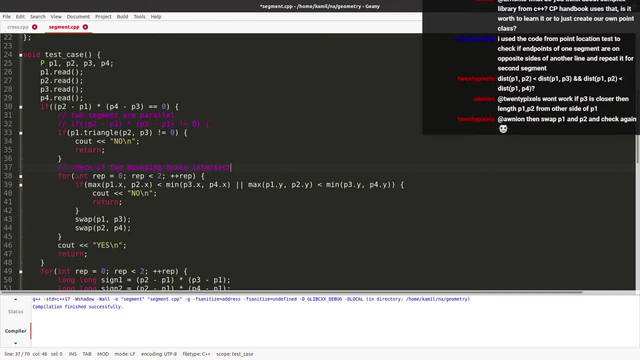 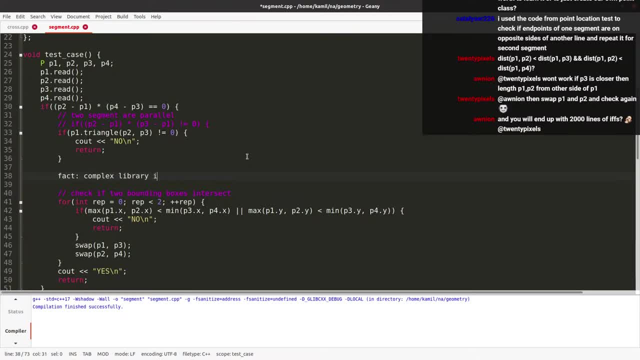 complex library from C++ is slow. interesting fact: complex library from C++ is slow. interesting fact: complex C++ complex library is slow. don't use complex library from C++ is slow. interesting fact: complex library is slow. don't use complex library from C++ is slow. don't use it for non non easy problems somebody. 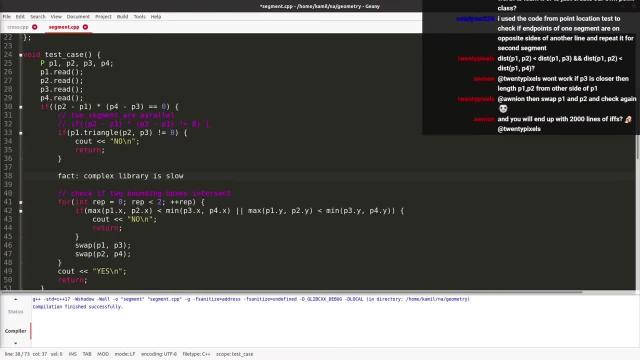 it for non non easy problems. somebody it for non non easy problems. somebody wants to compare distances. I mean you wants to compare distances. I mean you wants to compare distances. I mean you don't. well, you for sure there are, don't well you for sure there are. 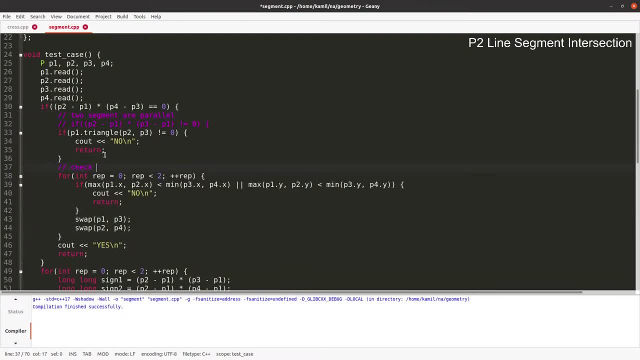 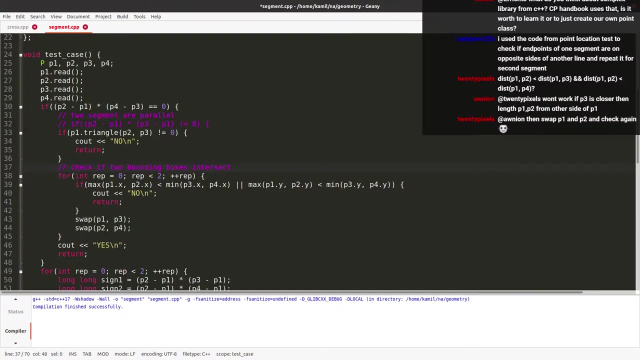 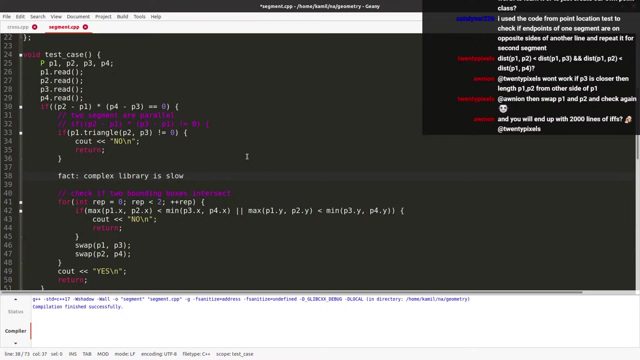 This is check if two bounding boxes intersect. Now I will answer chat a little bit. Complex library from C++ is slow. Interesting fact: C++ complex library is slow. Don't use it for non-easy problems. Somebody wants to compare distances. 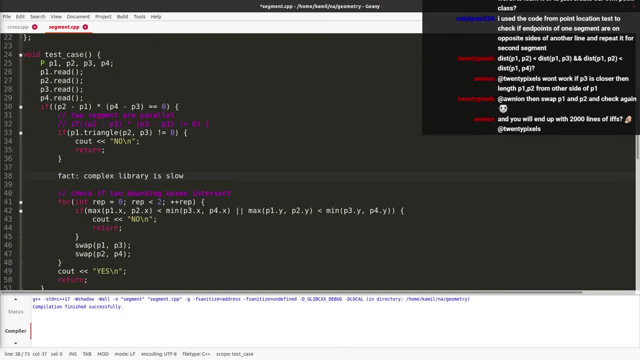 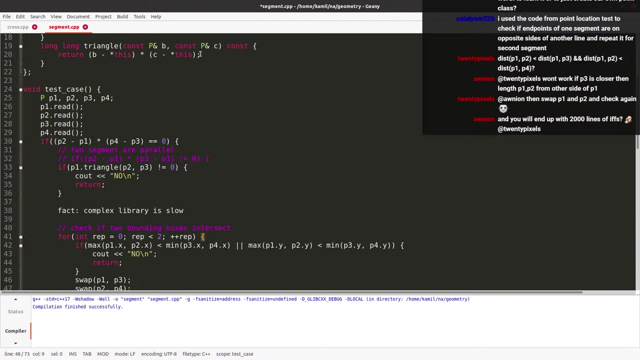 And I mean You don't. Well, For sure, there are alternatives to this, But notice how computation, Computational, Computational light, This solution is. I don't compare any distances, I only compare. Cross product is fast Because it doesn't use any division. 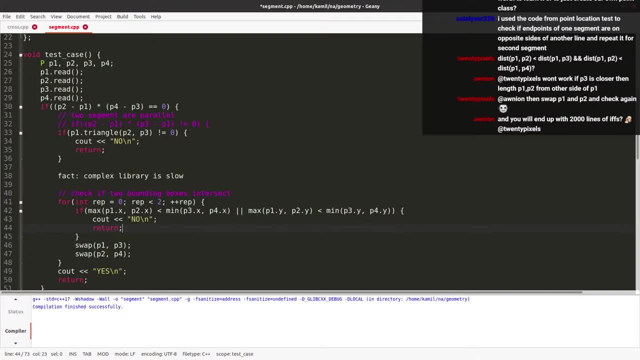 So it's just elegant. You can do everything in geometry with cross product. I don't really want to figure out If your if is enough- 20 pixels, Maybe Onion apparently found a counter example. I don't. You don't want to have a lot of ifs. 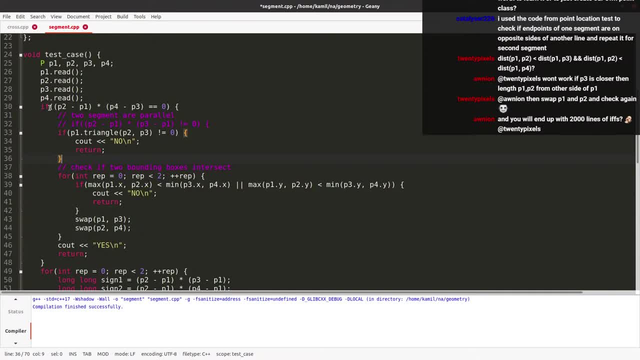 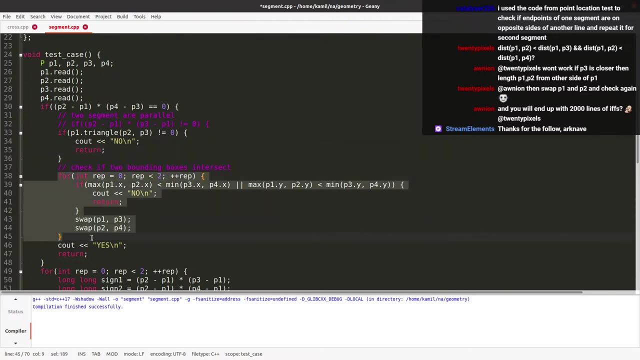 Summary of my code is Is this: If two segments are Parallel, Then If they are not collinear, One segment is next to the other. Otherwise, We need to check If bounding boxes intersect, And you can do it in different ways. 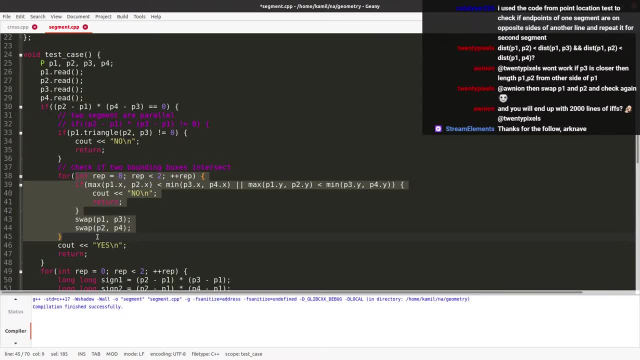 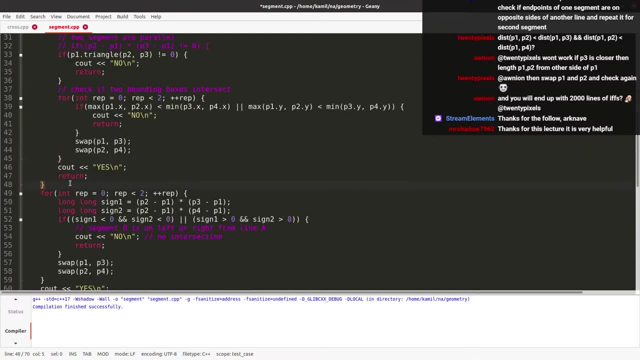 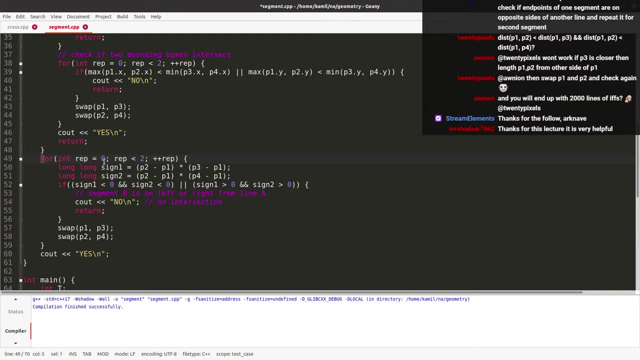 This is not a hard problem. It's not geometry. Given two rectangles, Check if they intersect Other. This is end of if For parallel case. Now, if the two segments are not parallel, Then you need to check If B is completely on the right from A. 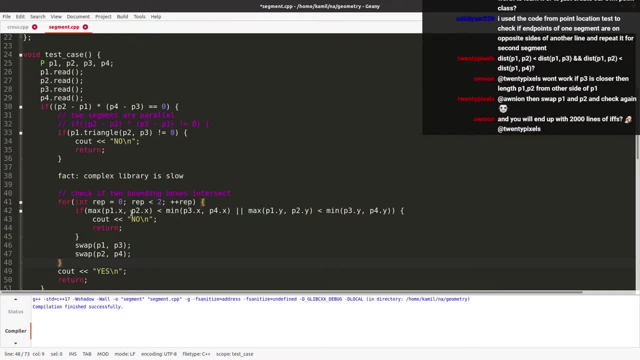 don't. well, you for sure, there are alternatives to this, but notice how alternatives to this. but notice how alternatives to this. but notice how computation and computational computation, computation and computational computational computation and computational computational computation light. this solution is I- computational light. this solution is I, computational light. this solution is I don't compare any. 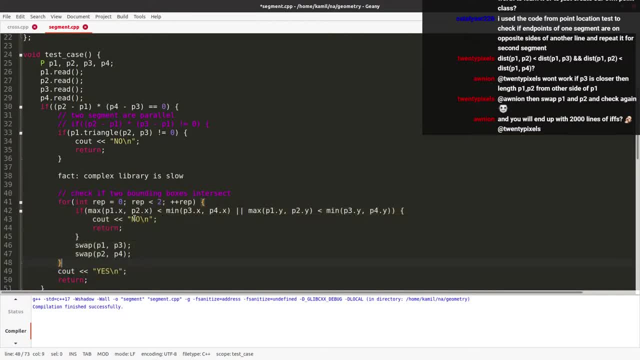 don't compare any. don't compare any distances. I only compare like cross product distances. I only compare like cross product distances. I only compare like: cross product is fast because it doesn't use any, is fast because it doesn't use any, is fast because it doesn't use any division. so it's just elegant, you can do. 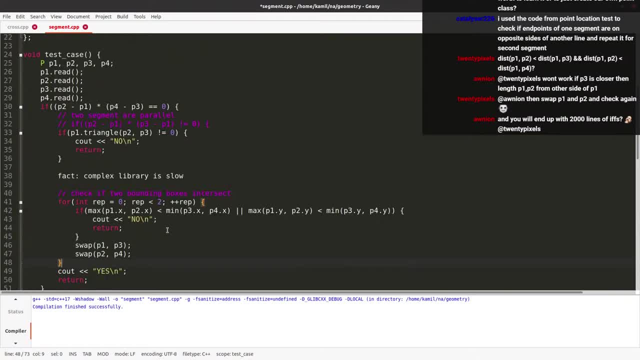 division, so it's just elegant. you can do division, so it's just elegant. you can do everything in geometry with cross, everything in geometry with cross, everything in geometry with cross. product almost everything. I don't really product almost everything. I don't really product almost everything. I don't really want to figure out if your if is enough. 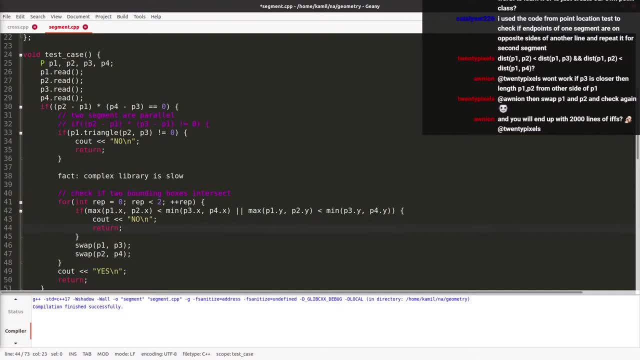 want to figure out if your if is enough. want to figure out if your if is enough: 20 pixels. maybe I've onion apparently 20 pixels. maybe I've onion apparently 20 pixels. maybe I've onion apparently found a country example. yeah, you don't found a country example. yeah, you don't. 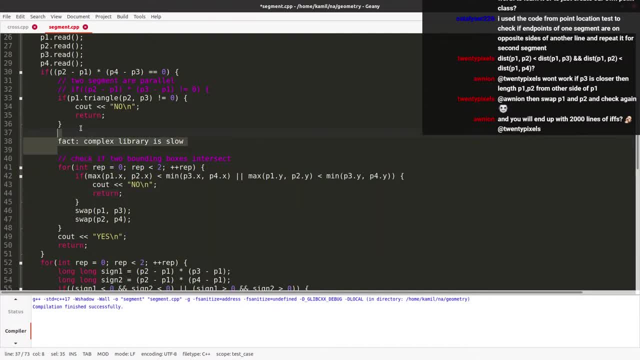 found a country example. yeah, you don't want to have a lot of it's summary of my. want to have a lot of it's summary of my. want to have a lot of it's summary of my. code is: is this, if two segments are, code is: is this if two segments are: 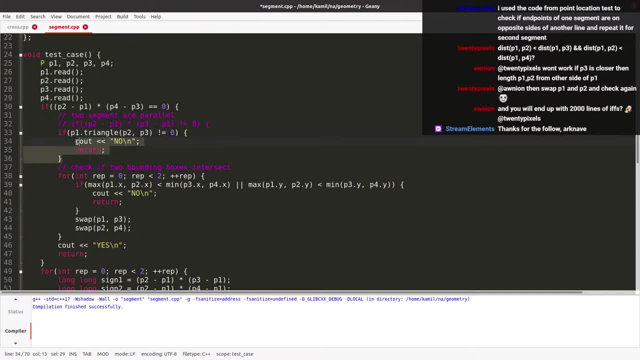 code is: is this: if two segments are parallel, then if they are not collinear parallel, then if they are not collinear parallel, then if they are not collinear. one segment is next to the other, then we one segment is next to the other, then we one segment is next to the other, then we say no. otherwise we need to check if 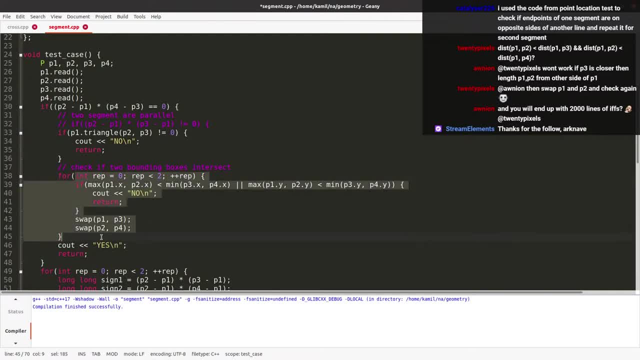 say no, otherwise we need to check. if say no otherwise, we need to check. if bounding boxes intersect and you can do bounding boxes intersect and you can do bounding boxes intersect and you can do it in different ways. this is not a hard, it in different ways. this is not a hard. 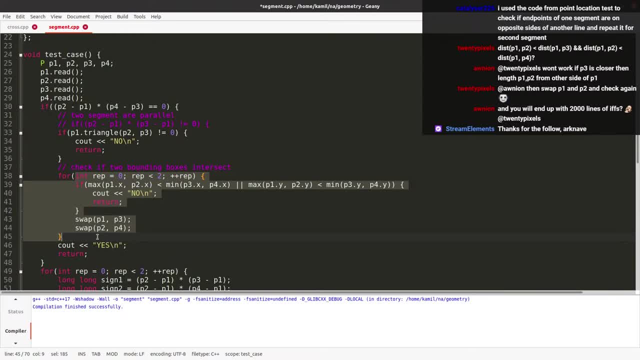 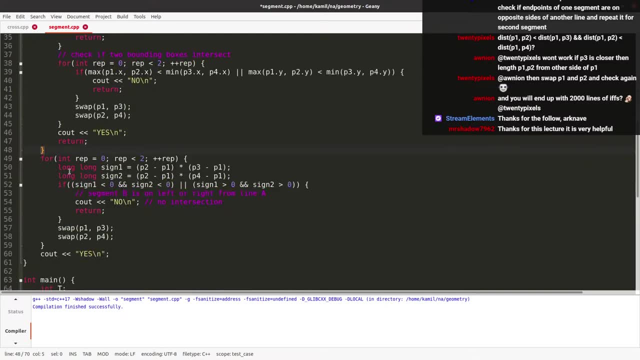 it in different ways. this is not a hard problem. it's not geometry. you given two problem. it's not geometry: you given two problem. it's not geometry: you given two rectangles. check if they intersect other rectangles. check if they intersect other rectangles. check if they intersect other. this is end of if for parallel case now. 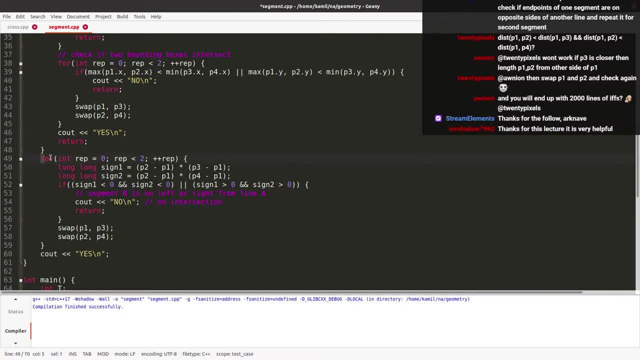 this is end of if for parallel case now. this is end of if for parallel case now. if the two segments are not parallel. if the two segments are not parallel, if the two segments are not parallel, then you need to check if B is, then you need to check if B is. 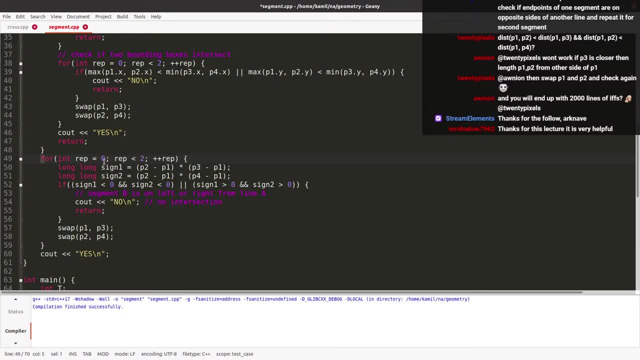 then you need to check if B is completely on the right from a or on the completely on the right from a, or on the completely on the right from a or on the left, and then on the other way around, left and then on the other way around. 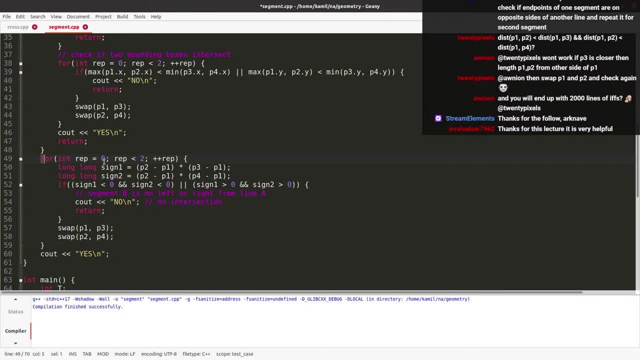 left and then on the other way around. if what I said, if a is on the left or if what I said, if a is on the right, or if what I said, if a is on the right or right from B and if B is on the right or 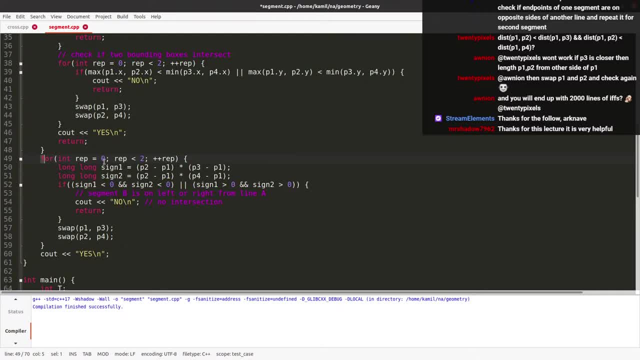 right from B and if B is on the right or right from B, and if B is on the right or left from a. now it's done, of course. the left from a- now it's done, of course. the left from a- now it's done, of course. the problem could be easier. they could say: 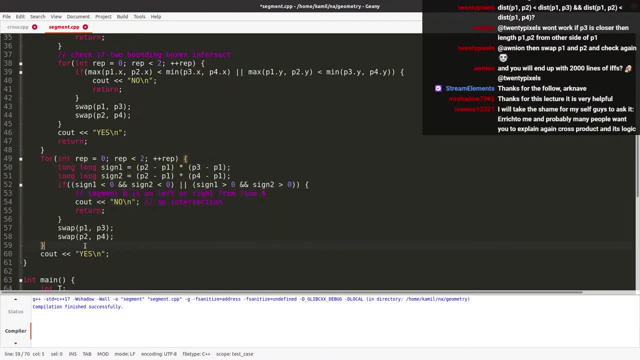 problem could be easier. they could say: problem could be easier. they could say: nothing is collinear, then you would have nothing is collinear, then you would have nothing is collinear, then you would have. just that, by the way. imagine how this, just that, by the way. imagine how this. 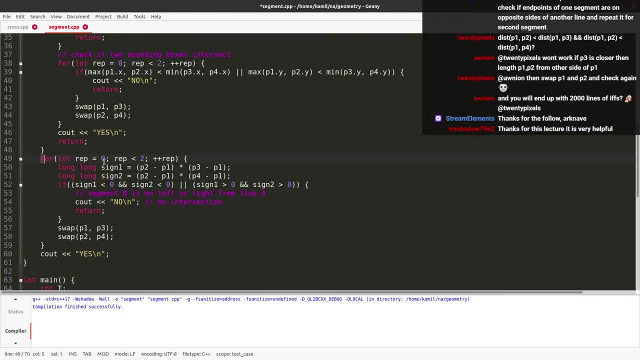 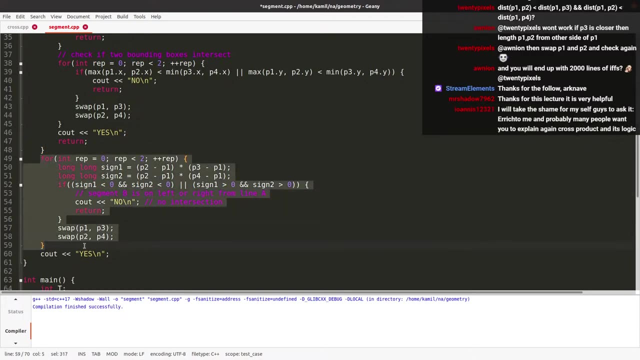 Or on the left. If What I said, If A is on the left or right from B And if B is on the right or left from A, Now it's done. Of course, The problem could be easier. They could say: 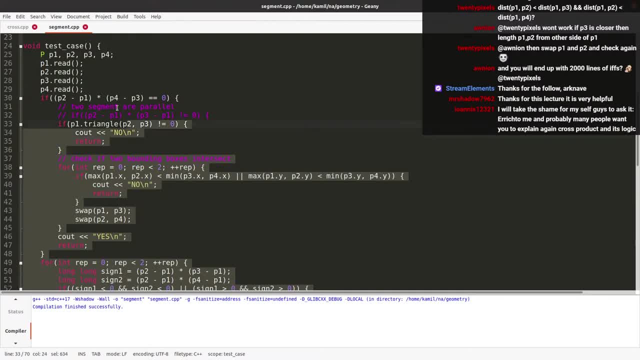 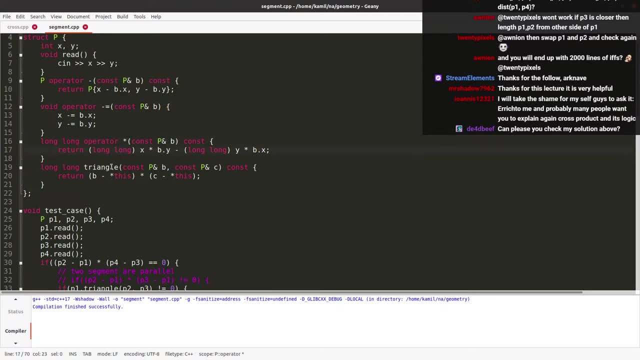 Nothing is collinear, Then you would have just that. By the way, Imagine how ugly this code would be If we didn't have prewritten functions For minus and for times. And let's, With respect to me, Check two points. 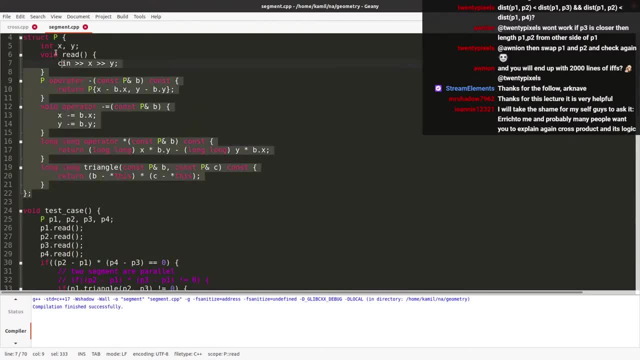 just that, by the way. imagine how this code, how ugly this code would be if we code, how ugly this code would be if we code, how ugly this code would be if we didn't have three written functions, or didn't have three written functions, or didn't have three written functions, or minus and four times. and let's indeed. 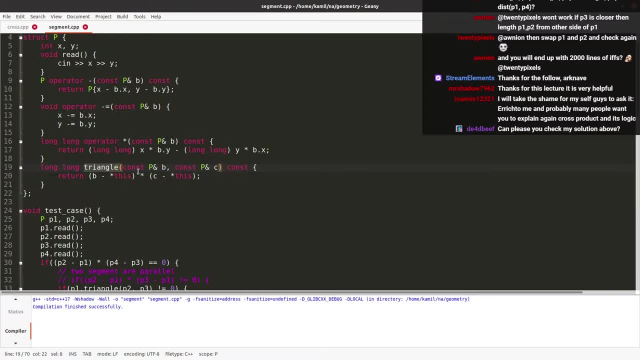 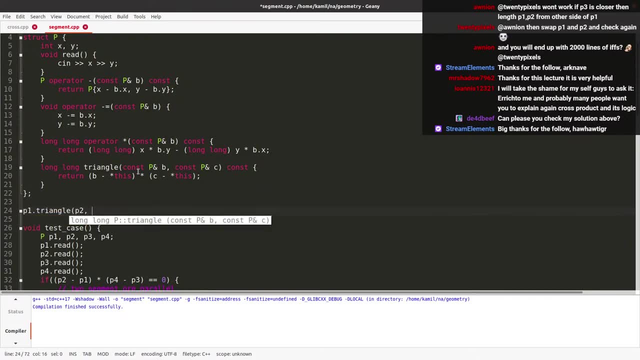 minus and four times. and let's indeed minus and four times, and let's indeed start using triangle again. triangle is start using triangle again. triangle is start using triangle again. triangle is, with respect to me, check two points. say, with respect to me, check two points. say, with respect to me, check two points. say you want triangle, it to be free with. 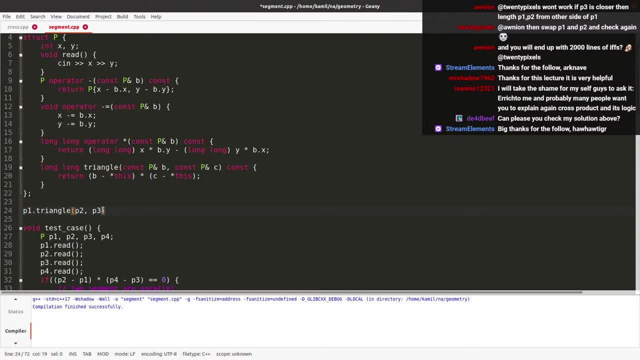 you want triangle it to be free with. you want triangle it to be free with respect to P 1 checks. if P 2 is on the respect to P 1 checks, if P 2 is on the respect to P 1 checks, if P 2 is on the left from P 3, then cross product will be. 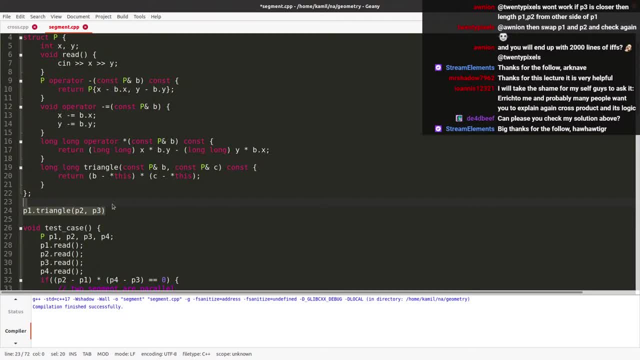 left from P 3, then cross product will be left from P 3, then cross product will be negative. I want to explain again negative. I want to explain again negative. I want to explain again cross-product and his logic. well, I did. cross-product and his logic. well, I did. 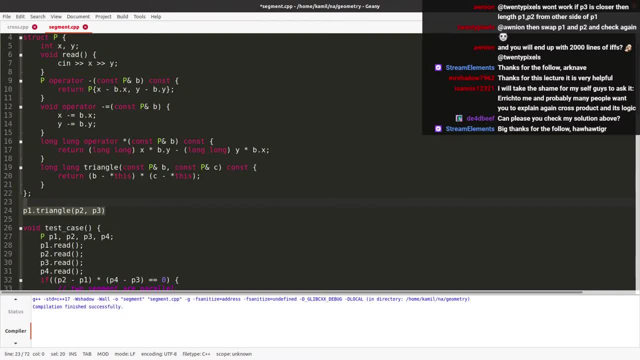 cross-product and his logic. well, I did that at the beginning. I don't know how that at the beginning. I don't know how that at the beginning, I don't know how else I would describe it, so I guess my else I would describe it, so I guess my. 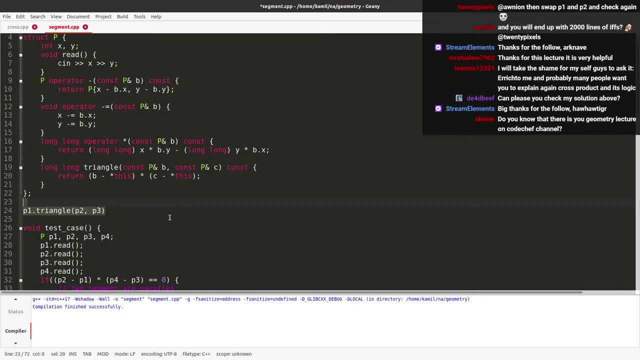 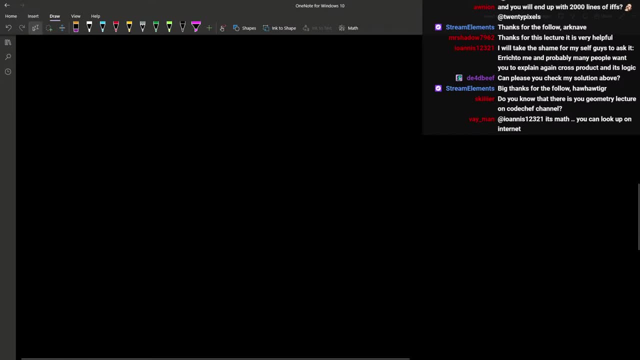 else I would describe it. so I guess my suggestion is watch the beginning again, suggestion is watch the beginning again, suggestion is watch the beginning again after the lecture can be on YouTube, very after the lecture can be on YouTube, very after the lecture can be on YouTube very shortly, just for a minute, is what. 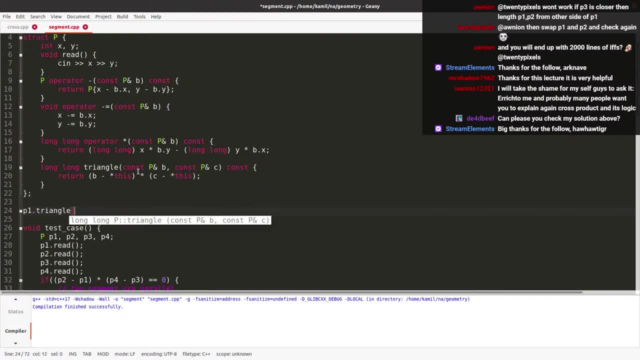 Say: P1 triangle, P2, P3. With respect to P1. Checks: if P2 is on the left from P3. Then cross product will be negative. Want to explain again Cross product and its logic. Well, I did that at the beginning. 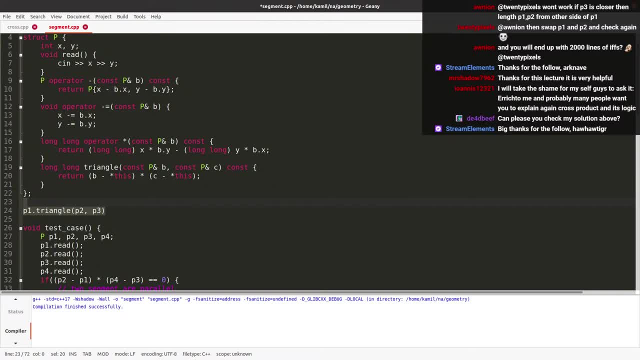 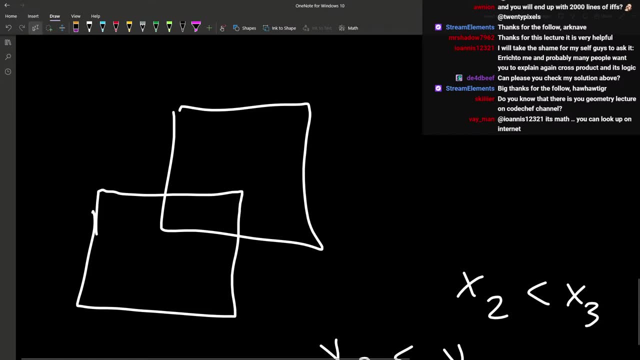 I don't know how else I would describe it, So I guess my suggestion is Watch the beginning again Through the lecture. It can be on YouTube Very shortly, Just for a minute- Is what cross product gives us. Doesn't matter how it works internally. 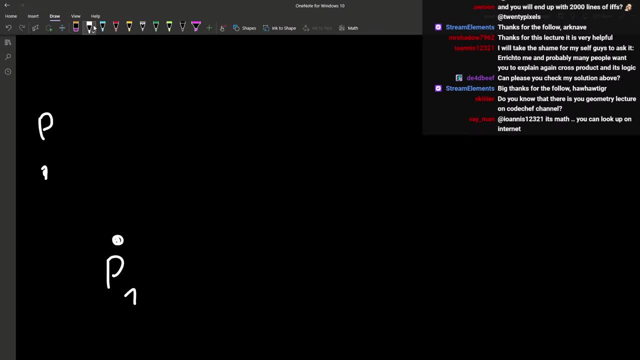 With respect to one point And you have two other points: P2 and P3.. Assuming that you are a human Standing in this point And you look at direction of P2. You will be given information If P3 is somewhere on the right. 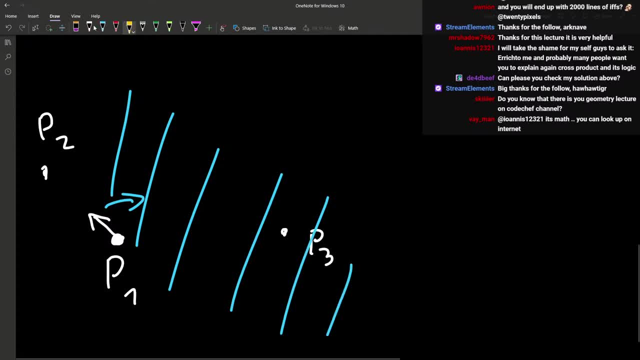 So in this half plane, Or maybe on the left In this half plane, Or maybe, cross product is zero. This means collinearity, The slope being the same. This is case of cross product zero If P2 is on the left from P3.. 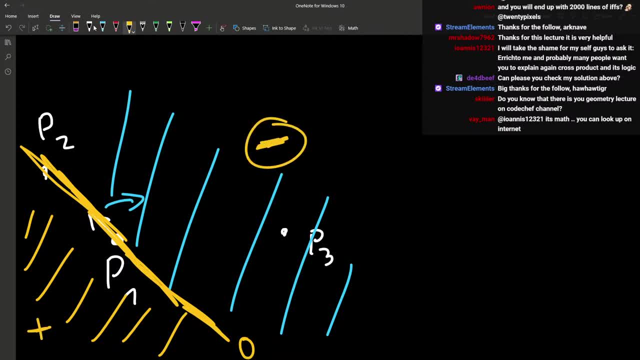 Then cross product is negative, It's here And positive is here. This is vector. In math you would likely write Vector from P1 to P2.. Cross product With P1 to P3.. Compare those two directions, Those two slopes. 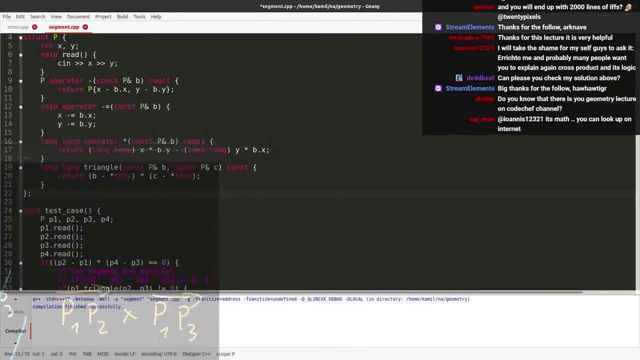 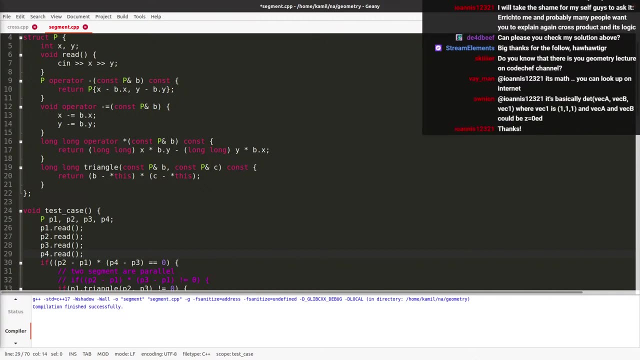 This is cross operated. That's just a very short recap. I don't want to again Go through the beginning of the lecture. Can you check my solution above Solving equations for a root? You want to have some quadratic function. That's very ugly. 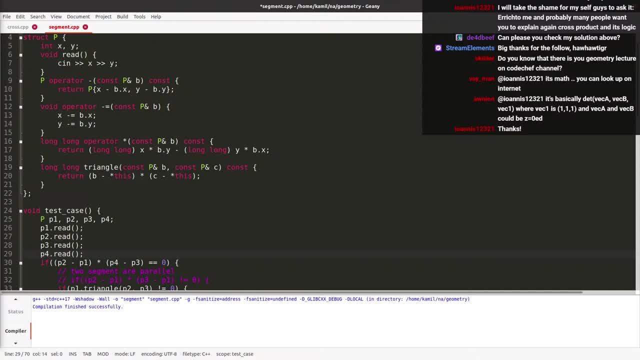 It's root of something else. The third beef: What about this? If you have more questions, I will Later on YouTube. Below this stream on YouTube, You can ask them in comments And I will try to reply to them. It will be hard now for me to go through everything. 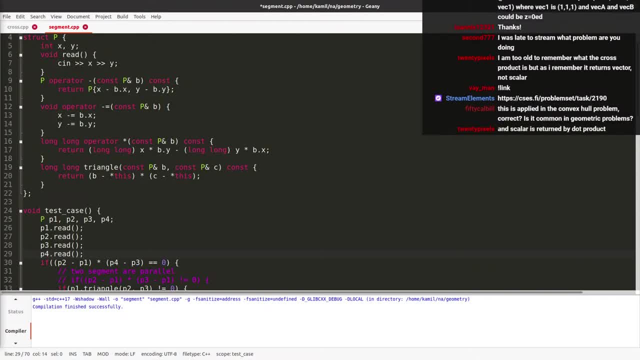 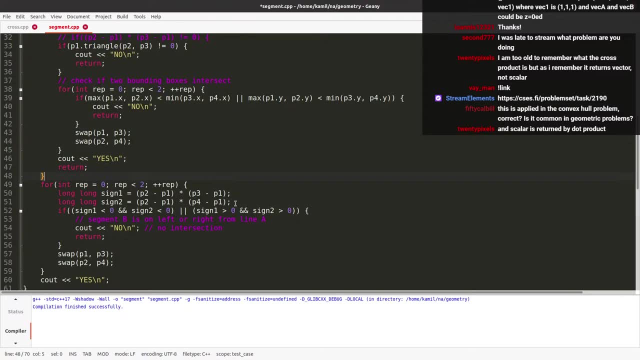 I'm sure that there are other methods, But there is a reason why This one is well known. This is good. This is good. This checks all the cases. If you come up with everything else, I would say It's very likely that you miss some case. 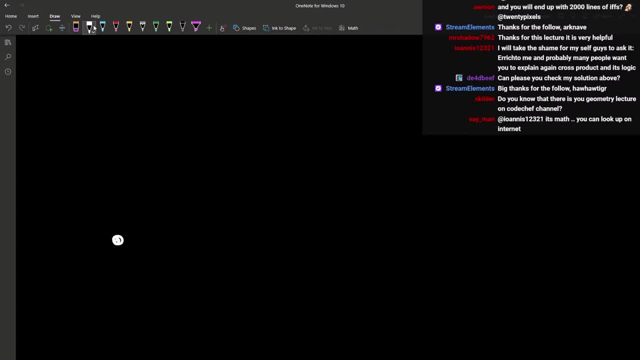 shortly, just for a minute, is what, shortly, just for a minute, is what cross-product gives us doesn't matter. cross-product gives us doesn't matter. cross-product gives us doesn't matter how it works internally. with respect to how it works internally, with respect to how it works internally, with respect to one point, and you have two other points. 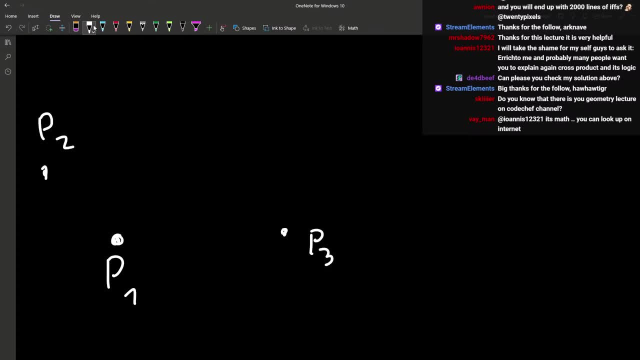 one point and you have two other points. one point and you have two other points- p2 and p3- assuming that you are human- p2 and p3. assuming that you are human- p2 and p3, assuming that you are human, standing in this point and you look at: 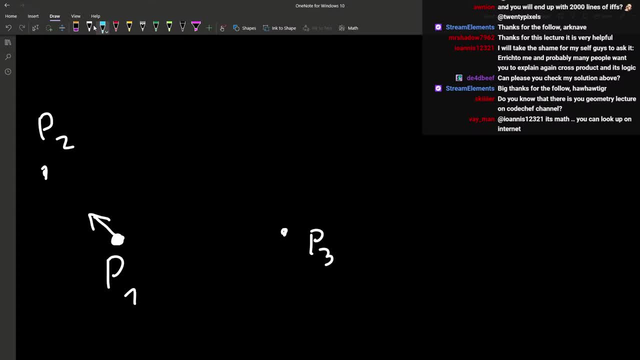 standing in this point and you look at standing in this point and you look at direction of p2, you will be given direction of p2. you will be given direction of p2. you will be given information if pre p3 is somewhere on the information, if pre p3 is somewhere on the. 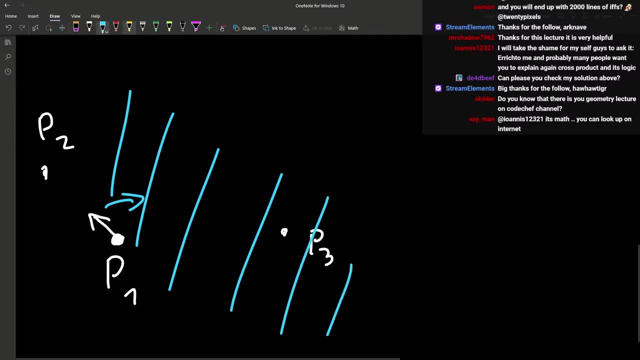 information: if pre p3 is somewhere on the right, so in this half plane, or maybe right, so in this half plane. or maybe right, so in this half plane. or maybe on the left in this half plane, or maybe on the left in this half plane, or maybe. 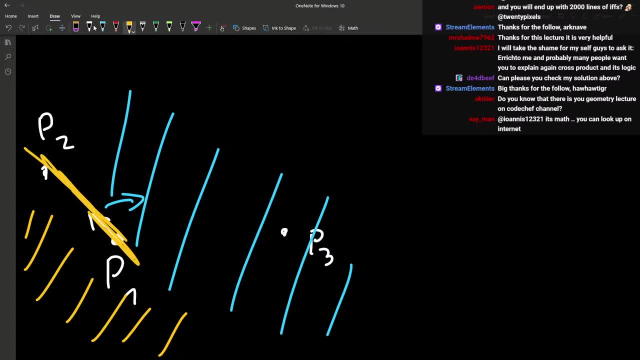 on the left in this half plane, or maybe cross product is zero. this means cross product is zero. this means cross product is zero. this means collinearity, the the slope being the same, collinearity, the the slope being the same, collinearity, the the slope being the same. this is case of cross product zero. 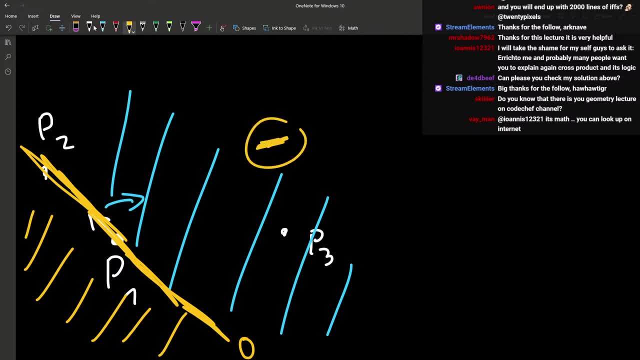 this is case of cross product zero. this is case of cross product zero. if p2 is on the left from p3, then if p2 is on the left from p3, then if p2 is on the left from p3, then cross product is negative. it's here. 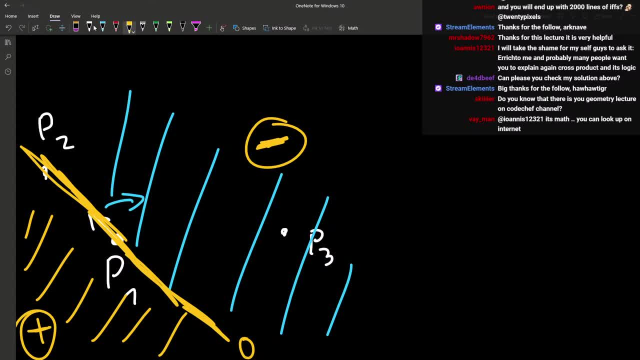 cross product is negative, it's here. cross product is negative. it's here, and positive is here, and positive is here and positive is here. this is this is. this is vector in math. you would likely write vector in math. you would likely write vector in math. you would likely write vector from p1 to p2. 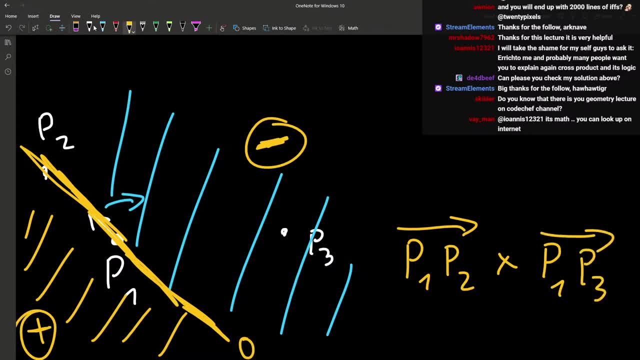 vector from p1 to p2. vector from p1 to p2. cross product with p1 to p3. cross product with p1 to p3. cross product with p1 to p3. compare those two directions, those, those compare those two directions, those those compare those two directions, those, those two slopes. this is cross operated. two slopes, this is cross operated. two slopes, this is cross operated. that's just a very short recap. i don't. that's just a very short recap. i don't, that's just a very short recap. i don't want to you know again. want to you know again. 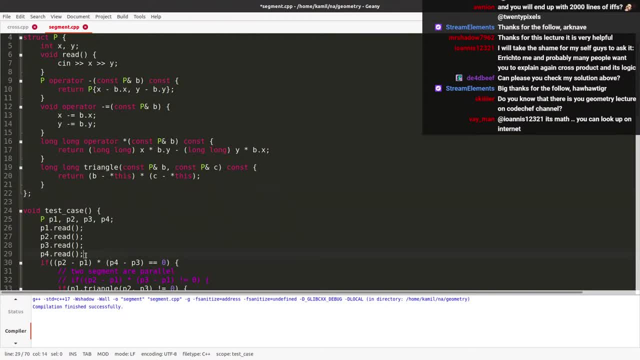 want to you know again. go through the beginning of the lecture. can you check my solution above? solving equations for a root. solving equations for a root. solving equations for a root. you want to have some quadratic function. you want to have some quadratic function. you want to have some quadratic function. that's. 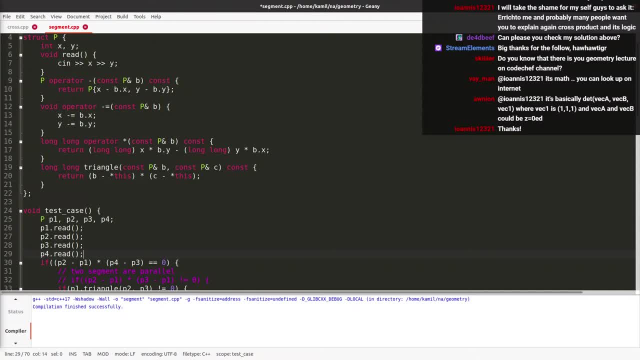 that's, that's very ugly, or it's root of something else, or it's root of something else, or it's root of something else. therefore, the beef. what about this? if, therefore, the beef? what about this? if, therefore, the beef, what about this? if you have more questions, i will. 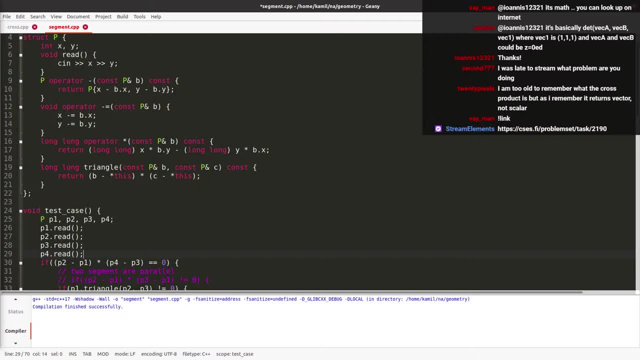 you have more questions, i will you have more questions? i will later on youtube below this stream, on later on youtube below this stream. on later on youtube below this stream on youtube. you can ask them in comments and youtube. you can ask them in comments and youtube. you can ask them in comments and i will try to reply to them. 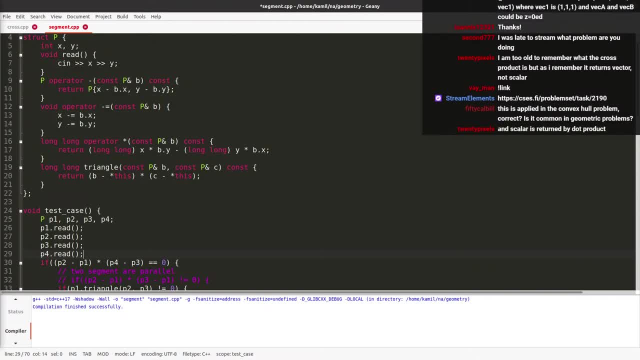 i will try to reply to them. i will try to reply to them. it will be hard now for me to go through. it will be hard now for me to go through. it will be hard now for me to go through everything, everything, everything. i'm sure that there are other methods. 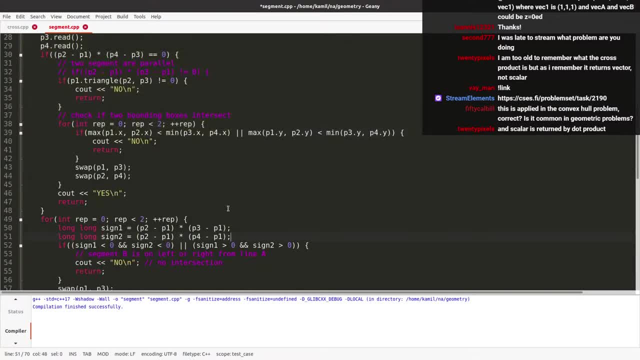 i'm sure that there are other methods. i'm sure that there are other methods, but there is a reason why this one is. but there is a reason why this one is. but there is a reason why this one is well known. this is good. well known: this is good. 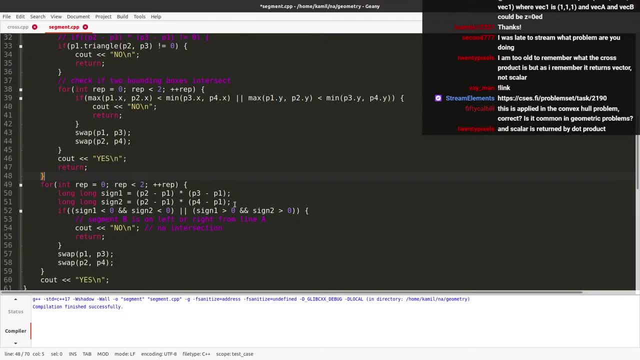 well known. this is good. like this: checks all the cases. if you like, this checks all the cases. if you like, this checks all the cases. if you come up with everything else, come up with everything else. come up with everything else. it's, i would say it's very likely that. 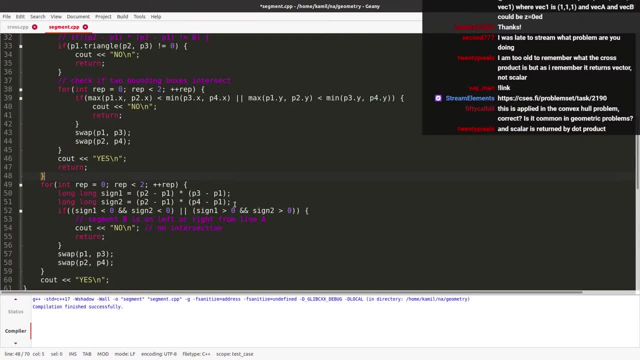 it's. i would say it's very likely that it's. i would say it's very likely that you miss some case, or that you need you miss some case, or that you need you miss some case, or that you need real values, and then you deal with. 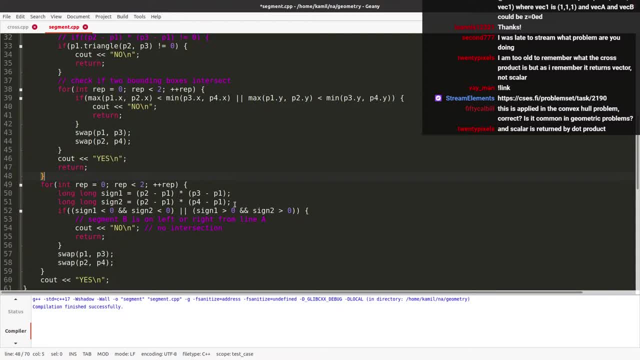 real values. and then you deal with real values, and then you deal with precision errors. precision errors, precision errors. it's harder than to check if something it's harder than to check if something, it's harder than to check if something sucks. you don't need that product. 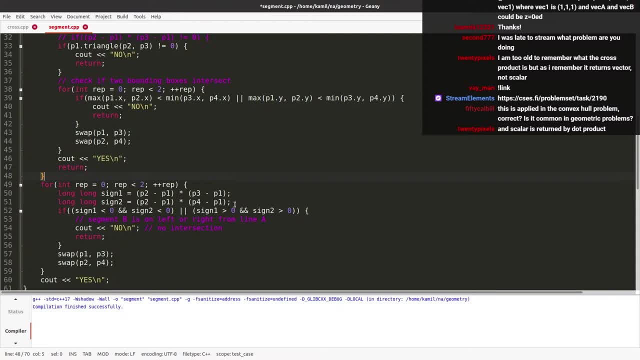 Or that you need real values And then you deal with precision errors. It's harder than to check if something is positive or negative When it's close to zero. Cross product is indeed needed in convex hull And dot product sucks. You don't need dot product. 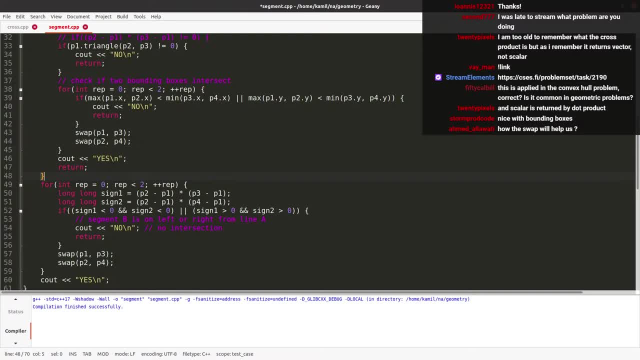 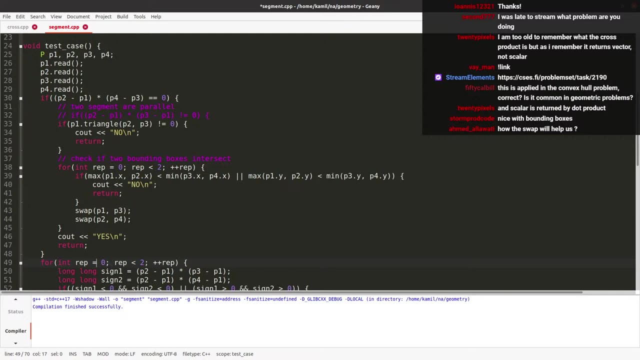 Cross product is superior. It's not a problem. It's just a problem How the swap will help us Depends in which part, As I went through the code, I described what I'm doing In this case. I wanted to say: 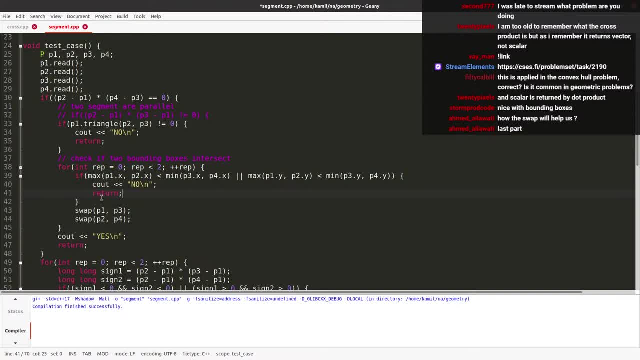 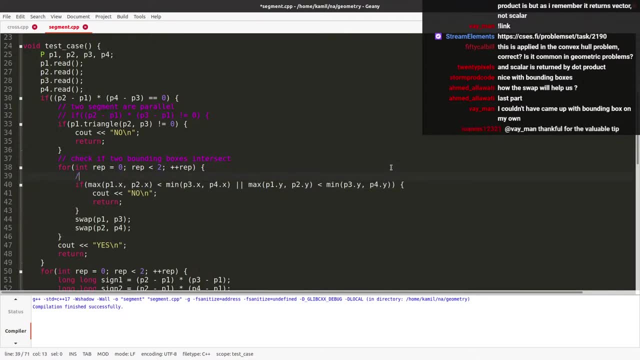 To check if the two rectangles intersect. I wanted to detect a case where they don't intersect. This line says: This line says Rectangle, Let's call it rectangle F, Rectangle F, Rectangle A, On left from rectangle B, Or 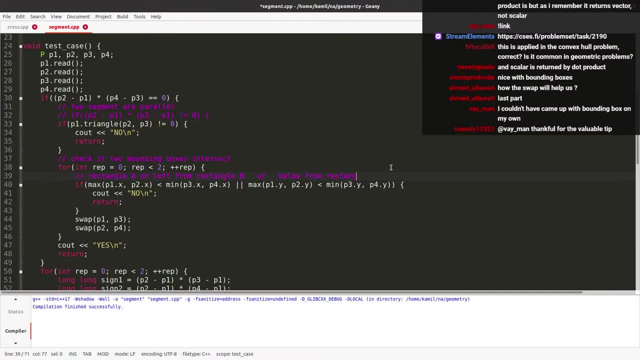 Below from rectangle B. This checks exactly those two cases. A is on the left, So Xs are smaller than Xs for B, Or same with Ys. But this is not the only case where A and B are disjoint. It can be the other way around. 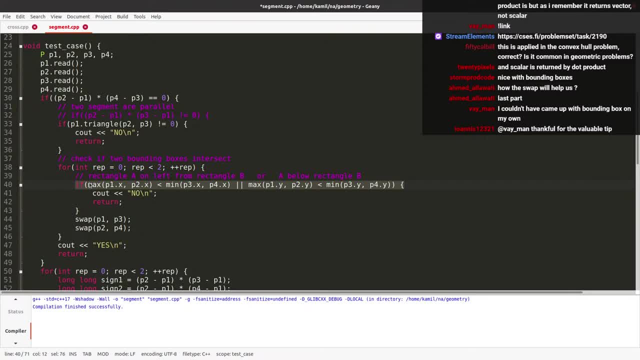 A can be above. You can copy paste this Another. if What I did is I swapped the two rectangles A and B, Maybe this code would be a bit nicer with F function. Anyway, We just Check for intersection of two rectangles. 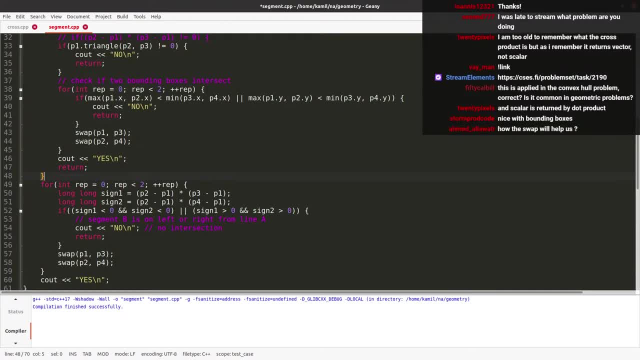 sucks, you don't need that product. sucks, you don't need that product. cross product is superior how the swap will help us and it depends how the swap will help us. and it depends how the swap will help us and it depends in which part i this as i went through. 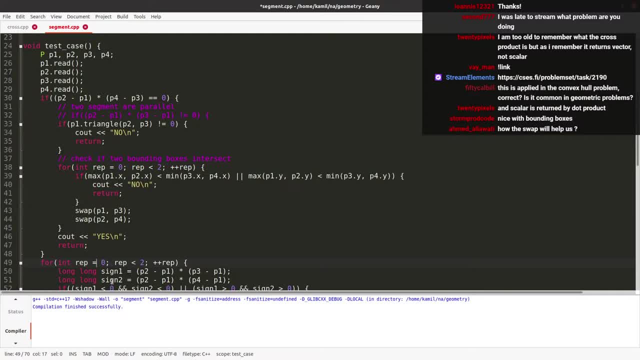 in which part i this as i went through, in which part i this, as i went through the code. i described what i'm doing, the code. i described what i'm doing, the code. i described what i'm doing in this case. i wanted to say: in this case, i wanted to say: 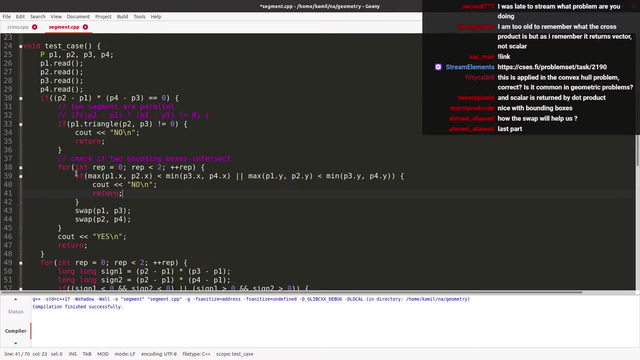 in this case, i wanted to say, to check if the two rectangles intersect. to check if the two rectangles intersect. to check if the two rectangles intersect, i wanted to detect a case where they. i wanted to detect a case where they. i wanted to detect a case where they don't intersect. 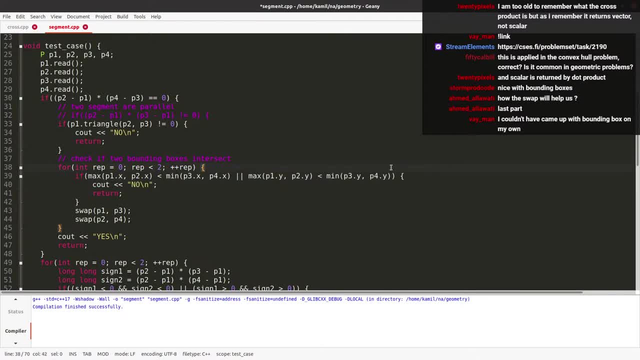 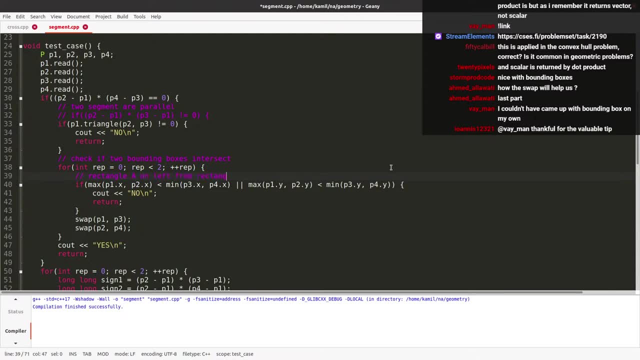 don't intersect. don't intersect. this line says: this line says rectangle, let's call it. this line says rectangle, let's call it. this line says rectangle, let's call it rectangle a, rectangle a. rectangle a. on the left from rectangle b, on the left from rectangle b. 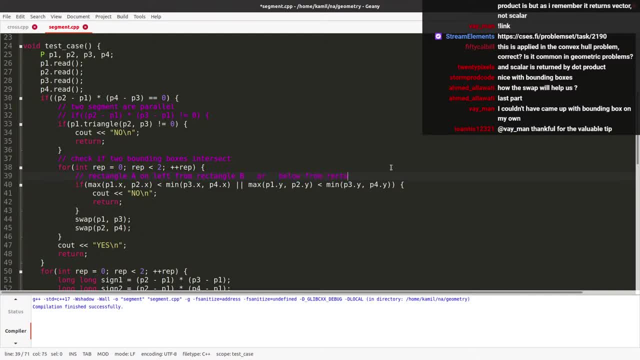 on the left from rectangle b or below from rectangle this checks exactly those two cases. ace. this checks exactly those two cases. ace. this checks exactly those two cases ace. on the left, so x's are smaller than x. on the left, so x's are smaller than x. 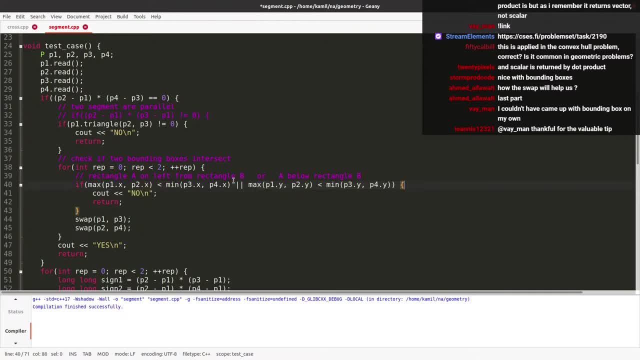 on the left, so x's are smaller than x is for b is for b is for b or some of with wise, but this is not the or some of with wise. but this is not the or some of with wise. but this is not the only case where a and b are disjoint it. 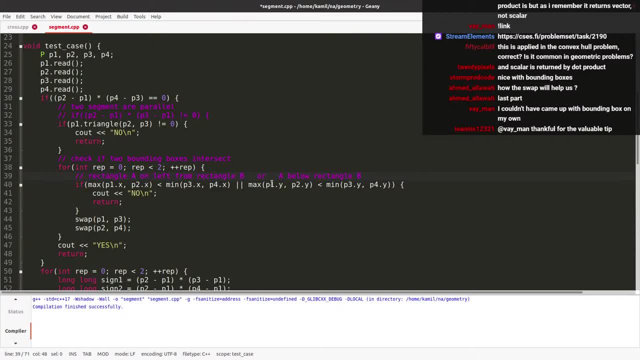 only case where a and b are disjoint. it only case where a and b are disjoint. it can be the other way around. a can be- can be the other way around. a can be, can be the other way around. a can be above, above, above. so you can copy paste this and make you. 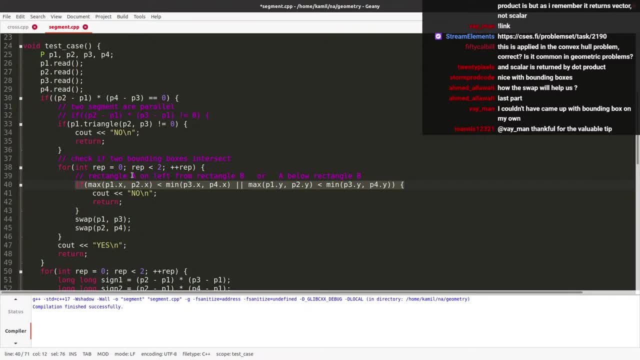 so you can copy paste this and make you. so you can copy paste this and make you know another. if what i did is i swapped, know another. if what i did is i swapped, know another. if what i did is i swapped the two rectangles a and b. 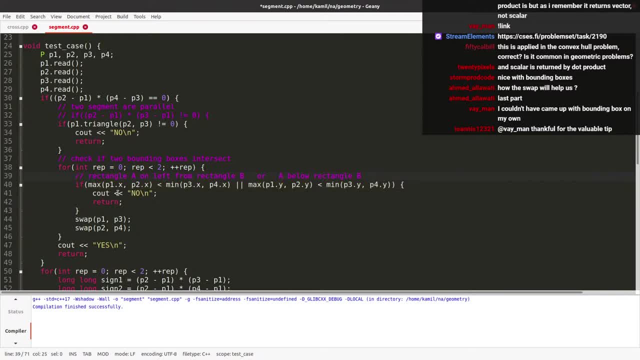 the two rectangles a and b, the two rectangles a and b. maybe this code would be a bit nicer with, maybe this code would be a bit nicer with, maybe this code would be a bit nicer with a function anyway, anyway. anyway, we just, we just, we just check for intersection of two rectangles. 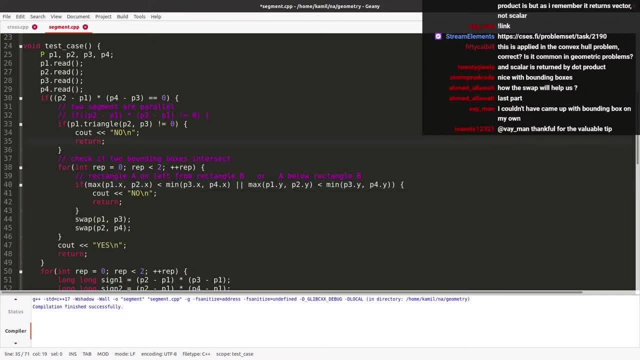 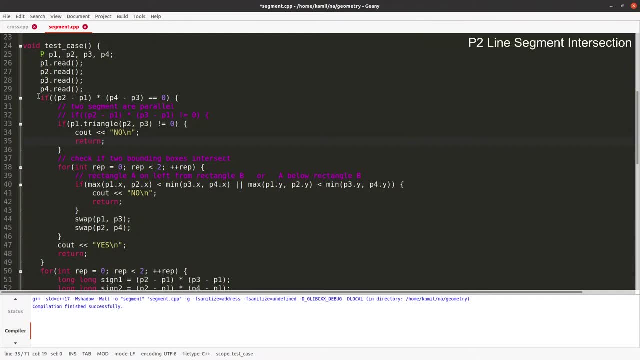 check for intersection of two rectangles, check for intersection of two rectangles being bounding boxes on the two segments, and as a disclaimer, and as a disclaimer, and as a disclaimer, i'm not 100 sure if this is the easiest. i'm not 100 sure if this is the easiest. 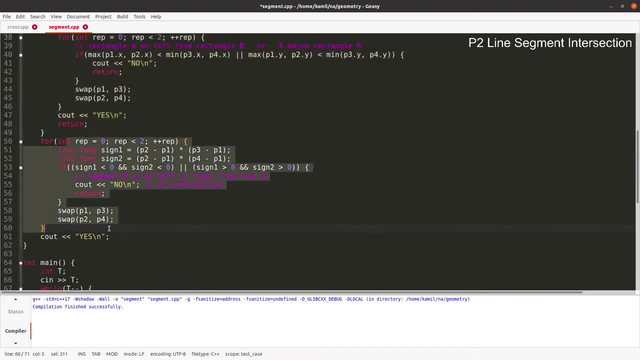 i'm not 100 sure if this is the easiest method. i'm quite sure that this is the method. i'm quite sure that this is the method. i'm quite sure that this is the easiest method for a non-parallel case. easiest method for a non-parallel case. 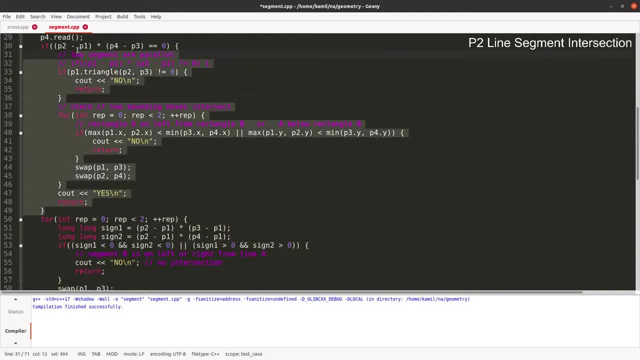 easiest method for a non-parallel case. this is how everybody do it. this is how everybody do it. this is how everybody do it for here, for here. for here, maybe there is something slightly easier, maybe there is something slightly easier, maybe there is something slightly easier, but always in geometry. 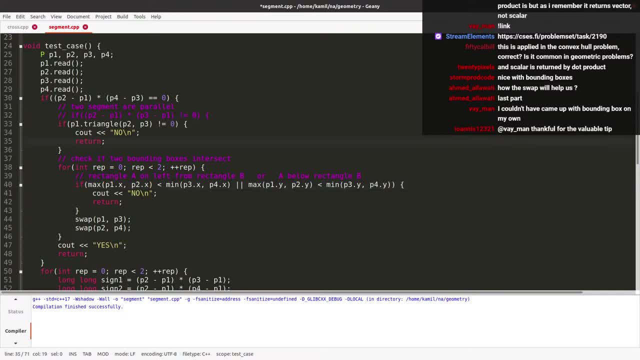 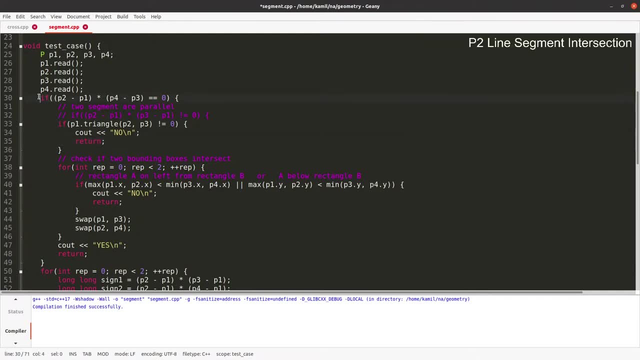 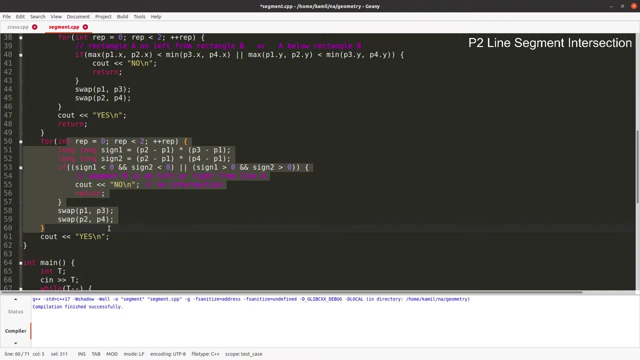 Being bounding boxes on the two segments As a disclaimer. I'm not 100% sure if this is the easiest method. I'm quite sure that this is the easiest method for non-parallel case. This is how everybody do it For here. 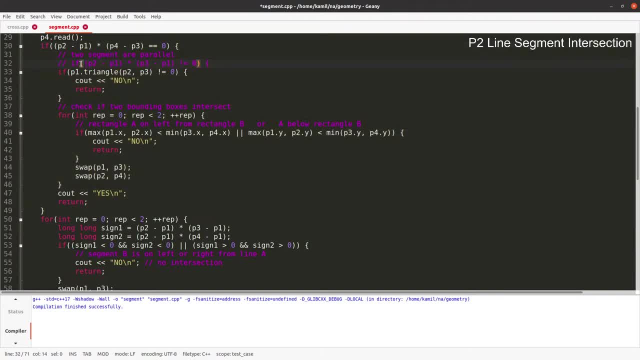 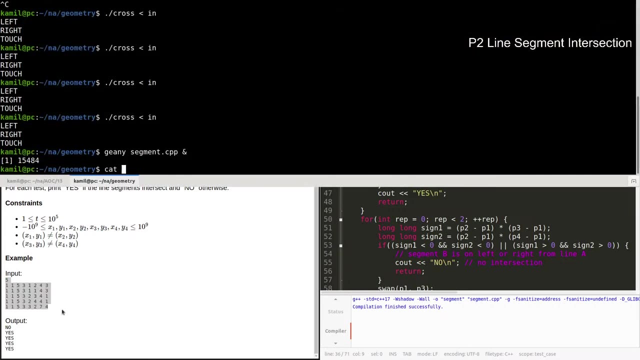 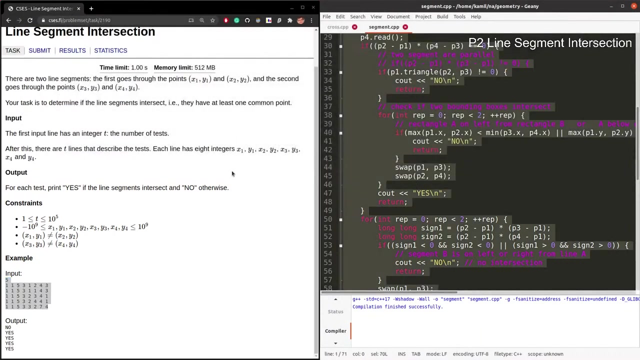 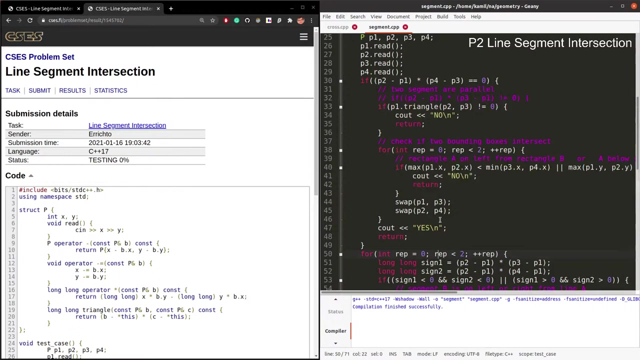 Maybe there is something slightly easier, But always In geometry, Expect some pain To deal with parallel case. Now I really hope I get AC with this. Let's see Past sample test. Alright, Nice, We can move on. 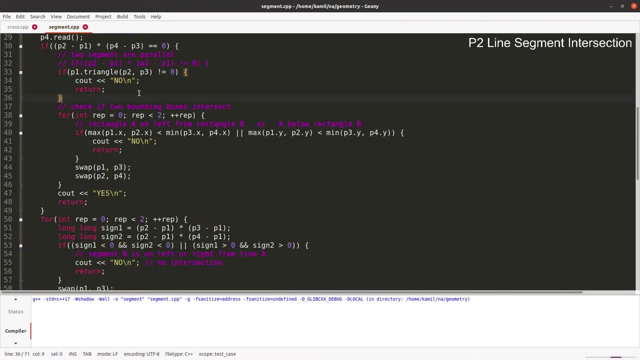 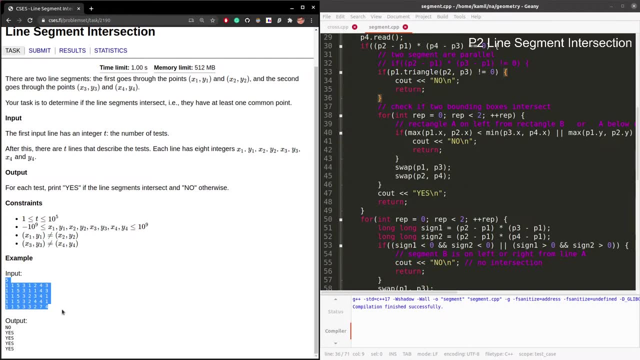 but always in geometry, but always in geometry. expect some pain to deal with parallel. expect some pain to deal with parallel. expect some pain to deal with parallel case, case, case. now i really hope i get now. i really hope i get now. i really hope i get ac with this. 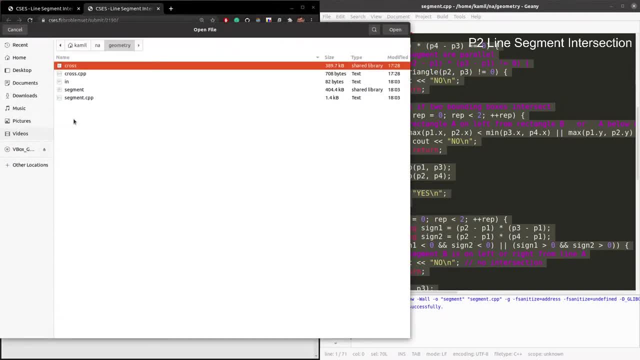 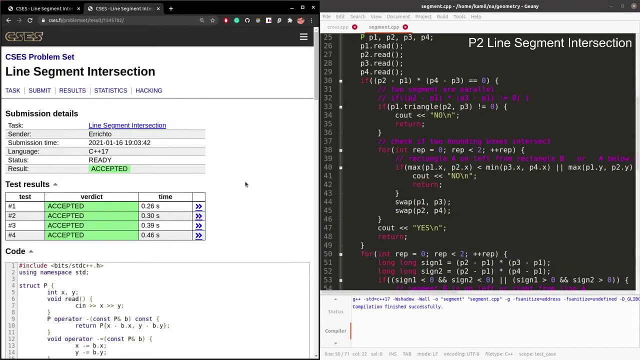 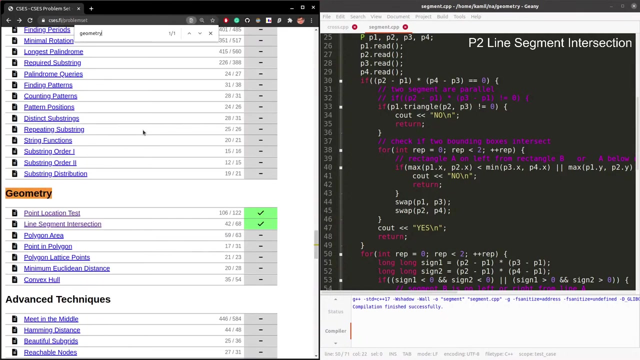 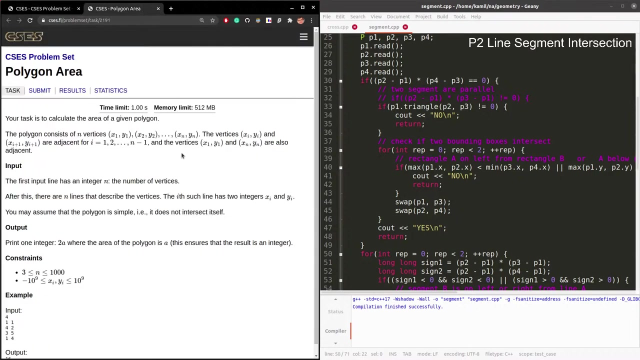 past sample test. all right, all right, all right, nice, nice, We can move on. One hour passed and we need to also today go through some harder problems. Now, polygon area. If we go very slow, then maybe I will split this stream into two parts, but I would prefer to do everything today. 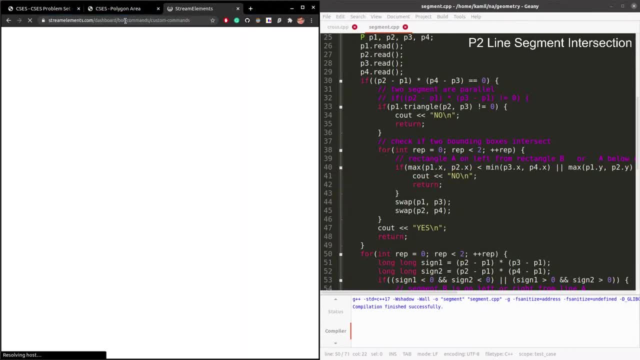 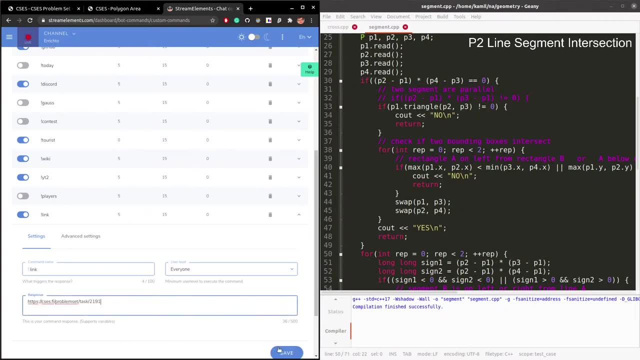 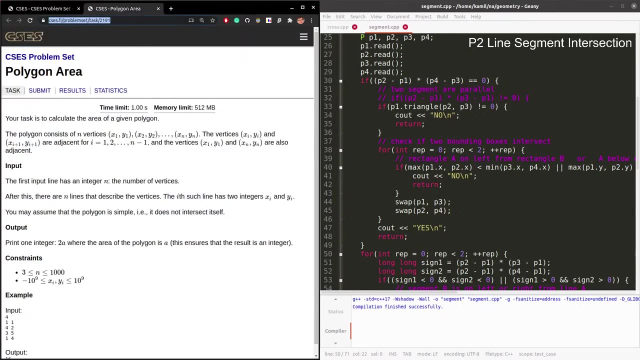 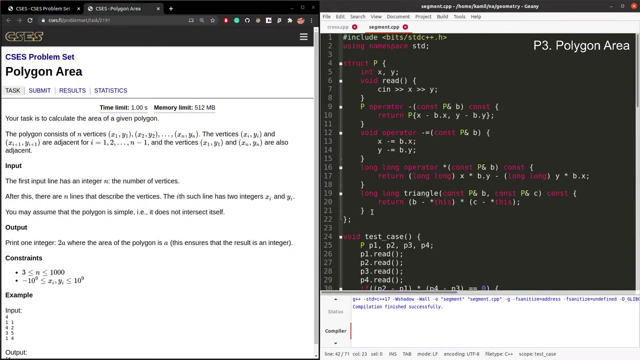 Giving you the link. That's the third problem. Polygon area: We already know that we can compute triangle area, Actually the function triangle. in my code, this one, it's enough to now say p1, the triangle, p2, p3. Now, absolute value of that to ignore the sign. and I told you a long time ago that. 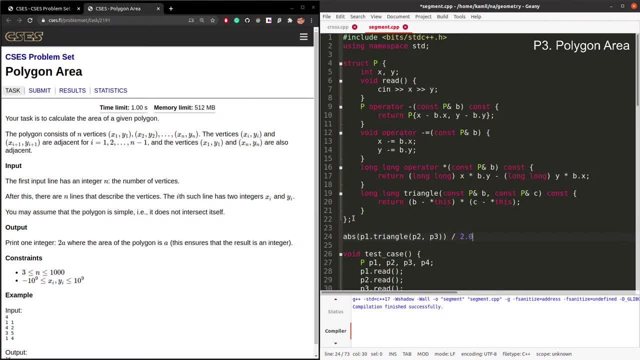 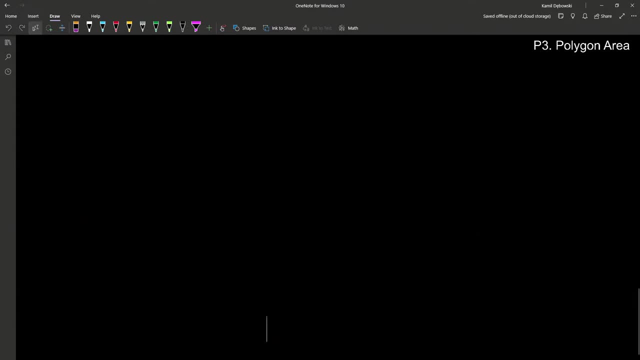 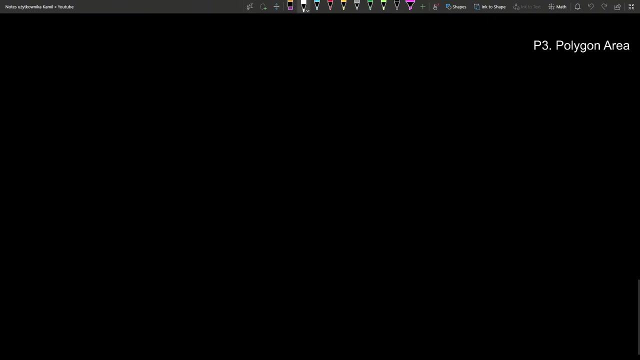 cross product is twice the triangle. This divided by 2. This is area of triangle, Exactly that. But we need to deal with polygon, And first let's assume that polygon is convex And first let's assume that polygon is convex. If we know how to deal with triangles and you need to compute area of polygon, you can fix one point. 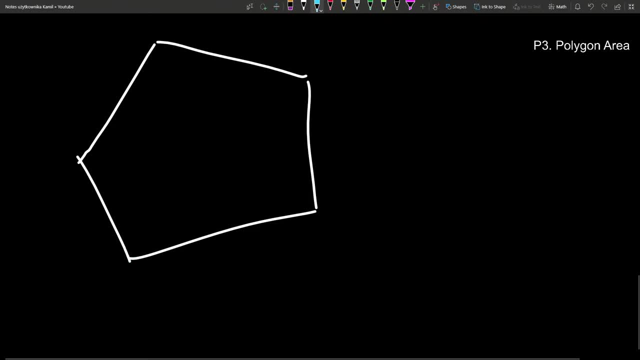 Let's say one of the endpoints. let's say, Or maybe first You can take some point inside, draw those segments and say that area of polygon is the sum of those five areas. It isn't easy, though, to choose some point inside. Step better, Little bit better, Take one arbitrary point of a polygon. 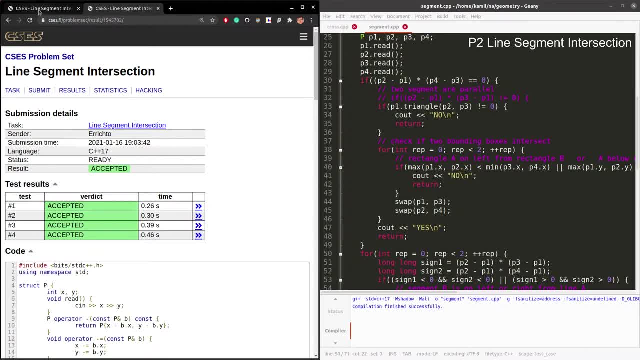 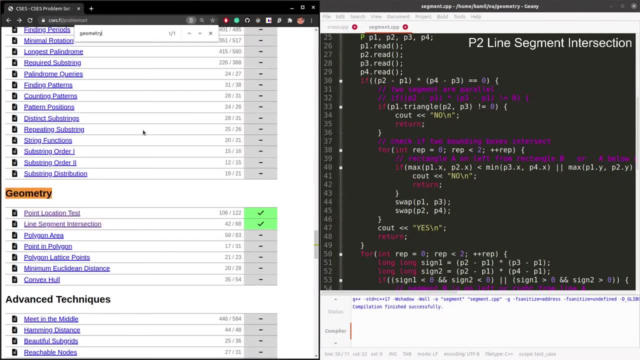 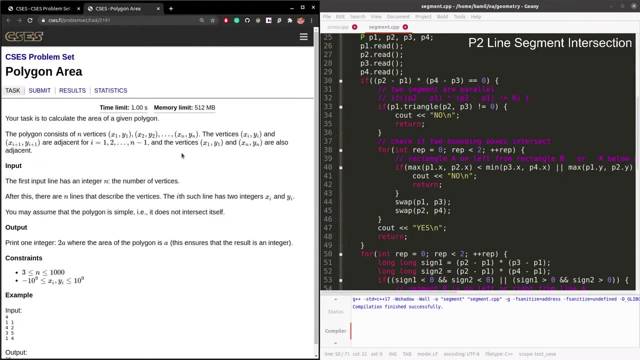 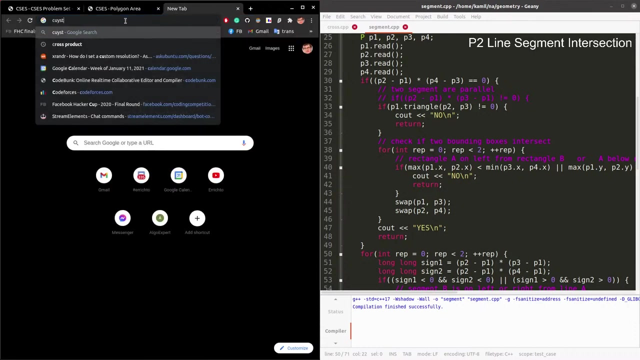 One hour passed And we need to Also today go through some harder problems. Now, Polygon area. If We go very slow, Then maybe I will split this stream into two parts, But I would prefer to do everything today. Giving you the link. 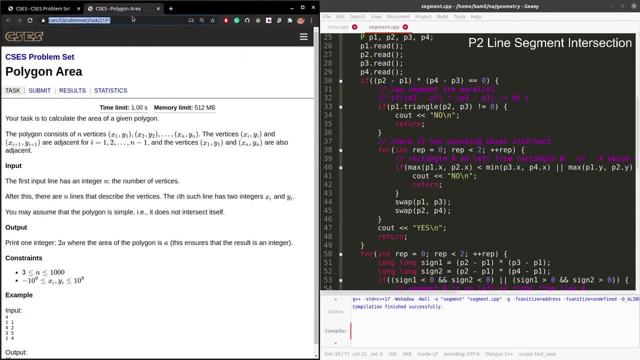 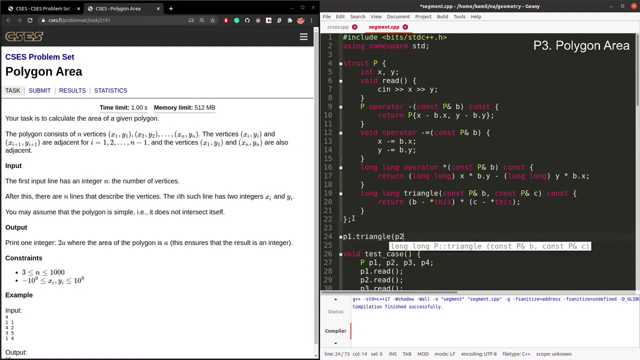 That's the third problem, Polygon area. We already know That we can compute Triangle area, Actually the function Triangle. in my code, This one, It's enough to now say P1.TriangleP2P3.. Now, absolute value of that. 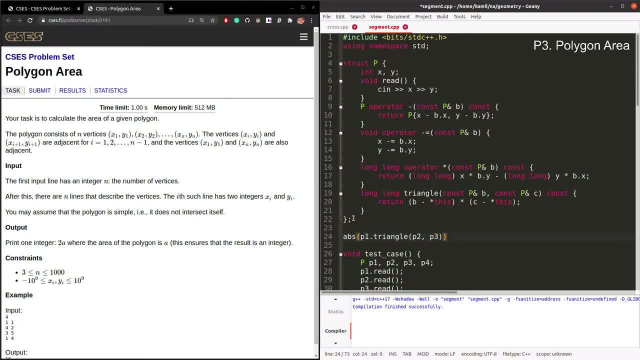 To ignore the sign. Let me go that Cross product is twice the triangle. This divided by two, This is area of triangle, Exactly that. But we need to deal with polygon, And first let's assume that Polygon is convex, If we know how to, 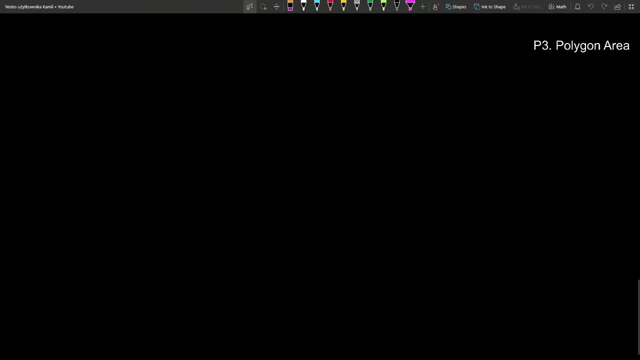 Deal with With triangles And you need to compute area of polygon. You can fix one, Let's say one of the endpoints. Let's say, Or maybe first You can take some point inside, Draw those segments And say that 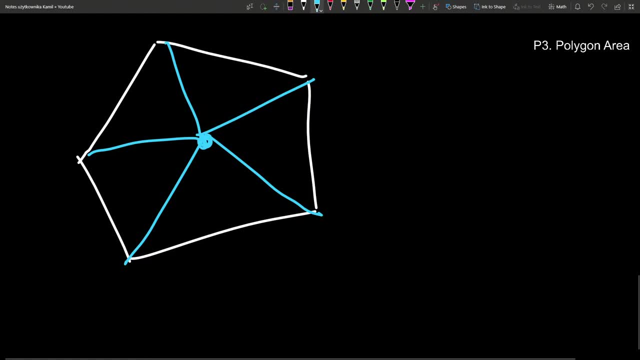 Area of polygon is the sum of those five areas. It isn't easy, though, To choose some point inside Polygon. Step better, Little bit better. Take one arbitrary point of a polygon, Draw those lines And your neighbors. The number of lines drawn will be n-3.. 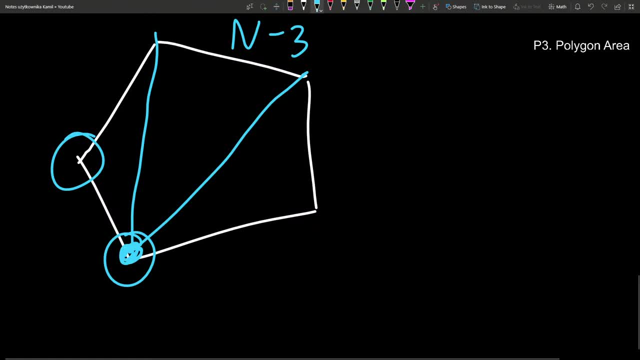 Everything other than me And my two neighbors And say that: Take some of those areas. What if Polygon is not convex? This is very magical. Either believe me Or you can understand. First, let's go with believing. I will tell you that. 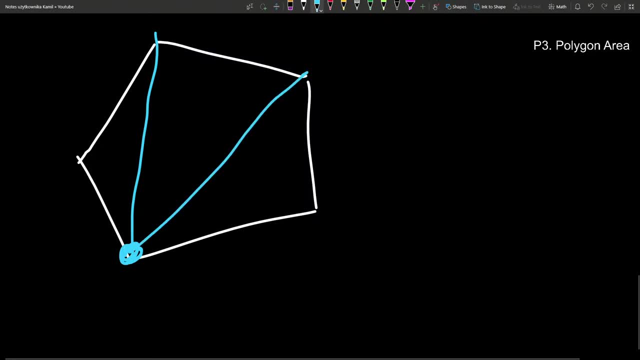 Draw those lines to everything other than your neighbors- The number of lines drawn will be n-3.. Everything other than me and my two neighbors- And say that you take some of those areas. What if? What if polygon is not convex? This is very magical and you can either believe me or you can understand, and we will. first, let's go. 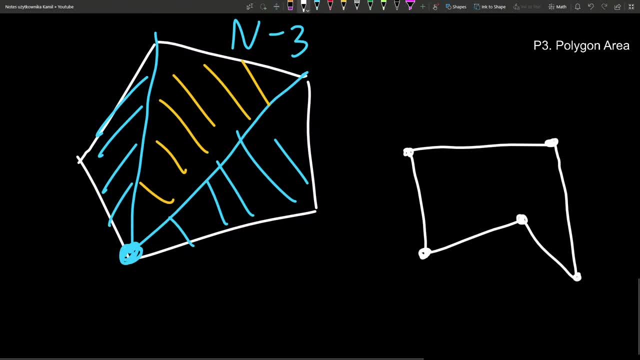 with believing. I will tell you that with respect to any point here, let's call it p1.. Then we have p2, 3, 4 and 5. The same code works for non-convex polygons. That is here from p1. first we looked at p2 and p3 and we took the area of this triangle right. 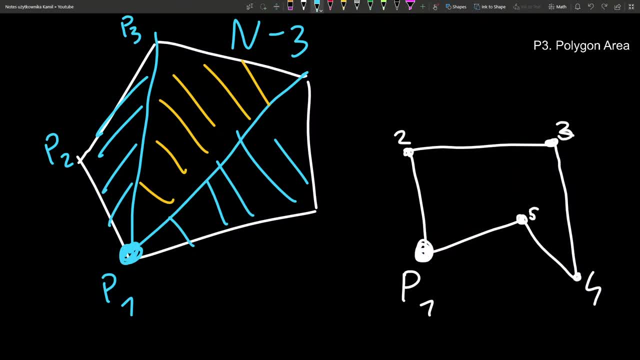 Same thing here. We add to the answer that, Then we add to the answer this area 3 and 4 and then watch out, we subtract area of 5, 4.. This should be subtracted. Fortunately we don't need any ifs. 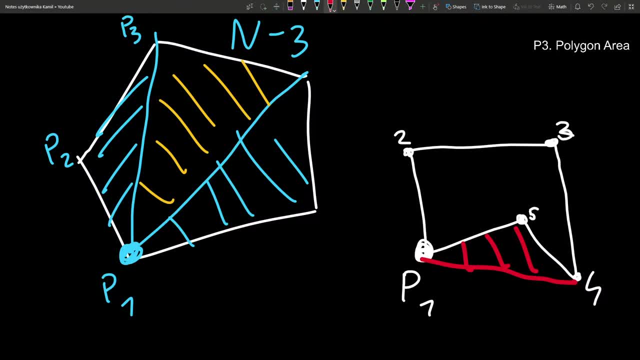 Cross product will already give us positive or negative area and we just should take it and not use absolute value, If we indeed go like that. So if points are given in clockwise order for the polygon, then whenever you take cross product of p2 and p3, like that, 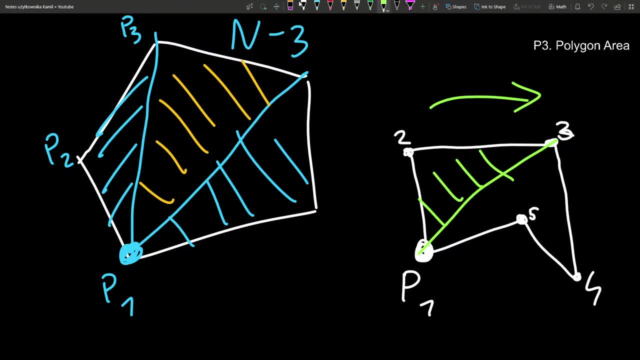 In this order, you will get something like that, some negative value, actually. okay, so let's say that this first triangle gave us minus 30, then this second one gave us minus 50, then this one. it would be positive, because 4 is on the right from 5. let's say that it is plus 12 and is: 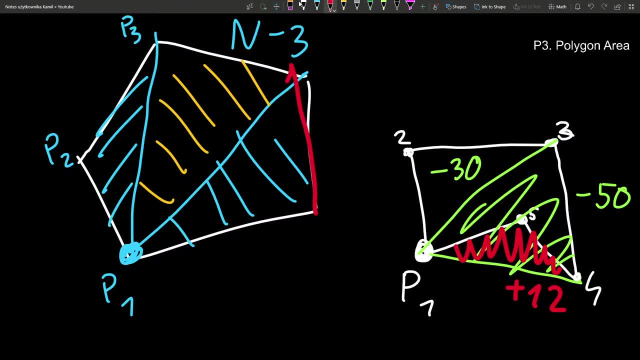 there anything more? oh, no, that's it. the last one is between 4 and 5 here. the last one is this: the answer in this case is that our sum of values is 80 minus 12. that's minus 68, and the answer is 68. you need to take absolute value at. 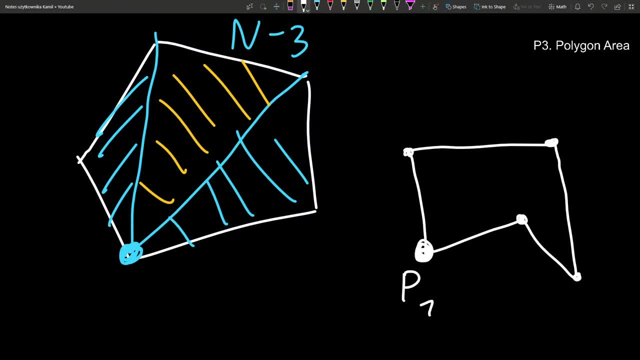 With respect to any point here. Let's call it p1.. Then we have p2, 3.. 4 and 5. The same code works For non-convex polygons. That is Here from p1.. First we looked at p2 and p3.. 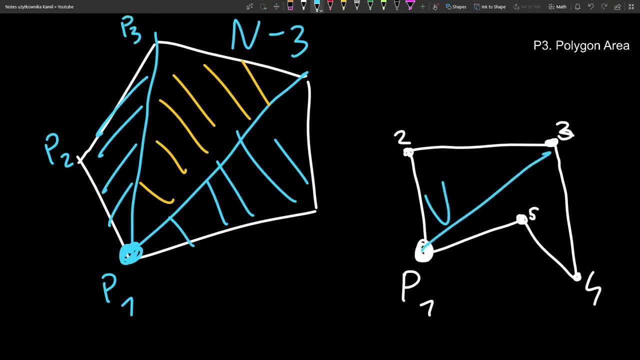 And we took the area of this Same thing here. We add to the answer that, Then we add to the answer This area 3 and 4. And then We subtract Area of 5, 4.. Should be subtracted. 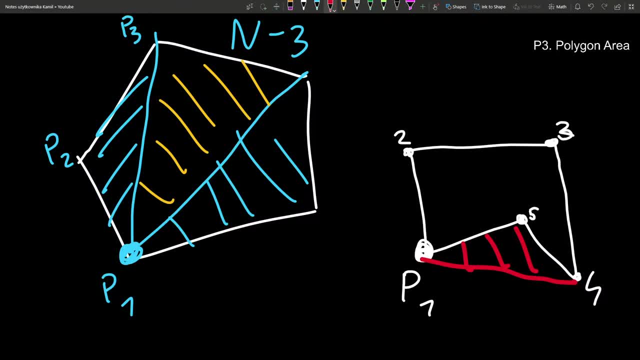 Fortunately We don't need any ifs. Cross product will already give us Positive or negative area And we should just take it Negative value If We indeed go like that. So if points are given in clockwise order For the polygon. 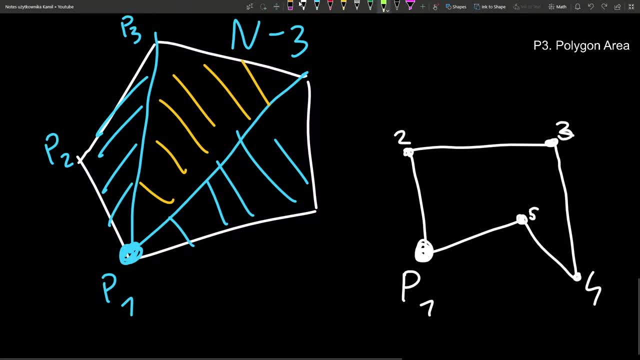 Then whenever you take Cross product of p2 and p3 like that In this order, You will get some negative value actually. So let's say that this first triangle Gave us minus 30. Then this second one Gave us. 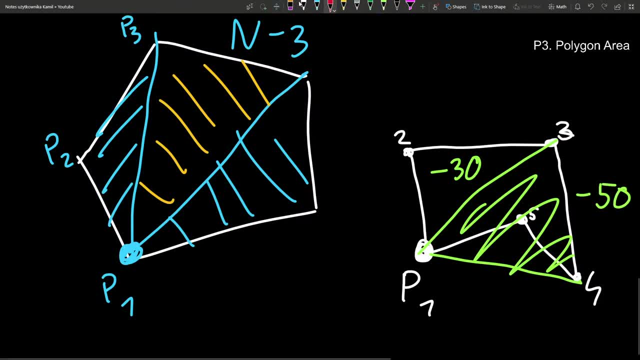 Minus 50.. Then This one. It would be positive, Because 4 is on the right from 5. Let's say that it is Plus 12. And is there anything more? That's it. The last one is between 4 and 5.. 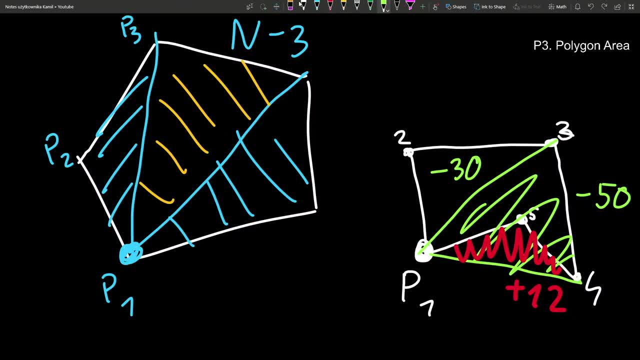 The answer in this case is: Our sum of values Is 80 minus 12.. That's minus 68. And the answer is 68. That's the end, Not for every triangle, If you take 30 plus 50 plus 12.. 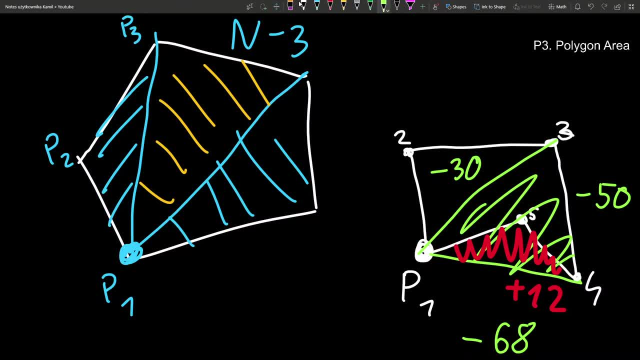 the end, not for every triangle. if you take 30 plus 50 plus 12, that's wrong. you need to take values given to you by cross product with sine, sum them all up and then the meaning of sine here is this: you need to take values given to you by cross product with sine. sum them all up and then the meaning of sine here is this: 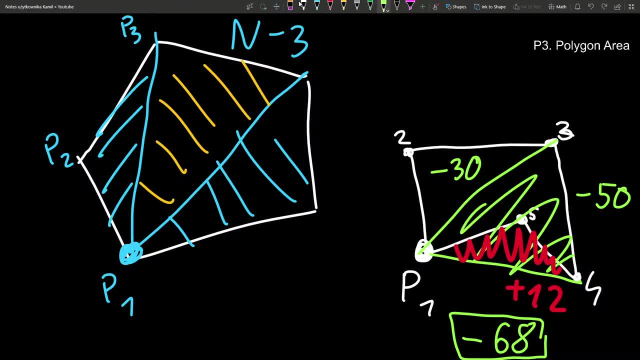 68 is exactly area of polygon. well, minus will tell you if you went. 68 is exactly area of polygon. well, minus will tell you if you went disease clockwise or counter clockwise through polygon, if you ever need that in: disease clockwise or counter clockwise through polygon, if you ever need that in. 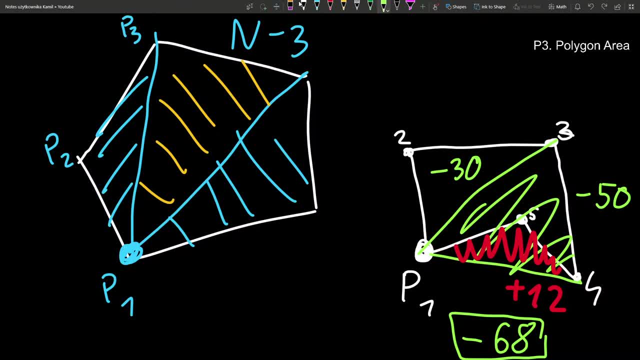 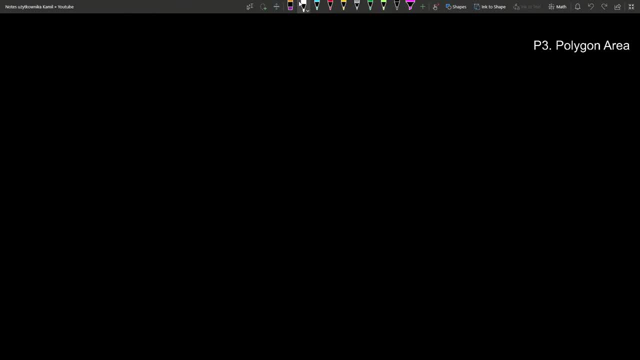 this problem. we will ignore it. at the end I print absolute value of this. one more way to look at it is that, with respect to any point P 1, when you already covert some part, then you already keep area of this. when you move forward, then you add area of a new triangle, possibly sometimes subtracting, and then, yeah, you might. 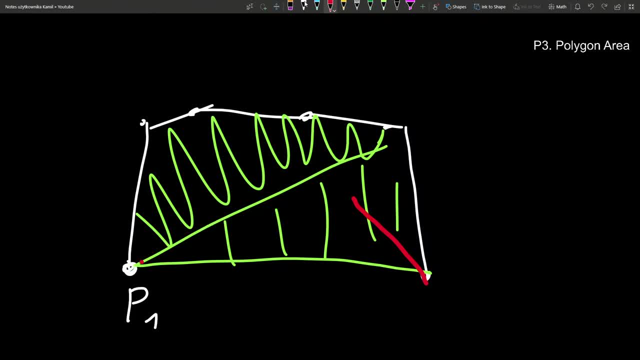 subtract, you might add again: like that polygon can look very crazily. let's say that it looks like this. you know, it's not easy to believe that. if this is the case, of course, assume that every small segment is a segment. it doesn't have curves, but this is a polygon, not convex, but it is a polygon. 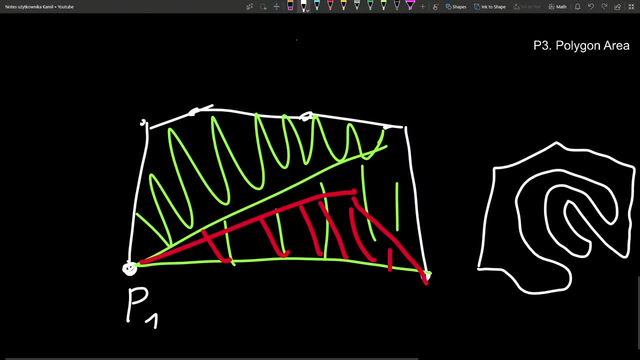 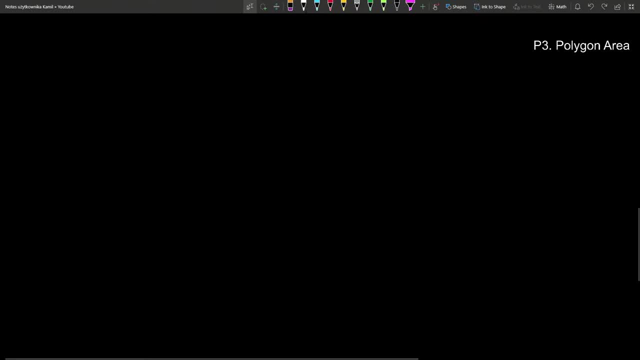 why does it still work? how to feel more convinced about it? this: this would be a little bit better with real life experiment, but i don't have sand. imagine, though, this would be a little bit better with real life experiment, but i don't have sand. imagine, though, the. 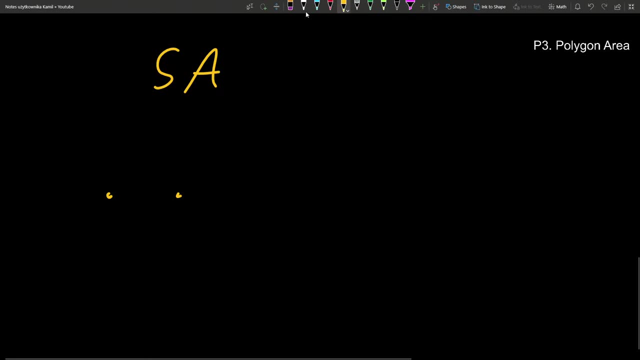 that there is some sand here, right, and you you have, there is a pole or anything like that, some kind of nail, and you have a broom or not, maybe not a broom. this is a line. i mean a rope. yeah, i mean a rope or not, maybe not a broom, this is a line, i mean a rope. 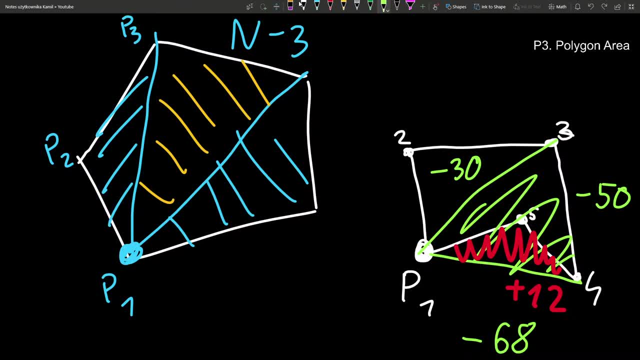 That's wrong. You need to take Values given to you by cross product With sign, Sum them all up And then the meaning of sign here is this: 68 is exactly area Of polygon, While minus will tell you If you went clockwise or counterclockwise. 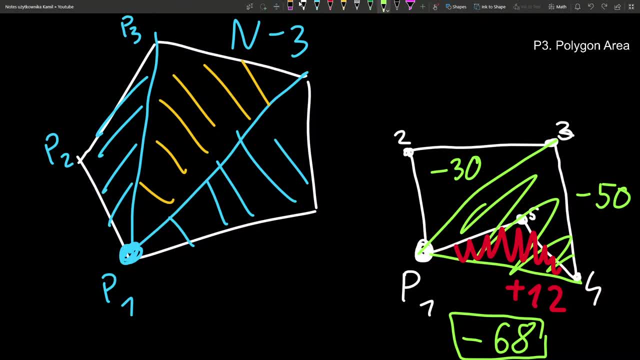 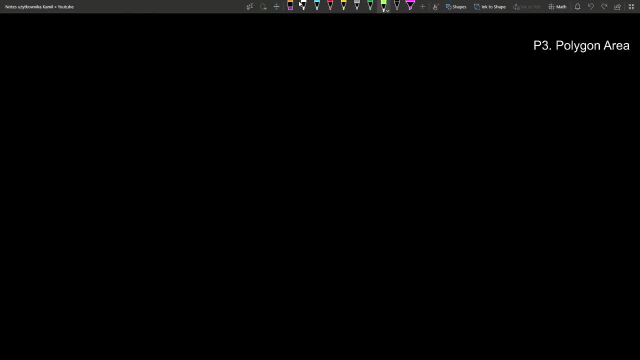 Through polygon. If you ever need that, At the end I print absolute value of this. One more way to look at it Is that With respect to any point P1. When you already covered some part, Then you already keep. 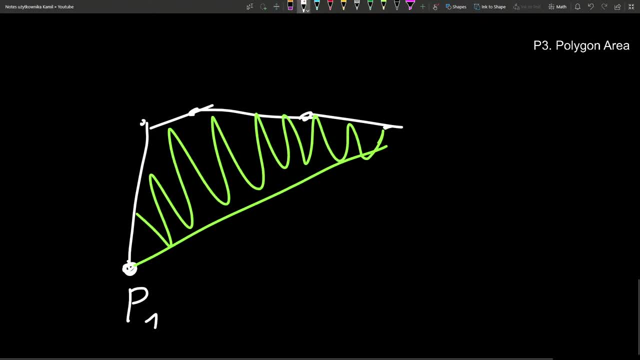 Area of this When you move forward, Then you add area of a new triangle, Possibly sometimes subtracting, And then You might subtract, You might add again: Polygon can look very Crazily. Let's say that it looks like this: 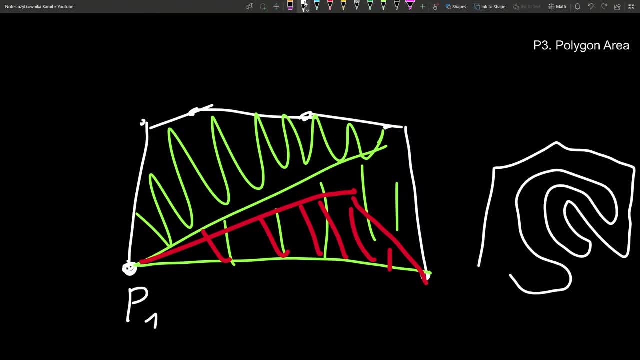 You know, It's not Easy to believe that. if this is the case, Of course, Assume that every small segment is a segment. It doesn't have curves. But this is polygon, Not convex. Why does it still work? How to feel more convinced about it? 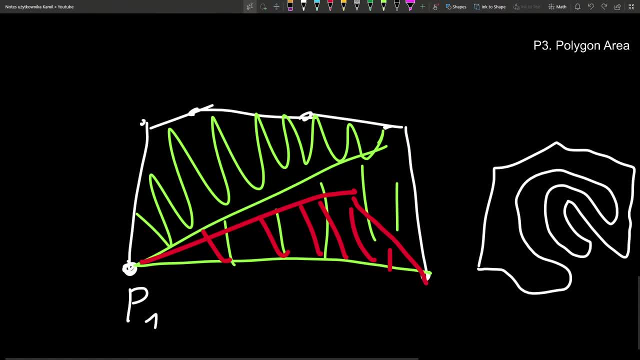 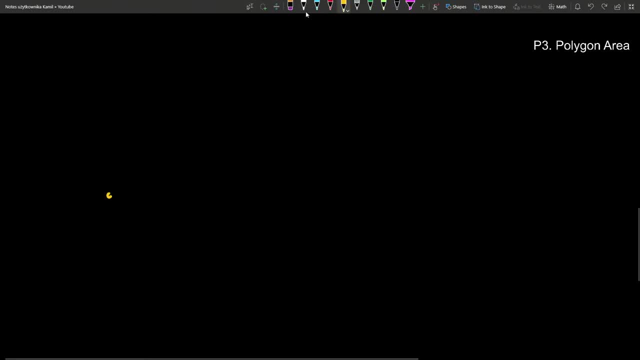 This. This would be a little bit better With real life experiment, But I don't have sand. Imagine, though, That there is some sand here, Right, And you You have. There is a pole Or anything like that, Some kind of nail. 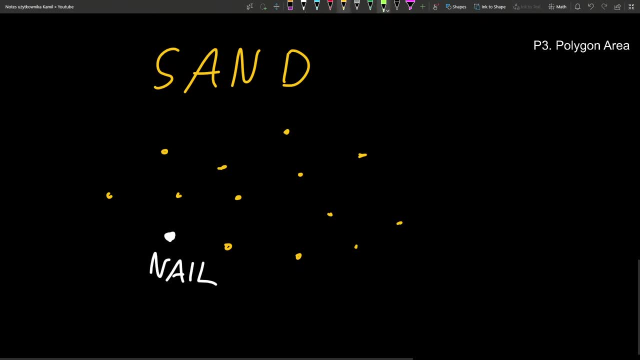 And you have a broom, Or maybe not a broom. This is a line. I mean a rope, I mean a rope, And you are a human. You stand there And you keep moving, Whenever you move to the right. 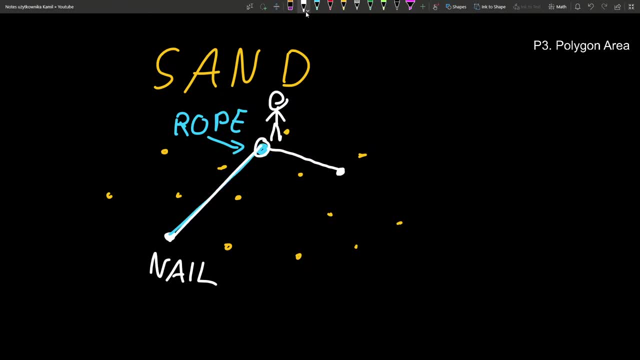 Looking from nail. Then this rope moves along you And it is elastic, The length changes, It adjusts. At some moment rope is here, Then it is here, It is there, And so on. And now this area that you covered. 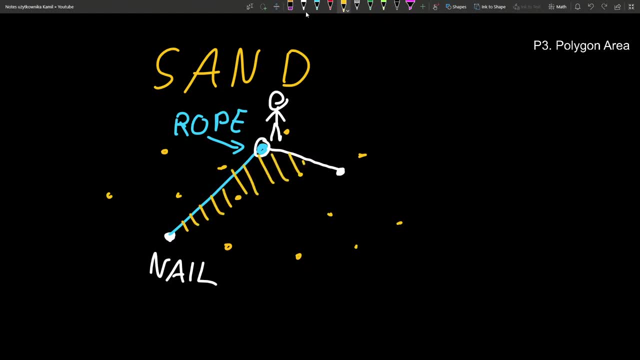 Let's say that you even out a sand. Then, after you move, This sand is smooth, Smooth sand. But here is the thing: This rope is Actually not symmetrical. Imagine that this is: This is a rope, And when you move to the right, 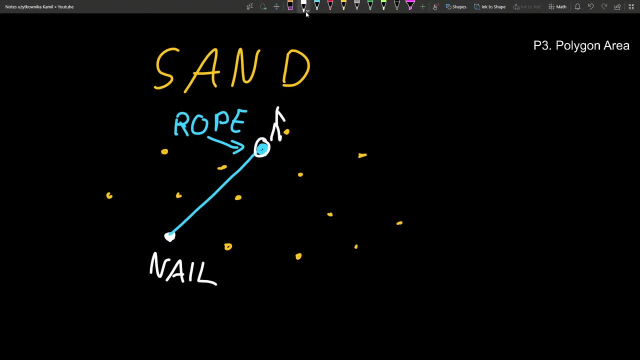 and you're a human. you stand there and you keep moving. whenever you move to the right, looking from nail, then this rope moves along you, alongside you, and it is elastic: the the length changes, it adjusts. at some moment rope is here, then it is here, it is there, and so on. and now this area that you covered. 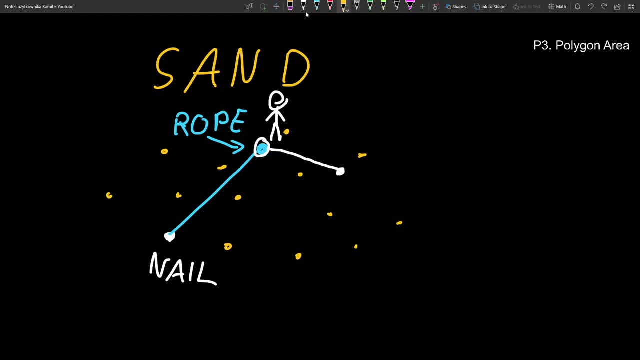 let's say that you even out a sand, like then, after you move. this sand is smooth, smooth sand. but here's the thing: this rope is actually not symmetrical. imagine that this is: this is a rope. but here's the thing: this rope is actually not symmetrical. imagine that this is: this is a rope. 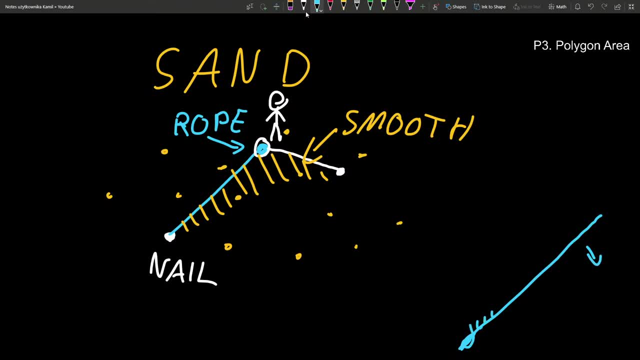 and when you move to the right it's very nice, because here it has some nice material, but actually in the other direction it has spikes. should i move it like that? uh, maybe not. so let's say that here it has nice material. when it touches the sand, there it's nice. 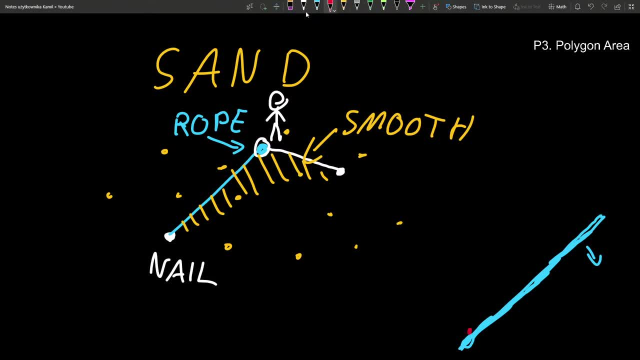 but whenever you move to the other direction, it has spikes and it makes sand not smooth. those are spikes, right. so then, whenever you now move to the right, to the left, you will destroy some sand. in this case, let's say this one, and this way you will cancel nice sand and make nice sand. 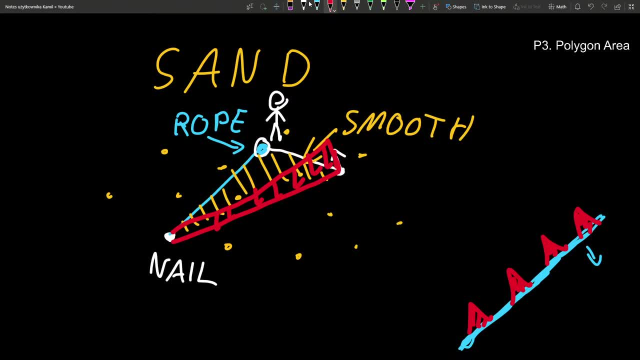 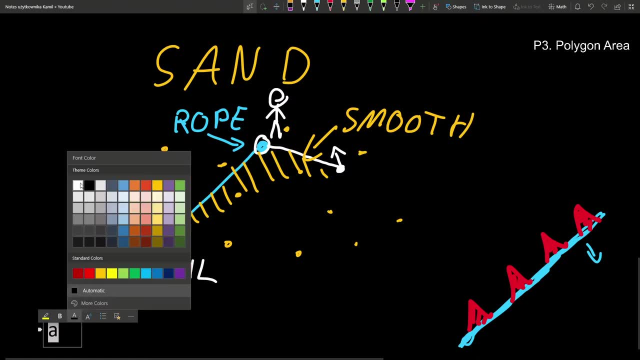 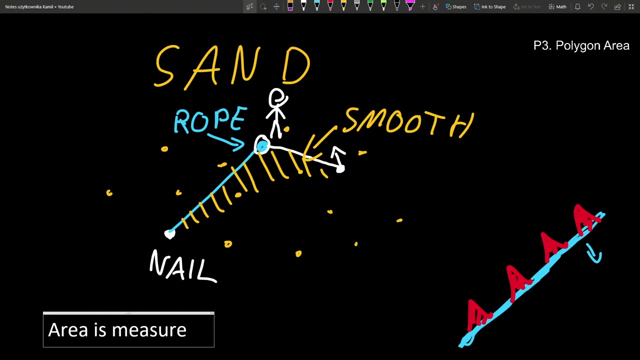 i know it's quite crazy analogy, but eventually you need to understand this. uh, let me write this down because this is very important. area is equal to is defined basically as the kind of amount of points inside the triangle right whenever somebody asks you to compute area of polygon, it is in some way equivalent. 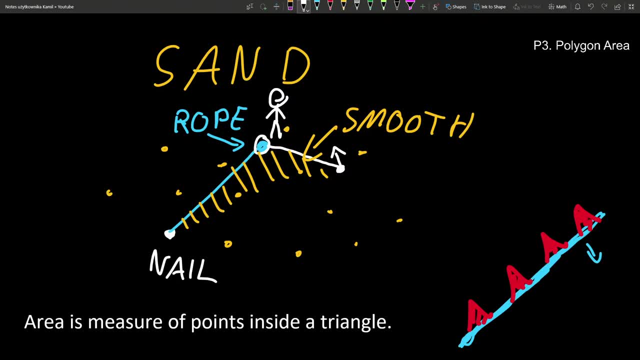 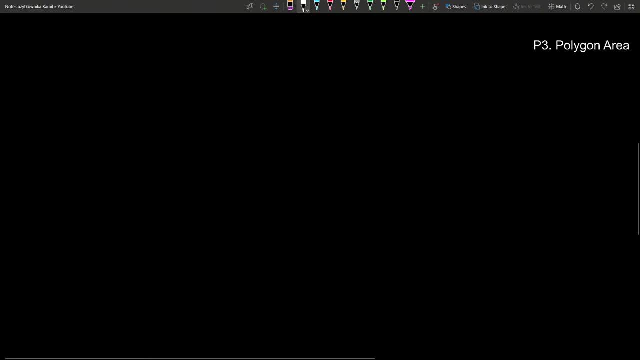 to asking how many points are inside. there are infinite number of them, but it is some amount, some kind of measure. in other words, we could look at every point and check if it is inside a polygon. how to do it? if we look at single point and this nail the point with respect to which we move and we have rope. 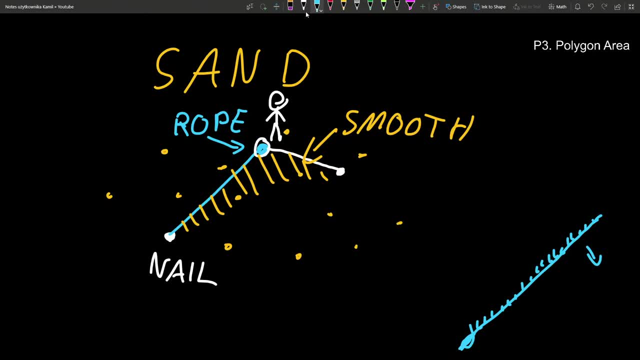 It is very nice Because here it has some nice material, But actually in the other direction It has spikes. Should I move it like that? Maybe not. So let's say that Here it has nice material When it touches the sand there. 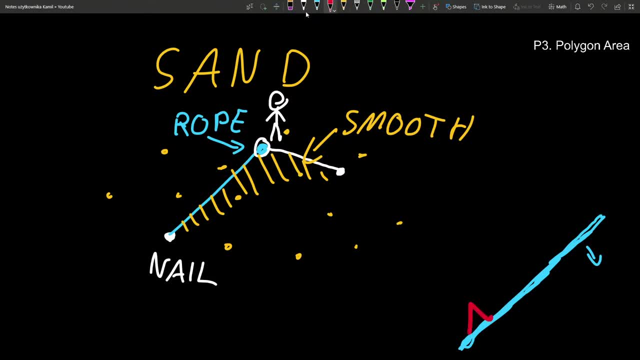 It is nice, But it has spikes And it makes sand not smooth. Those are spikes. So then, Whenever you now move to the left, You will destroy some sand. In this case, Let's say this one And this way: 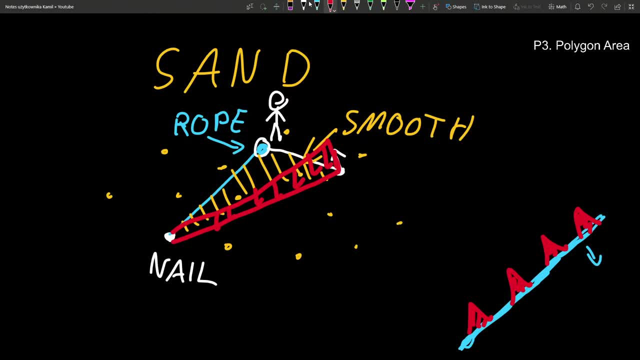 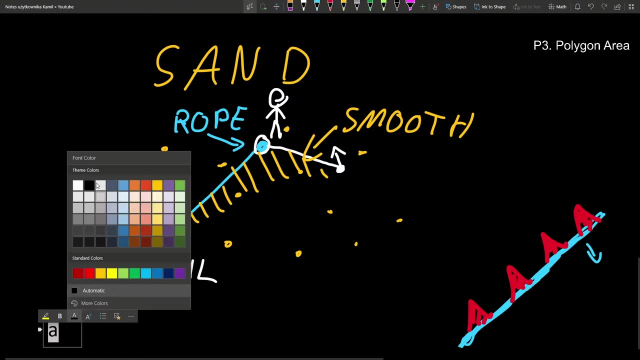 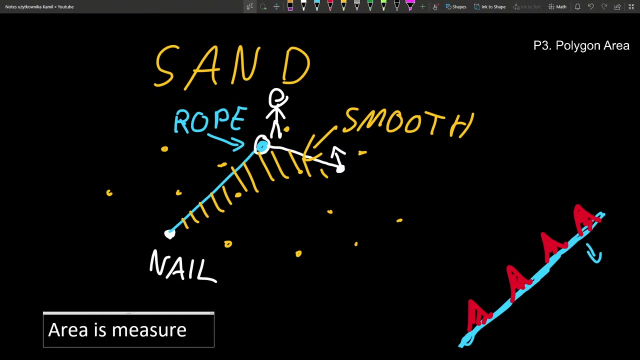 You will cancel Nice sand And make nice sand. I know This is quite crazy analogy, But Eventually You need to understand this. Let me write this down Because this is very important. Area Is equal to Is defined basically. 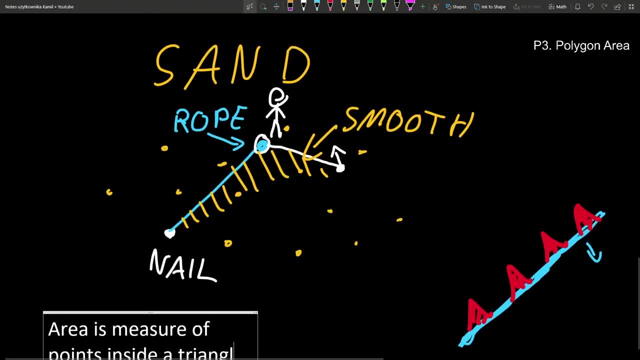 As the amount of points Inside a triangle. Whenever somebody asks you to Compute area of polygon, It is in some way Equivalent to asking How many points are inside. There are infinite number of them, But it is some amount, Some kind of measure. 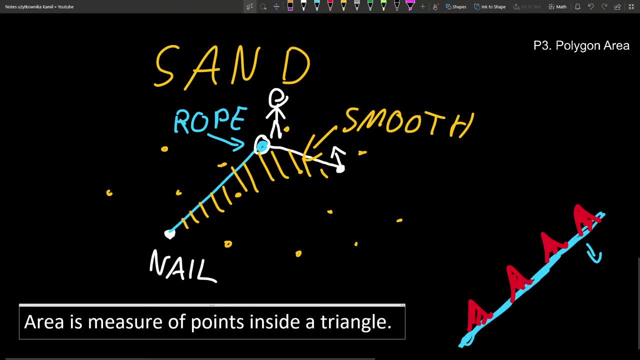 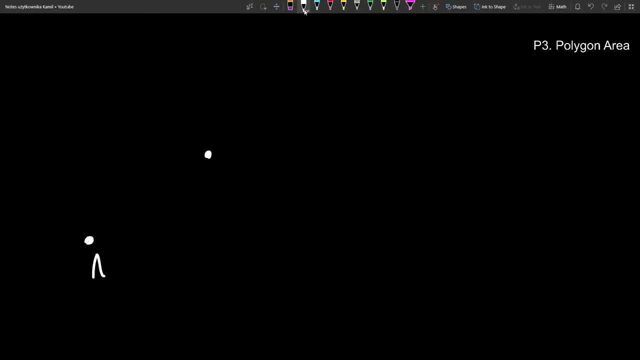 In other words, We could look at every point And check if it is inside a polygon, How to do it? If we look at single point And this nail Point with respect to which we move And we have rope, And we are here. 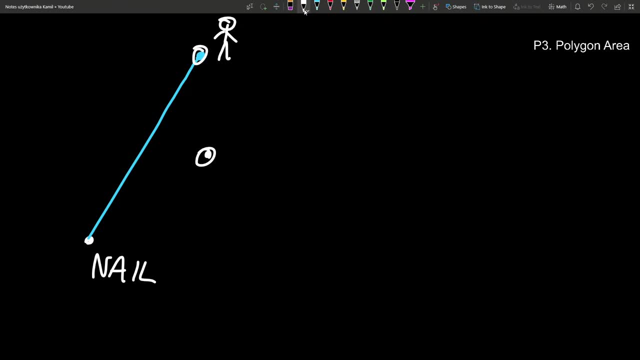 You can, for a single point, Investigate what happens with it. Whenever we move To the right And we touch it with nice part of the rope, Then This point becomes Evened out. It becomes nice smooth sand, Let's say, the next point of polygon is here. 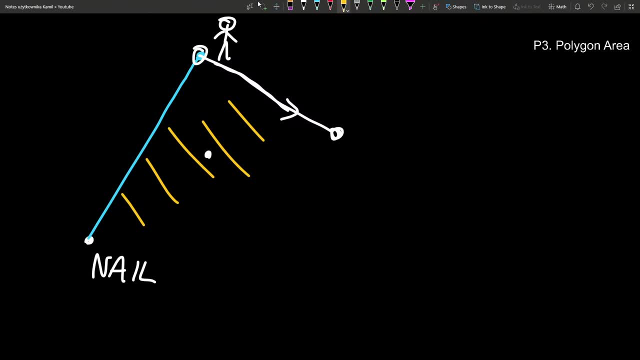 Then everything here Becomes smooth. Then, When we move To the left, Everything here Will become bad And you just need to look at point And investigate What happened with it As you moved along Whenever you. This is our point. we are investigating. 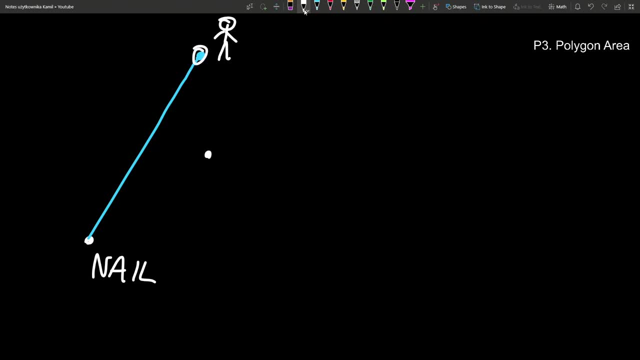 and we are here. you can, for a single point, investigate what happens with it. whenever we move to the right and we touch it with nice part of the rope, then this point becomes evened out. it becomes nice smooth sand, right when, let's say, the next point of polygon is here, then everything here became smooth. 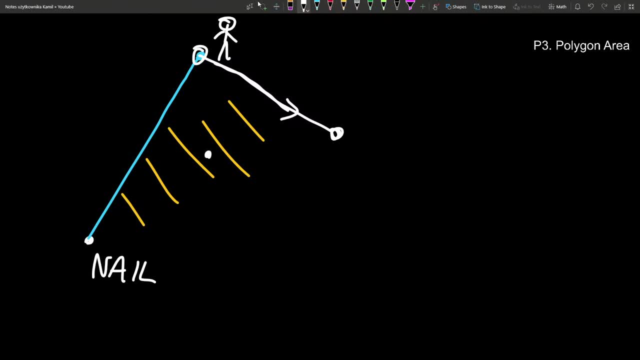 then when we move, let's say there, everything here will become bad and you just need to look at point and investigate what happened with it as you moved along whenever you- this is our point we are investigating- whenever you move to the right, this becomes good. whenever you move to the left. 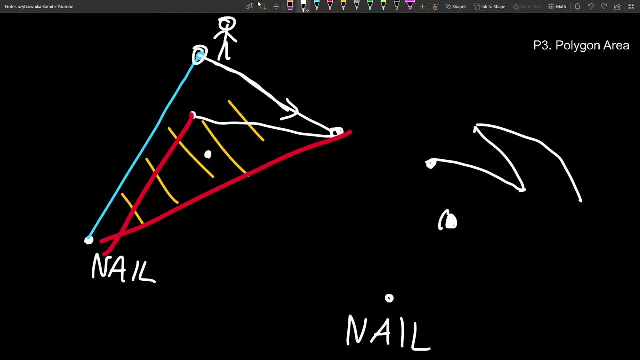 this becomes bad when you move to the right. this becomes good when you move somewhere here. nothing happens. this does not work. do anything with this point. why? because right now our rope is here. it does not touch this. so this interpretation- surprisingly, this interpretation with rope- correctly understands when we say we point is inside a polygon. 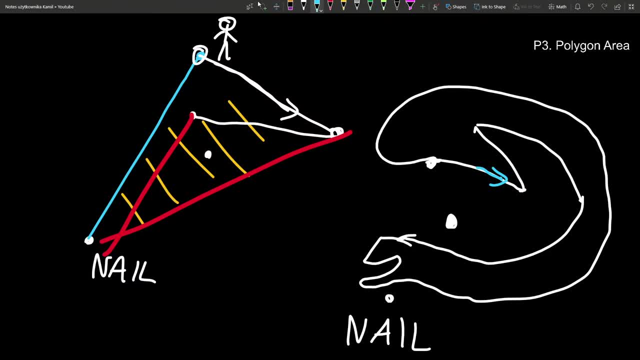 like when, when only i went like that, i said, this become became good. like this, this became bad because at this point my rope was like that: it moved to the left, so it touched my point with spikes. later, like that became good. eventually, when we move here to the left, we touch the. 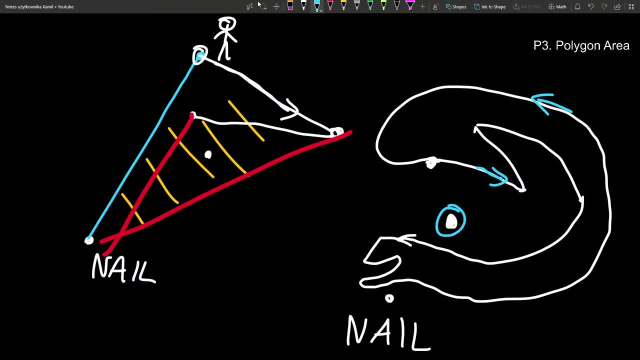 point with spikes. so eventually this became bad again. four times the rope touched point. two times it was with spikes, two times it was with nice material. so at the end this is not nice, not smooth, meaning not inside the polygon. this interpretation will be useful later too, for 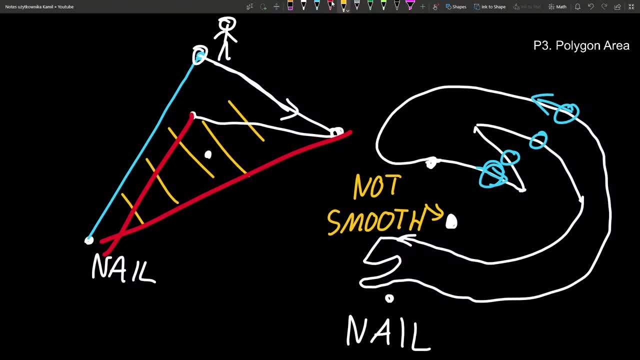 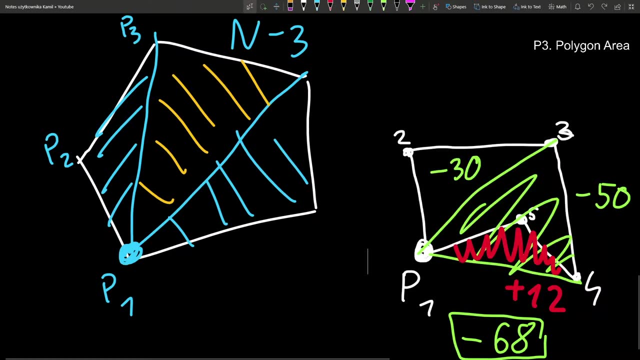 checking if there is a problem. check if point is inside the polygon. nail is point with respect to which we compute. everything like when i told you about this: p1 would be a nail here. p1 would be a nail, but surprisingly it doesn't be. it doesn't have to be part of a polygon. also, we started with 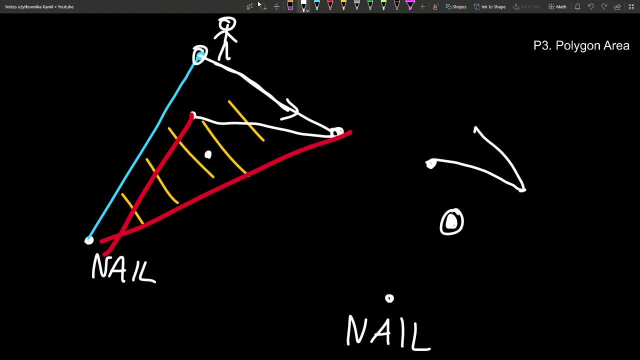 Whenever you move to the right, This becomes good. Whenever you move to the left, This becomes bad. When you move to the right, This becomes good. Then everything with this point? Why? Because right now our rope is here, It does not touch this. 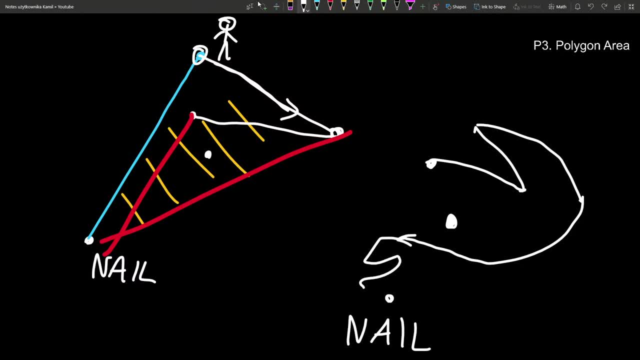 So this interpretation- Surprisingly This interpretation with rope- Correctly understands When we point is inside a polygon Like when, When only I went like that, I said, this became good Like this. At this point, my rope was like that. 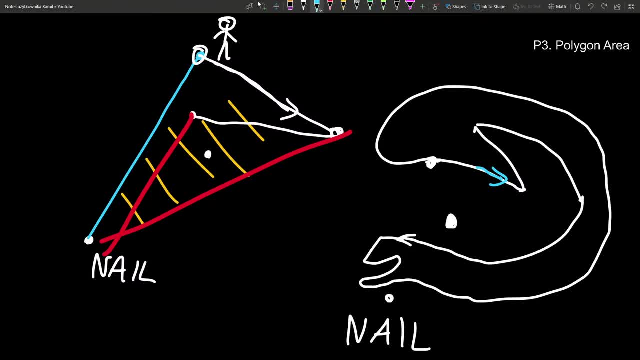 It moved to the left So it touched my point with spikes Later, like that, became good. Eventually. When we move here to the left, We touch the point with spikes, So eventually this became bad again. Four times the rope touched point. 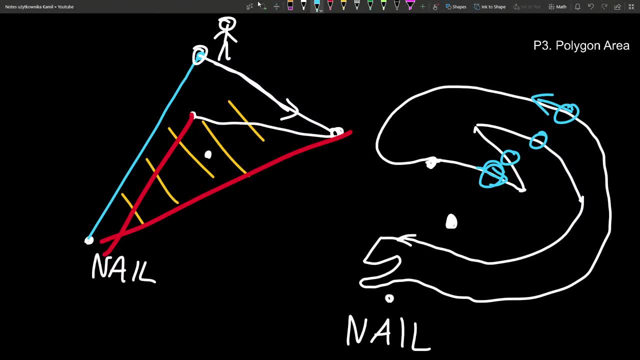 Two times it was with spikes, Two times it was with Nice material. So at the end this is Not nice. It does not move Meaning Not inside the polygon. This interpretation will be Useful later too For checking if there is a problem. 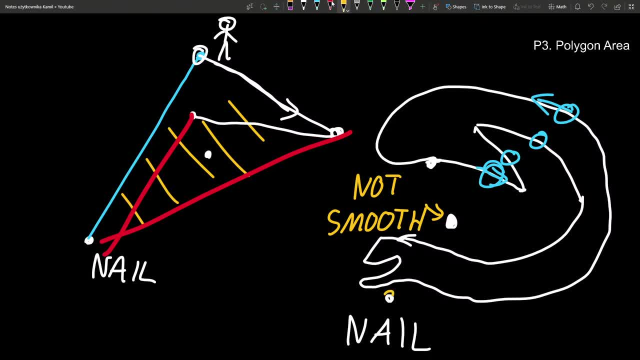 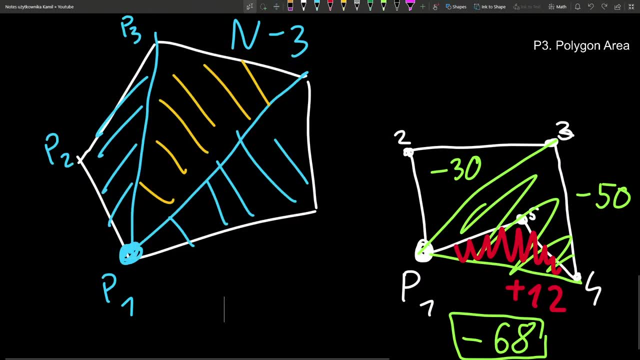 Check. if point is inside the polygon Nail is point with respect to which We compute. everything Like when I told you about this: P1 would be a nail Here, But surprisingly It doesn't be. It doesn't have to be. 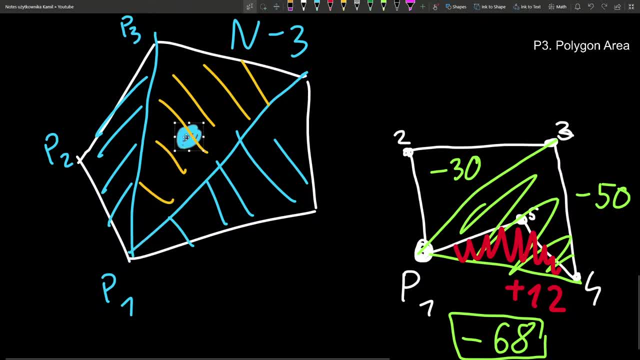 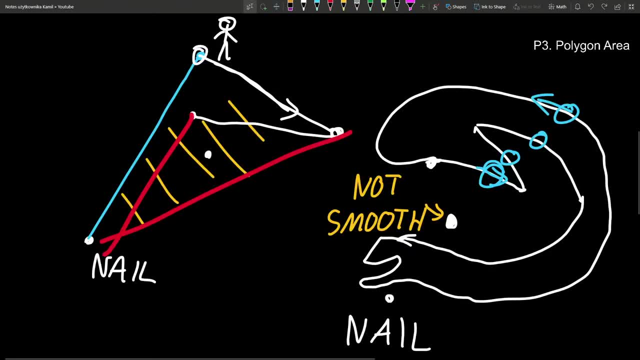 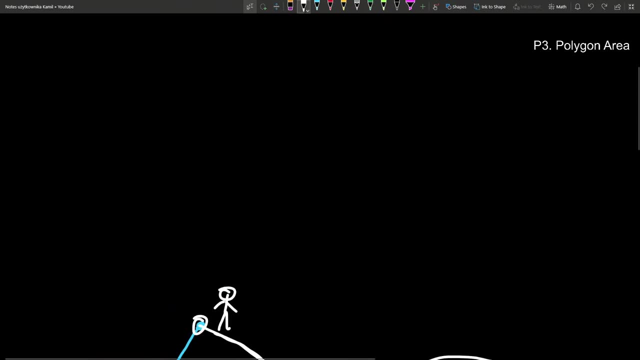 Part of a polygon. Also, we started with saying that We take with respect to point Inside the polygon. It can be outside as well. So this nail Doesn't need to be inside a polygon Or anything like that. It doesn't have to be part of a polygon. 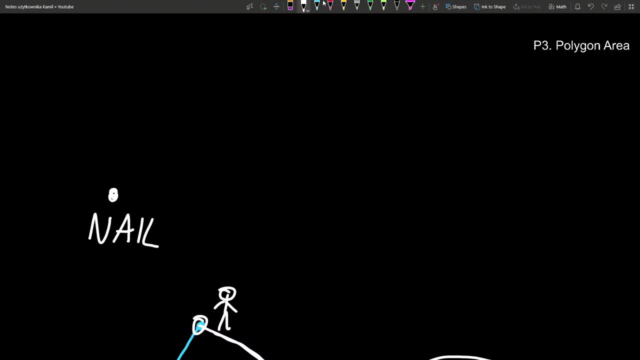 So when this is nail Or in geometry, Point zero, zero, And then we investigate this, Let's say just four points. We can start from Whenever, Wherever. Let's say, this is the first point, And then we move there. 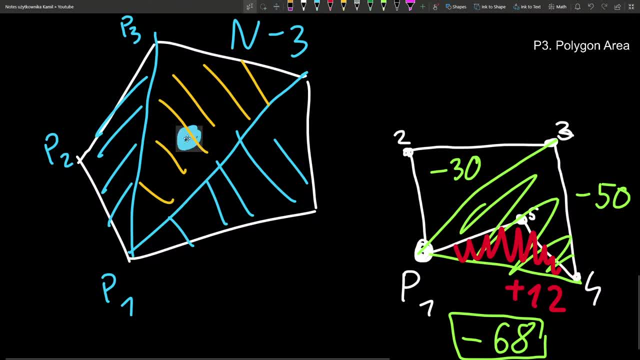 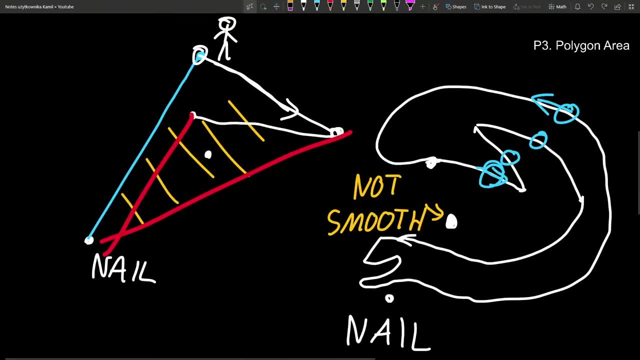 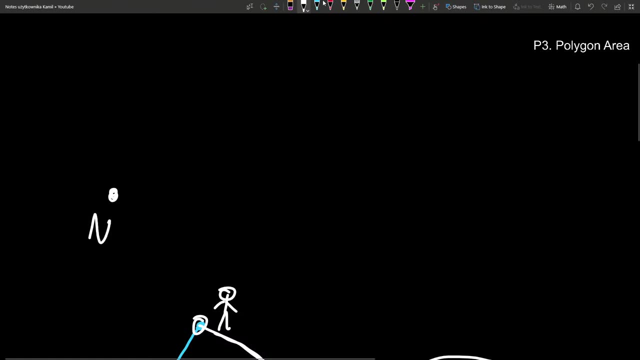 saying that we take with respect to point inside the polygon, it can be outside as well. so this nail doesn't need to be inside a polygon or anything like that. it doesn't have to be part of a polygon. so when this is nail or in geometry, point zero, zero. 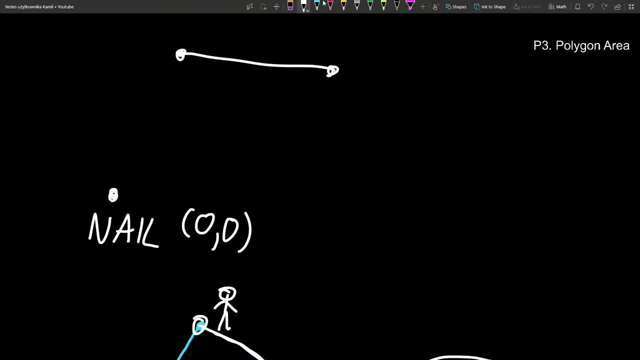 zero and then we investigate this. let's say just four points. we can start from whenever, wherever. let's say this is the first point and then we move there. so our human starts here. has this rope, the rope we moved with rope to the right. this area becomes nice now. 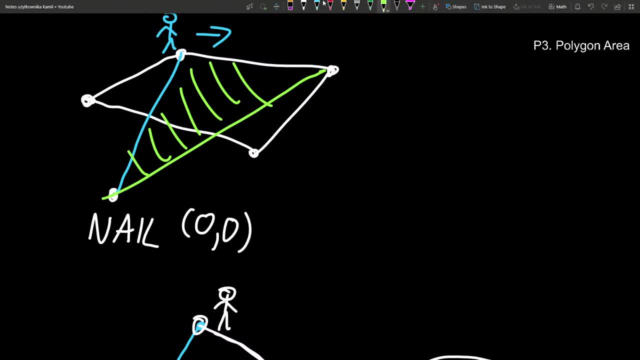 now for all points here inside. i would say that it is smooth, a smooth point. then we move there, so we also cover this part. what happens next? from here? we move there. rope follows this pattern, but it moves to left, so it touches this area with spikes. every point becomes bad. 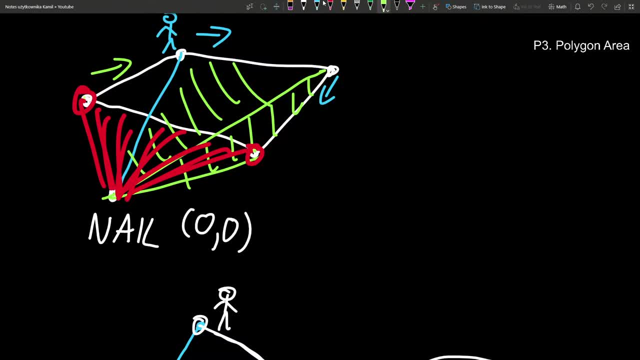 and then we go again clockwise with respect to the nail. so we add this area almost there, so everything here almost there, subtracted once added, or in terms of rope: it was once touched nicely and once badly with spikes, so it cancelled out. it cancels out for any point here. we would say that it becomes once bad was. 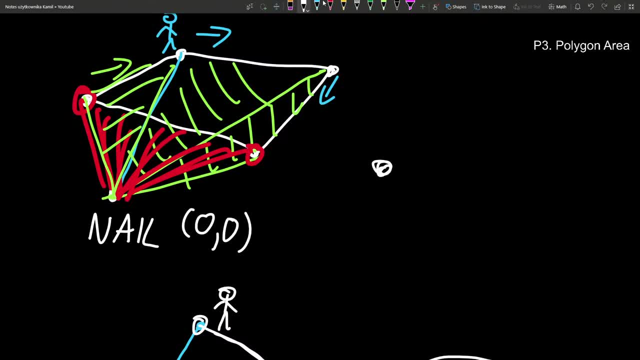 good, so it's neutral, like any point here, outside it's. it is outside and for this just green area, it is area of a polygon, everything inside the polygon. it was touched nicely, more by once than touched badly, and this explains another very well-known algorithm. when you want to test, 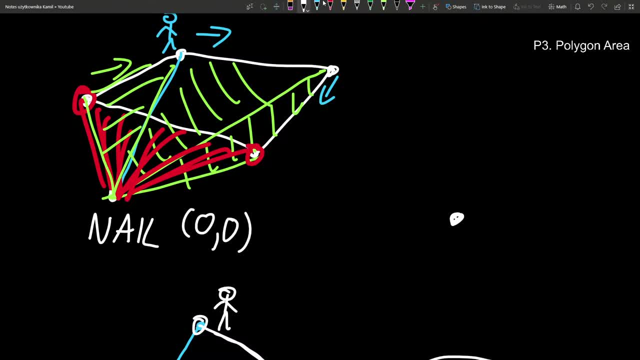 if point is inside a polygon, and this polygon can really be crazy. i can even draw such a case that it will be hard for me to say if it's inside or not. now i don't know how to finish the polygon, sorry, okay, like when i draw a point here, is it inside or not? 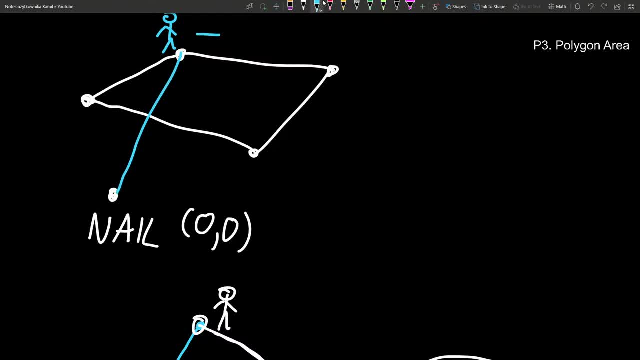 Our human starts here, Has this rope. We move with rope to the right. This area becomes nice. Now, for all points here inside, I would say that it is smooth, A smooth point. Then we move there. We also Cover this part. 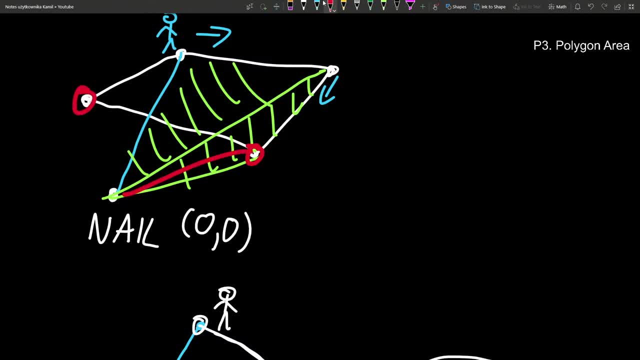 What happens next? From here we move there. Rope follows this pattern, But it moves to left, So it touches this area with spikes. Every point becomes bad, And then we go again Clockwise with respect to the nail. So we add this area. 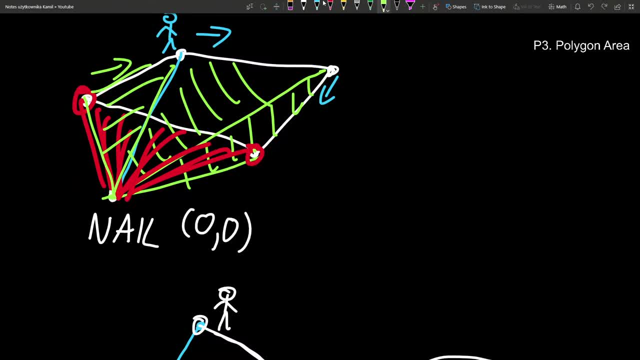 Everything here Was once subtracted, once added, Or in terms of rope, It was once touched nicely And once badly. with spikes It cancels out For any point here. We would say that it becomes once bad, once good, So it's neutral. 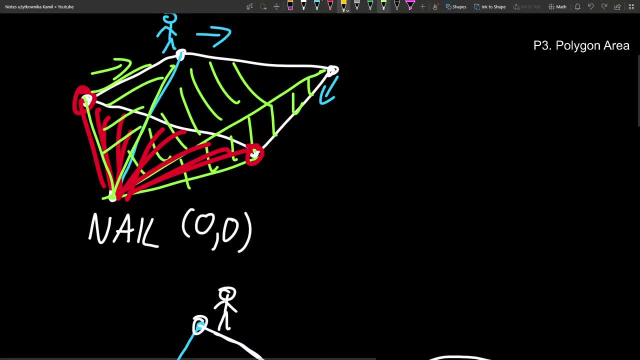 Like any point here, outside It is outside And for this just green area It is area of a polygon, Everything inside a polygon. It was touched nicely More by once And this explains Another very well known algorithm. When you want to test, 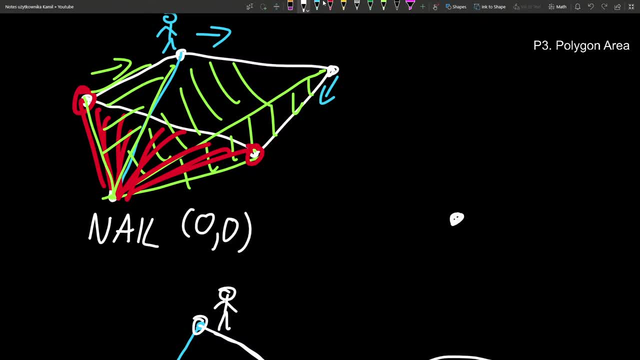 If point is Inside a polygon, And this polygon can really be crazy. I can even draw such a case That it will be hard for me to say If it's inside or not. Now I don't know how to finish the polygon. 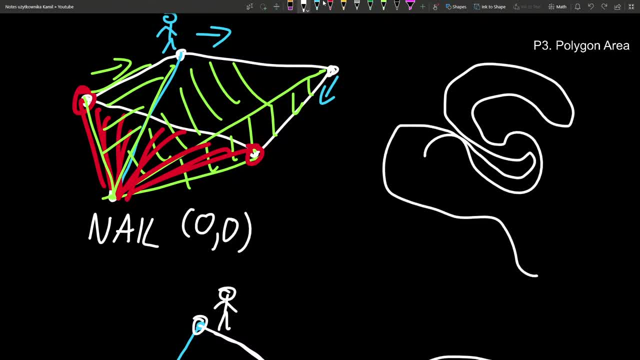 Sorry, When I draw a point here, Is it inside or not? This one? I can always draw any kind of ray And investigate The number of intersections, Whether it's even or odd. Maybe this is more correlated With the fact that. 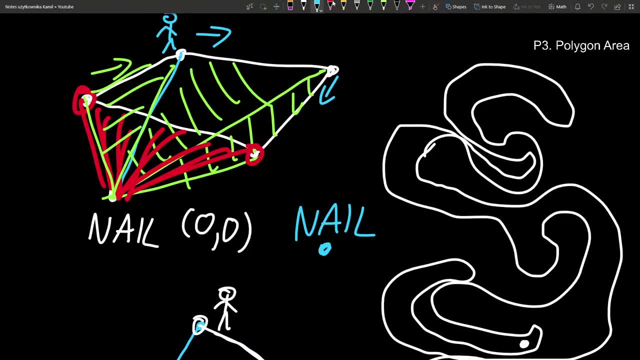 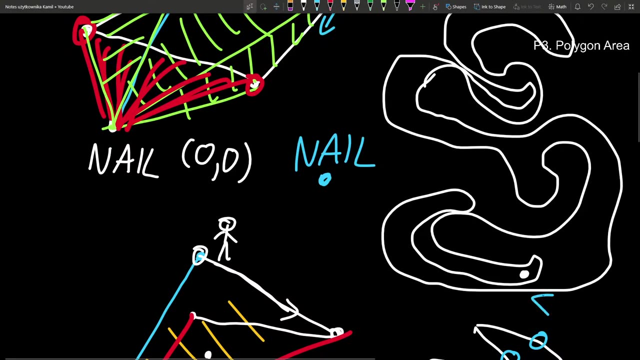 If it's outside, Then It's a bit easier to understand What happens. Because We Touched this point, we've eroped In two points. I will scroll this a little bit down And we will remove that. Sorry about some chaos here. 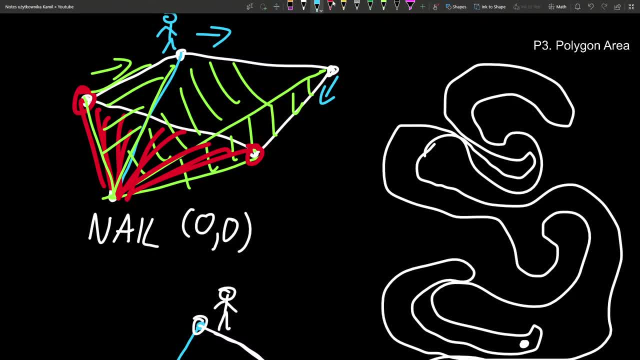 this one. i can always draw any kind of ray and investigate the number of intersection, intersections, whether it's even or odd, like. maybe this is more correlated with the fact that, well, if this is a nail here, if it's outside, then it's a bit easier to understand what happens, because 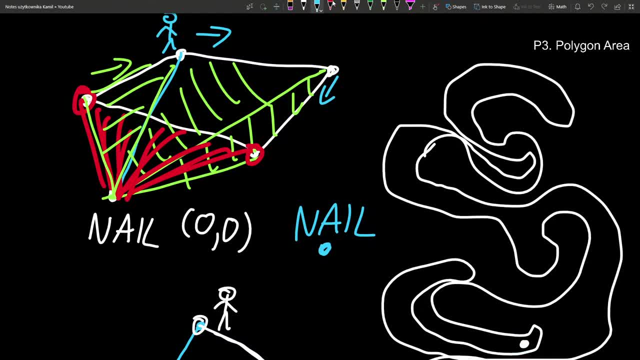 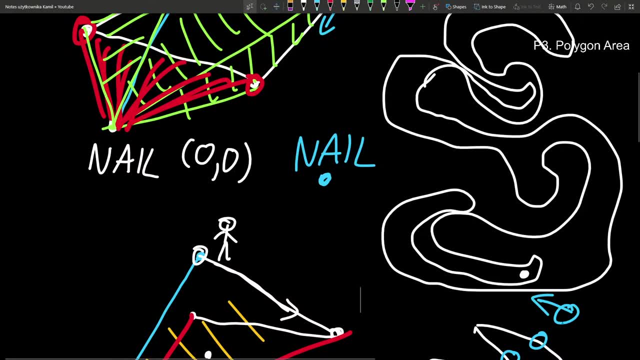 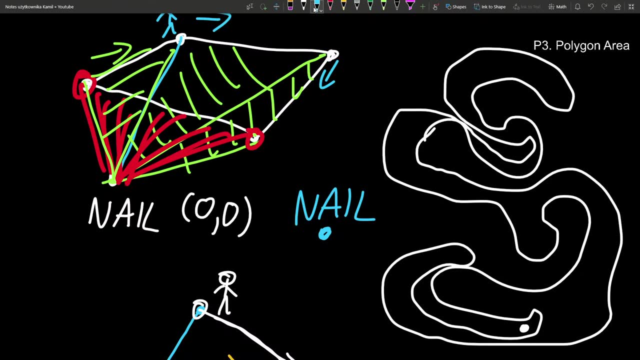 we touched this point with a rope in two points. i will scroll this a little bit down and we will remove it. sorry about some chaos here. this is not an easy concept, right? how many times we touched this point with a rope when we started from there and we followed this white path? 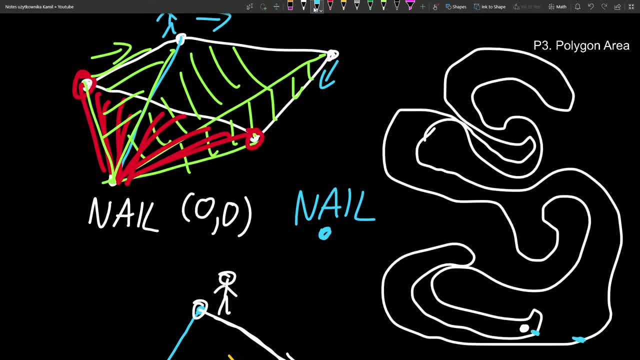 in two places: this one when we were here, and there when we crossed this point. the rope was like that, so it crossed this point. in other words, and this is the well-known algorithm- we draw a ray, infinite ray, starting from point we are investigating with direction opposite to. 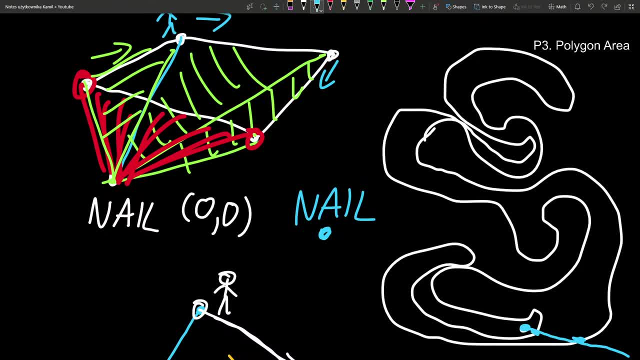 the nail, the point with respect to it. if we compute area of polygon and now if it's even number of intersections, it means it was, let's say, k times to the left, k times to the right. it must be like that, otherwise once more we moved in one direction. it means it is inside. 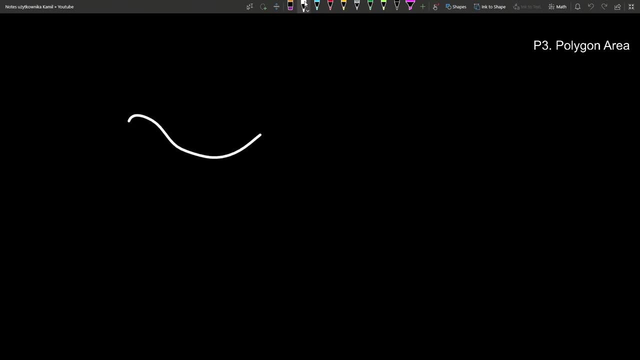 so whenever you see the algorithm to check if something inside is inside the polygon and you use the algorithm by counting number of intersections with polygon, with any kind of ray, this is equivalent to saying that the nail is here nail, actually, it doesn't need to be inside. 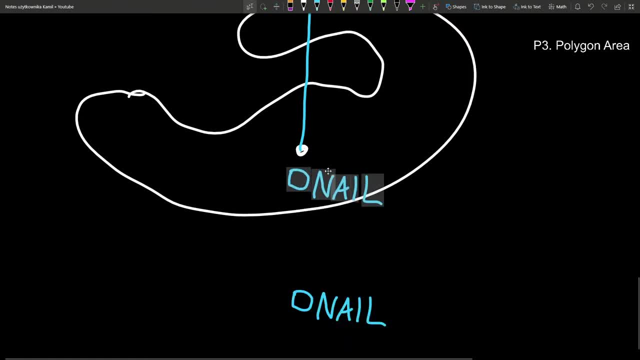 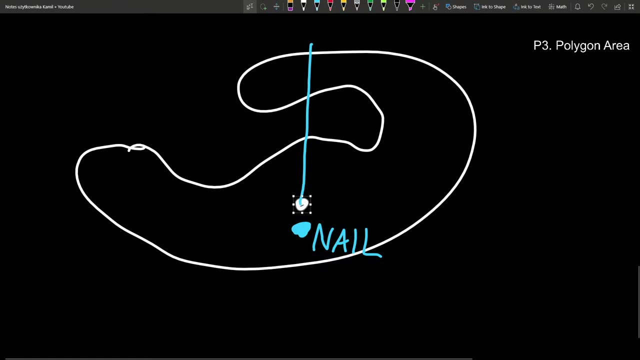 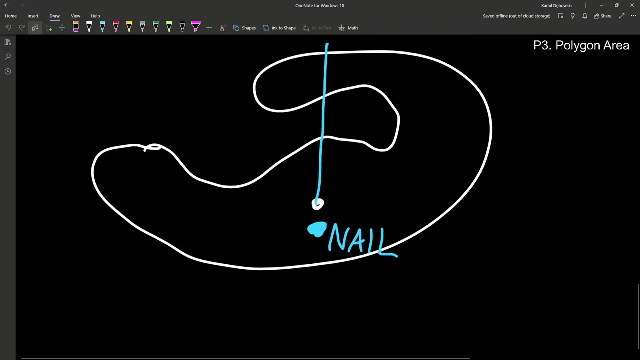 everything i said would be equally true if it was here. maybe this is point not really. a square nail is here and then whenever you intersect here, here, there, something will happen with this point. we're investigating- right, that was a long tangent- how to compute area of polygon. we will, that's easy. 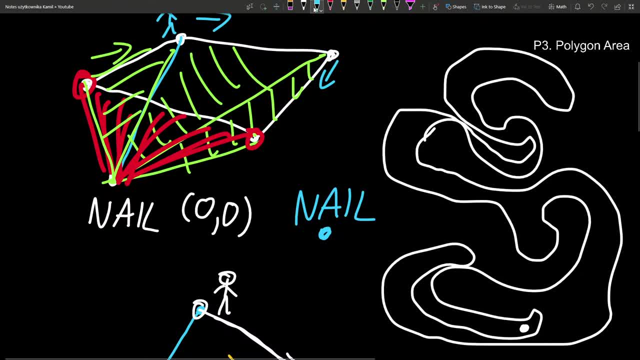 This is not an easy concept, Right. Many times We touched this point with a rope When we started from there, And we followed this white path In two places: This one When we were here and there When we crossed this point. 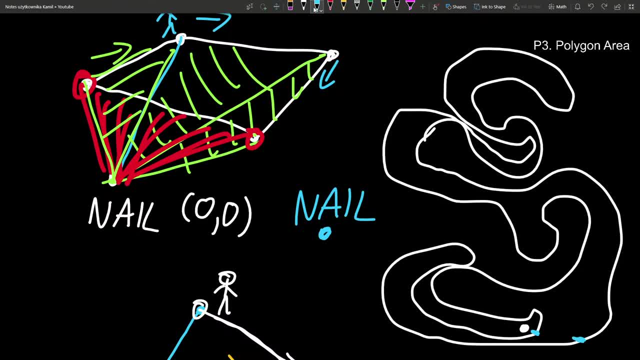 The rope was like that, So it crossed this point. In other words, And this is the well-known algorithm, We draw a ray, Infinite ray, Starting from point we are investigating, We compute area of polygon, And now, If it's even number of intersections, 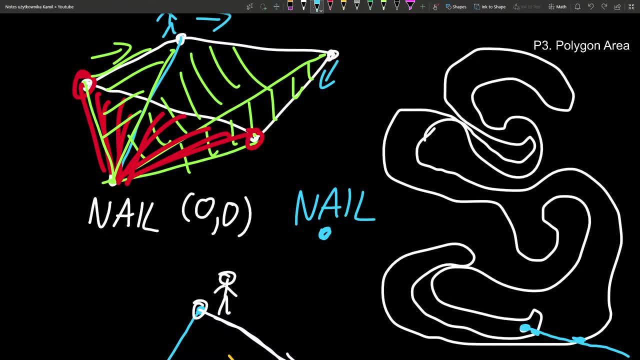 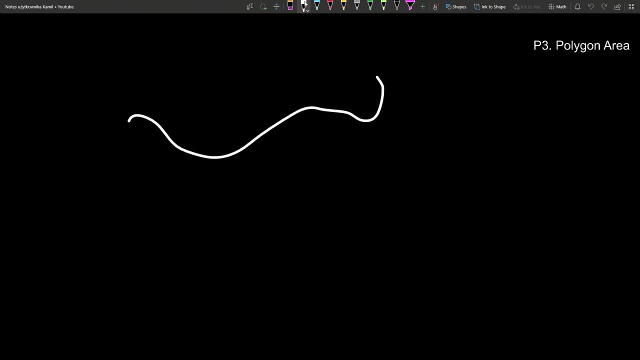 It means it was, Let's say, k times to the left, K times to the right. It must be like that, Otherwise, Once more we moved in one direction. It means it is inside, Whenever you see the algorithm To check. 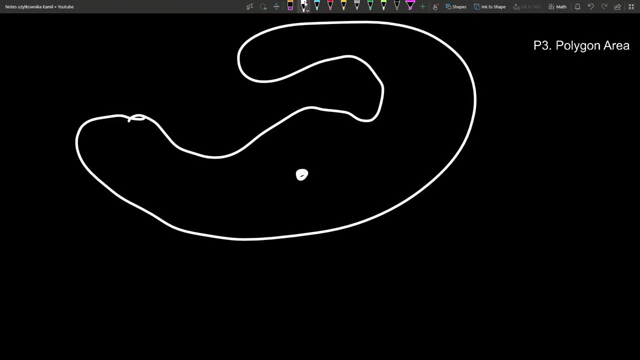 If something inside Is inside the polygon And you use the algorithm To check number of intersections With polygon with any kind of ray, This is equivalent to saying That the nail is here Nail. Actually, it doesn't need to be inside. 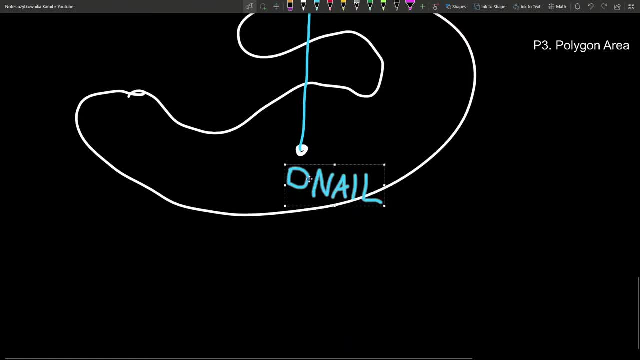 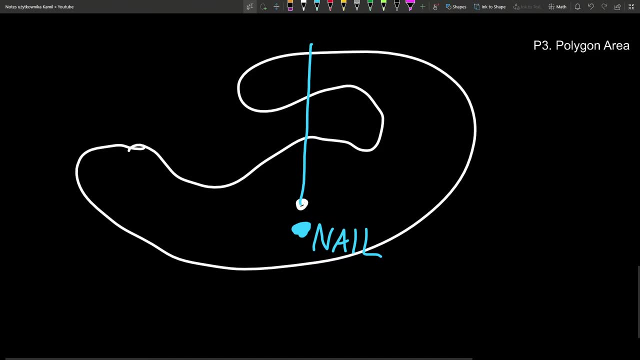 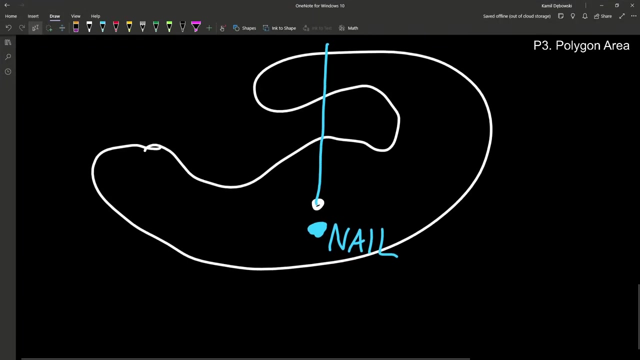 Everything I said would be equally true If it was here. This is point, Not really. a square Nail is here, And then, whenever you intersect here, Here, There You are investigating. Right, That was a long, tangent. How to compute area of polygon. 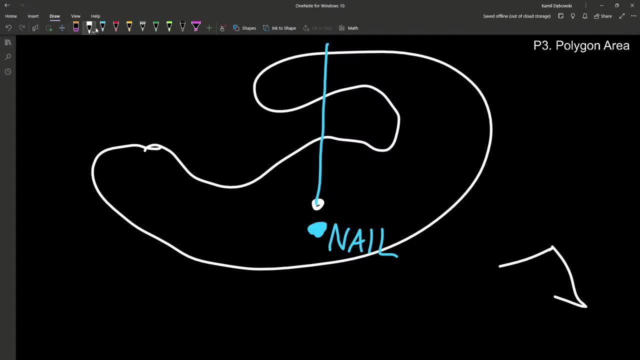 We will. That's easy With respect to point zero- zero. Because it's easiest to work With respect to point zero- zero, I will take cross product Of every two consecutive points in a polygon To add or subtract Area of triangle. 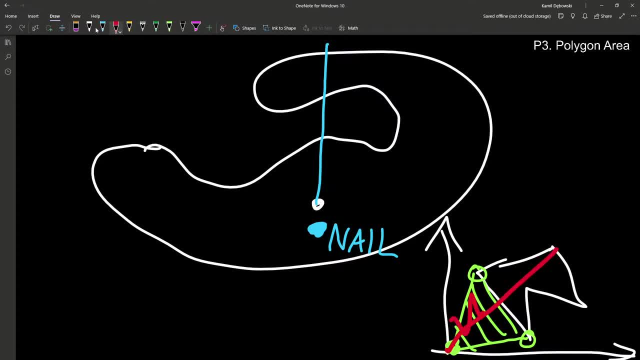 This will be taken with one sign. This will be taken with the other. So when I say, I look at these two consecutive points, Their cross product is, let's remember, Area Of this triangle, And sign will tell you Automatically if it's left or right. 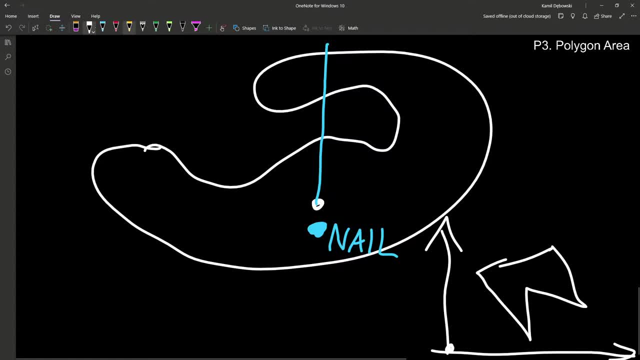 with respect to point zero- zero, because it's easiest to work with respect to point zero- zero. so we will take cross product of every two consecutive points in a polygon to add or subtract area of triangle. this will be taken with one sign. this will be taken with the. 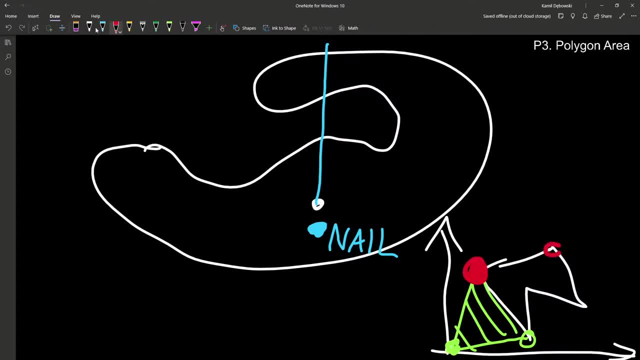 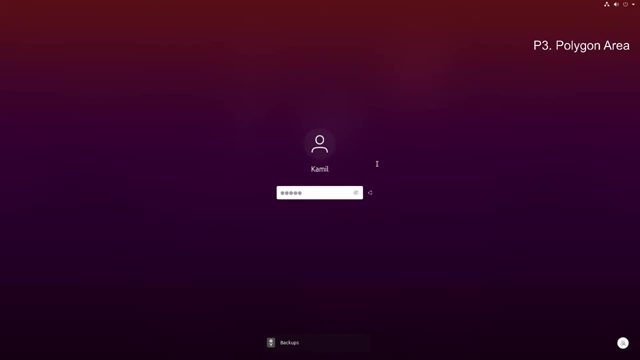 other. so when i say why i look at these two consecutive points, their cross product is, let's remember, area of this triangle and sign will tell you automatically if it's left or right, like if you should add or subtract. so this, this is basically the whole thing. i'm aware of the fact that 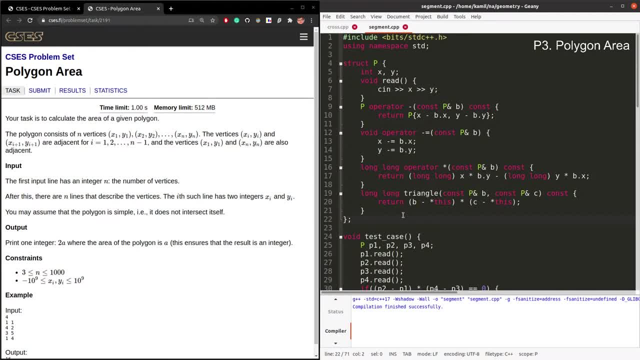 in explaining all the logic was like 10 times slower than now time needed to code it, so copy paste the template. this time. we don't have test cases. you need to read n points. click the right button and let's show the next page. i'm reading the text in text box. 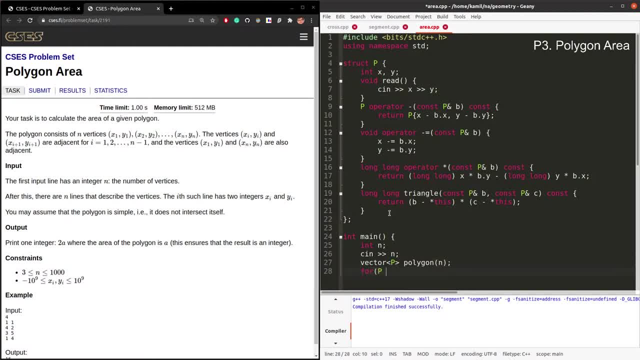 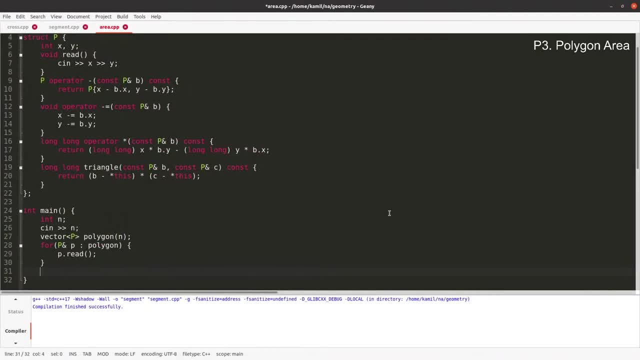 so copy paste the template, create a vector of size n, iterate over every point p and read it. what do we do now? every two consecutive points. so we take polygon of i multiplied by polygon of i plus 1, and this is automatically with plus or minus. 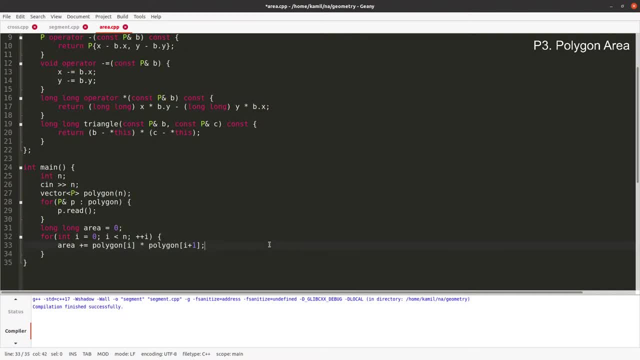 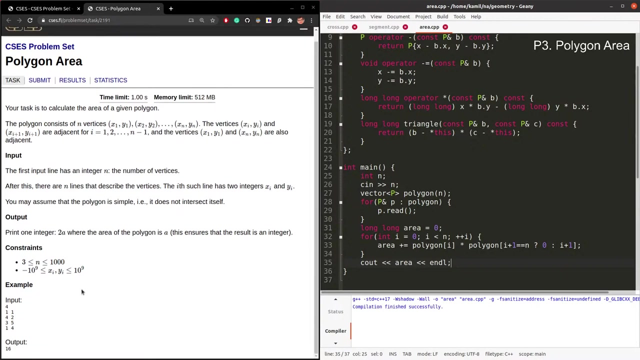 i plus 1 can overflow. i mean not overflow can be n, this is n, then 0, otherwise this. there are different ways to implement this there. whatever, let's for now print the area you ok chat. now tell me what else should I do with area at the end? 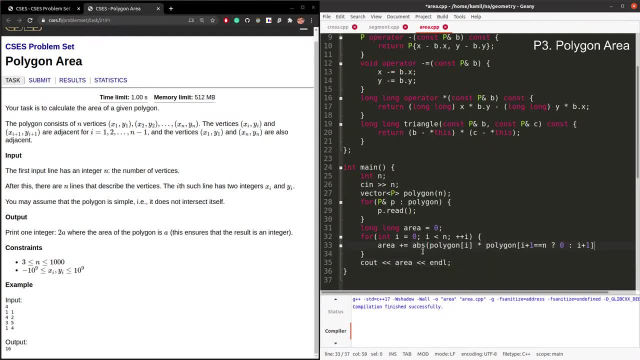 what you should already know is that I cannot take the area. I can't take absolute value here. I don't take area of every triangle. I need to take it with plus or minus. however, cross product tells me this is 16 chat. guess what value will I get here from printing area? 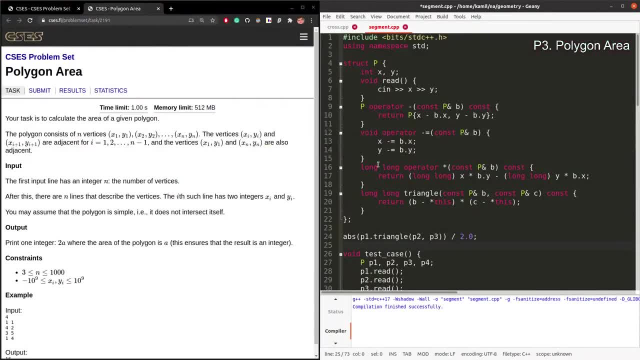 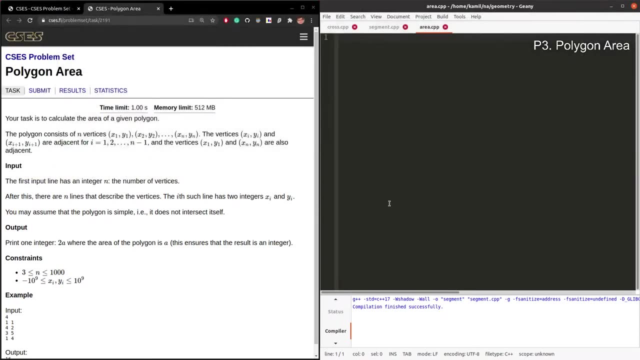 Like if you should add or subtract. I'm aware of the fact That in Explaining all, the logic Was like 10 times slower. Now Time needed to code it. Copy paste the template. This time we don't have test cases. 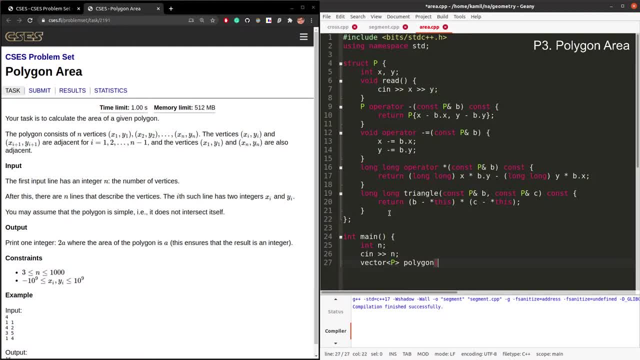 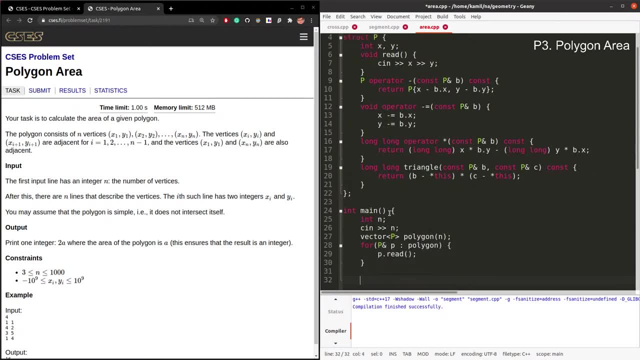 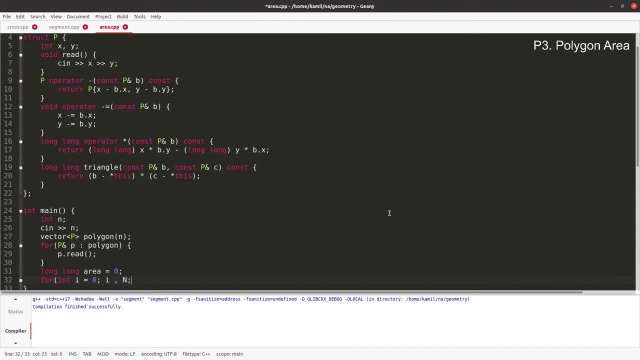 We need to read N points, Create a vector of size n, Iterate over Every point p And read it. What do we do now? Area Every two consecutive points. So We take polygon of i Multiplied by polygon of i plus one. 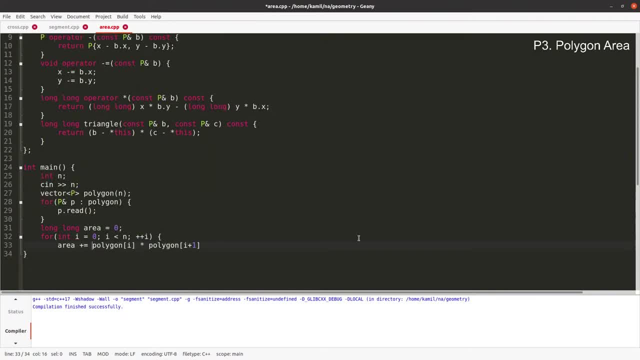 And this is automatically With plus or minus. i plus one can overflow. I mean not, overflow Can be n. This is n, Then zero. otherwise this Is not a good way to implement this Term. Let's for now print the area. 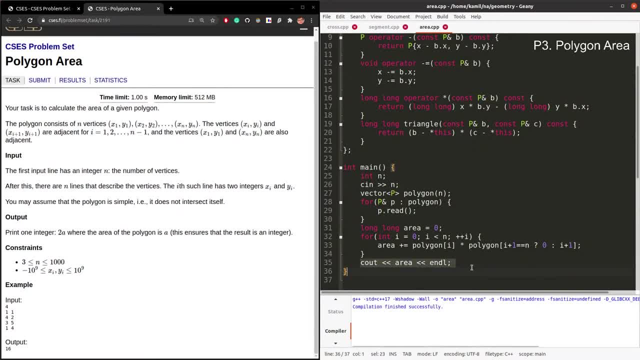 You Okay chat. now tell me, What else should I do with area at the end? What you should already know Is that I cannot take absolute value here. I don't take Area of every triangle. I need to take it with plus or minus. 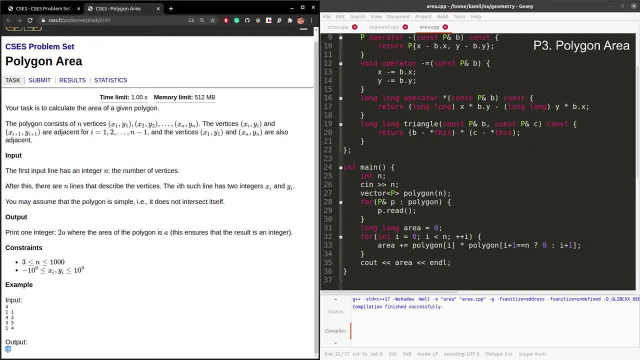 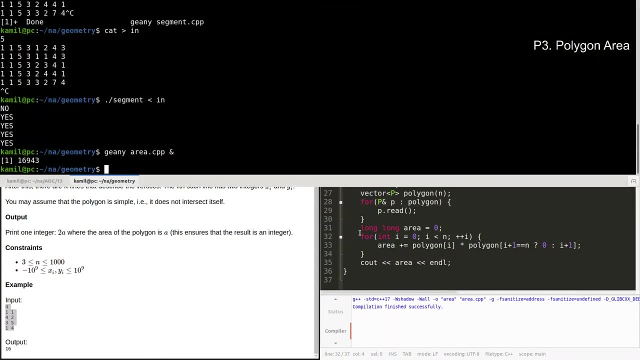 However, cross product tells me This is 16.. Chat: guess what value will I get Here from printing area? It should be 16.. We have 8 and 32 in the chat We got. I'm confused. What's going on? 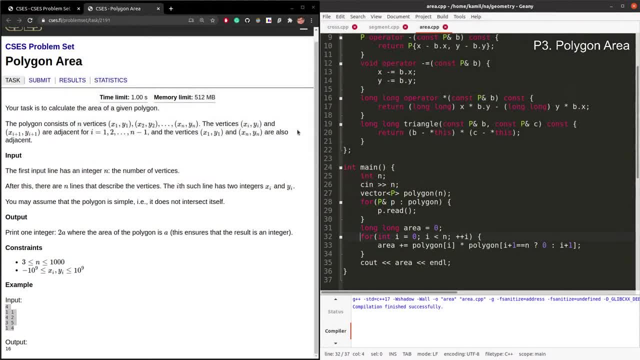 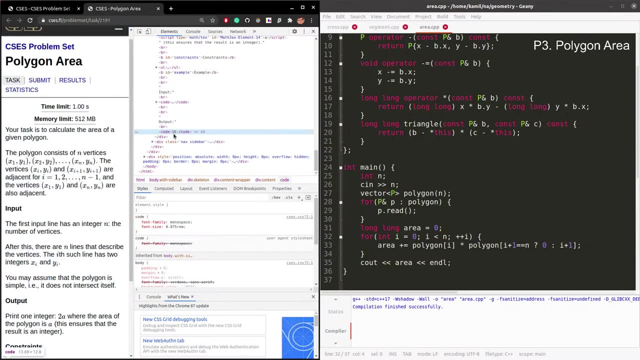 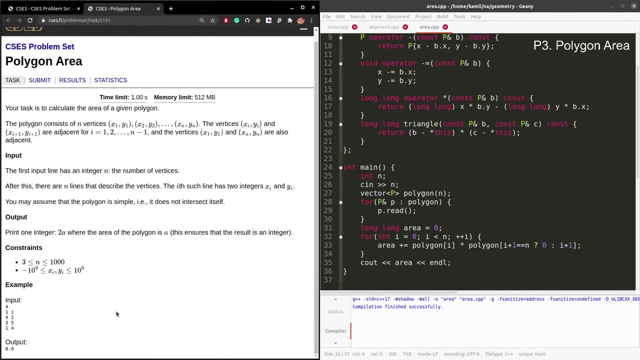 Oh, Okay, Okay, Okay, Sorry. They tell us to print twice the area. So Let's imagine it like that. If they really asked us about Area, The code would be like that: Right, This is a valid problem. 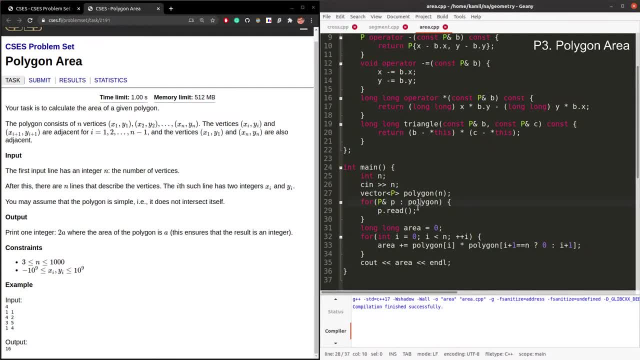 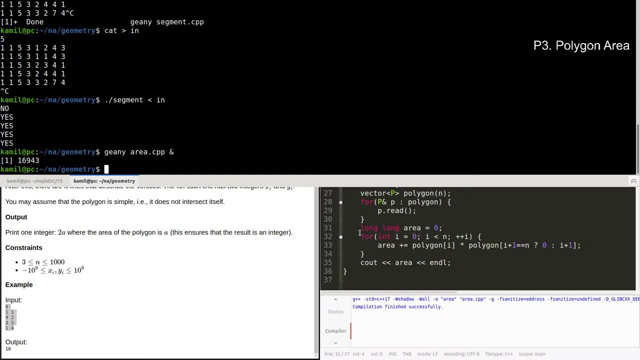 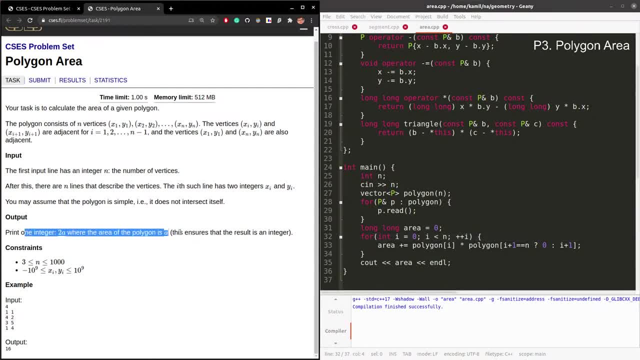 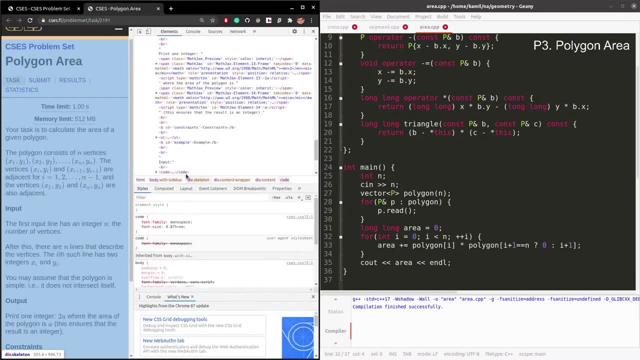 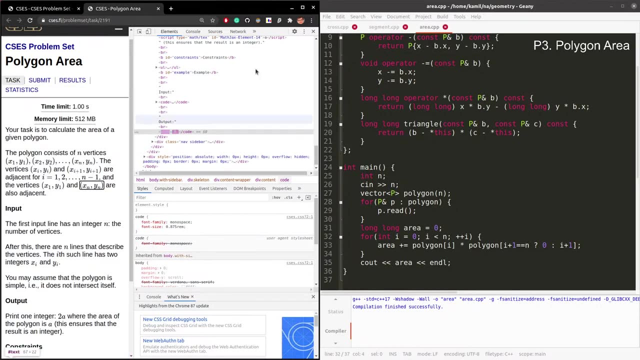 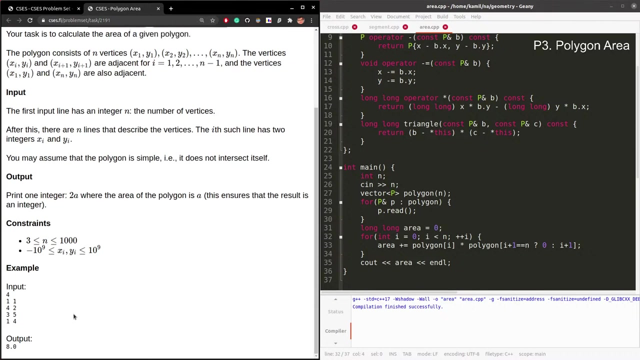 oh, ok, ok, ok, sorry. they tell us to print twice the area. so let's imagine it like that. if they really asked us about area, the code would be like that: this is a valid problem if it says compute area of polygon. area of this polygon is 8. 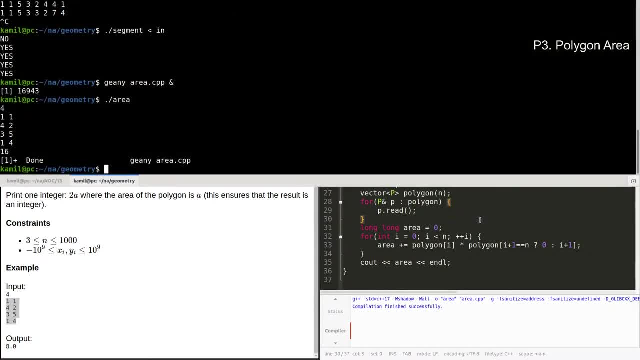 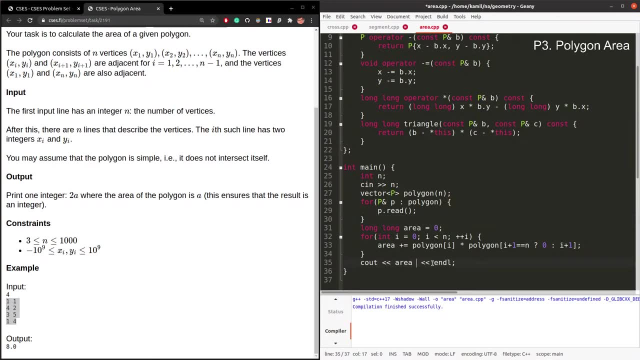 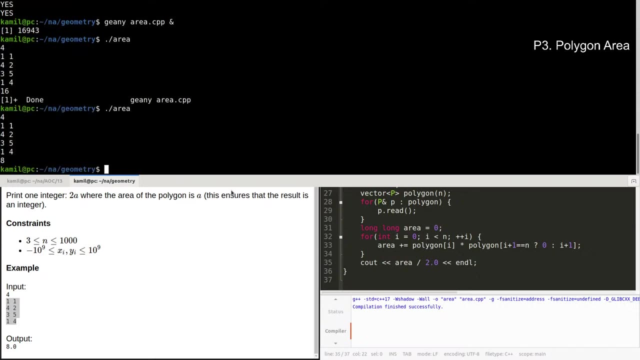 8.0, let's say. then I- not rightly- I got 16. and now to really print the area, I should divide by 2. and now my program prints the area. and now my program prints the area. and now my program prints the area. 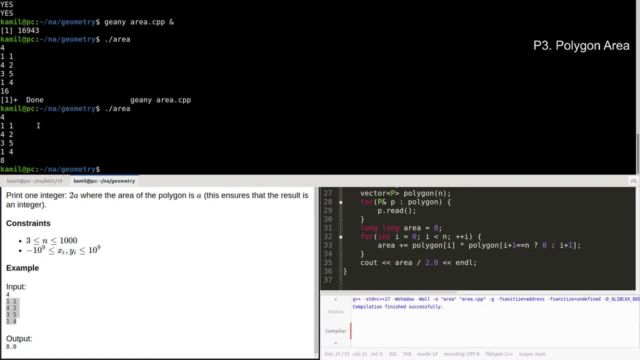 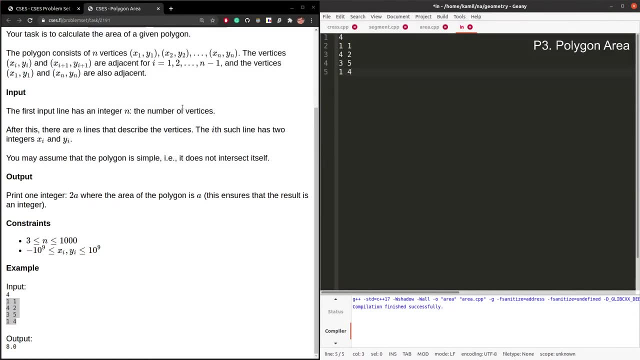 it's 8 there. actually there were two case, two possibilities for what my program will print and for that let me create this, take this input and now reverse it, so it will be 1, 4, 3, 5, 4, 2. 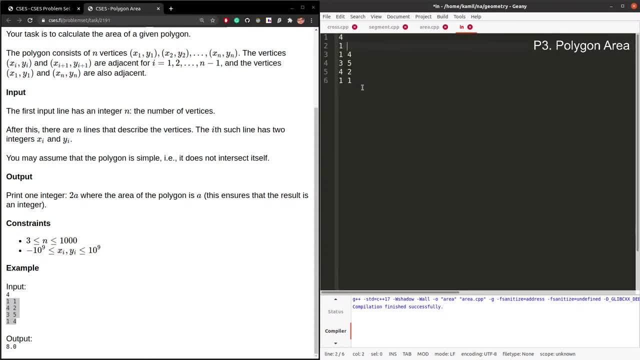 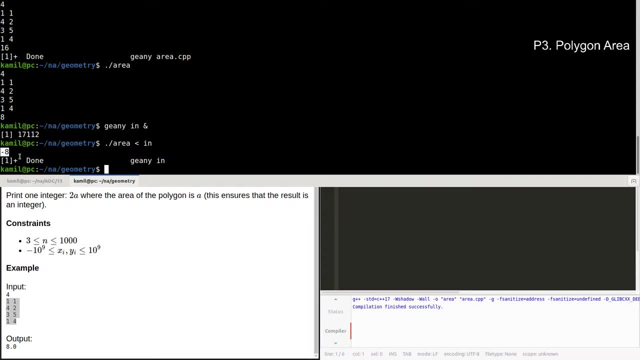 and 1, 1. providing points in different order will actually give me the other solution will actually give me the other solution. the value I computed was 16. the value I computed was 16, and divided by 2, it's minus 8, and divided by 2, it's minus 8. 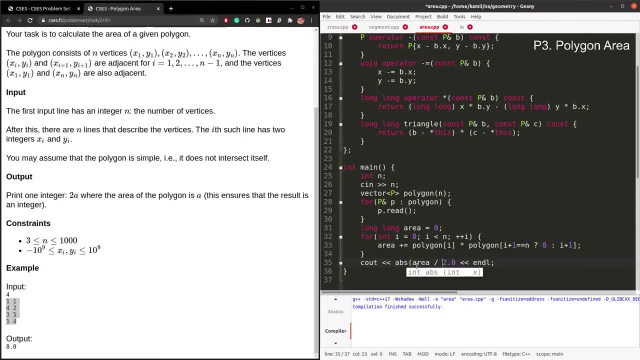 so I need, if I want to print area. it's this: you can take absolute value after dividing by 2, or absolute value of area divided then by 2 is fine as well, but they say: print twice the area, because this ensures that the result is integer. 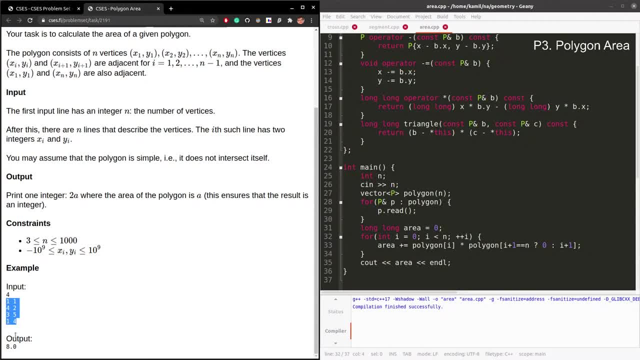 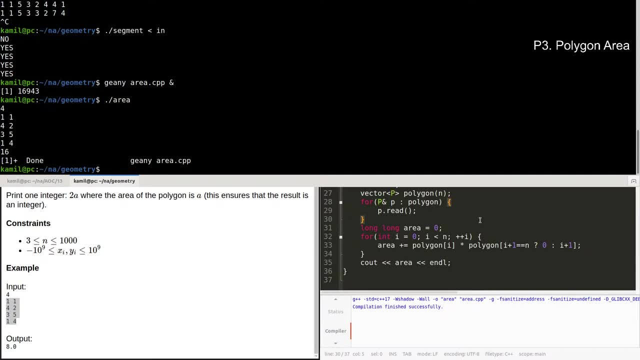 If it says compute area of polygon. Area of this polygon is 8.. 8.0. let's say, Then I- Not rightly, I got 16.. And now to really print the area I should divide by 2.. And now my program. 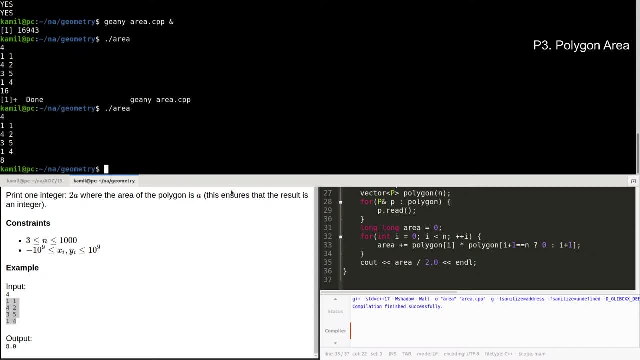 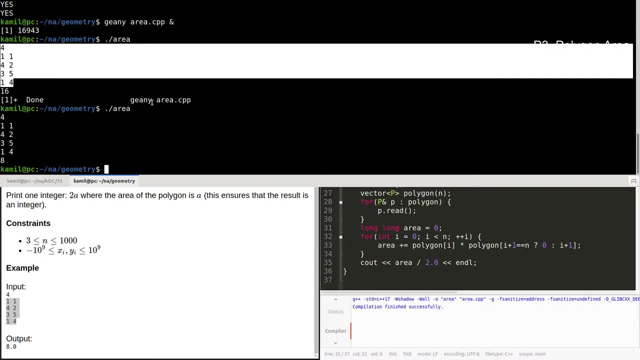 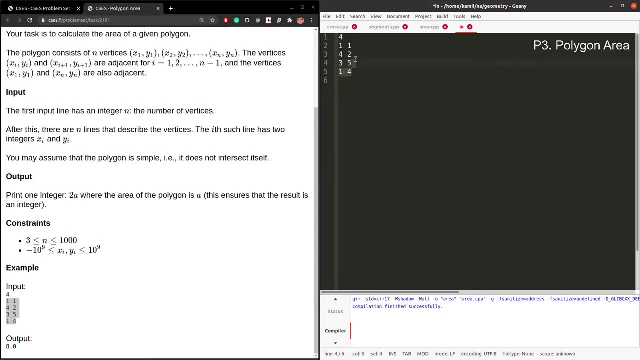 Prints the area. It's 8.. There actually There were two case, Two possibilities for what my program will print, And for that Let me Take this input And now reverse it, So it will be 143542.. 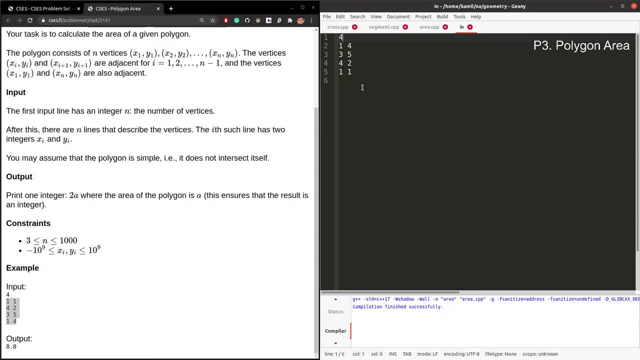 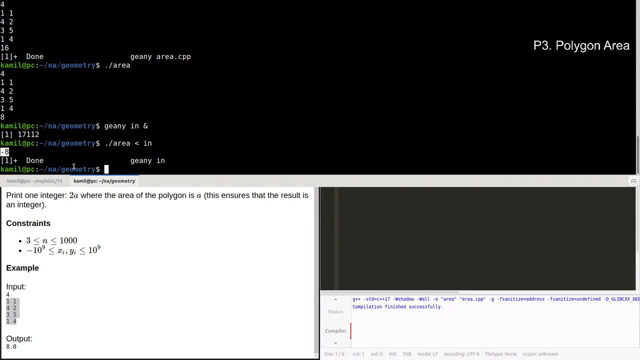 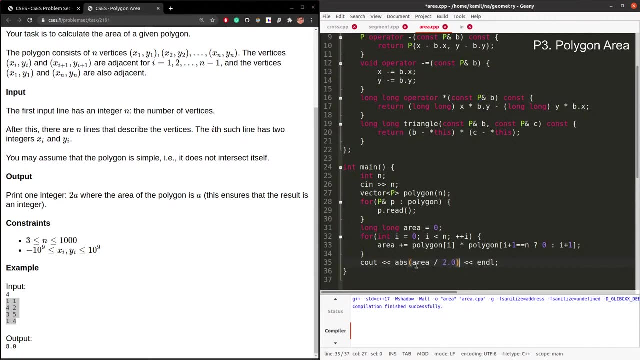 And 11.. Providing points in different order Will actually give me The other solution. The value I computed was 16. And divided by 2 it's minus 8.. So I need, If I want to print area, It's this: 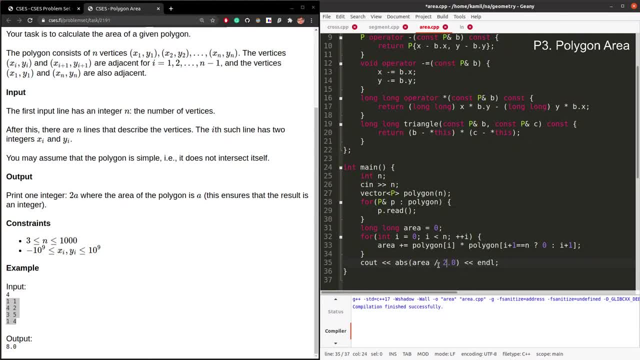 You can take absolute value after dividing by 2.. Or Absolute value of area Divided then by 2 is fine as well, But they say Print twice the area, Because this ensures that the result is integer. Author of the problem. 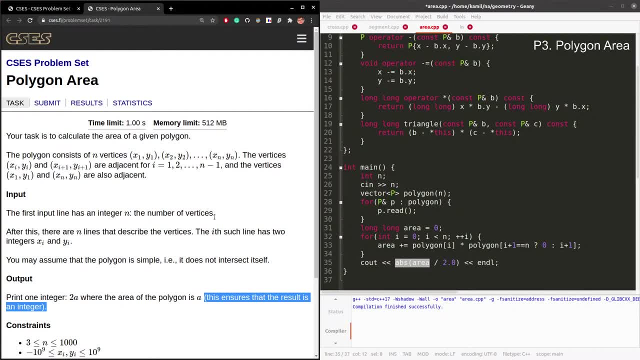 Knows that we use cross product And we can use just integers for this problem, So We can do this Twice the area. This helps us avoid To deal with real values. Alright, I told you. This is Much faster. 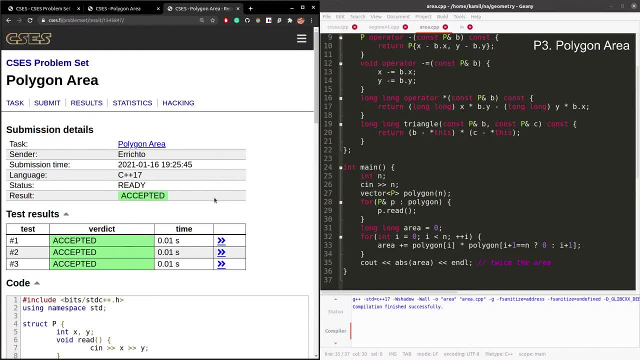 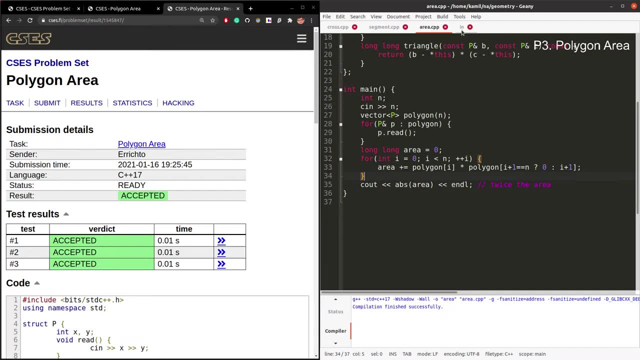 Shorter than My explanations. Why not just divide by 2. By 2.0. Because I want real values. I will show you a case Where dividing by 2 doesn't work. Let's say that I need to. 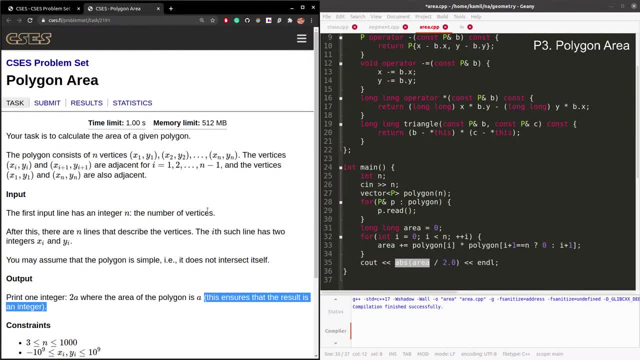 author of the problem knows that we use cross product and we can use just integers for this problem, so we can do this twice the area. this helps us avoid to deal with real values. this helps us avoid to deal with real values. alright, submit, I told you this is. 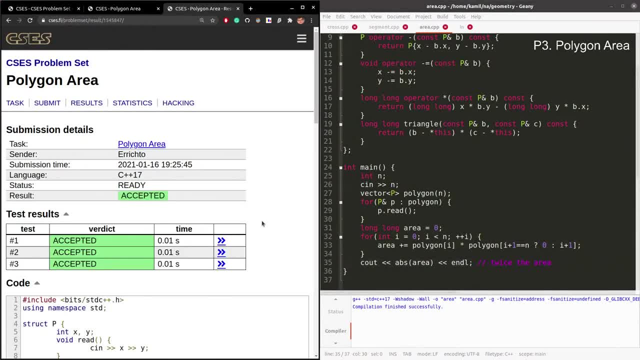 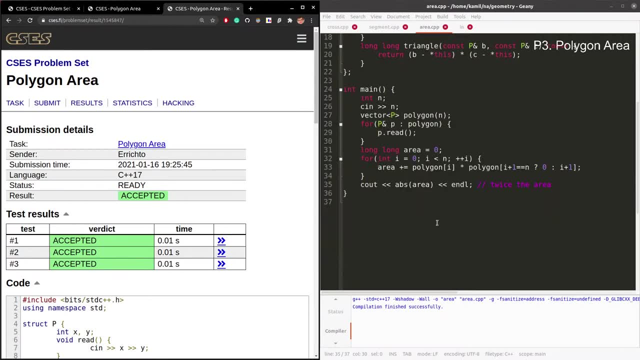 this is much, much faster, shorter than my explanations. why not just divide by 2 by 2.0? why not just divide by 2 by 2.0? because I want real values. I will show you a case where dividing by 2 doesn't work. 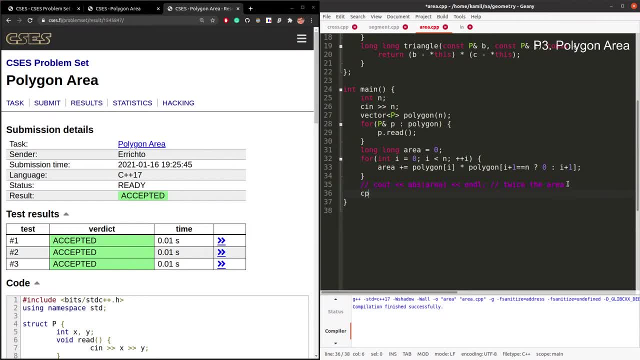 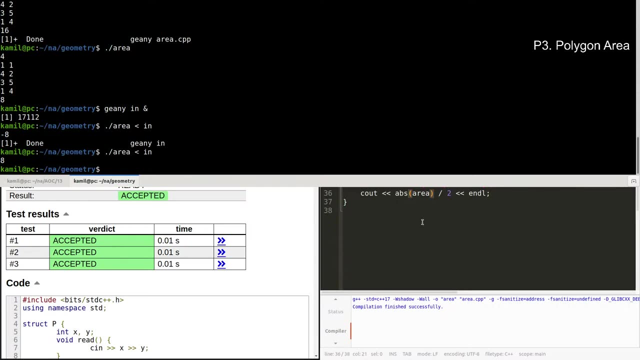 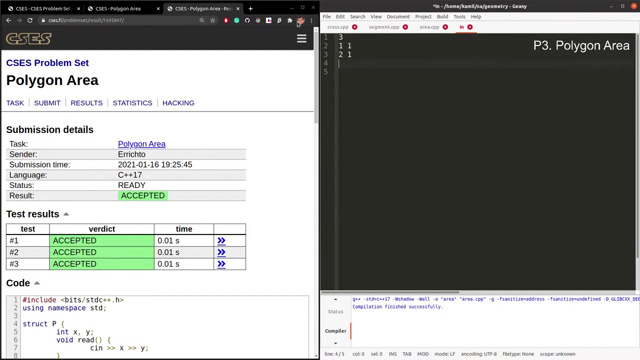 let's say that I need to print area. let's say that I need to print area. this is wrong. this is wrong. it will work here. 8 is correct area of polygon in the input. but let me modify this to a simple test of 1,1 to 1,1,2. this is a triangle. 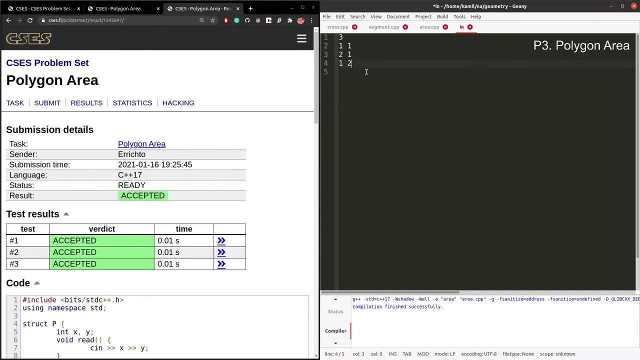 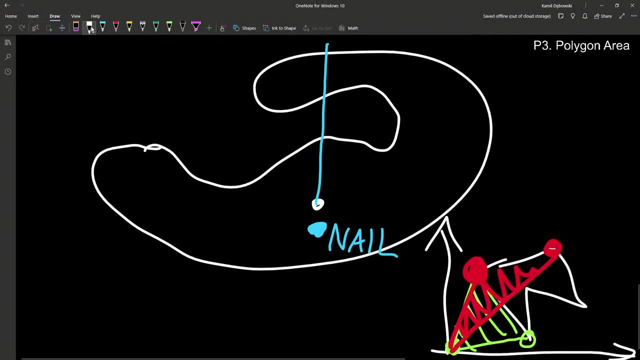 with 2 sides of length equal to 1. with 2 sides of length equal to 1. now my program printed 0. now my program printed 0. why? because we have something like this, because we have something like this. I created this test 1 by 1. 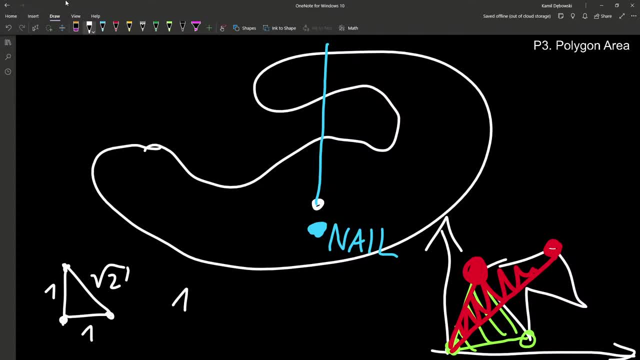 this is square root of 2, if you need it. but area of this is half. but area of this is half. when my program computed twice the area, it got 1. this is product of this vector- and this vector then divided by 2 using integers. division in C++. 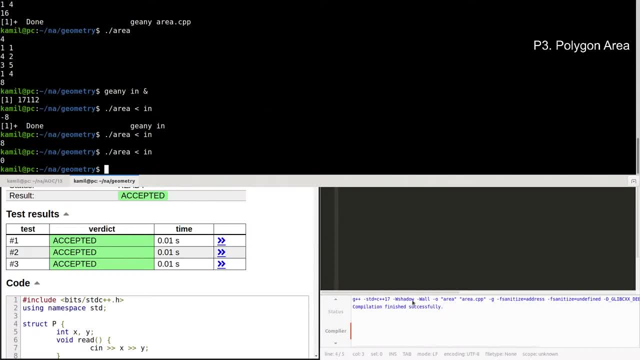 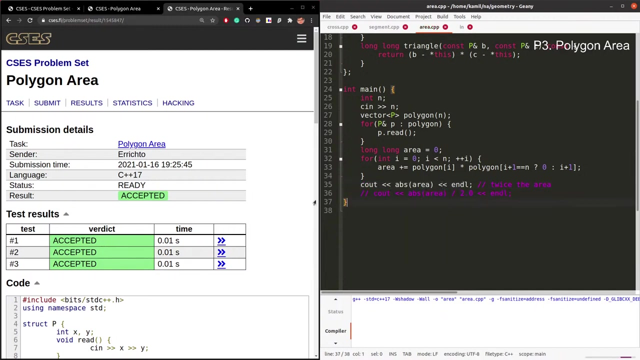 rounds towards 0 down, I got 0. instead. I should say this, and now it will be correct: area 0.5. area doesn't need to be integer, even if coordinates of points are integers. it can be integer 0.5, not 2. so 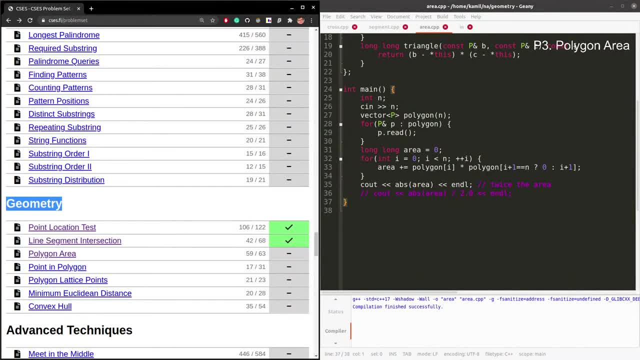 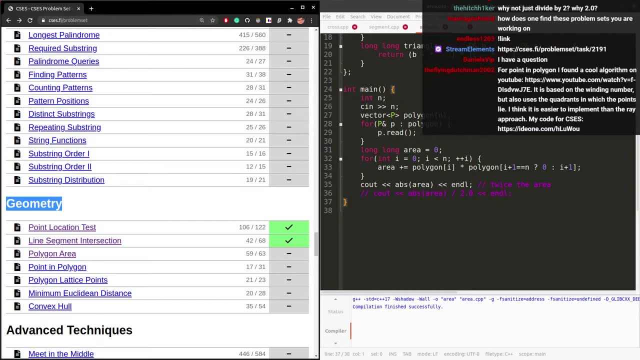 good, you move on. I have a question then ask it For point in polygon found a cool algorithm on youtube based on the Winding Number. eh are a lot of cool stuff in geometry and I don't have time to talk about everything. I believe you that there are other like alternative interesting stuff. 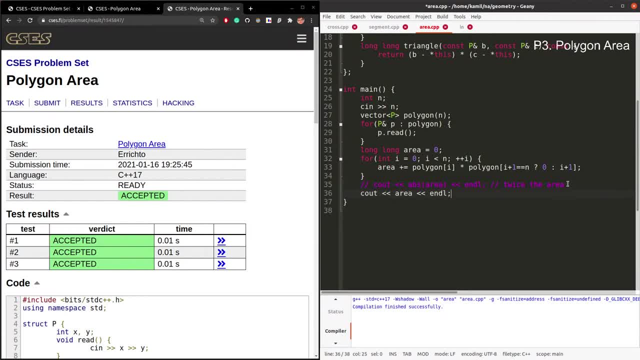 Print area. So This is wrong. It will work here. 8 is correct area Of polygon in the input. But let me modify this To a simple test of 1,1 to 1,1,2.. This is a triangle. 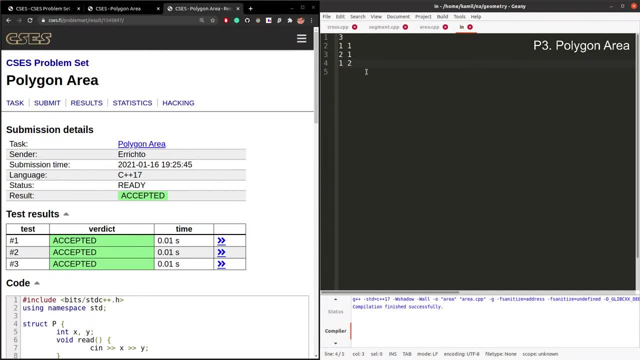 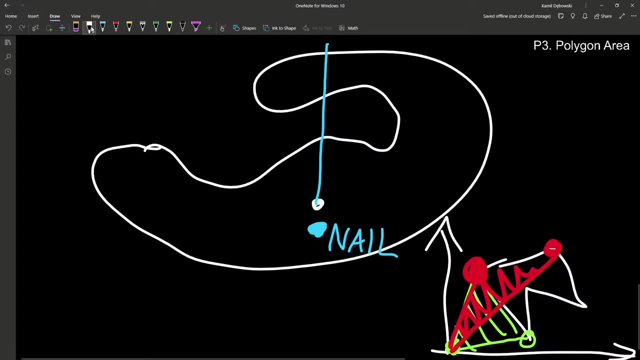 With 2 sides of length Equal to 1.. Now My program printed 0.. Why? Because we have something like this. I created this. Let's test 1 by 1.. This is square root of 2.. 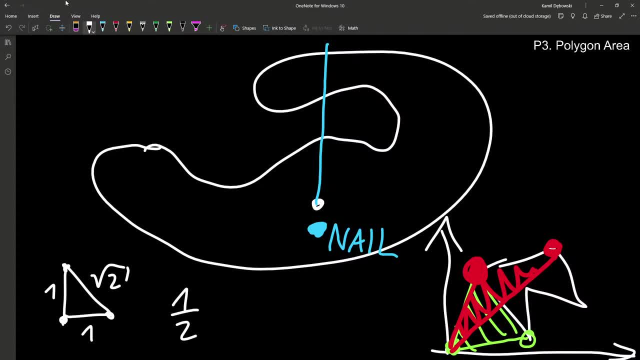 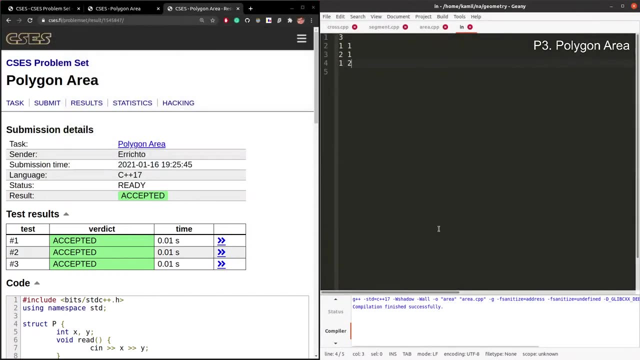 If you need it, But area of this Is half. When my program computed Twice, the area It got 1.. 1 is indeed cross product Of this vector And this vector Then divided by 2. Using integers. 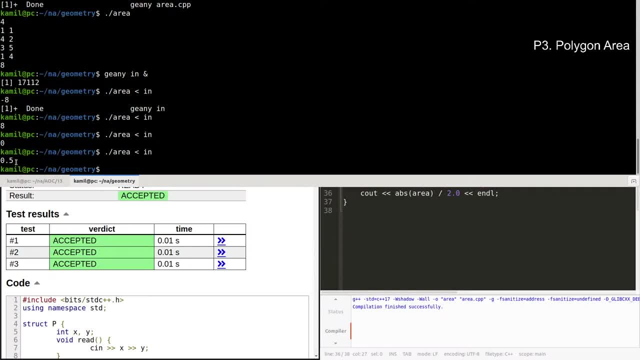 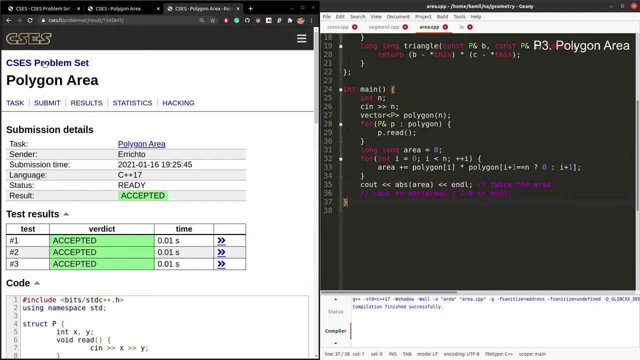 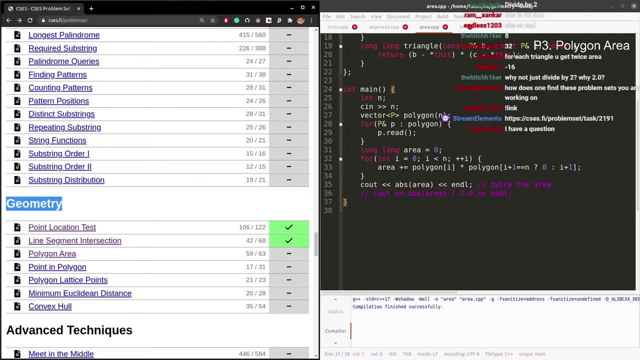 And now it will be correct: Area 0.5.. Area doesn't need to be integer, Even if coordinates of points are integers. It can be integer 0.5.. We move on. I have a question Then ask it. 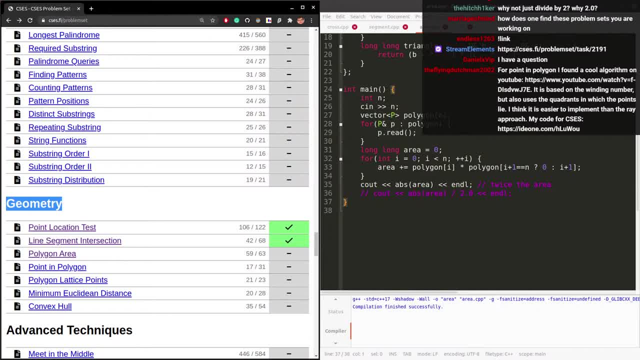 For point in polygon, Found a cool algorithm On YouTube Based on the winding number. There are a lot of cool stuff In geometry. I don't have time To talk about everything. I believe you that There are other Alternative. 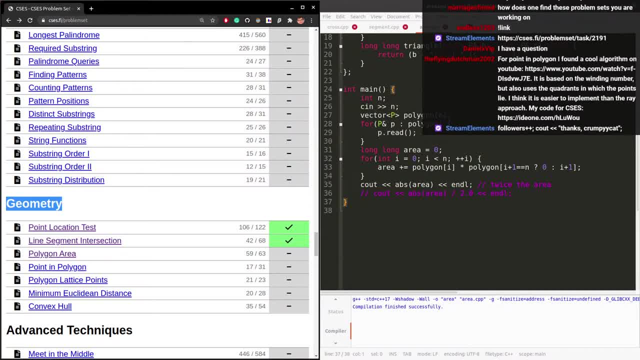 Interesting stuff, So Let's see Back winding number. I will not check it now, But You are all free to later See other solutions. How does one find these problems That you are working on? This is CSES website. 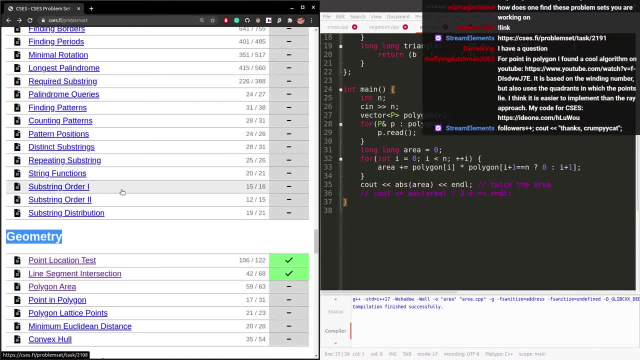 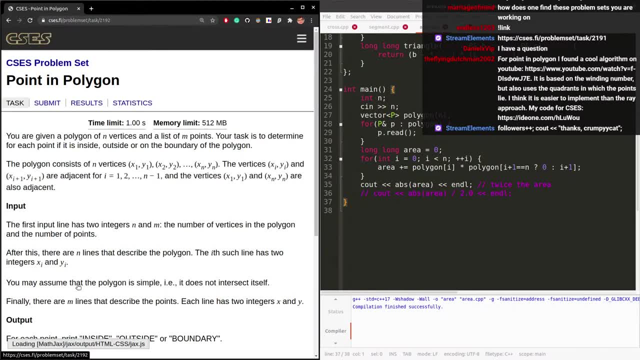 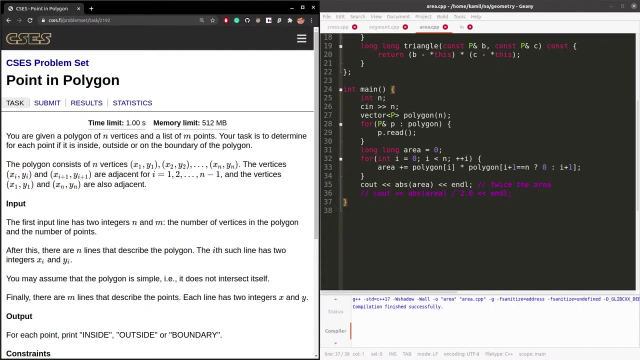 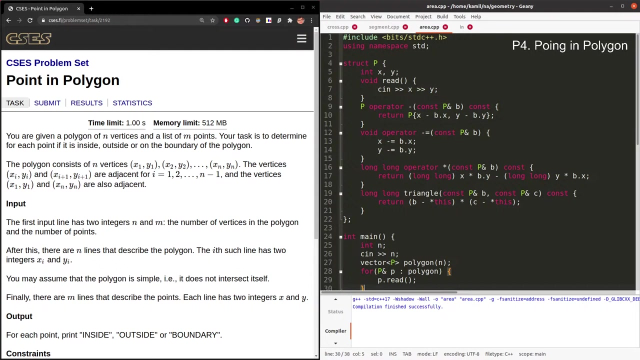 It's website with a lot of Categories and basic problems. Point in polygon. We already know How to deal with This is: This is P4. Point, Not point Point. You are given a polygon Of n vertices. 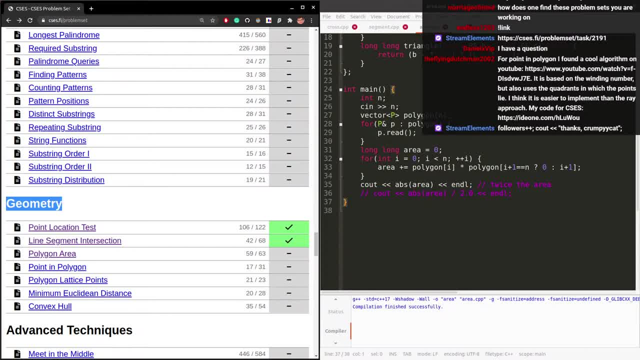 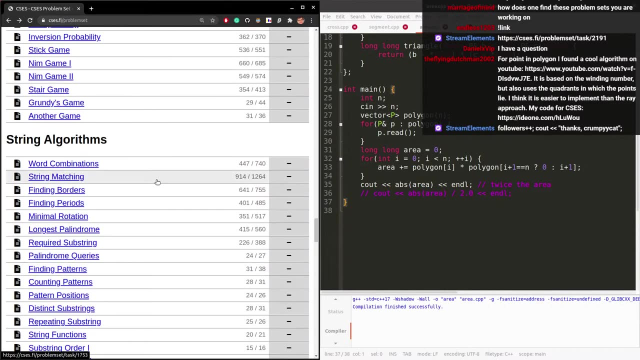 like winding number. I will not check it out now, but you are all free to later see other solutions. How does one find these problems that you are working on? This is CSES website. It's a website with a lot of categories and basic. 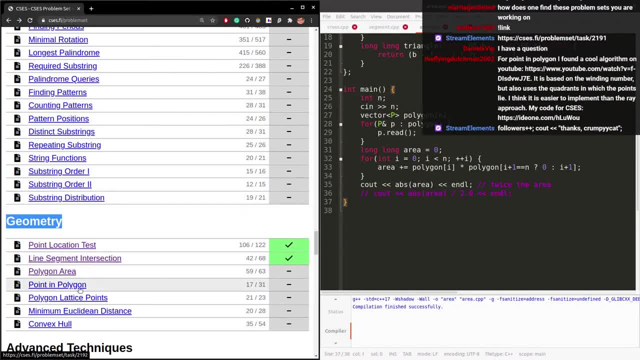 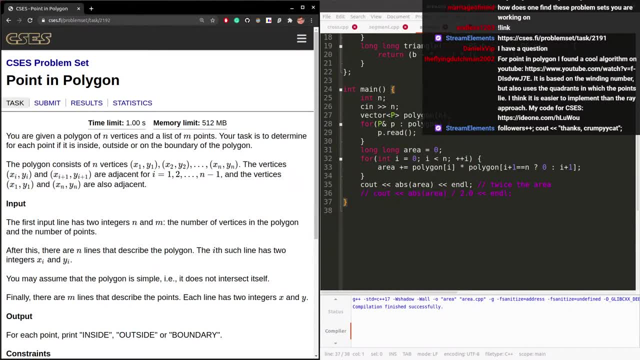 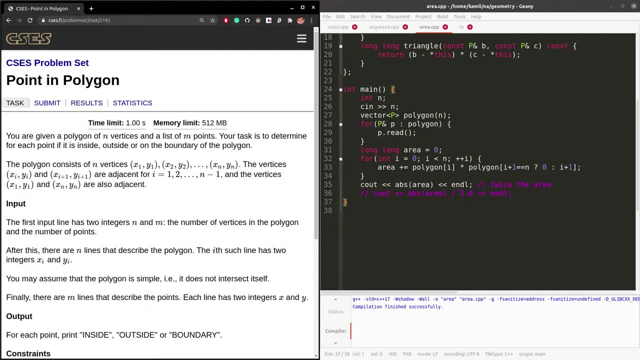 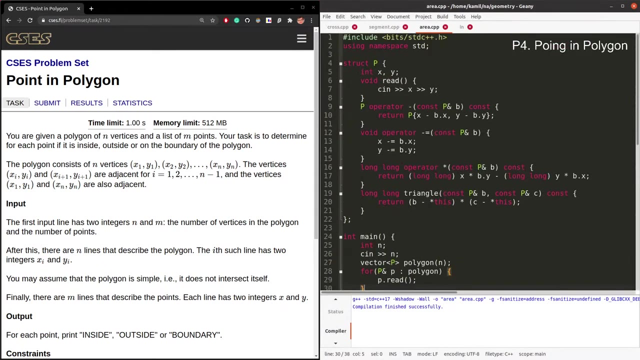 problems Point in polygon. we already know how to deal with This is P4 point. You are given a polygon of n vertices and a list of n points. Your task is to determine for each point if it is inside, outside or on the boundary of polygon. 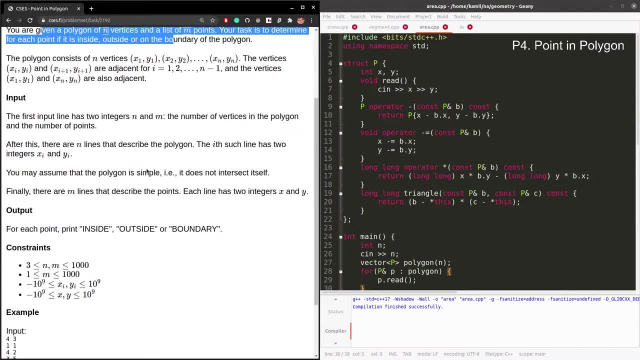 Constraints are low enough that we can process every point in linear time. We will try to get all of them in linear time, Each of n times m. Each of points we separately check and we will do it. complexity linear of n per point. It is possible to solve this problem faster. 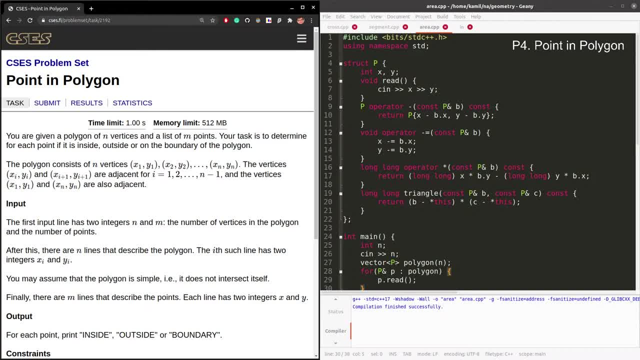 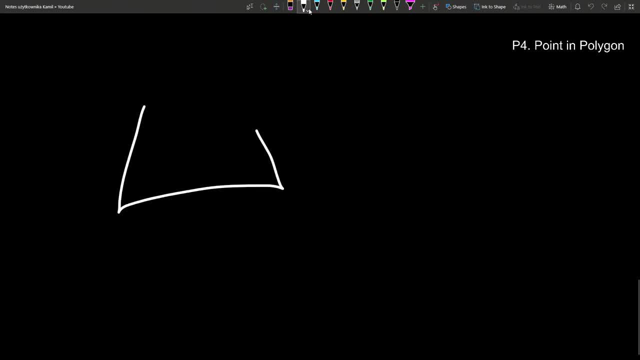 but it's beyond this stream. What is the plan? You have some polygon, not necessarily convex- How to check if point P is inside or not. You have some polygon- not necessarily convex- How to check if point P is inside or not. 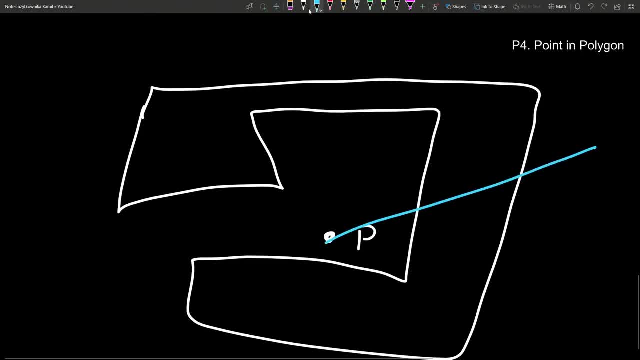 How to check if point P is inside or not. We need to draw some ray and compute intersections. It's tricky to deal with cases where some segment is exactly on this line. I need to choose such a ray, This ray. It shouldn't be collinear with any segment. The best. 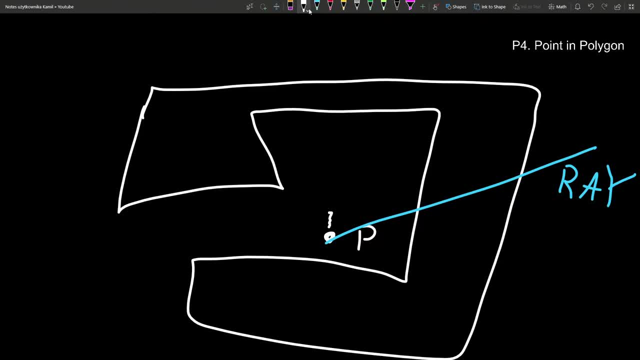 way for that is to choose something directly above point P. Now if I take 3 and 0.. If r also equal issues. So a cube having a two point P is leave as a permanent distant sector. This is once again an infinite device. 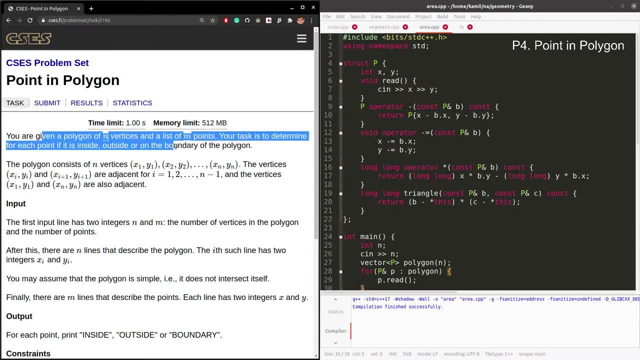 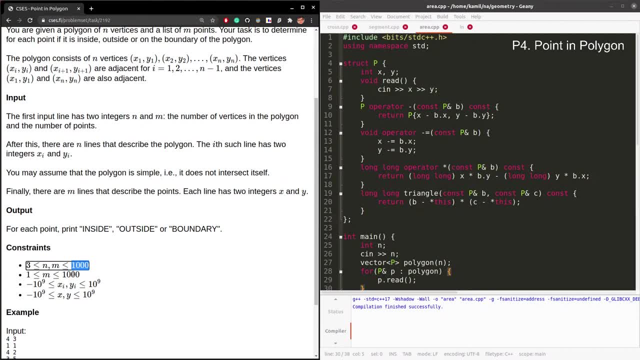 For each point If it is inside, Outside Or on the Boundary of polygon. Constraints are low enough That we can Process every point In linear time. We will try to get O Each of points We separately check. 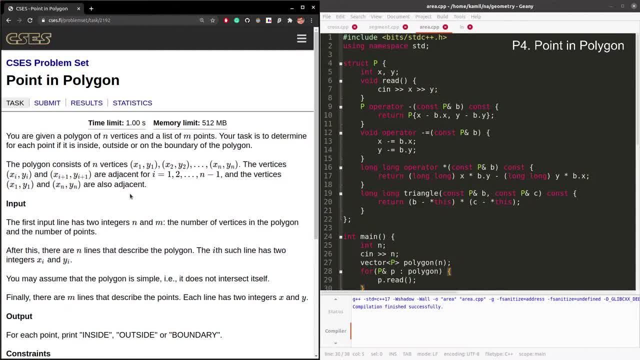 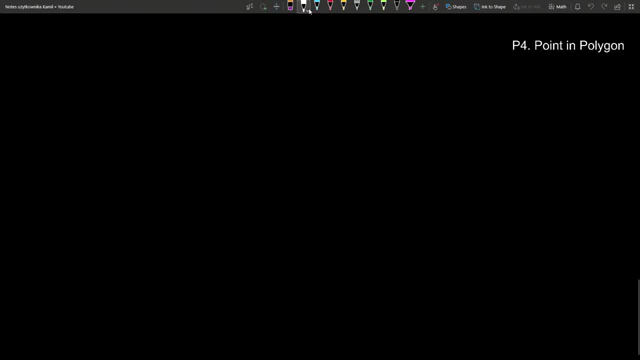 And we will do it. Complexity For each Point. What is the plan? We have some polygon, Not necessarily convex- How to check If point P is inside Or not? We need to draw some ray And compute intersections. 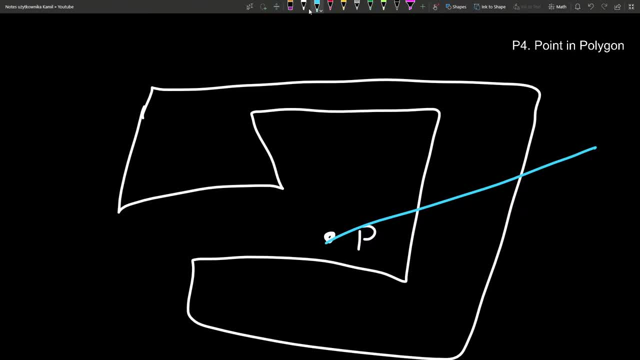 I. It's tricky to deal with cases Where P is This line. I need to choose such a ray, This ray. It shouldn't be collinear With any segment. The best way for that Is to choose point. 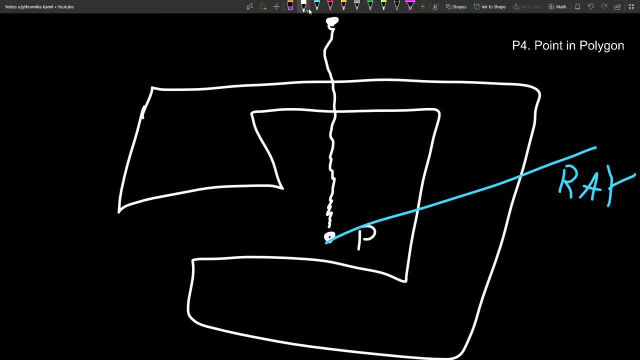 Something directly above point P In infinity. But this would be, This would be collinear With every vertical segment Here as well. Then shift it By one to the right. Then, here I take 4 comma, infinity, And this ray. 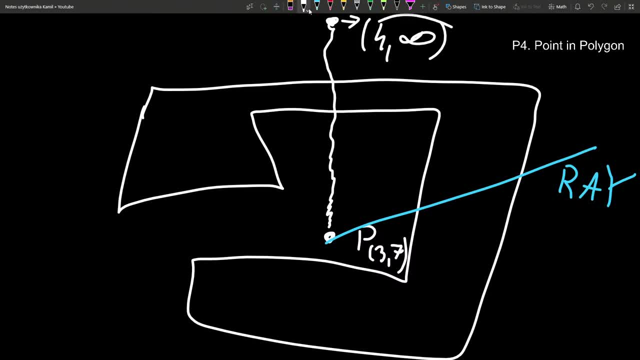 For this ray. I just take a segment from P To this point, very far away, And I say that this is a ray. This infinity should be big enough That it is outside of the polygon. Then Problem boils down to Checking intersections. 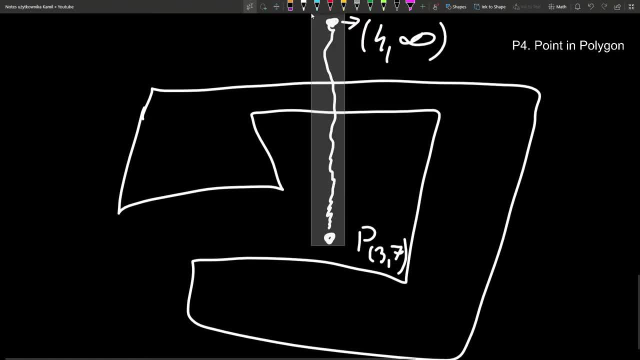 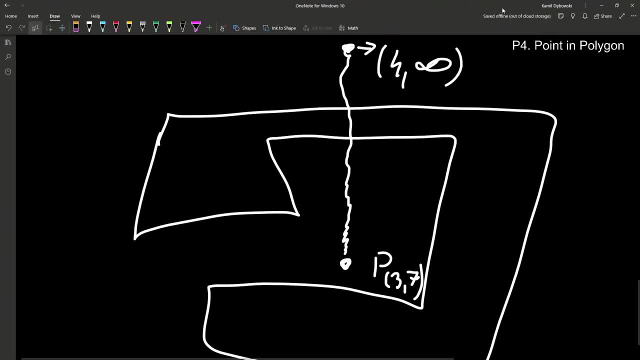 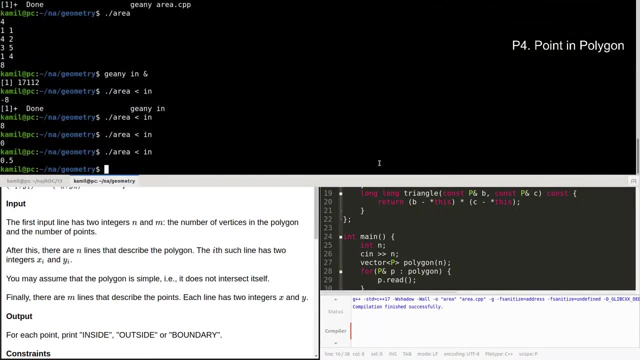 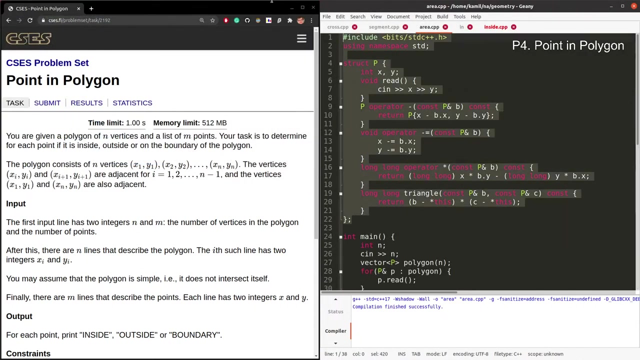 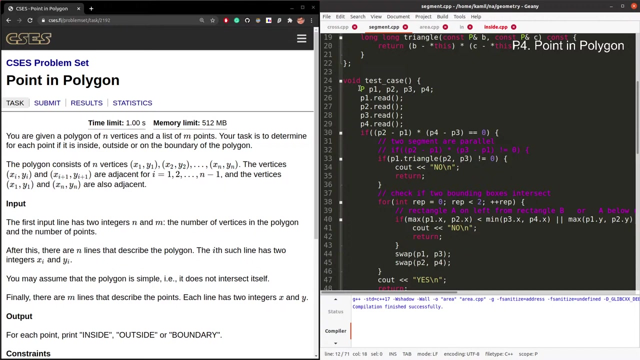 Of segments of a polygon, With my segment From P To the outside, And we already have a code for that. Coordinates are up to billion Right Inside. I'm copy pasting The template we already have And This thing: 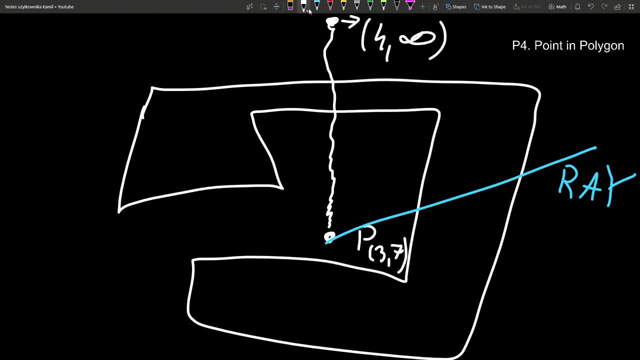 I can use this coordinate Y To solve this So I can have that four comma infinity. I use it here, Kol interior, with every vertical segment here as well. then shift it, but one to the right. If point P is 3, 7, Then I take 4, infinity to third mass For this ray. just take a segment from P to very far away, this point. 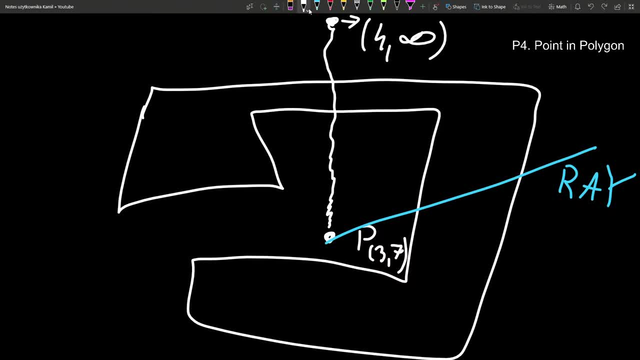 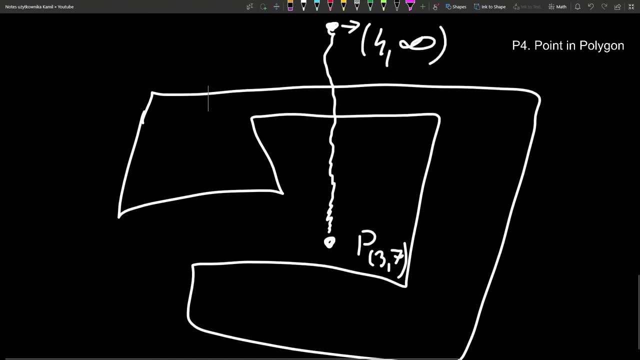 and I say this is a ray. This infinity should be equal my image measure, big enough that it is outside of the polygon. then problem boils down to checking intersections of segments of a polygon, with my segment from p to this thing outside, and we already have a code for that. 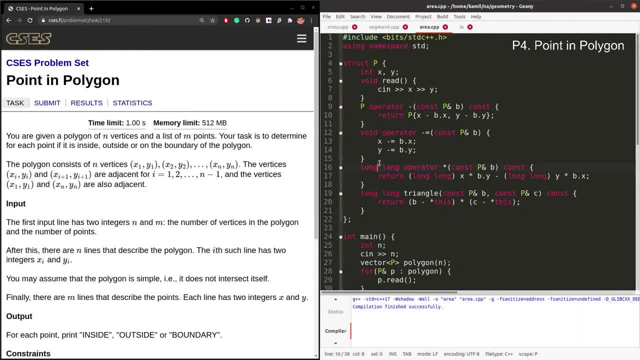 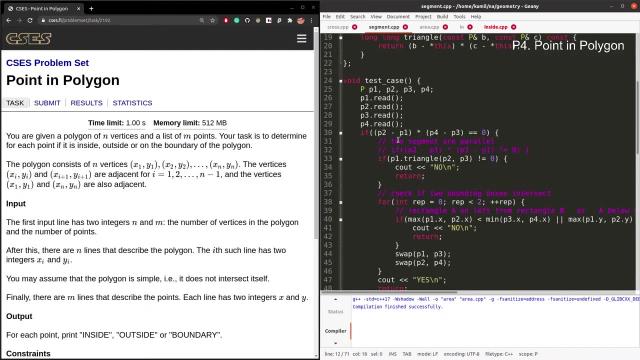 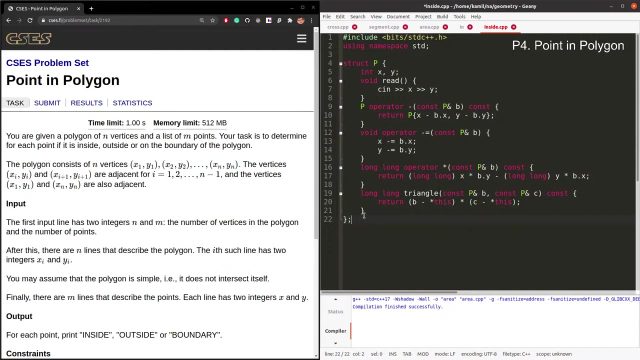 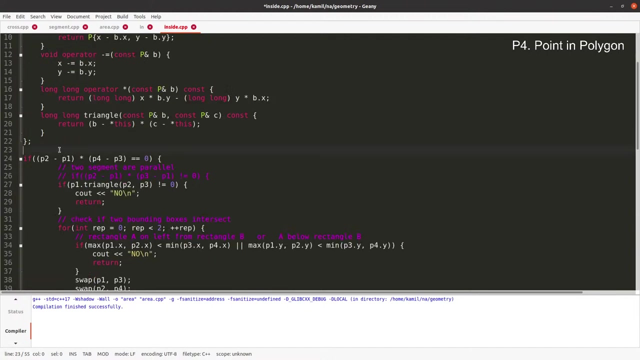 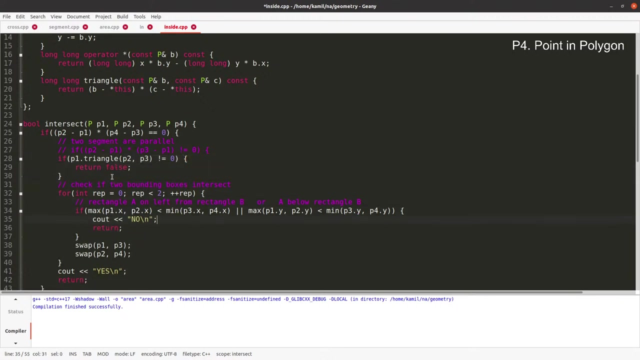 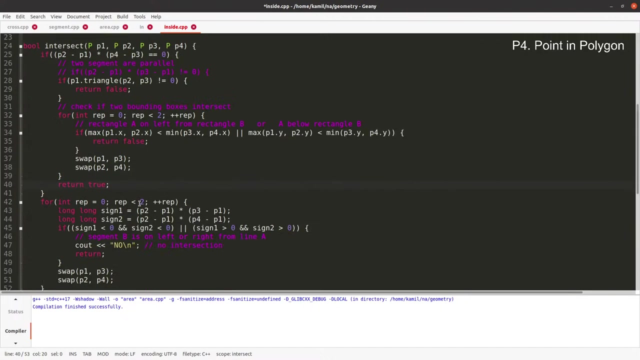 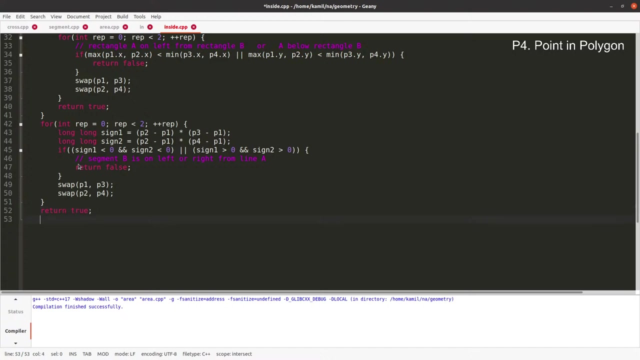 coordinates are up to billion right inside. i'm copy pasting the template we already have and this thing, this should should have been a function returning true or false. i copy pasted code for intersection of two segments: return false, return false. a true, false and true. let me know if you're seeing that i'm making some obviously stupid typo, you know. 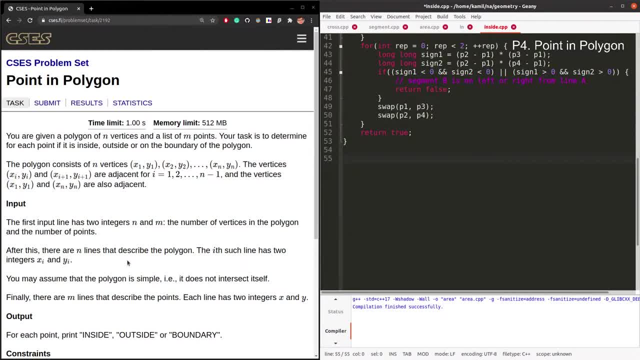 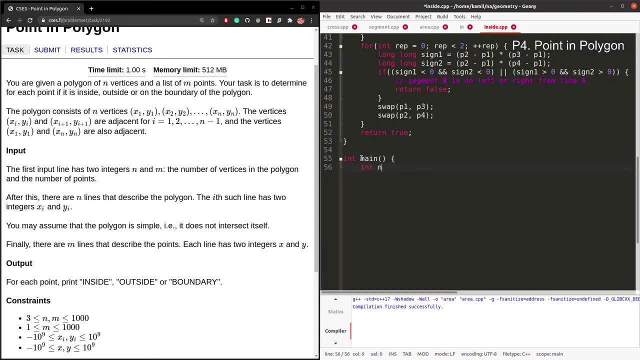 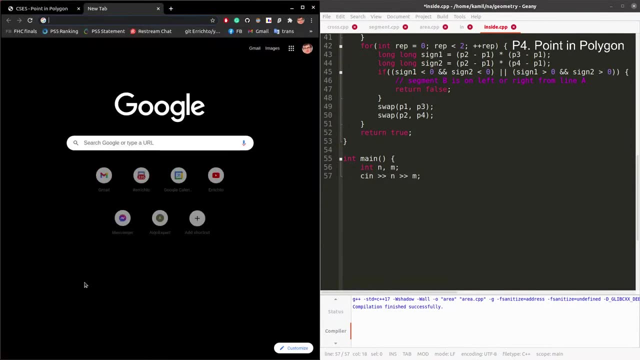 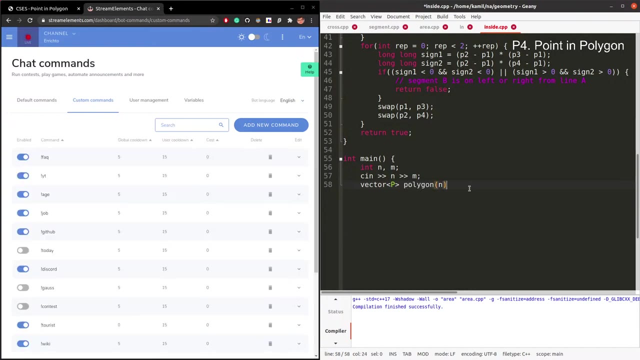 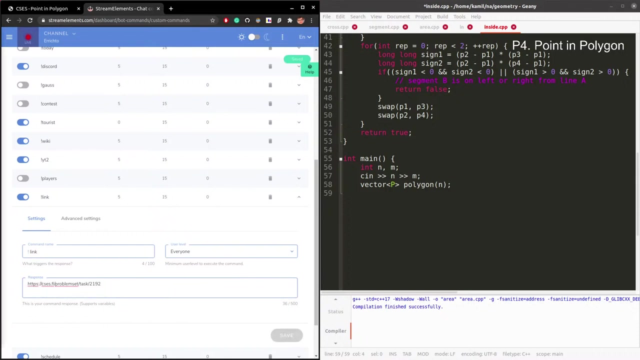 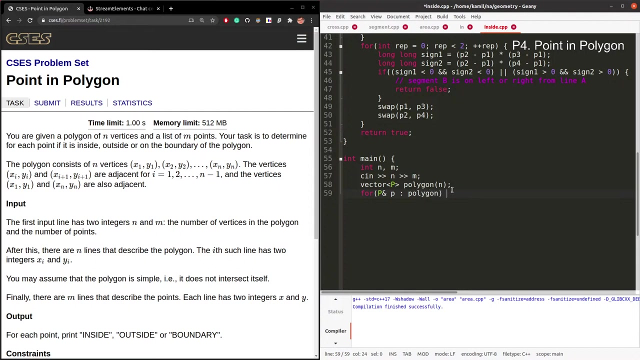 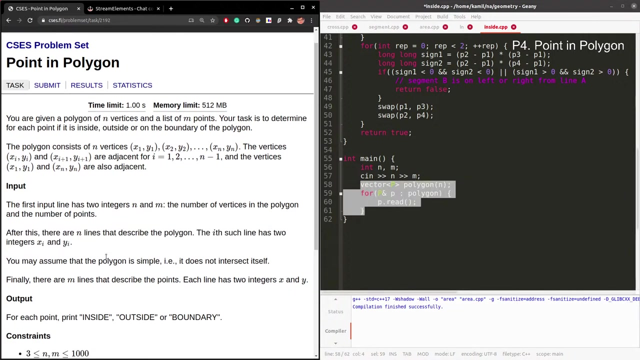 anything like that right now. point in polygon. so let's open it up. read the number of points in the polygon. at the number of points, a number of query points. i need to update the link if you want to open the problem. here is the link. I'm done reading the polygon. 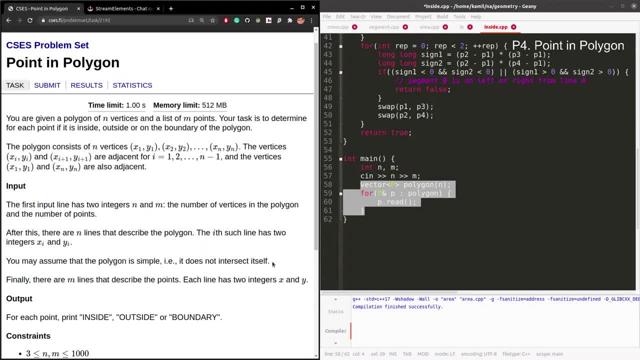 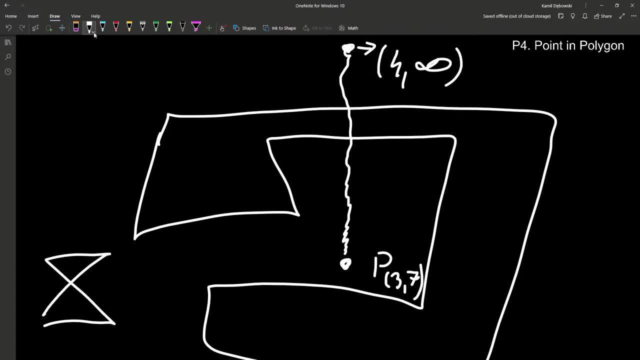 You may assume that the polygon is simple, that is, it does not intersect itself. We don't want such shapes because then this is not a good, not a valid polygon, because then it's a bit harder to say what is inside and what is not. 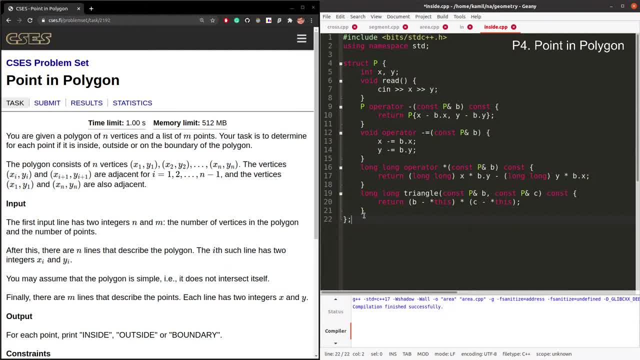 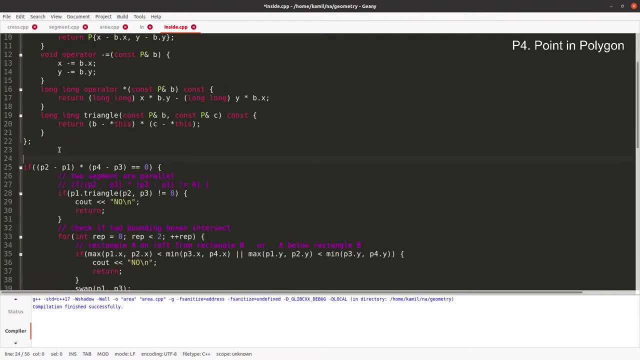 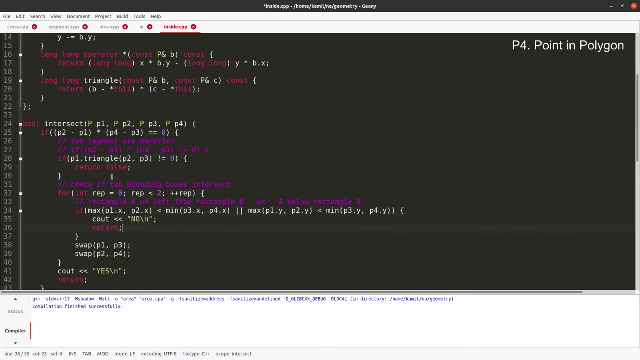 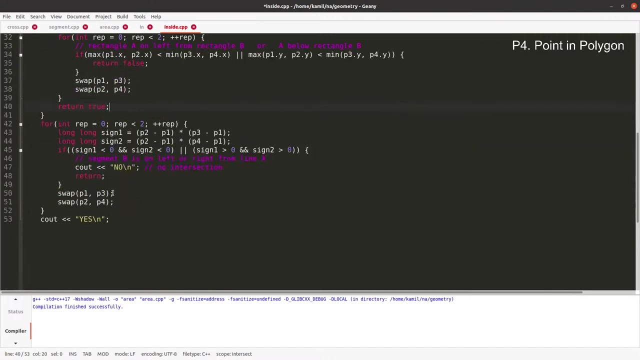 This should have been a function For returning true or false. I copy pasted Code for Intersection of two segments: Return- false. Return false, True, False and true. Let me know if you are seeing That I'm making some. 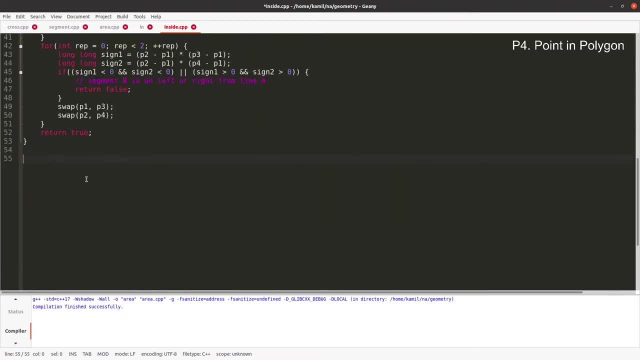 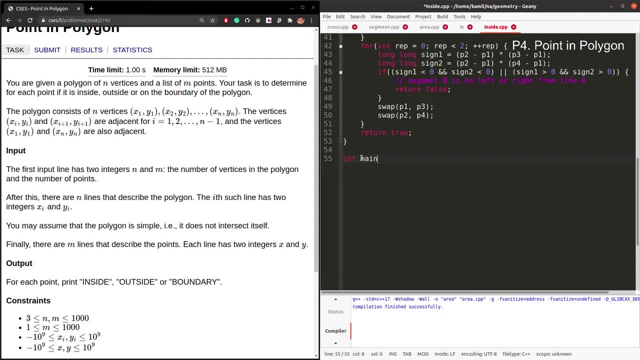 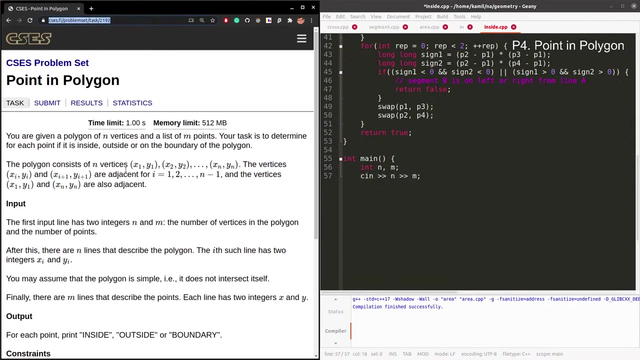 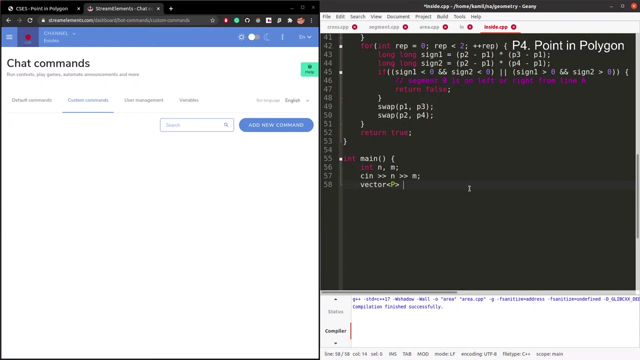 Obviously stupid typo Or anything like that. Right Point in polygon: Read the number of points In a polygon And the number of points And number of query points. I need to update the link. I need to update the link. 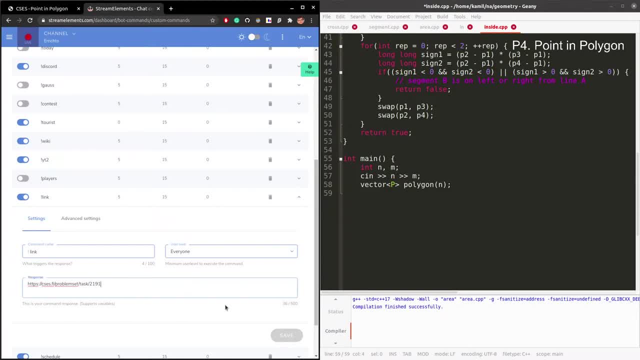 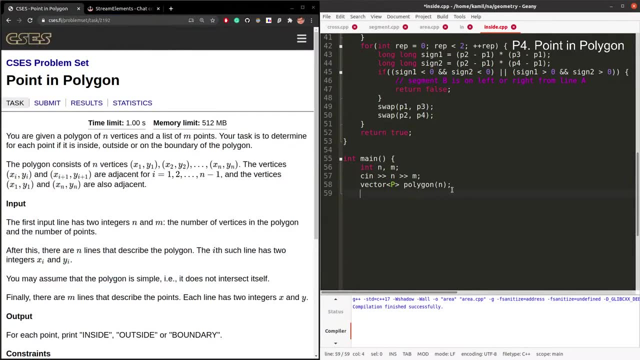 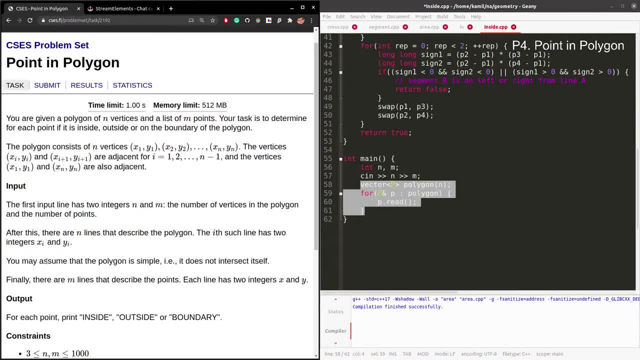 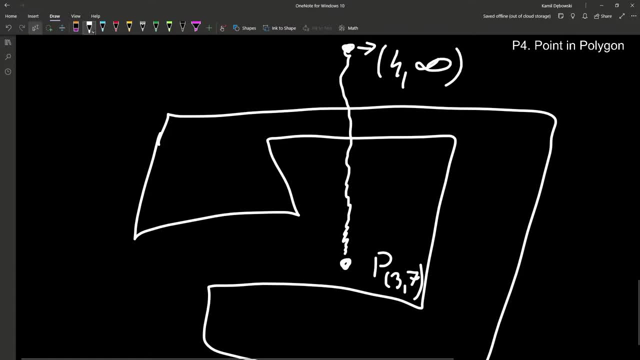 Done. reading the polygon, You may assume that The polygon is simple, That is, it does not intersect itself. We don't want Such shapes Because then This is not a valid polygon, Because then it's a bit harder To say what is inside and what is not. 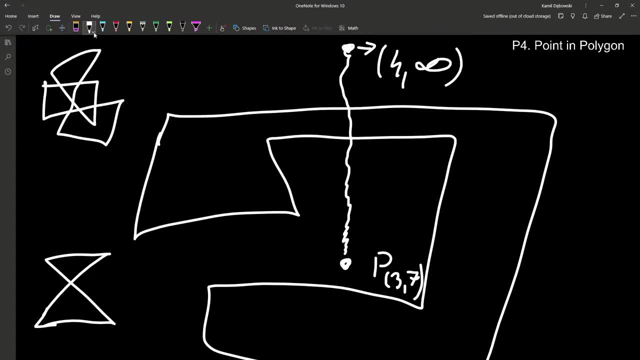 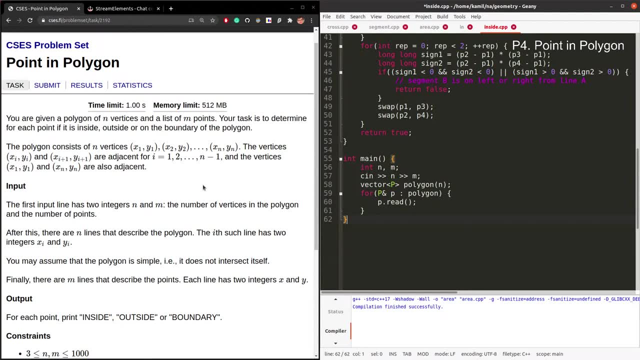 If I draw this, Then are we able To say what is inside. Still, The only valid definitions is this one With even number of intersections of array. Now, for every, Let's say, Repeat m times, I have point P. 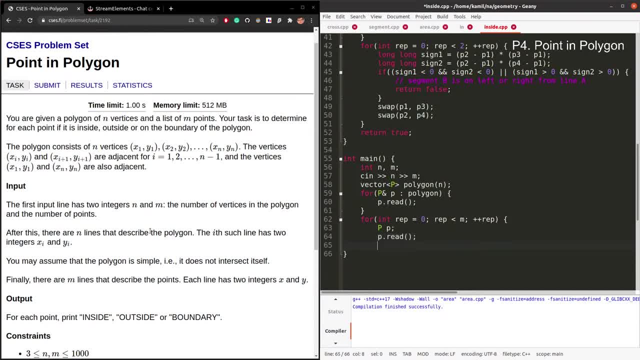 And I will Investigate what happens with point P. This point outside, As I said, is P dot x plus one Comma infinity. And now This infinity is slightly too small. It's not easy to understand why, But 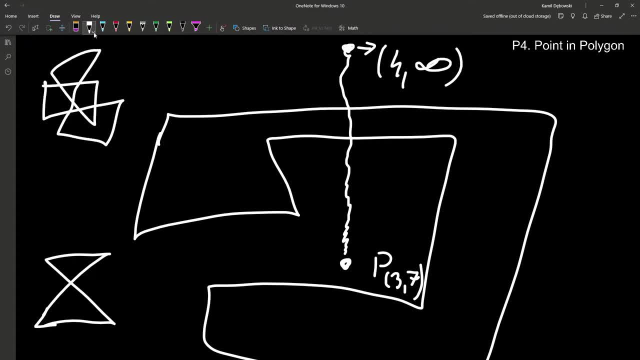 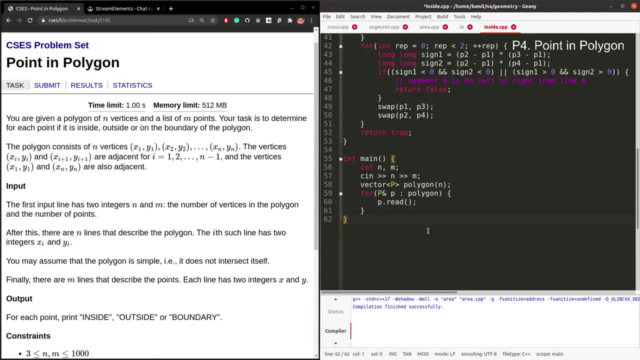 If I draw this, then are we able to say what is inside. Still, the only valid definitions is this one with even number of intersections of array. Now, for every, let's say repeat m times. I have point P and I will investigate what. 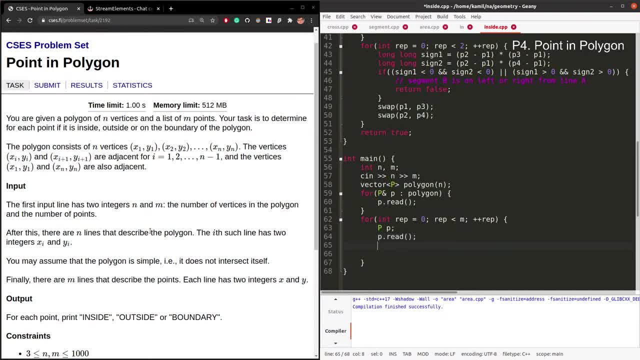 happens with point P. This point outside, as I said, is P dot x plus one comma infinity. And now this infinity is slightly too small. It's not easy to understand why, but I believe that we need here three billion. This actually not slightly too small. 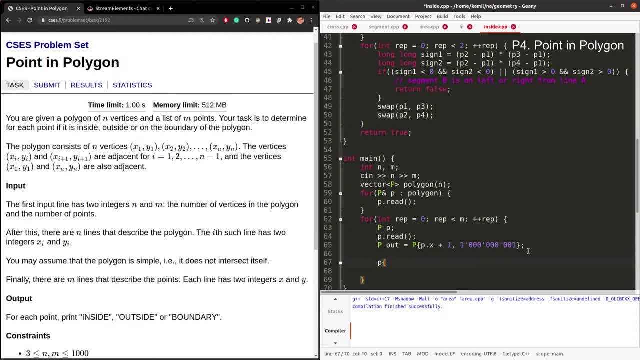 Imagine that P is something with coordinates. let's say this comma, the same For this point. if you're taking this one, it's just very close, It's actually nearby, It is far away. We cannot now say that line from P to this point outside is a vertical line, just slightly. 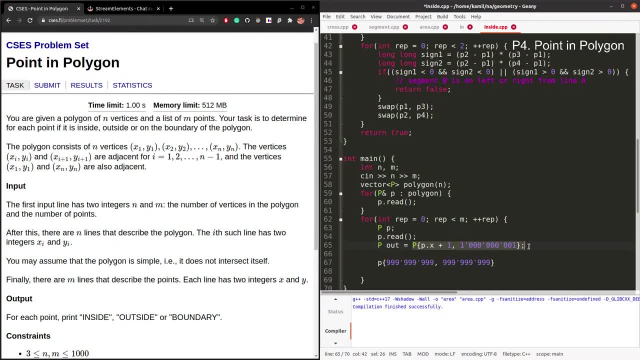 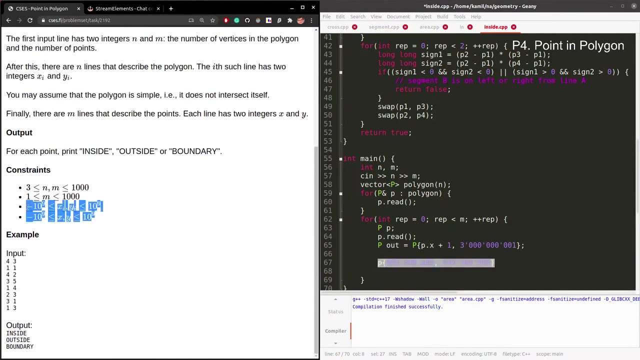 tilted to avoid it. It avoids it being vertical and being collinear with anything else, So it would be really like a vertical line. I believe we need this. Then the distance from this point outside to myself is at least two billion, And it is greater than this stuff here like significantly greater. 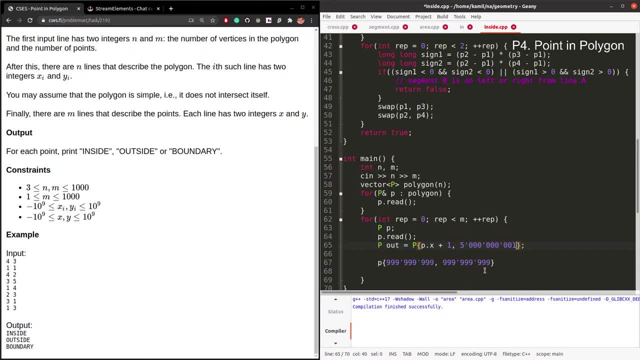 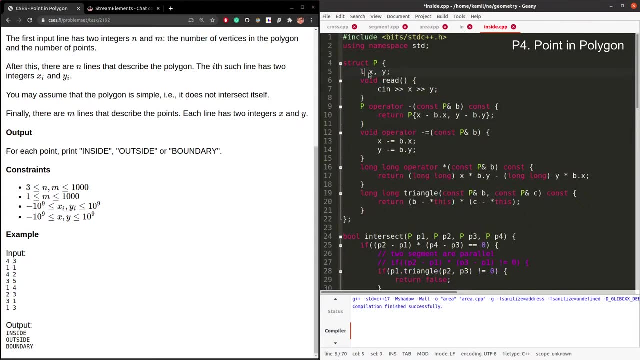 I would even be safer with doing this, but then I'm using long, longs. apparently, Five million square Will it fit in long long. Let's say this: I'm afraid about now, cross products overflowing long long. No, we need this. 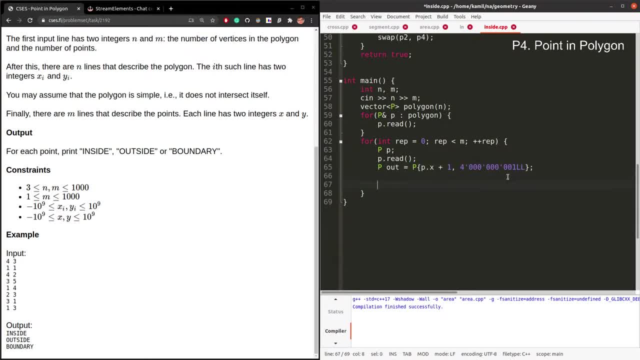 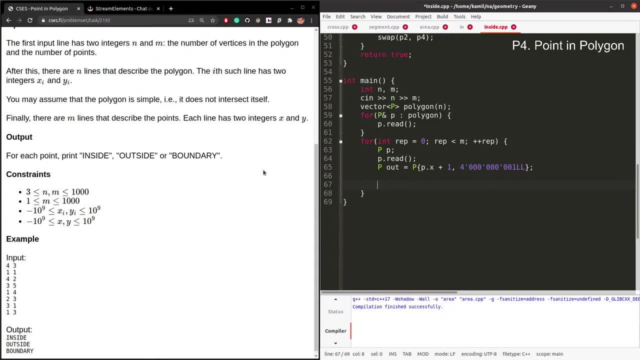 There is another way to deal with that without creating this point. I will mention it after I solve the problem. No, this is not a recorded video. I just don't have a facecam today because even chat, I hid the chat to just focus on. 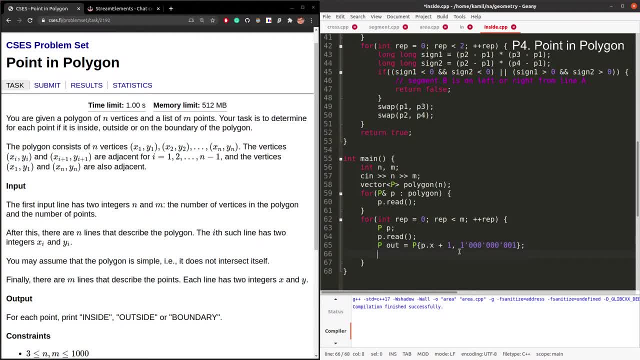 I believe that we need here Three billion. This Actually not slightly too small. Imagine that P, P is Something with coordinates. Let's say this Comma the same For this point. If you are taking this one, It's just very close. 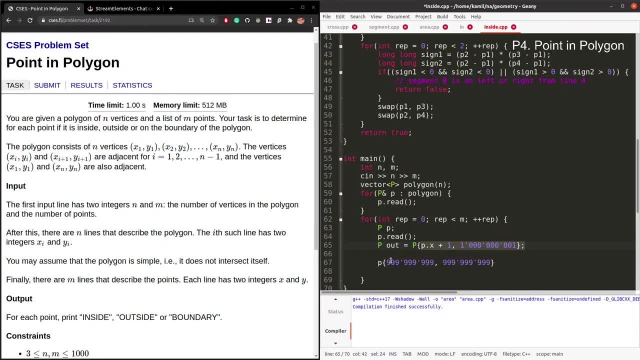 There is, It is far away. We cannot now say that Line from P To this point outside Is a vertical line, just slightly tilted To avoid it being vertical And being collinear with anything else. So it would be really like a vertical line. 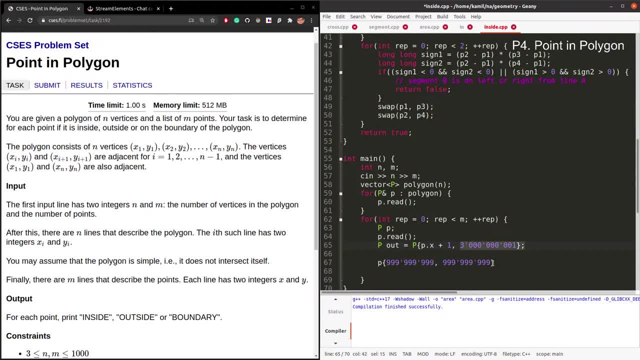 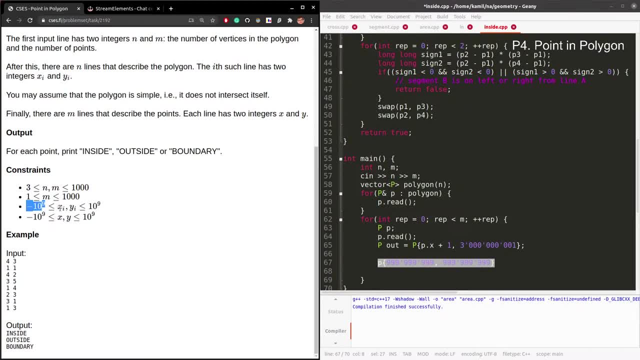 I believe we need this, Then the distance from This point outside to myself Is at least two billion, And it is Greater than What we have here, Like significantly greater. I would even be safer with doing this, But then I'm. 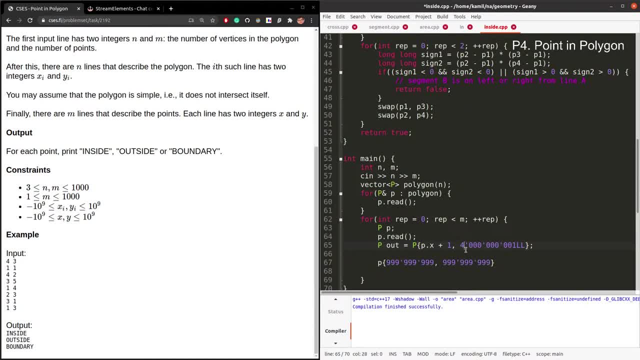 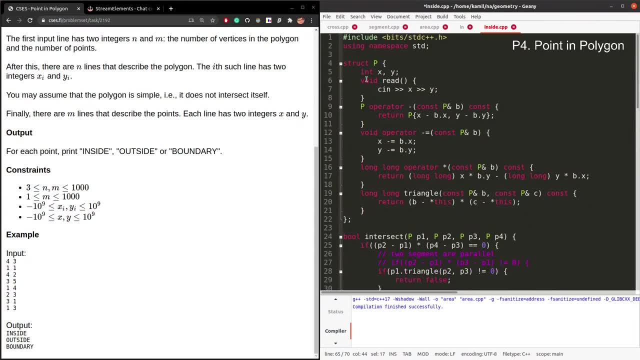 I'm using long-longs- apparently Five million square, Let's say this. I'm afraid about now cross products Overflowing long-long. Let's see, Now we need this. There is another way to deal with that, Without creating this point. 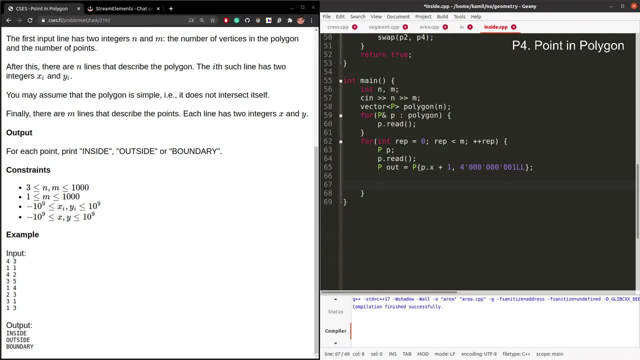 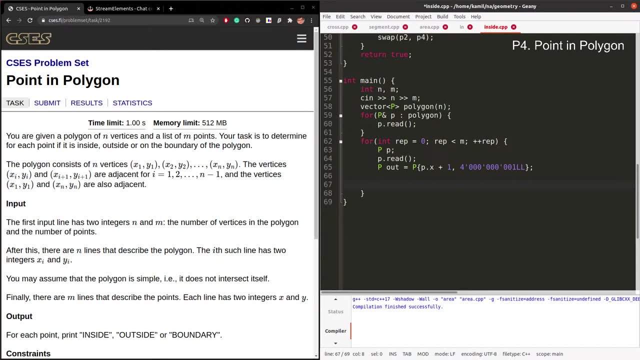 I will mention it after. No, this is not a recorded video. I just don't have a facecam today Because even chat, I hid the chat To just focus on what is on the screen. Fine, What now? For every segment of a polygon? 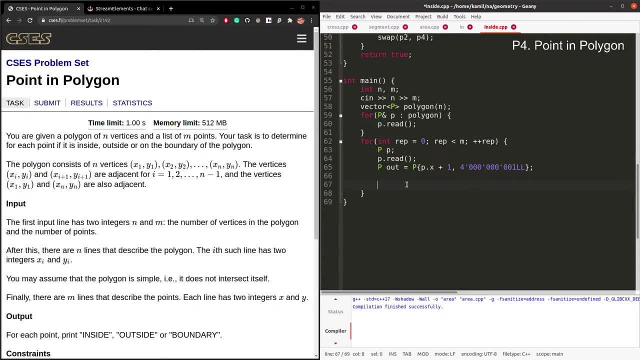 what is on the screen? Fine. What now? For every segment of a polygon? again. the next point is: if this is n minus one, then this point has index zero. otherwise it's i plus one. Actually, this time I wrote it differently than here, but it means the same. 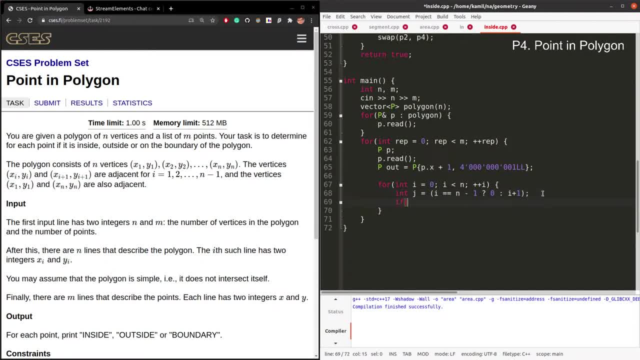 The next point: If, If segments intersect, P out versus polygon of i and polygon of j, Count intersections plus, plus. If it's even, it means that I'm outside because I was made smooth and then bad with spikes. Remember, Now we say outside. 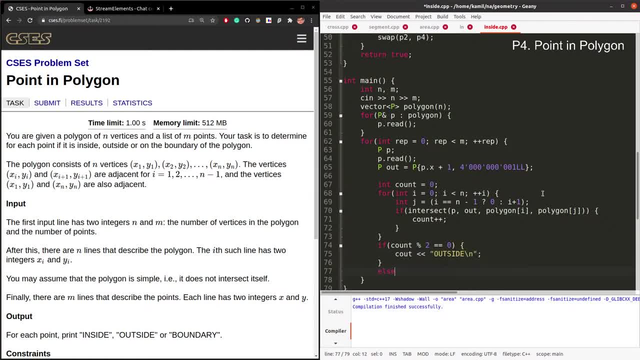 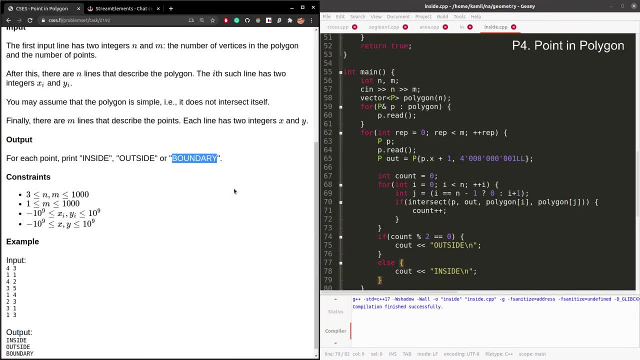 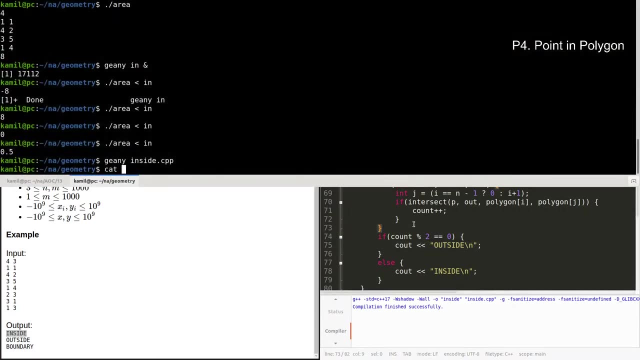 Else inside Here We just didn't care about case exactly on the boundary. If it was guaranteed in the problem that boundary never happens, then this is a correct code, I believe, And it is correct because I got inside and outside I don't detect. 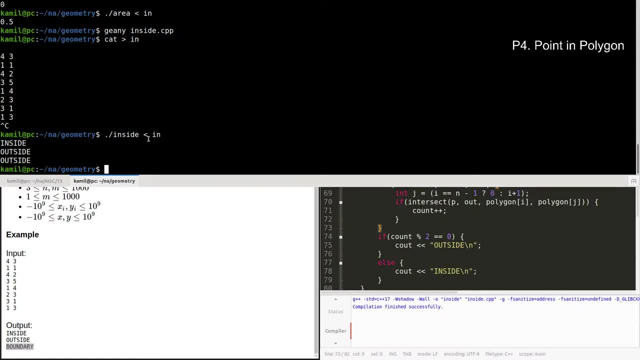 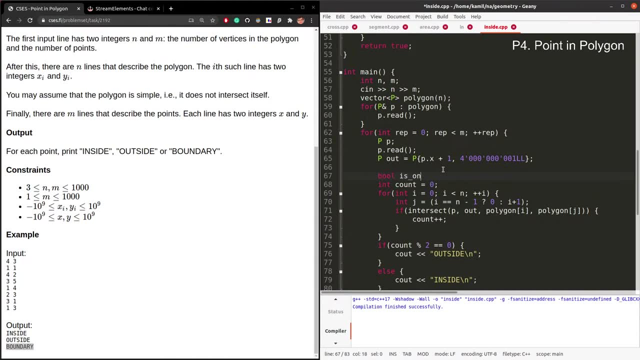 I don't detect boundary correctly, but boundary is on, boundary is true, false. Here I will do: if if point P is on the segment this one, then I detect that it is on. boundary Is on, boundary is true and you can break from for loop. then if you detect that this 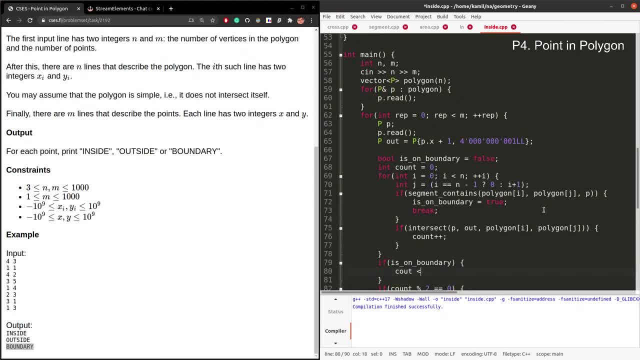 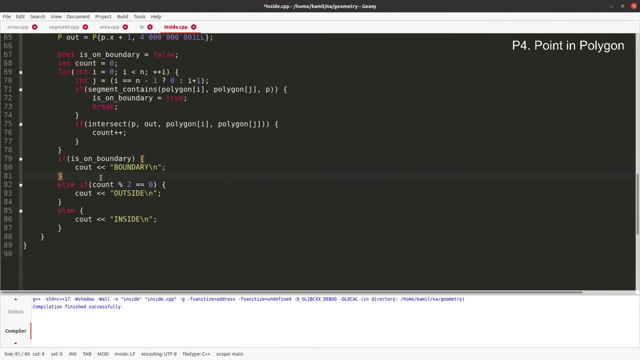 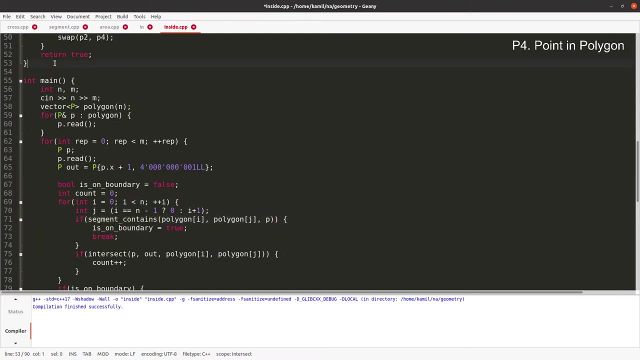 special case that we are exactly on some segment, then this: otherwise we check the parity of the number of intersections with arbitrary array. We need function segment contains. If this was some kind of on-site class with students, then I would now ask them to do: 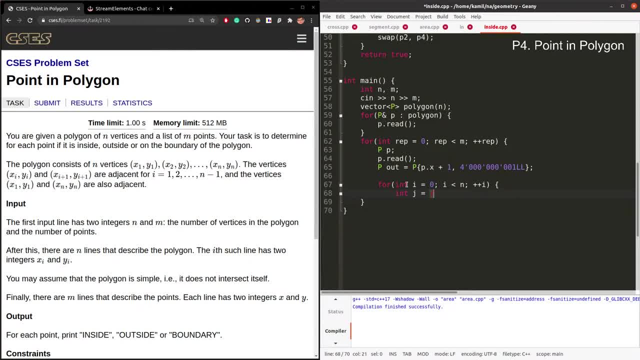 Again. the next point Is: If this is n minus one, Then this point has index zero, Otherwise it's i plus one. Actually, this time I wrote it differently than here, But it means the same. Next point: If The two segments intersect. 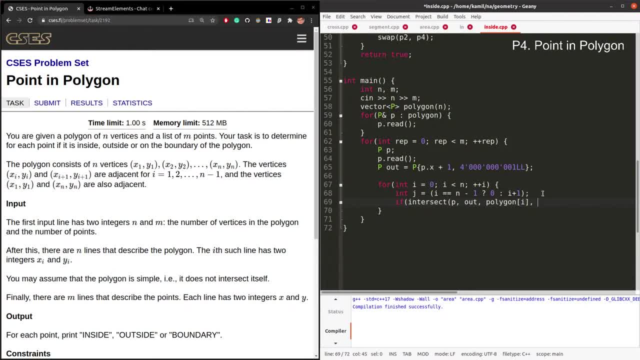 P out versus Polygon of i and polygon of j. Count intersections plus plus. If It's even, It means that I'm outside Because I was made smooth And then bad With spikes, Remember. So now we say outside. 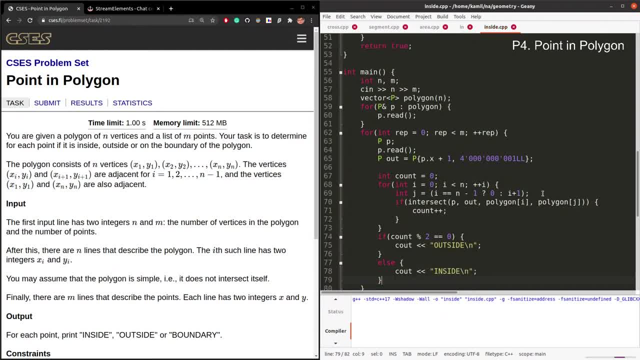 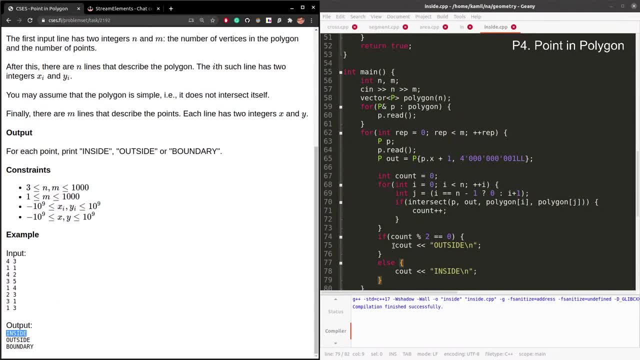 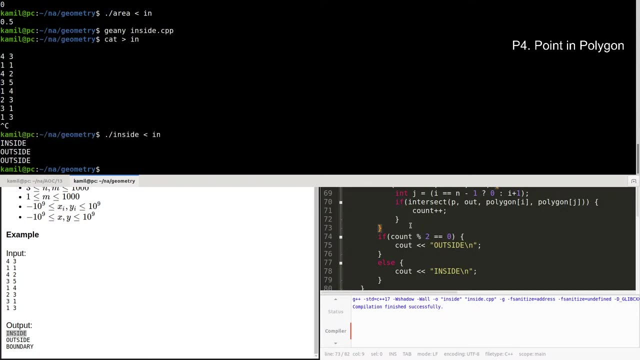 Else inside And here We just didn't Care about case exactly on the boundary If it was guaranteed in the problem That inside never happens. Sorry, boundary never happens. And It is correct Because I got inside And outside. 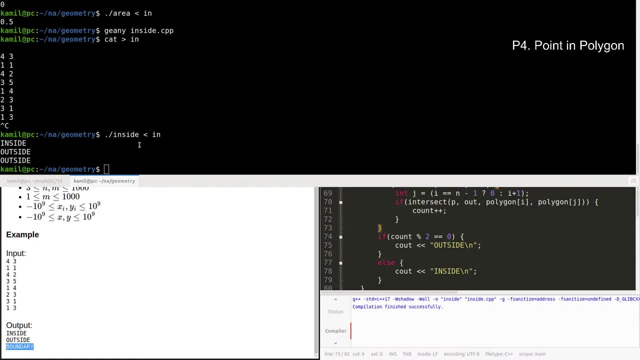 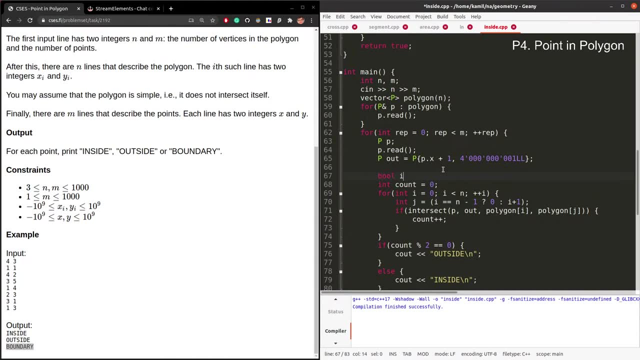 I don't detect boundary correctly, But Boundary. How to do? it Is on Boundary. Here I will do. If If point P Is on the segment, This one, Then I detect that it is on Boundary. 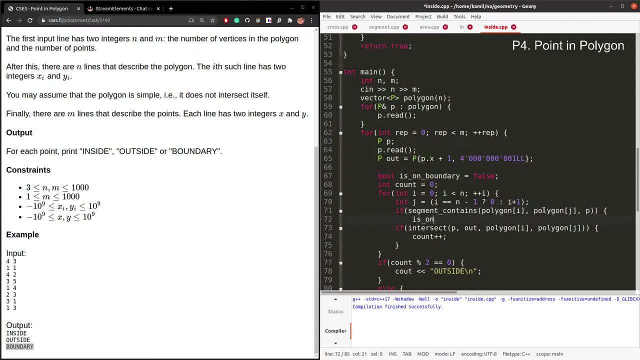 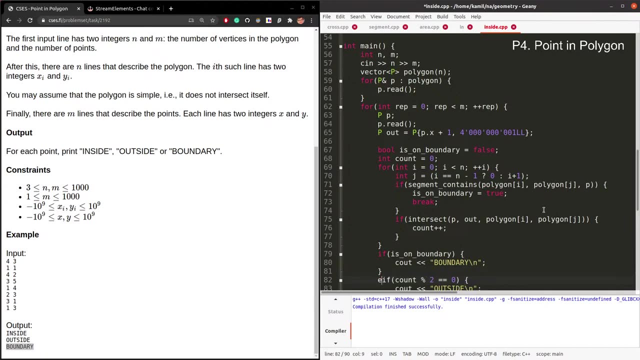 Is on Boundary Is true And you can break from for loop, Then If you detected this special case That we are exactly on some segment, Then this: Otherwise, We check the parity Of the number of intersections With arbitrary ray. 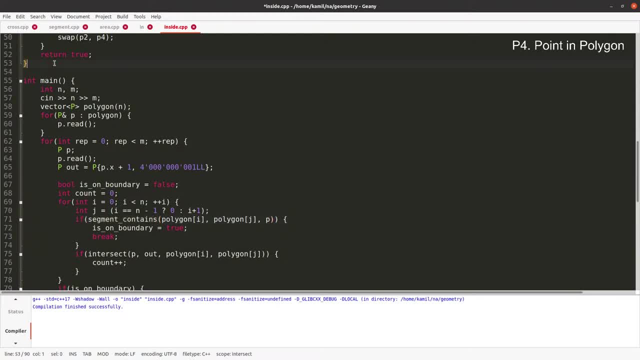 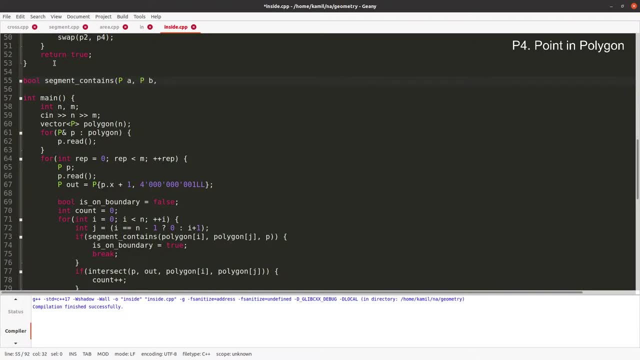 We need function Segment contains. If this was Some kind of on-site class With students, Then I would now ask them To do it. Streams are still a bit less interactive, Even though You can ask questions, But it isn't convenient to. 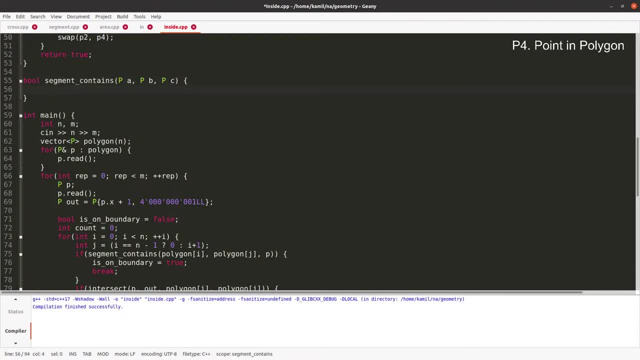 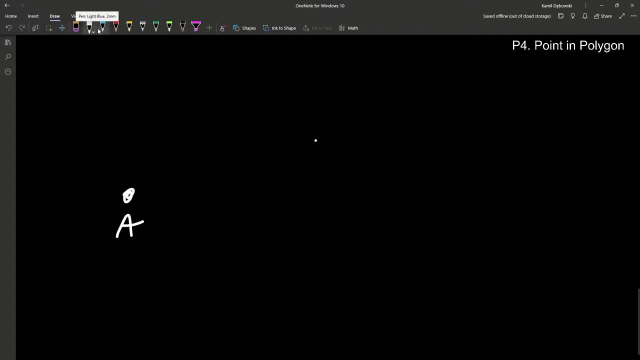 Read 10 answers So we get Some Easier subproblem Where we need to check If segment AB Contains Point C. If you remember What was happening earlier, We did almost the same When checking segment intersection. 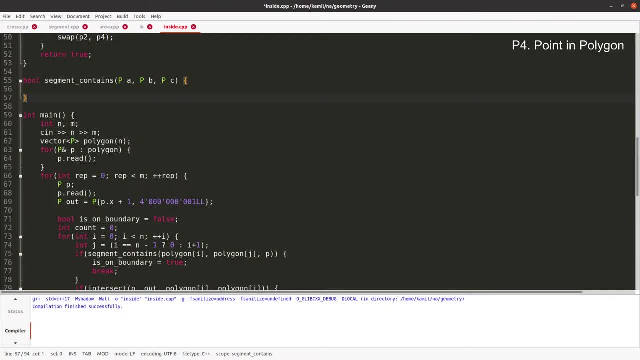 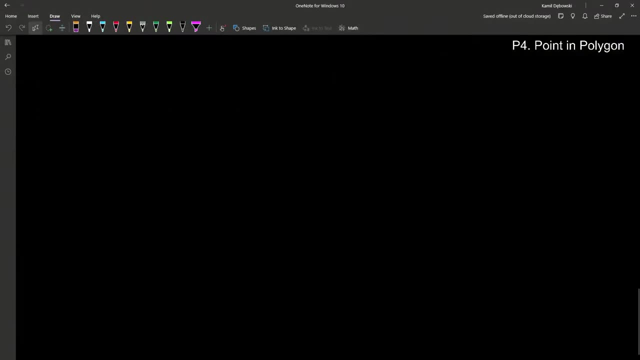 it. Streams are still a bit less interactive, even though you can ask questions, but it isn't convenient to read 10 answers. We get some easier subproblem where we need to check If segment contains point C. If you remember what was happening earlier, we did almost the same when checking segment. 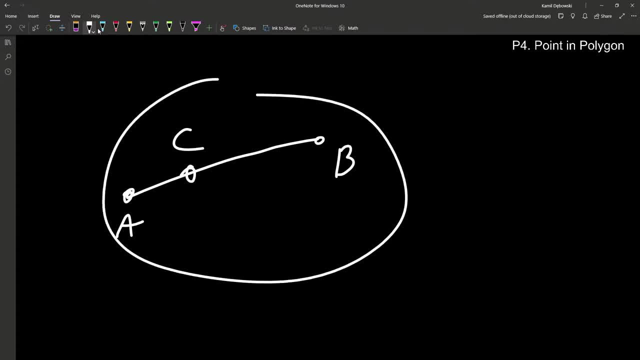 intersection. but this is such a simple problem that I will not even copy paste part of that code. I will just say that ABC must be collinear and I need to deal with such a case where C is outside Right, Even if ABC are. 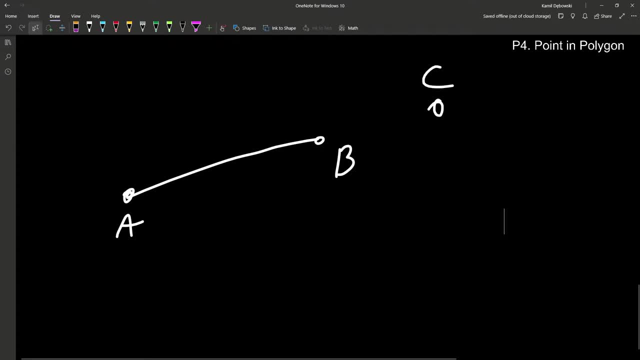 Collinear And this is the case. That's bad. So if collinear and C is between them, You can try some stuff with distances, like check. if distance AC plus distance BC is equal to distance AB, It's valid. Just you need to deal with precision. 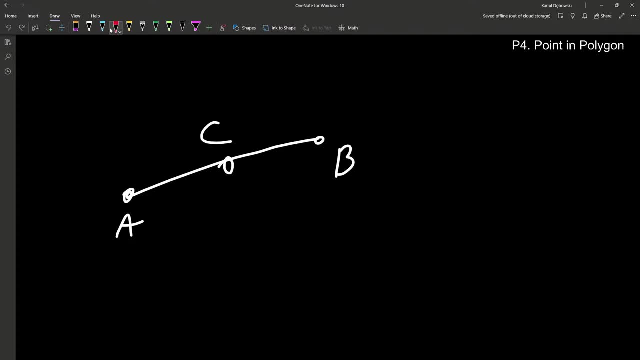 There are for sure a lot of more ways for that. Okay, But I will again use something similar to bounding box. I will say that X is sorted, AX is on the left from CX on the right from BX or the other way around, like A, C, B. 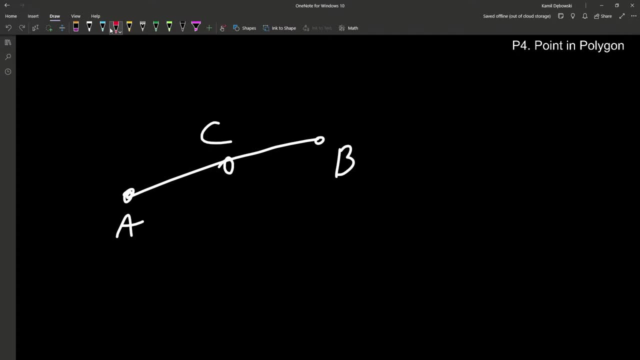 For when we compare Xs, the order must be AX, CX, BX or the other way around. This or that Same with Ys. If that's the case, then what I'm basically checking is if C is in the bounding box. 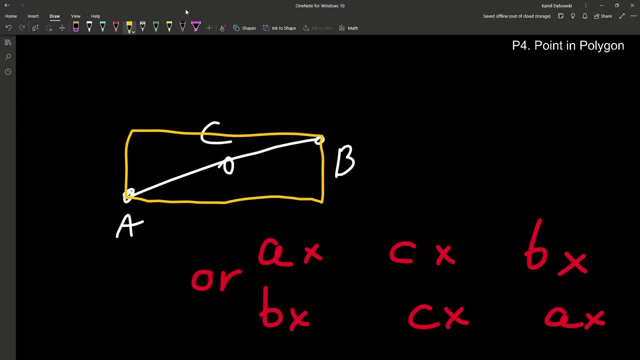 If you know that C is collinear with AB, then what's left to check is if C is in bounding box of AB. So minimum X of A and B, minimum smaller equals CX, smaller equals maximum of Xs, And the same with Ys. 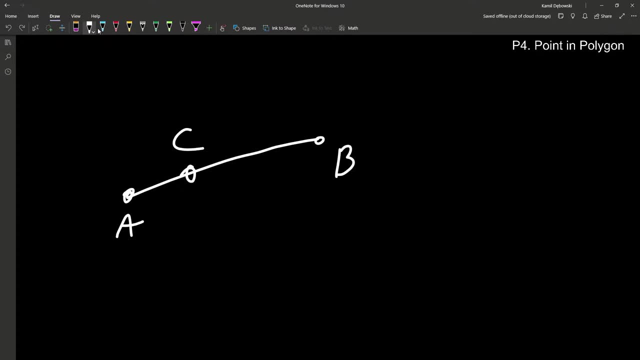 But this is such A simple problem That I will not even copy paste Part of that code. And I need to Deal with such a case Where C is outside, Even if ABC are collinear, And this is the case. 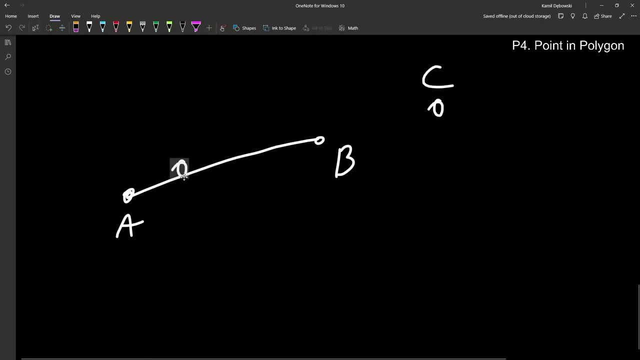 That's bad. If collinear And C is between them, You can try some stuff With distances, Like check. if Distance AC Plus distance BC Is equal to distance AB, You need to Deal with precision. There are for sure. 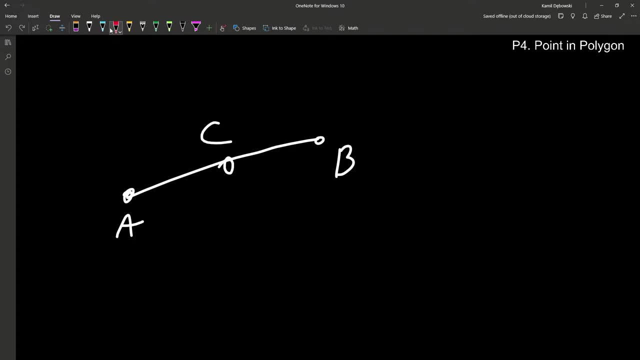 A lot of more ways For that, But I will again use something Similar to bounding box. I will say that X is sorted, AX is on the left from CX, On the right from BX, Or the other way around. 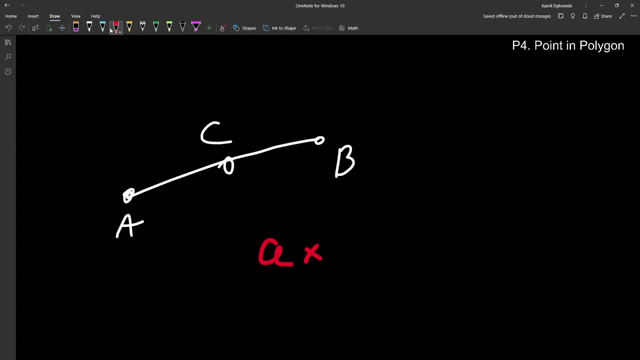 ACB When we compare Xs, XBX Or the other way around, This or that Same with Ys. If that's the case, Then what I'm basically checking Is if C is in the bounding box, If 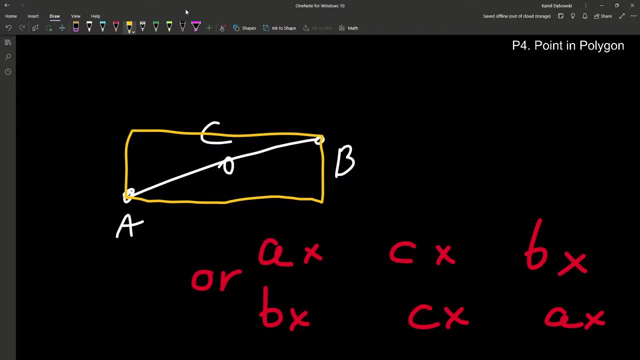 To check. If you know that C is collinear with AB, Then what's left to check Is if C is in bounding box of AB. So minimum X of A and B, Minimum BX, Smaller equal Maximum of Xs. 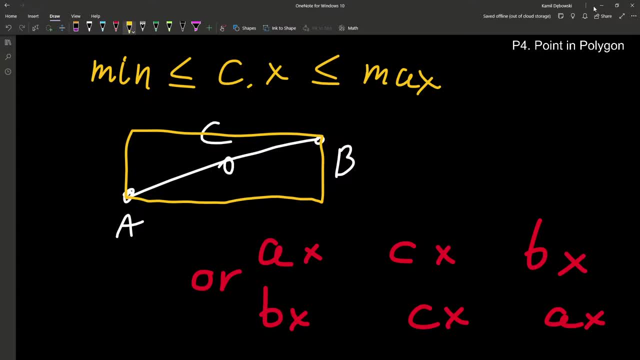 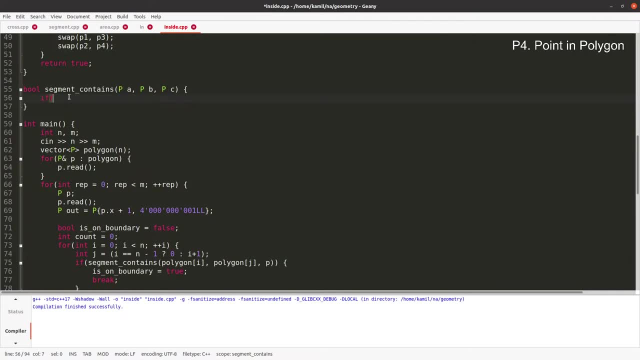 And the same with Ys, Then this way We check if something is in rectangle. Bounding boxes are very useful If, With respect to A Cross product of BC, If this is not 0. Then we don't have collinearity. 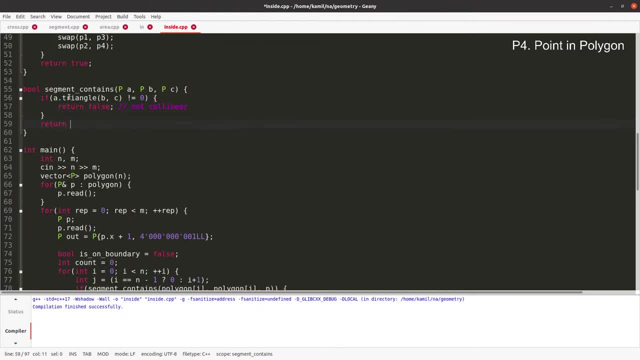 And otherwise Return the fact that Min X Smaller equal than CX And this is Smaller, equal than maximum And same with Ys. Now I'm copy pasting, Sorry about that. Sometimes You implement too much. 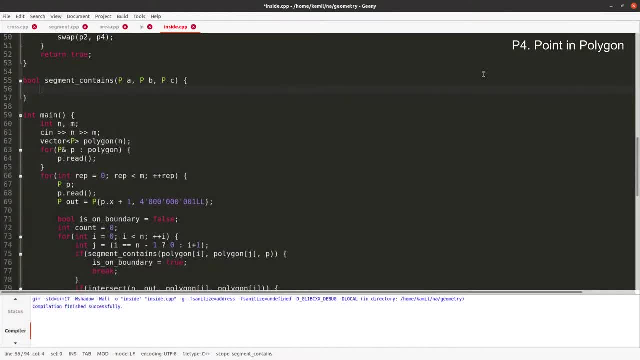 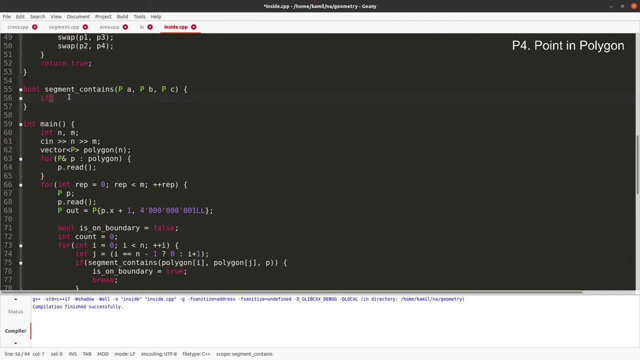 Then this way we check if something is in the rectangle. Bounding boxes are very useful If with respect to A cross product of BC. if this is not zero, then we don't have collinearity And otherwise return the fact that min X 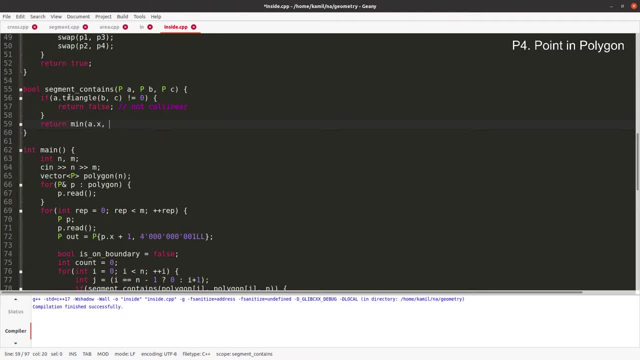 This is smaller, equal than CX. and this is smaller, equal than maximum, And same with Ys. Now I'm copy-pasting. Sorry about that. Sometimes you just implement too much. if you try to avoid copy-pasting, This should be a valid function. 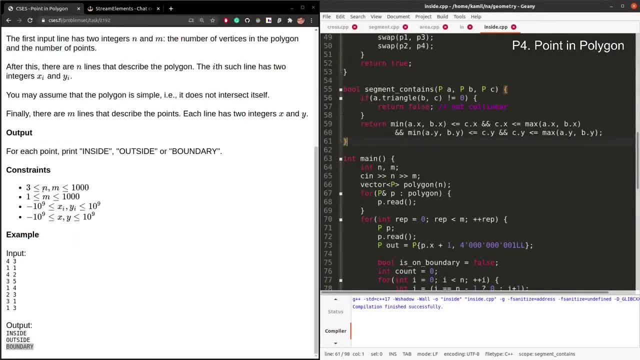 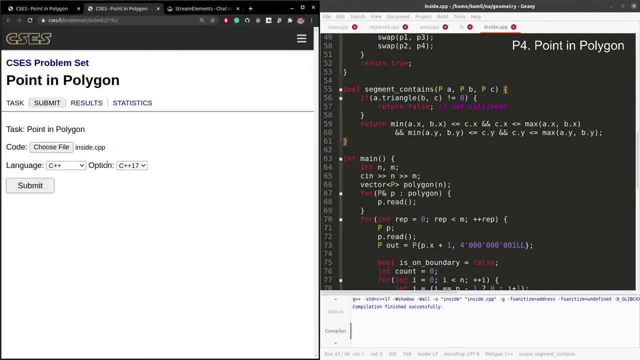 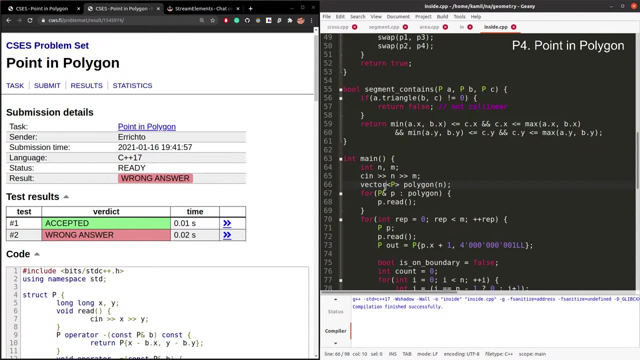 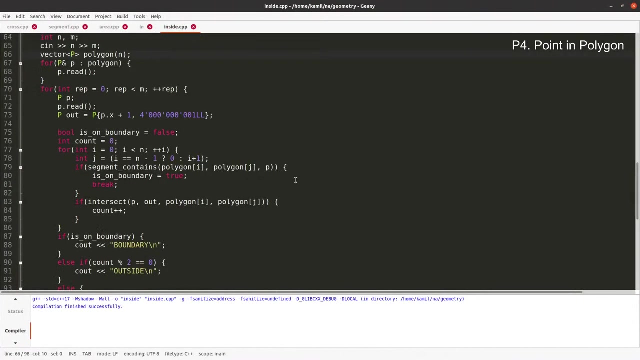 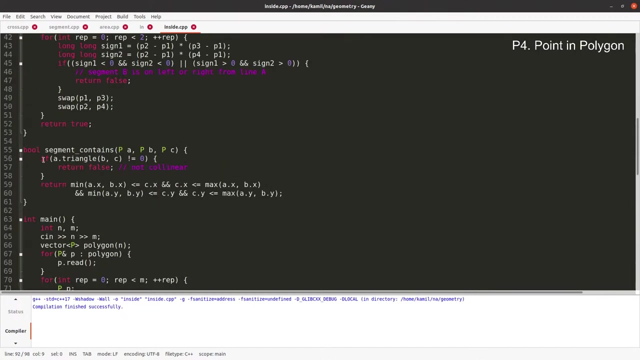 Bounding box issues Inside. outside boundary: submit What was it called inside. Wrong answer. All right, I expect infinity to be the issue, But I'm not sure. I'm not that sure. I will first read this function again. 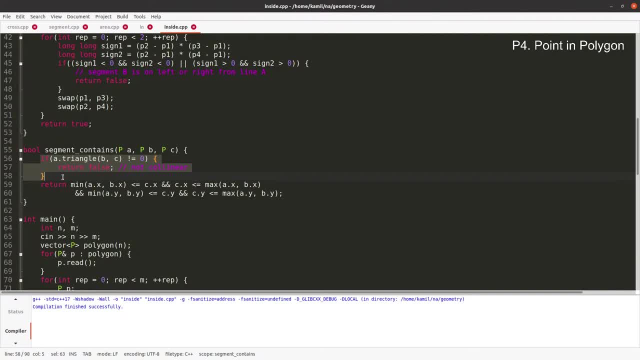 If ABC not collinear, And here we check if minimum X smaller equal C X smaller equal maximum minimum Y, CY maximum Y. Checking X shouldn't be enough, as we are checking collinearity. It is not enough because there can be vertical cases. 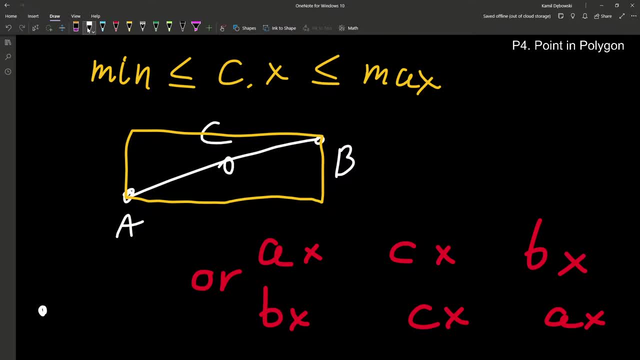 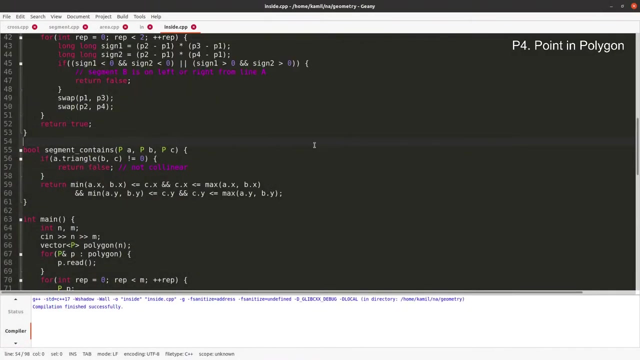 Never assume that X coordinate is enough. Consider this: A, B, C. Our inequality for Xs will say: if you ignore Ys, then here you will detect this as C belonging to interval ABC. It should be A between B and C in checking bounding box. 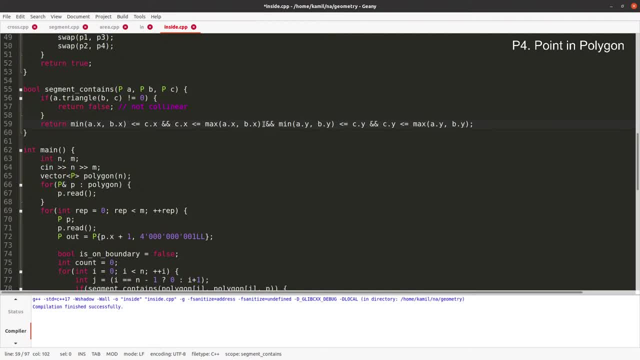 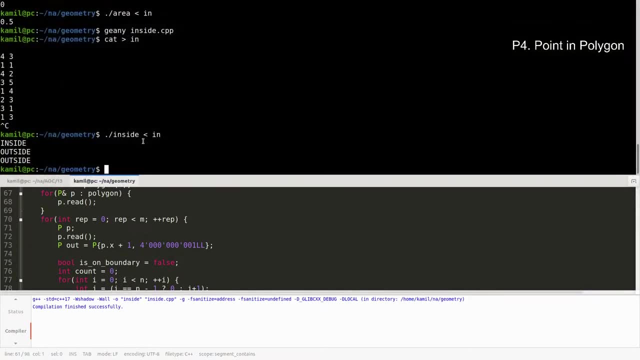 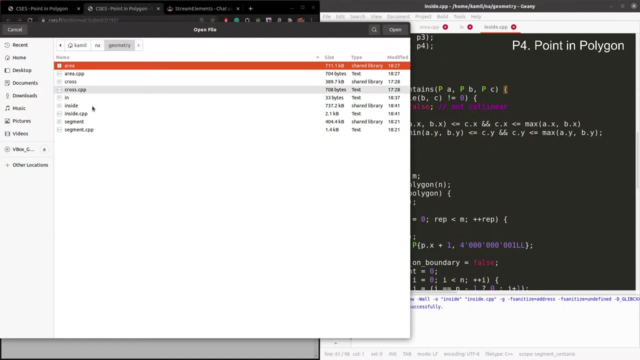 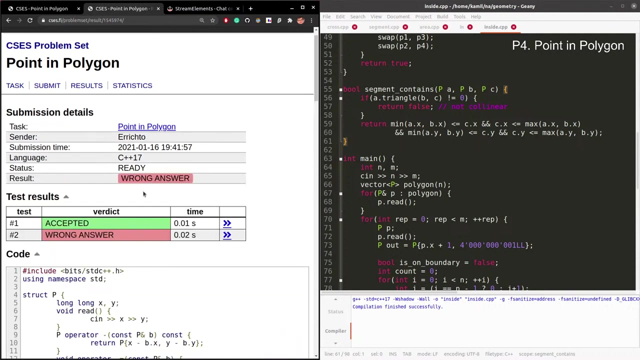 If you try to avoid copy paste, This should be a valid function. Bounding box issues Inside. Outside boundary Submit. What was it called Inside? Wrong answer. Alright, We expect infinity To be the issue, But I'm not that sure. 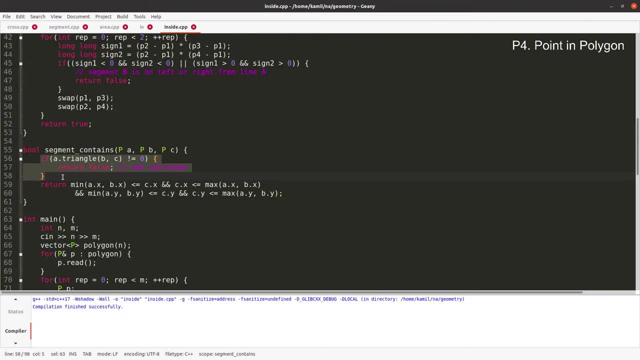 I will first read This function again: If ABC Not collinear, And here we check: If minimum of X Smaller equal C Smaller equal maximum Minimum Y, CY Maximum Y. Checking X shouldn't be enough. 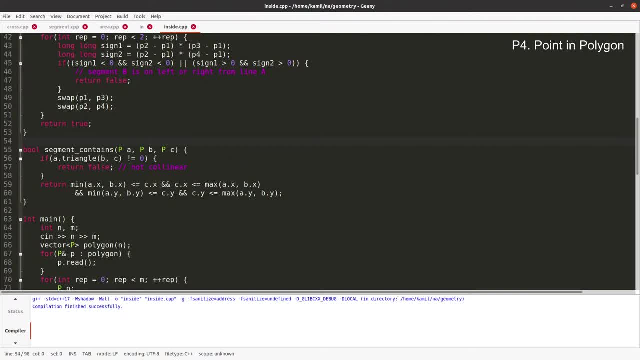 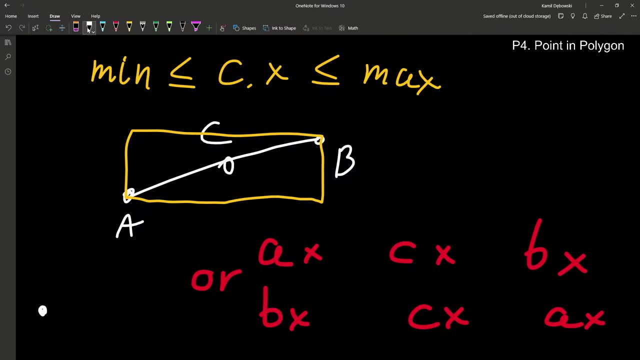 As we are checking collinearity, It is not enough Because there can be vertical cases. Never assume that X coordinate is enough. Consider this ABC: Our inequality. for You know, For Xs Will say If you ignore Ys. 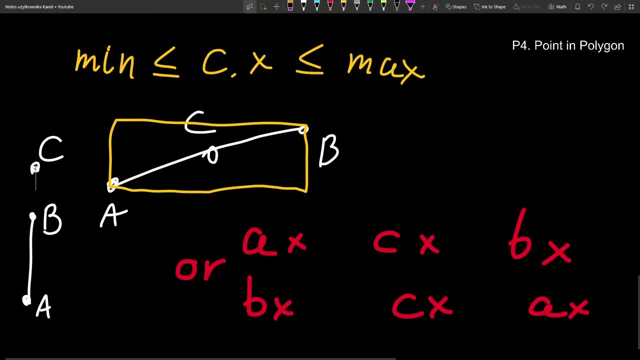 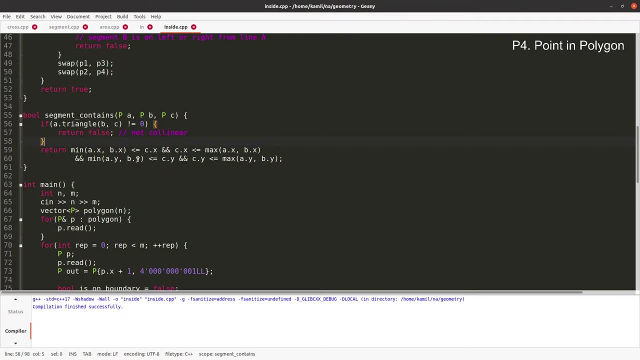 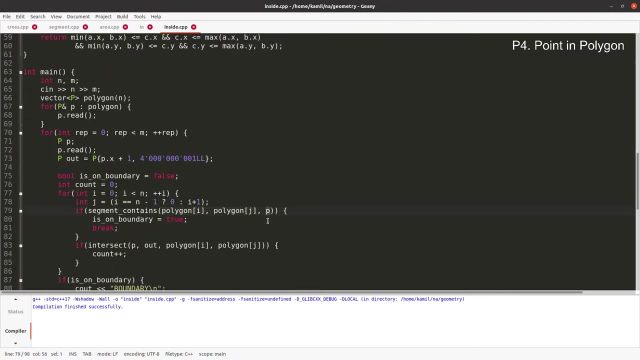 Then here you will detect this As C belonging to interval AB. It should be A between B and C In checking bounding box, Should it? We check if In this segment There is point P. I check if C is between AB. 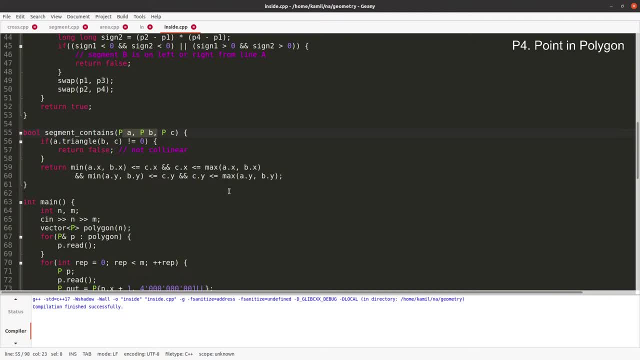 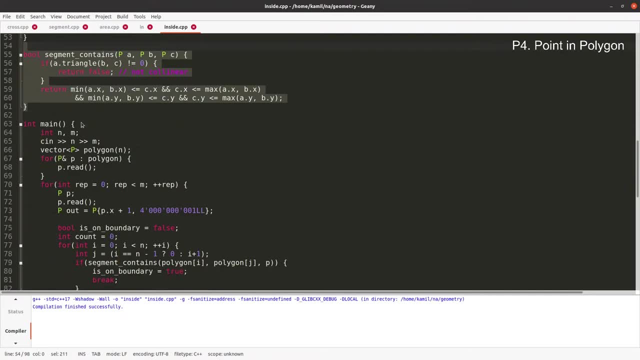 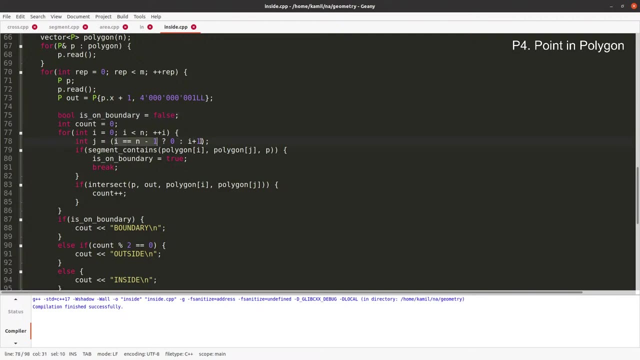 Right? Who gets it first? What's wrong here? I don't know. I didn't make a mistake on purpose. If you are wondering, I think the function is fine. What happens there? It's on boundary. If this is the last point, 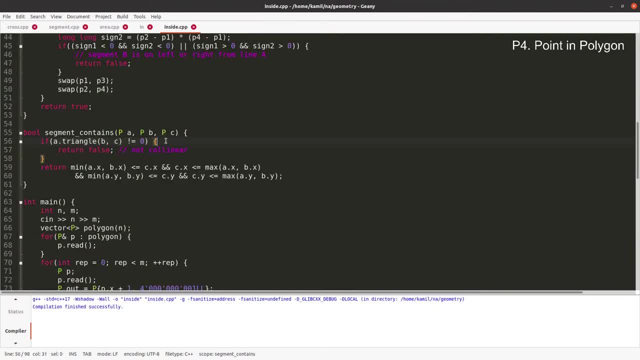 Then 0. Otherwise, A plus 1.. Shouldn't ABC triangle? this Doesn't matter, It will give you cross product 0. Their slopes will be the same. If they are not collinear, Then no matter which one you choose. 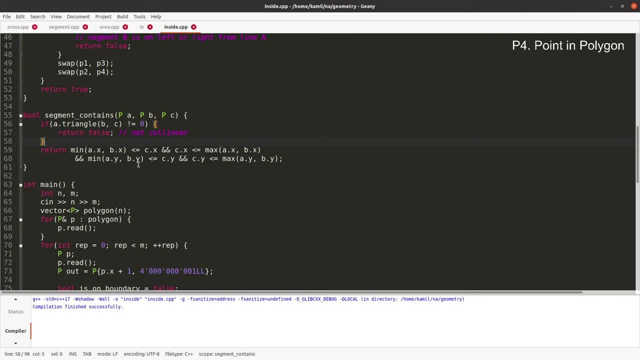 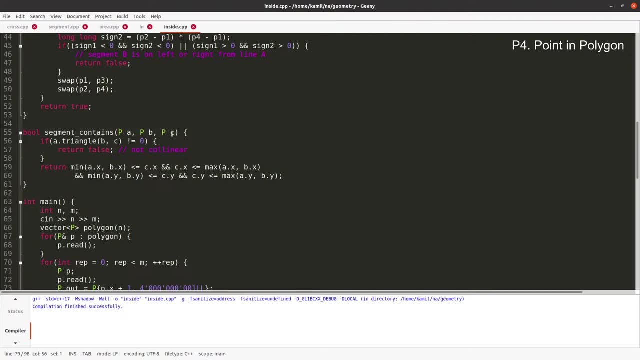 Should it? We check. if in this segment there is point P, I check. if C is between A, B, Right, Who gets it first? What's there? What's wrong here? I don't know, It's not. It's not. 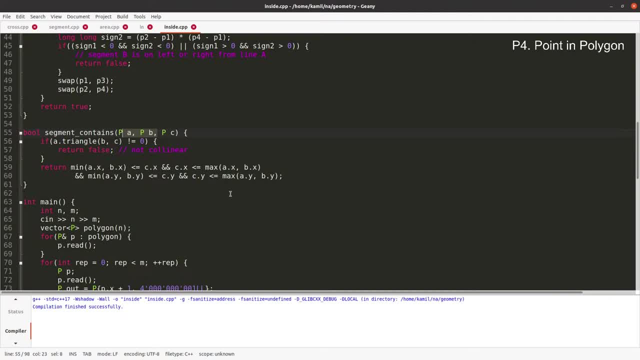 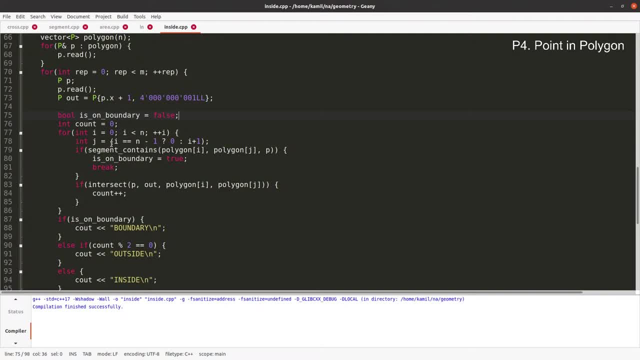 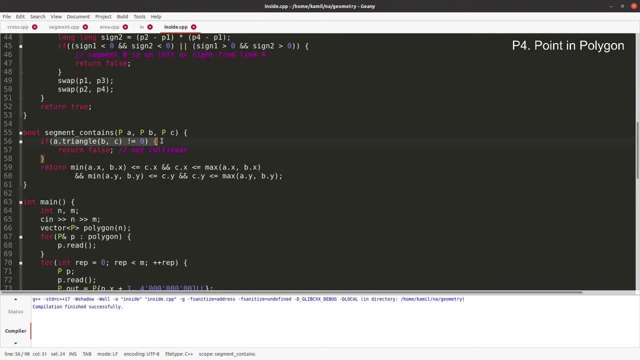 What happens there? It's on boundary. If this is the last point, then 0.. Otherwise, A plus 1.. Shouldn't ABC triangle? this Doesn't matter, I check if ABC are collinear. If collinear, then with respect to any of them, the other two will give you cross product. 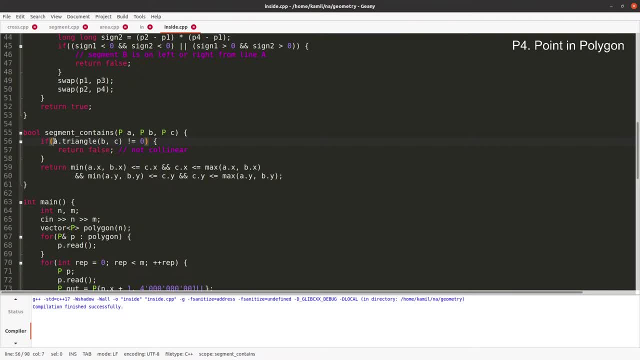 0. Their slopes will be the same If they are not collinear, Then Which one you choose. I could replace this with B Or with C, It's all the same. When just checking, comparing something with 0.. 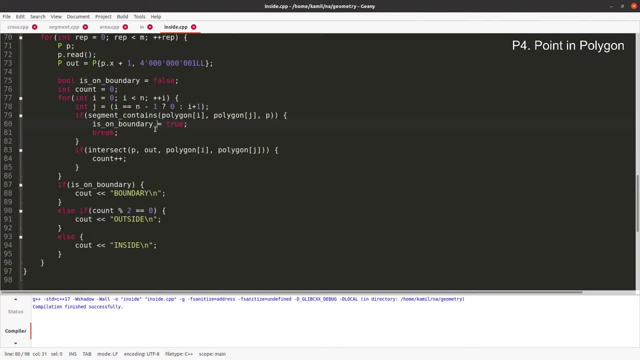 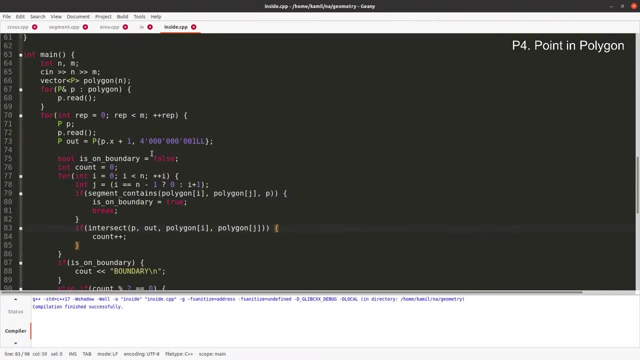 Return: true if this is inside, All right. Polygon IJ. if it contains P. If yes, then it's on boundary. All right, then this seems dangerous. 4 billion Multiplied by something of magnitude 1 billion Will give us 4 times 10 to 18.. 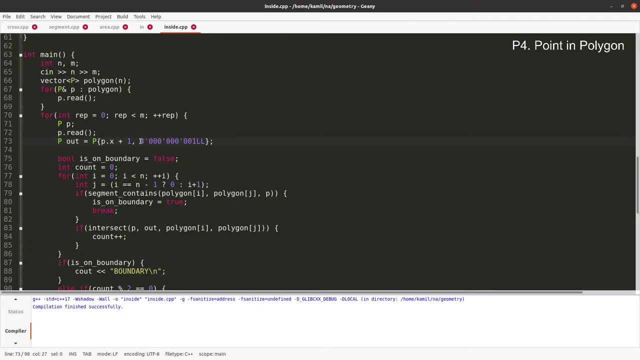 I'm curious if long, longs are enough, But I think they are. Well, we can later use something like out, Like when we do P minus some other point And then multiplied by something, When P has 4 billion as infinity. 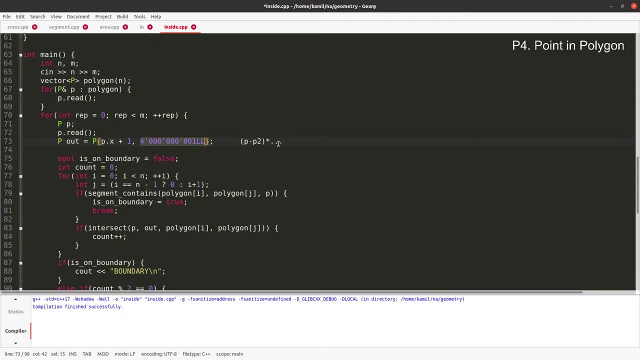 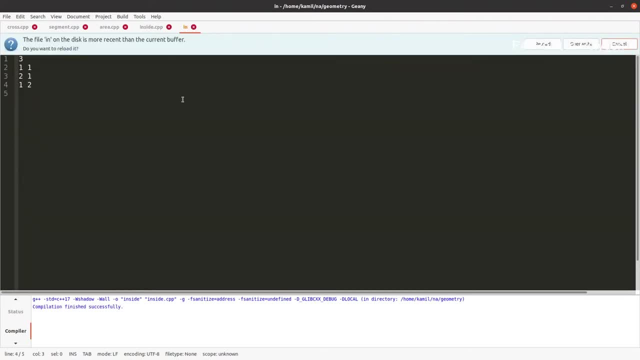 Then I would guess that's That's dangerous. Hmm, There is one way for me Maybe to check this. I will try some Infinities. I'm not sure if this is enough. Those are 4 infinities. 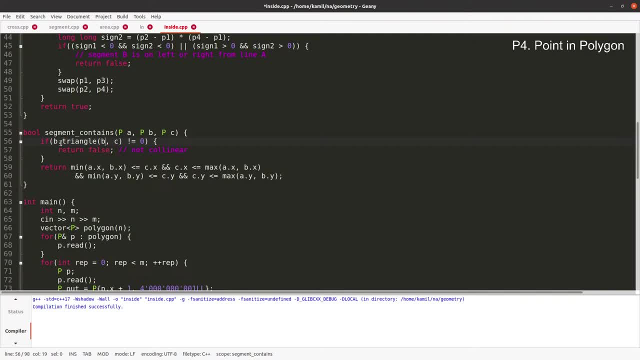 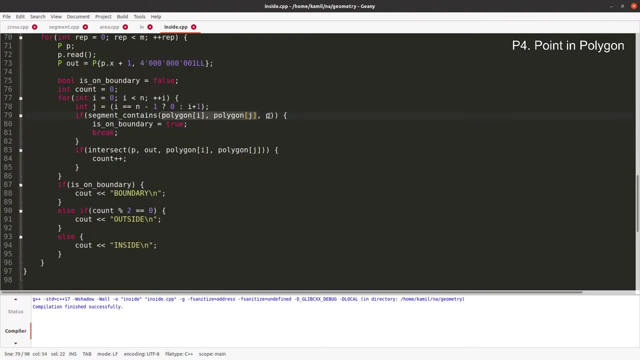 I could replace this with B Or with C, It's all the same. When Just checking, Comparing something with 0.. Return: true if this is inside Right Polygon IJ. if it contains P. If yes, Then it's on boundary. 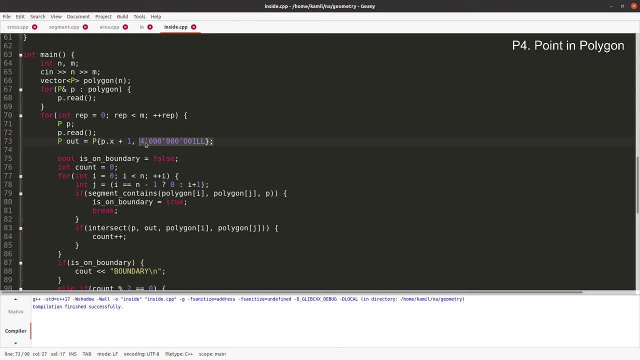 Then this: This seems dangerous: 4 billion Multiplied by something of magnitude 1 billion Will give us 4 times 10 to 18.. I'm curious if long-longs are enough, But I think they are. Well, we can. 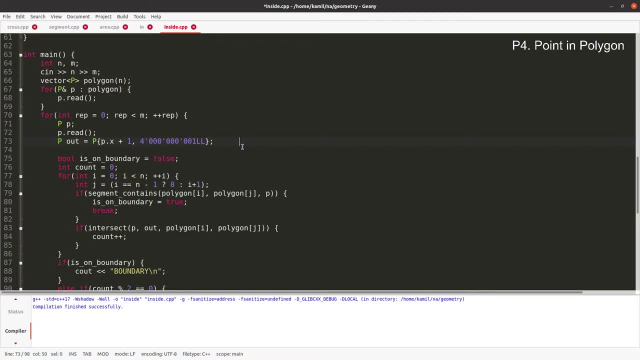 Later use something like When we do P minus some other point And then multiplied by something, When P Has the same value As 4 billion, as infinity, Then I would guess that That's dangerous. There is one. 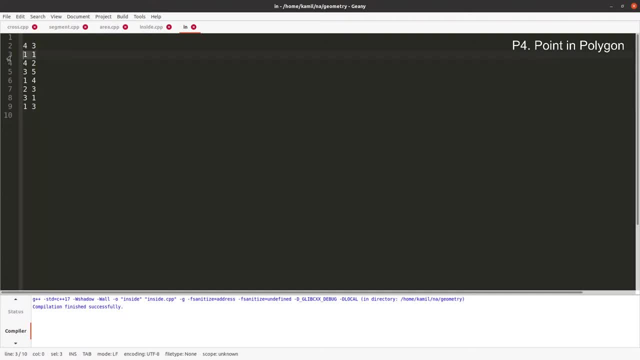 Way for me, Maybe to check this. I will try some Infinities. I'm not sure if this is Enough. Those are 4 infinities. Should they be in order? They are in order. Something wrong with input. 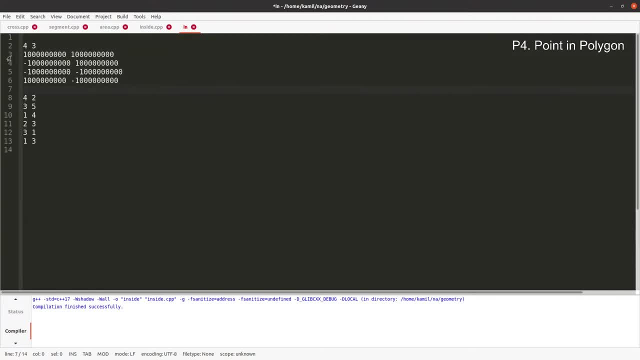 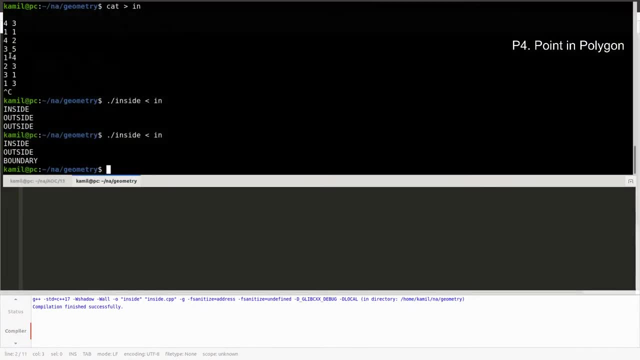 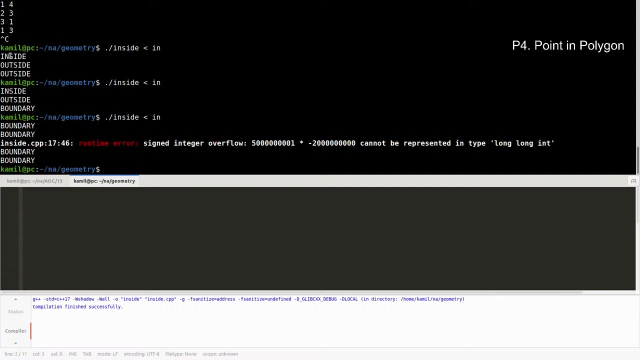 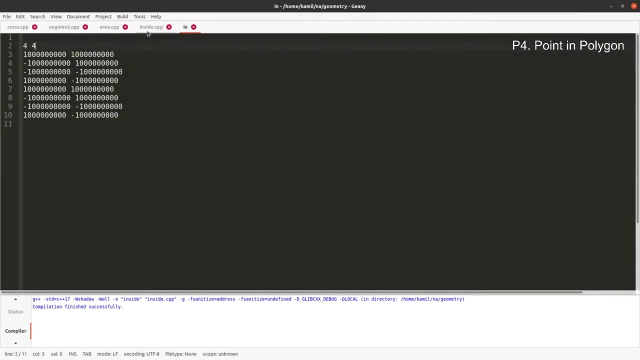 What's this? And then there are queries. Let's say, I just repeat those points. If I get any Overflow- Yes, I see it in red, That's great. 5 billion multiplied by 2 billion, That's an overflow on long-longs. 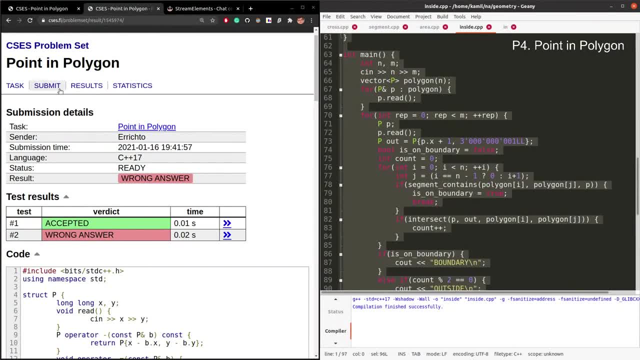 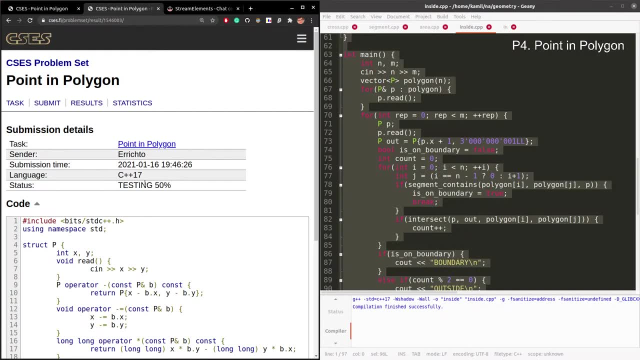 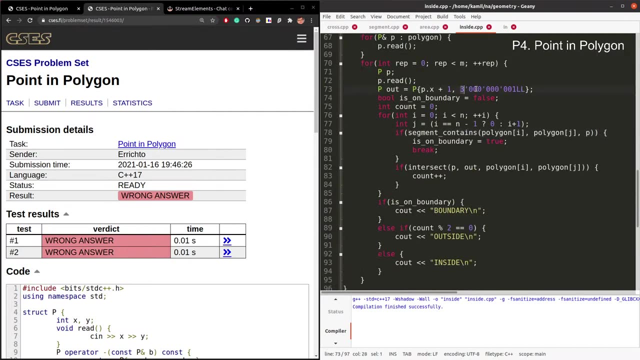 After taking 3 billion At least, I didn't get an overflow here. Let's hope that this was enough. It's obviously Dangerous To go above billion times billion. Did I mess up something, And maybe now This value is not enough? 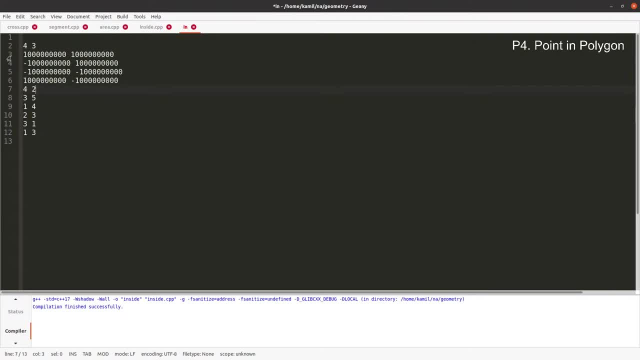 Are. Should they be in order? They are in order. Was something wrong with input? What's this? No. And then there are queries. Let's say I just repeat those points If I get any overflow. Yes, I see it in red. 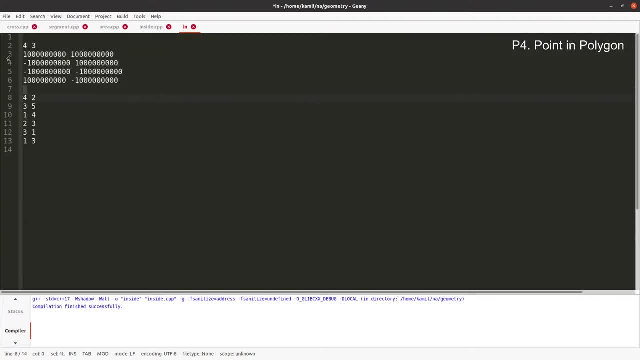 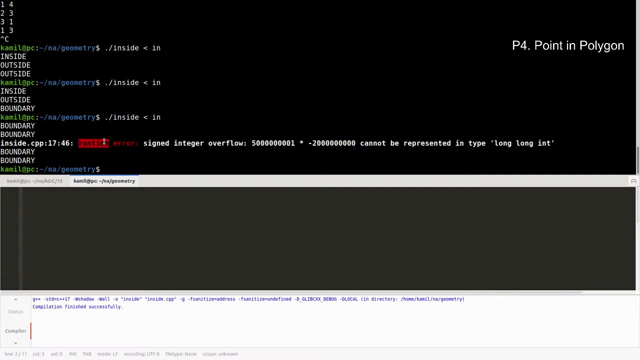 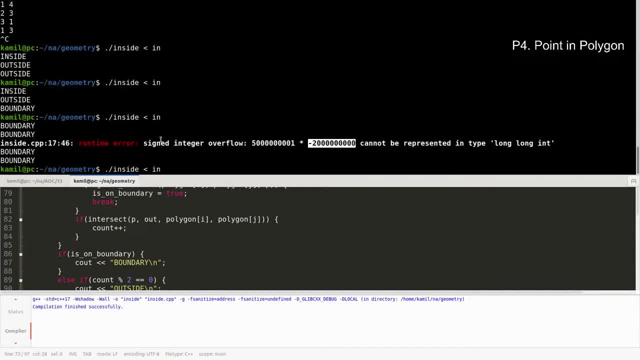 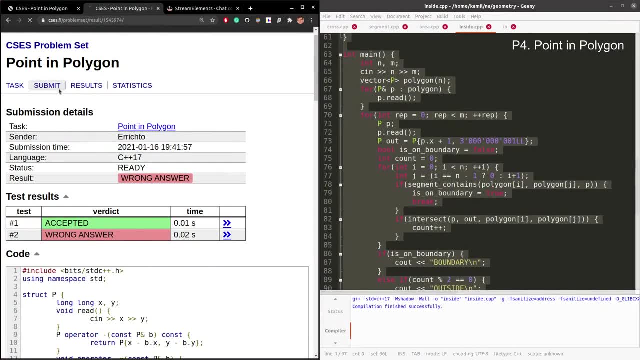 Yes, That's great. 5 billion Multiplied by 2 billion, That's an overflow on Logs After taking 3 billion. At least I didn't get an Overflow here, And Let's hope. 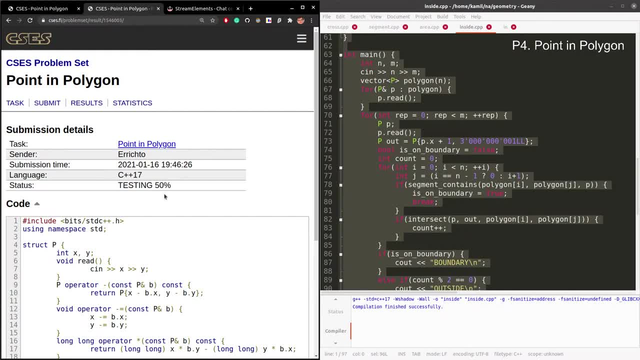 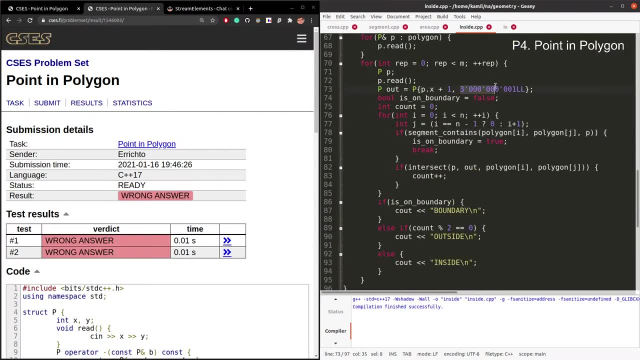 That this was Enough. It's obviously Dangerous To go above billion Times Billion and hope That They mess Up. Maybe now this value is not enough. that'd be a case. Well, I told you at the beginning of coding this solution that there is a way to avoid. 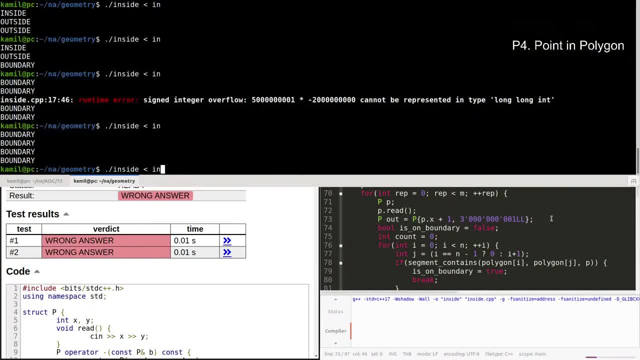 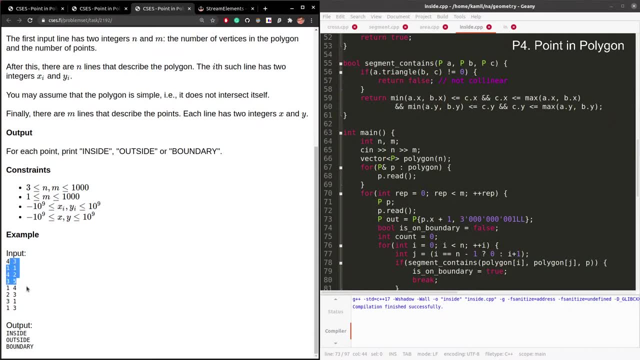 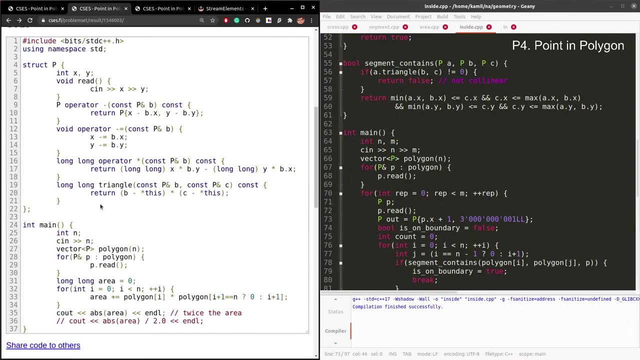 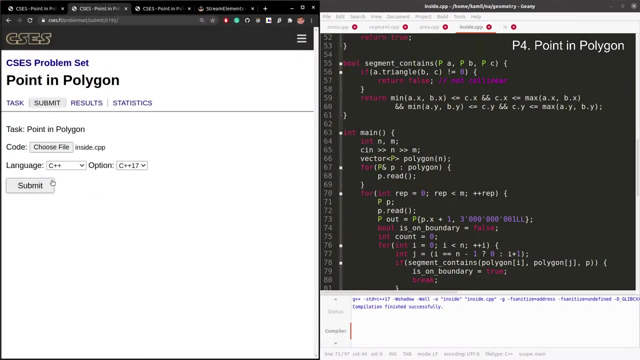 this And apparently we need to use it. Let's check sample test. Maybe I messed this up completely or maybe just 3 billion is not enough. You submitted the wrong file, did I? Yeah, I print, all right, thank you. thank you inside. 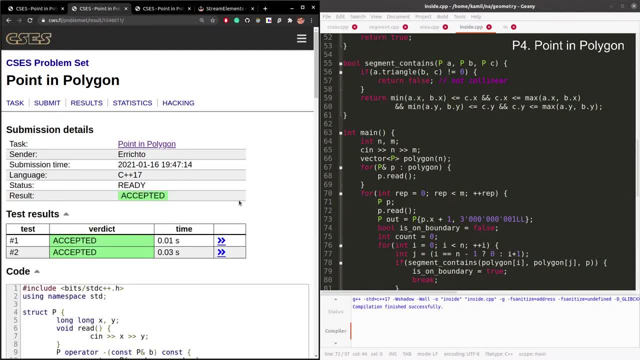 Thank you, chat. I would waste a lot of time. no Accepted. so it's good that we are not wasting time debugging a correct solution, And I believe that 1 billion here will be wrong, and I told you why. it can be very close. 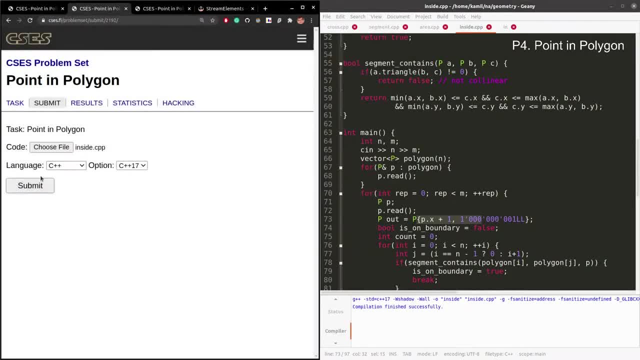 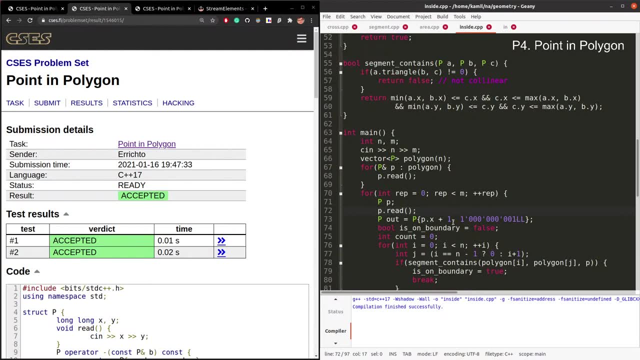 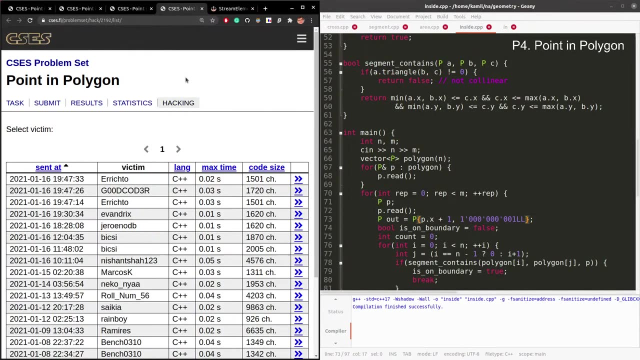 to our point. Okay, I think this is wrong submission. It isn't. Then tests are bad. I can come up with a test where a point is very close to billion. Actually, there is hacking feature. so I invite you to take this last submission of mine. 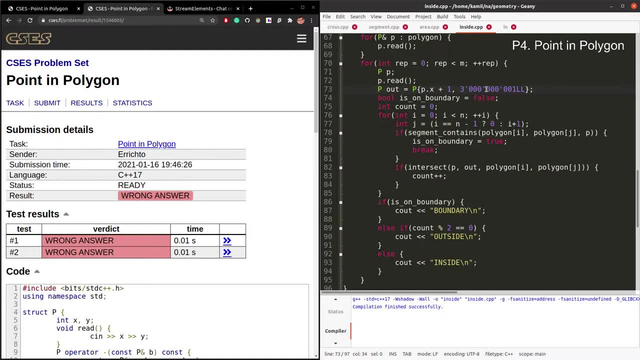 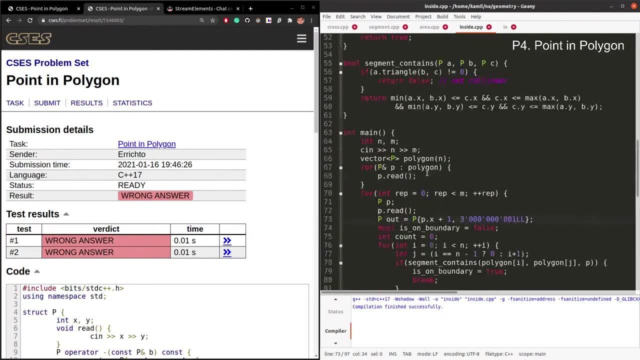 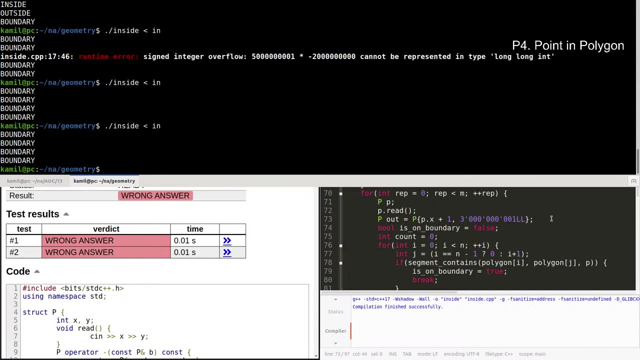 That'd be a case. Well, I told you at the beginning Of coding this solution That There is a way to avoid this, And apparently We need to use it. Let's check sample test. Maybe I messed this up. 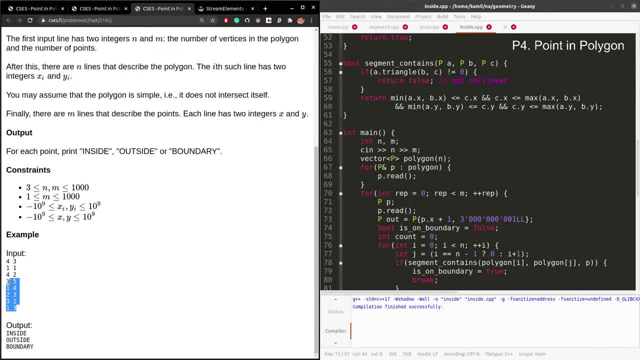 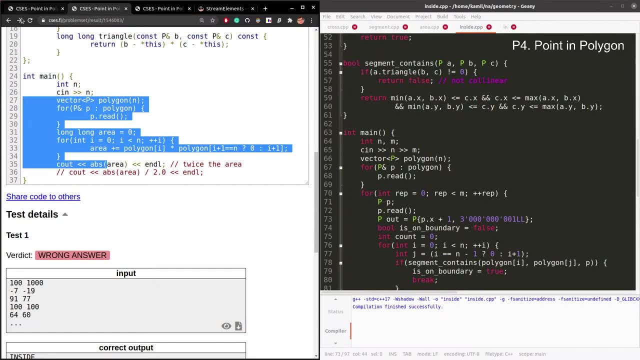 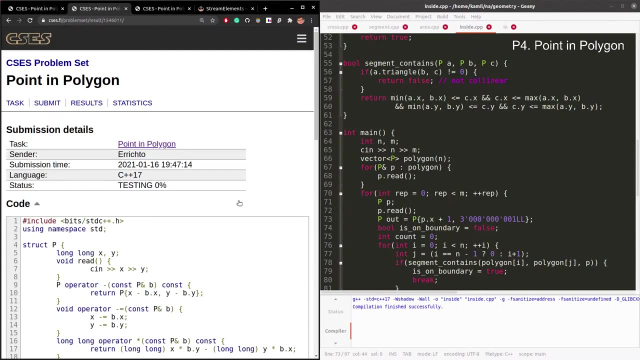 Completely, Or maybe just 3 billion is not enough. You submitted the wrong file, Did I? Yeah, I print Thank you Inside. Thank you, chat. I would waste a lot of time Accepted. It's good that we're not wasting time. 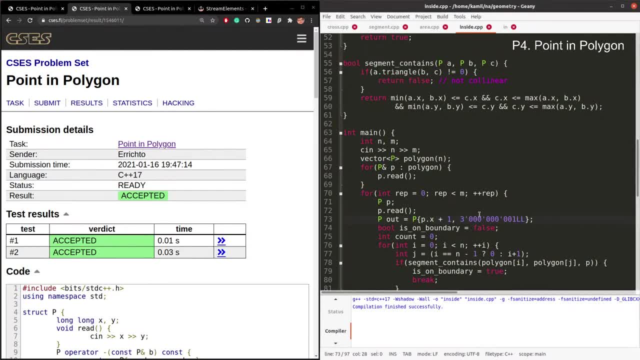 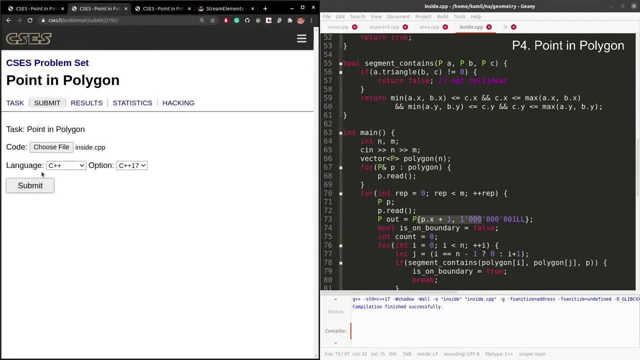 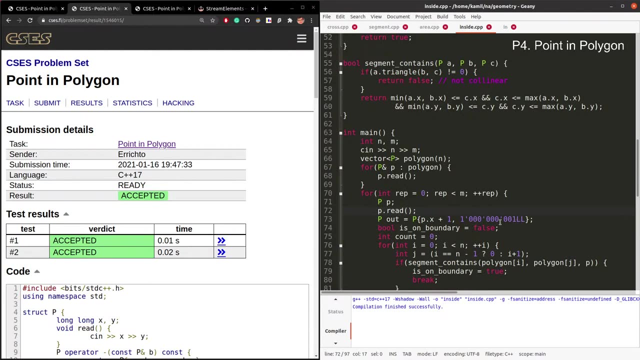 Debugging a correct solution. I believe that 1 billion here will be wrong. I told you why. It can be very close to A point. I think this is wrong. Submission It isn't, Then tests are bad. I can come up with a test. 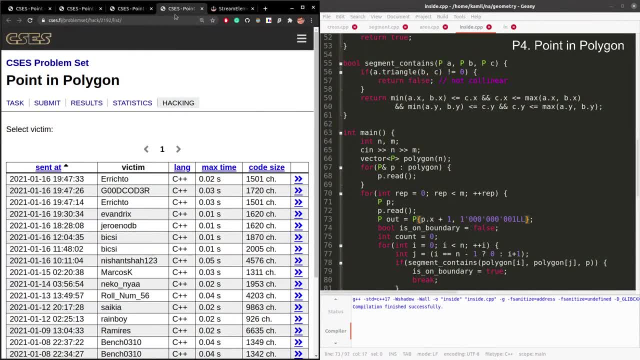 Where a point is very close to billion. Actually, there is hacking feature, So I invite you to Take this last submission of mine, This one With this timestamp, This ID, If you need it And try to hack it. Maybe then it will be added. 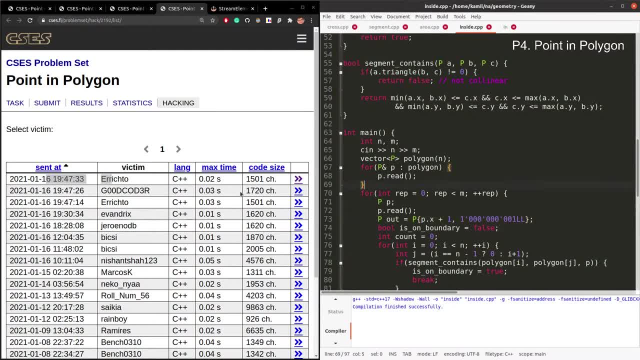 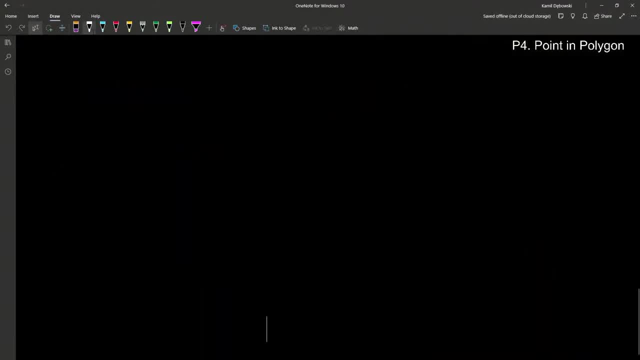 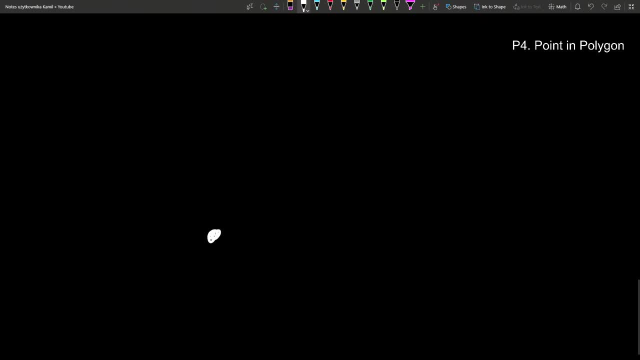 To all the tests. A few words about Alternative implementation. What can we do To avoid taking this arbitrary point At infinity? As I told you, What I want to achieve is Get any ray From this point P. That is not. 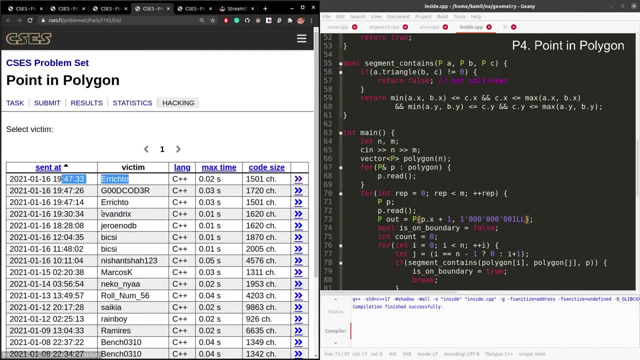 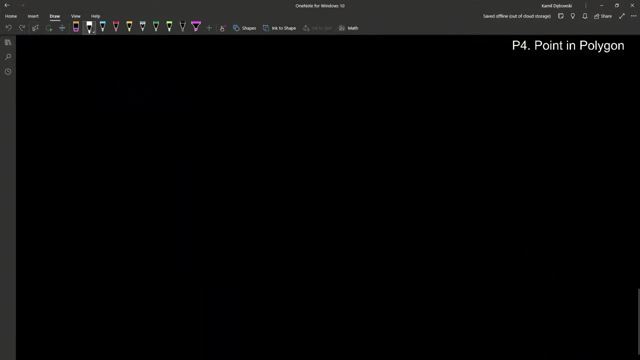 the one, this one with you know, this timestamp, this ID, if you need it and try to hack it, Maybe then it will be added. I will put all the tests. A few words about alternative implementation. What can we do to avoid taking this arbitrary point at infinity? 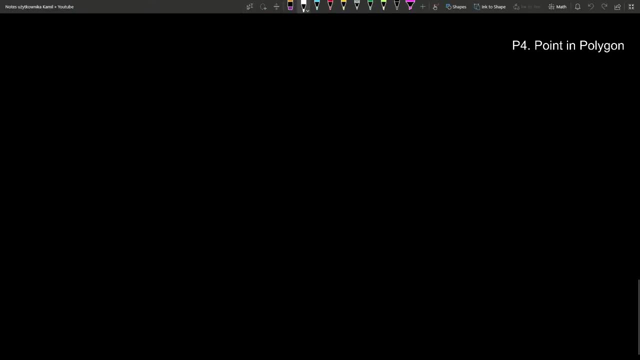 As I told you, what I want to achieve is get any ray from this point P that is not collinear with anything, Because you don't. It's tricky to handle cases like that. If you took this ray, then we always assume that we move to the left or to the right. 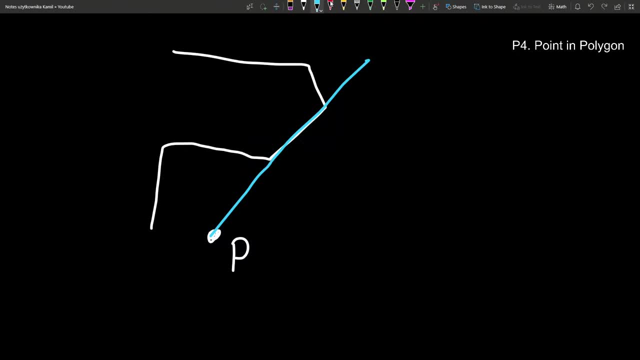 We didn't say exactly what happens in this case and it's very ugly. You don't want to deal with this case. If your ray contains some segment, that's terrible. I always And that's in real context What I do in ICPC when I have such a problem. 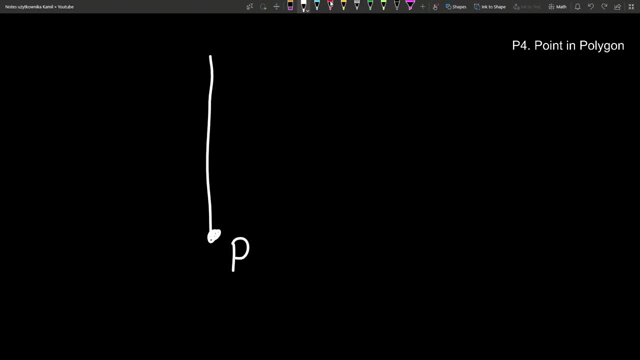 Then I imagine that I have vertical ray, But actually it's tilted to the right by epsilon And I don't create any point here. I just imagine that. Then what happens is, if you For any point when I deal now with some segment AB. 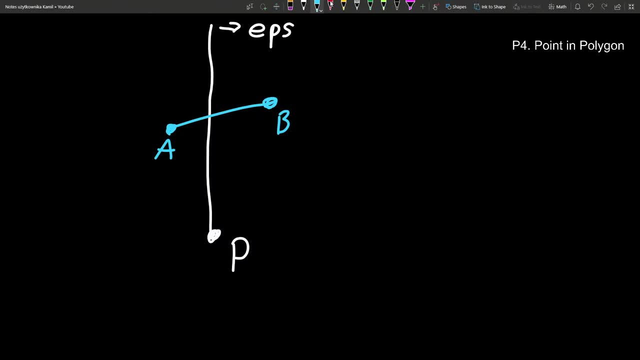 For A and B. I need to decide if they are on the left or on the right of This thing. And I say this: Everything here, including the line, is on the left And everything, excluding the line on the right, is on the right. 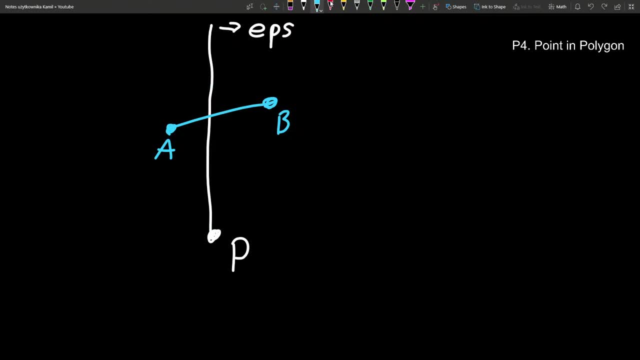 What I do in code is I check if, with respect to P, the cross, or We call it, I think, triangle, Not even that. Sorry, I'm overcomplicating- I check if A dot X is smaller equal than P dot X. 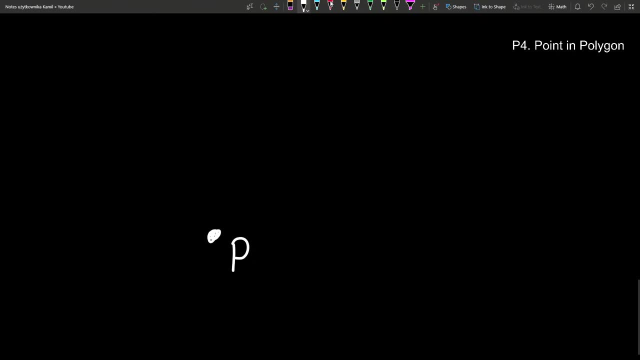 Collinear with anything, Because you don't Need to handle cases like that. If you took this ray, Then We always assume That we move to the left or to the right. We didn't say exactly what happens in this case. 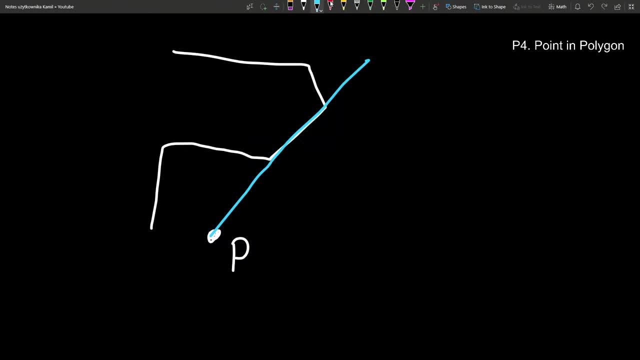 And it's very ugly. You don't want to deal with this case. If your ray contains some segment, That's terrible. I always, And that's in real context, What I do in ICPC When I have such a problem. 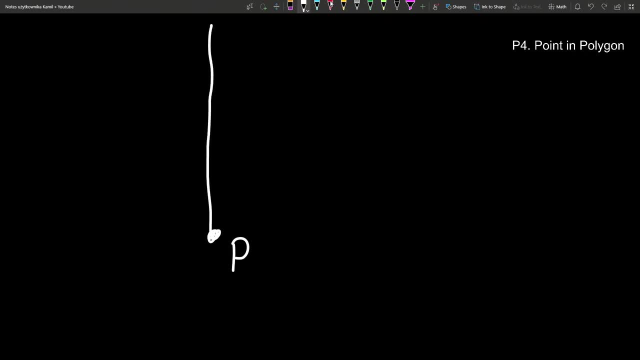 Then I imagine Vertical ray, But actually it's tilted To the right by epsilon And I don't create any point. I just imagine that. Then What happens is, If you For any point When I deal now with some segment, 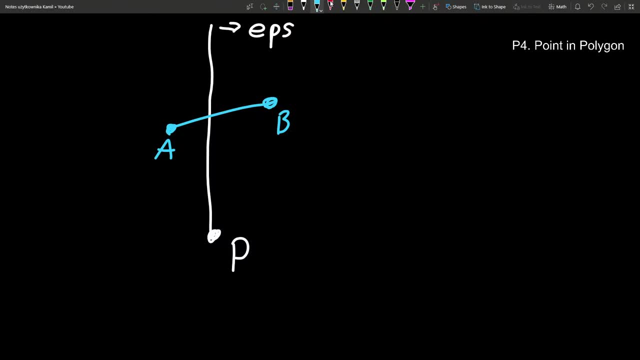 AB For A and B. I need to decide Whether on the left or on the right Of this thing. And I say this: Everything here Including the line Is on the left And Everything excluding the line On the right. 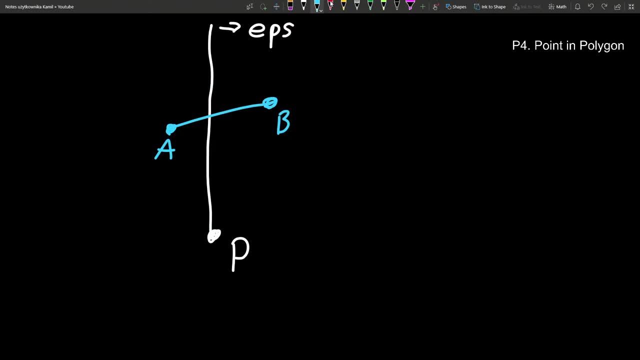 Is on the right. What I do in code Is I check if, With respect to P, The cross Angle- Not even that I'm over complicating- I check if AX Is smaller, equal than PX, Then I say: 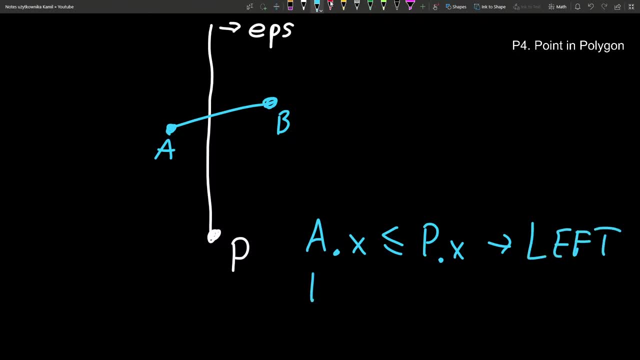 A is on the left. If Same with BX, Then left. If both are true, Left. If both are true, Then the case is like this, And I say no intersection If both are false. So it's like this: 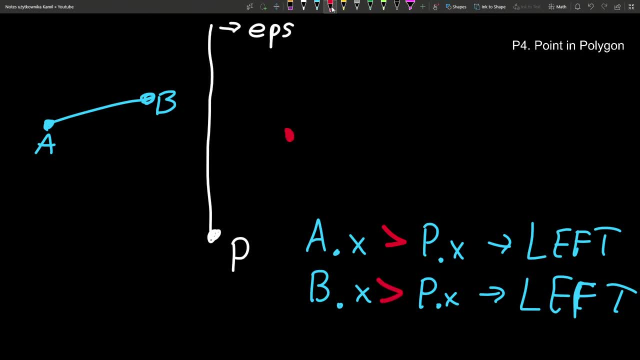 Then both are to the right, Then it's this case. No intersection If they are different, So one is like this And the other like that, Then there might be intersection. So if they gave me different values, So one is greater. 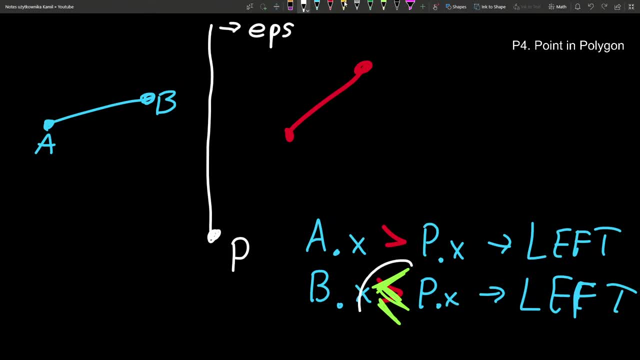 Strictly greater, One is smaller, equal. And I explain to you Why I check with this Inequality. I imagine that this is tilted A little bit to the right. If something is directly above P, It belongs to the left half. 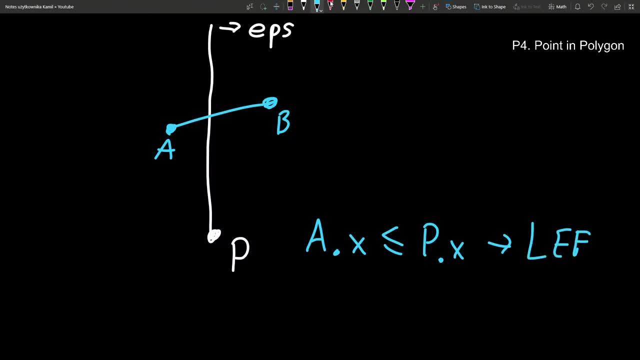 Then I say: A is on the left. If same with B dot X, Then left. If both are true, left. If both are true, Then the case is like this And I say no intersection If both are false. So it's like this: 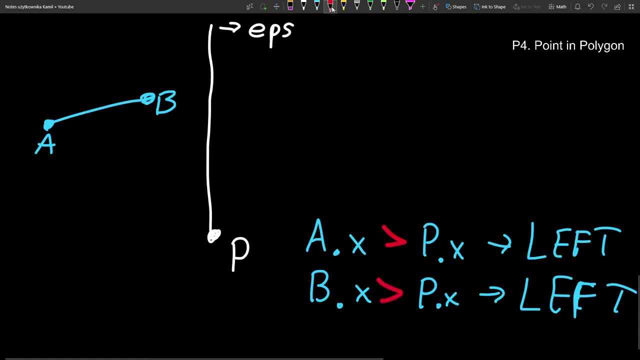 Then both are to the right, Then it's this case. No intersection If they are different, So one is like this and the other like that, Then there might be intersection. So if they gave me different values, So one is greater. 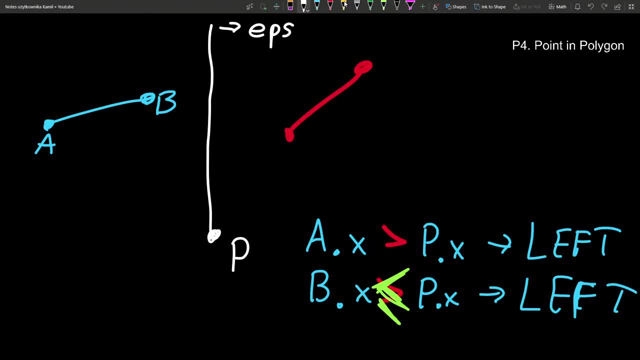 Strictly greater. One is smaller, equal. And I explain to you why I check with this inequality: X smaller than equal. I imagine that this is tilted a little bit to the right. If something is directly above P, it belongs to the left half. 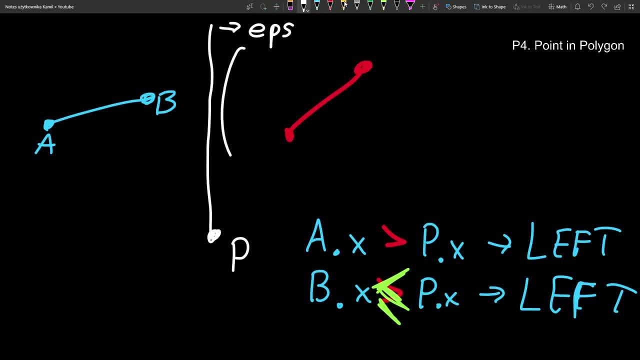 And anything on the Like, with X greater than this is on the right, But this case doesn't necessarily mean intersection. Maybe, For example, this case will indeed have greater and smaller equal. This case, This one Also, something like that. 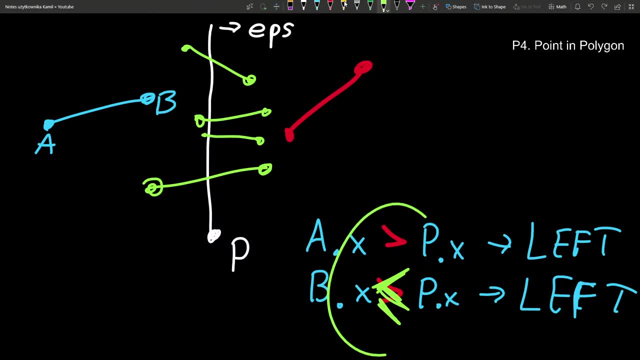 Where this point is exactly above P. But this case would also detect something like that And we don't want it Or this Or that. So we also need to say that this point in this segment is in some way above, And how we do it. 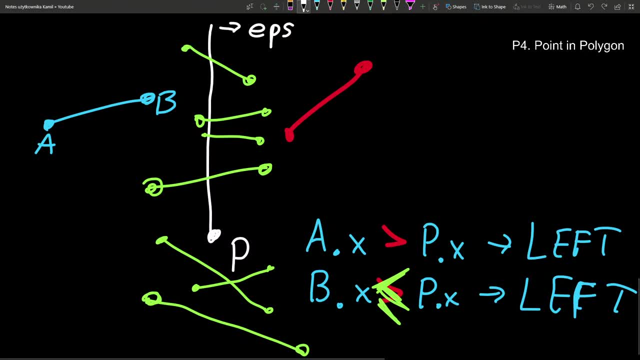 For that we use cross product. If we know this, This means exactly that A is on the right And B is on the left. So I check with respect to P. if B is on the left, I check P dot triangle Of B, comma A. 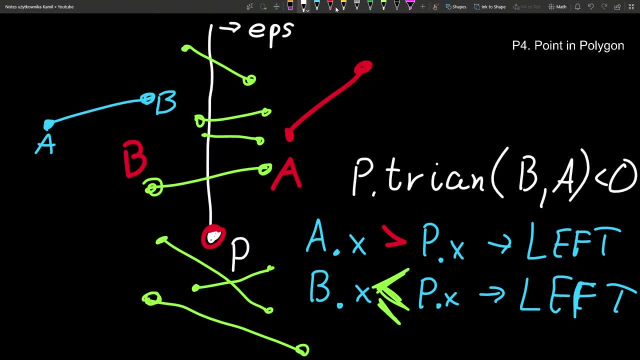 This must be negative. So B must be on the left. That's a case here, Assuming that those are inequalities, So B- The inequalities say that B is X- is on the left. But if you have this thing- B and A- 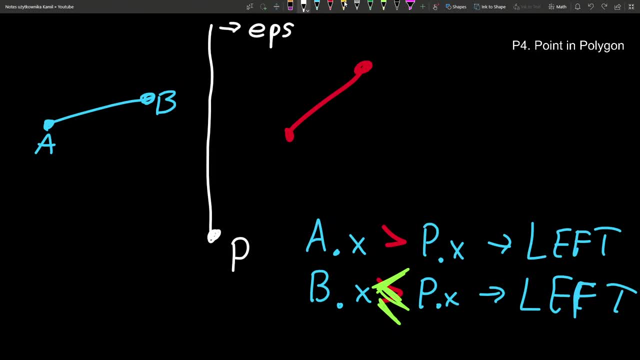 And anything on there, Like with X greater Than this is on the right, But this case doesn't necessarily mean intersection. Maybe, For example, this case Will indeed have greater and smaller equal. This case, This one Also, something like that. 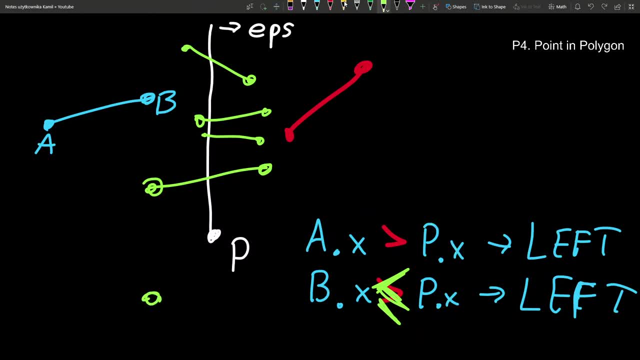 Where this point is exactly above P. But this case would also detect Something like that And we don't want it Or this Or that. So we also need to say That And how we do it. For that we use cross product. 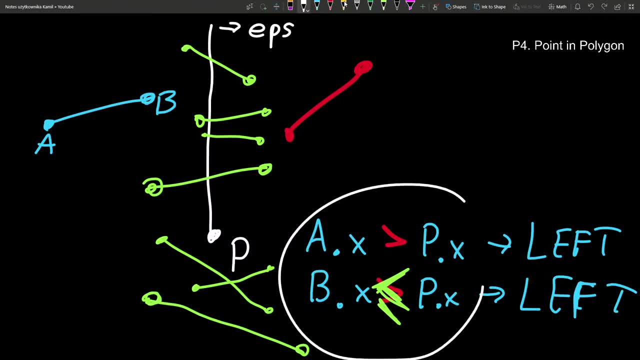 If we know this, This means exactly that A is on the right And B is on the left. So I check with respect to P. If B is on the left, I check P dot. triangle Of B, B comma A. 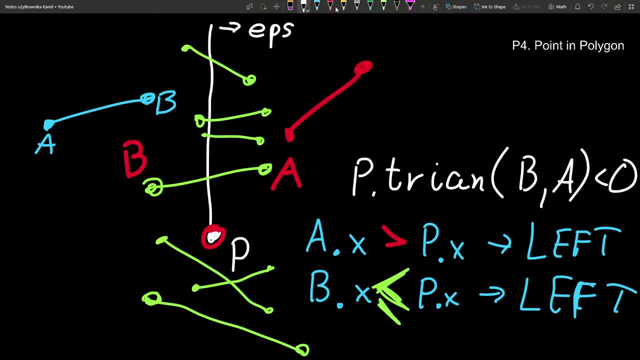 This must be negative. So B must be on the left. That's a case here, Assuming that those are inequalities, So B- The inequalities say that B is X- is on the left. But if you have this B and A, 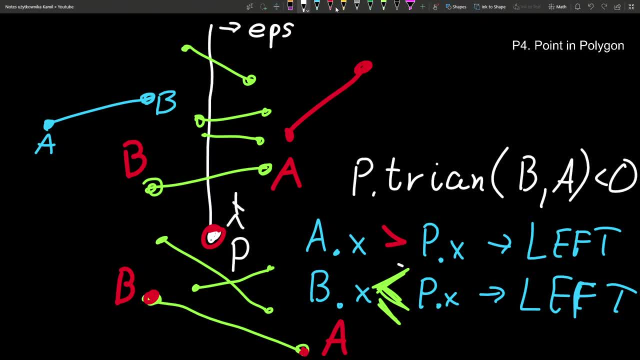 With respect to P. When you are a human standing there, A is on the left. Cross product will give you The other sign here: A is on the left from P Than B. When you are human, When you look in direction of A. 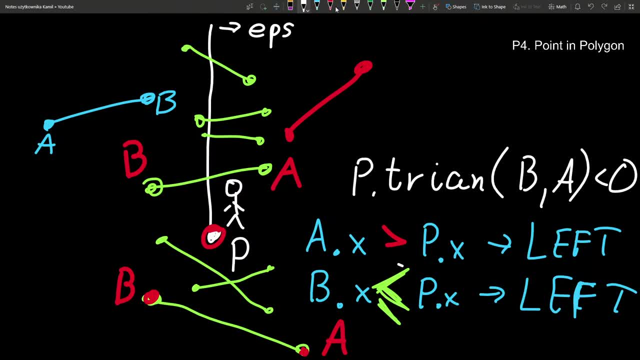 B is on the right, So you need to do this, And this is what I use in contests. I don't create any infinity point. You saw that it's dangerous. I got it wrong. I chose 4 billion and I got overflow. 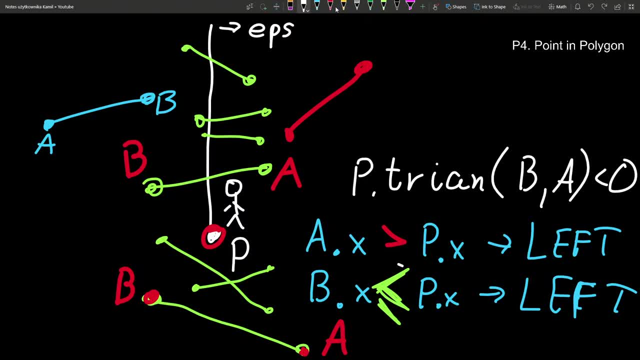 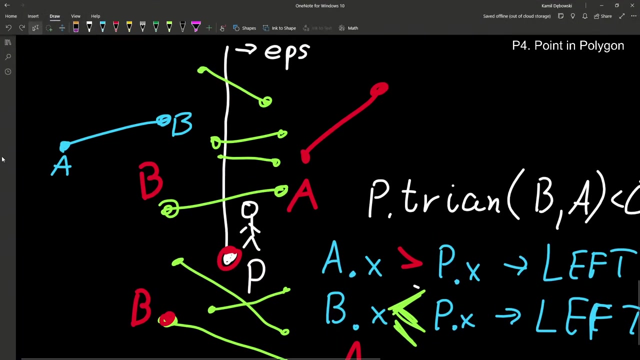 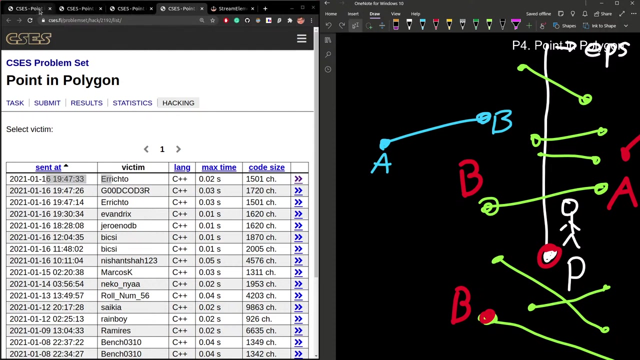 No, This is better. There are a few ifs here, Sure, And then it's always better. Vertical to what There was a question. Vertical just means that It goes straight up. I Can, I guess, Implement this alternative method. 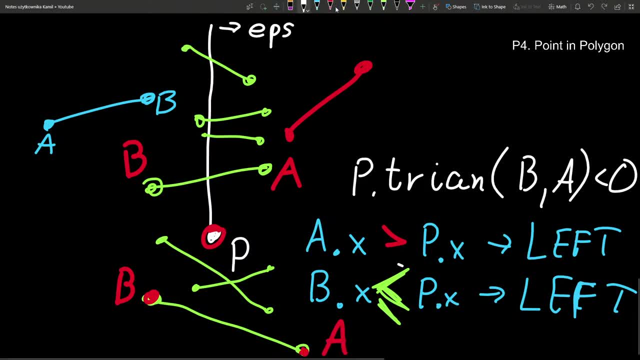 With respect to P. When you're a human standing there, A is on the left. Cross product will give you, Like the other sign here, A is on the left from P Than B When you're human, When you look in direction of A. 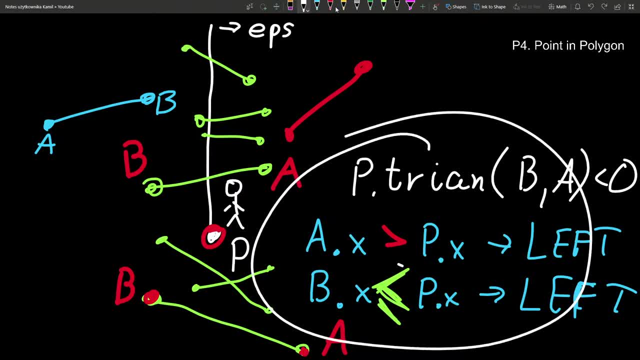 B is on the right, So you need to do this, And this is what I use in contests. I don't create any infinity point. You saw that it's dangerous. I got it wrong. I chose 4 billion and I got overflow. 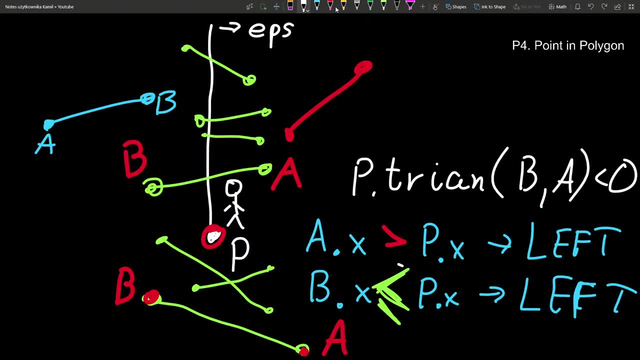 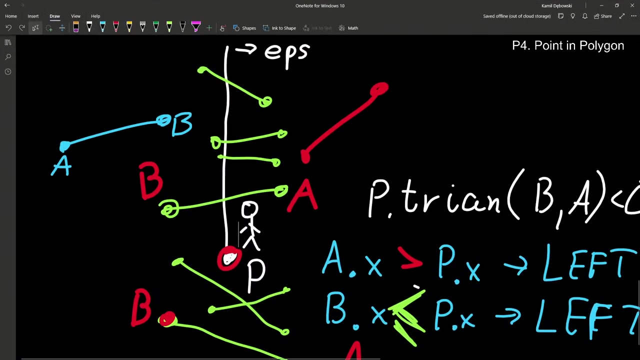 No, This is better. There are a few ifs here, Sure, But you don't have any assumptions about coordinates Thanks to that, And then it's always better. Vertical to what There was a question. Vertical just means that It goes straight up. 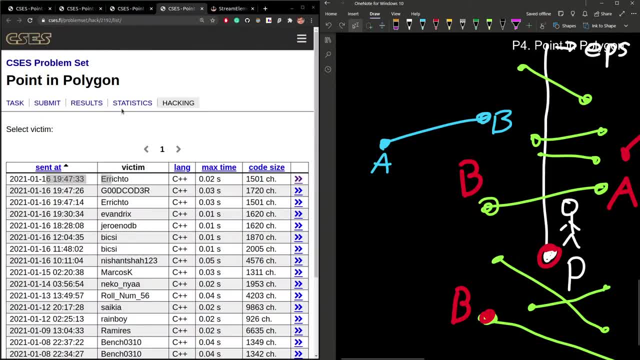 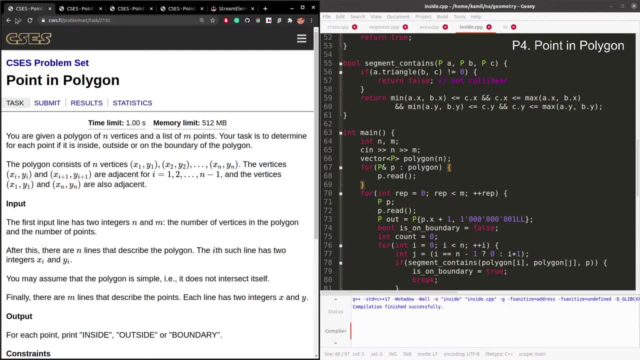 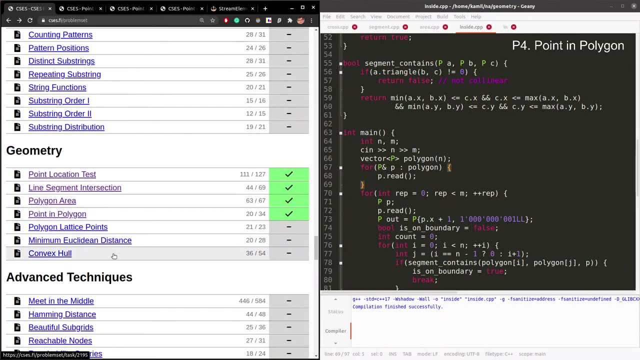 I can, I guess, implement this alternative method, But I need to look at the time And decide if I want to do everything today. Maybe we should do anything other than the sixth problem, Which is, I would say, harder, And it just follows some algorithm. 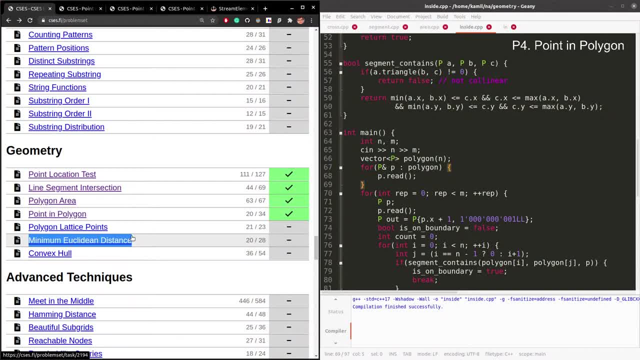 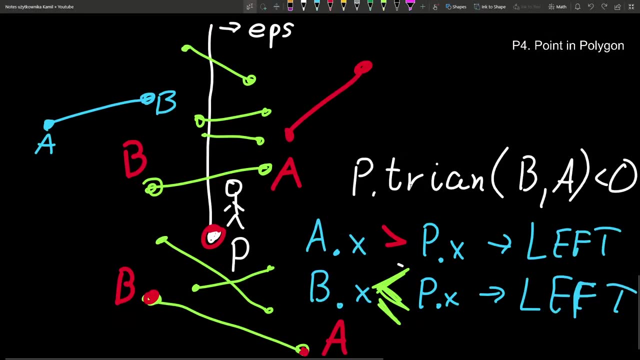 I'm happy with this. I would happy with this decision. I don't want to make a stream that lasts 3 or 4 hours, Because it also will be too much for you. I'd like to watch in one sitting. If you implement this alternative method with my style of code. 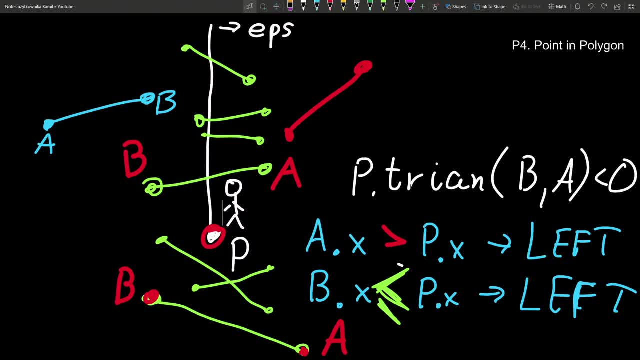 Then put a link to your submission in comments below YouTube And I will pin your comment. We need to check with respect to p, Maybe first With respect to px. We check if every point, Every segment, a, b, If one point is on the left from this vertical ray. 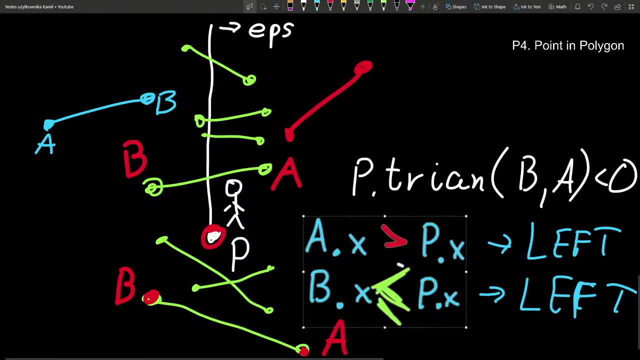 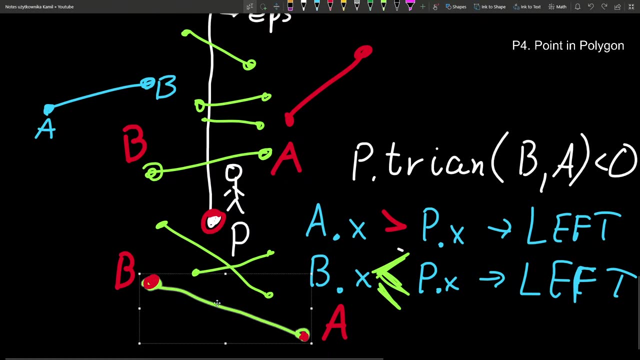 And one is on the right, And we discussed how we decide about ties, How to decide about points being exactly on this ray, Because we imagine that ray is tilted to the right a little bit, And then to avoid those cases, To avoid counting these cases that are below p. 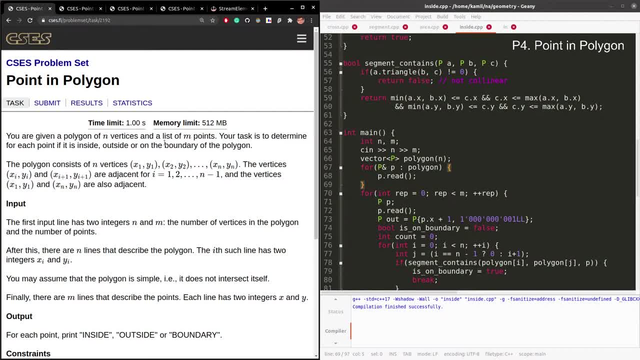 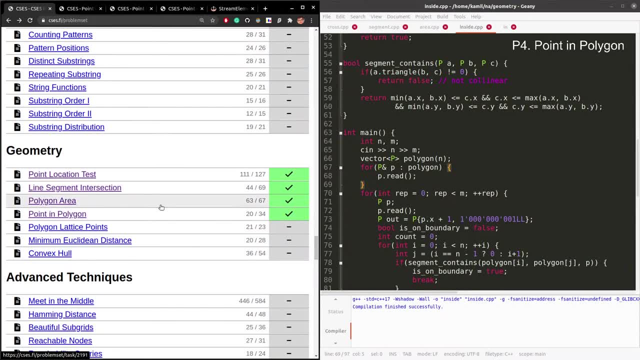 But I need to look at the time And decide if I want to do everything today Or not. Maybe we should do anything Other than the sixth problem, Which is, I would say, harder And it just follows some algorithm. Yeah, 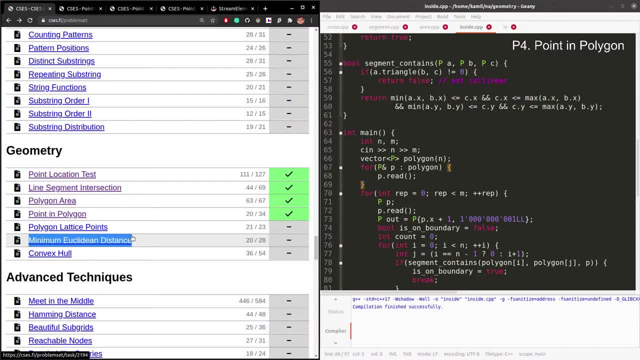 I'm happy with this. I would happy with this decision. I don't want to make a stream That lasts 3 or 4 hours, Because it also will be too much for you. So If you implement this alternative method With my style of code, 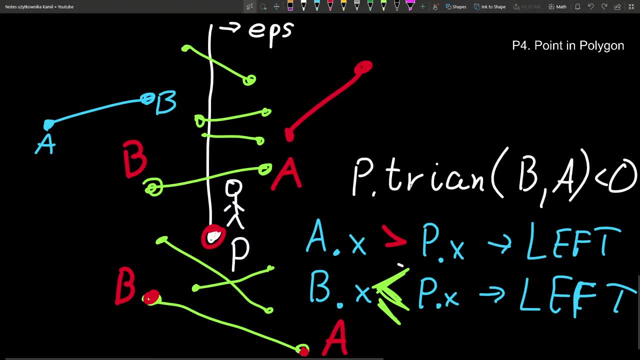 Then Put a link to your submission In comments below YouTube And I will pin your comment Right. We need to check With respect to p, Maybe first With respect to px. We check if every point, Every segment ab. 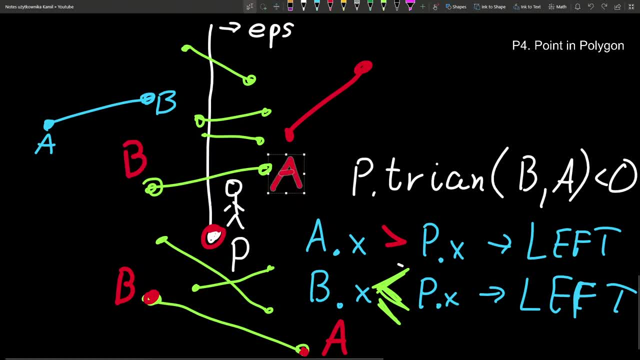 If one point is This vertical ray And one is on the right, And we discussed How we decide about ties, How we decide about points Being exactly on this ray, Because we imagine that ray Is tilted to the right a little bit. 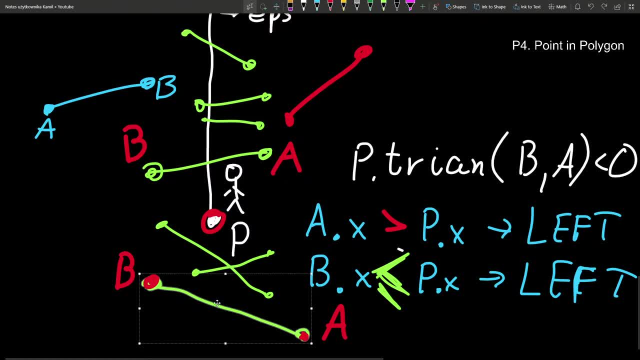 And then to avoid those cases, To avoid counting these cases That are below p On the drawing, We use cross product. YouTube deletes links, sometimes In comments. If it doesn't work, If from incognito, Then you don't see your comments. 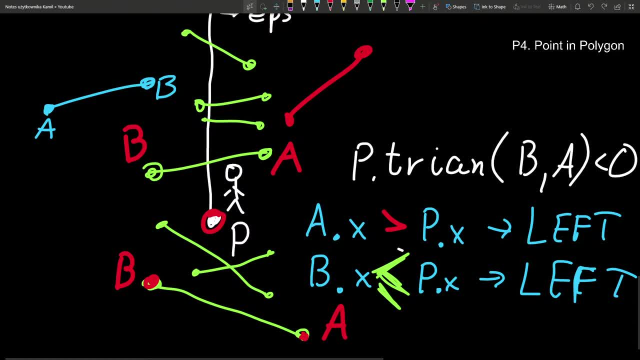 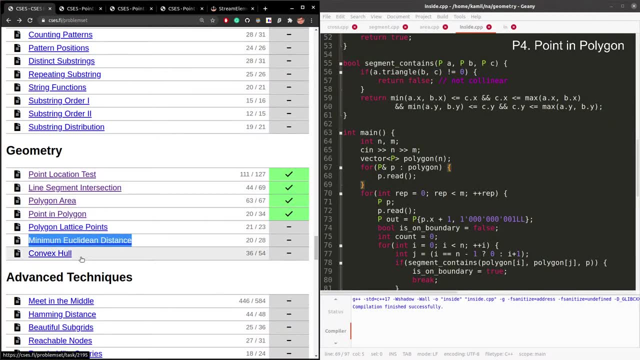 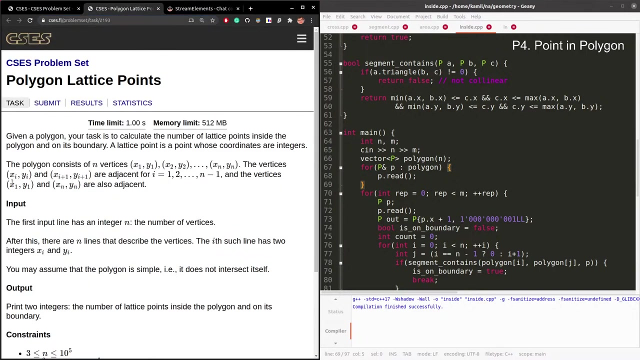 Let me know in private And I will do something about it. Alright, We move on. We will now do polygon lattice points, Then convex hull. We skip minimum euclidean distance For now. For today, Polygon lattice points Isn't an important problem. 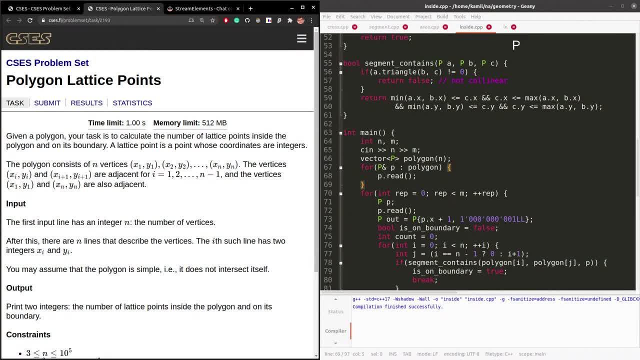 It's just something We need to use: A particular formula That you need to guess. Remember, You need to know it in the first place. Given a polygon, Your task is to calculate the number of lattice points Inside the polygon. 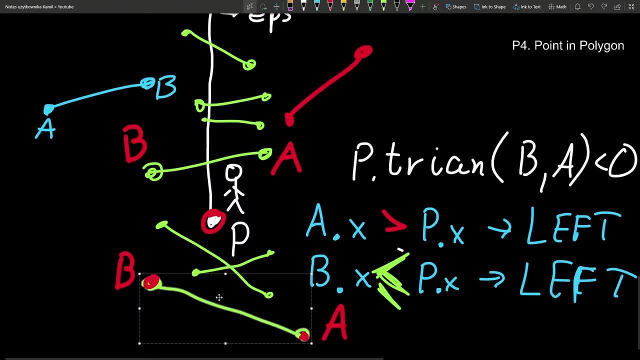 On the drawing. We use cross product. YouTube deletes links, sometimes in comments, But only sometimes. If it doesn't work. If from incognito Then you don't see your comments, Let me know in private And I will do something about it. 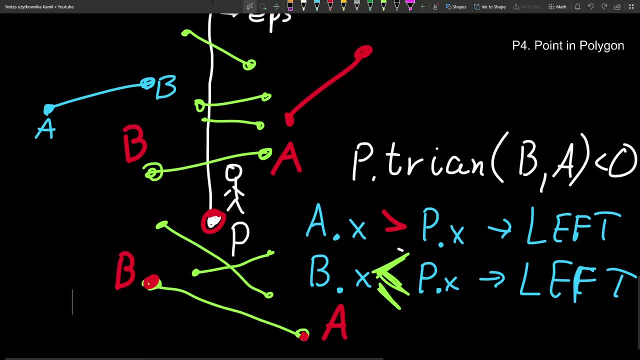 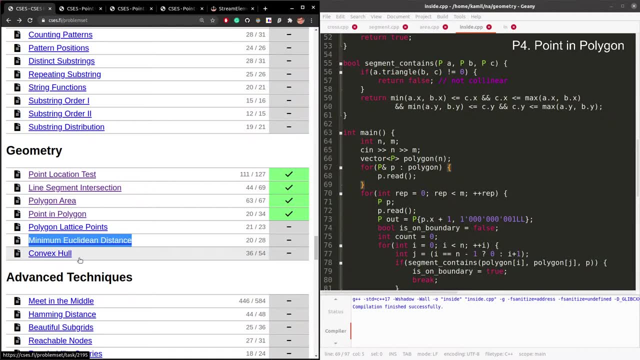 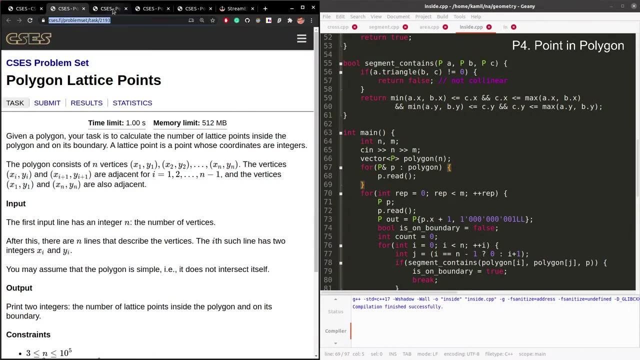 All right, We move on. We will now do polygon lattice points, Then convex hull. We skip minimum Euclidean distance for now, For today. We move on. We will now do polygon lattice points, Polygon lattice points. Polygon lattice points isn't an important problem. 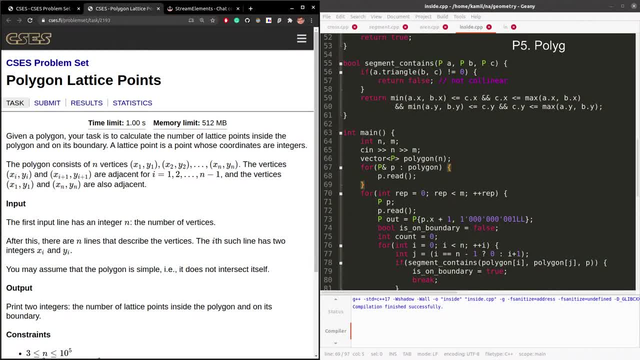 It's just something We need to use, a particular formula That you need to guess. Remember, You need to know it in the first place. Given a polygon, There are a number of lattice points Inside the polygon And on its boundary. 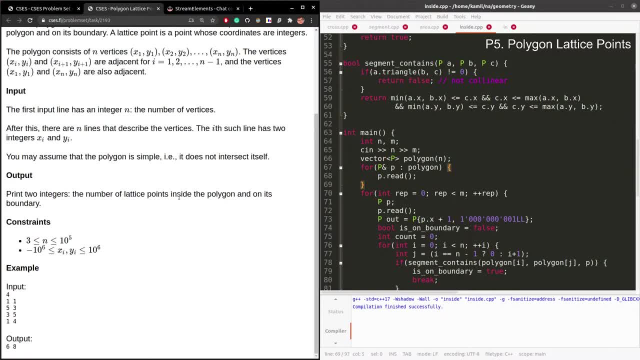 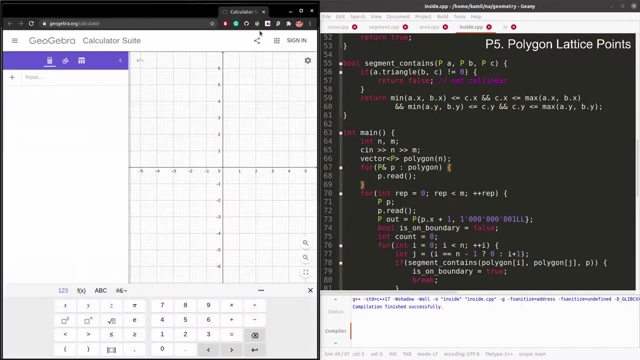 Lattice point is a point Whose coordinates are integers. I would appreciate an example here With drawing. But let's actually draw this And we use Actually. Will this have Lattice points marked? Yes, it will have. Let's try to plug this. 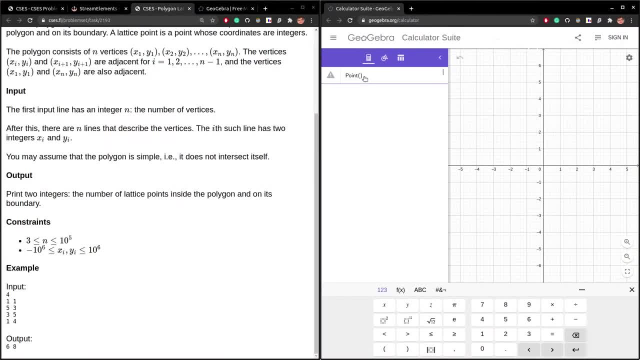 Here, Point one one. No, That didn't work. If you know how to use this, Please let me know. Alright, I see now. P1 is one one. P2 is five, three, Five. This is, I don't know how to pronounce it. 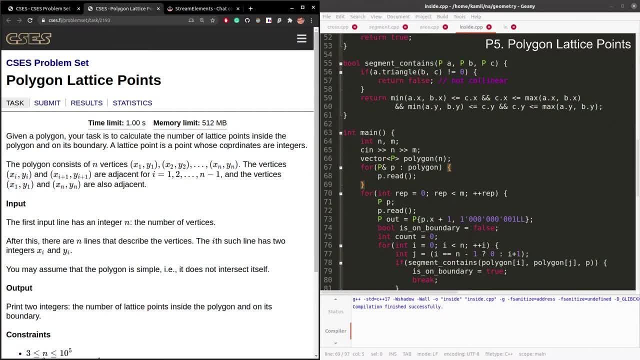 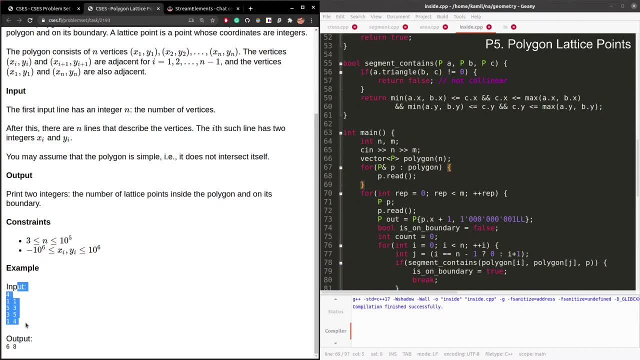 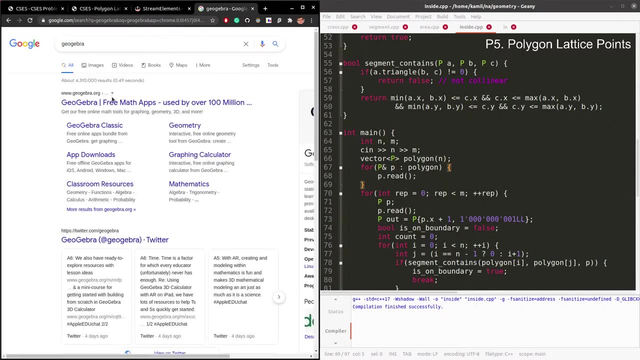 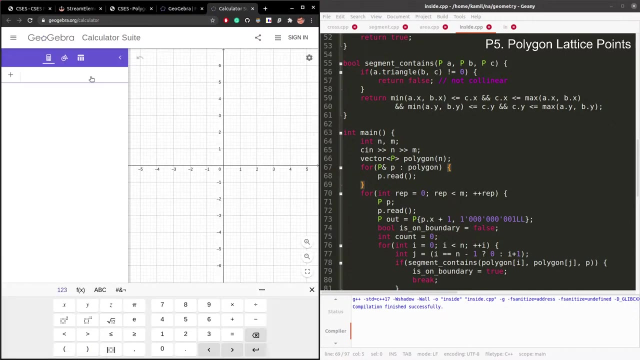 And on its boundary, The number of integers. I would appreciate An example here With drawing. But let's actually draw this And we use Actually. Will this have lattice points marked? Yes, It will have. Let's try to plug this here. 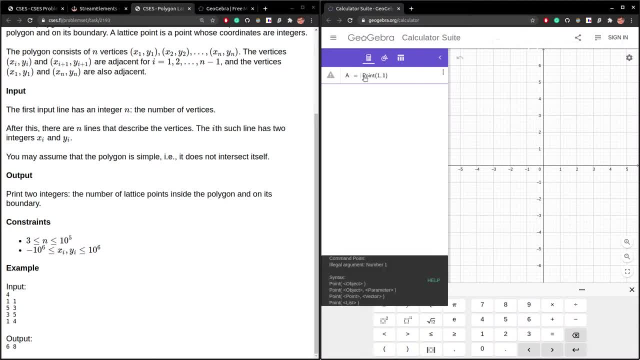 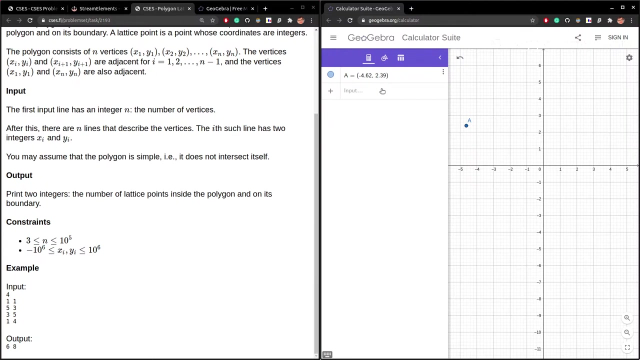 Point one one. No, That didn't work. If you know how to use this, Please let me know. Alright, I see now. P1 is one, one, P2.. P2 is Five, three, Five. This is: 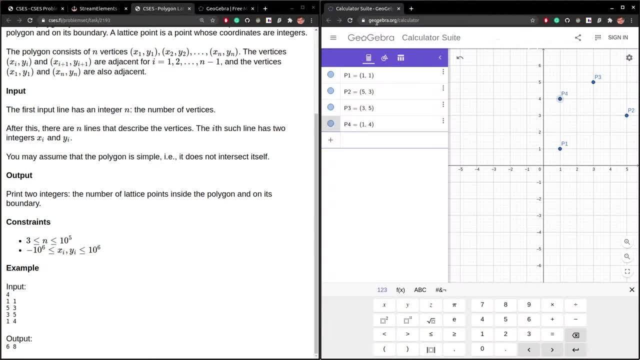 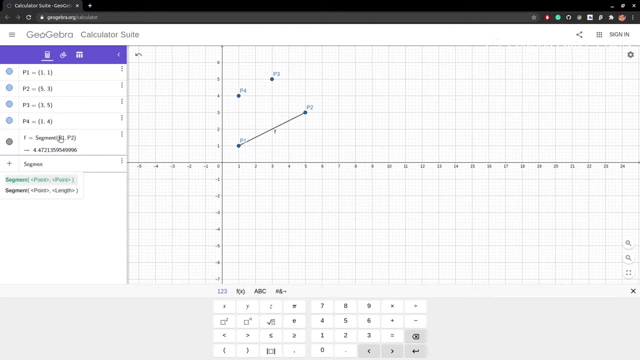 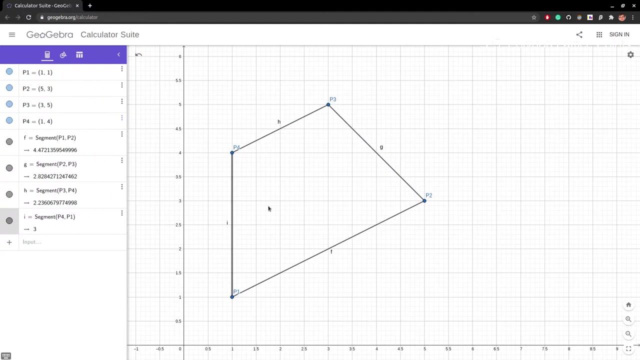 Geo- I don't know how to pronounce it- GeoGebra, GeoGebraorg. A useful tool. I didn't use it for some time. Now I want Segment Windows. Nice, This is the input. And now? 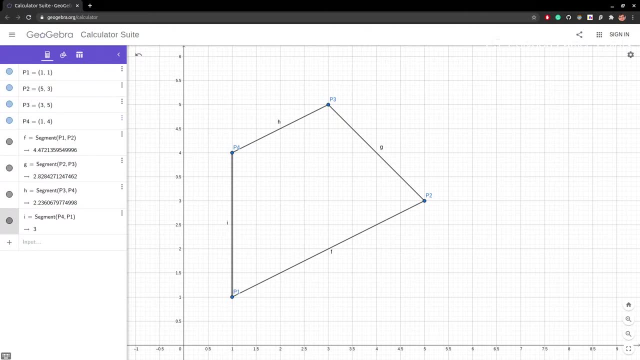 We need to count Points inside With integer coordinates And points on the boundary. On the boundary We have one, Two, Three. I think we don't. We shouldn't count vertices, Points that belong to a segment But not here. 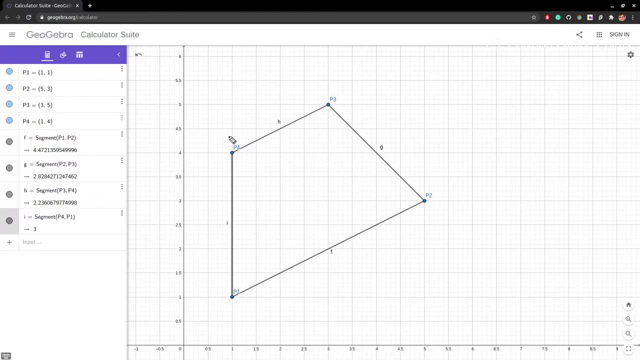 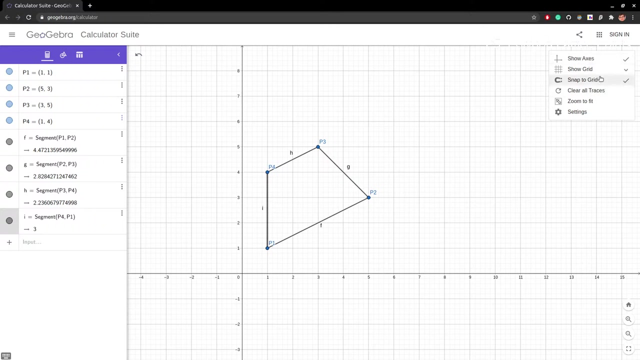 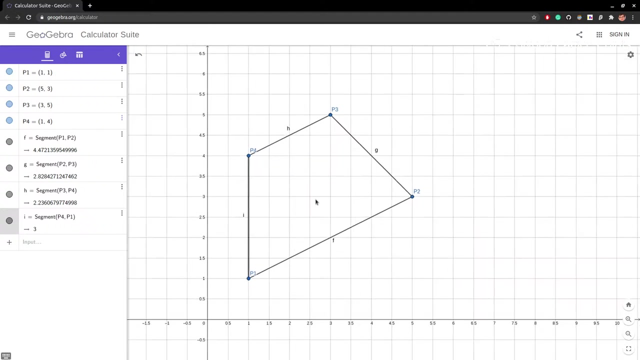 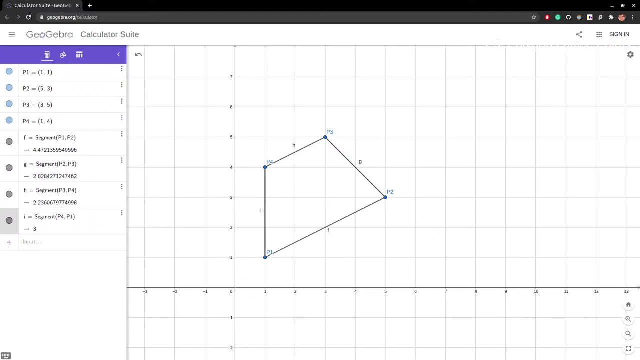 And they have integer coordinates. Also, this is 4.5, which is confusing. That's bad. That's bad. Can I Here hide? Show grid, No grid. Great, This will be much better. One, Two, Three. 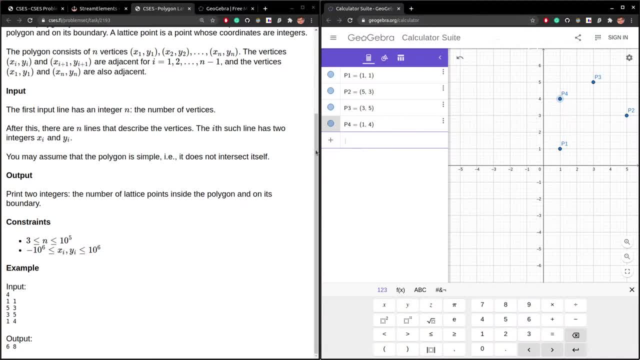 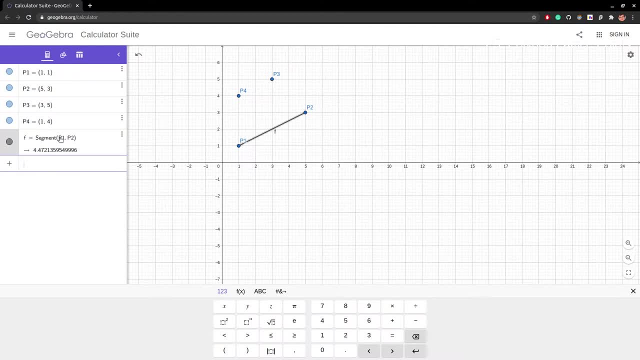 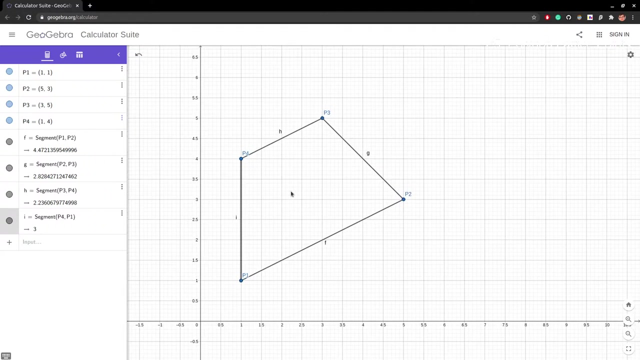 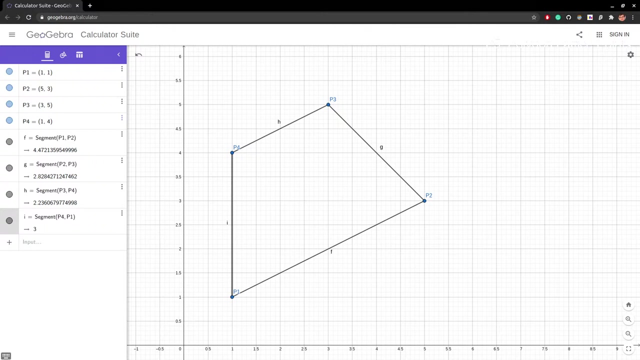 GeoGebraorg, A useful tool. I didn't use it for some time. Now I want To implement Windows. Nice, This is the input, And now We need to count Points inside With integer coordinates And points on the boundary. 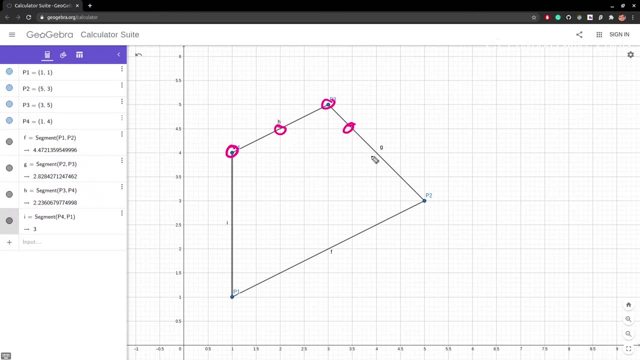 We have one, Two, Three, Four, Five, Six, Seven. I think we don't, We shouldn't count vertices, Points that belong to a segment But not here, And they have integer coordinates. Also, this is four, point five. 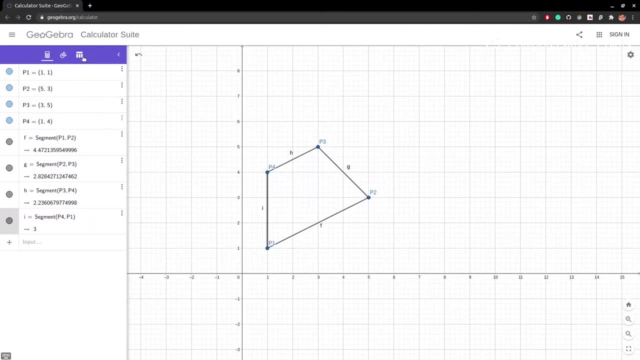 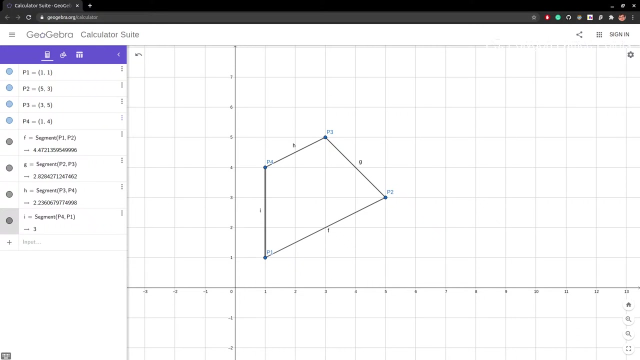 Which is confusing. I have here Hide, Show, grid, No grid, Major lines- Great, This will be much better. One, Two, Three, Four, Five, Six And six points Inside. Tell me if this is not the answer. 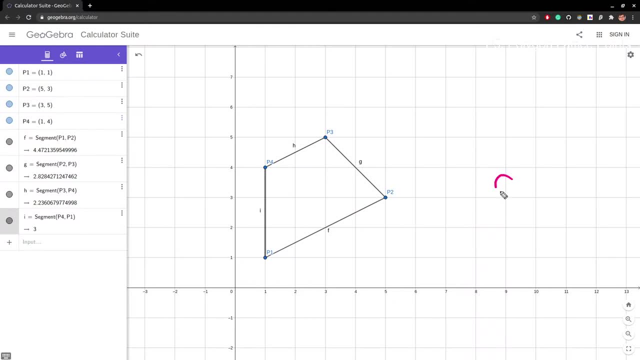 I don't want to switch windows Right. How to compute this? Focusing on the boundary Is easier If we have a vertical segment. That's just some simple math, Not related even to cross product or anything Where Like in this. 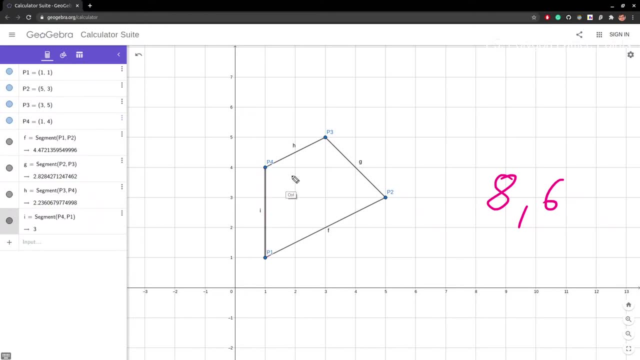 If we have a vertical segment, Then you know Its length corresponds to the number of points here. If you have something tilted like that, Then This is a case where we have in the middle Point that has integer coordinates. It is related to the fact that 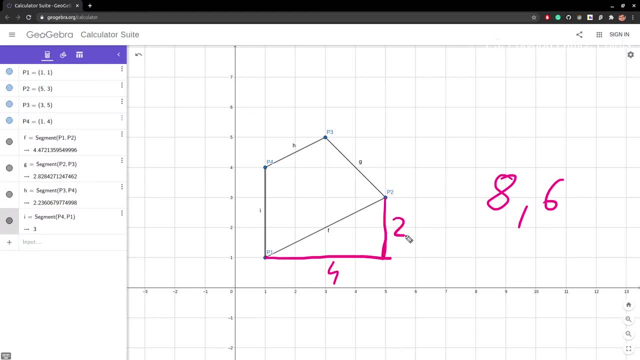 Width and height here The distance in terms of x and y. They are not co-prime, Both are divisible by two. So there is something exactly in the middle. If I move from a point To a point here, To the right, by six. 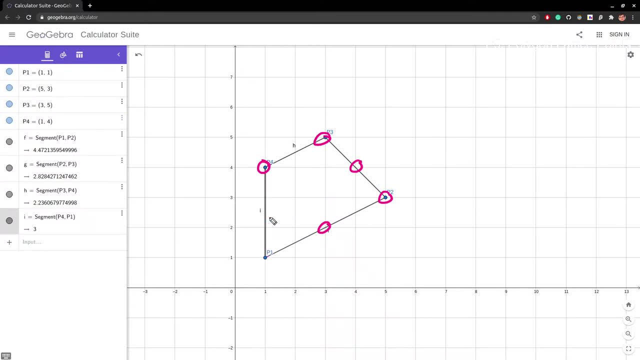 Four Five, Six, Seven, Eight, Four Five, Six And six points inside. Tell me if this is not the answer. I don't want to switch windows Right. How to compute this? Focusing on the boundary is easier. 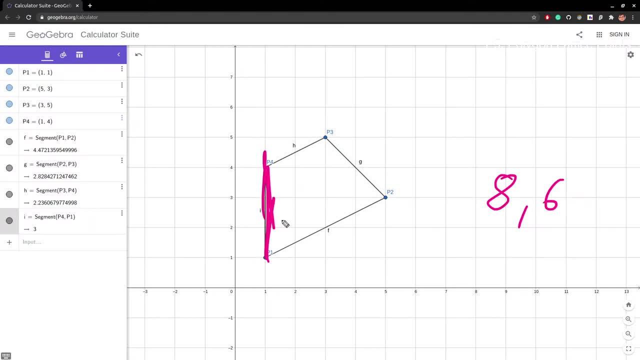 Because when you look at segment- That's just some simple math, Not related even to cross product or anything Where Like in this- Then you know Its length Corresponds to the number of points here. If you have something tilted like that, 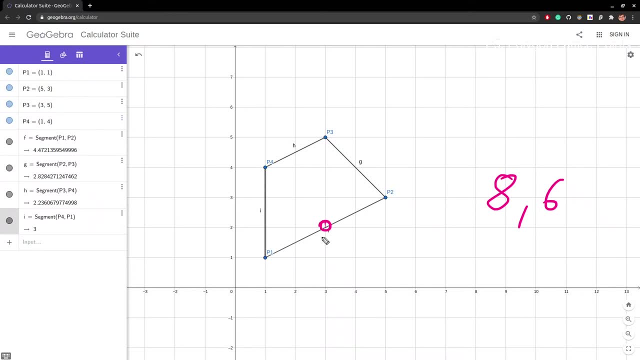 Then This is a case where we have in the middle Point that has integer coordinates. It is related to the fact that Width and height, here The distance in terms of x and y, They are not co-prime, Both are divisible by two. 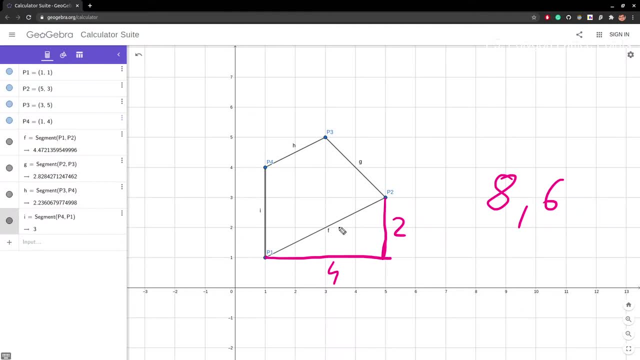 So there is something exactly in the middle. If I move from a point To a point here, To the right, by six, This is plus six Plus three. When compared to this first point, Every third of a way I will have an integer point. 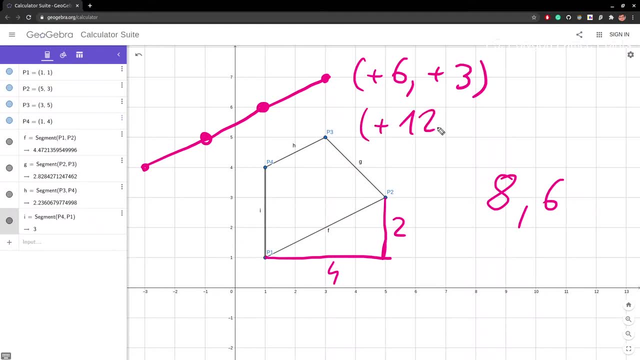 The same will happen if you have Plus twelve And plus eight. Then, Because this vector of transition Is divisible by this Four plus Plus three, comma plus two, So from the first point You can make those small jumps By plus three and plus two. 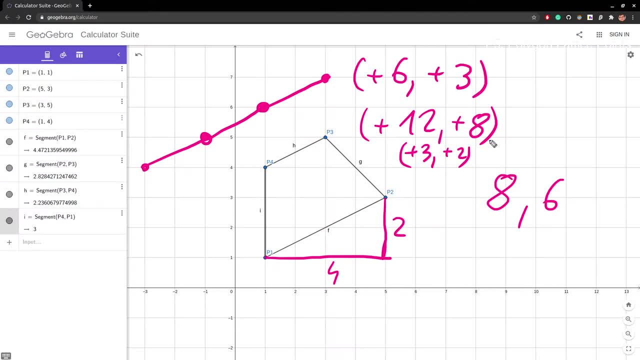 And you will eventually get there After four such jumps. So I claim that here. This splits into four segments Like that. So it will have. It will be like this: One segment, second, third and fourth. This says what happens If the distance between 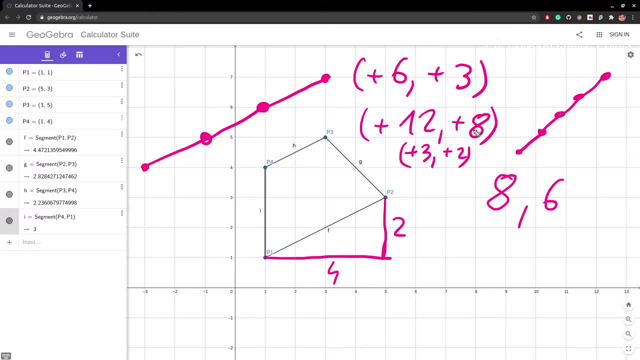 The next points. In our polygon, The distance is plus twelve And plus eight. We are doing some geometry today And how to compute this? By what we can divide a vector. To get this smaller vector We can use greatest common divisor. 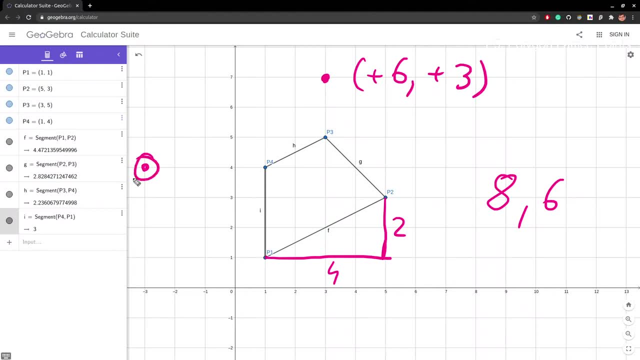 This is plus six, Plus three. When compared to this first point, Every third of a way I will have an integer point. The same will happen If you have plus twelve And plus eight, Then Because this Vector of transition, 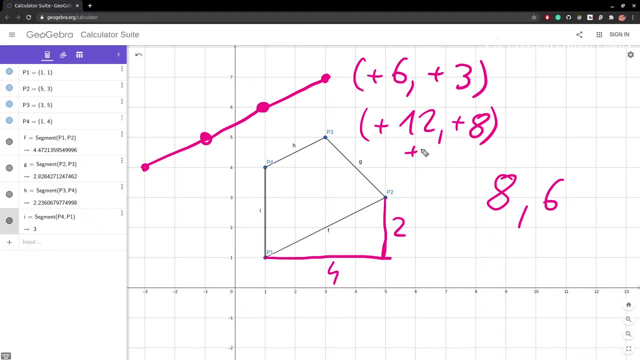 Is divisible by this: Plus four, plus Plus three, comma plus two. So from the first point You can make those small jumps By plus three and plus two And you will eventually get there After four such jumps. So I claim that here. 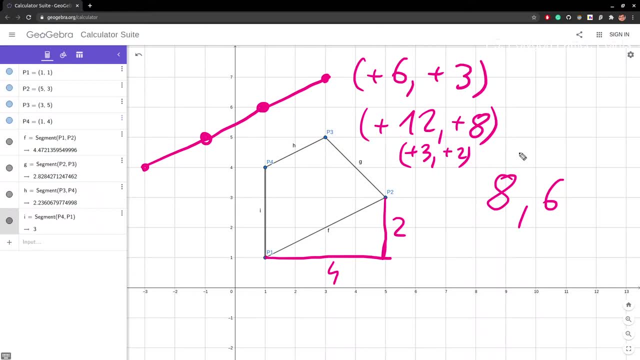 This splits into four segments like that, So it will have. It will be like this: Second, Third And fourth. This says what happens If the distance between two next points In our polygon, The distance, is plus twelve And plus eight. 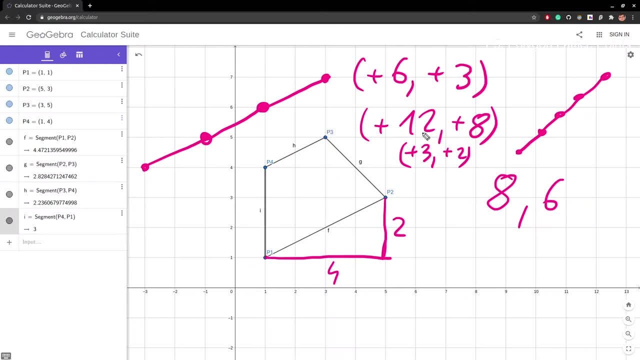 We are doing some geometry today And how to compute this. By what we can divide a vector To get this smaller vector, We can use greatest common divisor, In this case, When you have transitioned From one point to the next one. 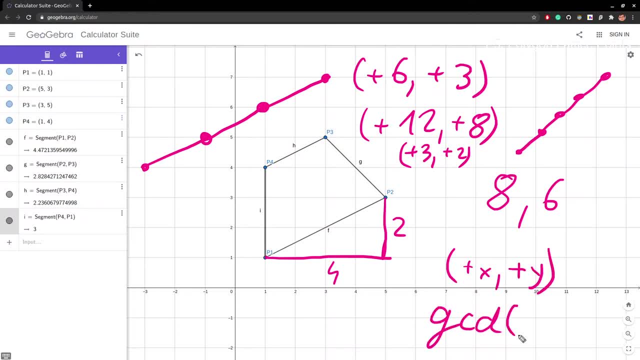 By plus x, plus y. Then you need to compute gcd of x and y. This will tell you By how much you can divide this To get smaller integer vectors Like this. Here we have six and three gcd of, that is three. 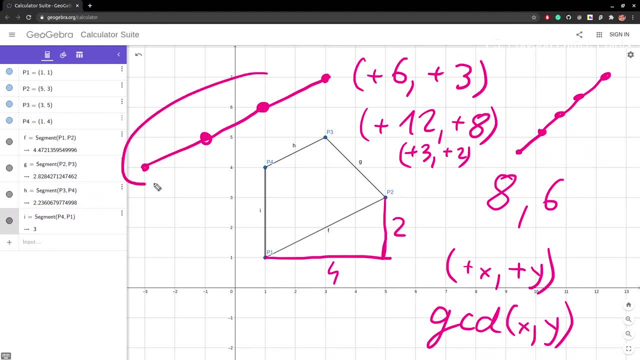 So Vector plus six plus three Splits into three Equal vectors, Smaller vectors With integer coordinates. So three separate jumps, So four points in total. But if you don't want to Double count Here you had some segment. 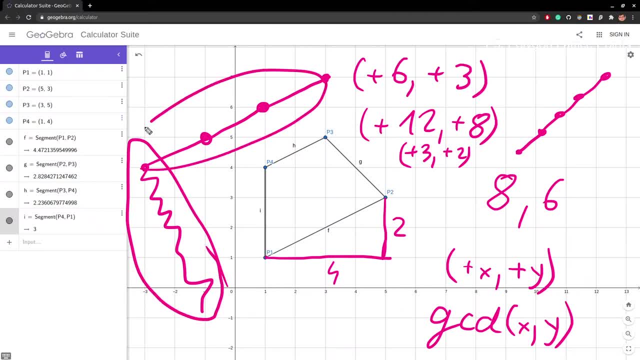 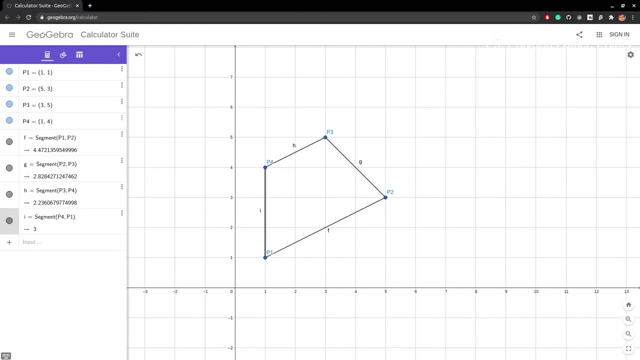 You already counted its points. Then here, When you see three segments, You just add three. Because you see three new points, You compute those. Now Let's use all of that To get the answer For this sample test. Let's say we start here. 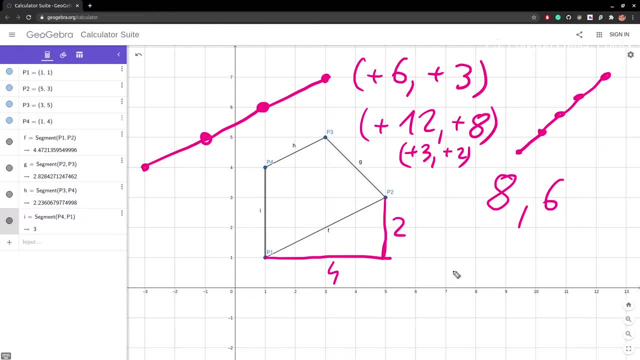 Of twelve and eight, in this case, When you have Transition from one point to the next one By plus x To y, Then you need to compute gcd of x and y. This will tell you By how much you can divide this. 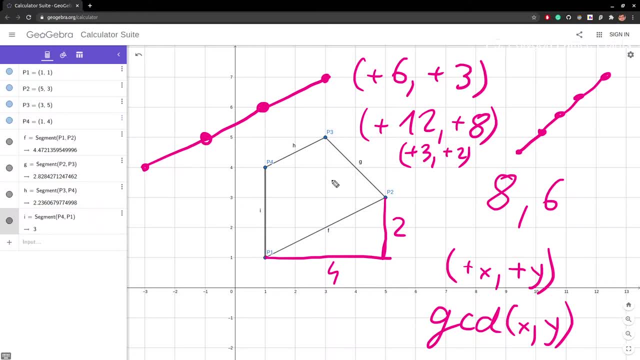 To get smaller integer vectors Like this: Here we have six and three Gcd of that is three. So vector Plus six plus three Splits into three Equal vectors, Smaller vectors with integer coordinates, So three separate jumps. 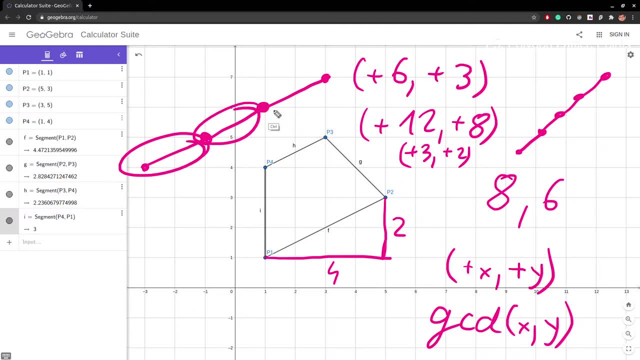 So four points in total. But if you don't want to Double count- And here you had some segment, You already Counted its points- Then here, when you see three segments, You just add three, Because you see three new points. 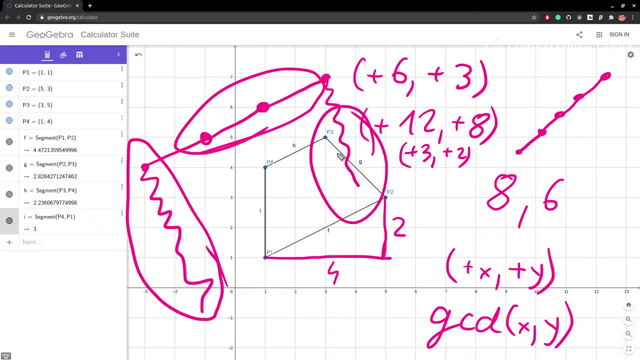 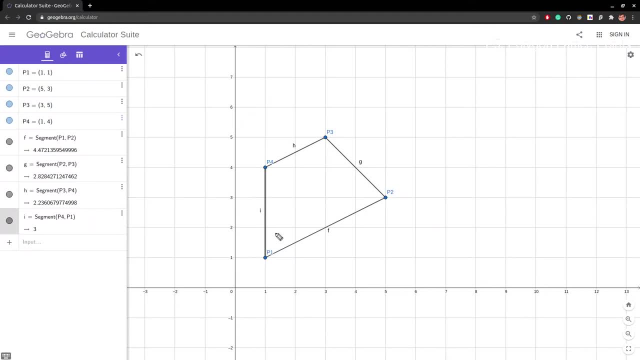 You compute those. Then here you have some other segment. You compute those. Now let's use all of that To get the answer. Let's say we start here In p1.. When we look at this We see Plus zero, plus three. 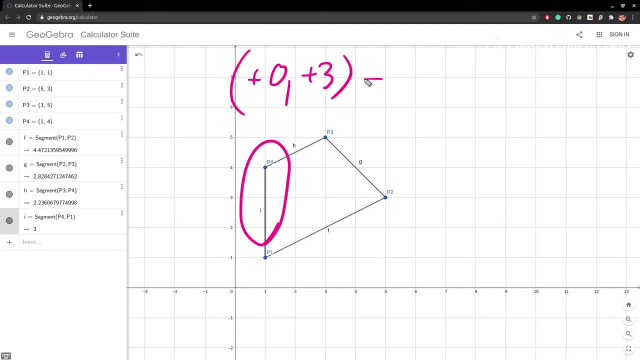 That's vector of transition from p1 to p4.. Gcd of that is three. This is Greatest divisor of both zero and three. So I add this to the answer. Then we have here Plus two x and plus one y. 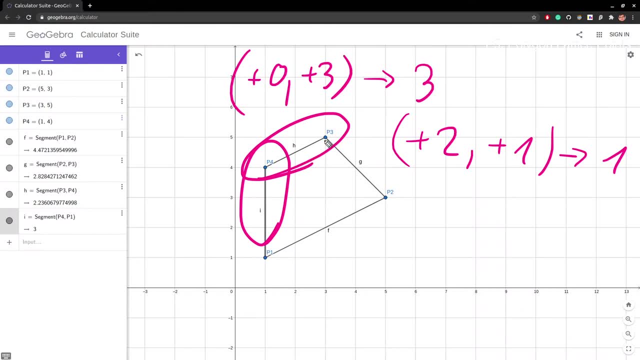 Gcd of that is one. We have a single segment in itself And we have one new point. For now I counted One, two, three points, Then one point. What do we have here? Plus two x, Minus two y. 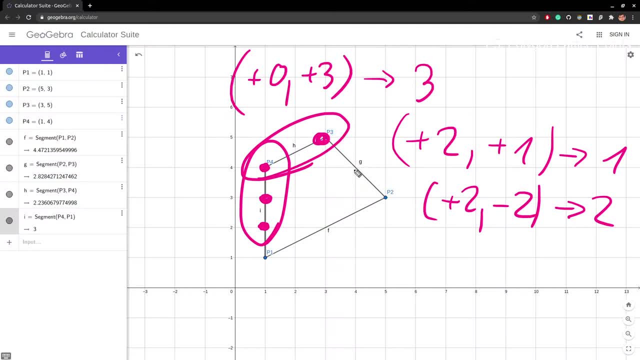 The gcd is two. This splits into two Consists of two segments. I counted this way: those two And finally this last vector, This last transition, Is minus four, minus two. This is divisor of both four and two. We don't care about negative or positive. 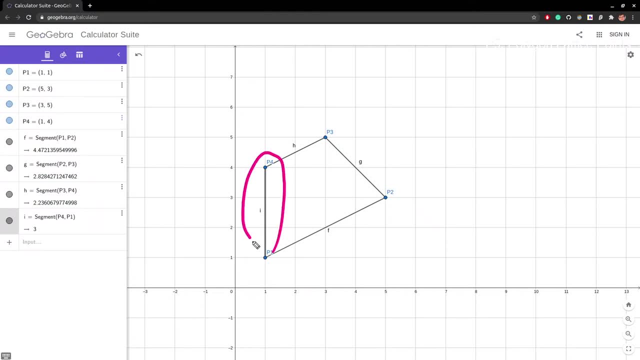 In p1. When we look at this We see Plus zero plus three. That's vector of transition From p1 to p4. gcd of that is three. This is greatest divisor Of both zero and three. So Then we have here: 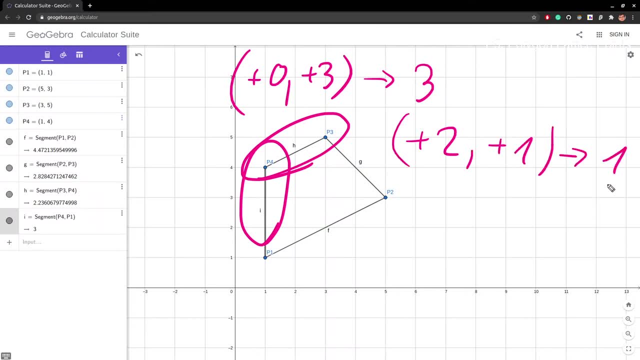 Plus two x and plus one y gcd. if that is one. This is a single segment in itself And we have one new point. For now, I counted One, two, three points, Then one point. What do we have here? Plus two x. 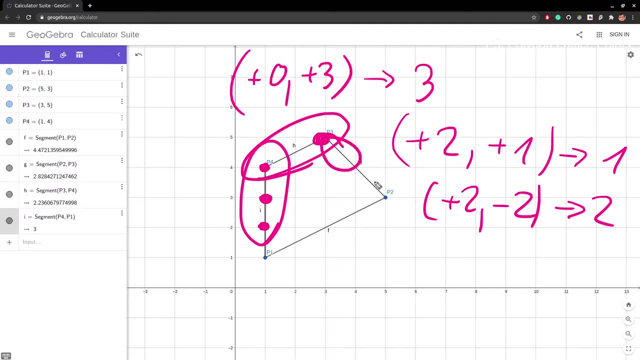 Minus two y, The gcd is two. This splits into two, Consists of two segments, Integer segments And finally, this last vector, This last transition, Is minus four minus two gcd, That's greatest divisor of both four and two. 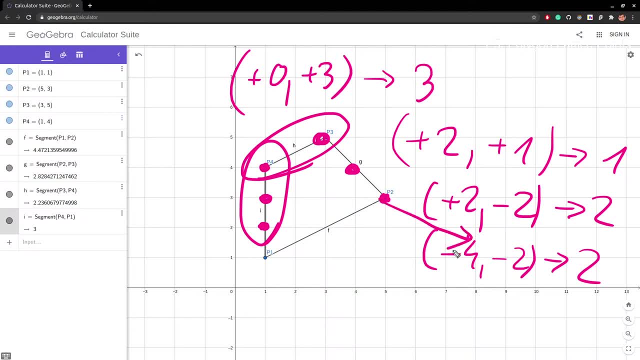 We don't care about Negative, positive If you go to the left versus If you go to the right. There needs to be the same number of points. Those two points are this one And this one. The answer: Three plus one plus two plus two. 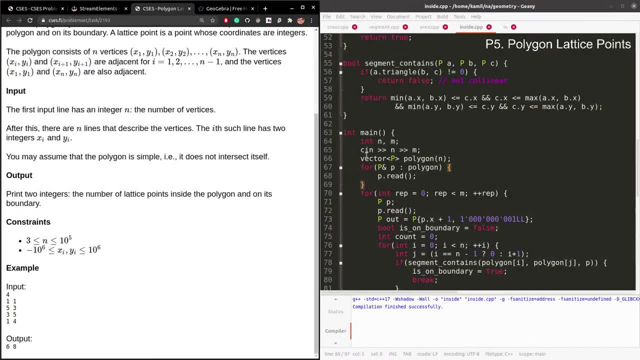 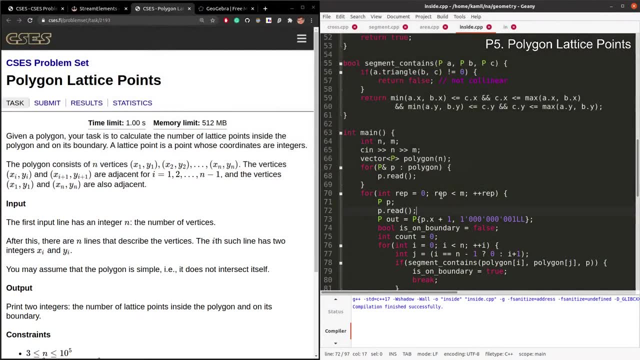 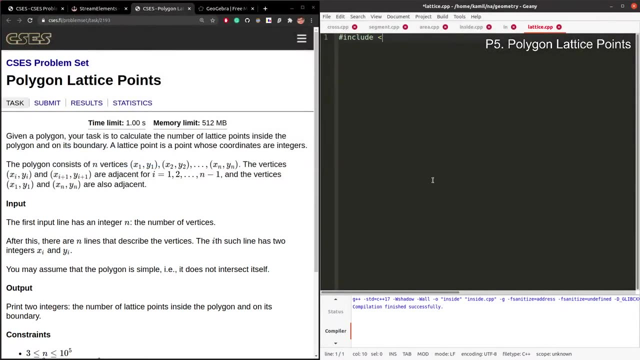 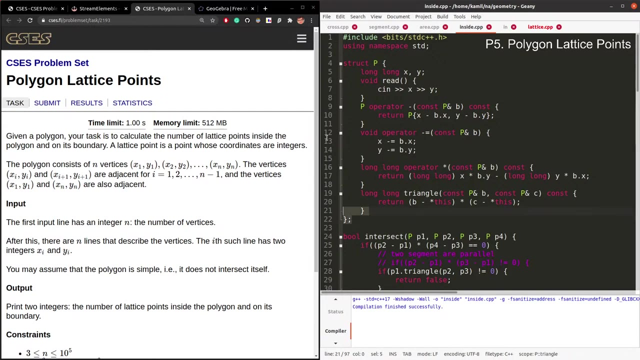 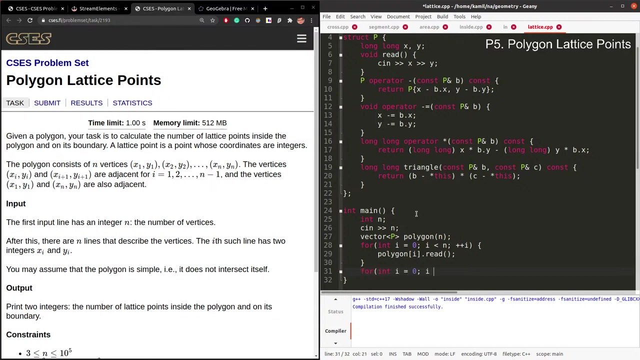 That's eight. And then talk about The full problem: How to count points inside Lattice. We can still Copy paste this. We read the polygon Of size n, Read all the points And For every segment, For every i. 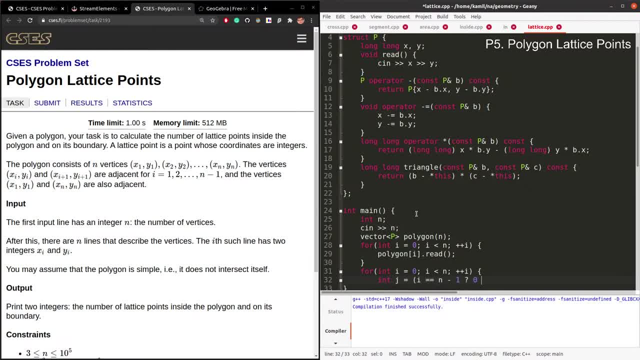 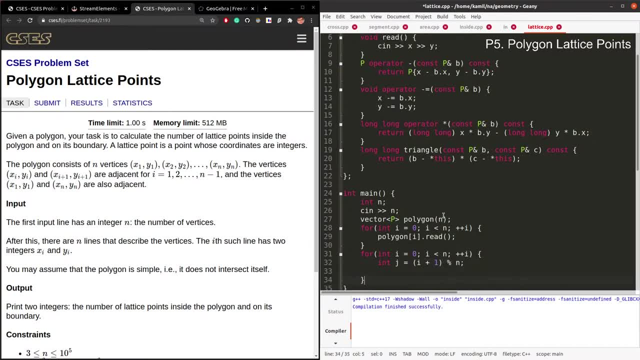 Look at j Being the next point, It's i plus one Modulo n. Let's actually use the third version. This is the index of the next point And You look at delta x Being polygon of j Minus polygon of i. 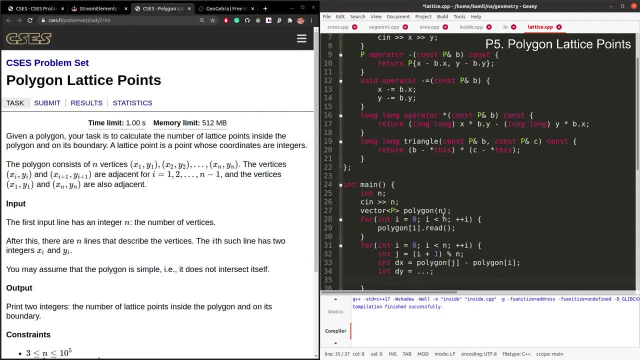 And delta y is the same for y's. Why should I implement, Why should I type this, When I can just say Difference, Like the vector of transition, is Polygon of j minus polygon of i, This already Delta x and delta y? 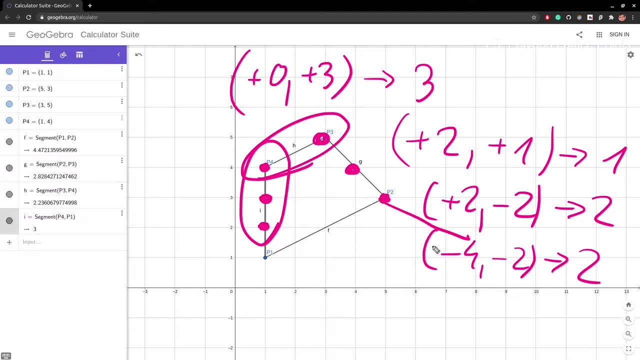 If you go to the left Versus if you go to the right, There needs to be the same number of points. Those two points are this one And this one The answer. Three plus one plus two plus two, That's eight. 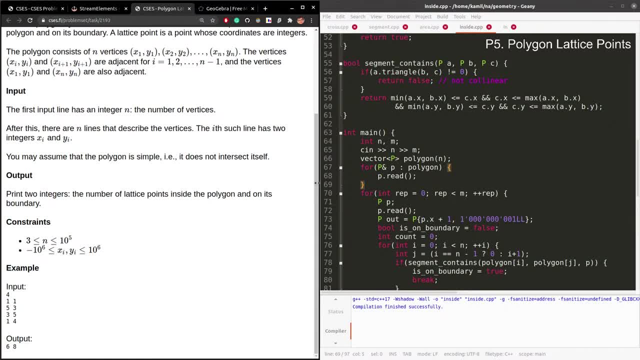 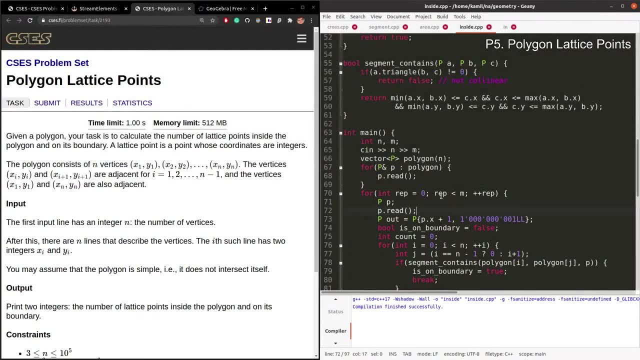 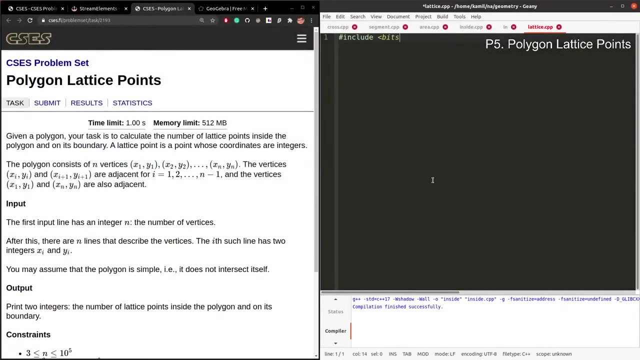 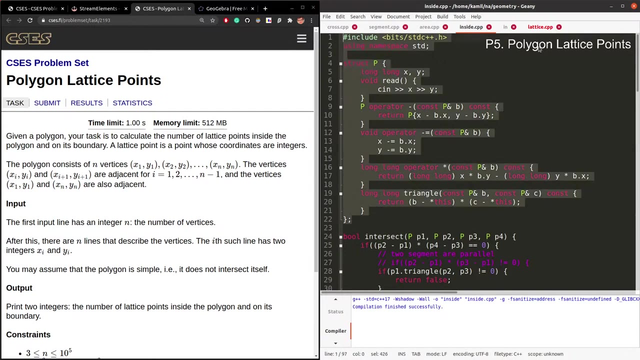 Let's implement it And then talk about The full problem: How to count points inside. Let's try. I'm going to install Lattice. We can still Copy paste this. We read The polygon: Obsize n. 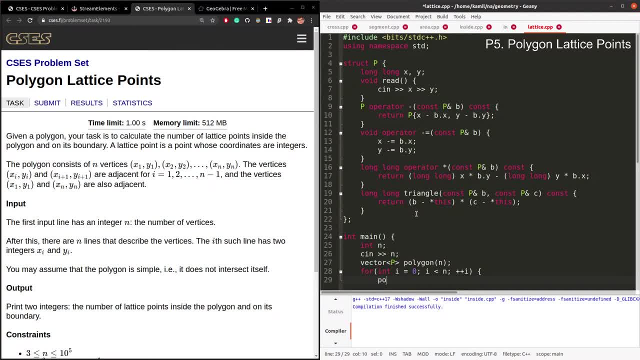 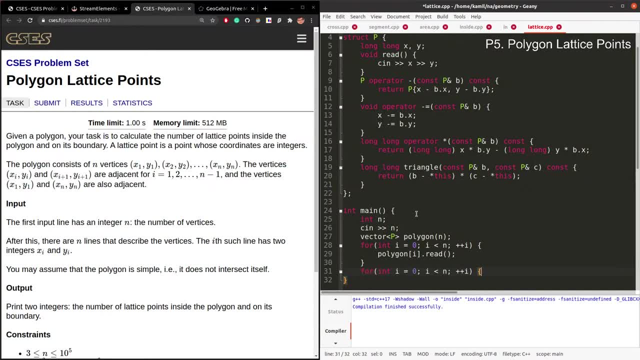 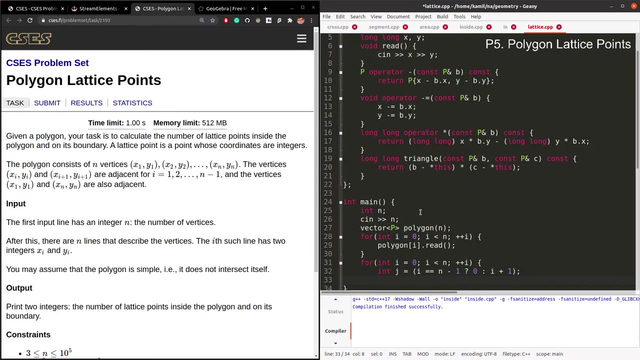 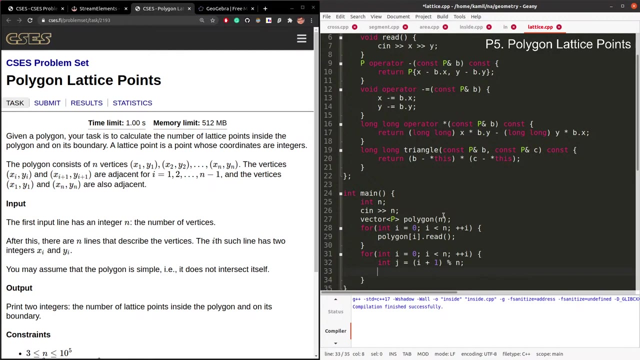 Read all the points and for every segment, so for every. i look at j being the next point. it's i plus 1 modulo n. let's actually use the third version. this is the index of the next point and you look at Delta X being polygon of J minus polygon of I. 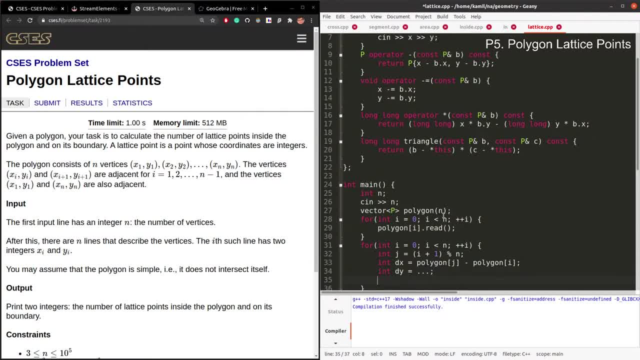 and delta Y is the same for Y's. why should I implement, why should I type this, when I can just say difference, like the vector of transition is polygon of J minus polygon of I. this already computes Delta X and Delta Y. take gcd of X and Y, and gcd actually isn't defined properly for zeros, so this: 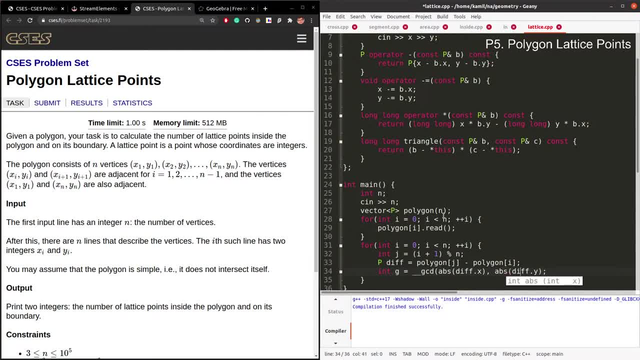 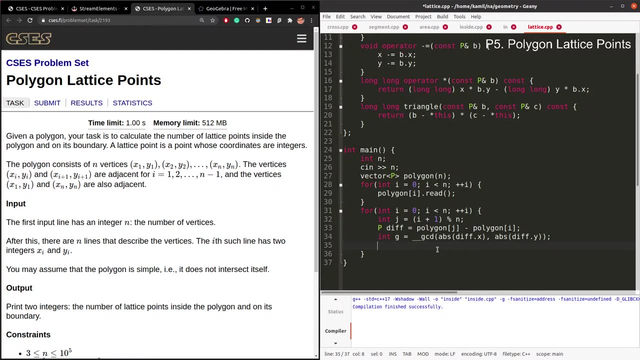 will not need to be changed, necessarily work. i mean gcd in c++. in terms of math, this is correct in terms of c++ gcd. in some compilers this doesn't work for zero, so it will not. it will give you an error for gcd of three, zero or zero three. i think my compiler will be fine here. let's see. maybe it will blow up. 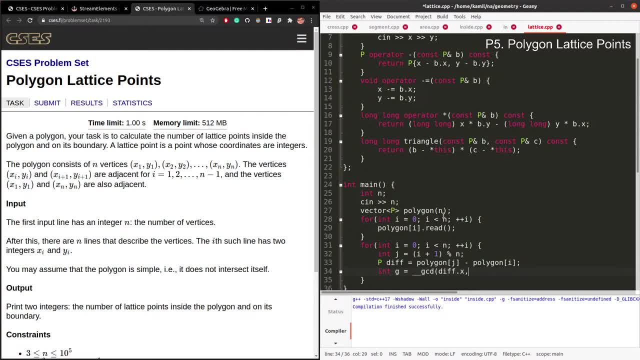 Take gcd Of x and y, And Gcd actually isn't defined Properly for zeros, So this will not necessarily work. I mean gcd in c++. In terms of math, This is correct In terms of c++ gcd. 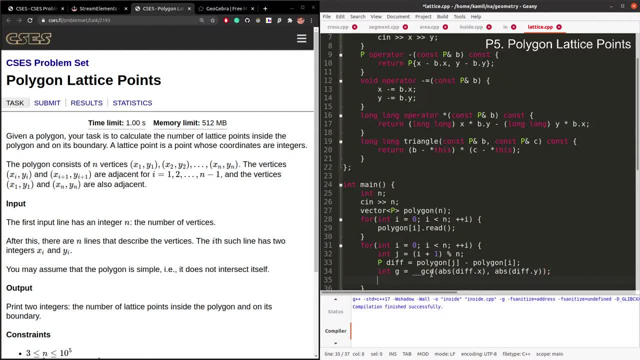 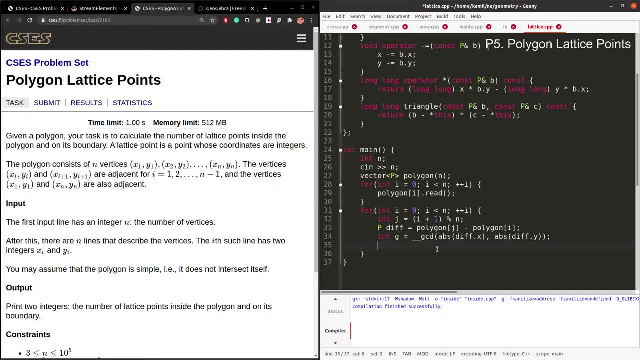 In some compilers This doesn't work for zero, So it will not. It will give you an error 0.3.. I think My compiler will be fine here. Let's see. Maybe it will blow up. Actually, you should here make some ifs. 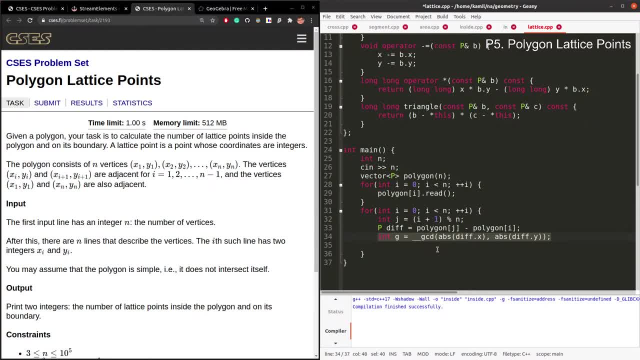 If diff x is 0. Then take diff y. If that other thing is 0. Then take diff x. Or just implement your own gcd. This is maybe not safe- Not safe for some compilers. Std gcd works fine, Alright. 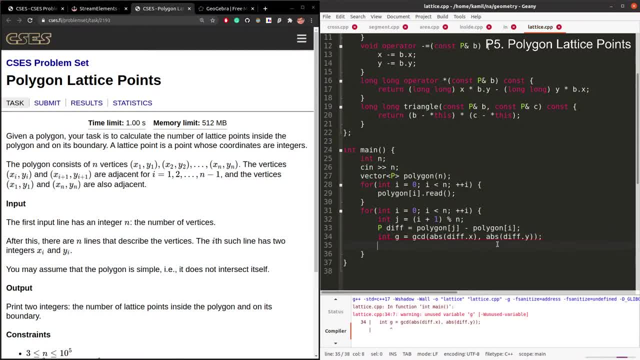 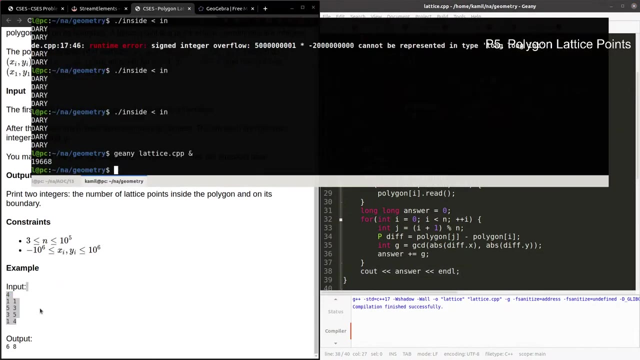 This compiles nowadays. Alright Cool, And I'm using long, long, Because maybe there are a lot of those, I don't know. if this is limited, I should get 8.. And then we move to the hard part, 8.. 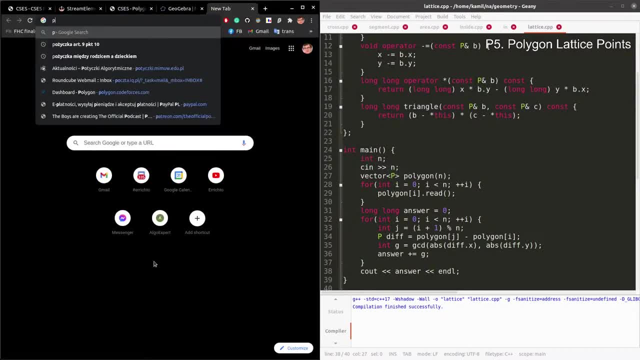 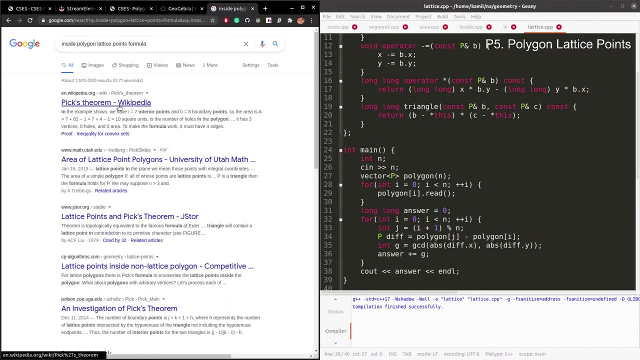 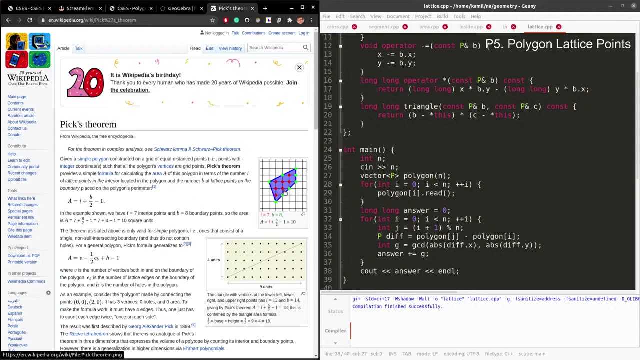 And now Inside polygon Latice points Formula. This is called Pick's theorem. It tells you exactly How to compute points inside And this is the formula i plus b, over 2. Minus 1. Where? 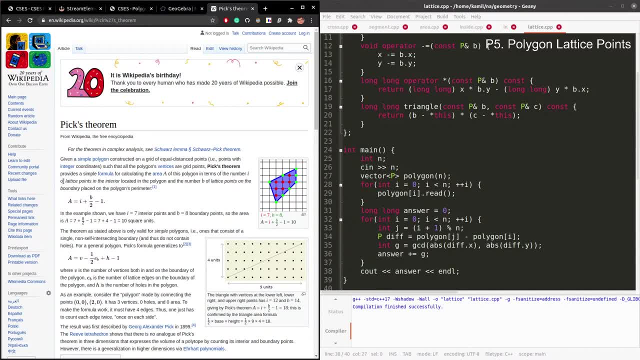 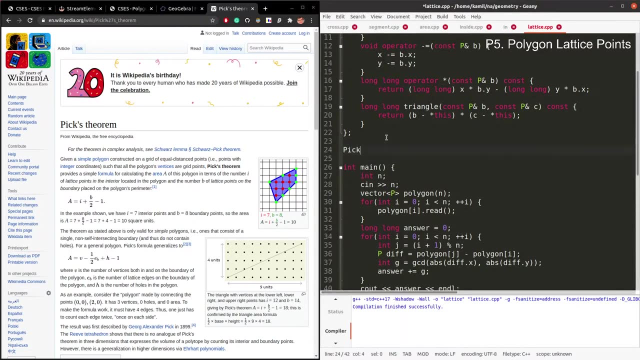 i Number. i is the number of lattice points in the interior. a is area, b is number of lattice points on the boundary, And then we have minus 1.. Pick's theorem Says Area is Interior Plus Boundary over 2.. 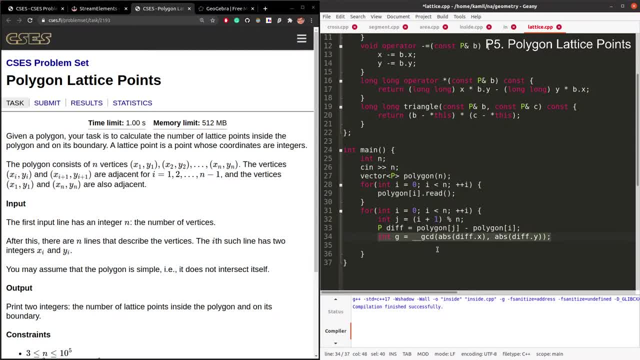 actually you should here make some ifs. if div x is, if div x is zero, then take div y. if that other thing is zero, then take div x or just implement your own gcd. so this is maybe not safe- not safe for some compilers. that std gcd works fine, all right, so this compiles nowadays. 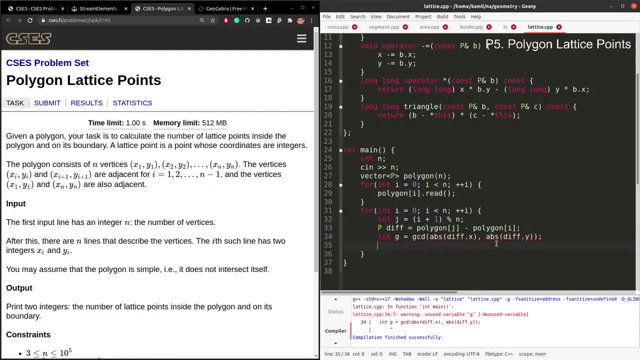 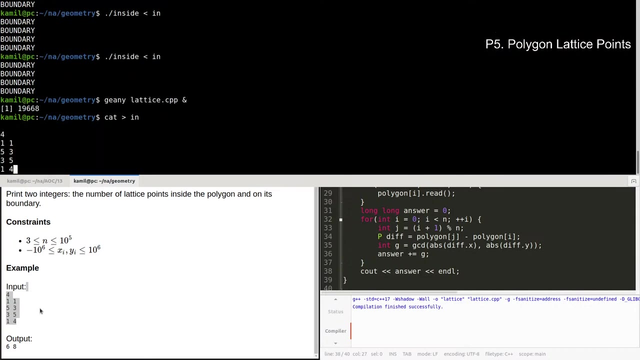 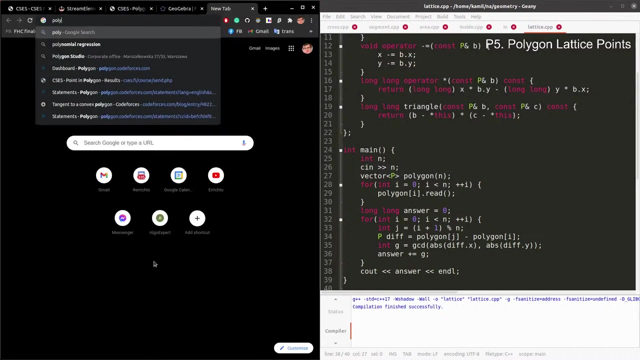 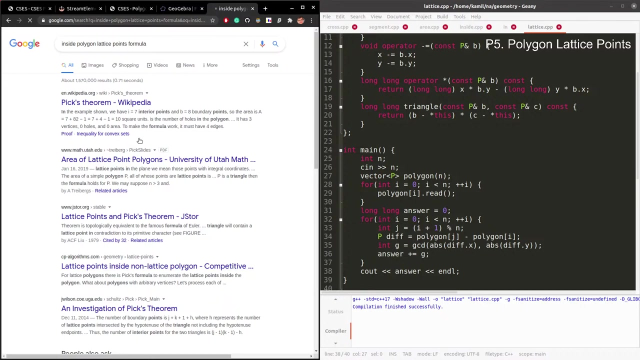 all right, cool. and you? i'm using long, long, because maybe there are a lot of those, i don't know. if this is limited, i should get eight. and then we move to the hard part, eight. and now inside polygon, lattice points formula. this is calledまк-анд. هذا называется. 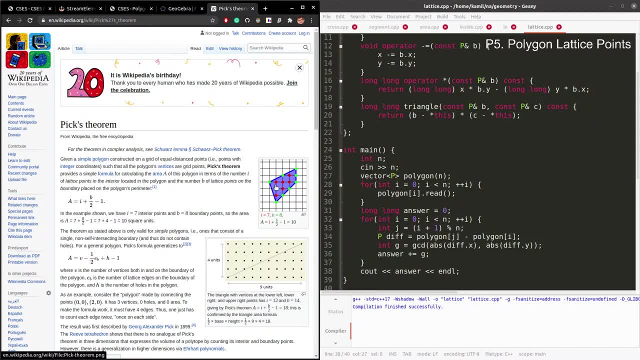 pygst street theorem. it tells you exactly how to compute points inside and this is the formula i plus b over two minus one, where i number, i is the number of lattice points in the interior. a is area, b is number of lattice points inside the interior. a is area, b is number of lattice points in the interior. a is area. b is number of lattice points in the interior area. b is number of lattice points in the interior. b is a. hmm well, and this is kind of a, i'm assuming, but cross, i should break this- of all kinds sofinity scooter u eas出 in this. 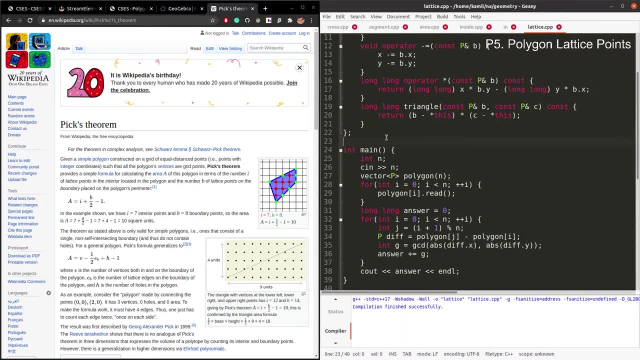 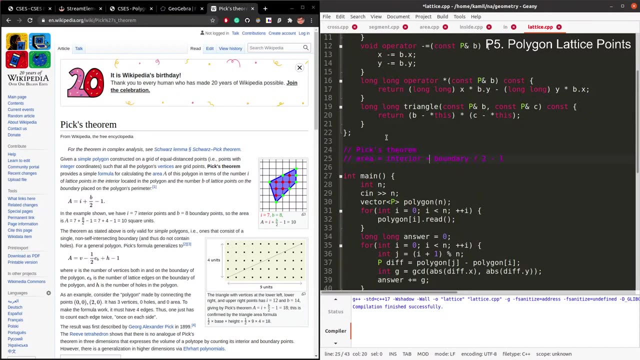 okay, great, monsieur im. so it's good. okay, okay, all right. so i just want to say: red his on the boundary, and then we have minus 1.. Peake's theorem says: area is interior plus boundary over 2 minus 1.. I will not explain it today, I don't. 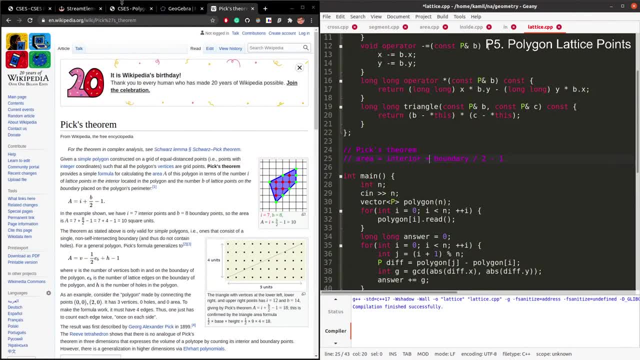 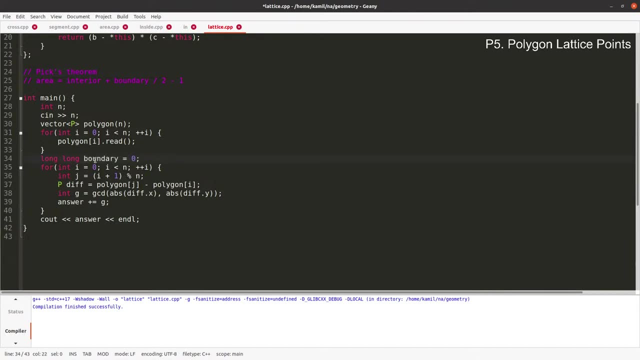 remember explanation of that For sure. this article explains it. if you want to do it, Here's link. And now the answer we computed is actually boundary, And from this how to compute interior. it is area minus boundary divided by 2 plus 1.. This also means that 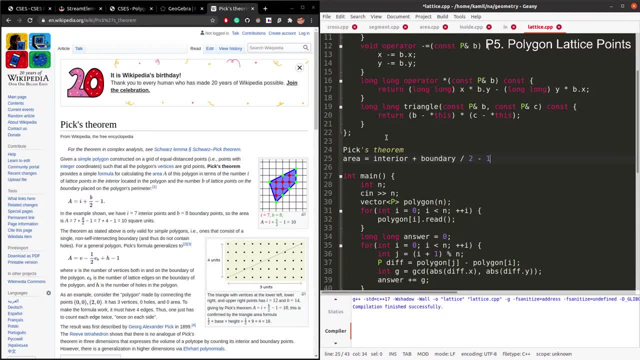 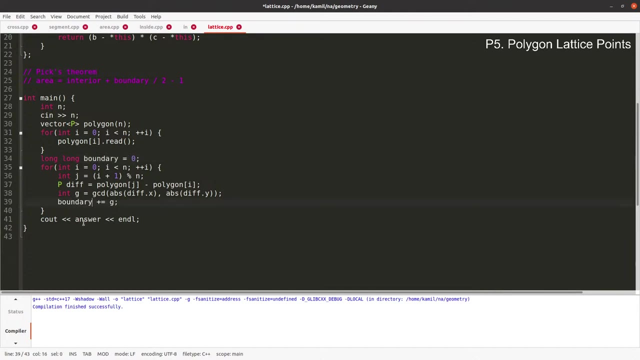 Minus 1.. I will not explain it today. I don't remember explanation of that For sure. this article explains it. If you want to do it, Here's link. And now The answer we computed is actually Boundary, And from this: 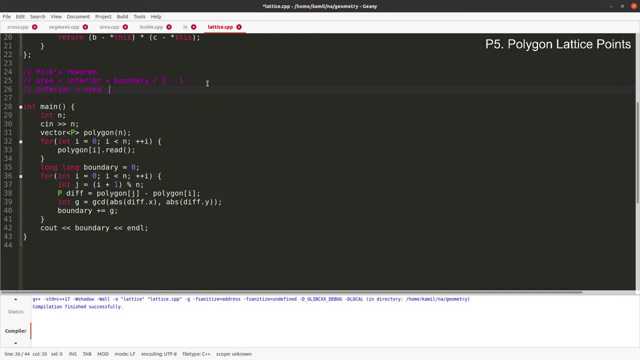 How to compute interior. It is Area minus boundary divided by 2. Plus 1.. This also means that Boundary must be Even. Oh yeah, Area can also be If boundary is like 3. Then this will give you 1.5.. 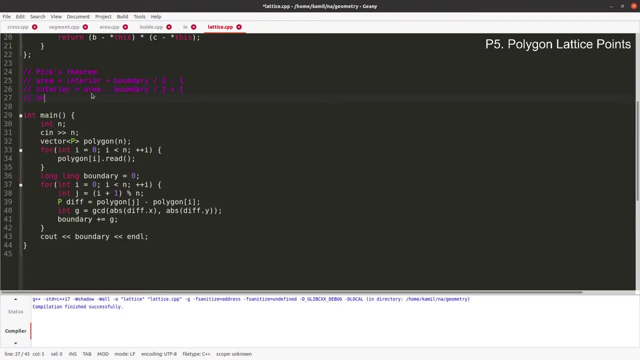 But also area, then is guaranteed to be Of the same parity. Might be the case that This will tell you that Interior is, for example, 7.5. Minus 1.5 plus 1. That's 6 plus 1.. 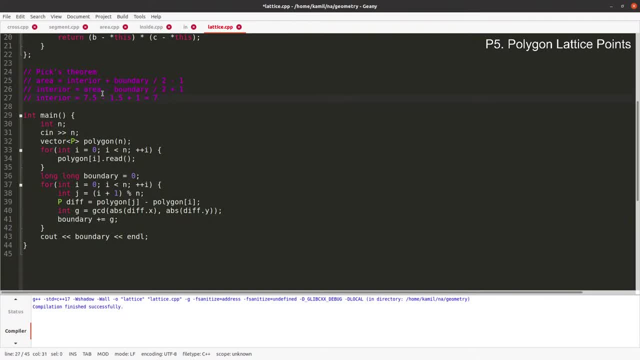 7. Are not integers? We need area? Here we go. I copy pasted it from area problem. Actually this is double area And that's actually convenient Because I will use a formula- interior, Twice, interior- To avoid any division. 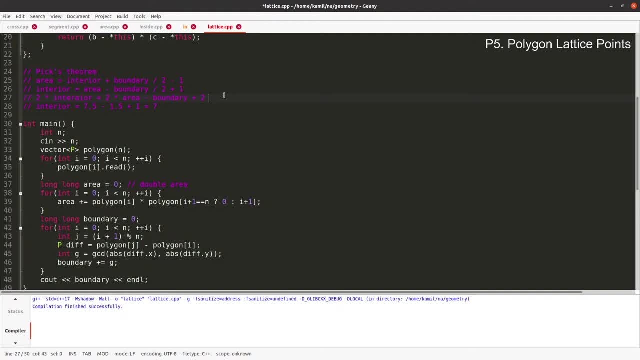 It's twice area minus boundary plus 2.. Let's focus on this formula: Twice interior Is twice area. I computed that After taking absolute value. Twice area Minus boundary Plus 2. Is twice area Minus boundary. 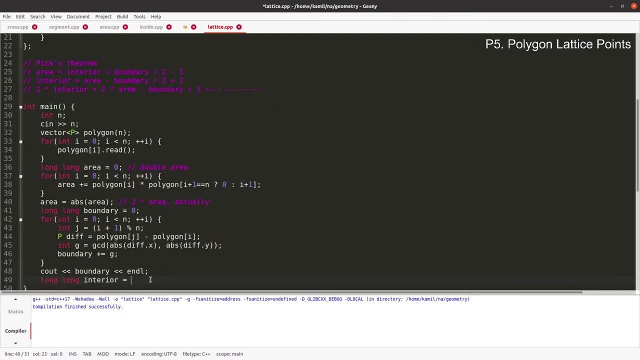 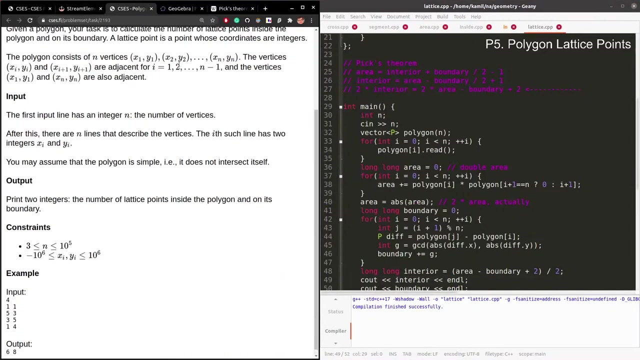 Plus 2. And this divided by 2. Because that's the formula For twice the interior. So That's the formula for twice the interior. This problem isn't harder Because they told us to count lattice points On the boundary. 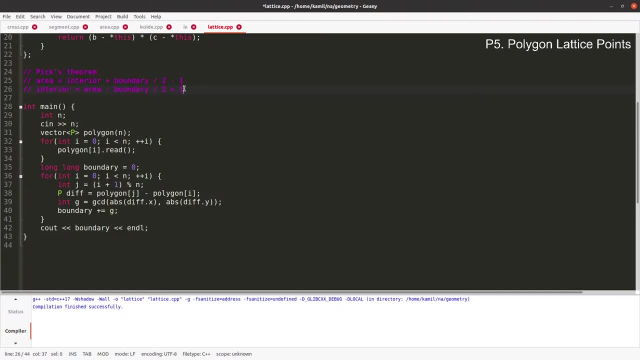 boundary must be. even What Something's? oh yeah, area can also be. if boundary is like 3, then this will give you 1.5, but also area then is guaranteed to be of the same parity. It might be the case that this will tell you that interior is for. 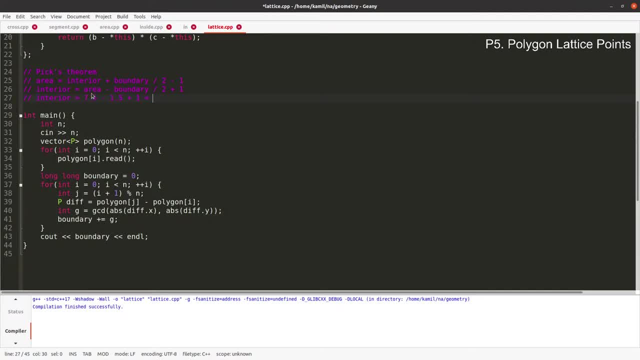 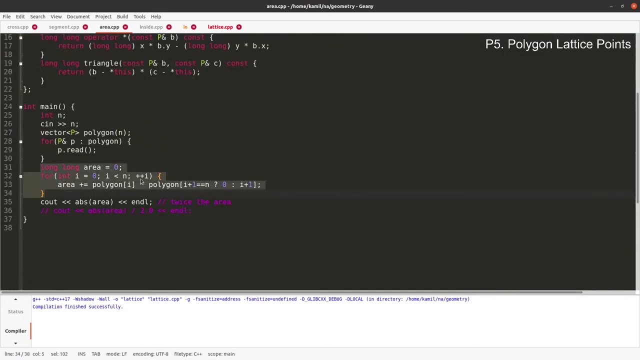 example, 7.5 minus 1.5 plus 1.. That's 6 plus 1, 7.. This always turns out integer, even though partial terms are not integers. We need area. So let's take a look at this problem and see what we can do with it. 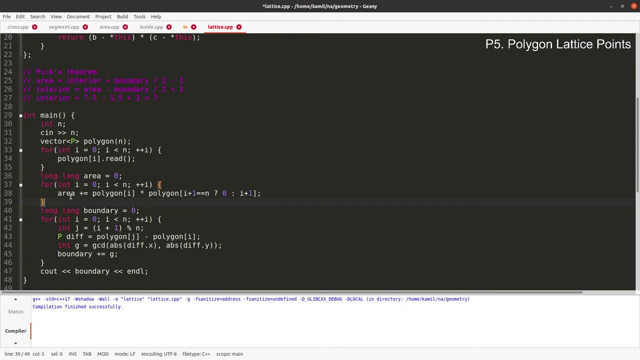 Here we go. I copy pasted it from area problem, Actually, that this is double area. and that's actually convenient because I will use a formula- interior twice interior- to avoid any division. It's twice area minus boundary plus 2.. Let's focus on 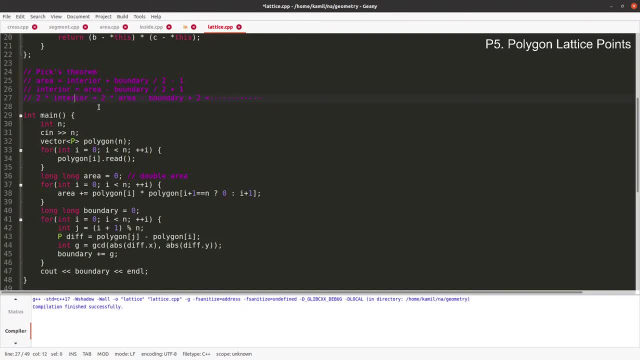 this formula, It's twice area. I computed that after taking absolute value: Twice area minus boundary plus 2.. It's twice area minus boundary plus 2.. And this divided by 2, because that's the formula for twice the interior. Let's see how it works. 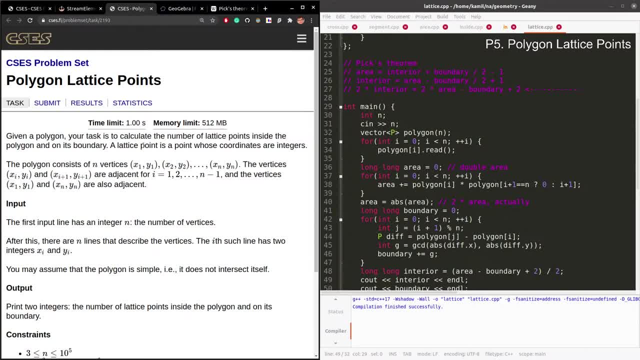 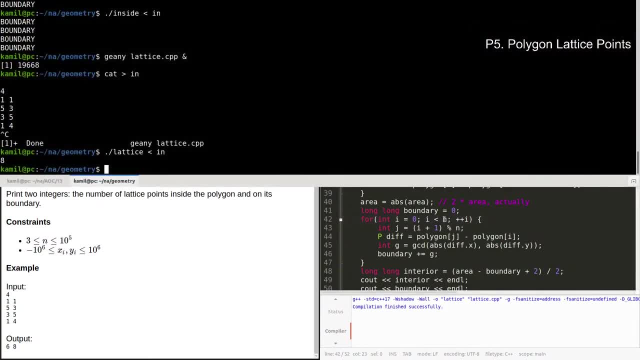 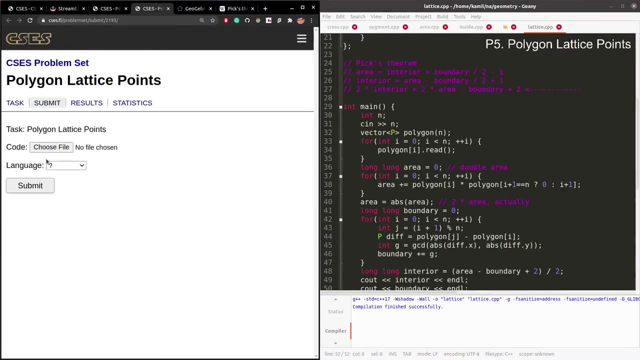 This problem isn't harder because they told us to count lattice points on the boundary. We need to do it anyway, to use Peake's theorem to compute lattice points inside 6, 8.. Everything is long, long, I hope It seems so. 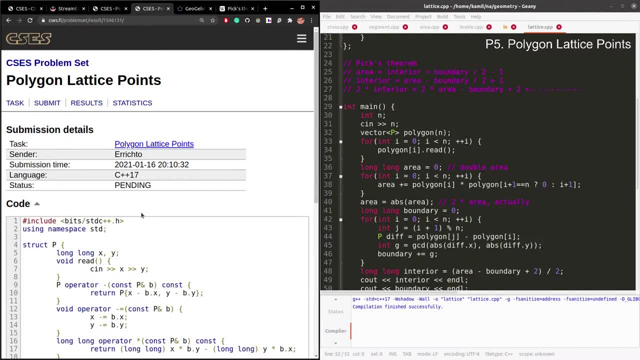 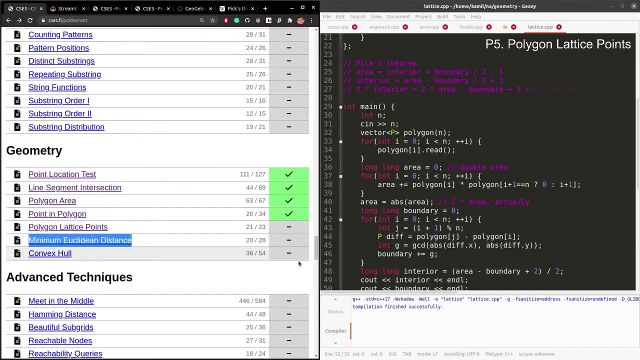 That's lattice. Hopefully that's accepted And it means we can move to the last problem for today. We skip minimum Euclidean distance and we move to convex hull, Because this is a hard problem and it isn't like a basic problem. you need to know convex. 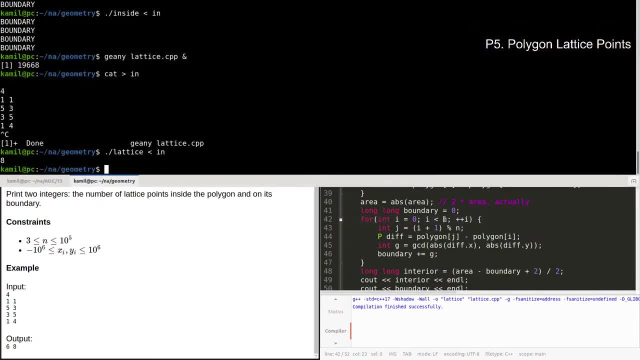 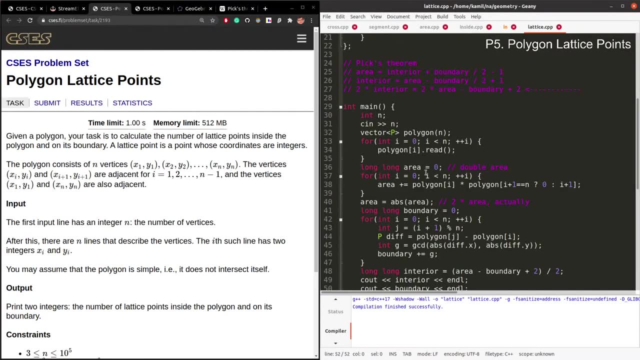 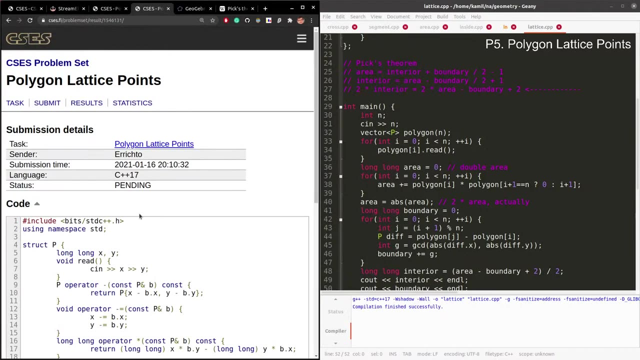 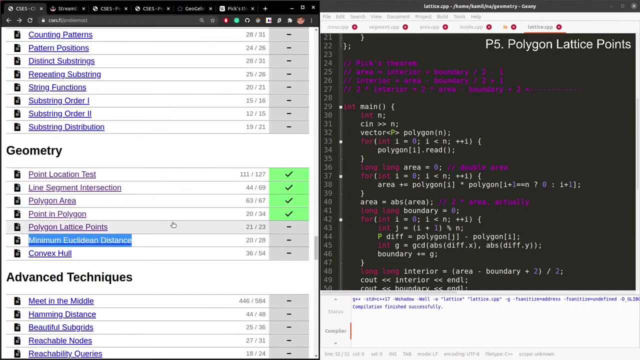 We need to do it anyway, To use Peake's theorem To compute lattice points inside 6, 8.. Everything is long, I hope, So That's lattice. Hopefully that's accepted And it means We can move to the last problem for today. 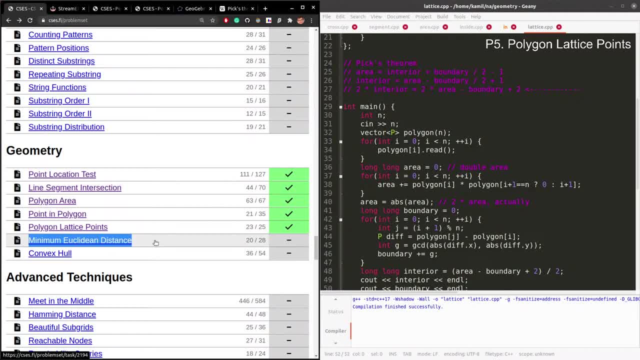 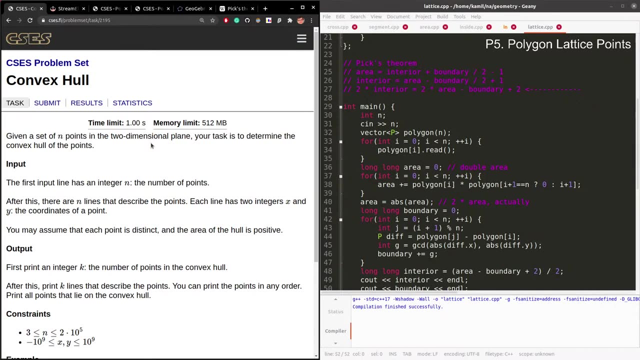 We skip minimum Euclidean distance And we move to convex hull, Because this is a hard problem And it isn't like a basic problem. You need to know Convex hull is And that will be the last thing We do today. 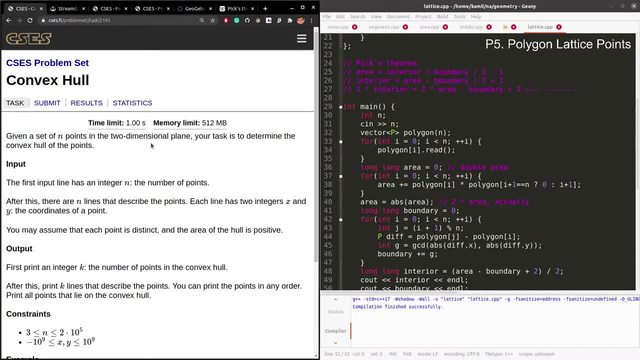 I will do the other one In some other stream. It's just a hard geometry problem. That other problem, Convex hull, is actually trivial In my opinion, For sure much easier than the other one. Alright, Last problem: Convex hull. 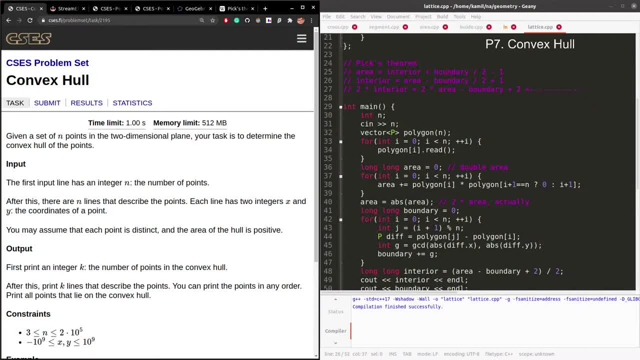 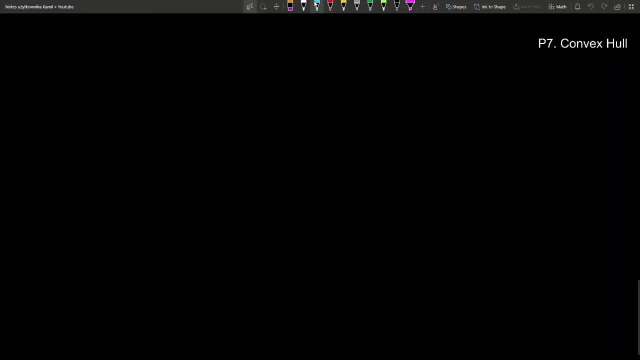 P7. Convex hull. Convex hull is a technically few, Maybe the most beautiful Algorithm In geometry. Hard to say. I don't have time Now to Give you some proper Tens of algorithms. Convex hull can be done in multiple ways. 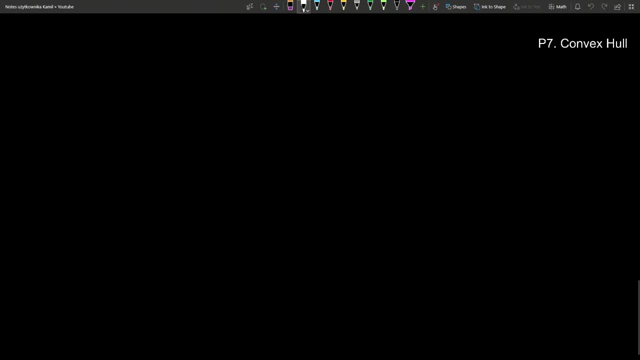 Convex hull is works, but it boils down to understanding definition, to know any kind of all right, given a set of points we need. let's say that those are sheep and you're like a farmer, sheep, farmer, maybe there's a word for that. Shepherd, yeah, I'm stupid, your Shepherd, this is your sheep. what is the smallest? 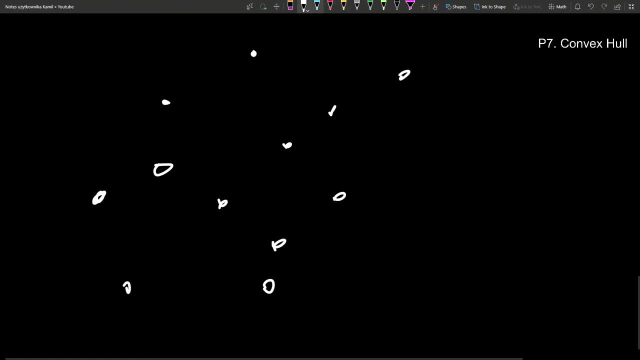 possible area to make boundary over those sheep. you need to build some kind of fence, but it cannot have holes. you cannot say that this is, your fence needs to be convex. convex means that every degree has smaller than 180 degrees. then the solution here is that that's convex hole of this set of points. 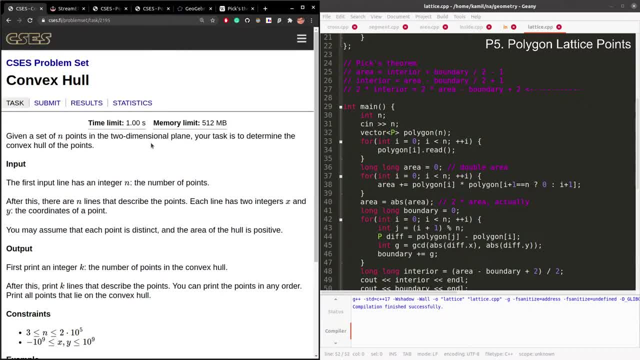 hull is, And that will be the last thing we do today. I will do the other one in some other stream. It's just a hard geometry problem. that other problem, Convex hull, is actually trivial in my opinion, For sure much easier than the other one. 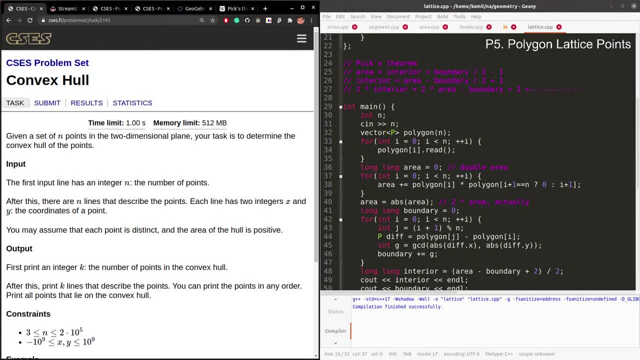 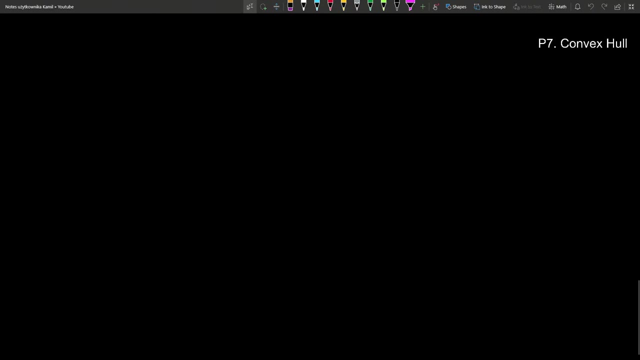 All right. last problem: convex hull P7, convex hull, Maybe the most beautiful algorithm in geometry, Hard to say. I don't have time now to give you some proper intuition- maybe not intuition, but to show you tens of algorithms. 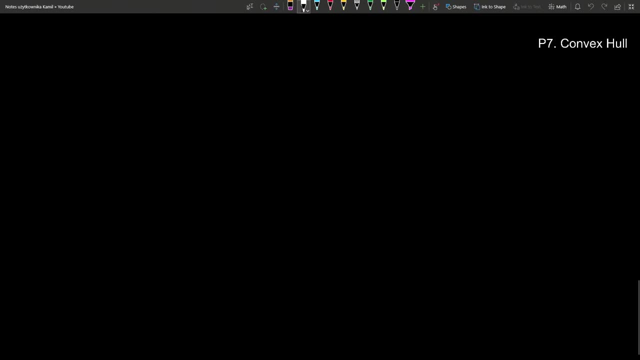 Convex hull can be done in multiple ways. It boils down to understanding definition, To know any kind of All right Given a set of points We need. let's say that those are ship and you're like a farmer, ship farmer, maybe there's. 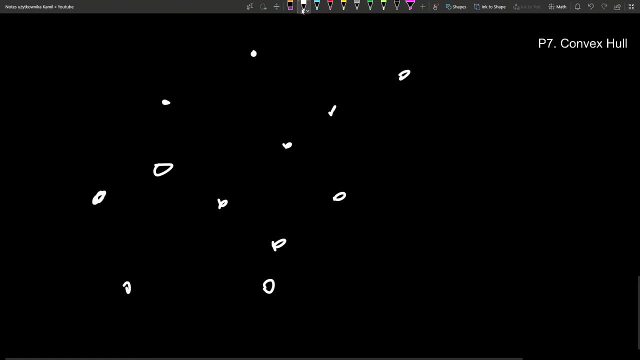 a word for that Shepherd. yeah, I'm stupid. You're a shepherd. This is your ship. What is the smallest possible area to make boundary over those ships? You need to build some kind of fence, but it cannot have holes. 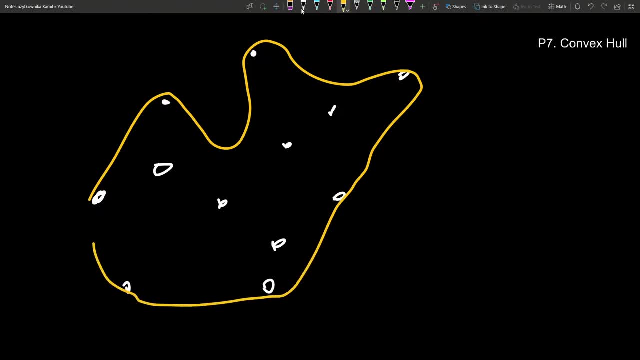 You cannot say that this is your fence. It needs to be convex. Convex means that every degree has smaller than 180 degrees. Then the solution here is that That's convex hull of this set of points You can. it means that we can ignore points inside other points in some way. 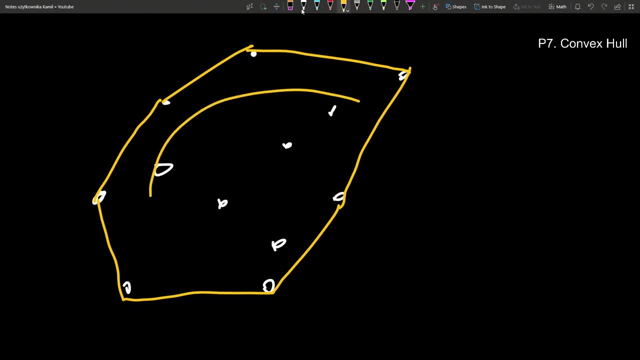 you can. it means that we can ignore points inside, other points in some way. you must be tired. now drink some water. good point, I will grab water up. what is any algorithm to do this? well, you can imagine, and this is one of kind of definitions- maybe not definitions, but one algorithm is to again imagine that we 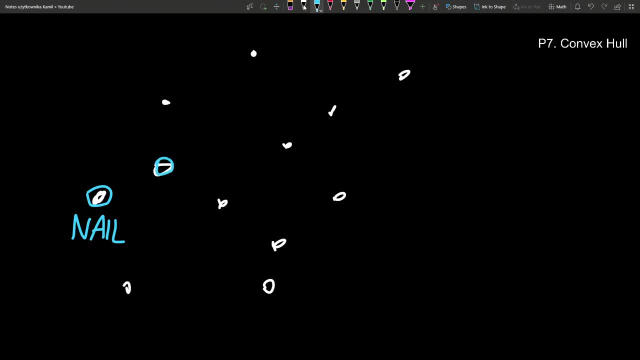 have a nail. actually, each of those is in that each white point is a nail and you put some rope around the leftmost nail and you move to the right and you, the human, move all the way like that and again here. then the rope will encircle. 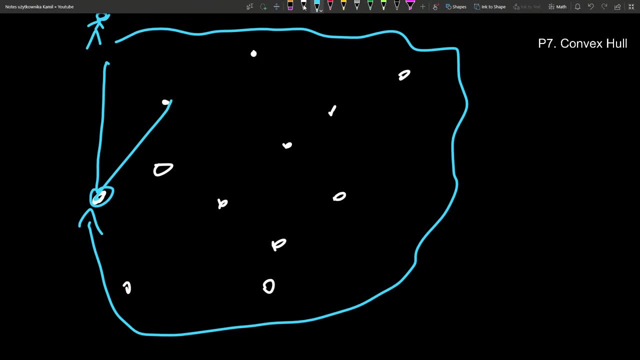 it will move around the points and it will stay exactly like that rubber band. yeah, that's proper wording. I'm not a native English speaker and sometimes I'm forgetting words that are not that technical, and this is called a Jarvis algorithm, I think. I don't remember properly. when you look, you find 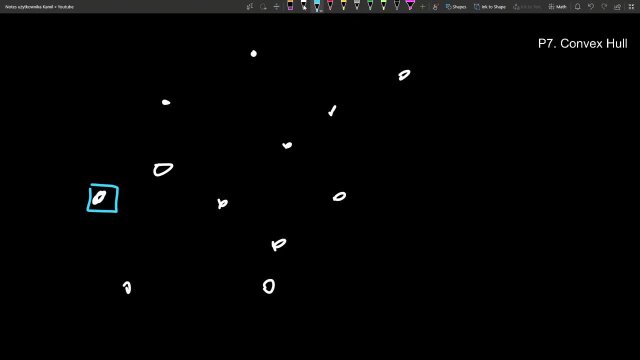 the leftmost point, and then you, among all the other points, you choose the leftmost one. with respect to the first point, when you want to compare two points, you can check that this one is more on the left using cross product. this way, you will say that this is leftmost. it is. 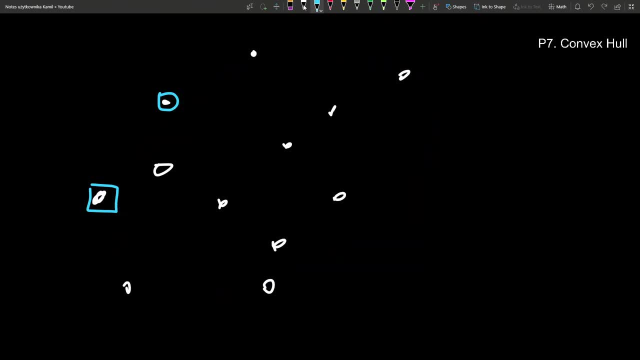 more on the left than everything else, just like when you can find minimum of a sequence. you can do it in linear time. the code goes like that, like you say, best is: let's say first a of zero, then for every i. you can do it in linear time. the code goes like that, like you say, best is: let's say first a of zero, then for every i. 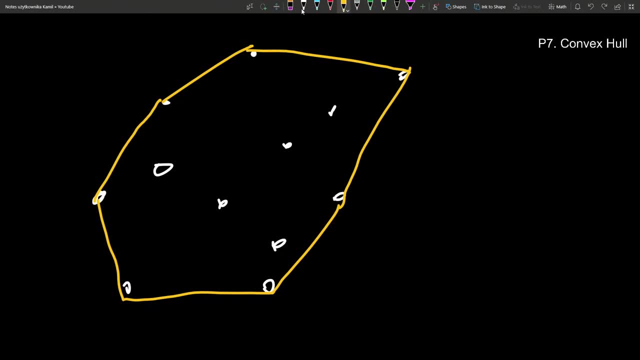 You must be tired now. drink some water, Good point, And then you need out some water here, carnal, Yeah, Same shit, same shit, The same shit. Okay, of definitions, maybe not definitions, but one algorithm is to again imagine that we have a nail. 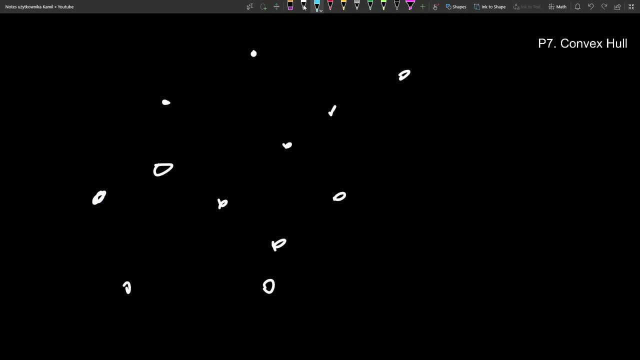 actually each of those is a nail, each white point is a nail, and you put some rope around the leftmost nail and you move to the right and and you, the human, move all the way like that and again here. then the rope will encircle, it will move around the points and it will stay exactly like that. 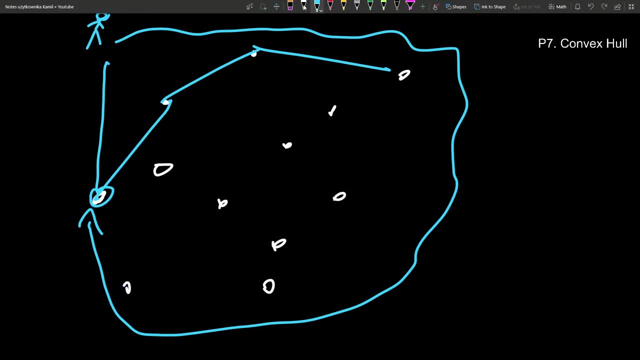 rubber band. yeah, that's proper wording. i'm not a native english speaker and sometimes i'm forgetting words that are not that technical, and this is called the jarvis algorithm, i think i don't remember properly. when you look, you find the leftmost point and then you, among all the other points, you choose the leftmost one with. 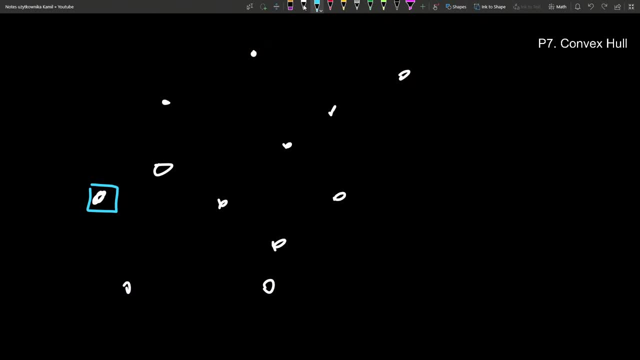 respect to the first one, when you want to compare two points, you can check that this one is more on the left using cross product. this way, you will say that this is leftmost. it is more on the left than everything else. just like when you can find minimum of a sequence, you can do it in linear time. 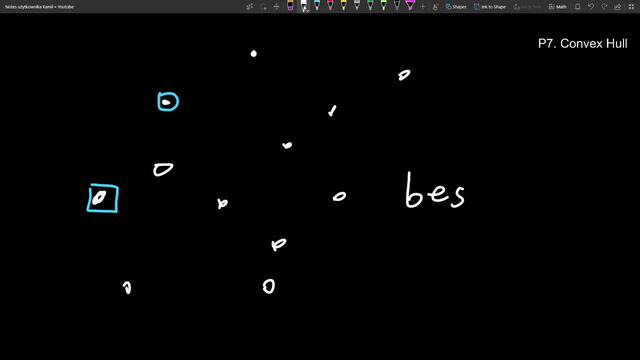 the code goes like that. like you say, best is, let's say first a of zero, then for every i, every i. if a of i is smaller than a of zero, none best. best is a of i. that's algorithm to find minimum in a sequence and it also works to find the leftmost among all. 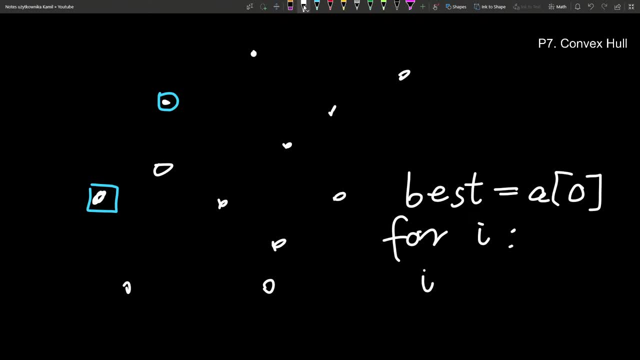 if a of i is smaller than a of zero, then best is a of i. that's algorithm to find minimum in a sequence, and it also works to find the leftmost among all the points. if this you interpret as comparing angles, so you just use cross product with respect to this, you go through all the points. 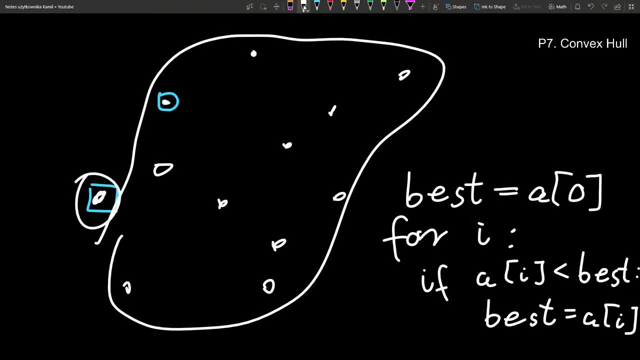 the n-1 points everything other than this one, and you need to find the best one. so, among few points, if you see that, okay, so far this is the best, and then you compare it with this one, you see that this is more on the left, so you: 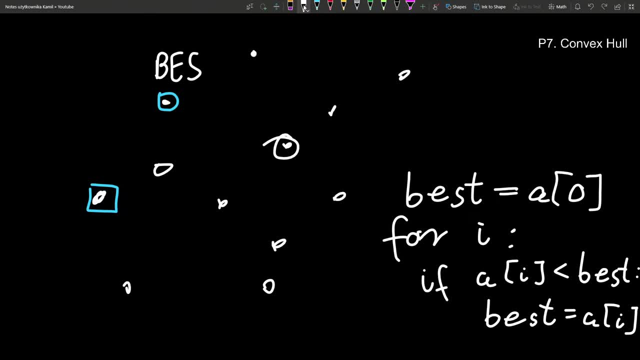 now say: this is best after all of this is done, looking from this point like so, saying that the rope will touch this guy. at now, we need to find the next point in this angle, in this direction, when let's say: rope moves like that, as you move here and eventually it will touch this. 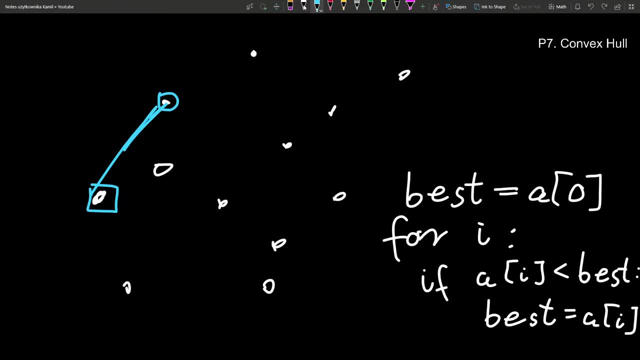 guy To find this, nail this point. you need to, among all the points, find the leftmost looking from here, And it's okay if you also try this one. It's fine to say: among n-1 points, find the leftmost with respect to this, It's okay. 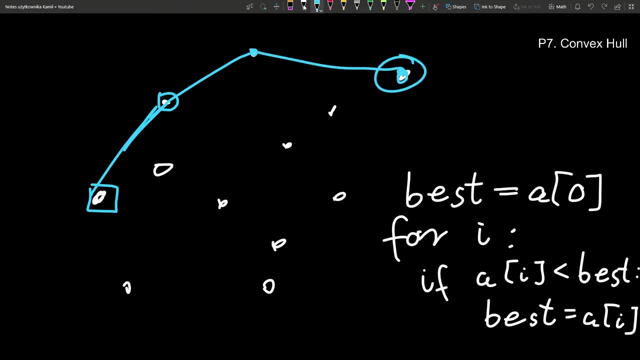 You move like that and you just continue. Now, with respect to this, among all n-1 points, find the leftmost. You will see this, then that, then this, Eventually, with respect to this, the leftmost is that, and if you got back, that's it, This algorithm. 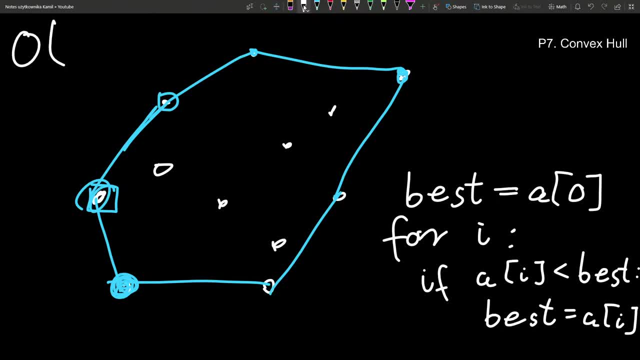 has complexity O of n multiplied by c, where c is size of the convex, so maybe I should say s Size of the convex and the number of vertices. It can be a case that that's actually n. This is n square and that's bad. There is a better algorithm: n square. 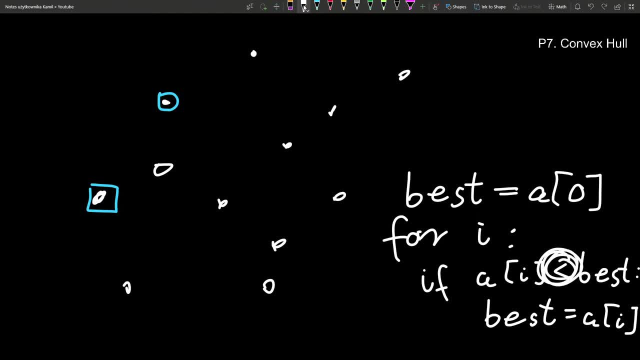 the points if this you interpret as comparing angles, so you just use cross product with respect to this. you go through all the n minus one points, everything other than this one, and you need to find the best one. so, among few points, if you see that, okay, so far this is the best, and then you compare. 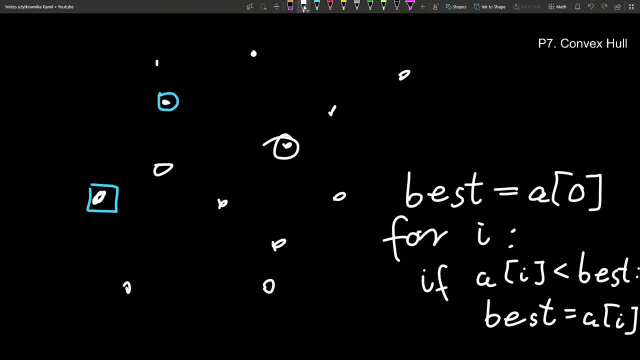 it with this one. you see that this is more on the left. so you now say: this is best. after all of this is done, looking from this point, like so saying that the rope will touch this guy. and now we need to find the next point in this angle, in this direction. so when let's say rope. 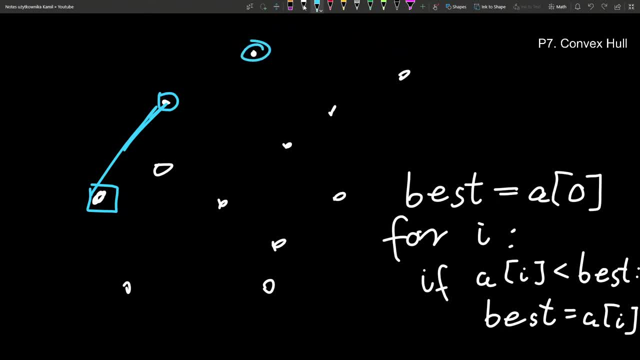 moves like that, as you move here, and eventually it will touch this guy. to find this, nail this point, you need to, among all the points, find the leftmost. looking from here, and it's okay if you also try this one. it's fine to say: among n minus one points, find the leftmost with respect to this. 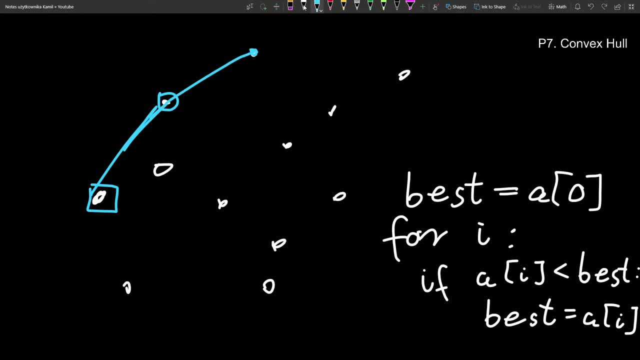 it's okay, you move like that and you just continue. now, with respect to this, among all n minus one points, find the leftmost. you will see this and that, then this. eventually, with respect to this, the leftmost is that, and if you got back, that's it. this algorithm has complexity: o of the multi n multiplied by c. 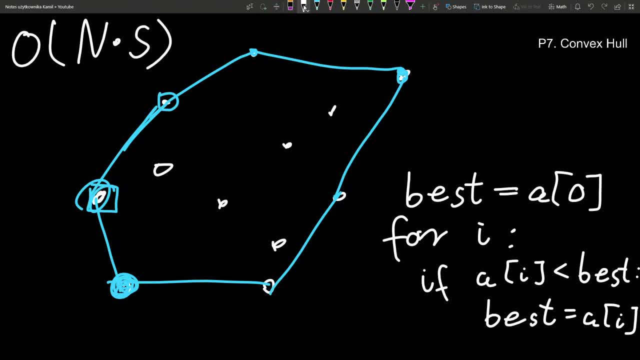 where c is size of the convex. maybe i should say s size of the convex and the number of vertices. but it can be a case that that's actually n. this is n squared and that's bad. there is a better algorithm. n square is too slow for these constraints. 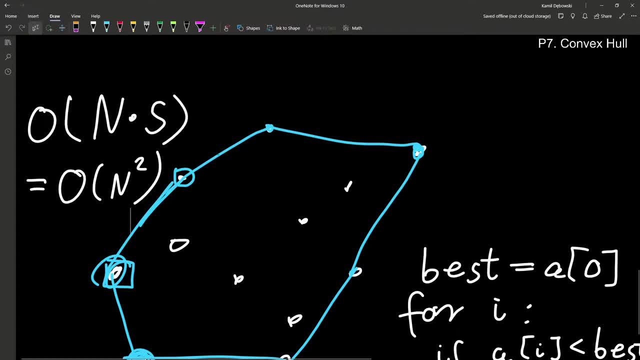 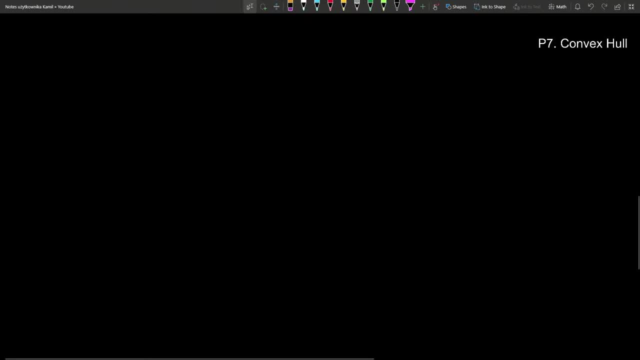 again. i believe this is called jarvis algorithm, but now we'll do something better: graham scan. oh, maybe it's called graham scan. yeah, i sorry, i think you're right, it's graham scan, not jarvis. and now the actual algorithm that we will use, and it is n log n, is that? 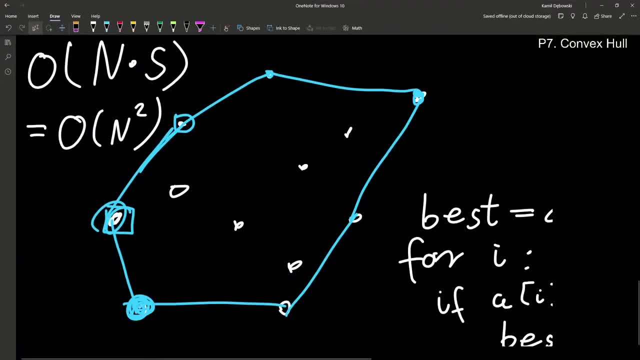 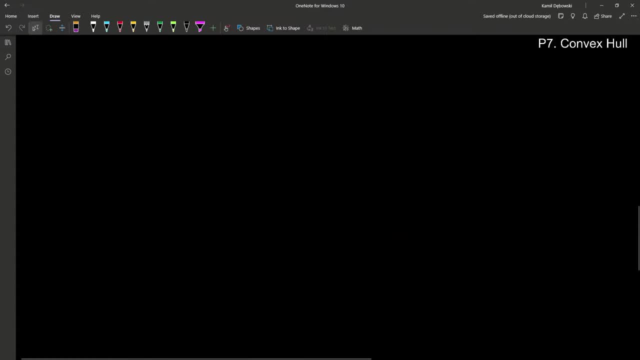 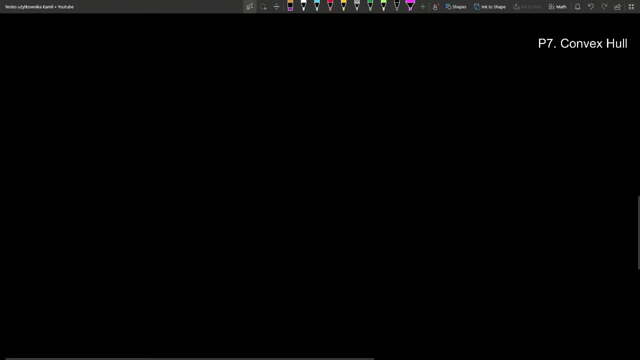 is too slow for these constraints. Again, I believe this is called Jarvis algorithm. but now we'll do something better: Graham scan. Oh, maybe it's called Graham scan. Yeah, I'm sorry, I think you're right. It's Graham scan, not Jarvis. And now the actual algorithm that we will: 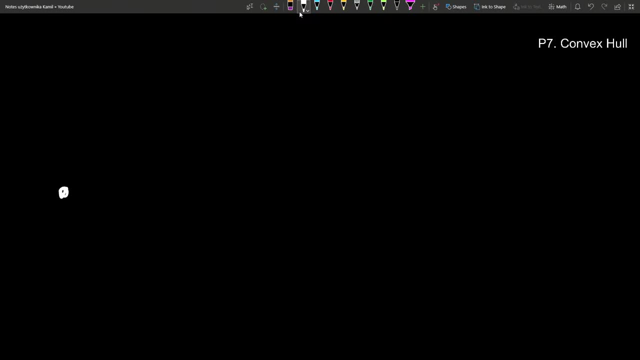 use, and it is n log n, is that we go through points from left to right and when you already considered some few points and you already understood what happens when you move, you, the human, you move with the rope to the right, all the way to the right here, to plus infinity. 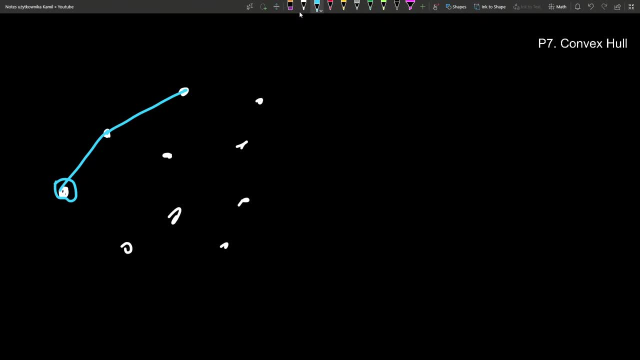 Then you will understand what's the current shape. And now you process the next point, The next after them, the next point to the right is, let's say here: Then you need to say that this is the next thing how the rope looks like. And now, if the next point on the 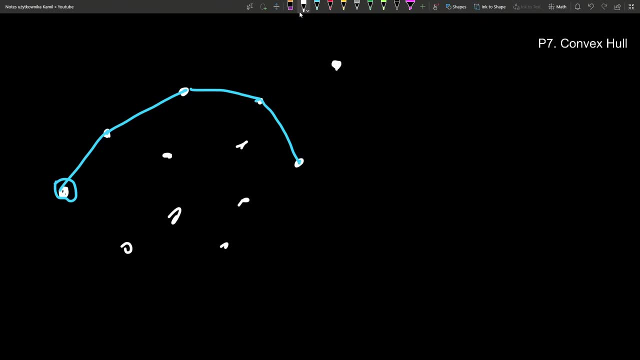 right is actually here. you need to update the current shape. You cannot say that this is the shape, because this is not convex when so when you are here, but actually the human went there and the rope should rest here, because it's kind of higher, but not really higher, It's all angle-wise. Then 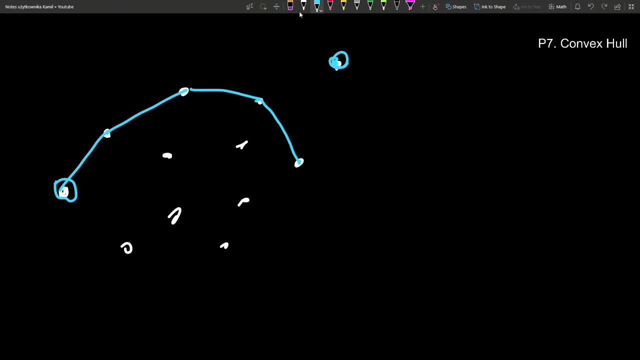 this point will not belong in convex hole, at least not in this top part. This is not a good convex hole. We need to relax it. So correct it a little bit And I will say: well, this doesn't belong to the convex hole, This does. Oh, and then. 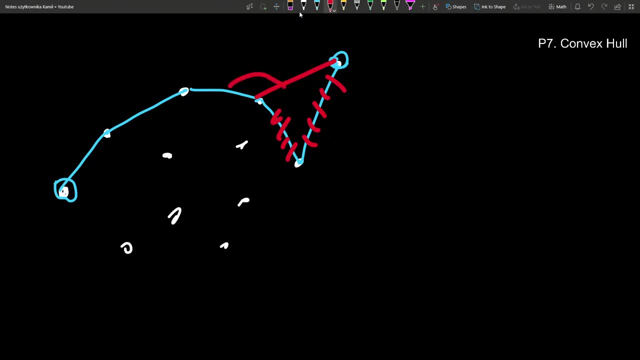 here. this is again not a convex angle. I mean, this thing is greater than 180 degrees. So I cancel this and I say: that's the convex hole And that's what we need to repeatedly do On the stack. we keep the convex hole. so far It is convex. Then, when we have new, 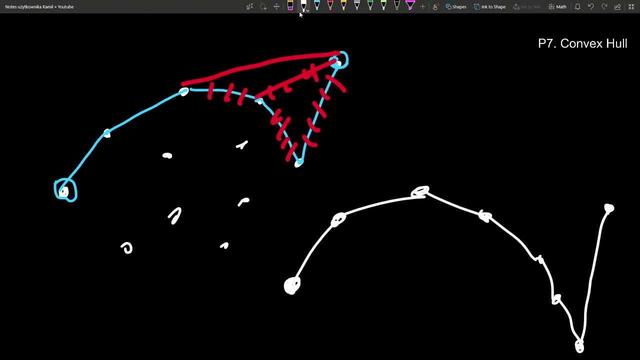 point on the right. we repeatedly change the point And this is important. We keep on checking how to check if we are in good angle with respect to the last segment. We check the two last points in current convex hole, Compare it with this new guy, And we check the angle using cross product. 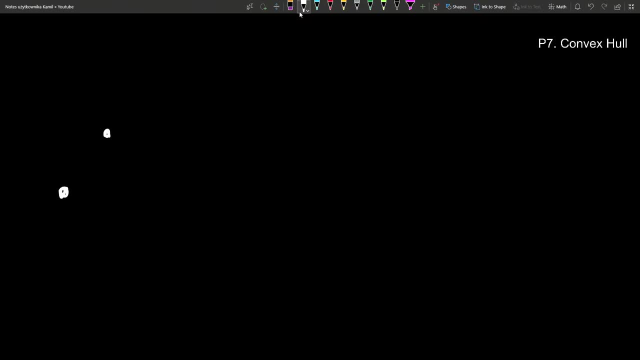 we go for points from left to right, and when you already considered some few points and you already understood what happens when you move, you, the human move, with the rope to the right, all the way to the right here, to plus infinity, then you will understand what the current shape. 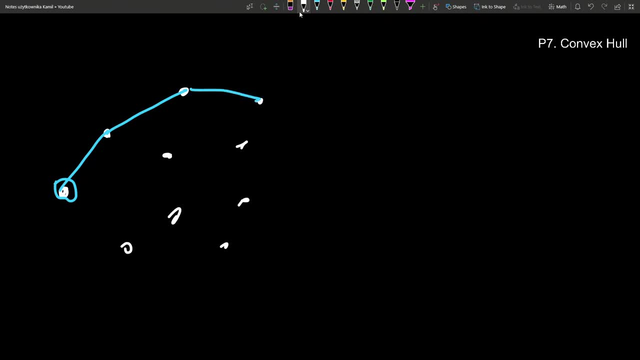 and now you process the next point, the next, after then the next point to the right is, let's say here. then you need to say that this is the next thing how the rope looks like. and now, if the next point on the right is actually here, you need to update the current shape. you cannot say: 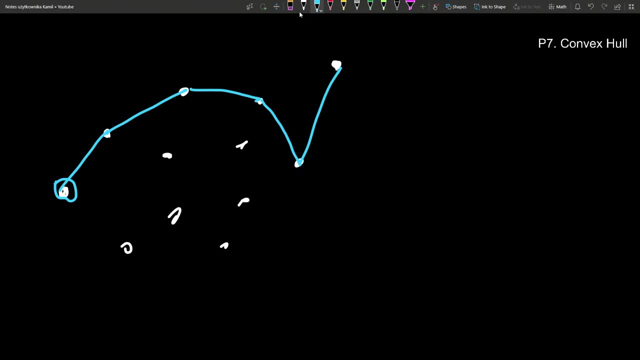 that this is the shape, because this is not convex when so when you are here, but actually the human went there and the rope should rest here because it's kind of higher, but not really higher, it's all angle wise, then this point will not belong in the convex hole. it not, at least not in this top part. this is not a 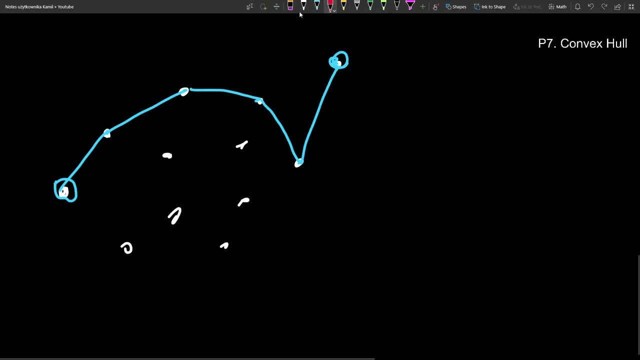 good convex hole, we need to relax it. so correct it a little bit and I will say: well, this doesn't belong to the convex hole, this does. oh and then here, this is again not a convex angle. I mean, this thing is greater than 180 degrees, so I 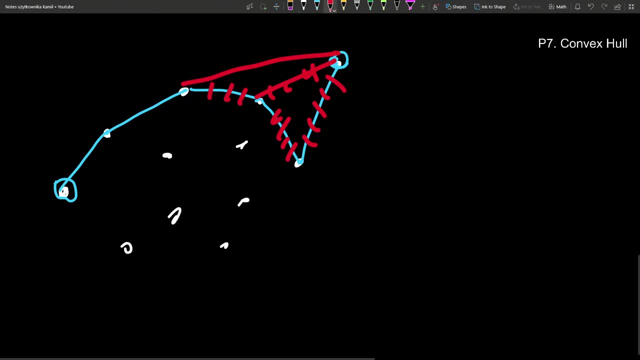 cancel this and I say: that's this, the convex hole, and that's what we need to repeatedly do on the stack. we keep the convex hole so far it is convex. then when we have new point on the right, we repeatedly check if we are in good angle. with respect to the last segment, we 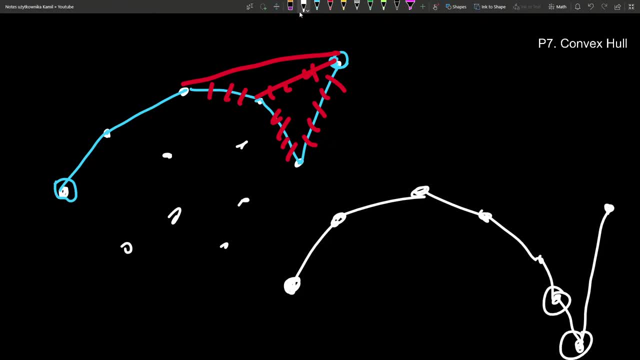 check the two last points in current convex hole, compare it with this new guy and we check the angle using cross product. this way, we will cancel this guy, this guy, this guy. let's say that already. we got down to here. what exactly we need to check? let's call this new point C and 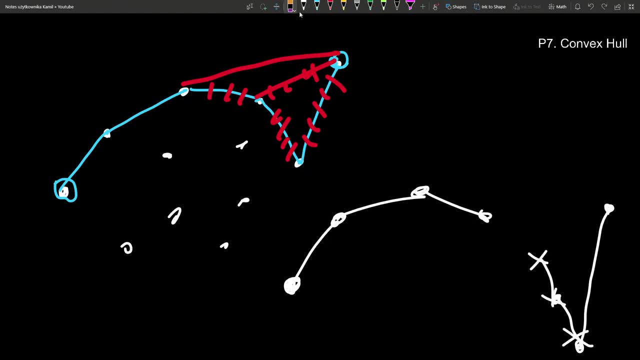 And yeah, this way we will cancel this guy, This guy, this guy. Let's say that already we got down to here What exactly we need to check. Let's call this new point C And convex hole AB. Let's say that these were the four points so far and now we have C. 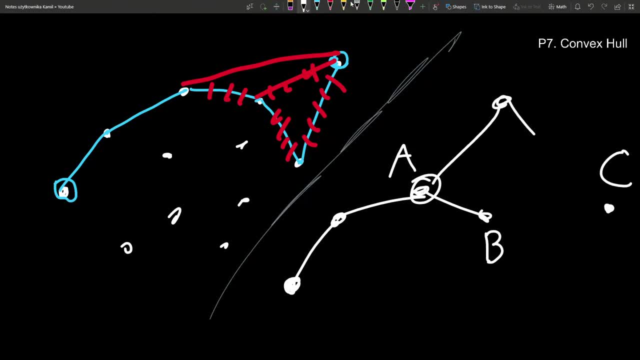 Everything is convex if we had something like A then B then C. So from A, B, C, this A dot triangle of BC should say that B is on the left. So it would be fine if it was A then B here, then C there. But if, looking from A, 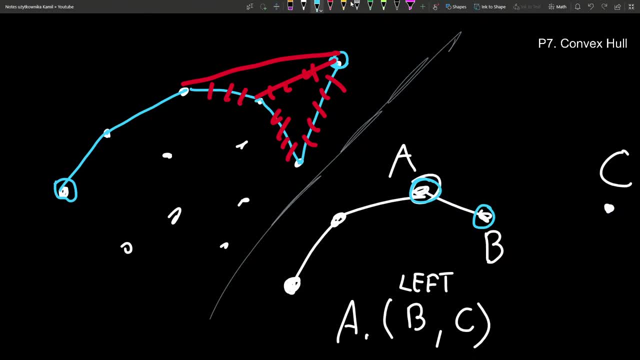 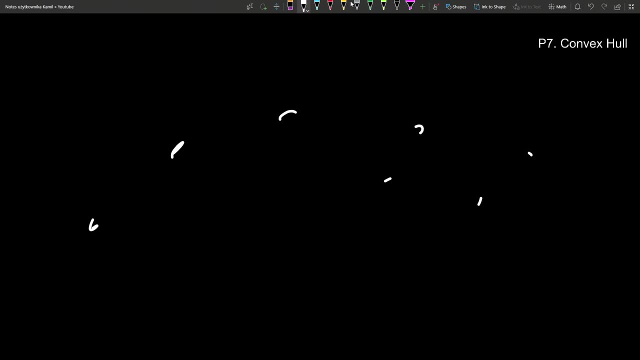 B is on the right, then C like this, then we need to cancel B. Then I remove this and I say that this is the convex hole. When I do this repeatedly and get to the very end, then eventually I will get the top part of the convex hole. 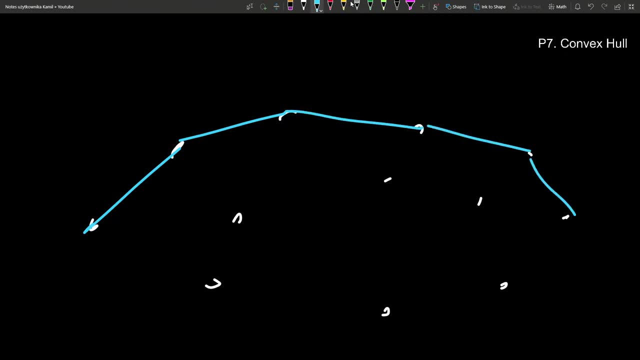 For this set of points. I will get that. Then I need to go here again and for that we will reverse the points and you can rotate the drawing, kind of. but this is not necessary. How to check the angle With cross product. Cross product allows us to check if something is on the left. 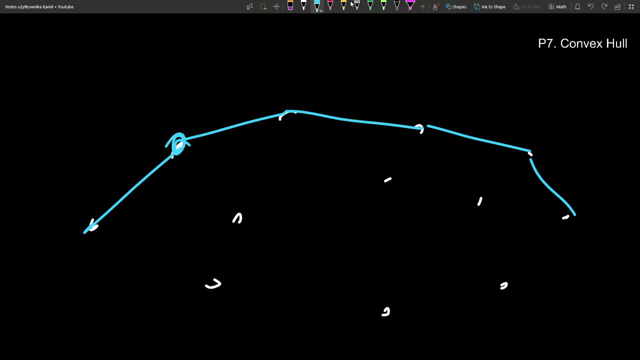 from something else. Generally, you can check if polygon is convex by doing this For every three consecutive points: A, B, C. you want this to be true. When looking from A, B is on the left from C, Then it's convex. Checking sign of cross product corresponds to: 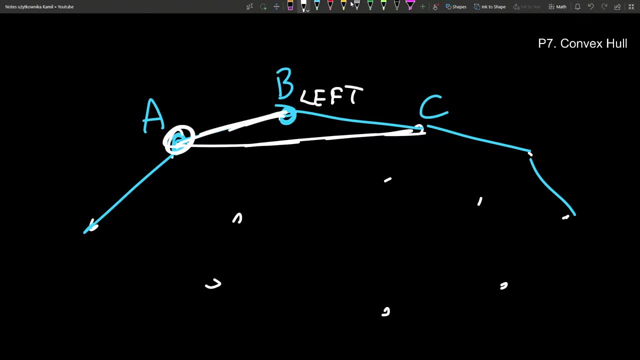 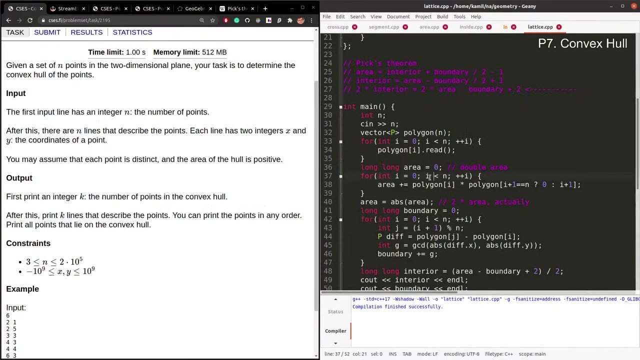 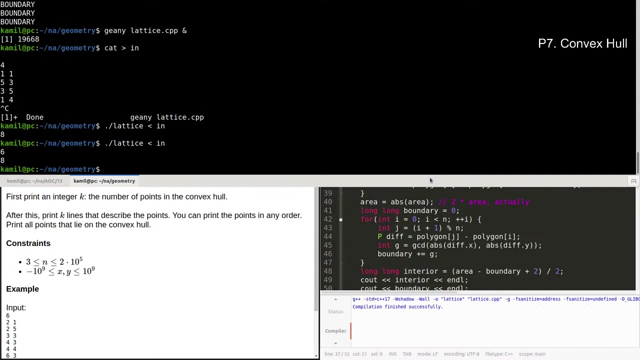 checking some kind of angle and comparing it with zero or with 180 degrees. Let's focus first on this top part. This is the last problem of today. then we finish. Anyway, I think the stream was too long and I don't see how anybody could focus for such a long time. 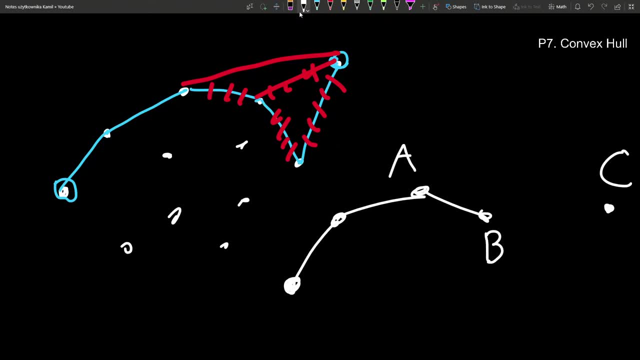 let's call two last points in the convex hole: a, B. let's say that this were the four points so far and now we have C. everything is convex. if we had something like a, then B, then C, so from a, B, C, this, this a, the triangle of B, C, should say that B is on the left. 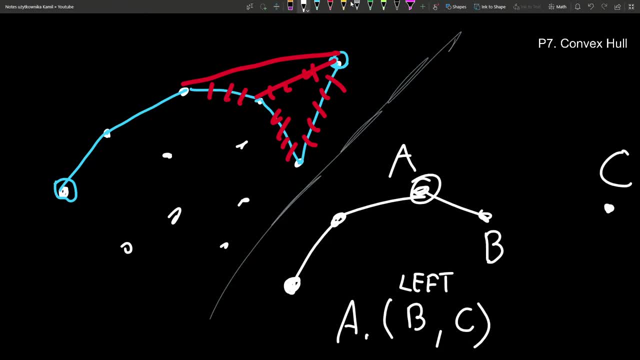 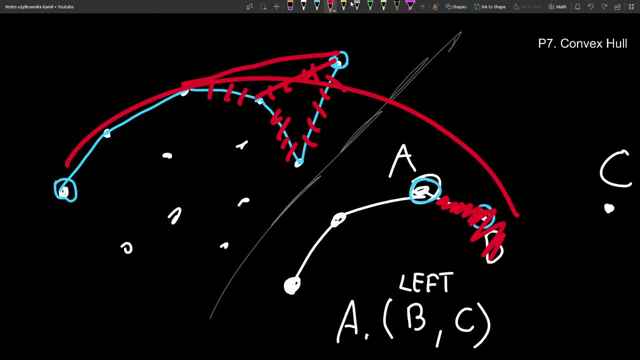 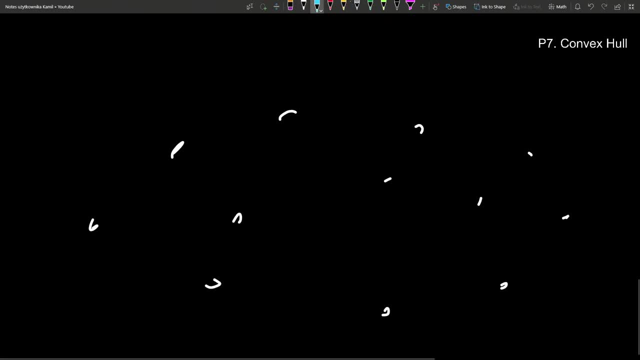 convex hole, convex hole. then I do this repeatedly and go to get to the very end. then eventually I will get the top part of the convex hole. for this set of points I will get that. then I need to go here again and for that we will reverse the points and you can. 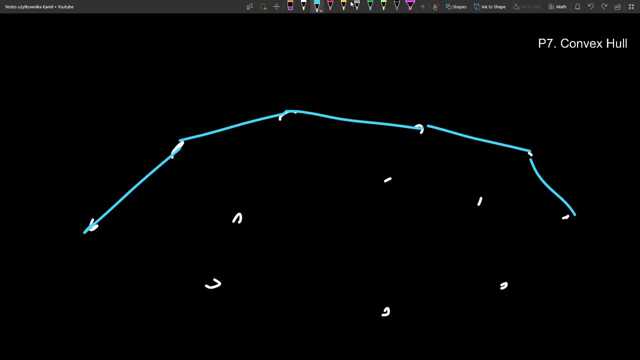 rotate the drawing kind of, but this is not necessary. how to check the angle with cross product. cross product allows us to check if something is on the left from something else. you can check if generally you can check if polygon is convex by doing this for every three. 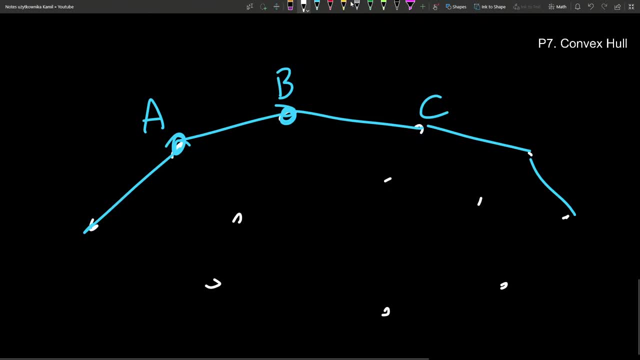 consecutive points a, B, C. you want this to be true. when looking from a, B is on the left from C, then it's convex. checking sign of cross product corresponds to come, corresponds to checking some kind of angle and comparing it with zero or with hundred eighty degrees. let's focus first on 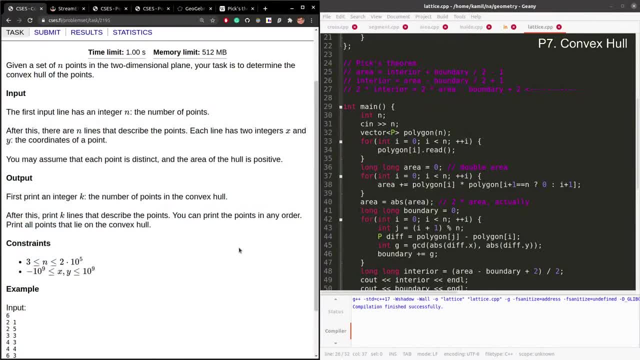 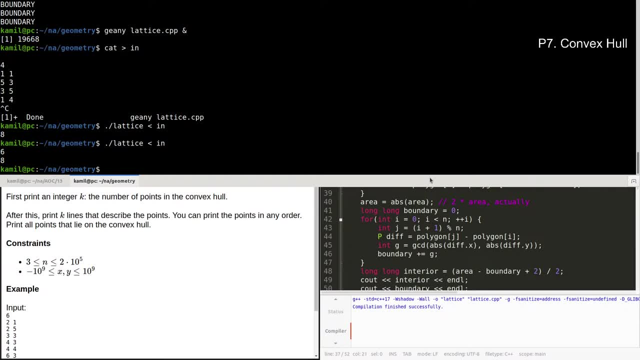 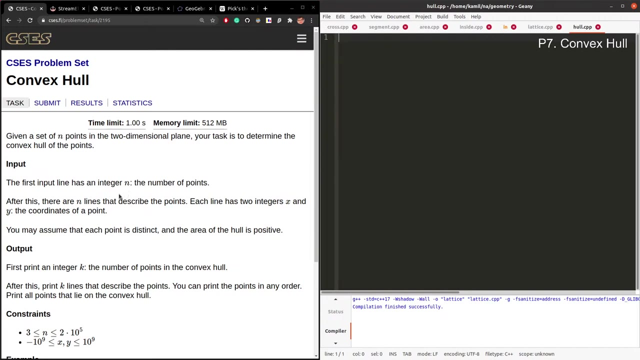 this top part. this is the last problem of today. then we finish. anyway, I think the stream was too long and I don't see how anybody could focus for such a long time. cool, that's all. the codes will be available in my avait repository. link is in the description in comments below. 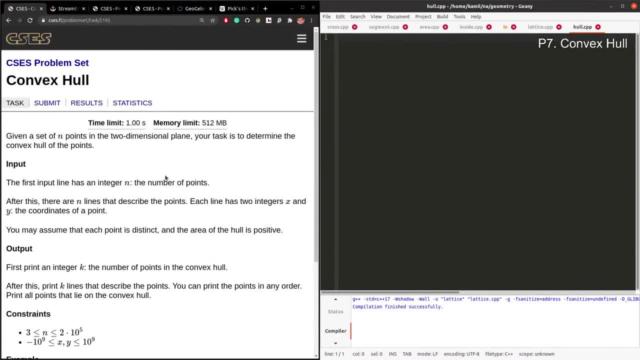 Hullcpp. All the codes will be available in my GitHub repository. Link is in the description in comments below YouTube Right Copy paste the short template: geometry template: Read the polygon. I will copy paste reading the polygon because I do it over and over again. 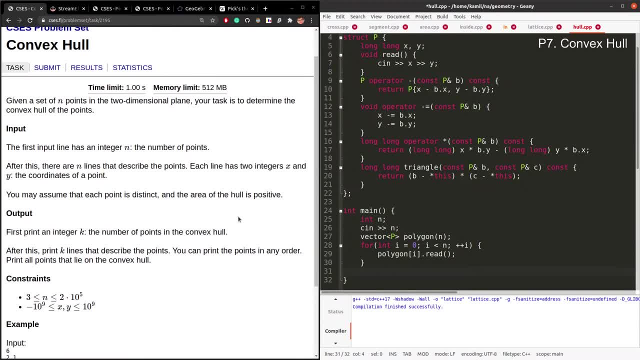 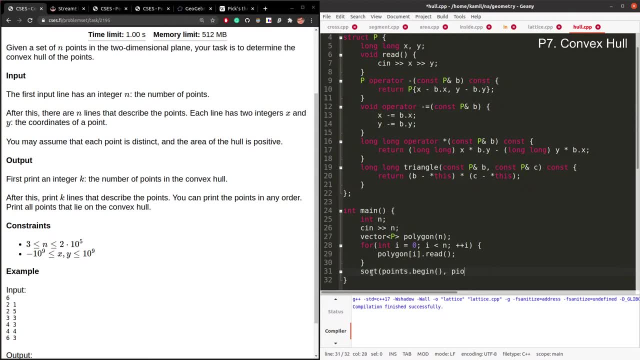 Sort points by x. Let's decide ties in some way. Let's say that, then sort by y. Nice thing with a struct is that you can implement smaller than operator. I will tell it that it should try to first compare by x, then by y. 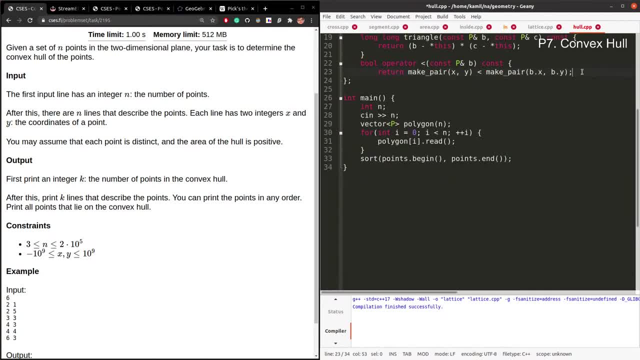 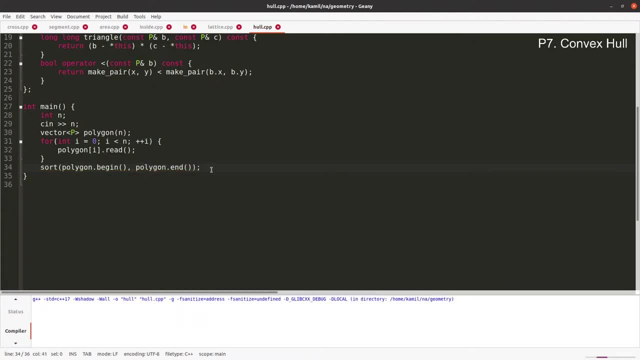 Then sort works Without this operator. sort wouldn't work because it wouldn't know how to sort two points. Oh, this is not a polygon, actually This is just a set of points. Let's call it Points. You sort them, Sort from left to right, Ties decide from bottom up. 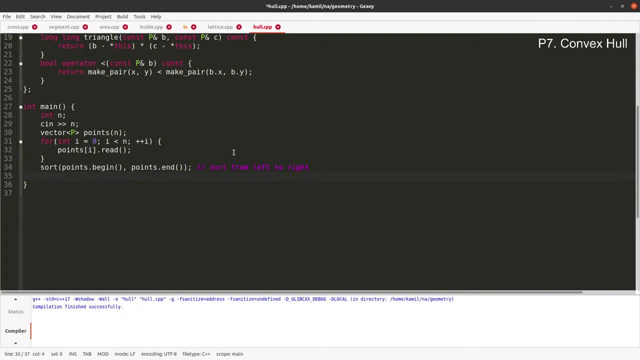 The first point is special. Ignore the first point. Let's say that we already have some part of the convex hull in general. for every new point and new point i call c. i repeatedly will do something like that, for now it's pseudocode. this is second last point. 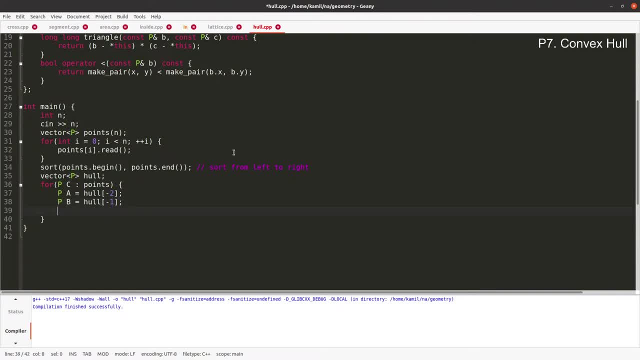 in a convex hole. last point: in a convex hole, again, pseudocode. for now it doesn't compile and i need to check if it goes like this is good shape, a then b, then c. looking from a, b is on the left, on the left, if a dot triangle of bc is negative, b on the left from c, then we need to say good, like, don't do. 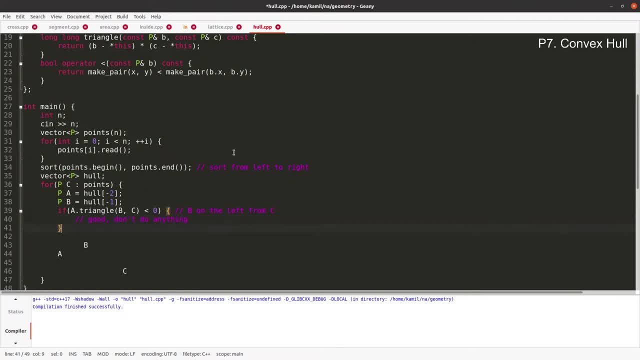 anything like continue. but actually i do this multiple times, multiple times. check the last two points in the convex hole: a, b. check if we have this good shape like a, b, c. remember we consider points from left to right, so it's exactly like this: a, then there is b, then 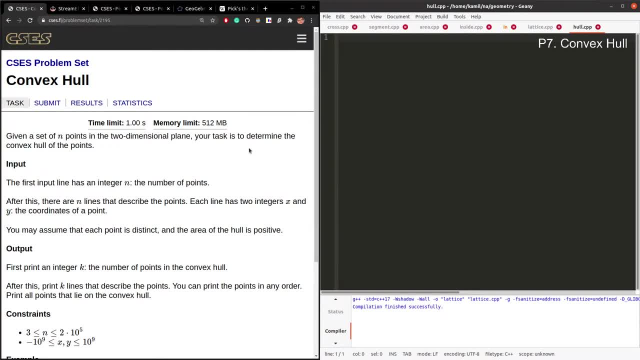 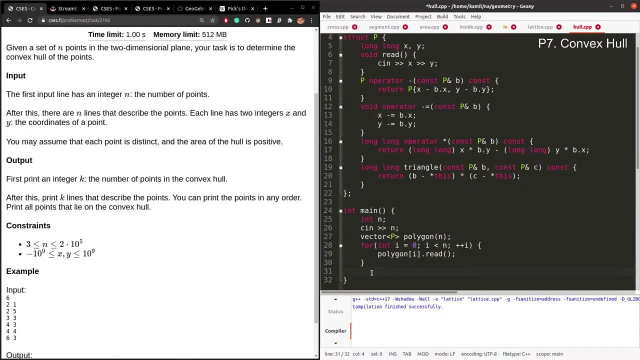 YouTube right. copy paste the short template: geometry template. read the polygon. I will copy paste reading the polygon, because I do it over and over again: sort points by X. let's decide tiles in some way. let's say that. then sort by y. Nice thing with extract is that you can implement. 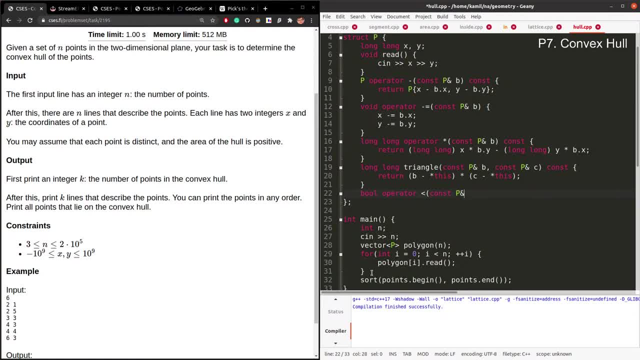 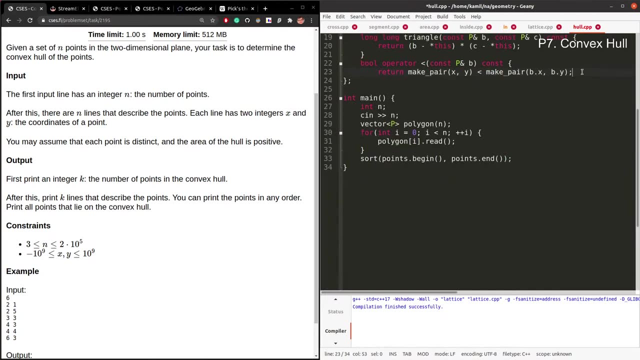 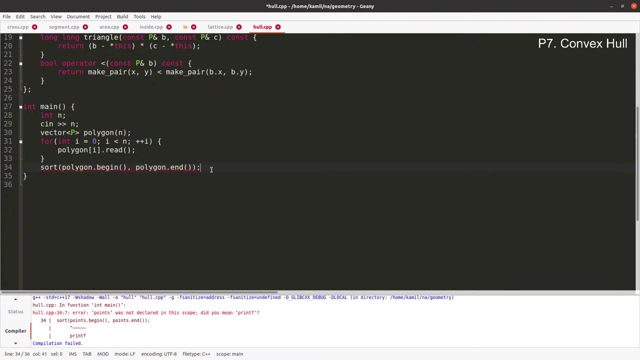 smaller than operator. I will tell it that it should try to first compare by x, then by y, Then sort works. Without this operator, sort wouldn't work, because it wouldn't know how to sort two points. Oh, this is not a polygon, actually, This is. 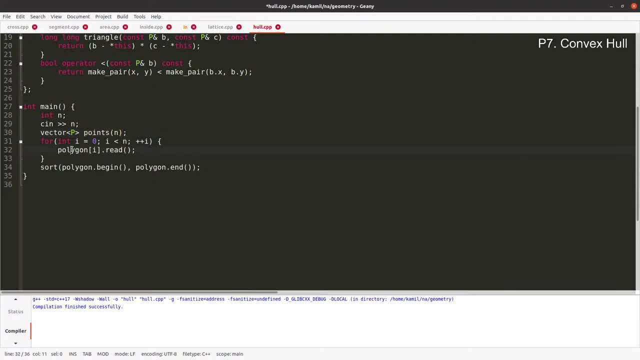 just a set of points, So let's call it points. We sort them, Sort from left to right And ties decide from bottom up. Why not? What now? The first point is special, And let's for now ignore the first point. Let's say that we already have some part. 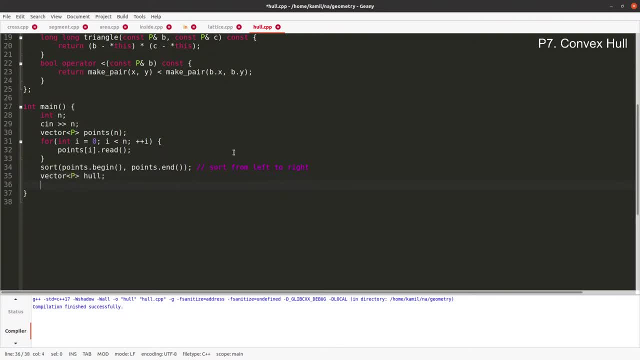 of the convex hole In general. for every new point and new point I call c. I repeatedly will do something like that. For now it's pseudocode. This is second last point in a convex hole. Last point in a convex hole, Again, pseudocode For. 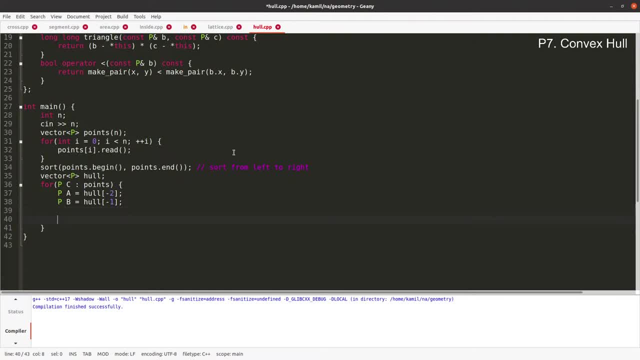 now it doesn't compile And I need to check. if it goes like this, This is good shape: a, then b, then c. Looking from a, b is on the left. On the left, If a dot triangle of b- c is negative, b on the left from c, then we. 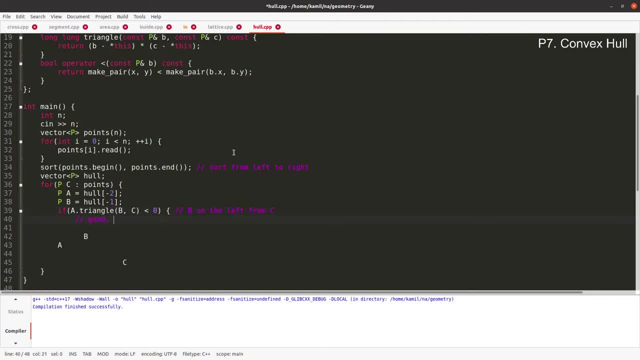 need to say good, Like don't do anything, Like continue. But actually I do this multiple times: Check the last two points in a convex hole, a, b. Check if we have this good shape Like a, b, c. Remember we consider points from left to right, So 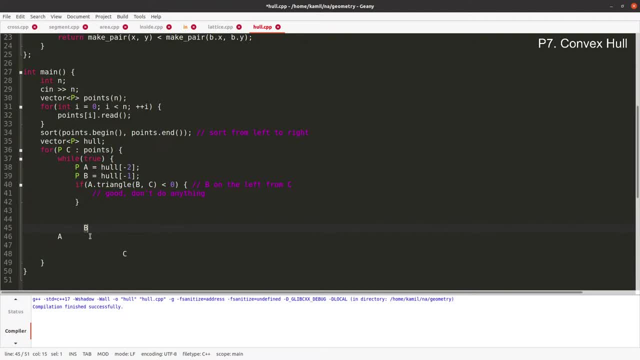 it's exactly like this: a, then there is b, then there is c. Of course, b can be below a, That's it, That's legal. But then we want c to be much lower, For it to be convex. we want, from a, to look at b, and this being more on the left than c. And 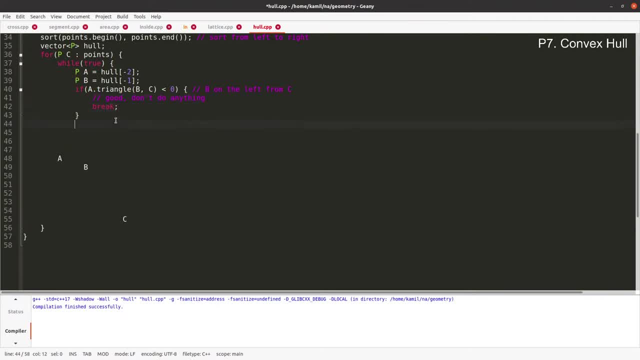 I will say break, But otherwise convex hole dot pop. This removes b Because if it's like this, this is not convex, not top part of the convex hole. We need to pop b because segment is from a to c And while this doesn't compile, this does. 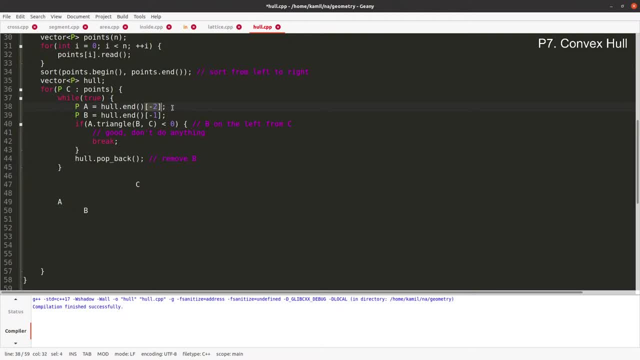 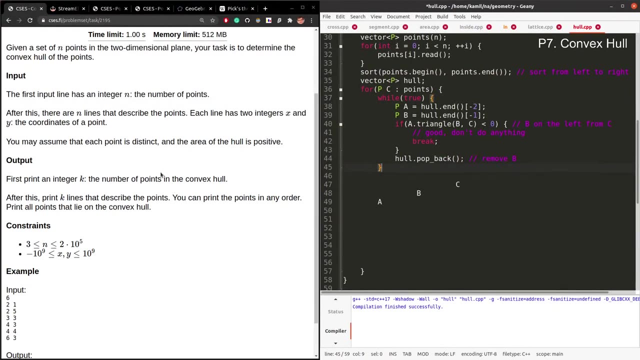 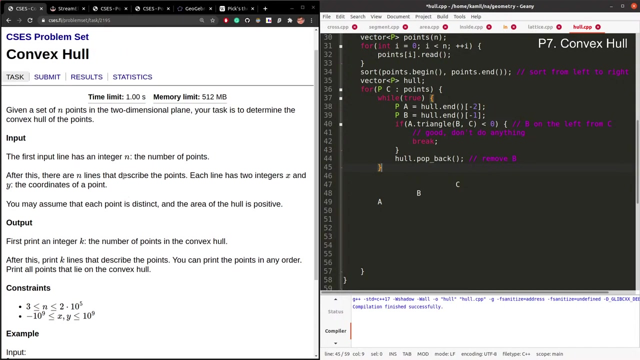 It's not a well-known C++ trick. So this is second last element. and the last element: What about zero? If it's collinear, then we need to look at the statement. what do they want us to do? Whether they are okay with this, We need to know what area of a determined convex. 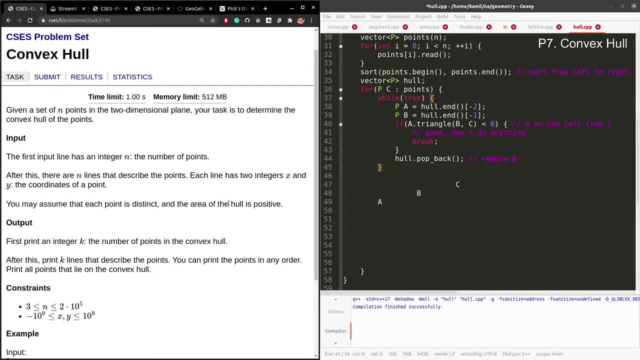 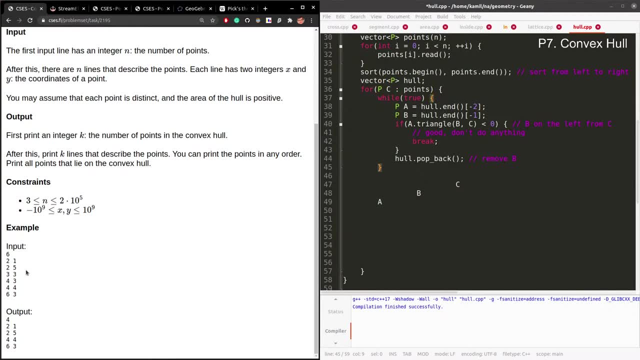 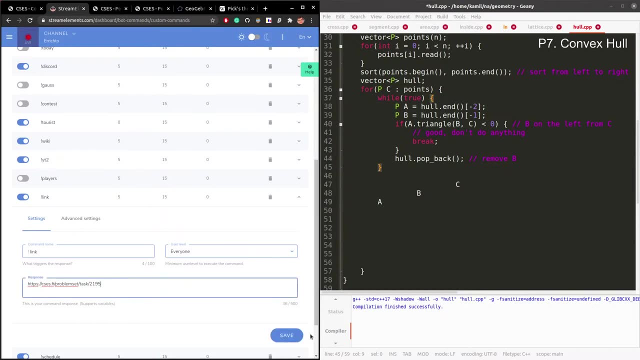 hole, Each point is distinct and area of the hole is positive. Oh, They didn't define. Maybe samples. test specifies that. I forgot to modify the link, Maybe, sorry? yeah, That's right Now, the link is good. we will not solve closest pairs. 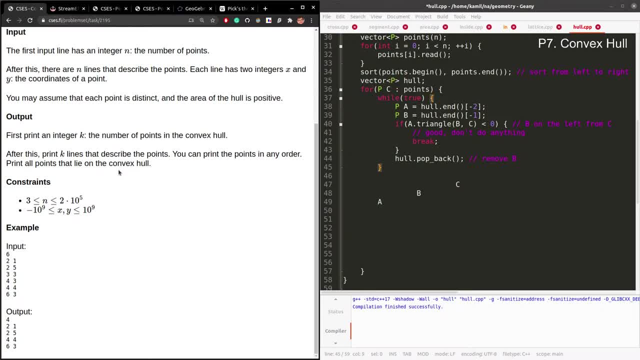 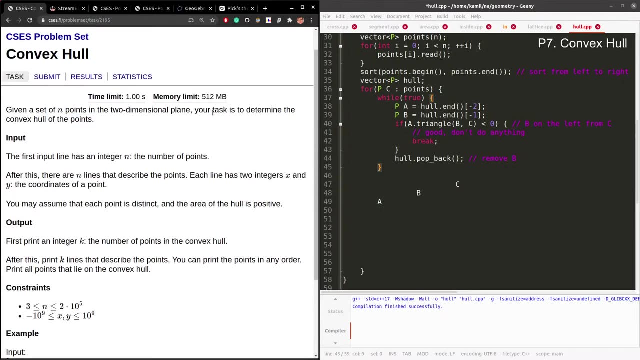 Problem today. I will do it another day because the stream is too long. Okay, Good, The definition of convex isn't obvious. It isn't easy to say if we should grab three consecutive points, I will assume that if it's consecutive then we should remove B and we should assume that B is not a part of. 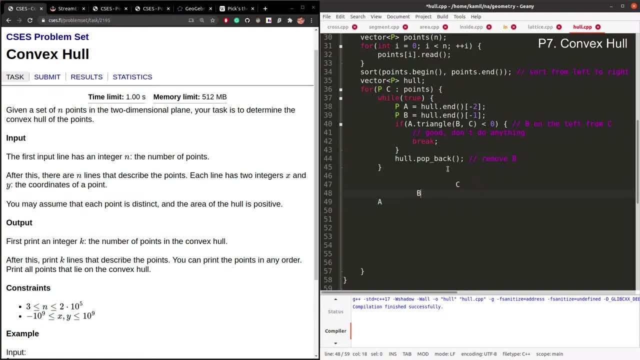 a convex whole. If that's the case, then I will say: if B is on the left, strictly on the left, then break. Otherwise, including this case, including collinear case. So in this case we will remove B. B will not be part of convex whole. that I. 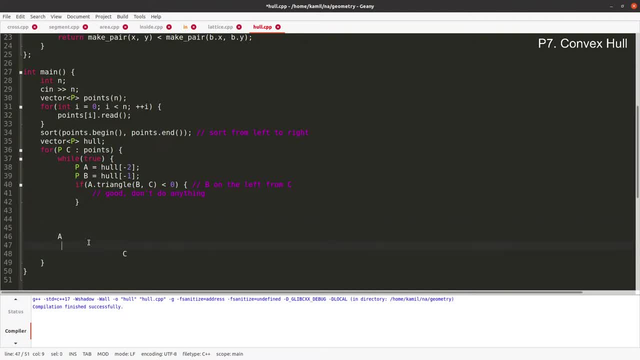 there's c. of course b can be below a. that's that's it, that's legal. but then we want c to be much lower, for it to be convex. we want from a to look at b, and this being more on the left than c, and then i will say break, but otherwise. 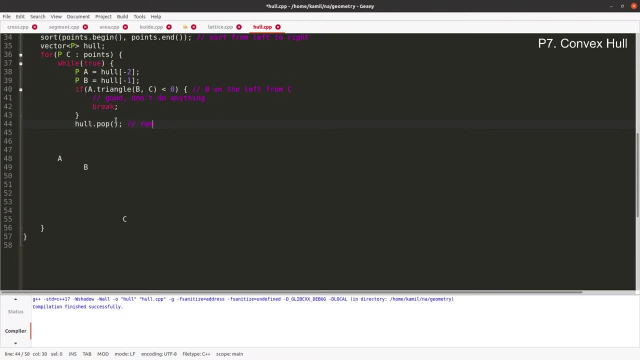 this is a convex hole. dot pop this removes b, because if it's like this, this is not convex, not top part of the convex hole. we need to pop b because segment is from a to c and while this doesn't compile, this does it's not a well-known c++ trick. now this is second. 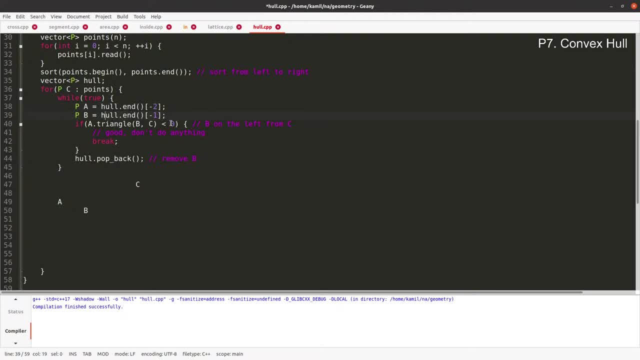 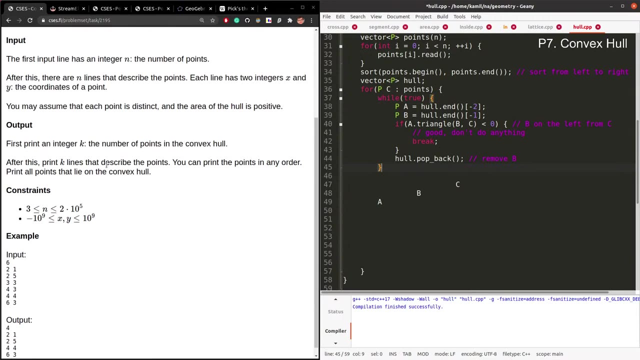 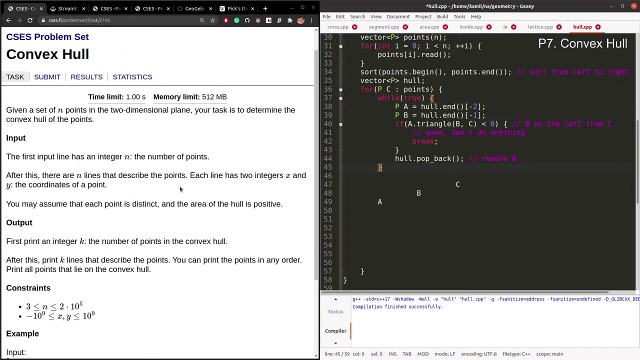 last element. and the last element: what about zero? if it's collinear, then we need to look at the statement. what do they want us to do? whether they are okay with this. we need to know what area determine convex hole. each point is distinct and area of the hole is positive. 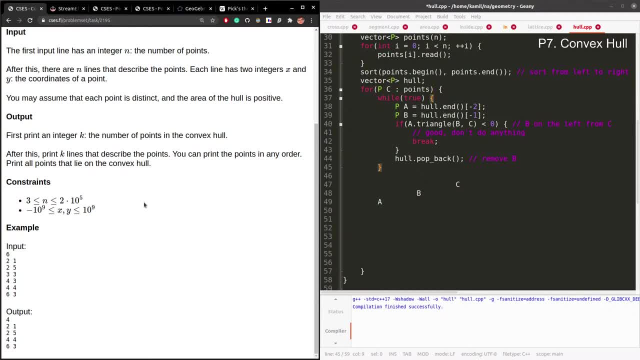 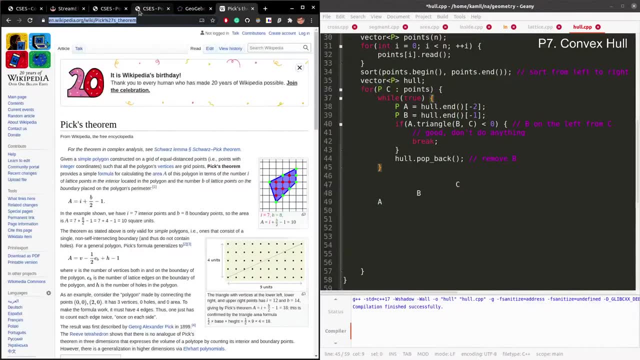 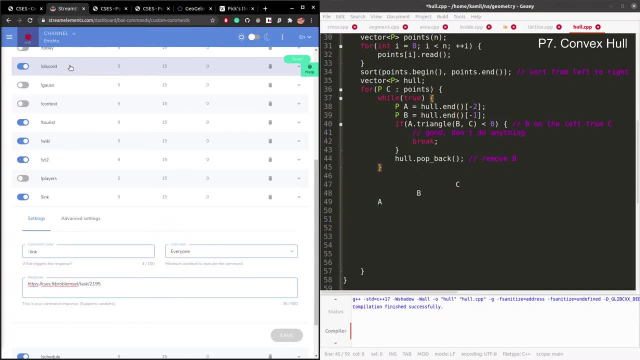 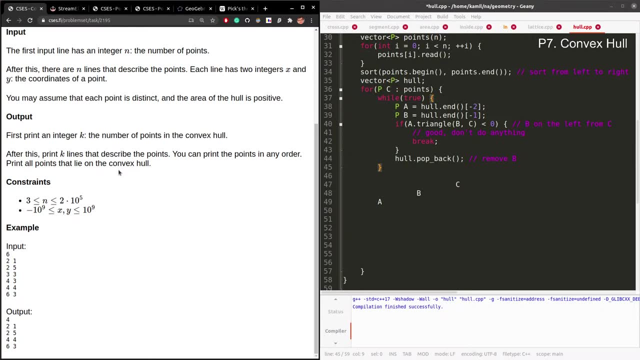 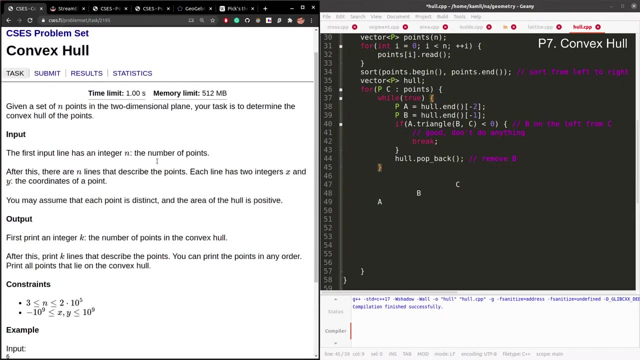 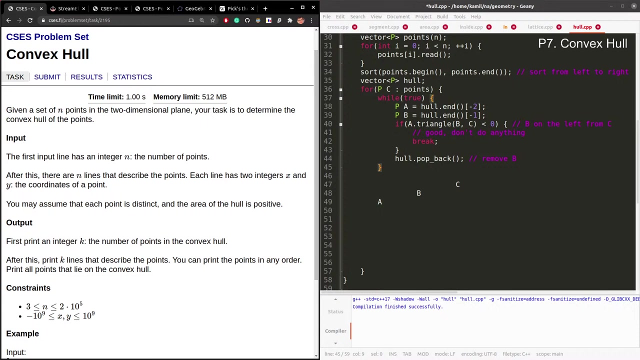 yeah, that's right now. the link is good. we will not solve closet pairs problem. we will not solve closet pairs problem today. i will do it another day. because the stream is too long. so the convex hole- i mean definition of convex- is long, isn't obvious. It isn't easy to say if we should grab three consecutive points. I 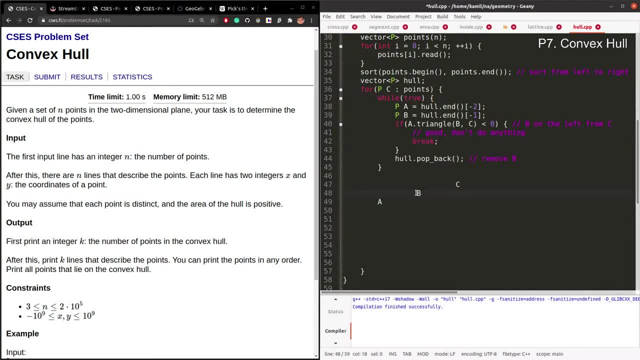 will assume that if it's consecutive, then we should remove B and we should assume that B is not a part of a convex hull. If that's the case, then I will say: if B is on the left, strictly on the left, then break. Otherwise, including this case. 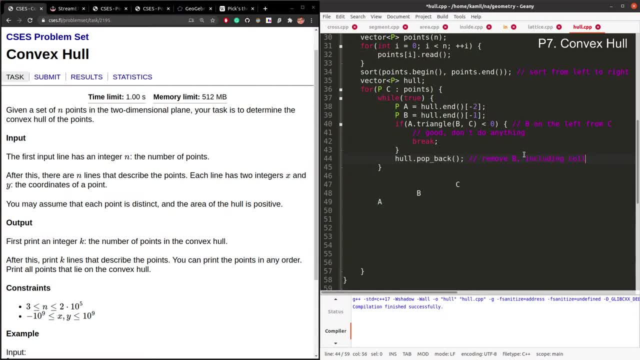 including collinear case. So this in this case we will remove B. B will not be part of convex hull that I print. I don't know if this is what the author wanted. They mean non-concave, I mean. so should we include collinear points or not? If not, then I will just 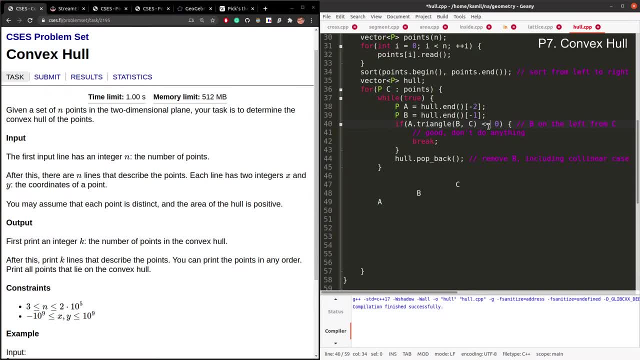 changing this into smaller than or equal to will keep B, Include them right. Keep B Or call linear In this case break, because we say everything is good, All right, I believe you, But if I get wrong answer chat it's your fault. 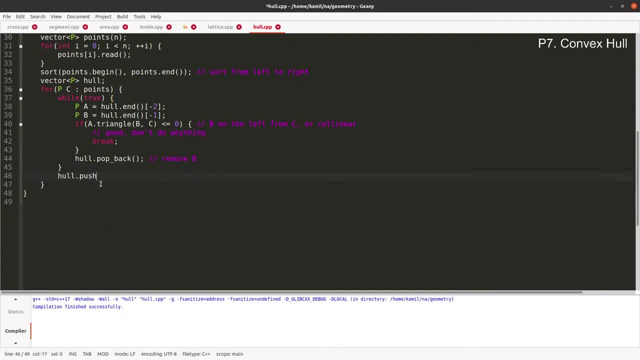 Eventually, whole pushback C, This new point, That's the code. We need to initialize whole in some way. Initially it's empty and I will say that this is enough. If whole size is smaller than two, then just you don't need to check everything. 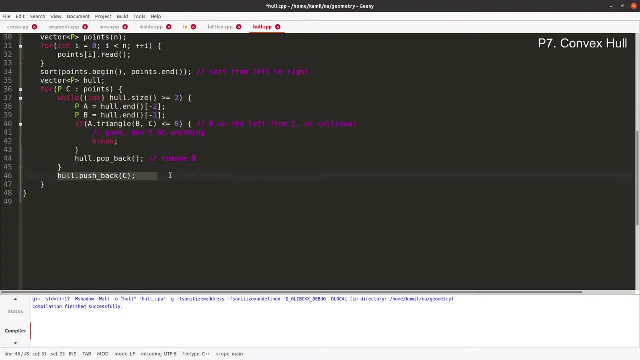 anything, then just whole pushback C. The first two points, the first leftmost points, will be included in the whole. Maybe the second one will be eventually popped. It's that easy, And after this we have the top part of the whole. 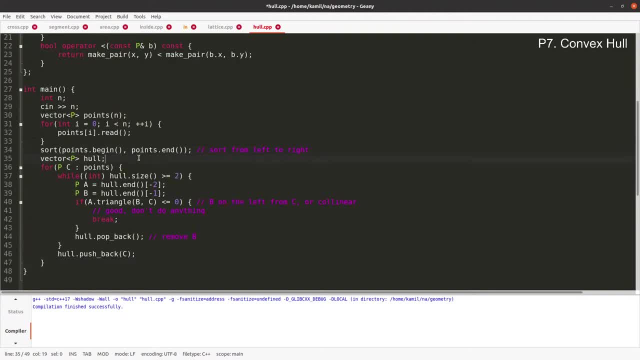 Now, of course, you can rotate the drawing in some way, modify the coordinates of some points, but we can be smarter about this. Repeat twice. Yeah, I think you already figured out that I like repeating something twice. Reverse the points. 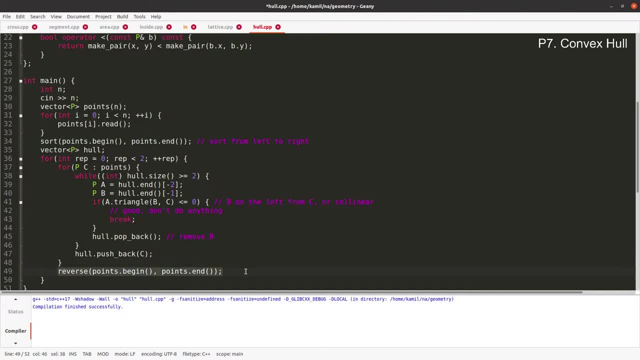 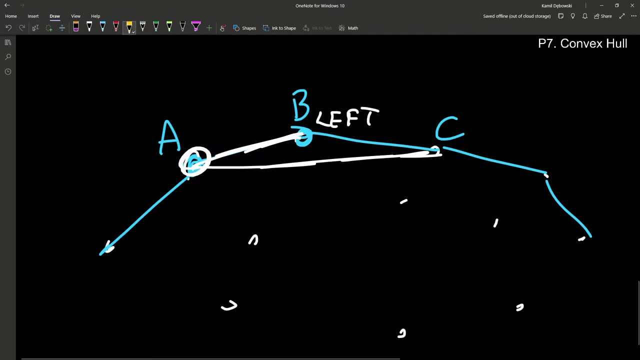 Right, This will go for points from the end, And something surprising is that actually it will find the bottom convex, Because now this what this logic will do: Looking from A, it will want B to be on the left from C, But this is the case for the bottom part. 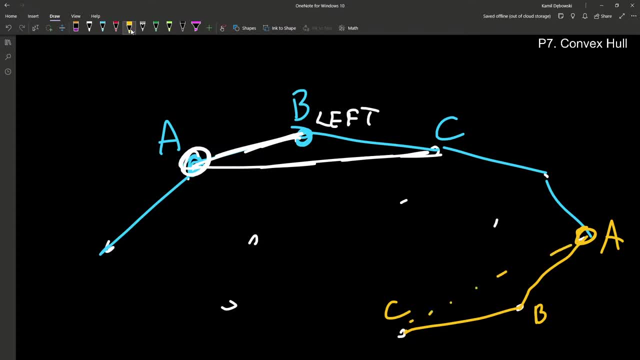 B is on the left from C, Looking from A. We don't need to do anything else. It will find this thing. Actually, what my program will print, it will print this point, then that, that, that, that and this. 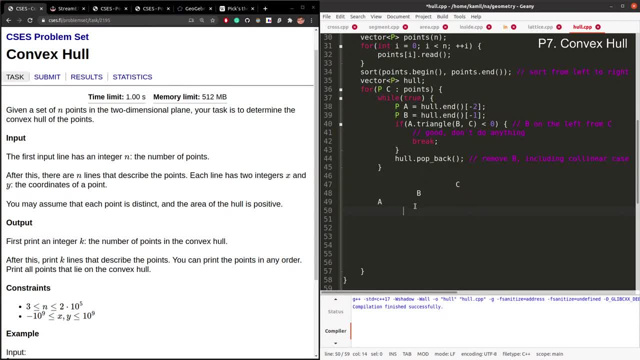 print. I don't know if this is what author wanted. They mean non-concave, I mean. So should we include collinear points or not? Yes, If not, then I will just you know. changing this into smaller than or equal to will. 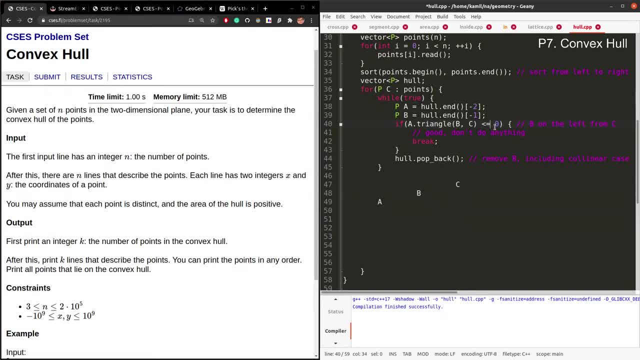 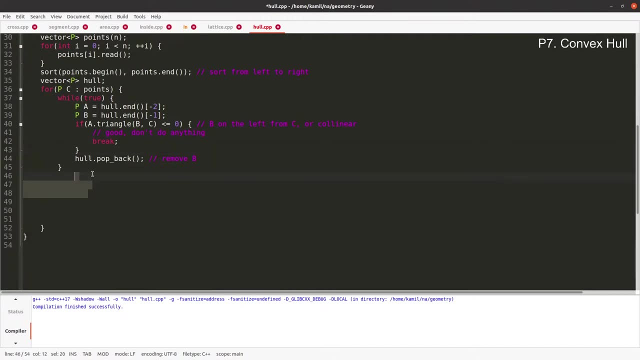 keep B, Include them right. Keep B Or collinear In this case, break because we say everything is good. Alright, I believe you, But if I get wrong answer, chat it's your fault. Eventually, who'll push? 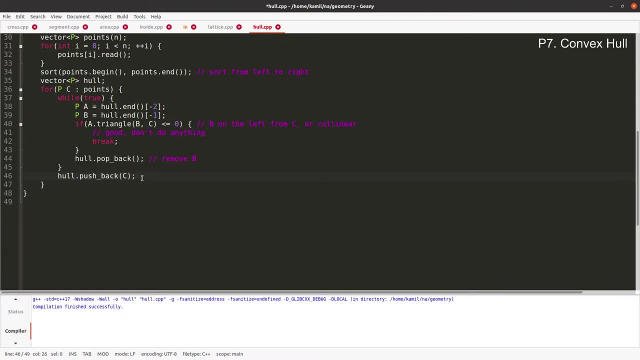 back. Push back C, This new point. That's the code. We need to initialize whole in some way. Initially it's empty and I will say that this is enough. If whole size is smaller than two, then just you don't need to check everything, anything, then just whole push. 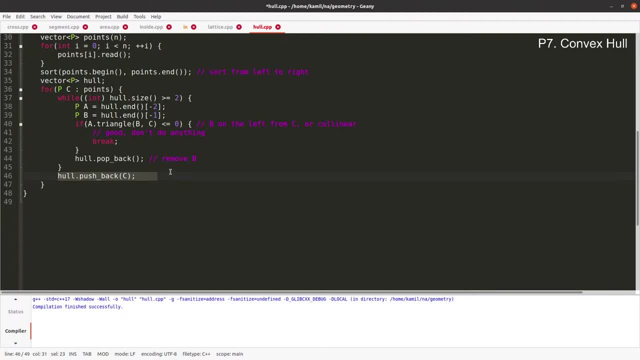 back. C. The first two points, the first leftmost points, the first two leftmost points, will be included in the whole. Okay, Okay, Okay, Maybe the second one will be eventually popped. It's that easy. And after this we have the. 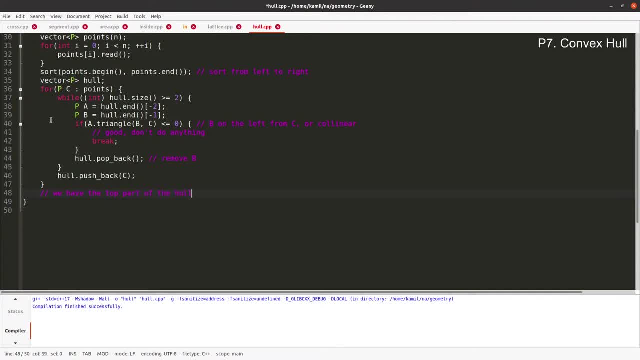 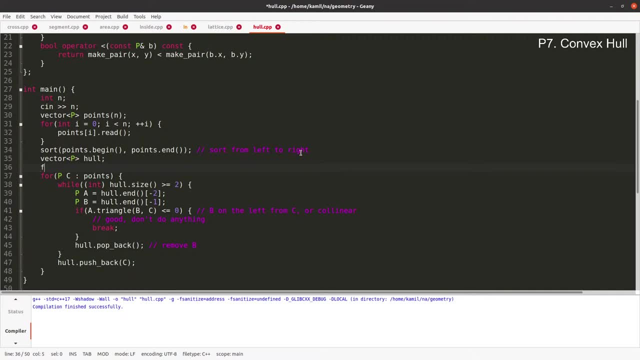 top part of the whole. Now, of course, you can rotate the drawing in some way, modify the coordinates of some points, but we can be smarter about this. Repeat twice. I think you already figured out that I like repeating something twice. 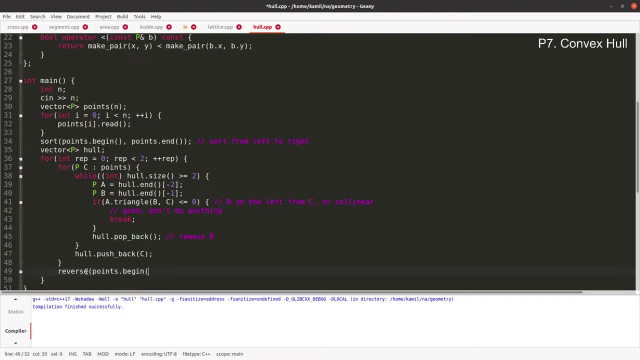 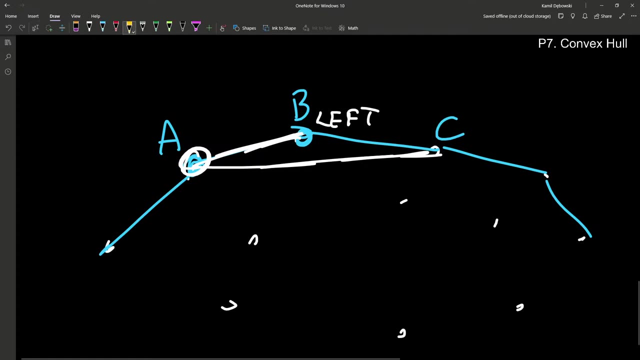 If all the things have a size, just reverse the points. Alright, This will go for points from the end, And something surprising is that actually it will find the bottom convex, Because notice what this logic will do. Looking from A, it part B is on the left. from C looking from A. We don't need to do anything else. 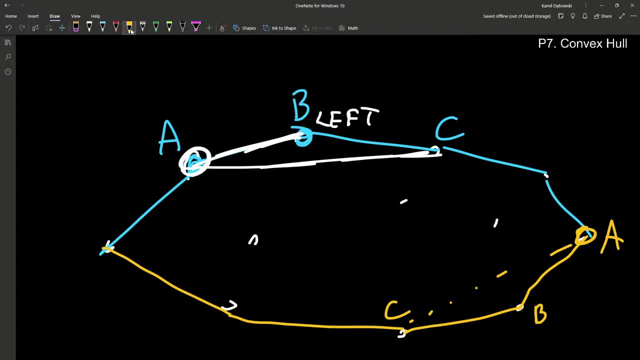 It will find this thing, Actually, what my program will print. it will print this point, then that, that, that, that and this, and then it will print the rightmost one again, then this, this, that, that, So that leftmost and rightmost points are doubled. 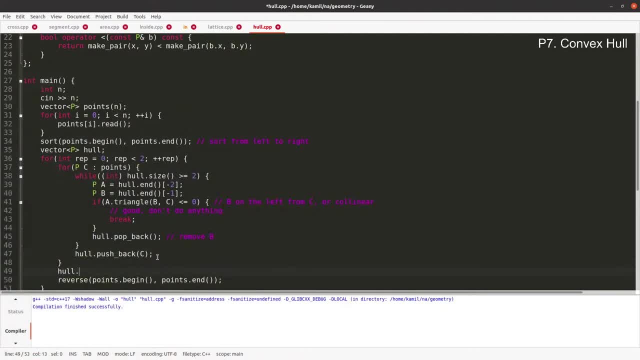 That's bad For that. this is the fix: Remove rightmost point. This is just because I repeat twice and I don't want this leftmost and rightmost to appear twice. And the last thing is that, because I repeat, this part becomes. 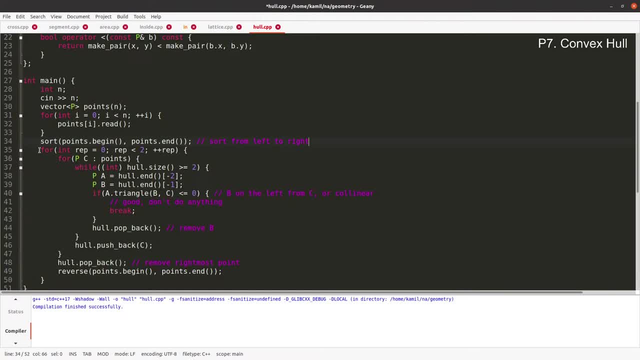 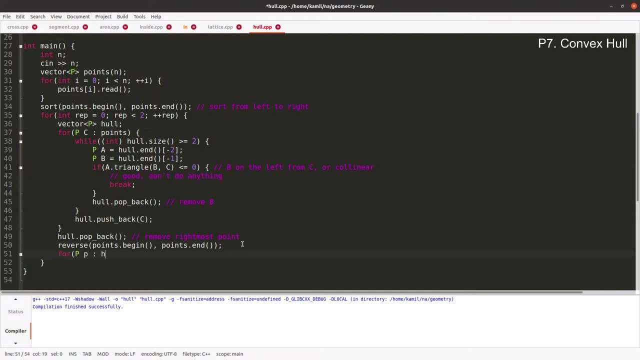 invisible. And the last thing is that because, I repeat, this part becomes invisible, valid, Like what I should really do is right, this is possible, right, and now I can print those points, But later I will tell you what I would really do. 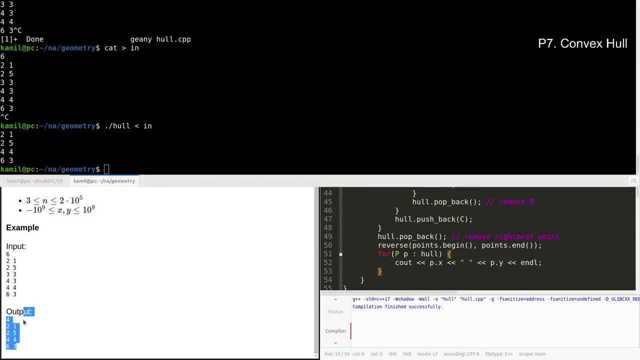 2, 1, 2, 5, 4, 4, 5, 6,, 7,, 8,, 9, 10.. 6, 3.. All right, good, but also I need to print the number of numbers. and now it's fine if you do this. 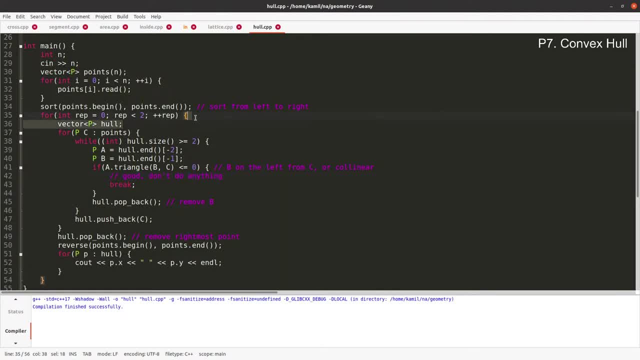 But I do it almost always we need to gather the full whole, Including both top and bottom part. and I do this strange trick where I declare whole ones and then, After I find top part, Sure, I pop back the last element. But then in the second run, this: it seems that this, while loop, changes definition a little bit. 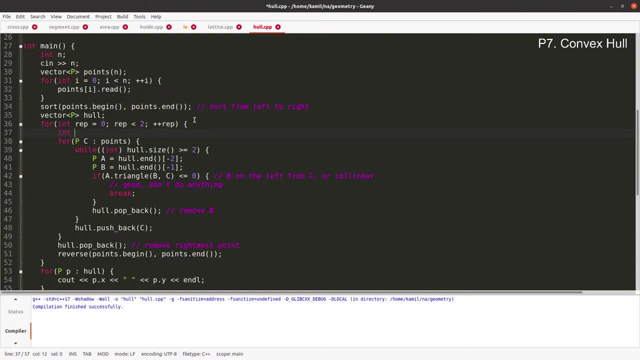 so Memo size, how to call it? Let's say s initial size is whole dot size. I will kind of magically change this to s plus 2, and it is a hack. If whole is empty initially, then s is 0, so this change does nothing. But if whole already contained five elements from the first run, 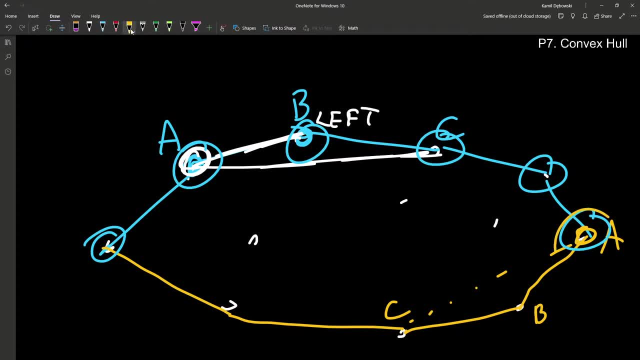 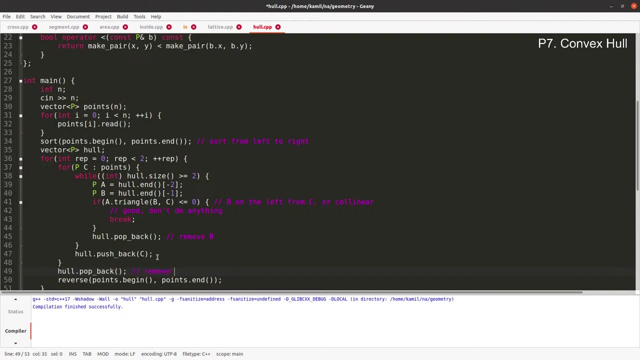 And then it will print the rightmost one again, Then this, This, That, That, So that leftmost and rightmost points are doubled. That's bad. For that. this is the fix: Remove rightmost point. This is just because I repeat twice and I don't want this leftmost and rightmost to appear twice. 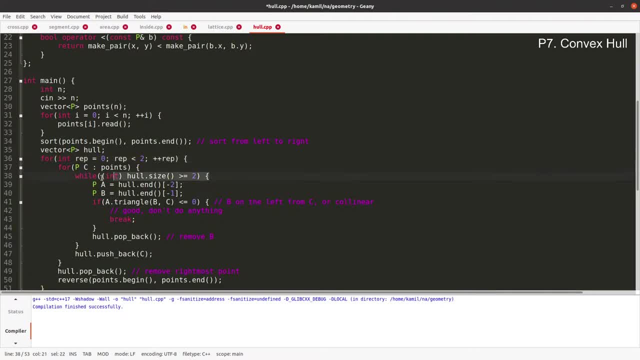 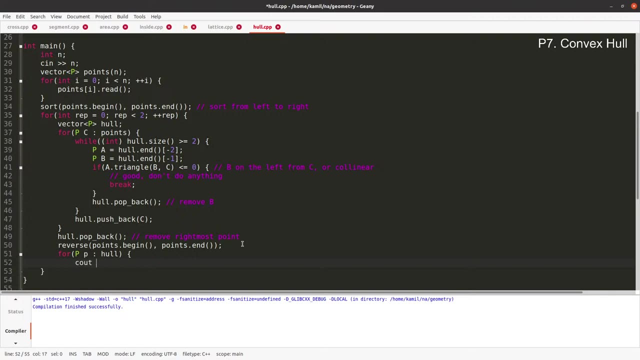 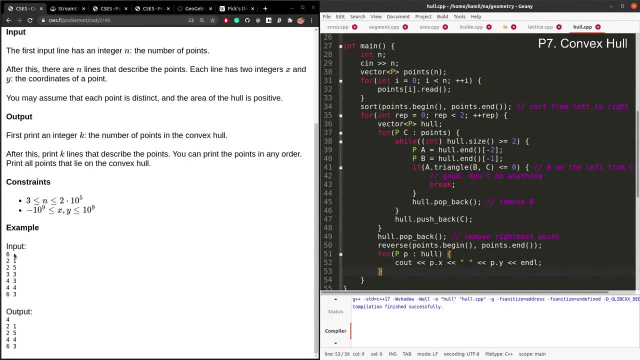 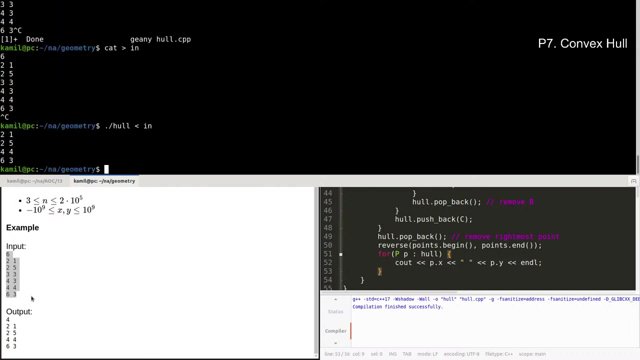 And the last thing is that, because I repeat, this part becomes invalid, Like what I should really do. Alright, this is possible, Right, and now I can print those points, But later I will tell you what I would really do: 2, 1, 2, 5, 4, 4, 6, 3.. Alright, good, 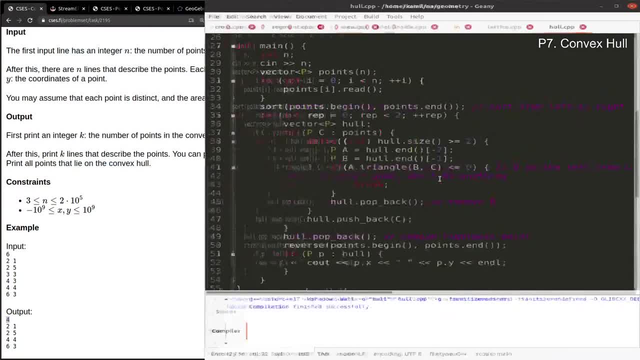 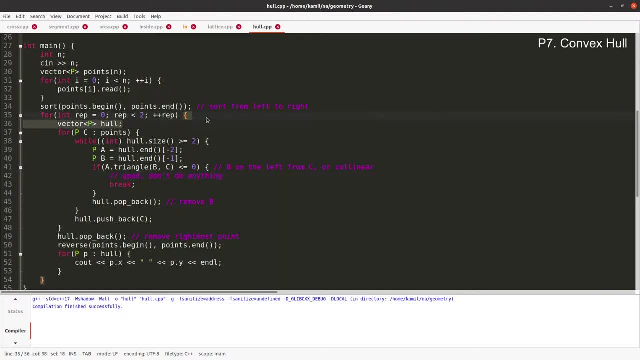 But also I need to print the number of numbers. And now it's fine if you do this, But I do it almost always. We need to gather the full whole, including both top and bottom part, And I do this strange trick where I declare whole once. 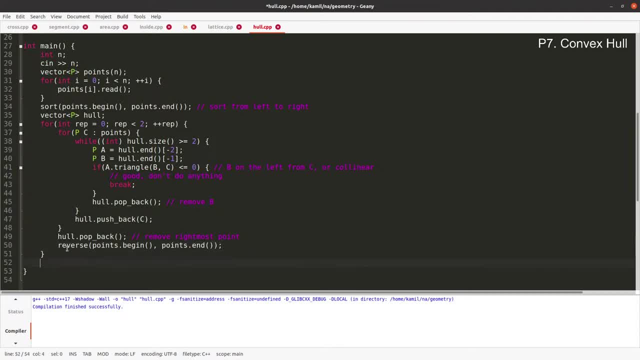 And then after I find top part, sure I pop back the last element. But then in the second run, this: It seems that this while loop changes definition a little bit. So Memo size, how to call it? let's say s initial size is whole dot size. 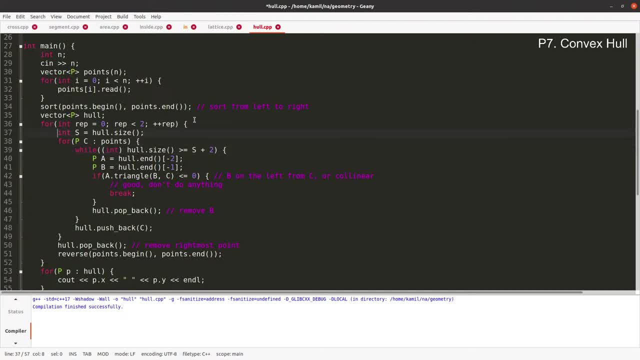 I will kind of magically change this to s plus 2.. And it is a hack. If whole is empty initially, then s is zero, So this change does nothing. But if whole already contained five elements from the first run, then here I want my vector to think that those five elements don't exist. 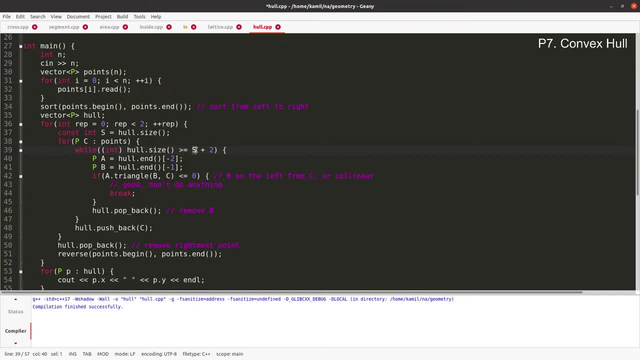 Then here, like I want my vector to think that those five elements don't exist, So if whole size is now six instead of five, I only have one element. Maybe it's better to think about it like that. This difference is the number of new elements, Because I don't want to. 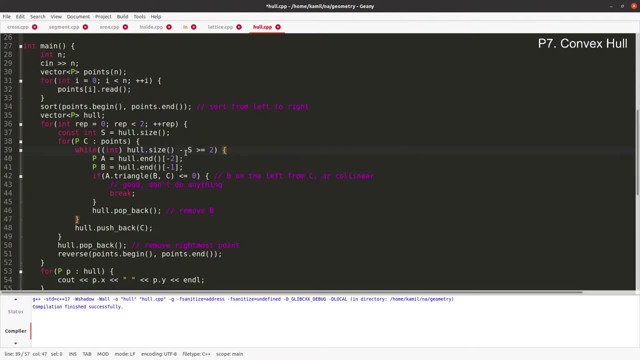 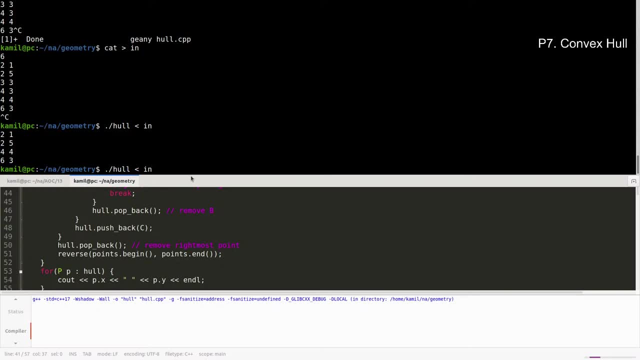 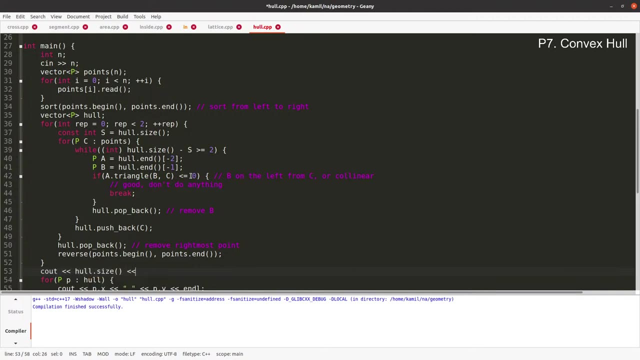 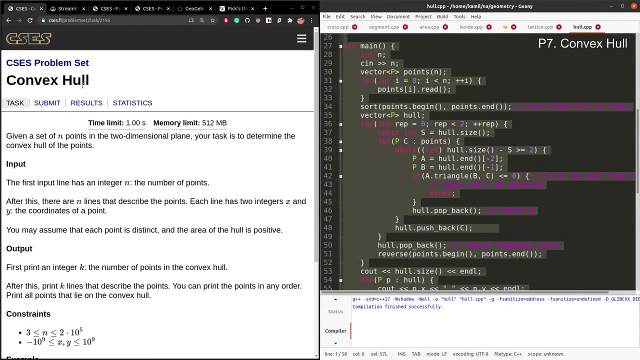 Access elements from the previous part to make it independent. This is how I implement and I'm not saying that this is the best method, but it works. I printed the same thing and now print also whole dot size. Let's submit, but there are a lot of things that I could mess up. 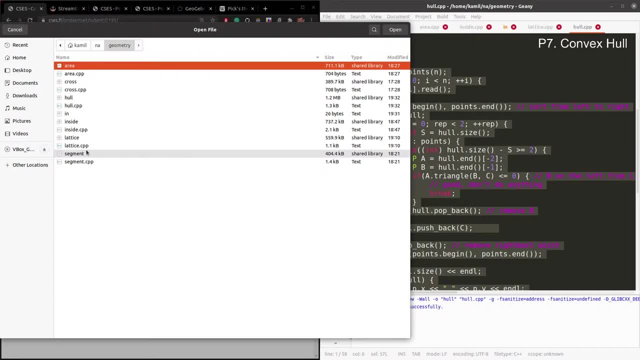 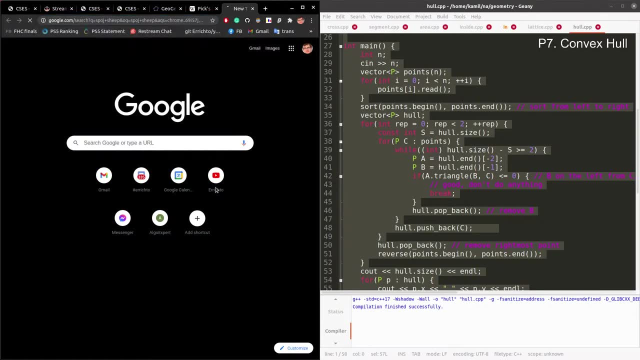 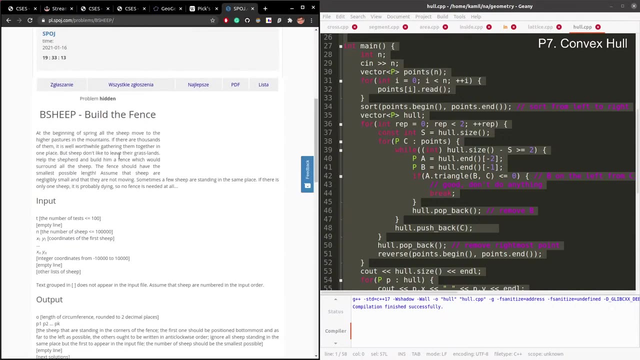 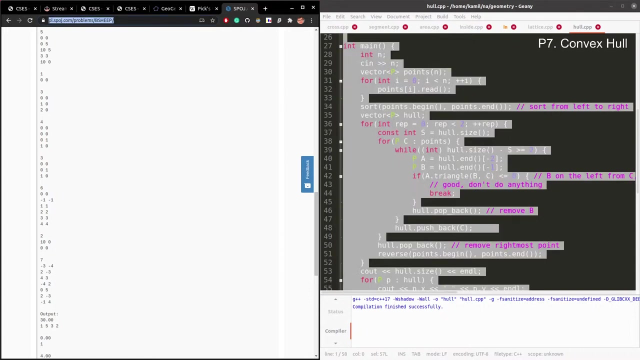 convex whole isn't an easy algorithm to get right. If you want harder version, I believe that SPOI ship is the hardest possible version, Where you need to care about edge cases like two ships, two ship being in the same point, Is it? or yeah, yeah, okay this. remember this as 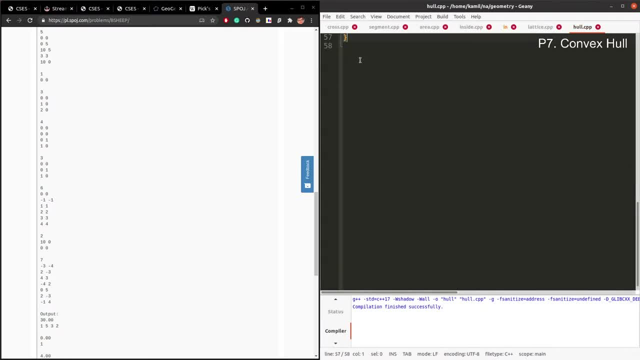 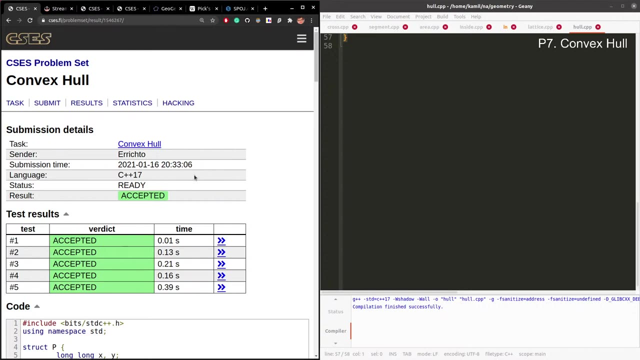 Very tricky version where you need to deal with the degenerate cases out of points in the same point. hard version. If you are a beginner, I don't. I don't recommend convex will accept. right. What is convex? sorry, what is concave pull here? what do you mean? I? 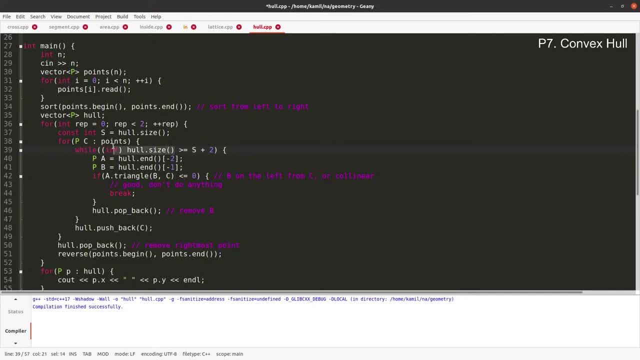 So if whole size is now six instead of five, I only have one element. Maybe it's better to think about it like that. This difference is the number of new elements, Because I don't want to access elements from the previous part to make it. 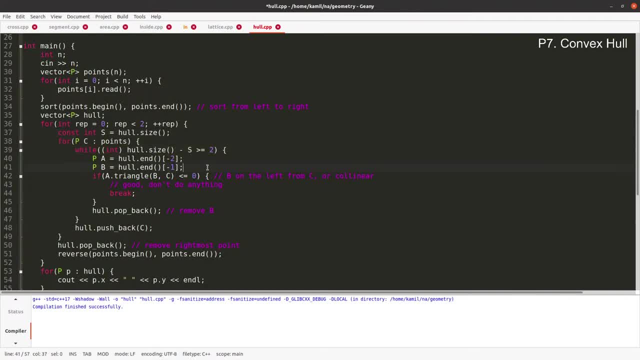 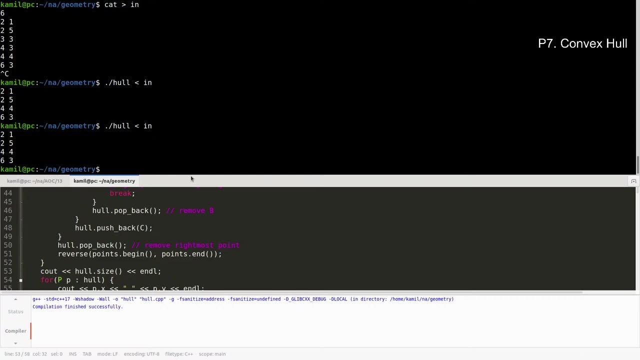 in the first run. It's independent. This is how I implement and I'm not saying that this is the best method, But it works. I printed the same thing and now let's print also whole dot size, Let's submit. but there are a lot of things that I could mess up. 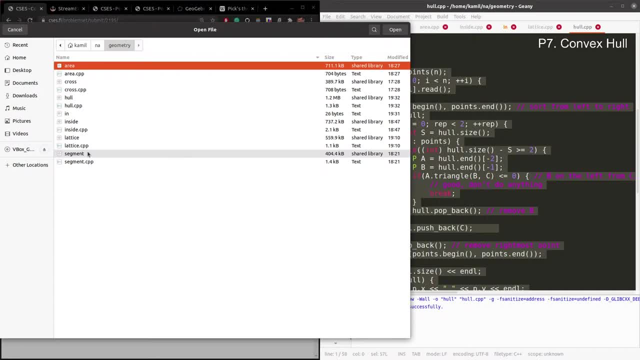 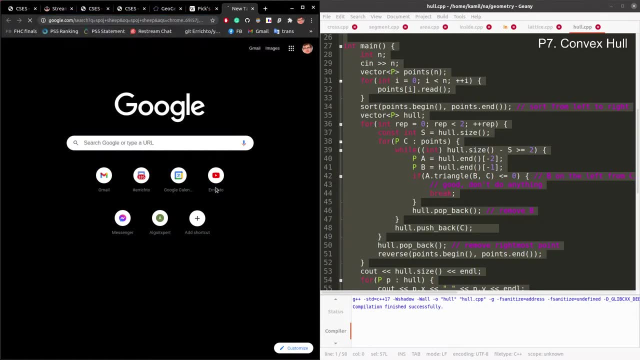 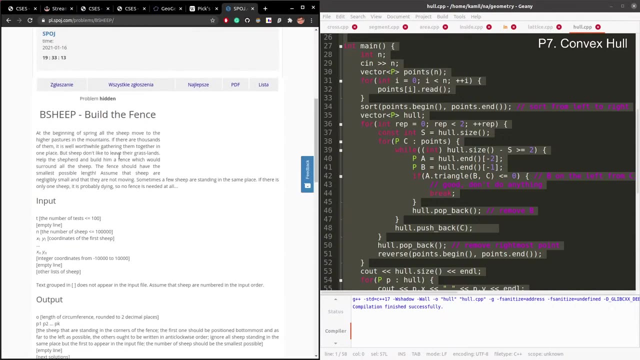 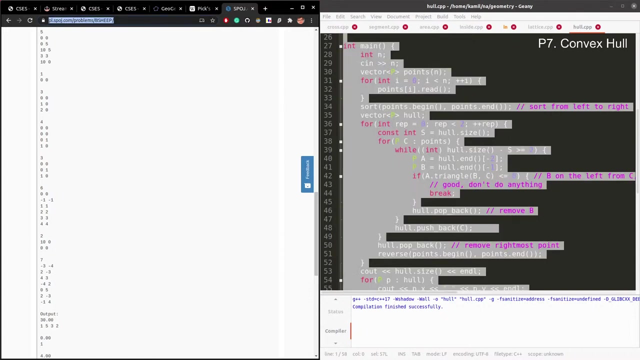 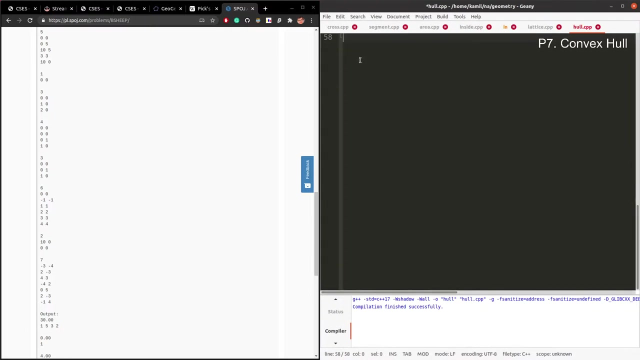 Convex whole isn't an easy algorithm to get right. If you want harder version, I believe that SPOI ship is the hardest possible version where you need to care about edge cases Like two ships being in the same point. Remember this as a very tricky version where you need to deal with. 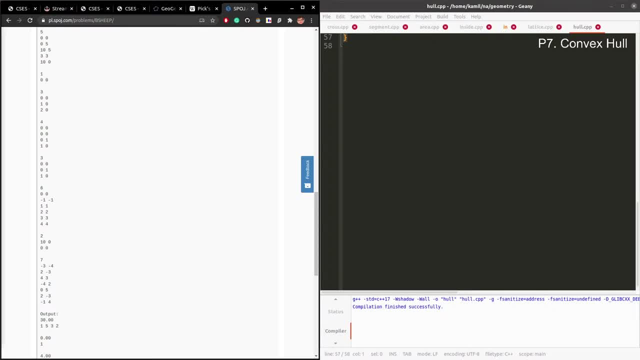 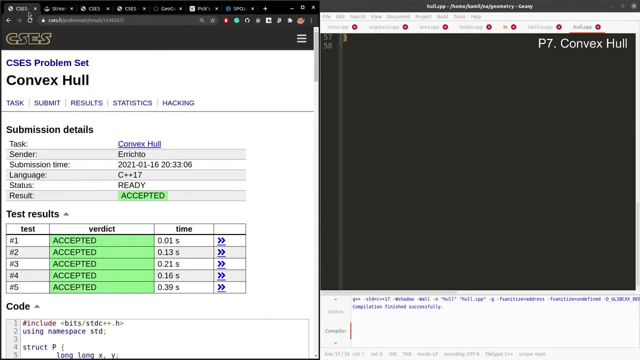 degenerate cases. A lot of points in the same point. Hard version. If you are a beginner, I don't recommend it. Convex whole- accepted, All right. What is concave whole Skier? what do you mean? I have no idea what concave whole is. 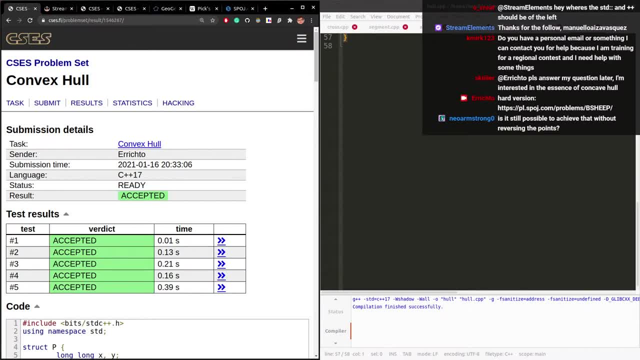 And I have personal email. I mean I cannot answer everybody. You can join the Discord server but I cannot talk in private with everybody. You know you can write to me a messaging, for example, code versus Discord. I mean you can construct it, just concave outer points, just not convex. 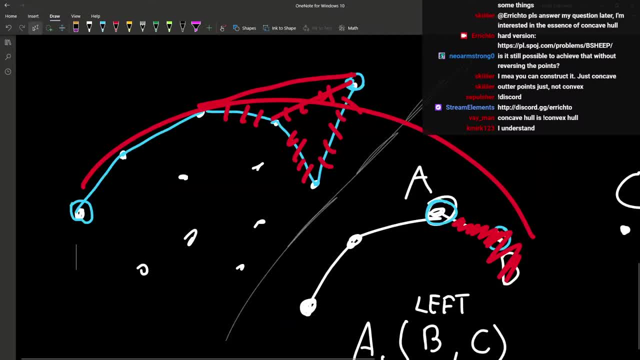 What is that? I have no idea. Like you need to define something in order to find it For this set of points. what is concave whole? You can connect points in any way. You can change signs in that code to the opposite and see what happens. 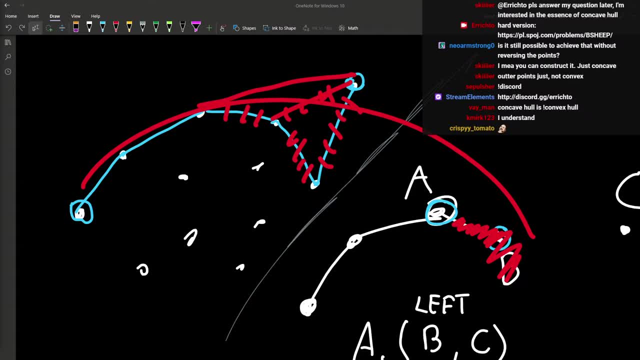 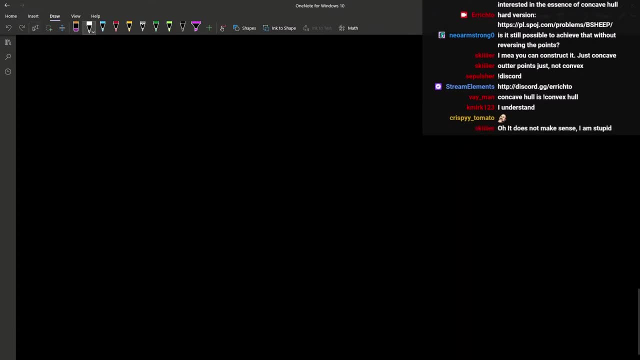 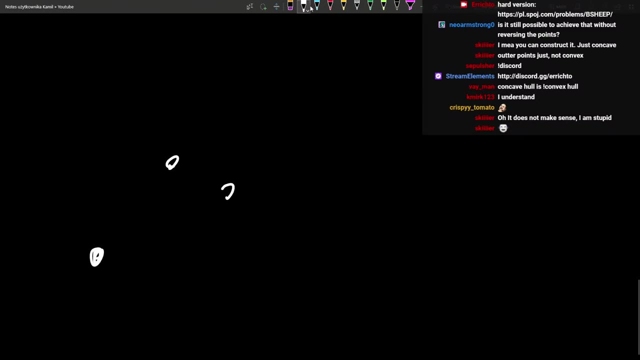 But I think it will be garbage. Achieve that without reversing points. Yes, it is Another version. another way to implement it is to grab leftmost point And now say that instead of going from left to right, you go angle-wise. 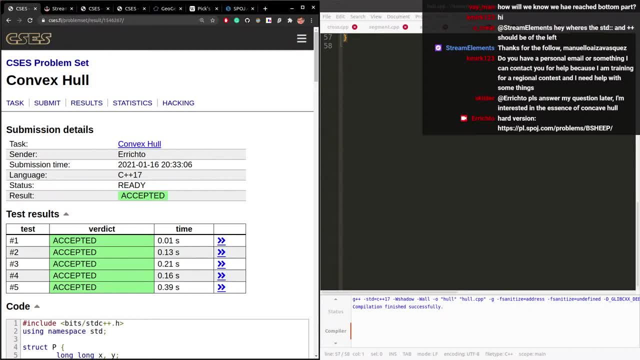 Have no idea what concave pull is. I Have And I have personal email. I mean I Cannot answer everybody. you can join the discord server. I Cannot talk in private with everybody, you know. you can write to me a message in, for example, code versus discord: I. 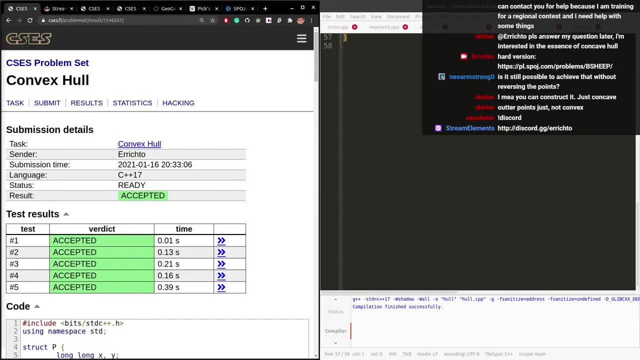 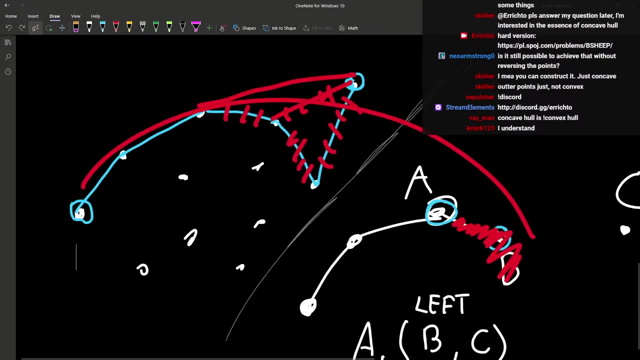 Mean: you can construct it, just concave outer points, just not convex. What is that? I Have no idea. click: you need to define something in order to find it For this set of points. What is concave? pull: you can connect con points in any way. 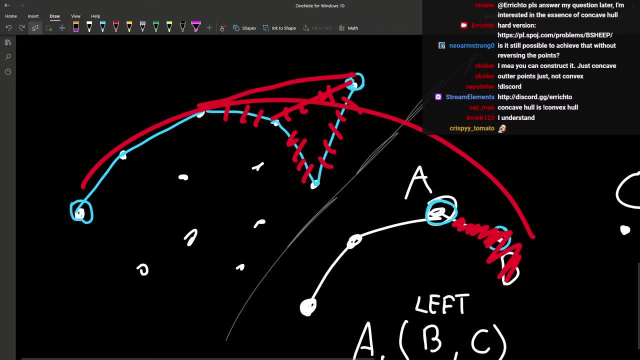 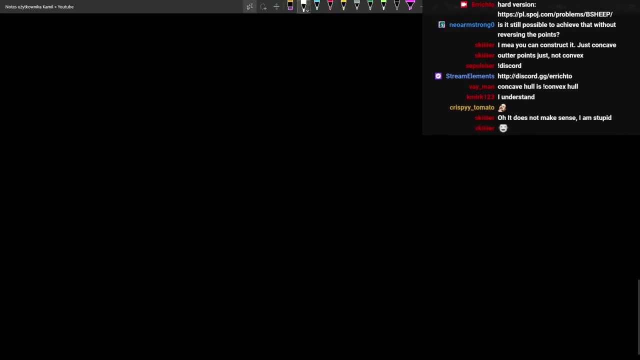 You can change signs in that code to the opposite and see what happens, but I think it will be garbage. Achieve that without reversing points. Yes, it is another version. another way to implement it is To grab leftmost point and Now say that instead of going from left to right, you go angle wise. 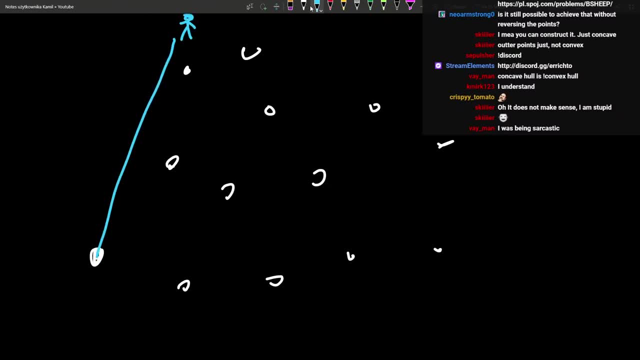 So imagine that our guy starts here with a rope but then ends here. I mean here, and For that you need to sort points by angle. with respect to p1, You need to consider them not from left to right, but in order: one, two, three, four. 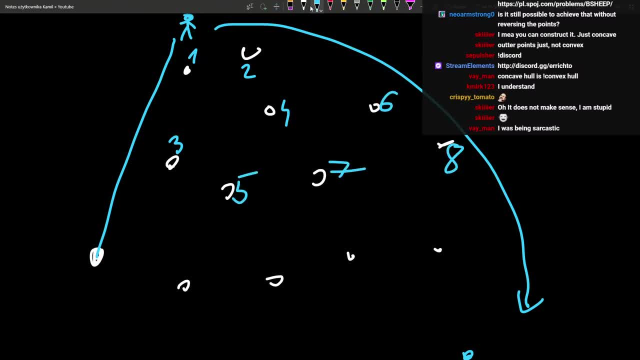 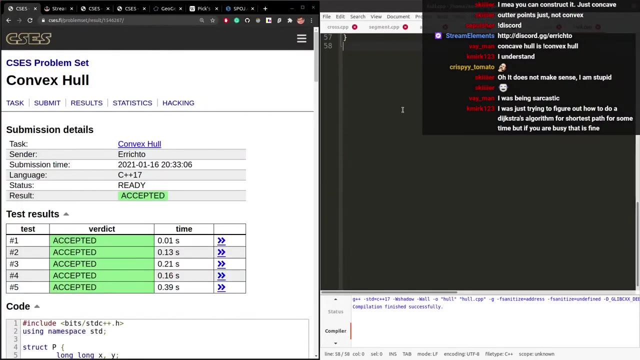 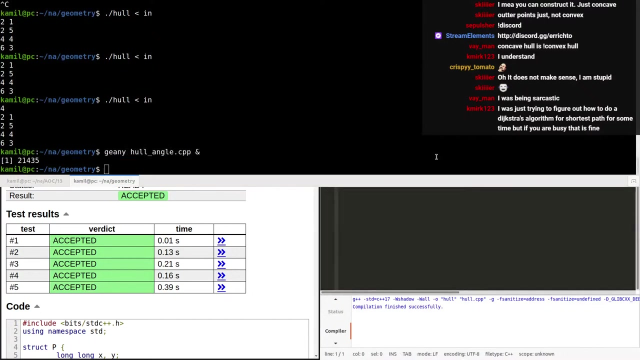 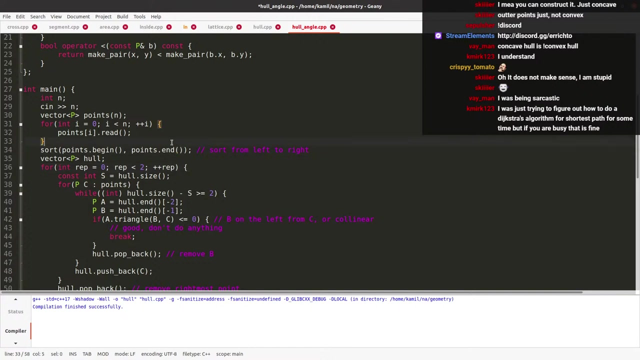 five, six, seven, eight, something like that- nine, ten, eleven, twelve- Sort them like this and then run the same algorithm. This is very easy to do, so I Don't see why shouldn't I modify my code a little bit. cool angle Now, without the two parts Sort points, and this time I want to sort them by angle. with respect to the first point, the leftmost point, 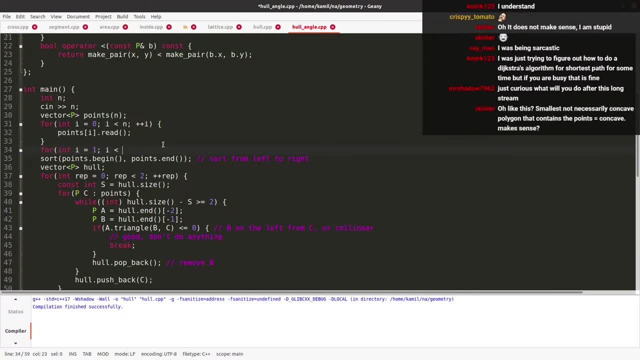 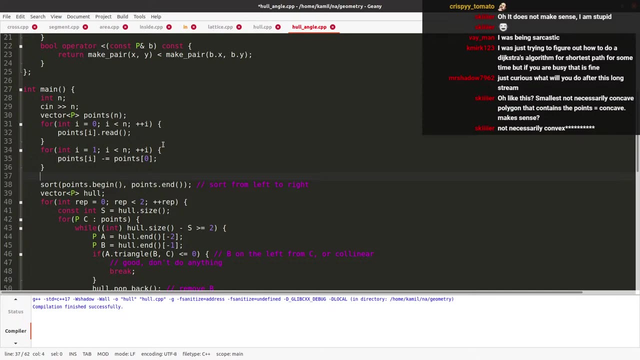 What do I need to do? For my convenience, because always I check with respect to p zero. I say points of I minus equal points of zero. Now Everything assumes that point zero is zero, zero. I don't sort all points. I sort all except for the first one. 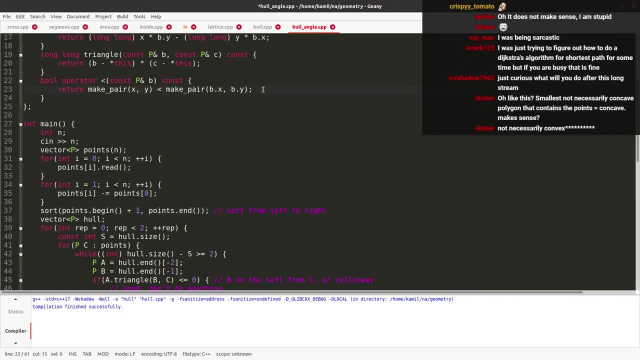 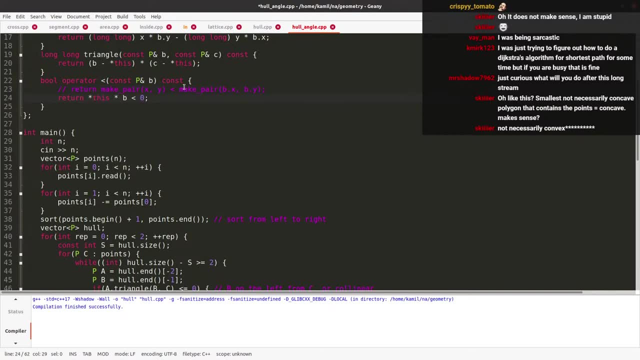 and now I change this to To what? to comparing by angle, Cross product of me and some other point is smaller than zero. if I'm more on the left, So then I want to say that I'm smaller than him. then this sorts points by angle With respect to zero. zero now, after I shifted. 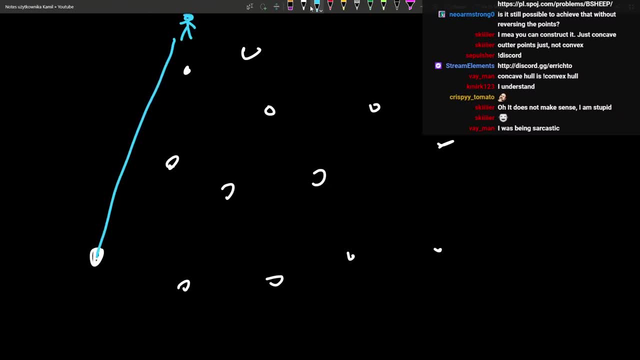 So imagine that our guy starts here with a rope but then ends here- I mean here- And for that you need to sort points by angle with respect to P1.. You need to consider them not from left to right, but in order: 1,, 2,, 3, 4,, 5,, 6,, 7, 8, something like that. 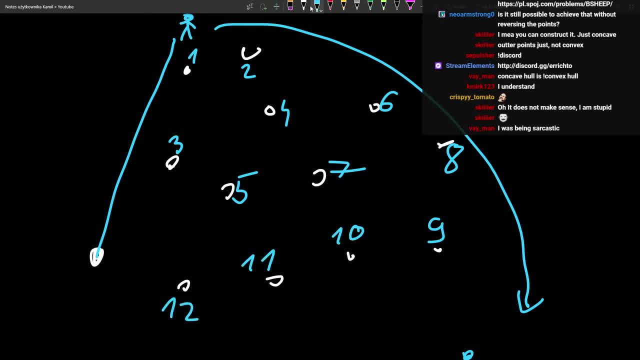 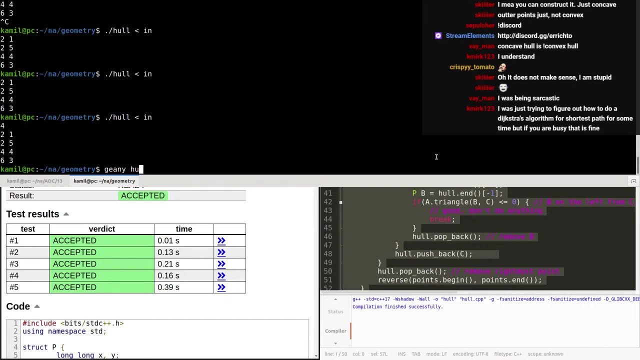 9,, 10,, 11, 12.. Sort them like this and then run the same algorithm. This is very easy to do, So I don't see why shouldn't I modify my code a little bit. Cool angle Now without the two parts. 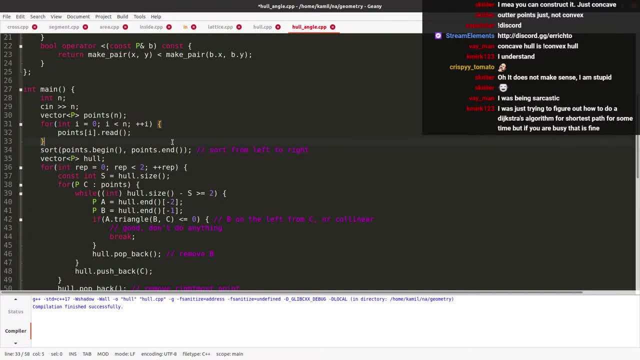 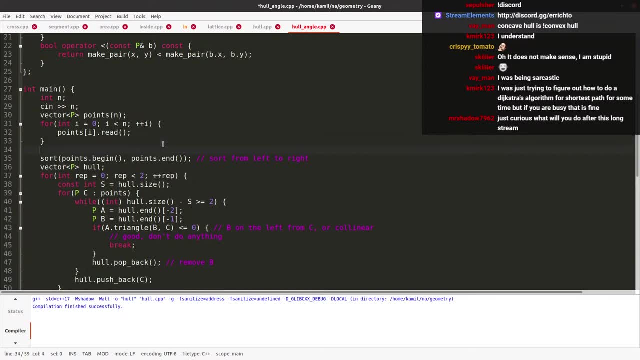 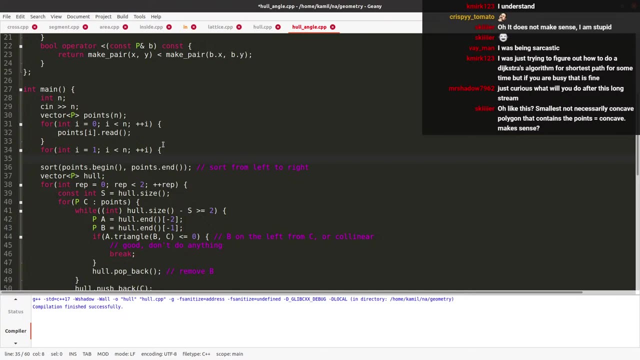 Sort points and this time I want to sort them by angle. with respect to the first point, the leftmost point, What do I need to do For my convenience, because always I check with respect to P0, I say points of i minus equal. 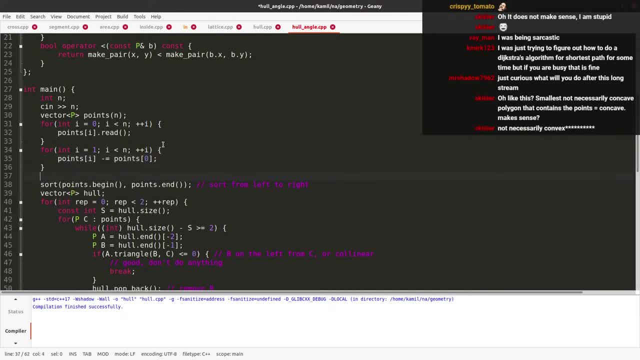 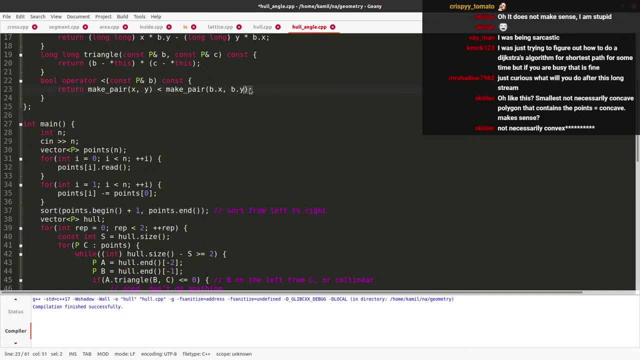 points of 0. Now everything assumes that point 0 is 0, 0.. I don't sort all points. I sort all except for the first one. And now I change this to comparing by angle Cross product of me. and some other point is smaller than 0 if I'm more on the left. 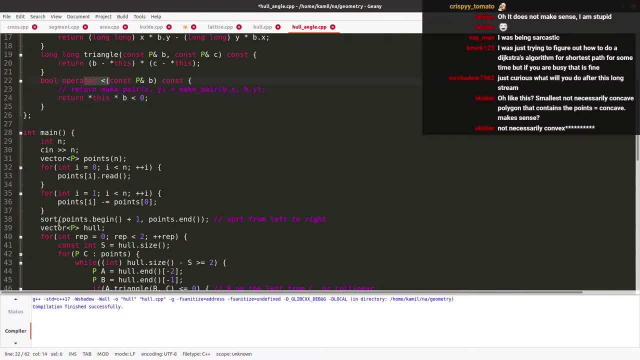 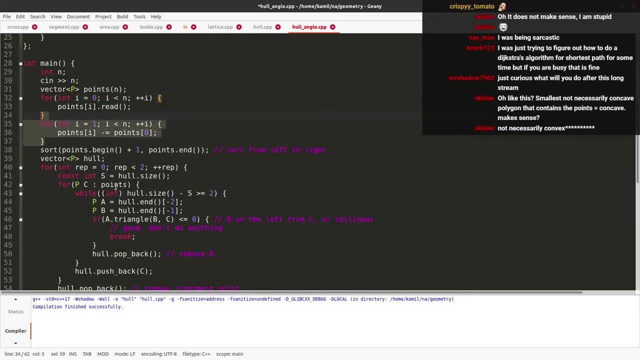 So then I want to say that I'm smaller than him. Then this sorts points by angle with respect to 0, 0. now, after I shifted Hull initially, I need to push back P of 0, 0. Because what I want to happen is I want to say that hull is like this point: 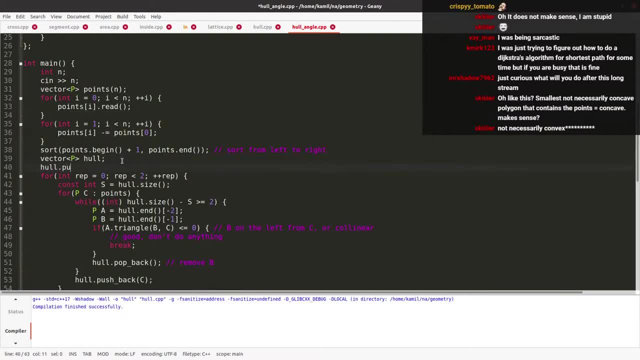 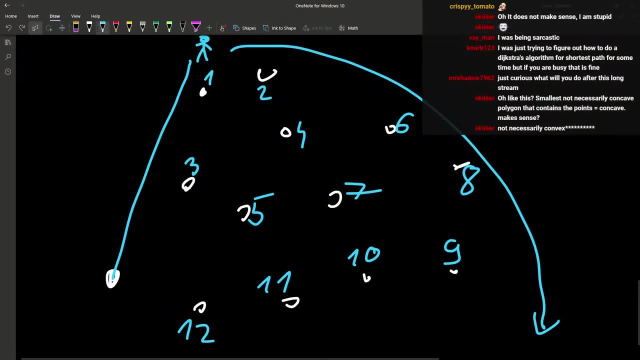 I need to. I need to Push back p of zero, zero, Because what I want to happen is I want to say that hole is Like this point, then say this point, then this point, and you know we continue Temporarily. it will be like that This will be popped and we will just have this, and so I want partial 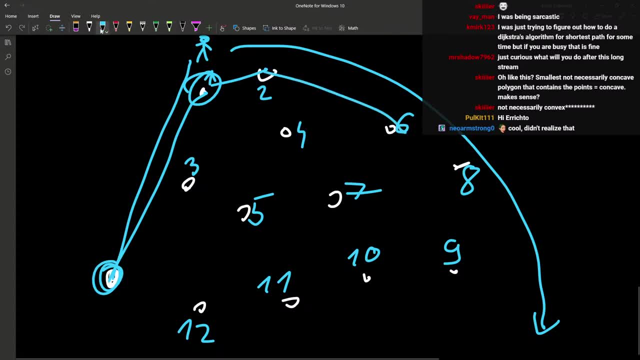 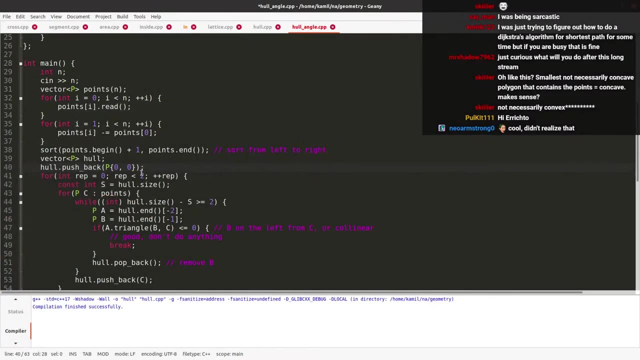 Convex hole to start from here and be maybe with different color. This is partial convex hole we have, maybe temporarily it's like that, but then eight will pop seven. it will be like this: All right now for all the points, except for the first one, This new point C. 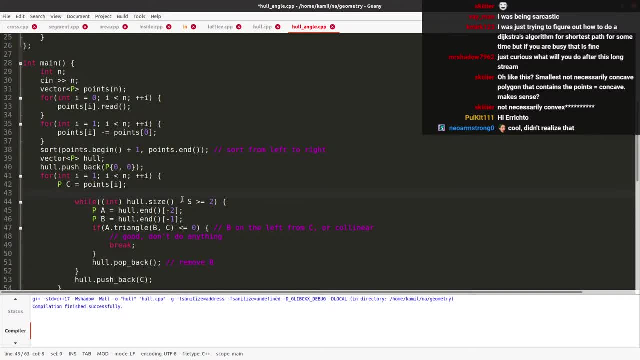 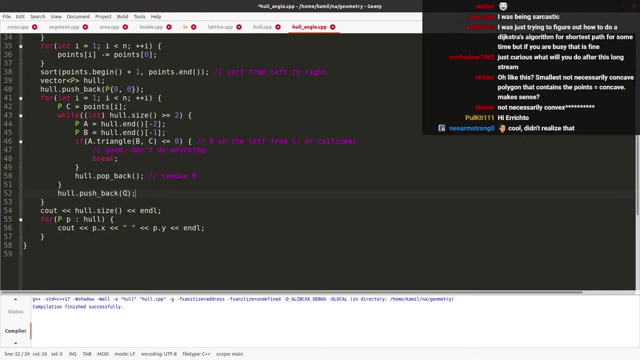 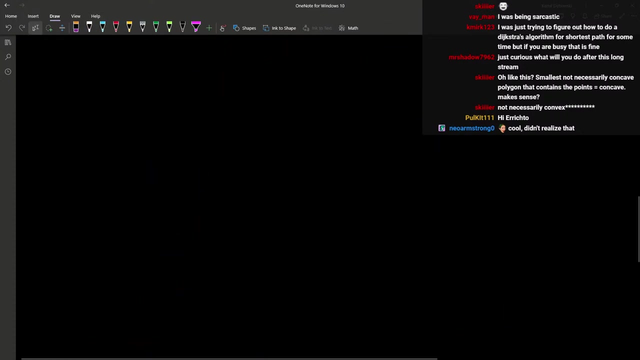 And what do we do? this I'll hole. size is at least two. consider popping, the logic doesn't change. then hole, push back C. All right, and this is almost good, Because at the end we might get some garbage. We might have something like this, Can we? 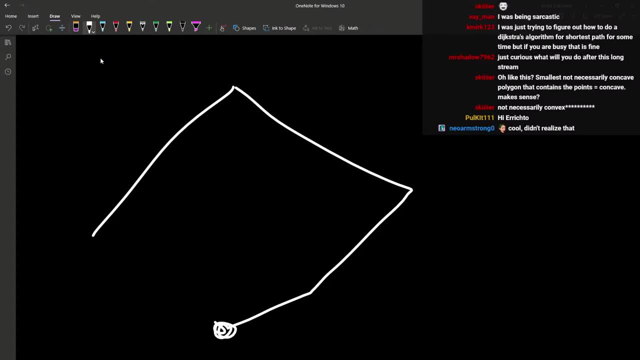 Oh no, it's fine, because the last point is just the rightmost, because it was last in sort. This is for sure the leftmost. this is the rightmost. everything else was here in between. It couldn't be here because it would be convex hull. and then this is a proper last segment. 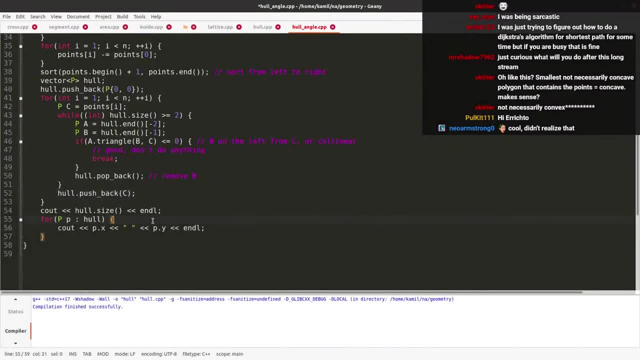 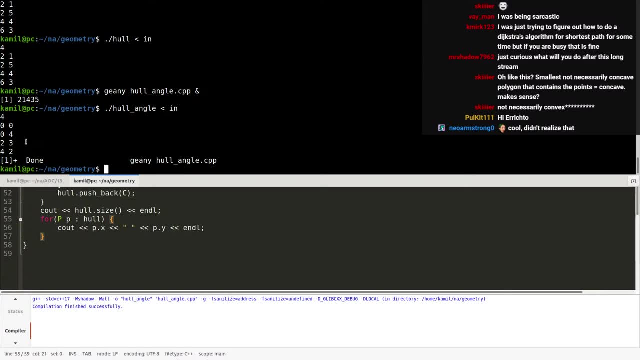 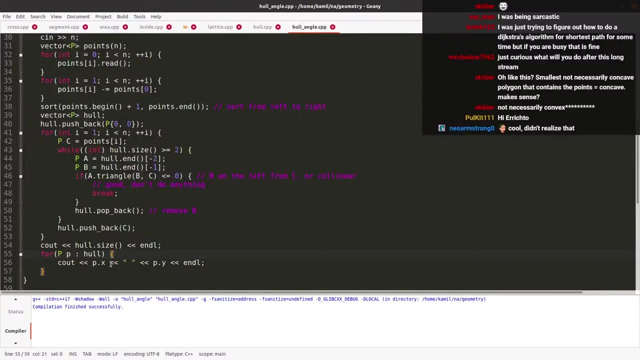 I believe this is everything, and if I print this, what's printed is a bit bad. We have some zeros there because I subtracted. What I should actually do is say px plus this vector by which I subtracted, and this should be the same. Let's sum it. 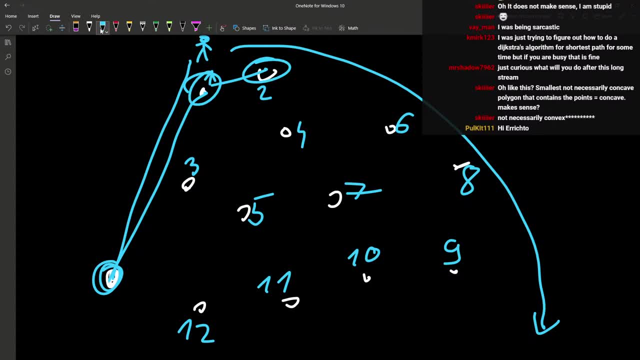 then let's say this point, then this point, and we continue Temporarily. it will be like that this will be popped and we will just have this, and so on. I want partial convex hull to start from here and be maybe with different color. 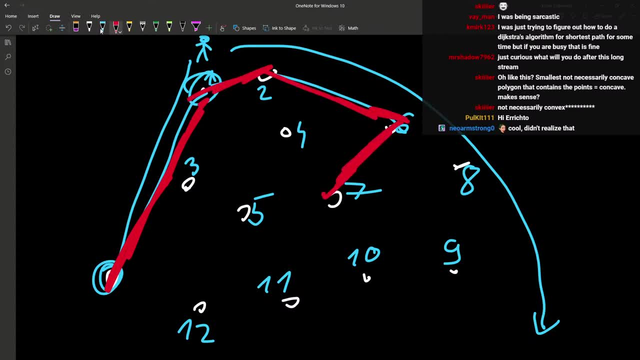 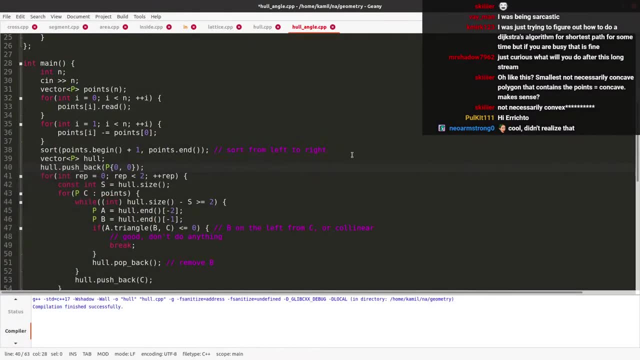 This is partial convex hull we have. Maybe temporarily it's like that, But then 8 will pop 7.. It will be like this: All right, Now for all the points, except for the first one, This new point C. And what do we do with this? 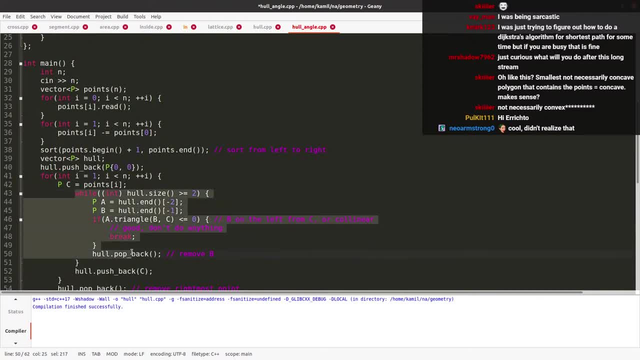 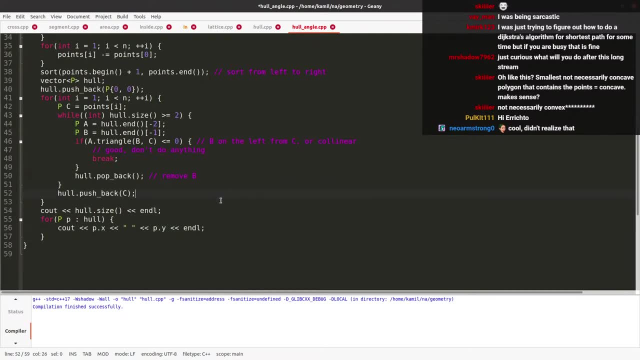 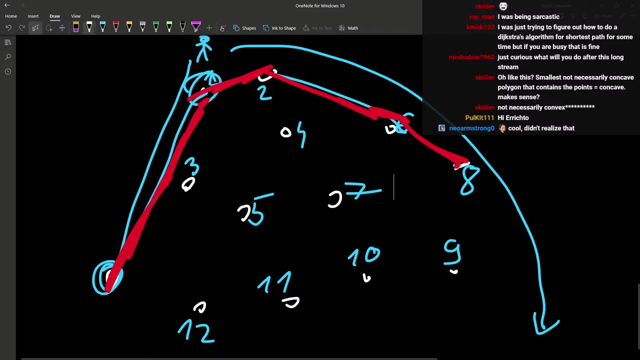 Well, hull size is at least 2.. Consider popping. The logic doesn't change. Then hull pushback C: All right, And this is almost good, Because at the end we might get some garbage. We might have something like this: 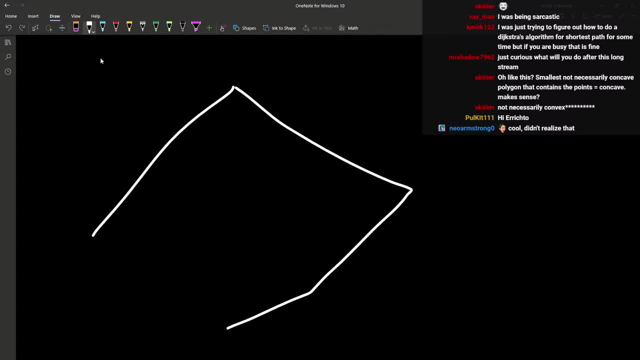 Can we? Oh no, It's fine, Because the last point is just the rightmost, because it was last in sort. This is for sure the leftmost, This is the rightmost. Everything else was here in between Couldn't be here because it would be convex hull. 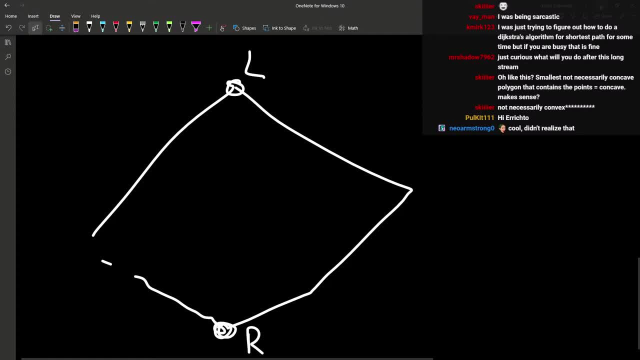 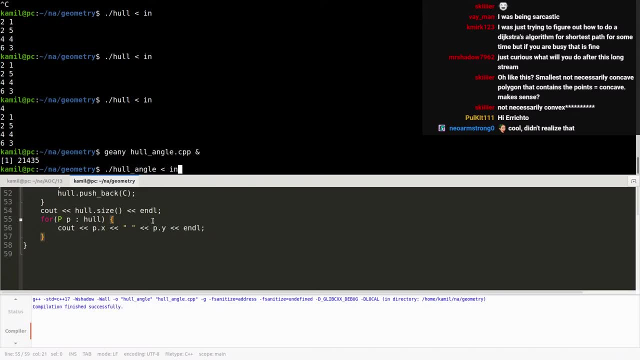 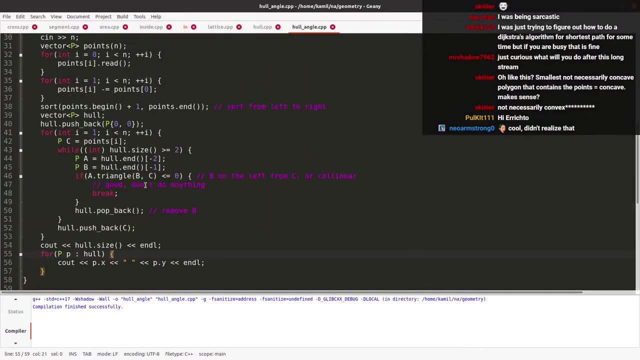 And then this is a proper last segment. I believe this is everything, And if I print this, what's printed is a bit bad. We have some zeros there because I subtracted. What I should actually do is say px plus 0.5.. 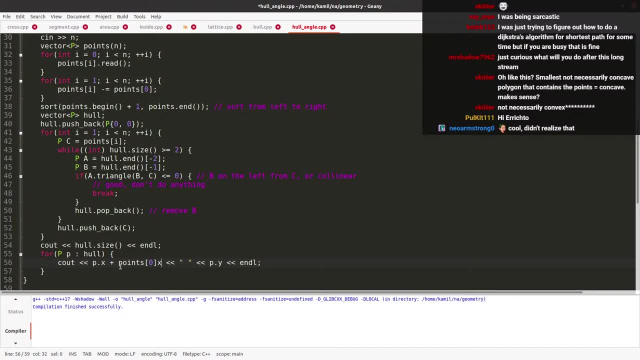 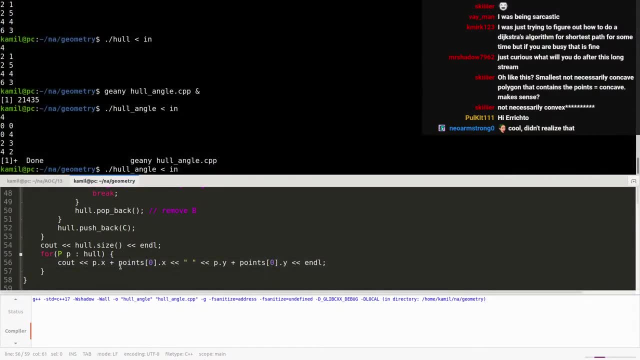 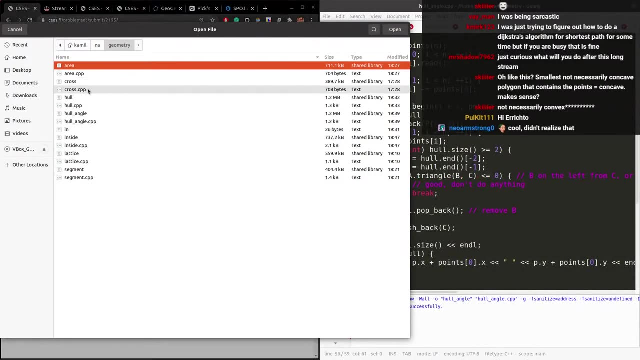 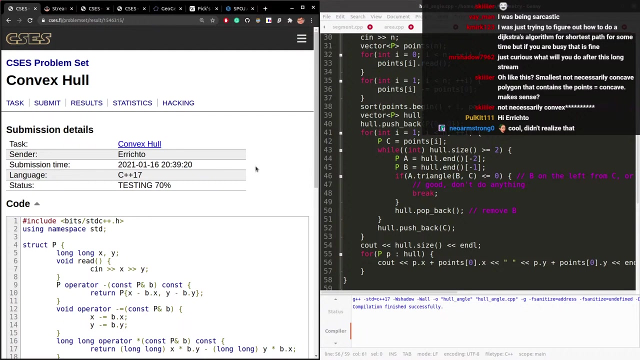 Say px plus this vector by which I subtracted. And this should be the same. Let's submit. I showed you first the version with top and bottom part, because sometimes you need it In some like dynamic programming problems. you need to only find bottom convex hull. 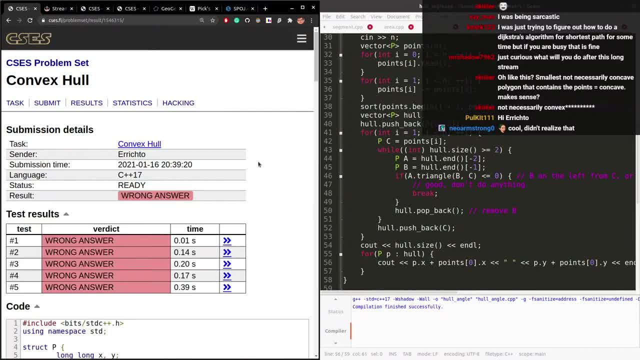 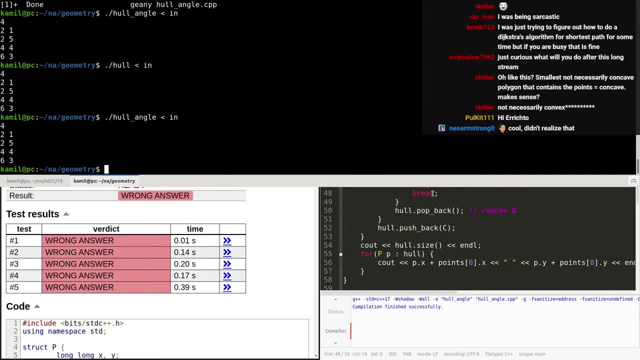 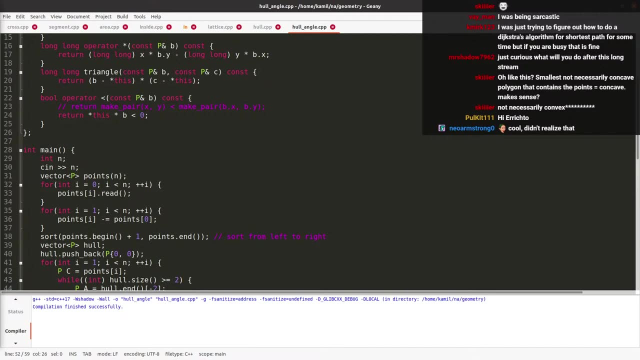 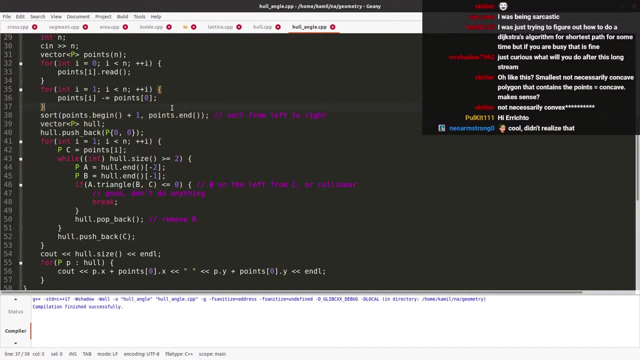 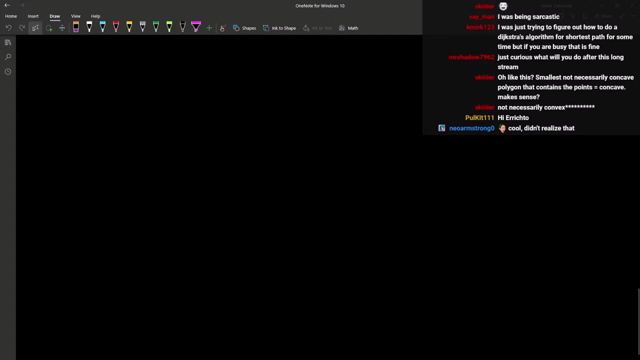 Why is it so slow? Did I make it? And what now? What now? Sort everything other than the first point. This is that point, I think ties I don't resolve correctly. Yeah, I'm quite sure about that, But no, I normally every day I implement the version with bottom and top convex hull. 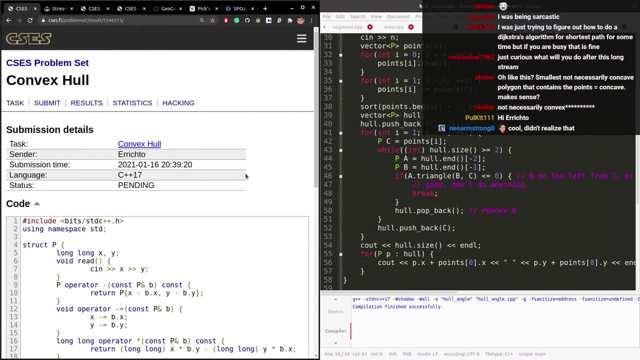 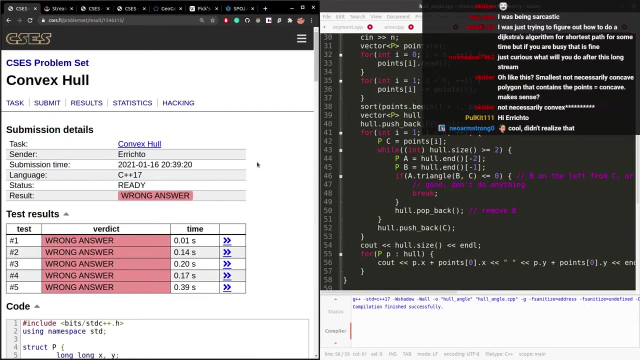 I showed you first the version with top and bottom parts, because sometimes you need it In some like dynamic programming problems. you need to only find bottom convex hull. Why is it so slow Did I make it? And what now? What now? 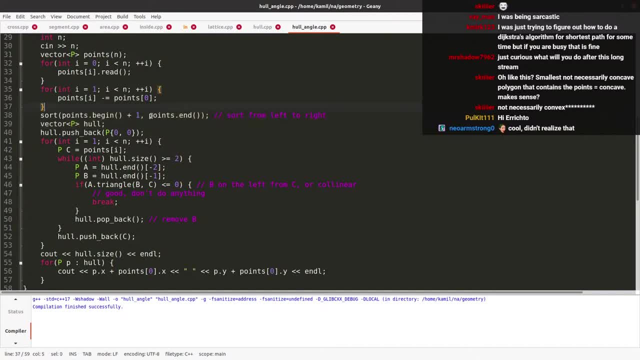 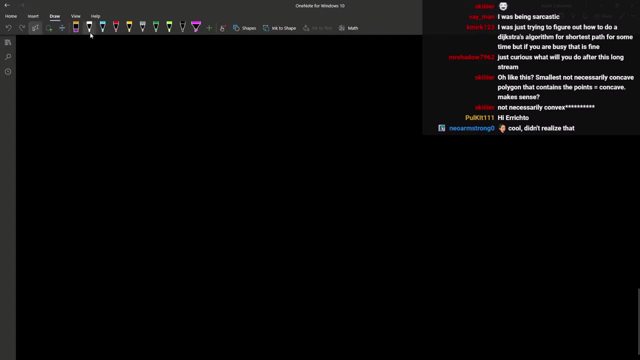 Let's sort everything other than the first point. This is that point. I think ties I don't resolve correctly. Yeah, I'm quite sure about that. But no, Normally every day I implement the version with bottom and top convex hull. It's harder to decide about ties here. I didn't tell you. 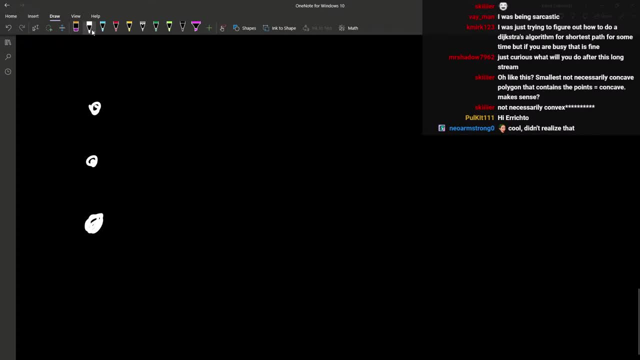 what exactly happens for multiple leftmost points in the first version. but we take the bottom most of them and it works. The convex hull will be like this, But for angles, if points can be collinear, you need to take them in this order: 1,, 2,, 3,. 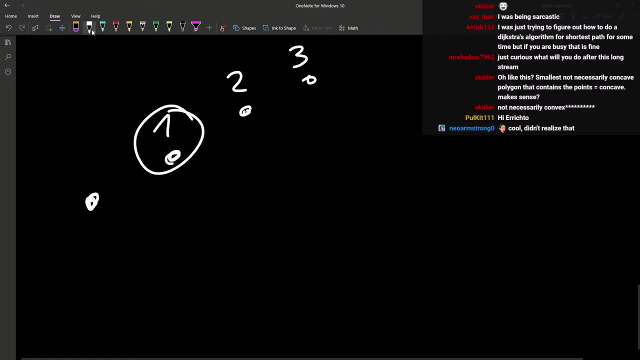 so, starting from the one closest to 0,, 0,, then here it doesn't matter, but at the very end you need to do the opposite order. Let's say this is number 12, then 13 and 14.. And now it becomes annoying. 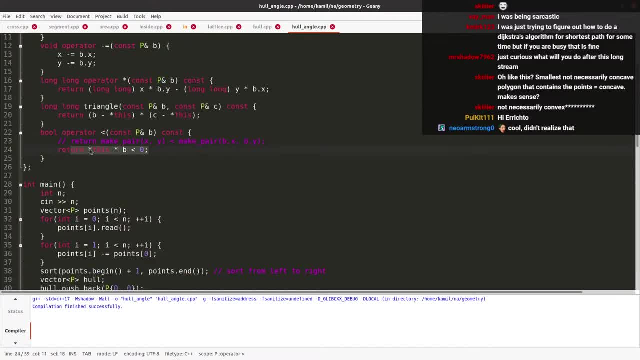 Right. So in this operator, if I do this, if they are collinear, return the fact that I'm closer. I am closer to 0, 0.. And now for closer, I will create something that in math is called a norm. 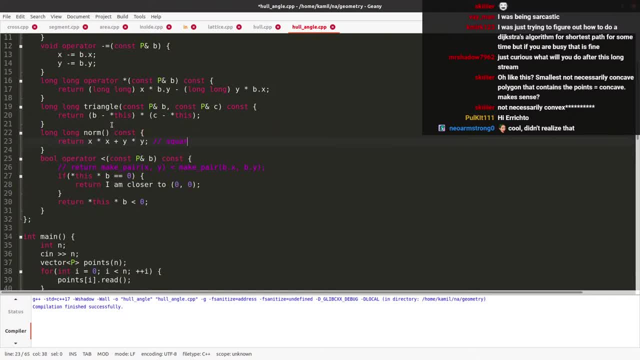 This is square of distance from 0, 0.. I don't want to go into detail because it will take too much time. Return norm smaller than bnorm. So for ties collinearity with 0, 0, I take closer one first. 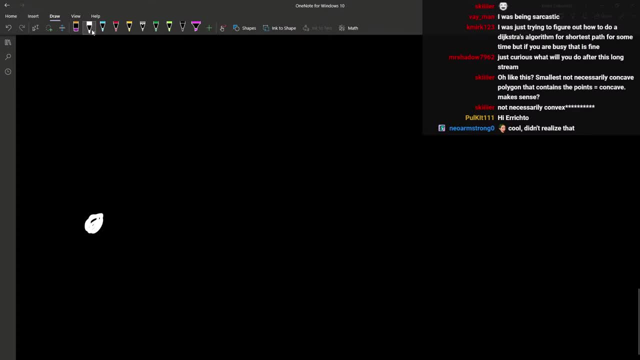 It's harder to decide about ties here. I didn't tell you what exactly happens for multiple leftmost points in the first version, but we take the bottom most of them and it works. The convex hull will be like this, But for angles, if points can be collinear, you need to take them in this order: 1 to 3.. 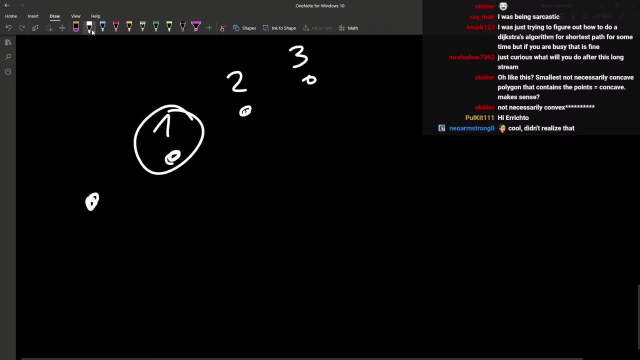 So, starting from the one closest to 0,, 0. Then here it doesn't matter, but at the very end you need to do the opposite order. Let's say, this is number 12, then 13 and 14. And now it becomes anonymous. 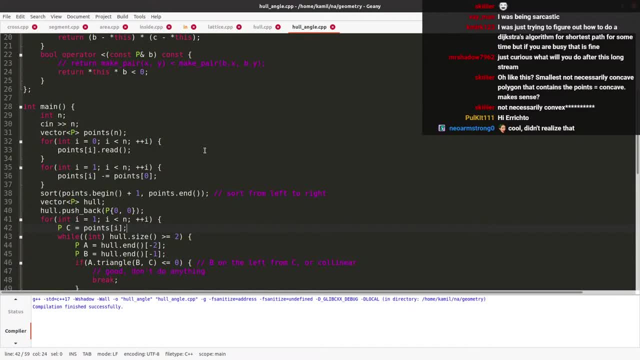 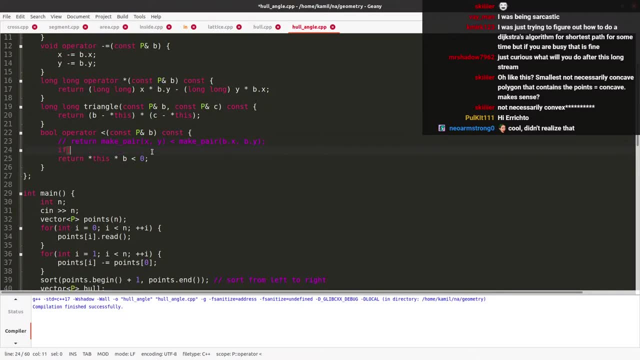 And so it's not going Right. So in this operator, if I do this, If they are collinear, Return the fact that I'm closer. I am closer to 0, 0.. And now for closer, I will create something that in math is called a norm. 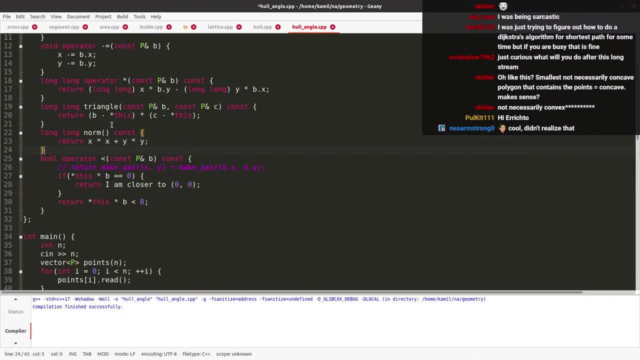 this is square of distance from 0, 0.. I don't want to go into detail because it will take too much time. Return norm smaller than bnorm. So for ties collinearity with 0, 0, I take closer one first, but I need to handle this thing. 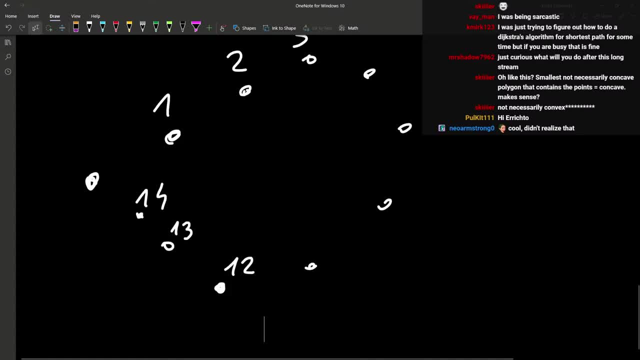 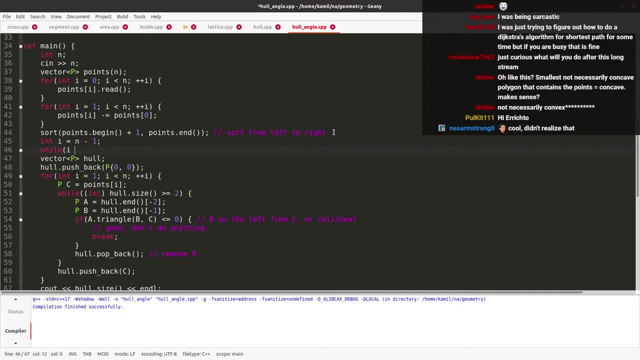 The points at the end. I need to do them in reverse order. Sure, I can deal with that in some way. Well, this and points of i minus one times points of i is zero. I need to find what suffix contains, what suffix of sorted points is. 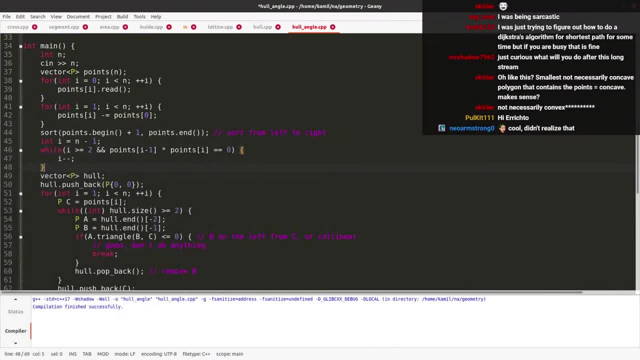 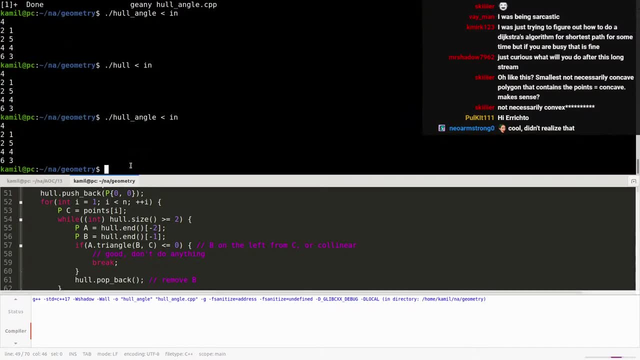 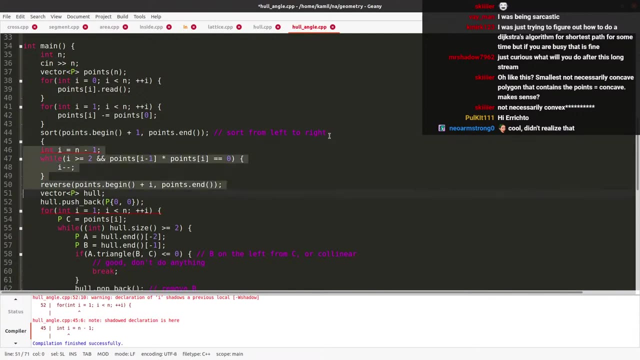 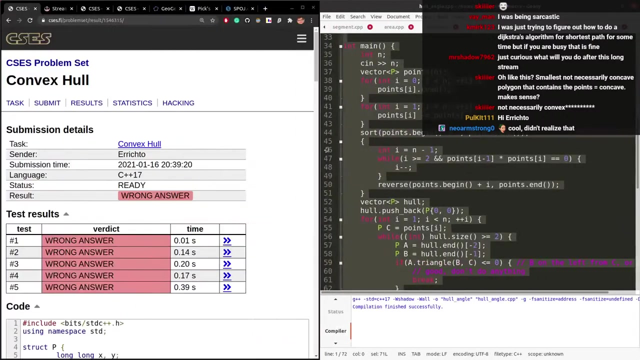 like this collinear with the last point and then reverse it. but you know, this is geometry. I I don't know if this works, just some hotfix they came up with. now I don't even have a test where it's it's needed, but let's submit and then create a test. 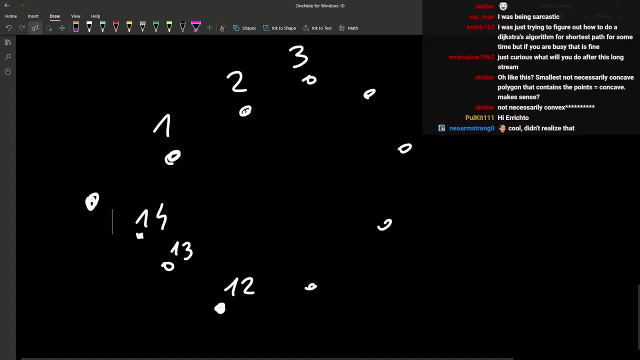 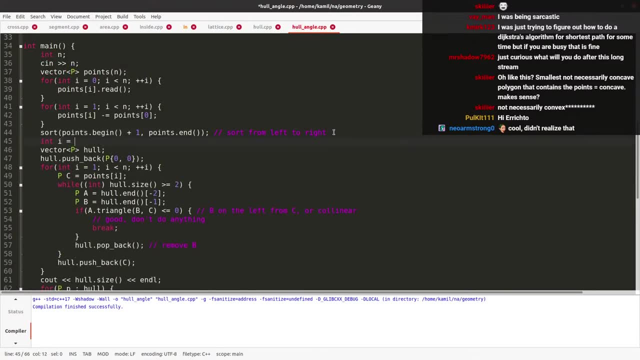 But I need to handle this thing. the points at the end, I need to do them in reverse order And sure I can deal with that in some way. Well, this and points of i-1 times points of i-0, I need to find. 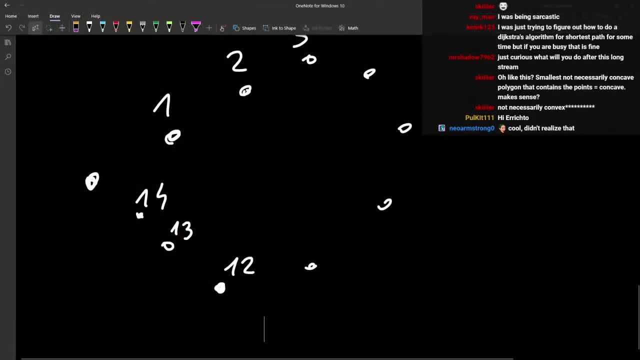 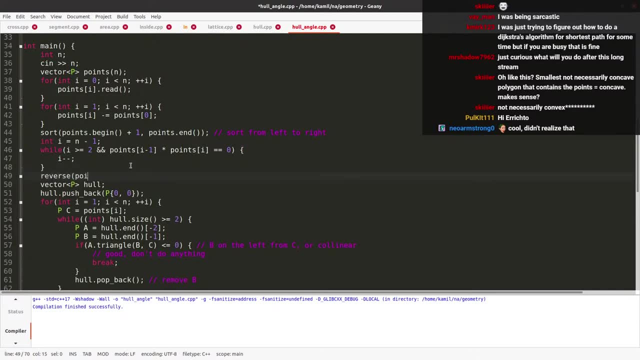 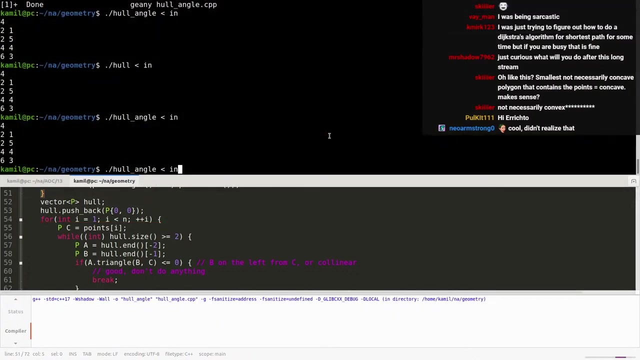 what suffix contains. what suffix of sorted points is like this collinear with the last dot point and then reverse it. but you know, this is geometry. I I don't know if this works, just some hotfix they came up with. now I don't even have a test where it's. 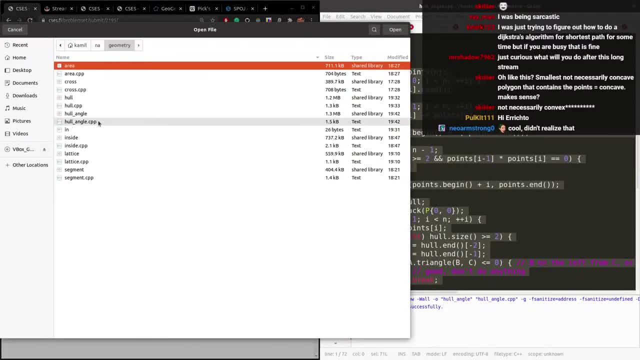 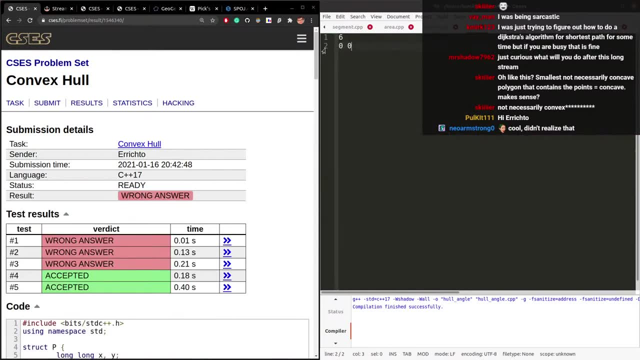 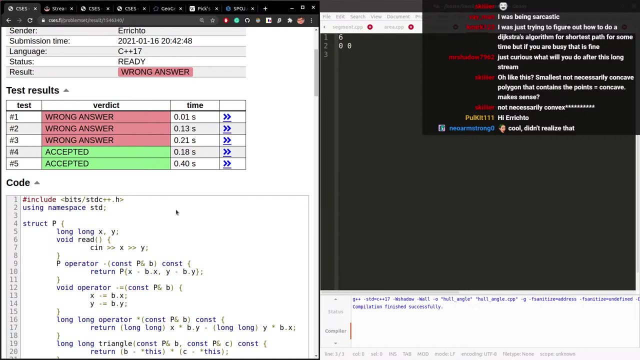 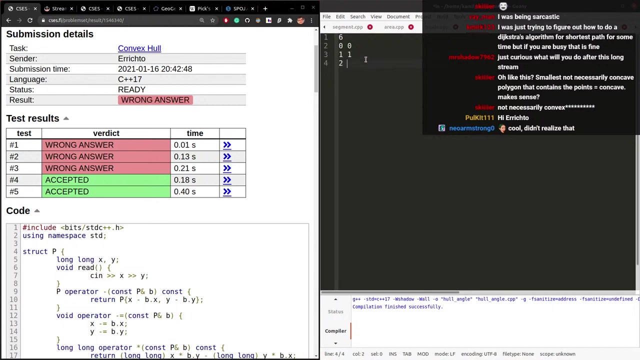 it's needed, but let's submit and then create a test starting from 0: 0. it's a little bit better. what's wrong? okay, if we have 0, 0, then 1, 1, 2, 2, 3, 3, then something more to the bottom: 0. 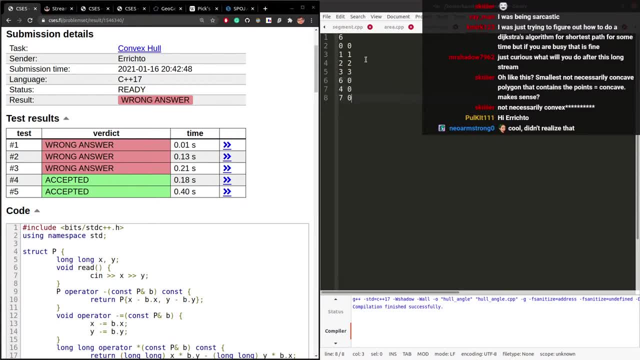 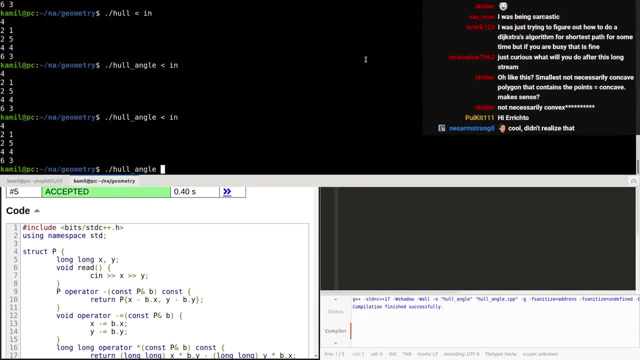 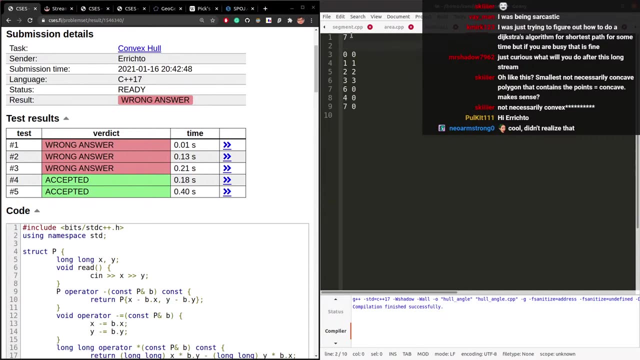 6, 0, 4, 0, 7, 0. will this sort it correctly? yes, it is sorted correctly, and something in the middle should be excluded. it is not excluded, so what's wrong? 3, 3, 3, 3 should be. 3, 3 should be. 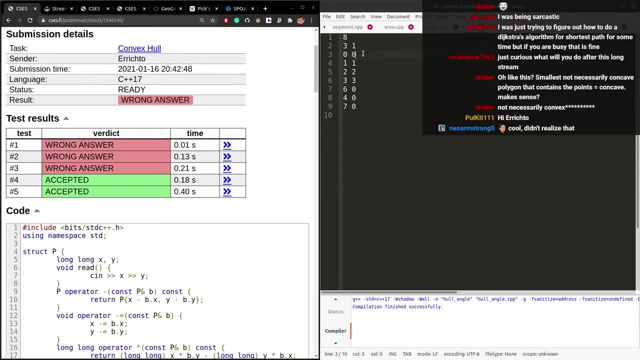 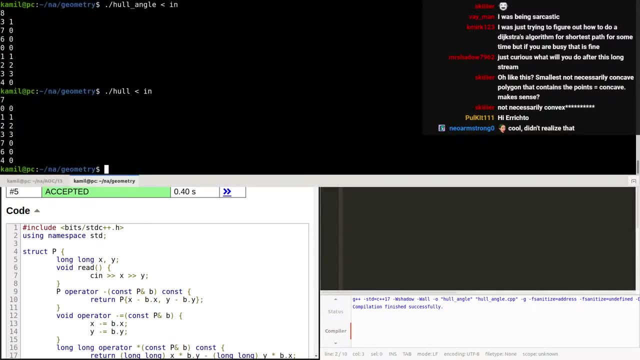 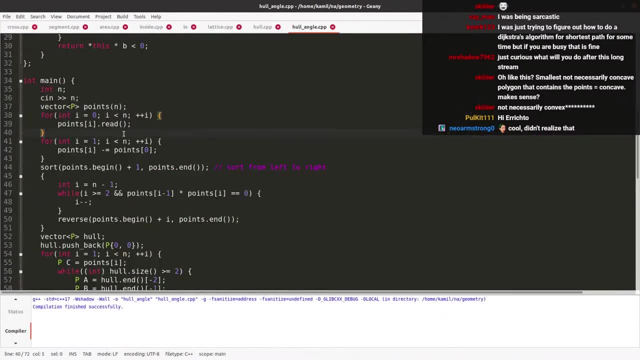 be. yeah, I'm quite sure that this should be excluded. we got a test worried my code doesn't work. doesn't work because who gives different number of points. why is this? I think I know why: because I want the first point to be point zero. I want this to be the leftmost one, right if you are more on. 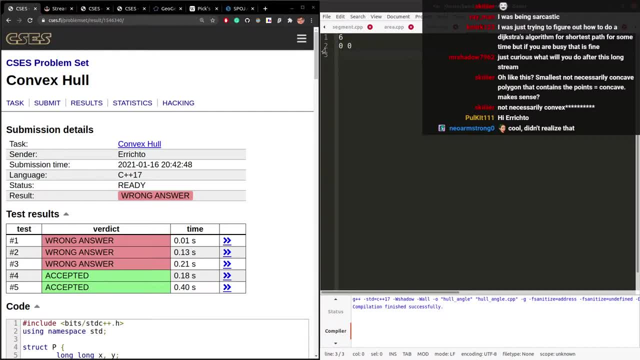 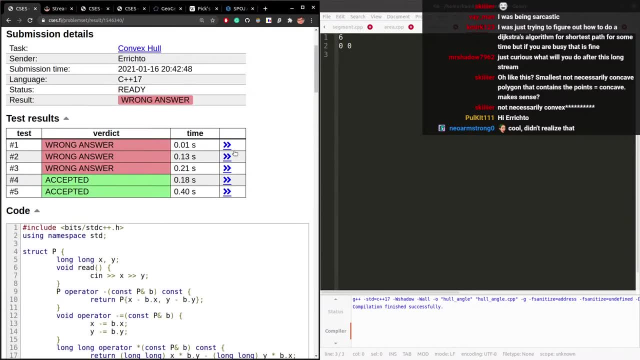 starting from 0, 0, it's a little bit better. what's wrong? okay, this is: if we have 0, 0, then 1, 1, 2, 2, 3, 3, then something more to the bottom: 0, 6, 0, 0, 6, 0. then 1, 1, 2, 2, 3, 3, then something more to the bottom: 0, 6, 0. 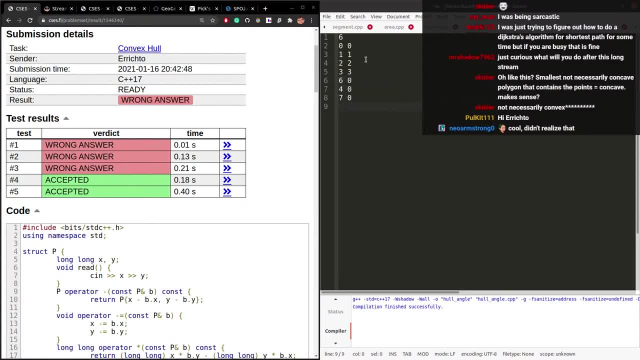 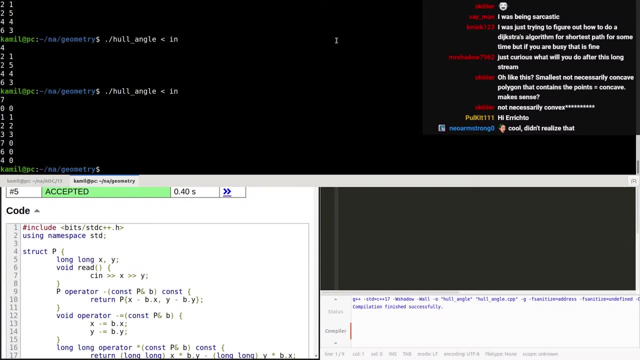 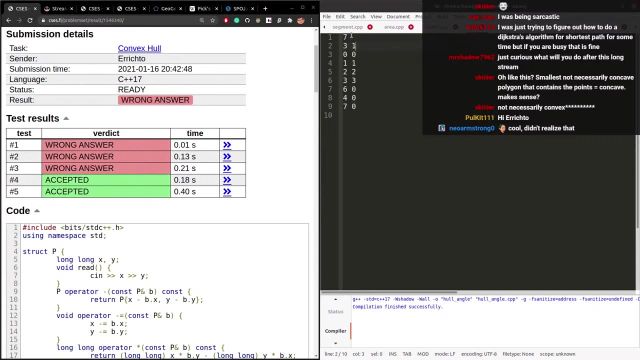 or 0: 0. will this sorted correct? yes, it is sorted correctly, and something in the middle should be excluded. it is not exclude, so what's wrong? 3- 3 should be. yeah, I'm quite sure that this should be exclude. we got a test. worried my code. 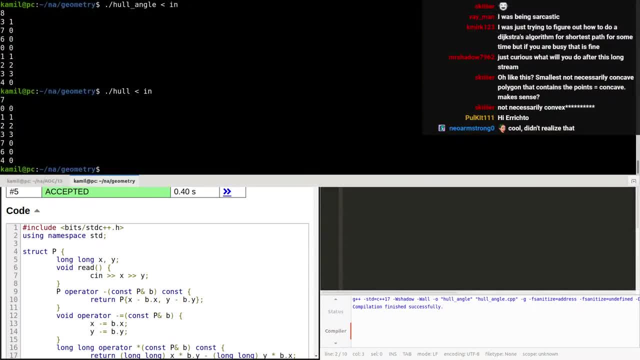 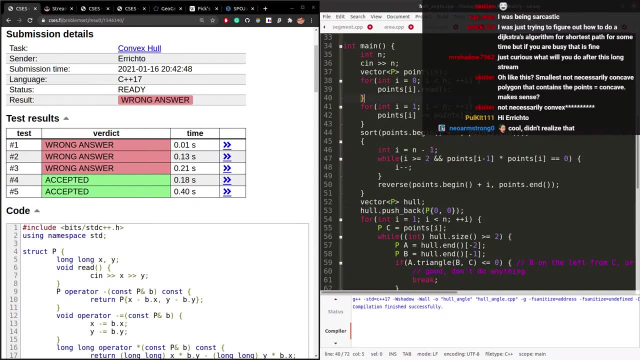 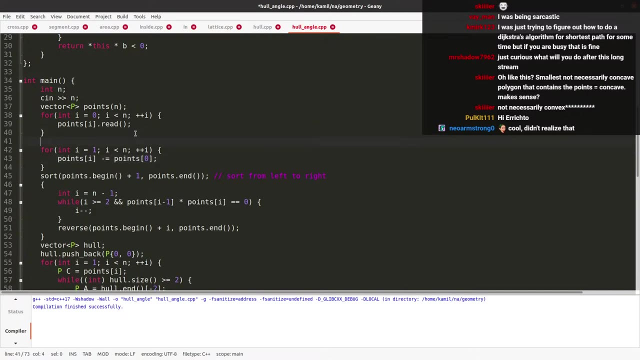 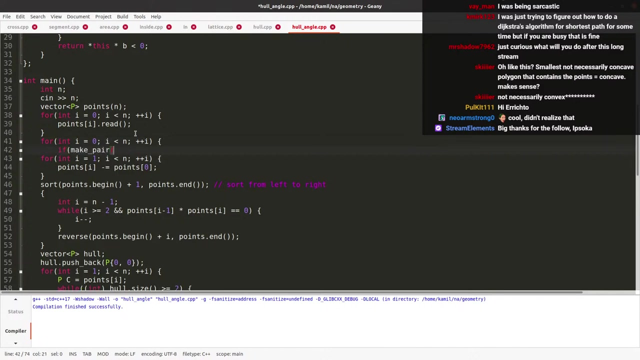 doesn't wrong. doesn't work because hole gives different number of points. why is this? I think I know why: because I want the first point to be point 0. I want this to be the leftmost one right. if you are more on the left screen, use the bomb. 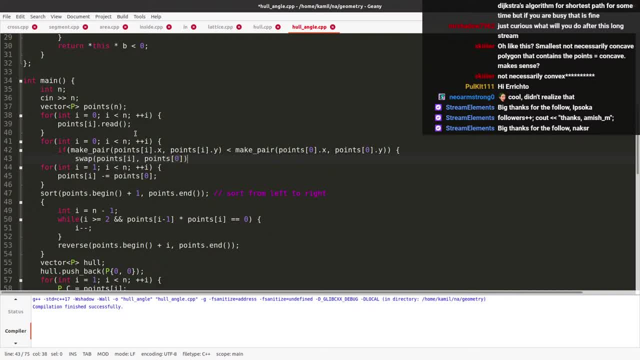 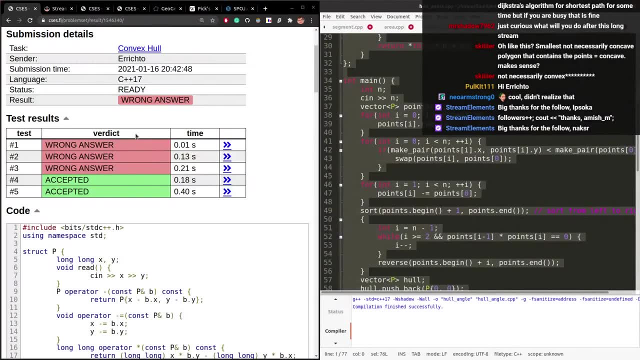 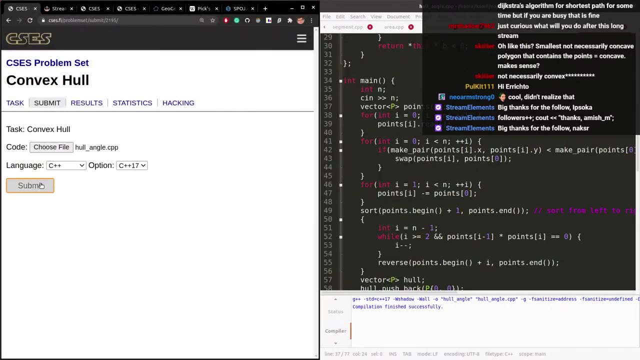 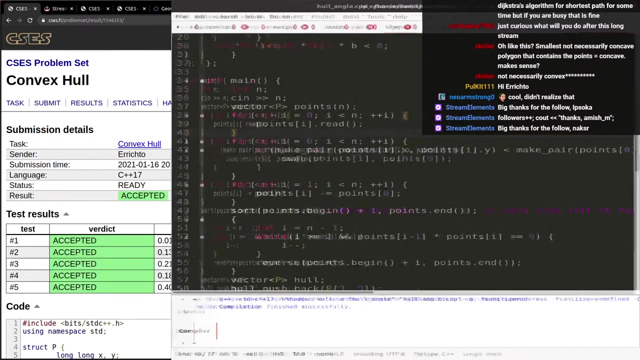 then the current points 0, then swap with point 0 and now it works. I keep copy paste. Nike keep copying the code, because this is how I submit in code forces: Hull angle submit. give me accepted, we're done, Right. yeah, this angle version is harder to do. 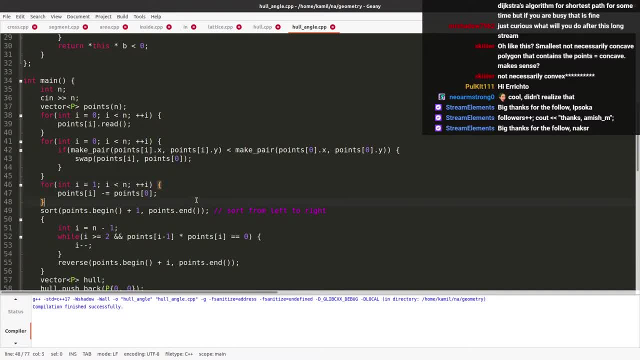 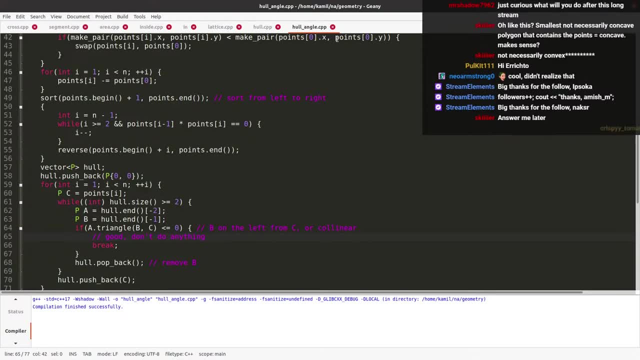 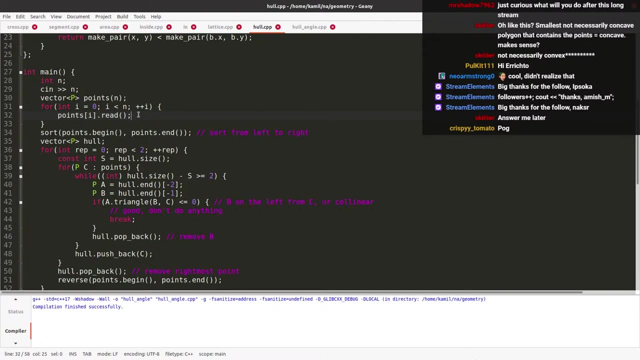 if there can be collinear points. If no collinear points, then angles are easier. but sometimes in, for example, dynamic programming, you need this top and bottom. I recommend you to learn this top and bottom: convex hull, Don't sort by angle. 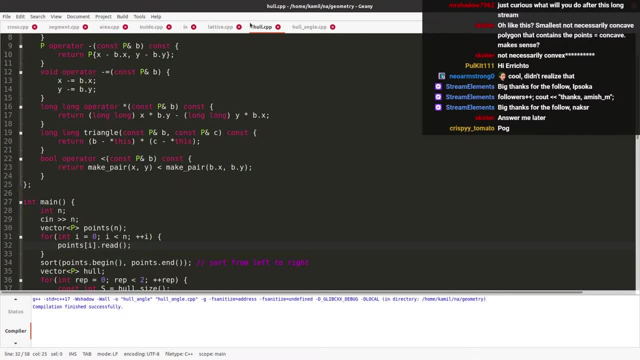 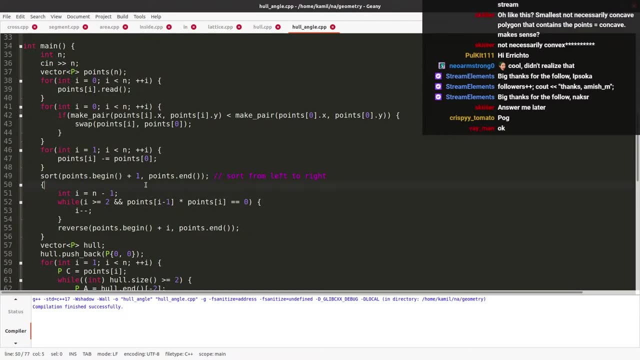 So in my github repository I recommend you to learn hullcpp, not hull angle, But for example, sorting by angle is useful. You need to know how to do it And, yeah, it's not really the best code for that. 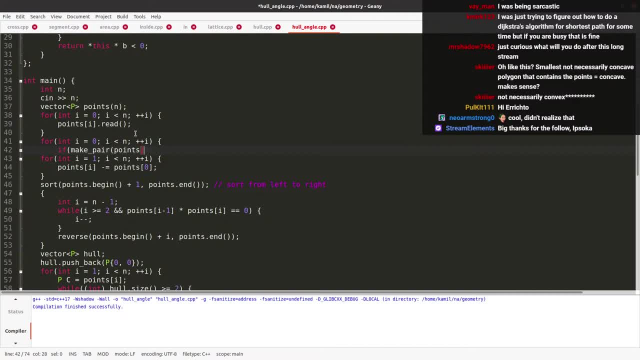 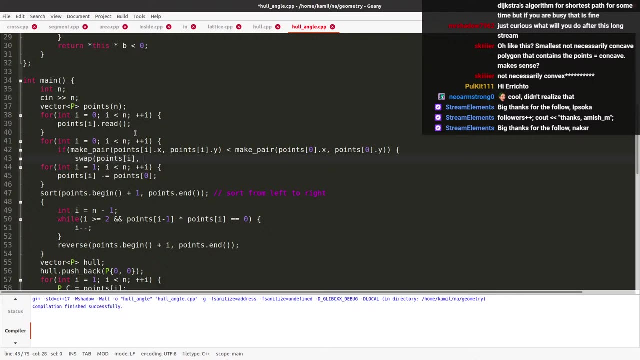 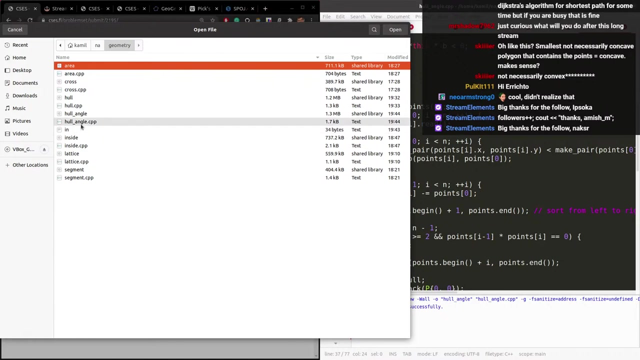 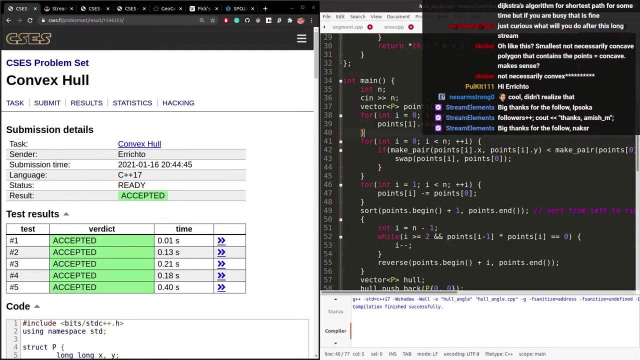 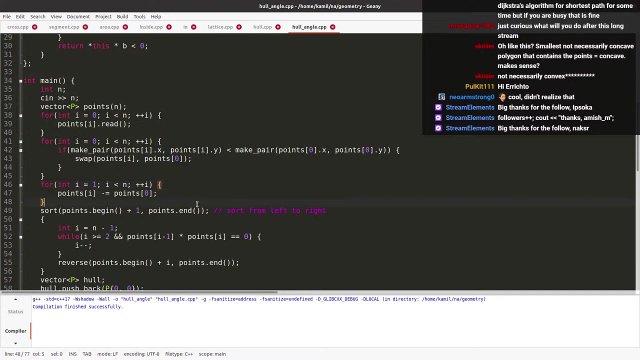 the left, then the current point zero, then swap with point zero and now it works. I keep copy paste. I keep keep copying the full code, because this is how I said it: submit in code. forces who angle submit. give me: accepted. we're done right. yeah, this angle version is harder to do if there can be collinear points, if no, 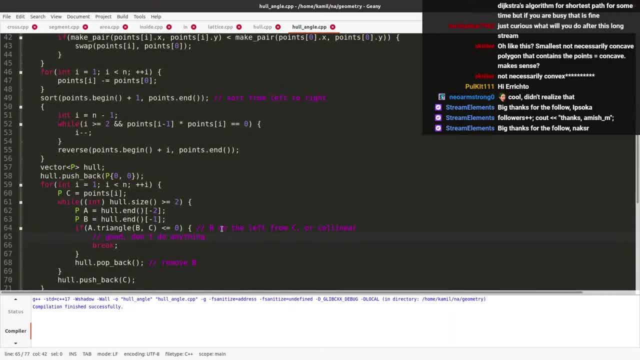 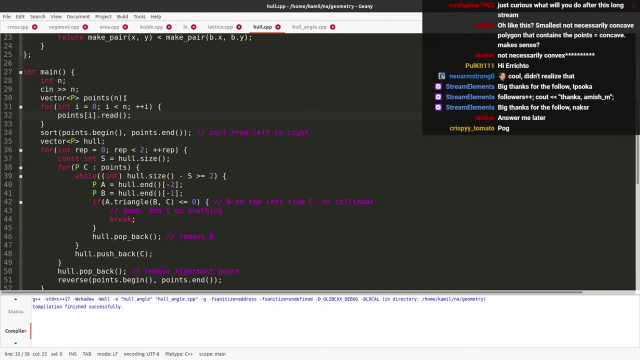 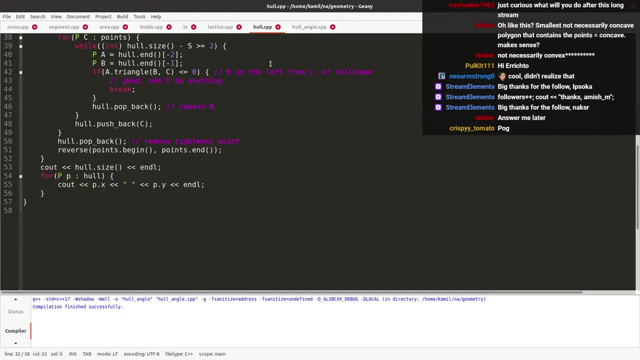 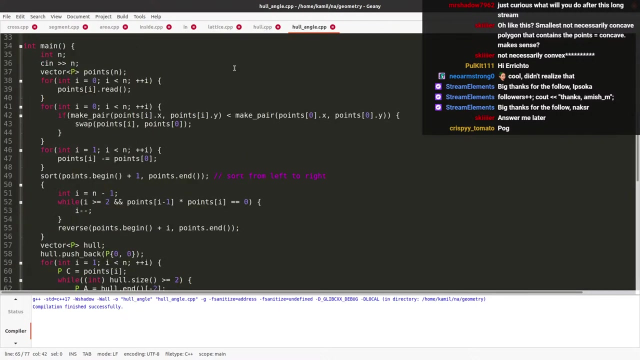 collinear points, then angles are easier. but sometimes in, for example, dynamic programming you need this top and bottom. I recommend you to learn this top and bottom. convex-whole don't sort by angle, so in my github repository I recommend you to learn whole and plural. 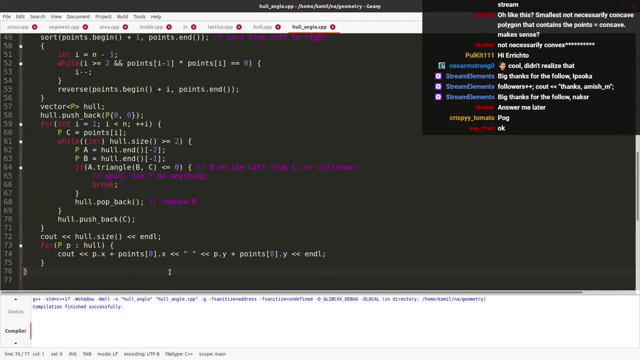 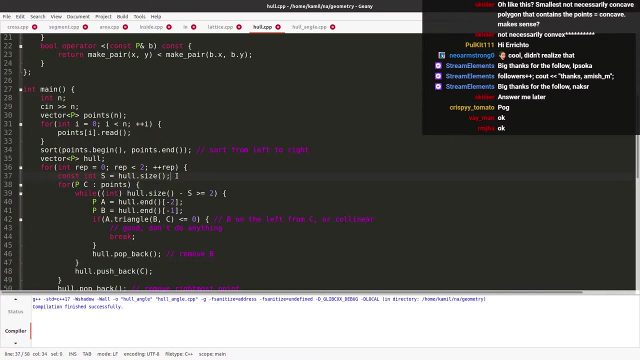 by angle is useful, you need to know how to do it, and it's not really the best code for that. I was just hotfixing something. I don't like how I sort it. don't copy this. don't use exactly that. this is nice, though, other than this, hack, Figure out, understand what happened and figure. 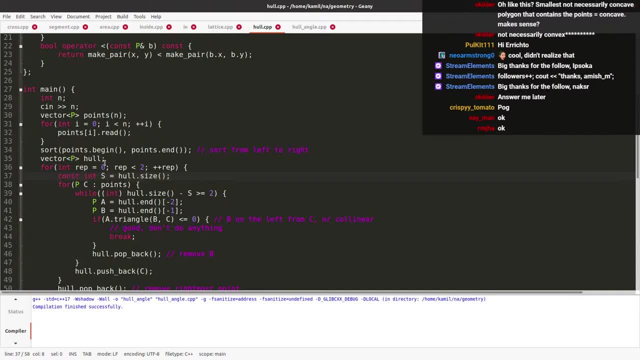 out your own version without my hack with size, Maybe just create two vectors and then at the end combine them. When you learn anything, including, like here, geometry in convex hull, it's best if now you try to reconstruct it. Go through CSCS problems, starting with the one where you check if point is on the 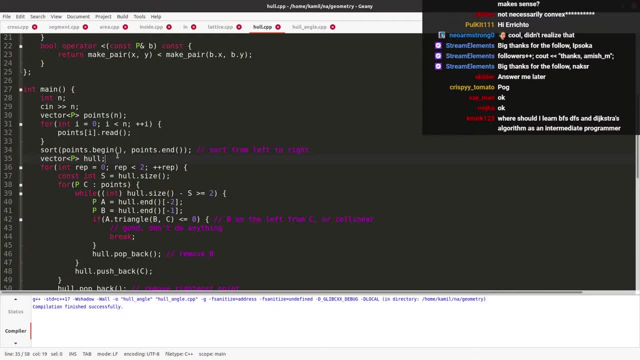 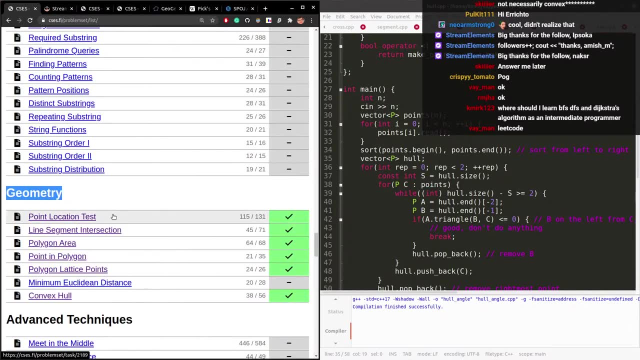 left and on the right. Maybe skip the problem about intersection of segments. It was too tricky. You should do point location test polygon area for sure. point in polygon, especially the second version. This lattice points is stupid And convex hull. Maybe in this order do those four problems. 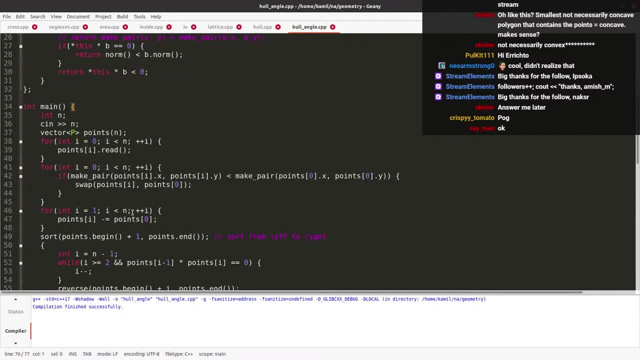 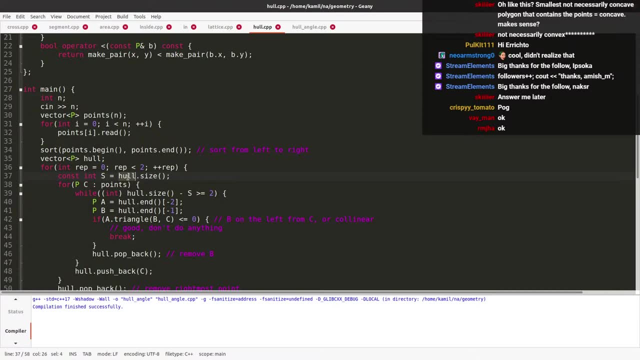 I was just hotfixing something. I don't like how I sort it. Don't copy this, don't use exactly that. This is nice, though, other than this hack, Figure out, understand what happened and figure out your own version without my hack, with size. 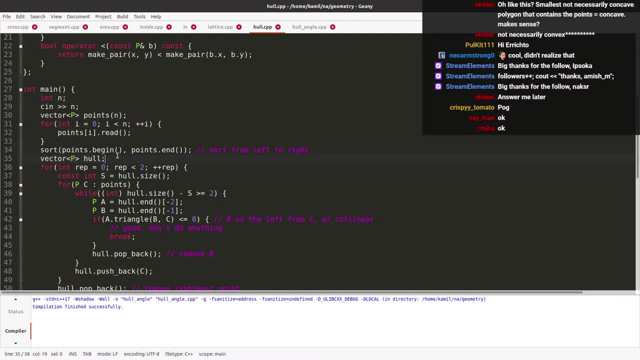 Maybe just create two vectors and then at the end combine them. You know, when you learn anything- including, like here, geometry and convex hull, it's best if now you try to reconstruct it, Go through CSCS problems, starting with the one where you check if point is on the left and on the right. 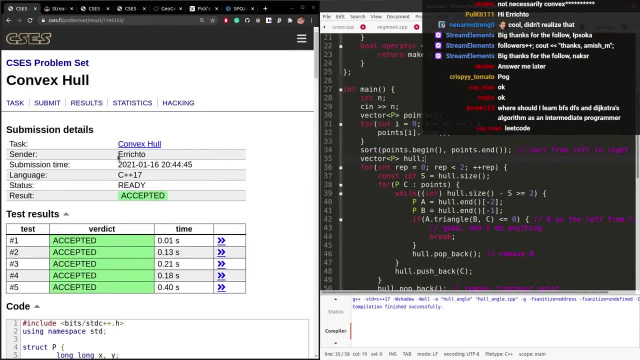 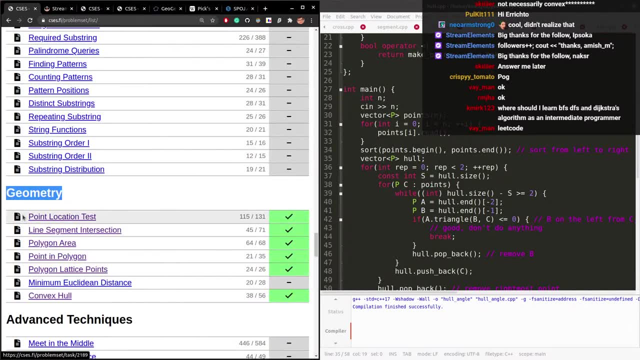 Maybe skip the problem about intersection of segments. It was too tricky. You should do point location test polygon area for sure. point in polygon: yeah, especially the second version. This lattice points is stupid And convex hull. maybe in this order, do those four problems. 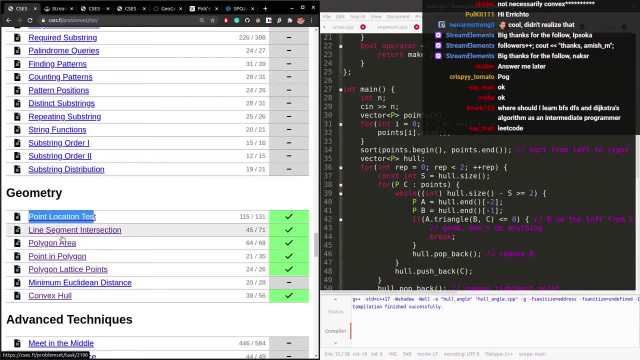 Again, point location: test first polygon area. point in polygon and convex hull And try first not to look at my chart. reconstruct them. do it slightly differently. If you can reconstruct something without looking at my code, then it means you understood it. 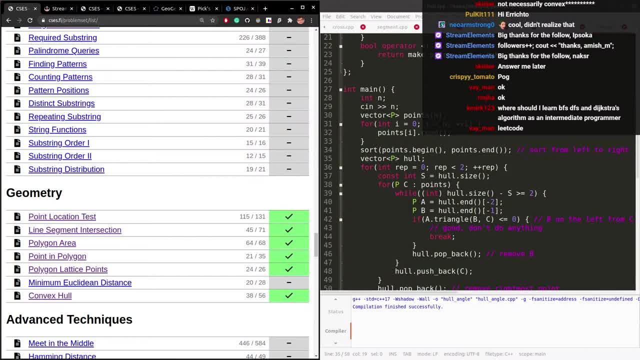 Geometry is ugly and it's especially hard to debug. I was lucky here to only spend in total a few minutes on any kind of debugging. Even though I'm experienced, I still make mistakes in geometry, and then for me still they are hard to debug. 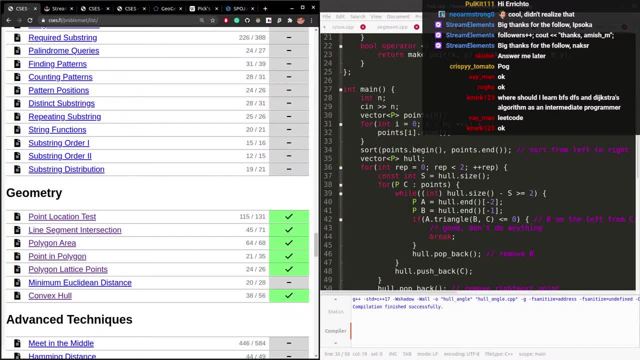 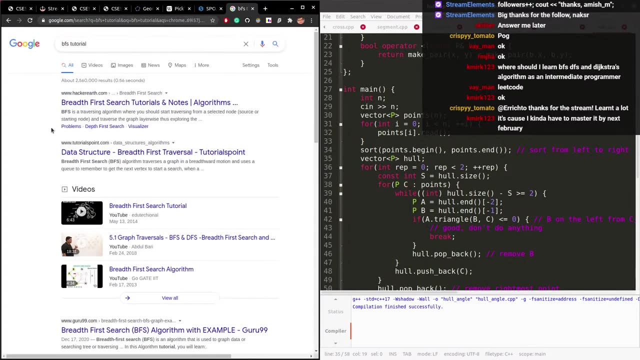 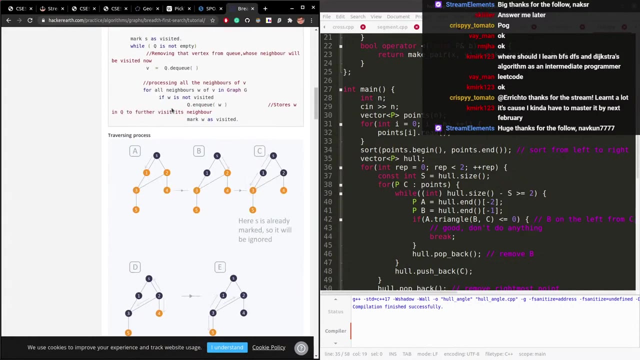 Right, thank you all for watching. Where should I learn BFS DFS? Maybe not leetcode, but I would say in Google BFS tutorial. There are a few possibilities. Hacker actually has fine tutorials. If you prefer videos, search for searching youtube. 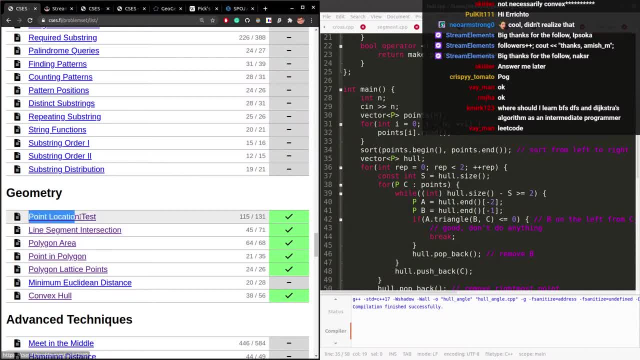 Again: point location test, polygon area. point in polygon and convex hull And try first to find the point location test And try first not to look at my codes, Reconstruct them. do it slightly differently If you can reconstruct something without looking at my codes. 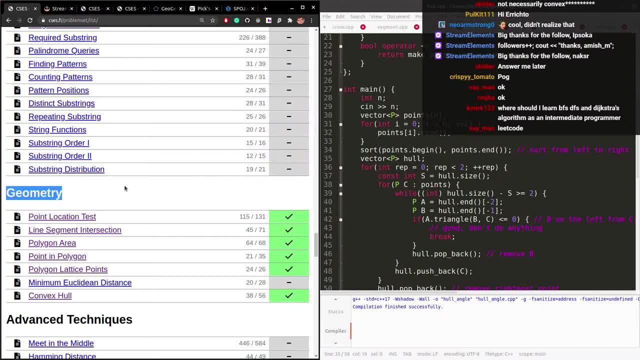 then it means you understood it. Geometry is ugly and it's especially hard to debug. I was lucky here to only spend in total a few minutes on any kind of debugging. Even though I'm experienced, I still make mistakes in geometry, and then for me still they are hard to debug. 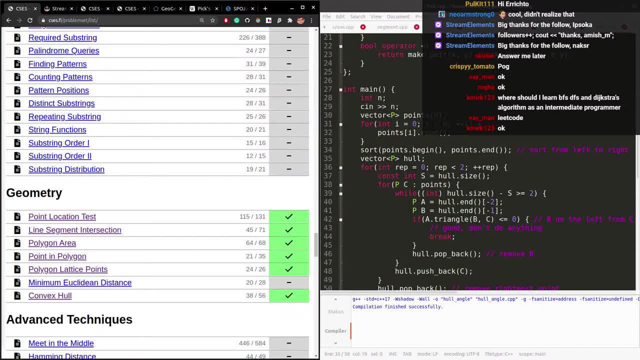 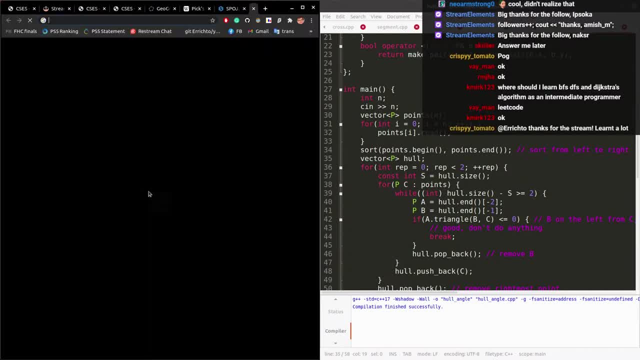 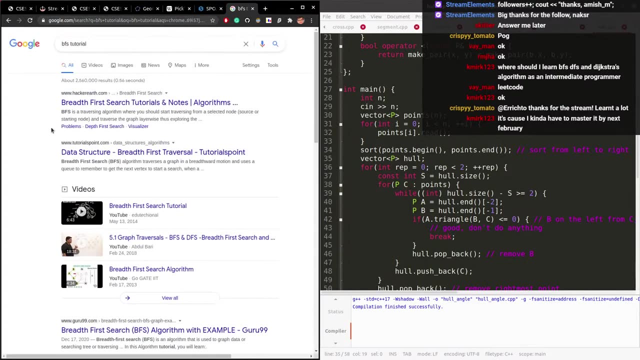 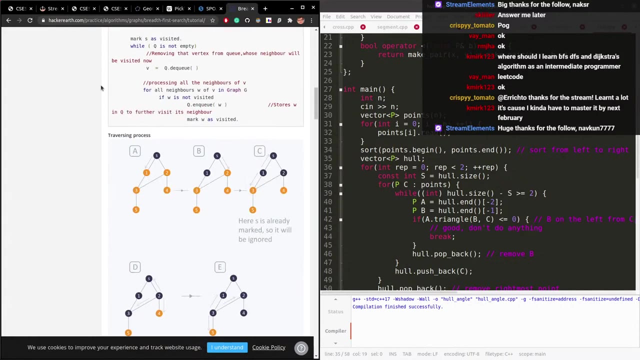 Right. Thank you all for watching. Where should I learn BFS DFS? Maybe not leetcode, but I would say in Google BFS tutorial. There are a few possibilities. Hacker actually has fine tutorials. If you prefer videos, search in YouTube. Leetcode is fine. 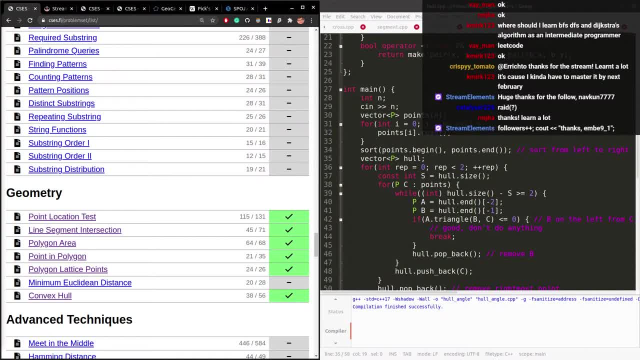 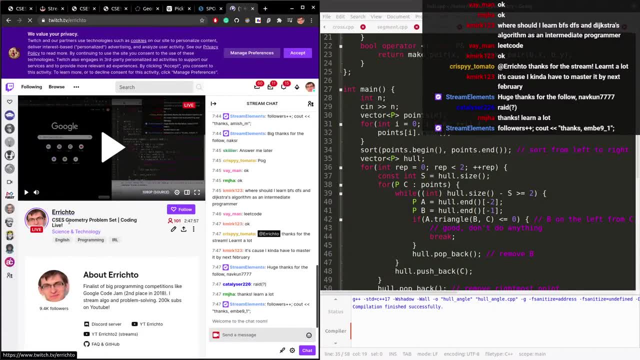 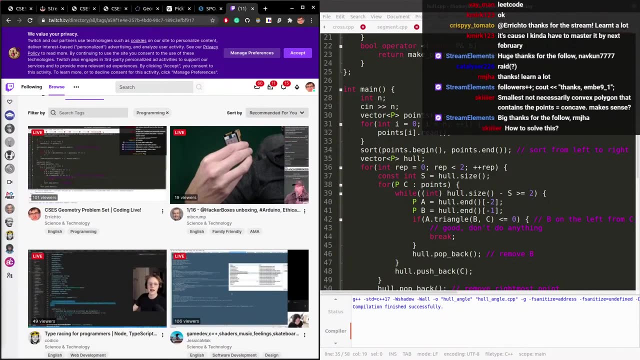 Not for competitive programming. We can do RAID if somebody is doing competitive programming, but otherwise not really. I don't want to tell you to watch something completely else. Follow me on Twitch, YouTube, Discord, all the stuff. I don't know if I will do the last problem in a stream or maybe make a 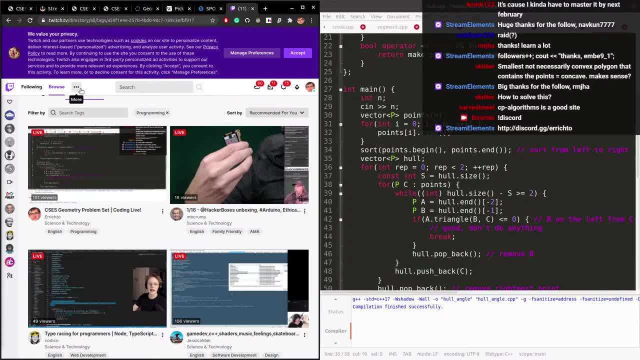 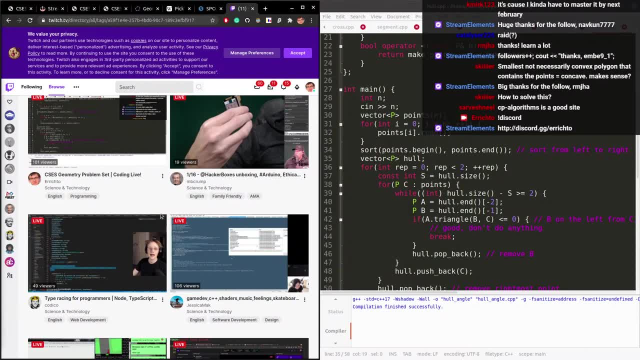 video on it. The problem I didn't solve is a hard geometry problem, but we are here almost at three hours, So see you in the next video. Bye, If you're watching this later, I hope you watch it in two parts. Type racing for. 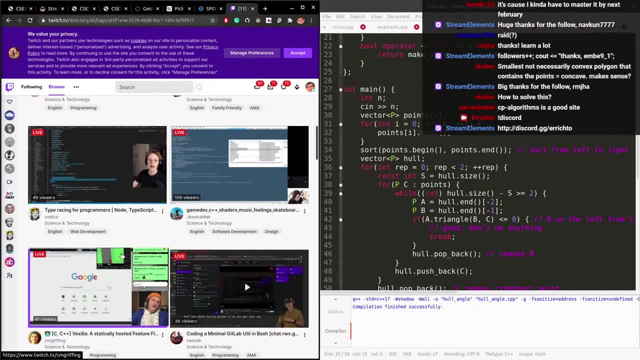 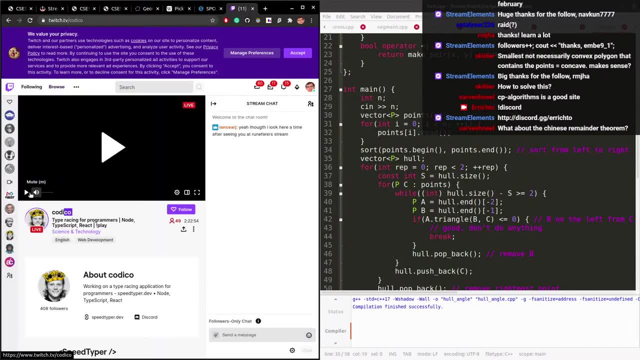 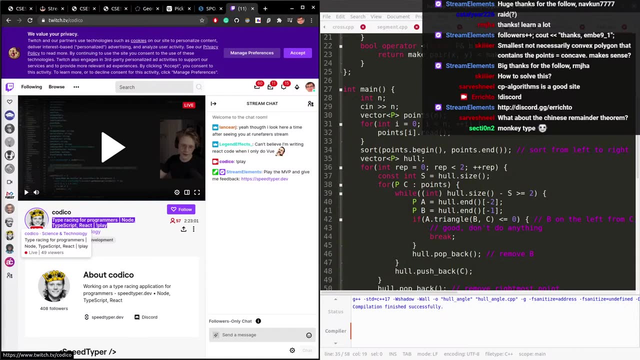 programmers. That sounds interesting but not really related. We're doing the RAID Codico. CpAlgorithm is a good site, but not for beginners. CpAlgorithm, I would say, is for hardcore, competitive programmers. What about Chinese remainder term? Remainder term- Yeah, I'm bad at doing. 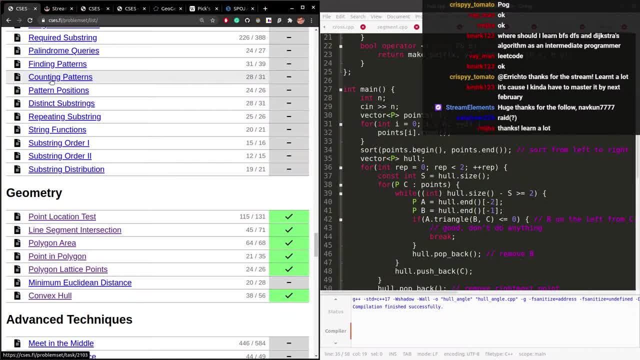 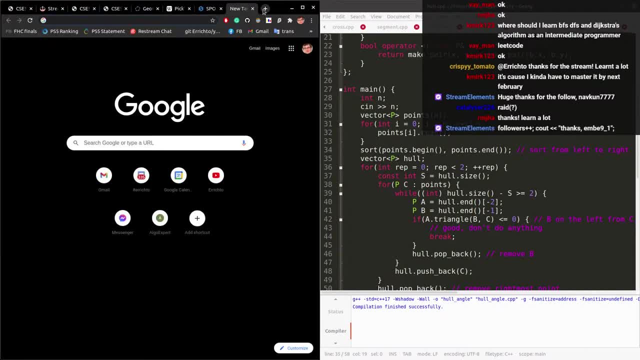 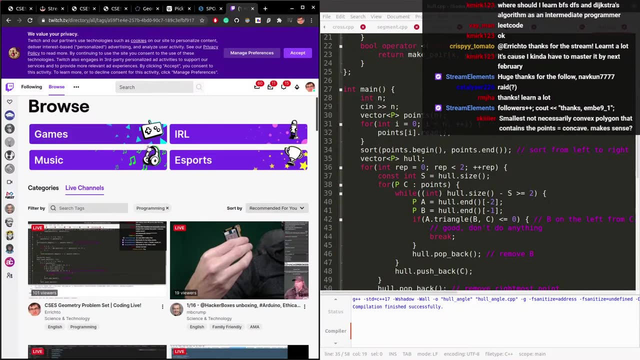 Like. leetcode is fine, Not for competitive programming. We can do RAID if somebody is doing competitive programming, but otherwise not really. I don't want to tell you to watch something completely else. Follow me on Twitch, YouTube, Discord, all the stuff. 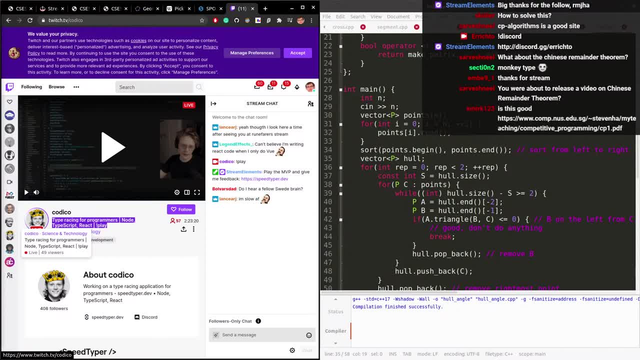 stuff. It will be Codico. I used RAID Right. Again, thank you all for watching. See you next time, Bye, bye.